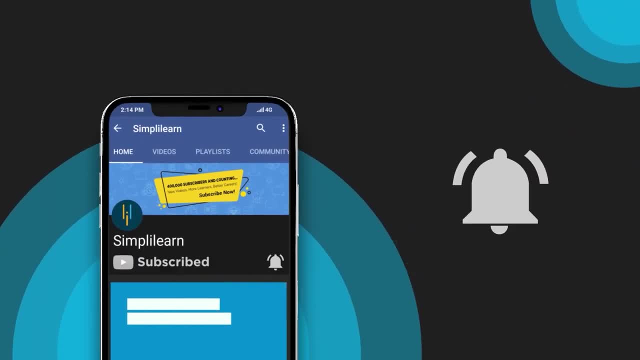 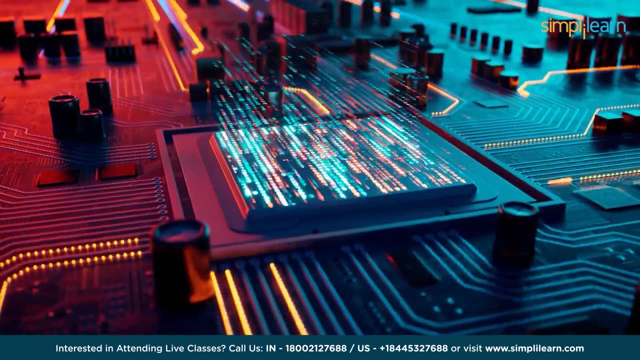 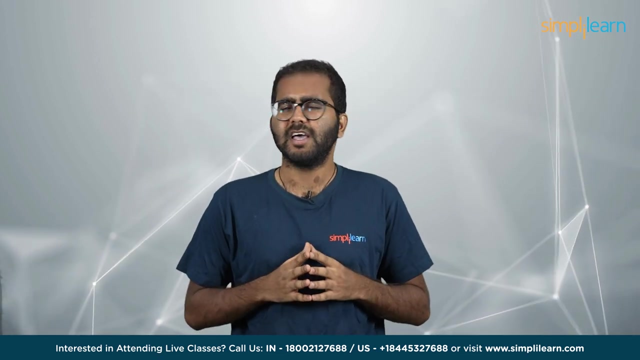 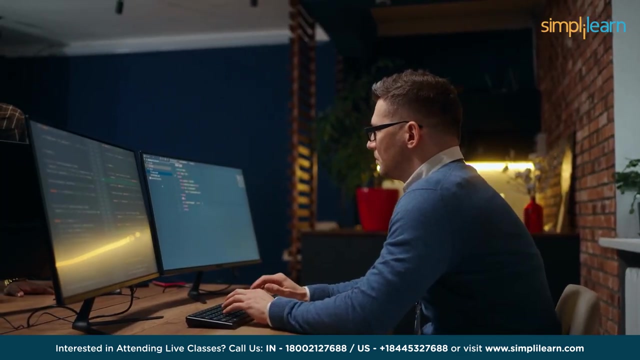 Welcome to the world of data science, where extraordinary becomes possible and unimaginable becomes real. In this captivating journey, we delve into the foundations of data science, exploring its boundless potential and unraveling the secrets behind its immense power. Whether you are a curious beginner or a seasoned professional, this data science basics course video will 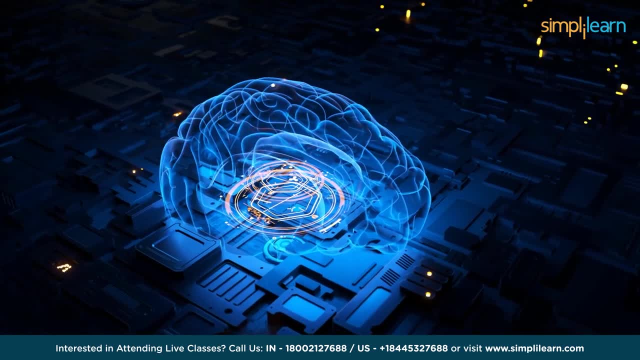 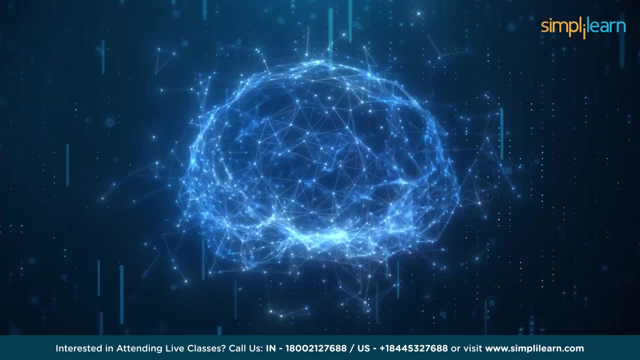 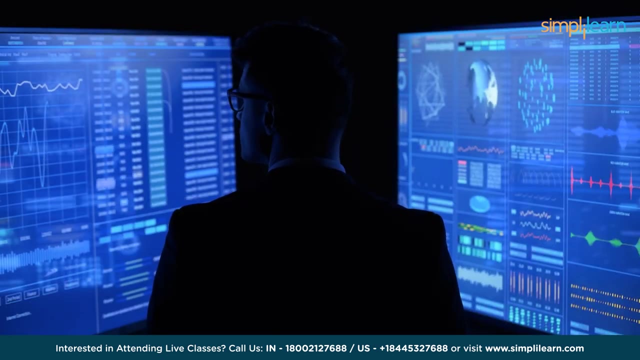 take you on an exhilarating ride through the realms of data science, machine learning and artificial intelligence. Discover the fundamental principles that underpin data science as we demystify complex algorithms and shed light on the inner workings of neural networks. Witness how data science revolutionizes industries, empowering business to make smarter. 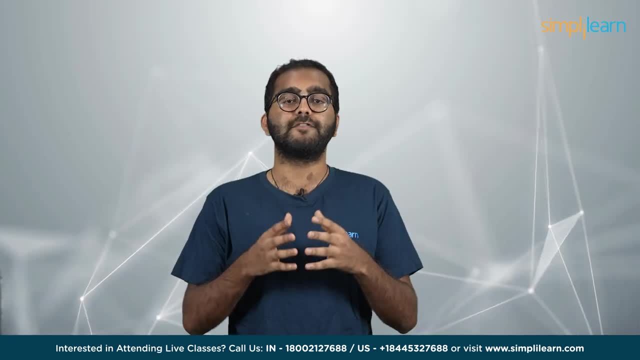 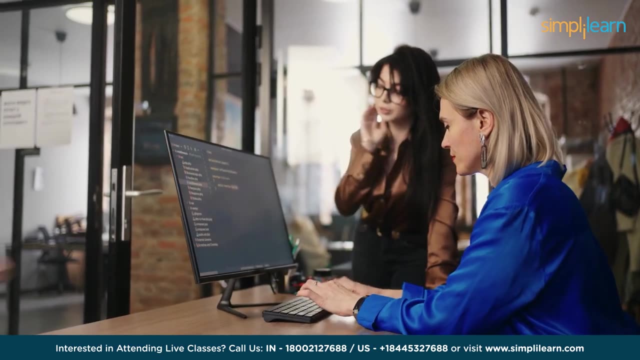 decisions, saving lives and propelling us towards a brighter future. Immense yourself in the captivating world of machine learning, where data science systems evolve, adapt and continuously enhance their performance based on data. Uncover the ethical considerations that surround data science, from privacy and bias to the 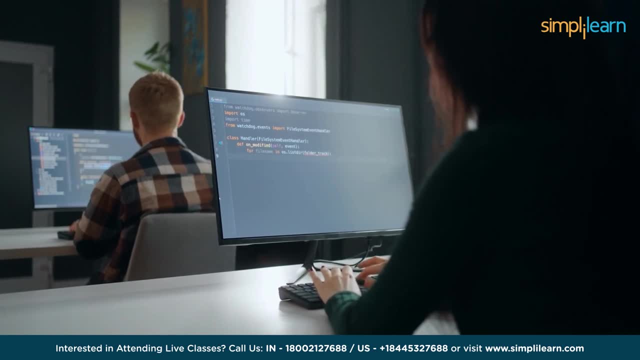 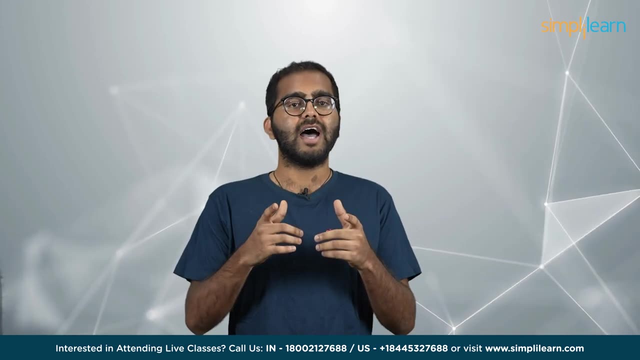 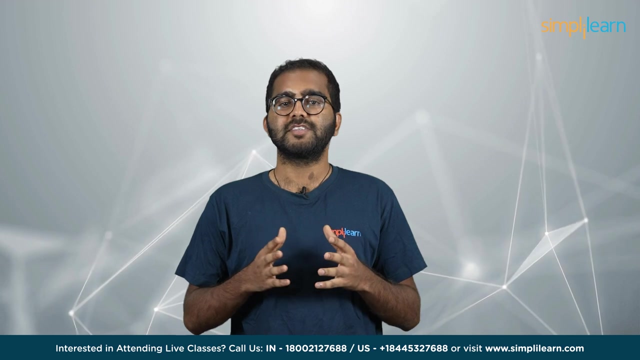 responsible users of these powerful technologies, ensuring a fair and inclusive future. Join us on this extraordinary quest as we unlock the secrets of data science, empowering you to harness its potential and shape the world of tomorrow. Get ready to embark on this transformative journey. Welcome to the data science basics. 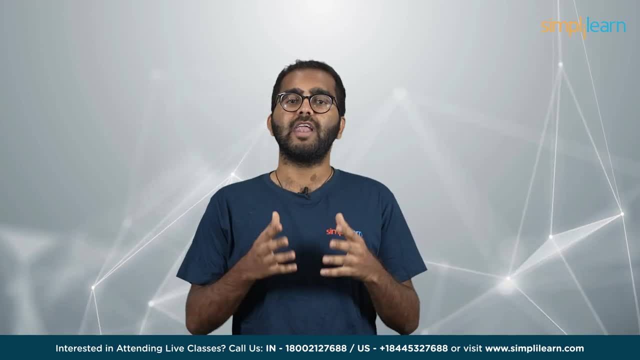 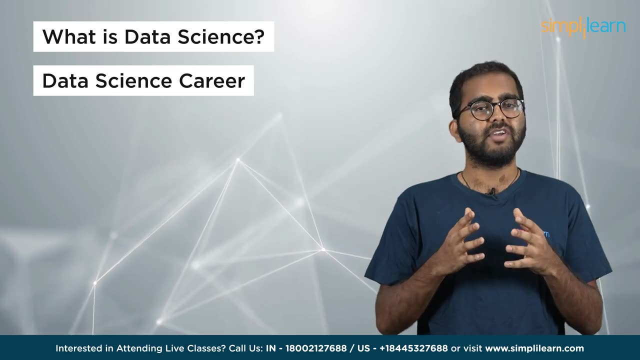 course. Today we will be learning the foundations of data science through the following docket below. First, we will unravel what is data science. First, we will unravel what is data science. First, we will unravel what is data science Moving ahead, we will discuss important reasons on why data science is a perfect career for 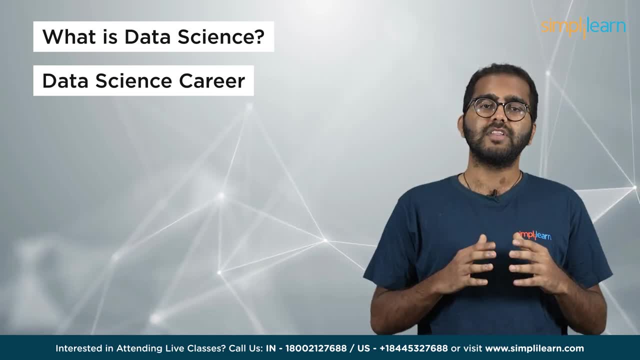 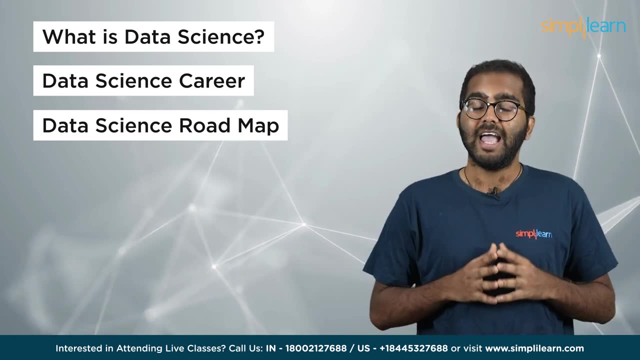 aspiring data scientists in 2023.. Once clear with these goals, let's start mapping our journey by discussing the tried, tested and result-oriented career path to data science. Later, we shall guide you with the perfect courses to begin your learning journey With. 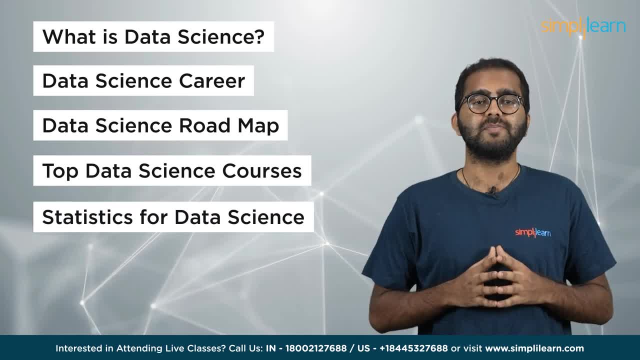 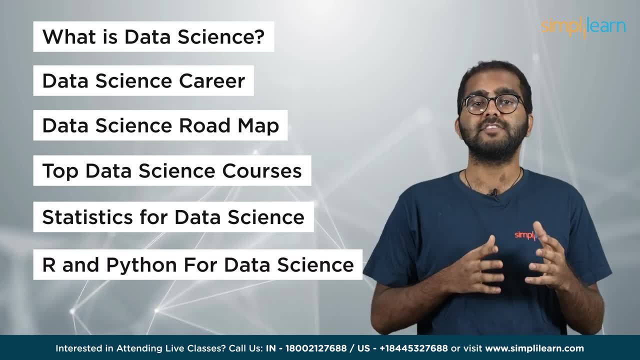 the critical aspects discussed. we will get started with our data science basics by learning mathematics and statistics for data science. Then we will get started with the true programming languages, also known as the two titans of data science, which are none other than. 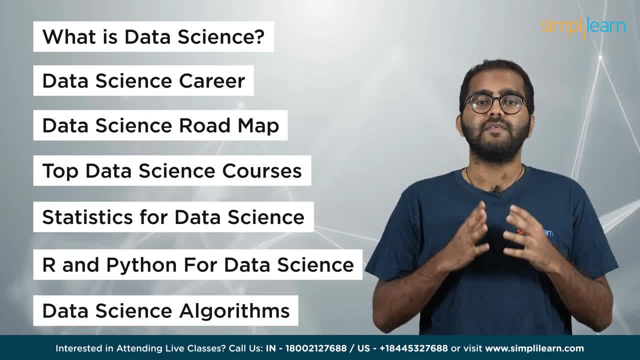 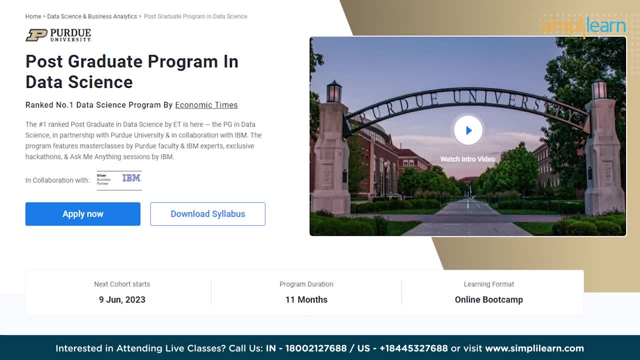 Python and R. And, last but not least, we will conclude the session by discussing the most important data science algorithms. With that having said, if you are someone who is interested in building a career in data science and ML by graduating from the best universities, or a professional who elicits 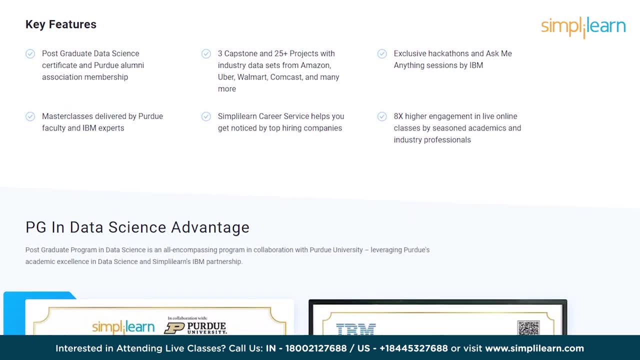 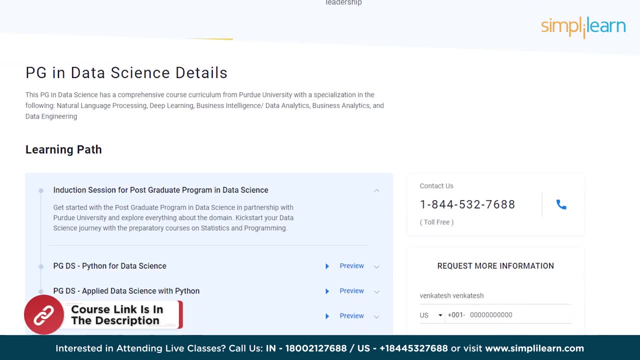 to switch careers with data science by learning from the experts, then try giving a shot at the Simply Learns postgraduate program in data science from Purdue University in collaboration with IBM. The link in the description box should navigate to the homepage, where you can find a complete 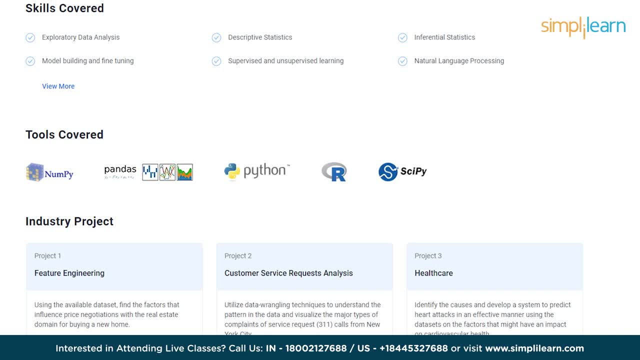 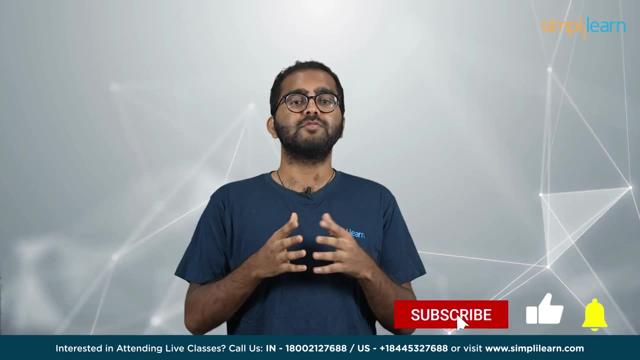 overview of the program being offered. Take action, upskill, get ahead. Let's take a minute to hear from our learners who have experienced massive success in their careers, And if these are the types of videos you would like to watch, then hit that subscribe button. 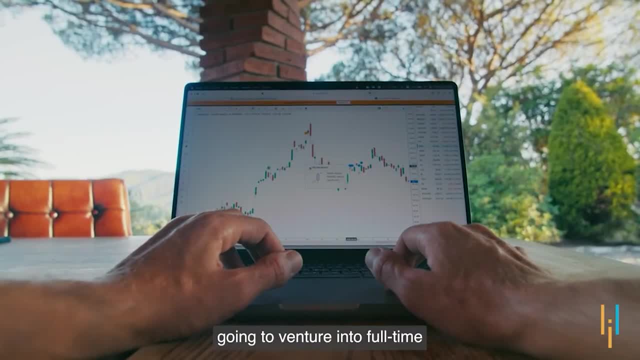 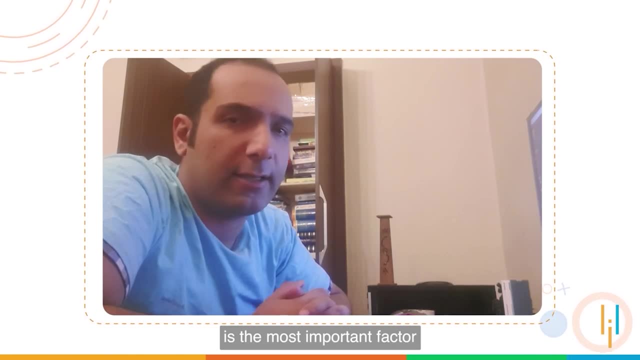 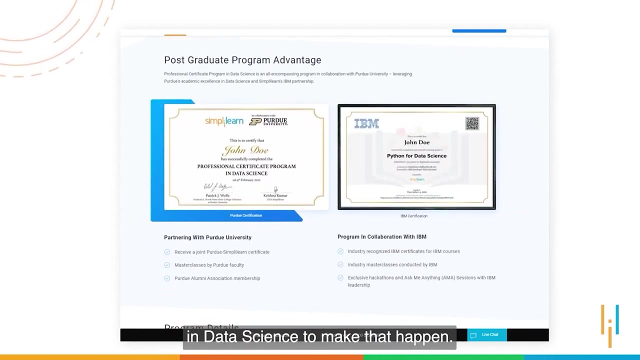 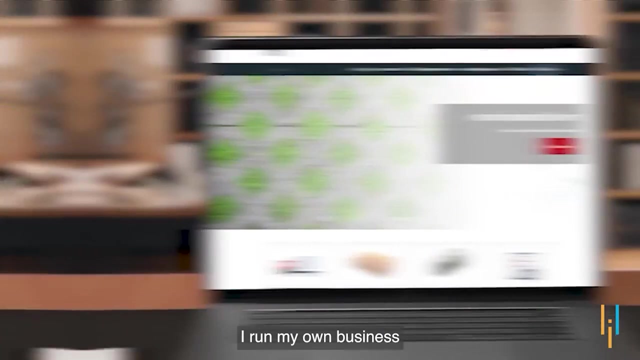 and click on the bell icon to never miss an update from us. I plan to use the Professional Certificate Program in Data Science to make that happen. Hey, I'm Ali Hindi. I live in Iran and I'm a civil engineering professional. I run my own business by the name of ARG CMO. 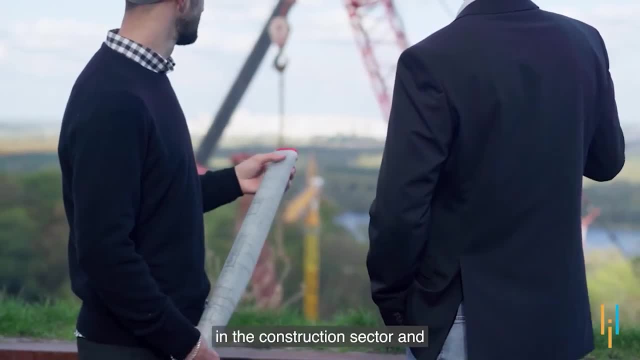 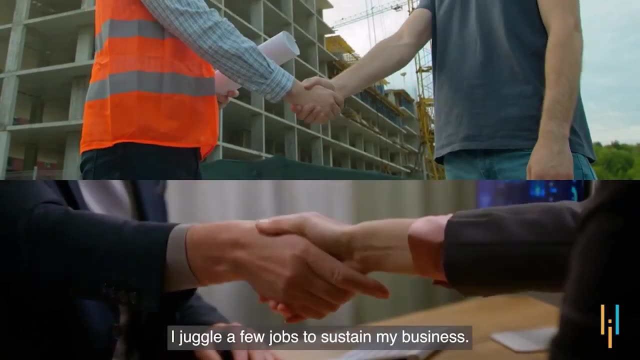 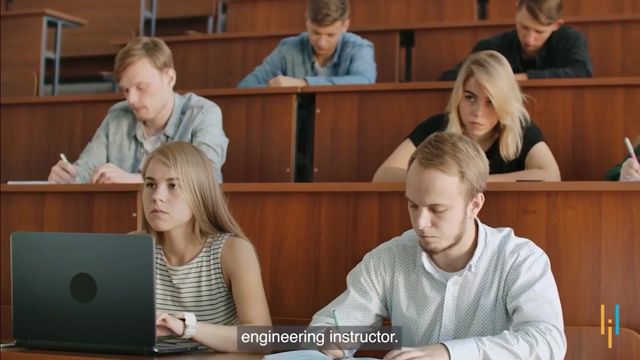 My business deals with providing consultancy in the construction sector and selling artificial stones and black components. I juggle a few jobs to sustain my business. I do some research, I do some research, I do some trading and I teach at the local university as a part-time civil engineering. 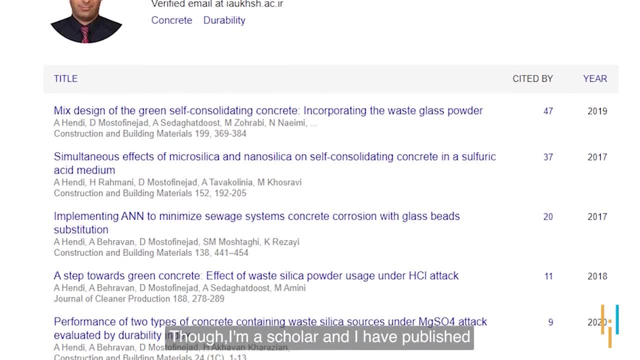 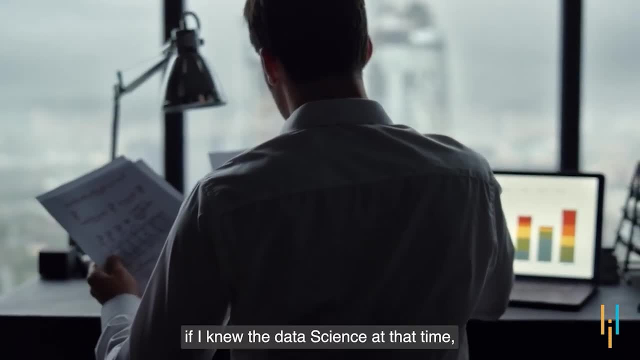 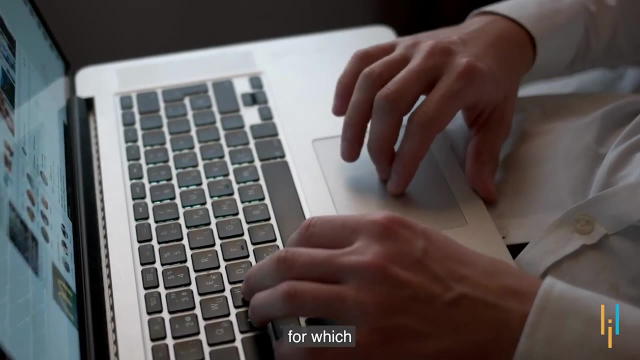 instructor, Though I'm a scholar, and I have published many articles on civil engineering. Now, when I look at them, I feel that if I knew data science at that time, many things would be different. I wanted to enhance my knowledge, for which I decided to take a course in design. 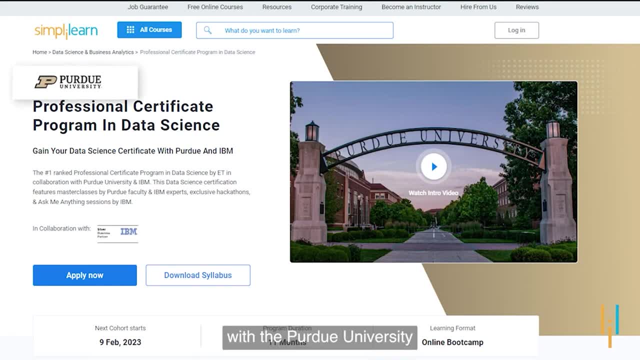 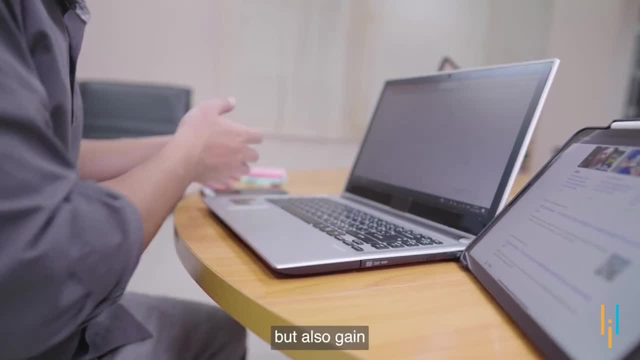 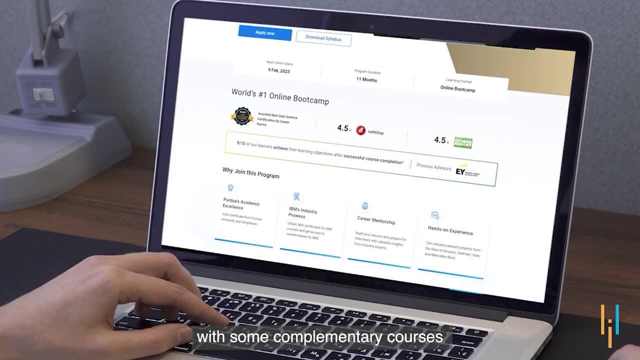 I chose SimpliData's course because of its association with Purdue University. I thought it's not just a good opportunity to learn data science, but also gain a certification from a highly-reputed university. SimpliData also provided me with some complementary courses in Python and Agile, which I think. 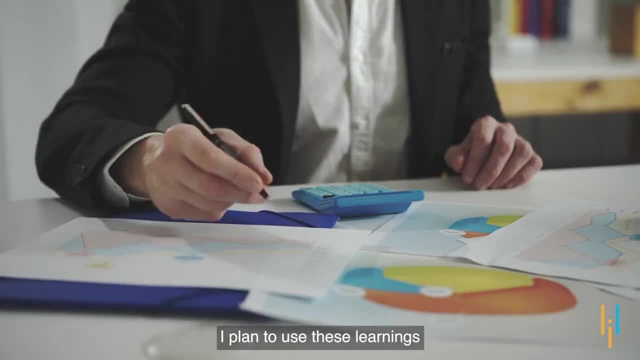 will be really helpful in the long run. I plan to use these learnings to expand my business and make it profitable. At the university, we have to deal with a lot of projects. That is why I decided to take a course in data science. 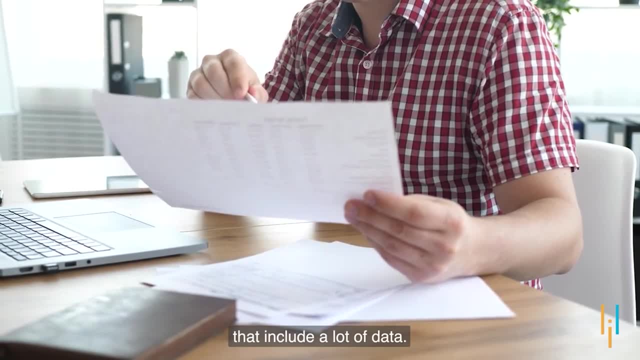 I plan to use these learnings to expand my business and make it profitable. At the university, we have to deal with a lot of projects. That is why I decided to take a course in data science. I plan to use these learnings to expand my business and make it profitable. 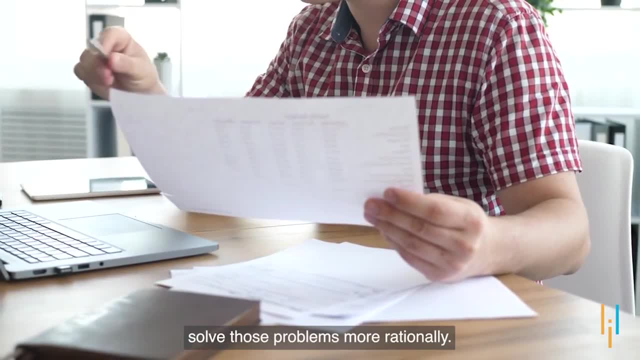 That is why I decided to take a course in data science. I plan to use these learnings to expand my business and make it profitable. I think this course will help me solve those problems more rationally. It will help me build my personal brand as a data scientist too. 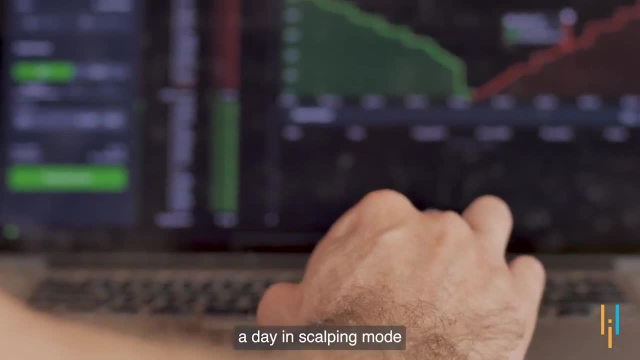 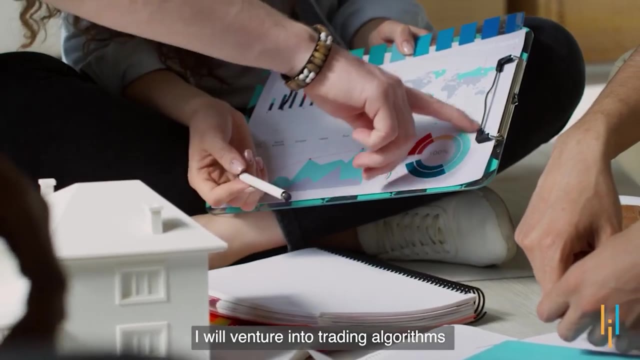 Right now, I spend my time in trading about 5 hours a day in scalping mode with my own strategy, but soon I will venture into trading algorithms which are in dire need of data analysis. I am happy that I am paving the road to success and removing obstacles. 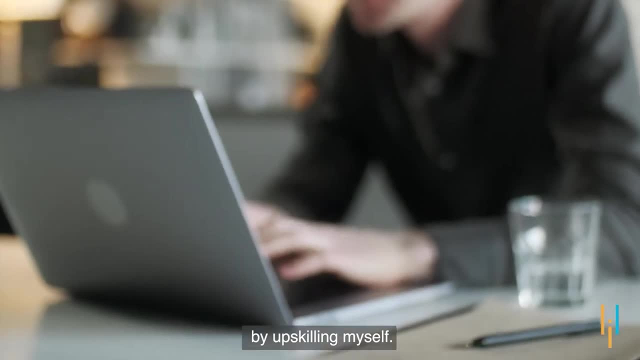 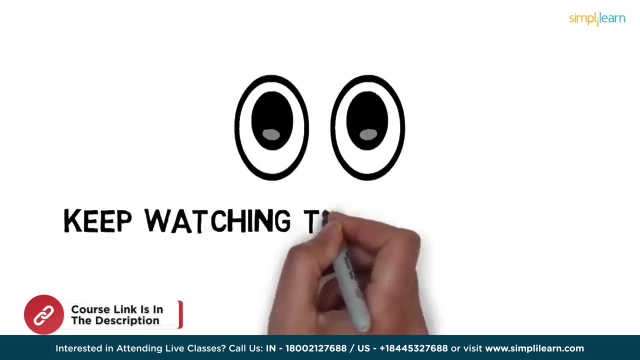 I can now start a new business. I am happy that I am paving the road to success in my way by upskilling myself. are you one of the many who dreams of becoming a data scientist? keep watching this video if you're passionate about data science. 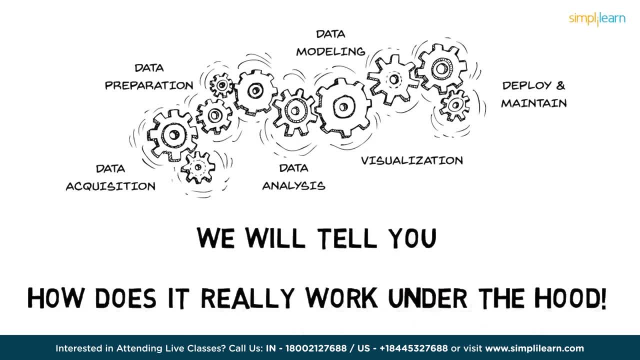 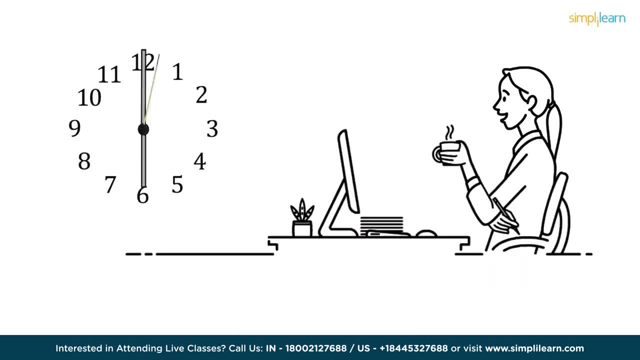 because we will tell you how does it really work. under the hood, Emma is a data scientist. let's see how a day in a life goes while she's working on data science project. well, it is very important to understand the business problem first. in our meeting with the clients, Emma asks relevant questions. 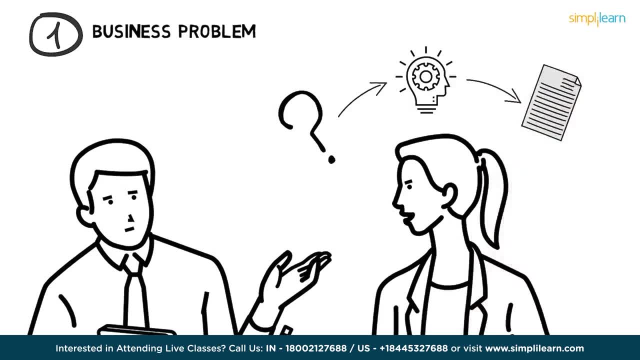 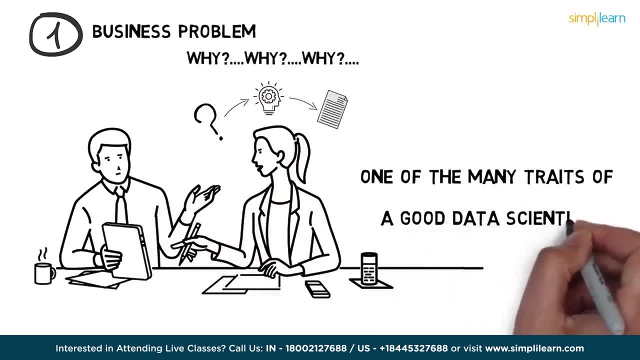 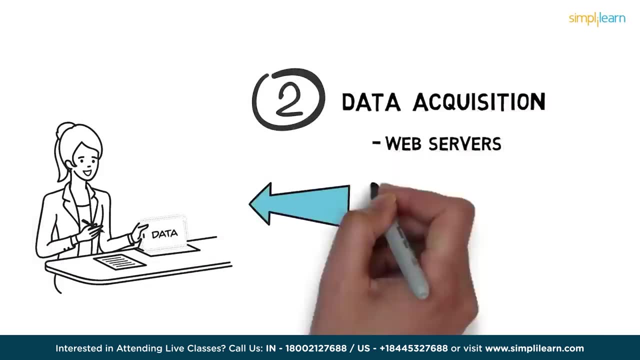 understands and defines objectives for the problem that needs to be tackled. she's a curious soul who asks a lot of eyes- one of the many traits of a good data scientist. now she cares up for data acquisition to gather and scrape data from multiple sources like web servers, logs, databases, API's and online. 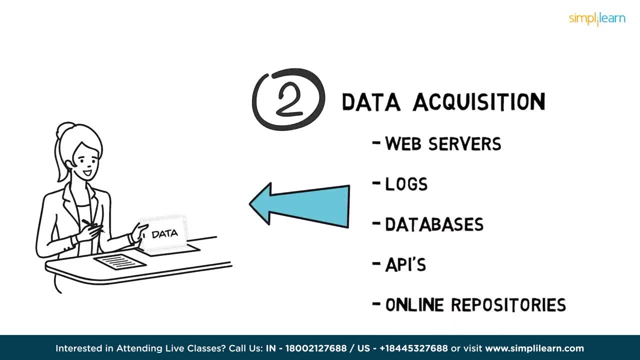 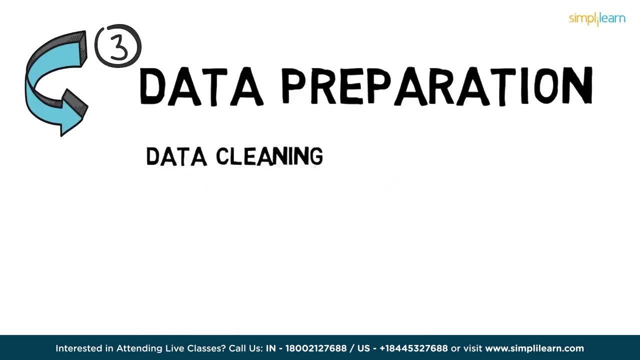 repositories. oh, it seems like finding the right data takes both time and effort. after the data is gathered comes data preparation. this step involves data cleaning and data transformation. data cleaning is the most time consuming process, as it involves handling many complex scenarios. here Emma deals with inconsistent data types, misspelled attributes, missing values, duplicate. 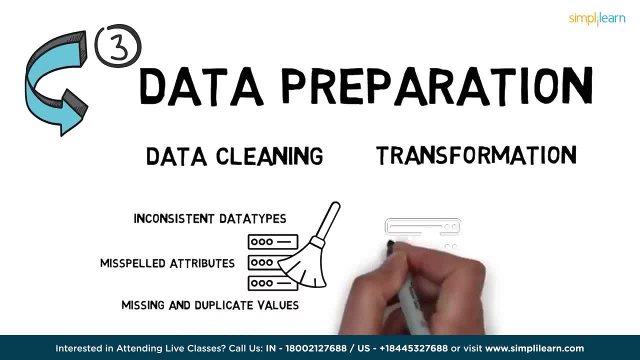 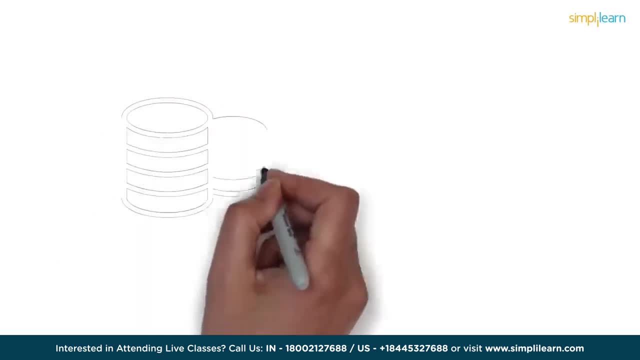 values and whatnot. then in data transformation, she modifies the data based on defined mapping rules. in a project ETL tools like talent and informatica are used to perform complex transformations. that helps the team to understand the data structure better. then understanding what you actually can do with your data is very 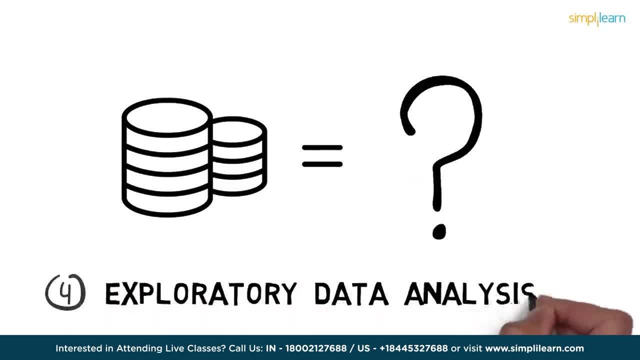 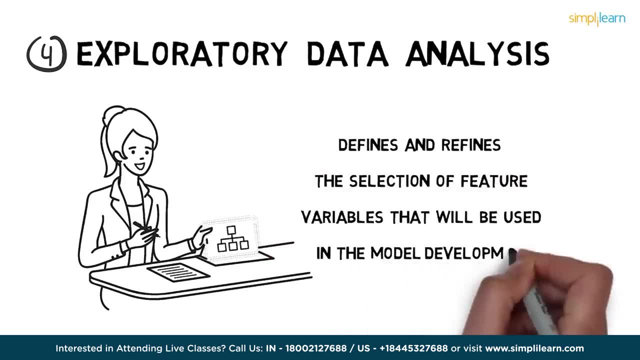 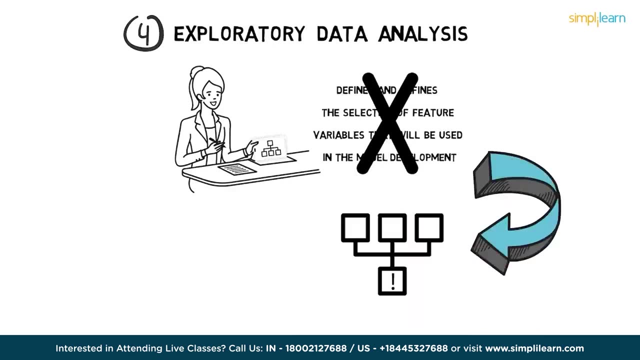 crucial for that. Emma does exploratory data analysis. with the help of EDA, she defines and refines the selection of feature variables that will be used in the model development. but what if Emma skips this step? she might end up choosing the wrong variables, which will produce an inaccurate model. thus, exploratory data 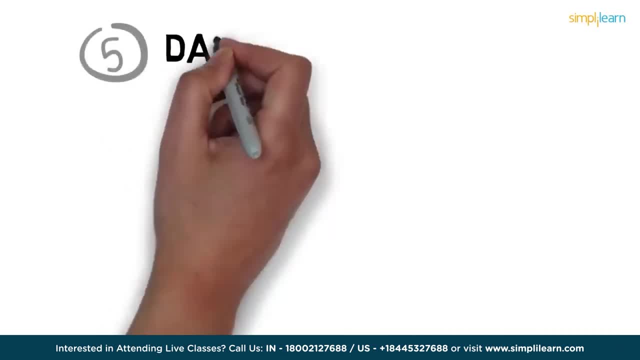 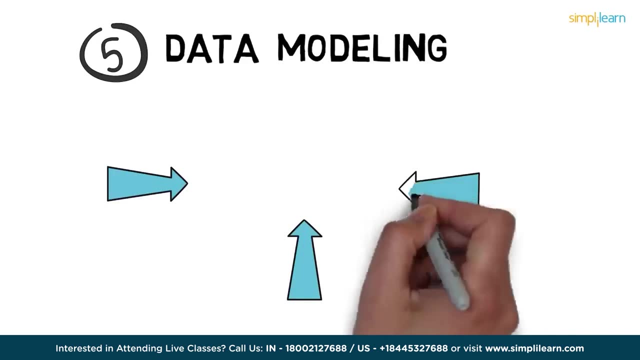 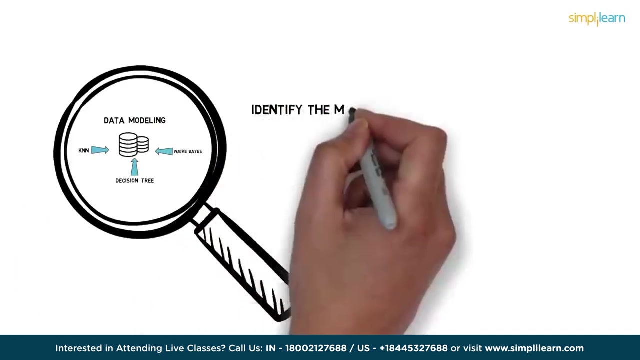 analysis becomes the most important step. now she proceeds to the core activity of a data science project, which is data modeling. she repetitively applies diverse machine learning techniques, like Gannon decision tree knife phase, to the data to identify the model that best fits the business requirement. she trains the models on the 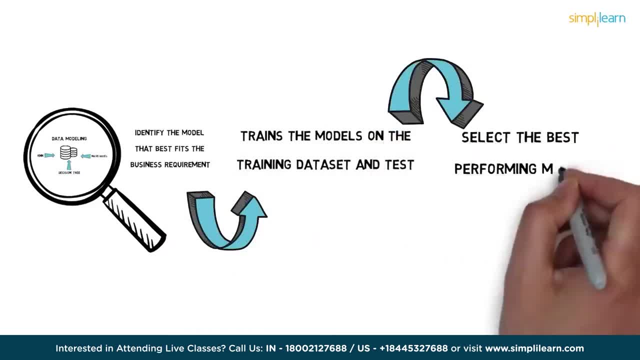 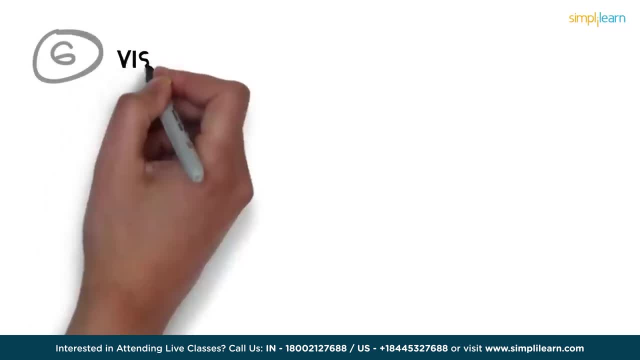 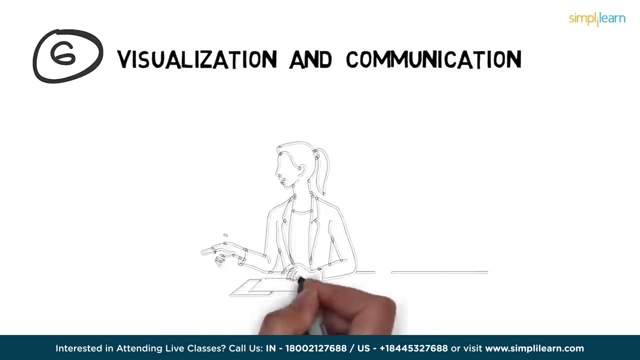 training data set and test them to select the best performing model. Emma prefers python for modeling the data. however, it can also be done using R and SAS. well, the trickiest part is not yet over: visualization and communication. Emma takes the clients again to communicate the business findings in a simple and 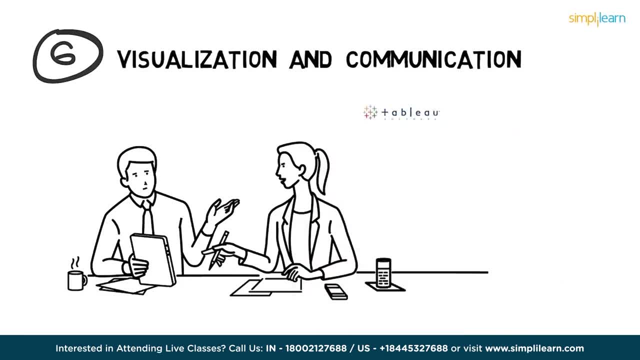 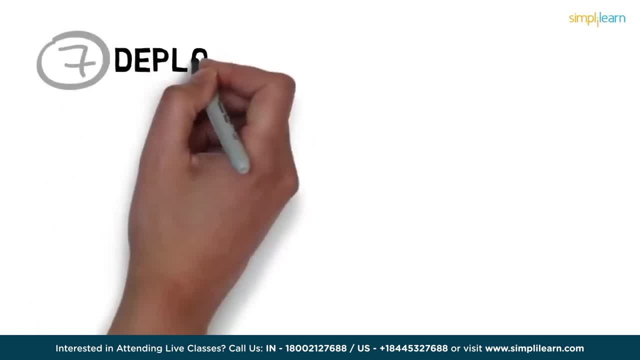 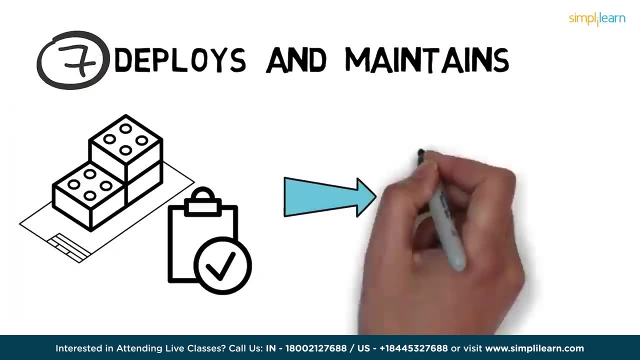 effective manner to convince the stakeholders. she uses tools like tableau power, BI and click view that can help her in creating powerful reports and dashboards. and then, finally, she deploys and maintains the model. she tests the selected model in a pre-production environment before deploying it in the 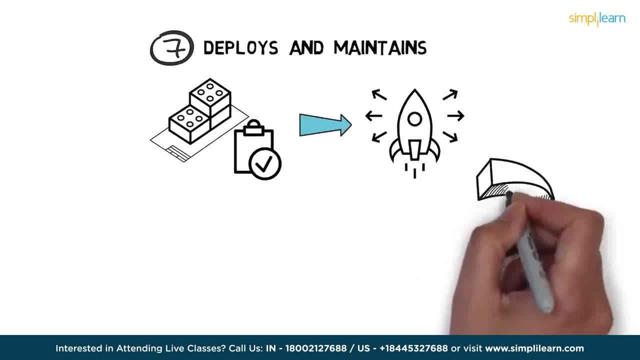 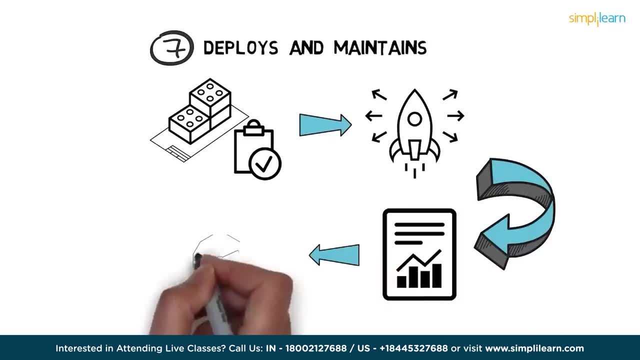 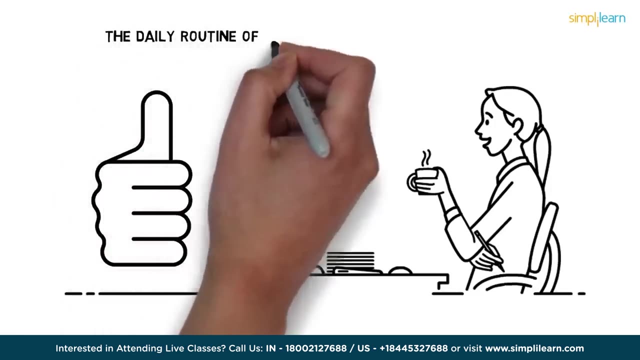 production environment, which is the best practice. right after successfully deploying it, she uses reports and dashboards to get real-time analytics. further, she also monitors and maintains the project's performance. well, that's how Emma completes the data science project. we have seen the daily routine of a data scientist is a whole lot of fun, has a lot of interesting aspects. 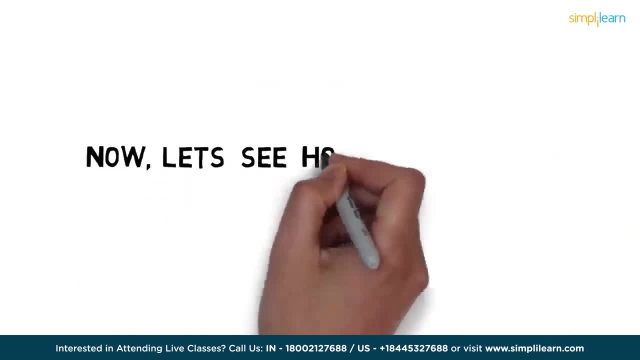 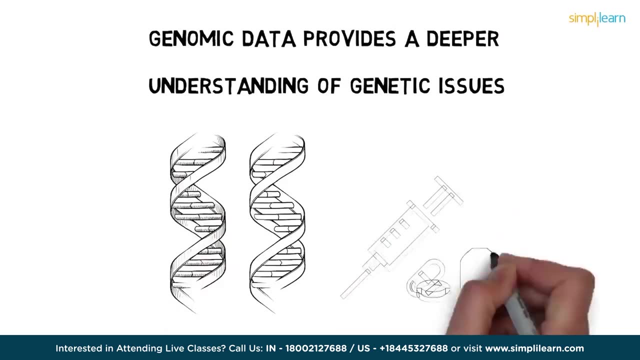 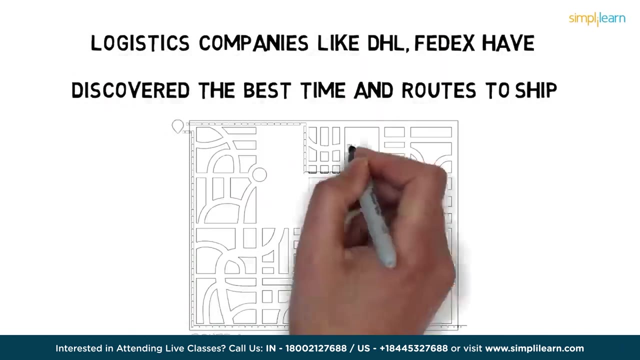 and comes with its own share of challenges. now let's see how data science is changing the world. data science techniques, along with genomic data, provides a deeper understanding of genetic issues in reaction to particular drugs and diseases. companies like DHL, FedEx have discovered the best routes to ship the. 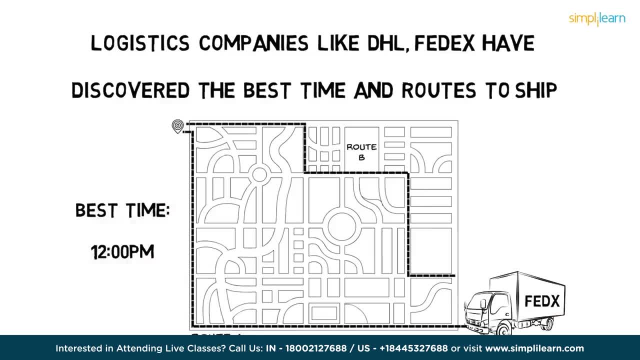 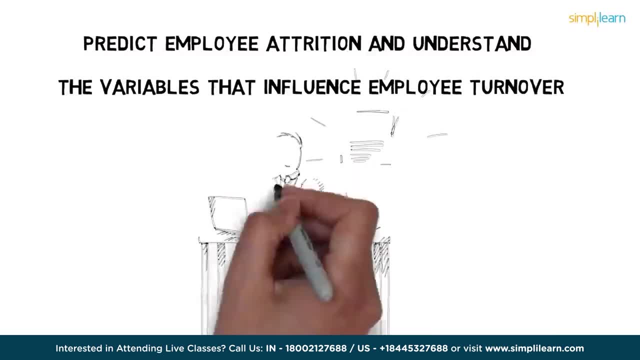 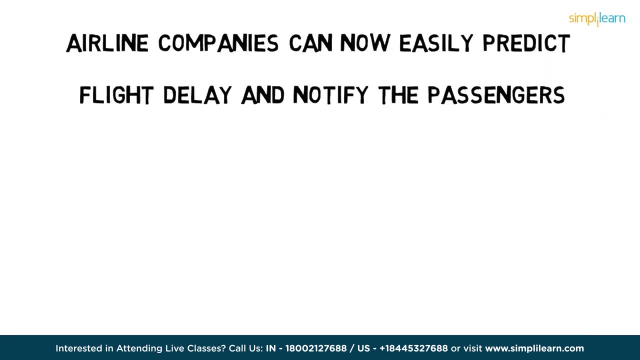 best suited time to deliver, the best mode of transport to choose, thus leading to cost efficiency. with data science, it is possible to not only predict employee attrition, but to also understand the key variables that influence employee turnover. also, the airline companies can now easily predict flight delay and 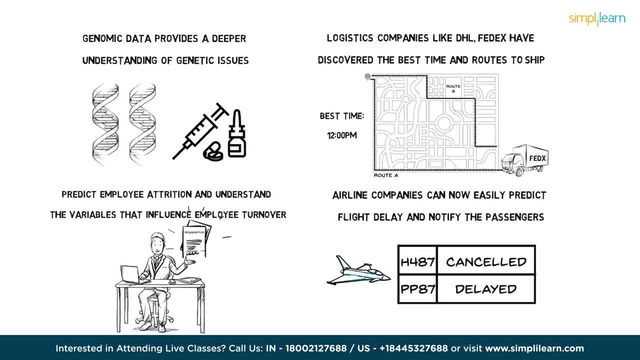 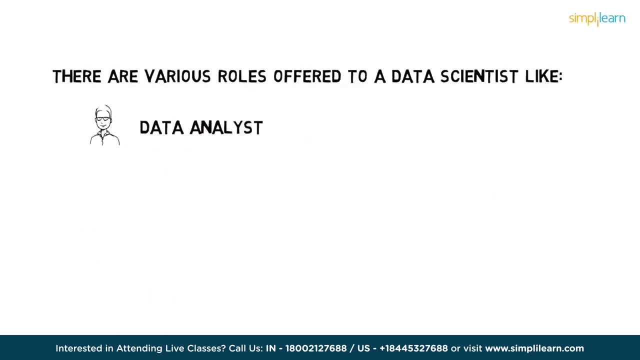 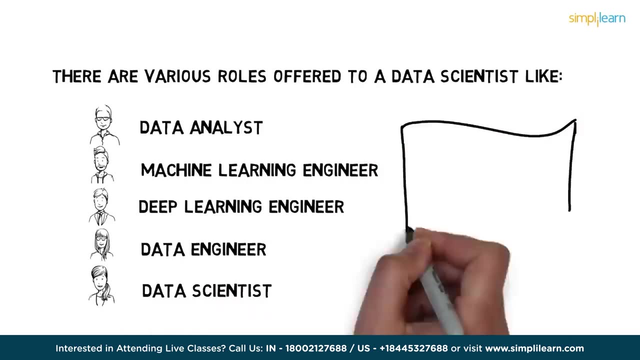 notify the passengers beforehand to enhance their travel experience. well, if you're wondering, there are various rules offered to a data scientist, like data analyst, machine learning engineer, deep learning engineer, data engineer and, of course, data scientist. the median based salaries of a data scientist can range from 95 000 to 165 000, so that was about the data. 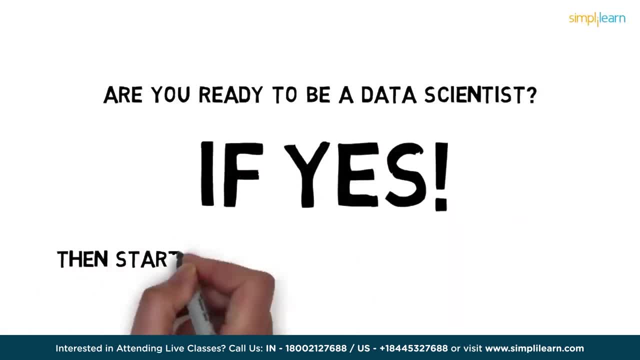 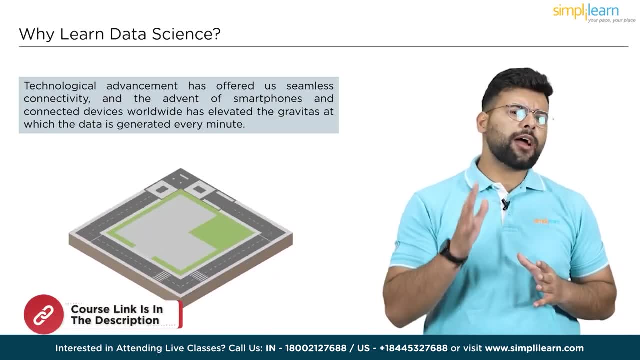 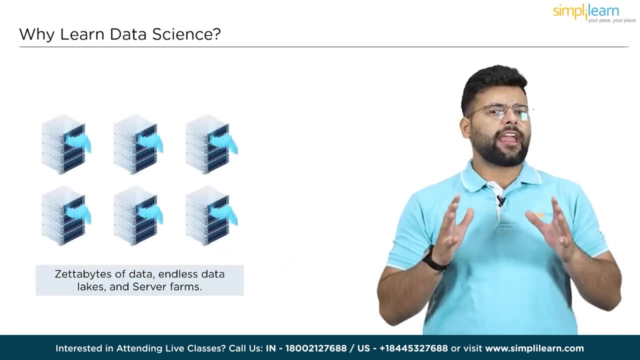 science. are you ready to be a data scientist? if yes, then start today. the world of data needs you. technological Advancement has offered a seamless connectivity, and the advent of smartphones and connected devices worldwide has elevated the gravitas at which the data is generated. every minute, zettabytes of data, endless data lakes and 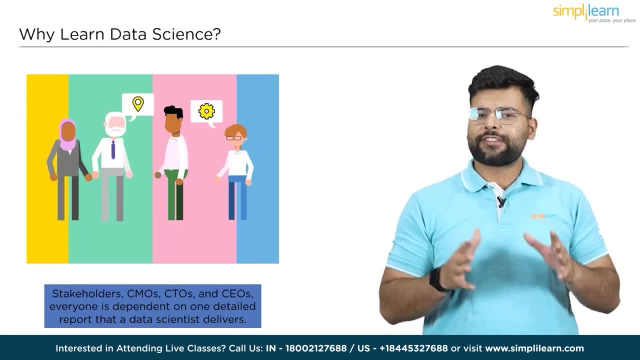 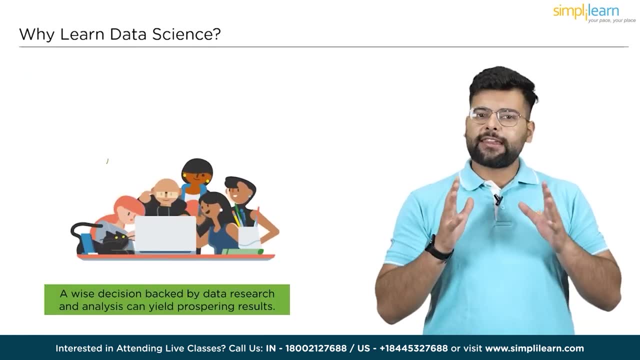 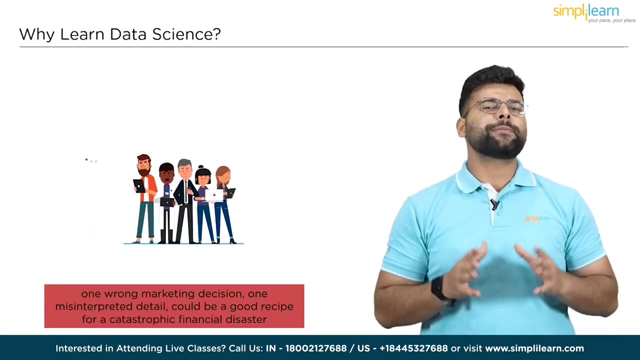 several farms, billion dollar investments, stakeholders, CMOs, CTOs and CEOs: everyone is dependent on one detailed report that data scientist delivers. a wise decision backed by data, research and analysis can yield prospering results. still on the contrary, one wrong marketing decision, one misinterpreted detail could be a good recipe for a catastrophic financial disaster for 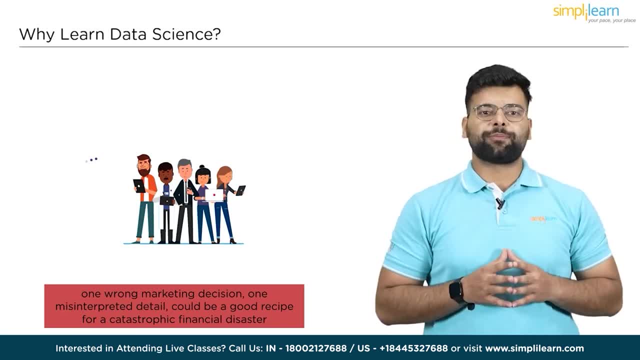 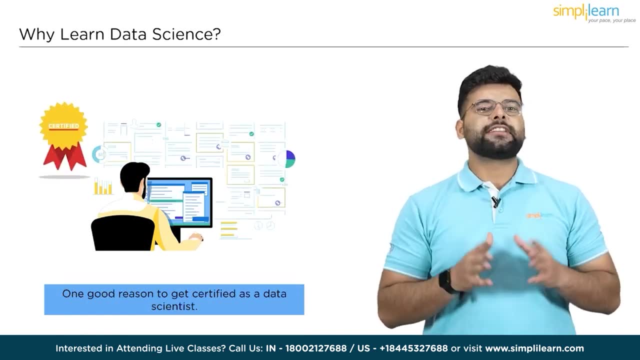 an organization. that's the pivotal role a data scientist pays in any organization. a data scientist caliber to device algorithm, to crunch numbers and extract precious information is invaluable. this is one good reason why data science is reported as a top IT profession in the current IT industry and 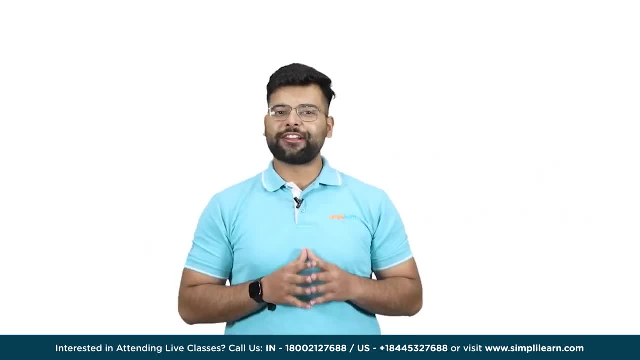 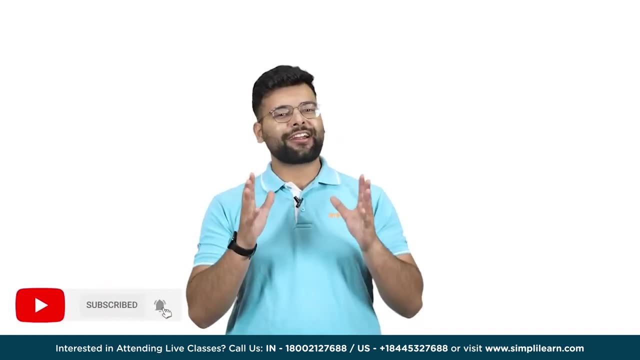 is projected to be on the top for a good time. welcome to simply lens YouTube channel. today, we will explain why you should learn data science. before we get started, take a moment to subscribe to us and hit the bell to get notified of our content. if you're watching this, I'm sure you 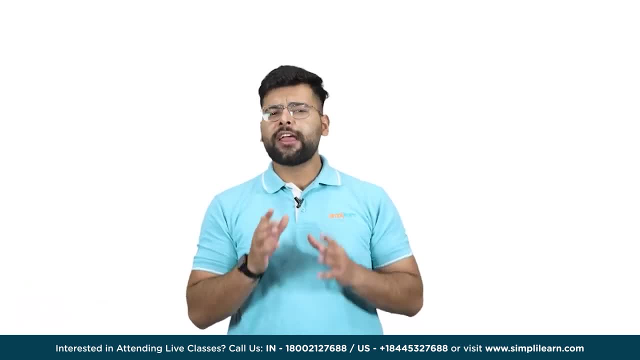 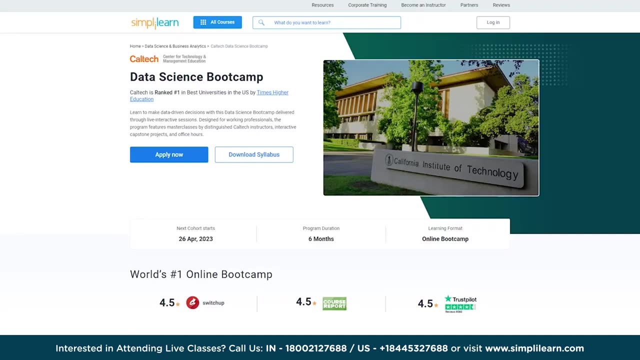 are interested in data science, looking for a flexible online training program that better suits you, like a glove and helps you get ahead in your career. well, your search ends here. simply learn is offering an online data science boot camp with Caltech in collaboration with IBM. here you will be mentored by real-time industry professionals aligning your 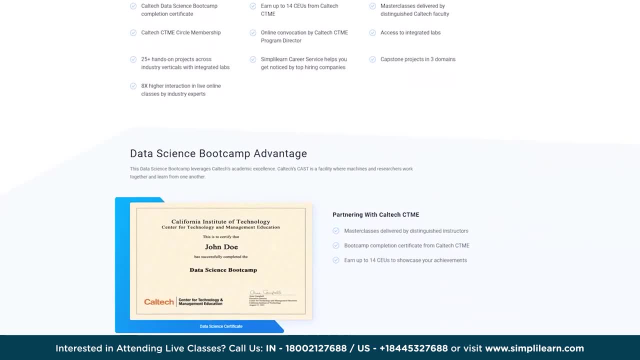 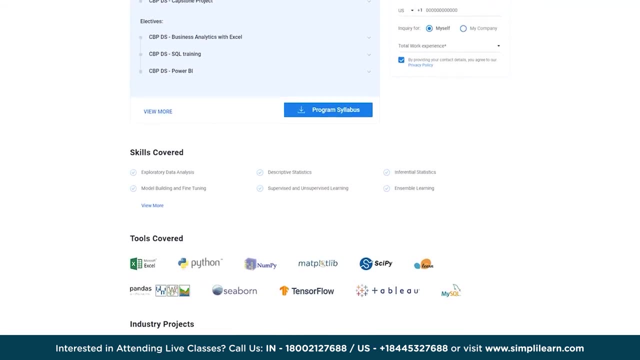 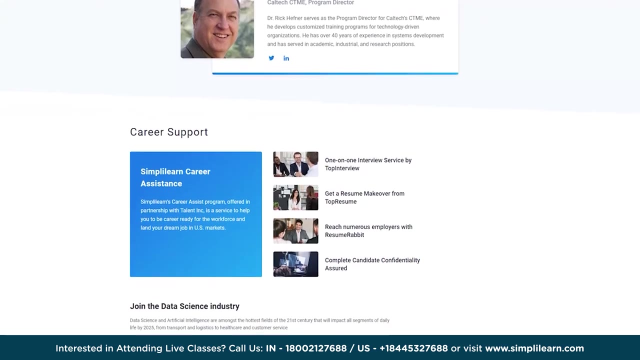 learnings to the current industry standards to get a better chance of planning your dream job. the course covers the most sought-after technical skills like exploratory data analysis, descriptive statistics, inferential statistics, model building and fine-tuning, supervised and supervised learning, ensemble learning, deep learning, data visualization, and the course will help you. 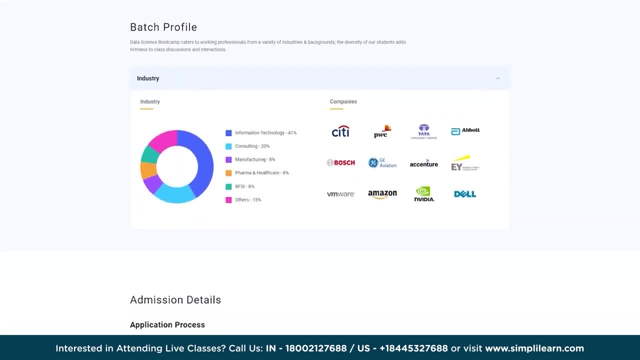 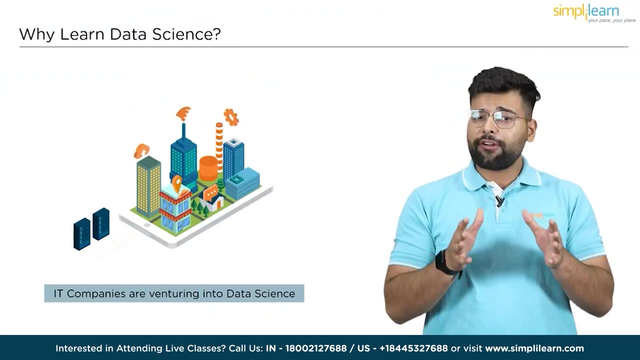 get hands-on with important tools like numpy, pandas, python, R and sci-fi. what are you waiting for? hurry up. for more details, check the link in the description box below. IT firms are venturing into data science, recognizing its potential to open the doors to wide spectrum of opportunities it enables. 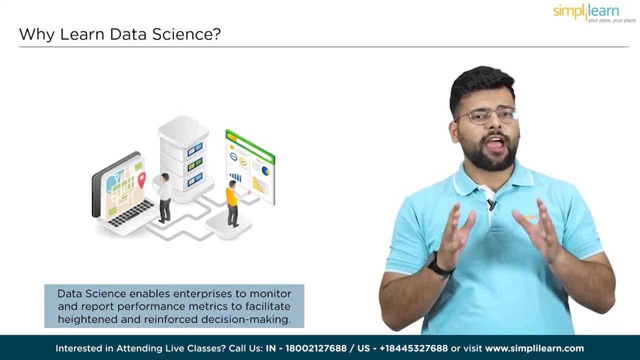 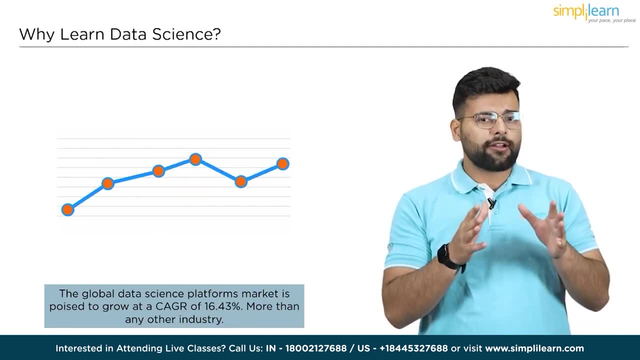 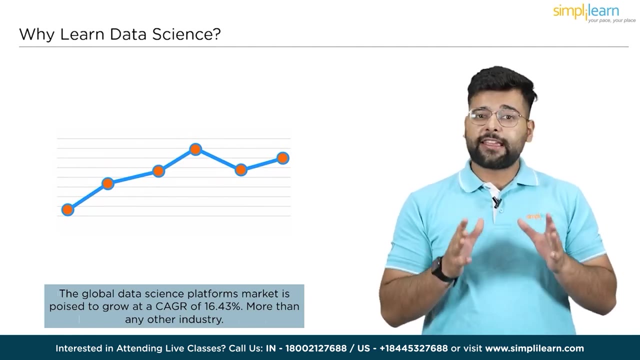 enterprises, to monitor and report performance metrics, to facilitate heightened and reinforced data and now analyze trends. to make critical decisions. to engage clients better, enhance company performance, boost productivity and increase profitability. the organizational importance of data science is increasing at a relentless pace. the global data science platforms market is poised. 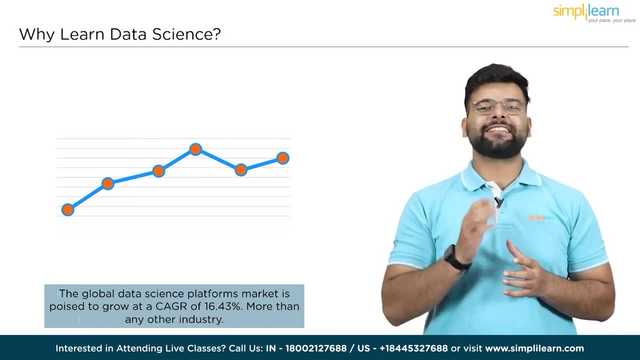 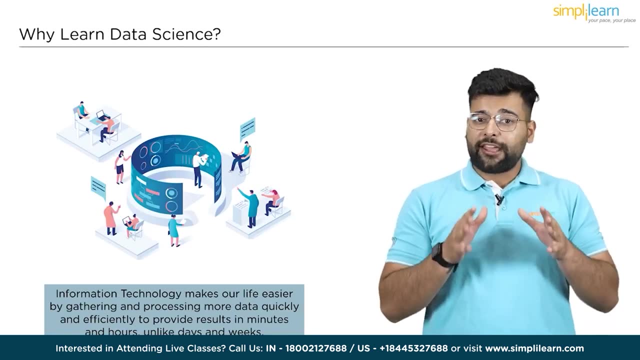 to grow at a CAGR of 16.43 percent, more than any other industry. converging to IT. data science facilitates it with its power to extract information from larger volumes of data. information technology makes our life easier by gathering and processing more data quickly and efficiently. to 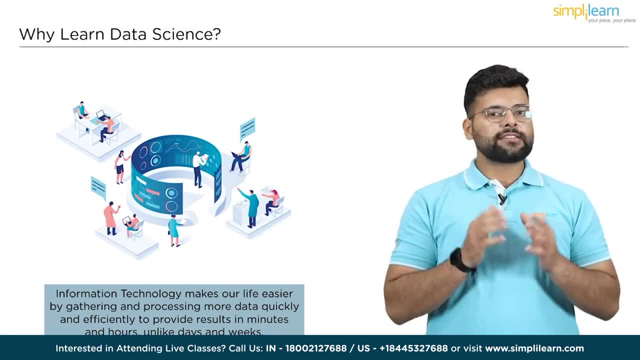 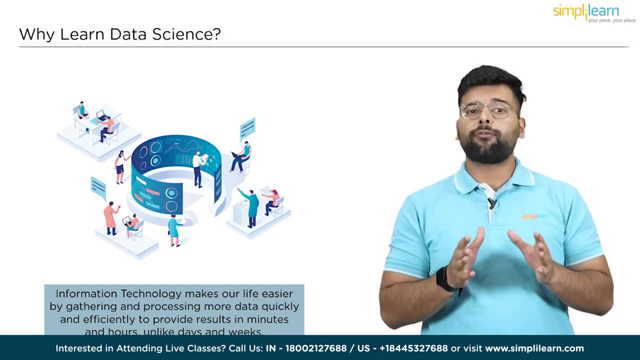 provide results in minutes and hours, unlike days and weeks. statistics and science have become the answer to complex data. data science enables tapping and analyzing massive amounts of untapped data from many sources to leverage productivity and profitability. this is one good reason why many tech experiments find data science to be the most interesting job profile apart from the 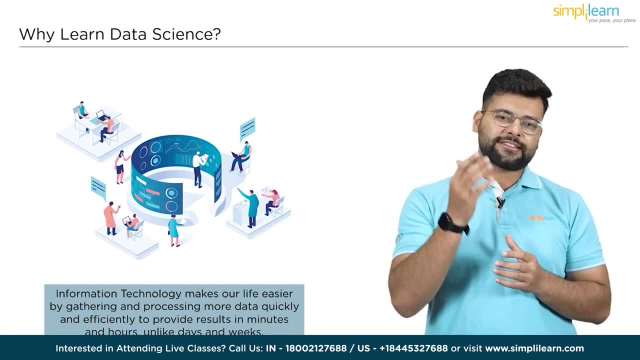 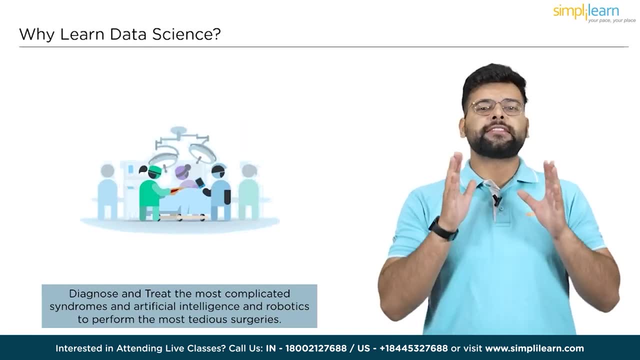 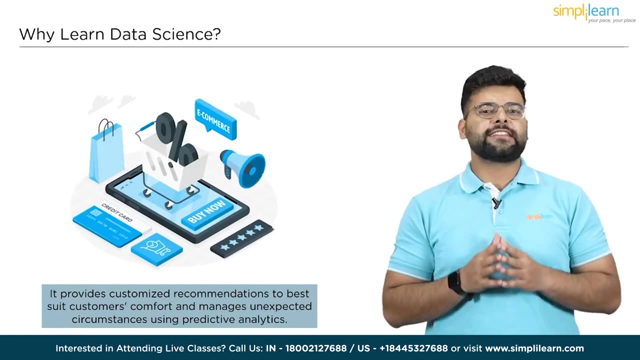 IT domain. data science has spread its roots into other fields. for instance, the healthcare sector is more inclined towards data science and artificial intelligence to diagnose and treat the most complicated syndromes, and robots to perform the most tedious surgeries. online stores and shopping websites depend solely on data science to manage the supply chain and enhance the user. 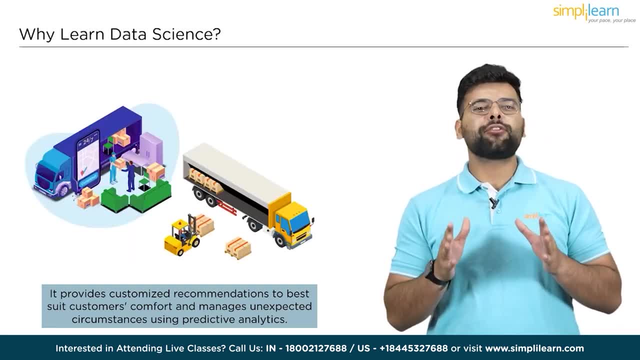 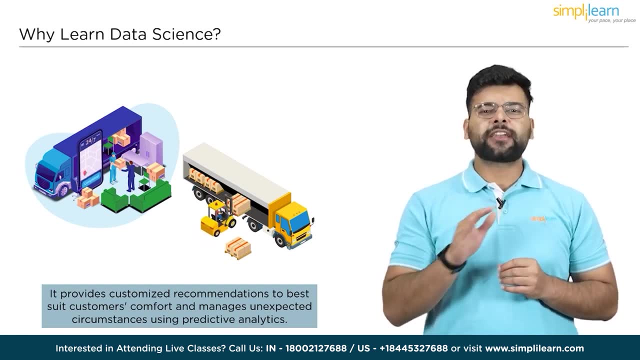 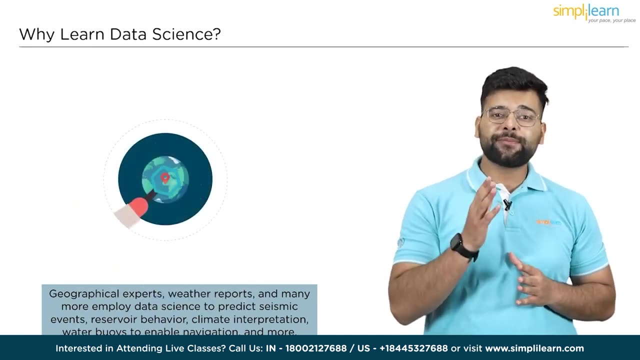 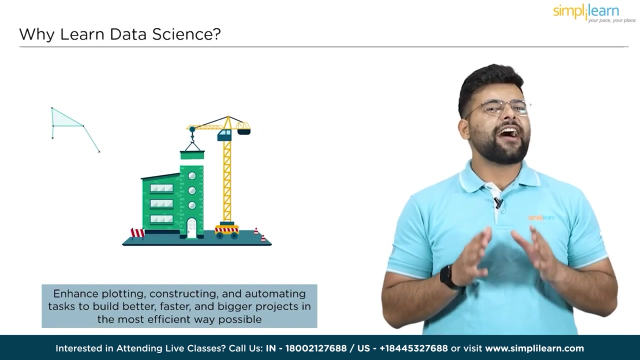 experience by recommending the right product. data science plays a pivotal role in transportation and logistics. it provides customized recommendations to best suit customers comfort and manages unexpected circumstances, using predictive analytics, geographical experts, weather reports and many more employee data science to predict systemic events, reservoir behavior, climate interpretation, water boys to enable navigation and more construction companies are. 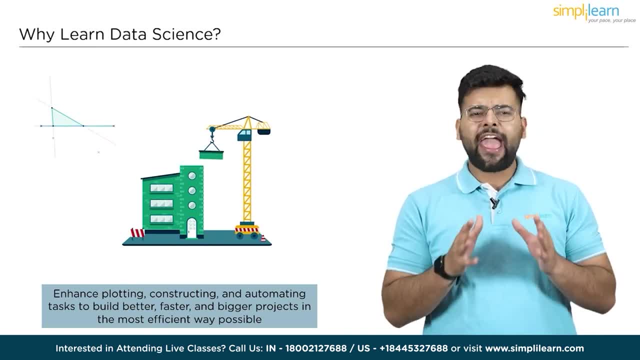 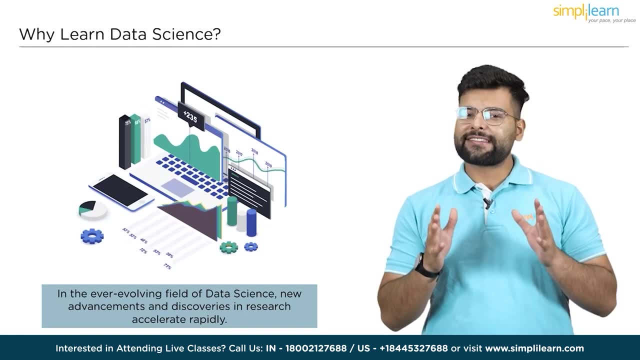 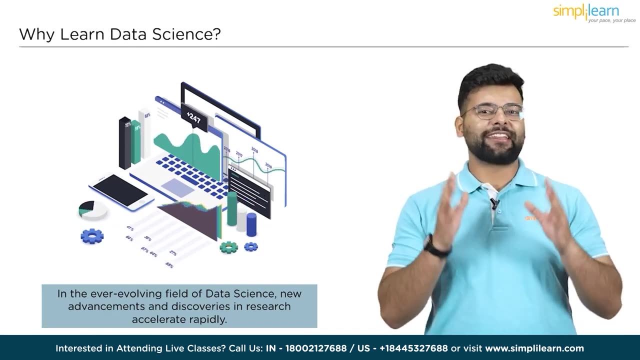 integrating their process with data science to enhance floating, constructing and automating tasks, to build better, faster and bigger projects in the most efficient way possible. in the ever evolving field of data science, new advancements and discoveries in research accelerate rapidly. you always get to learn something new, making every day's work exciting. new data science skills can be. 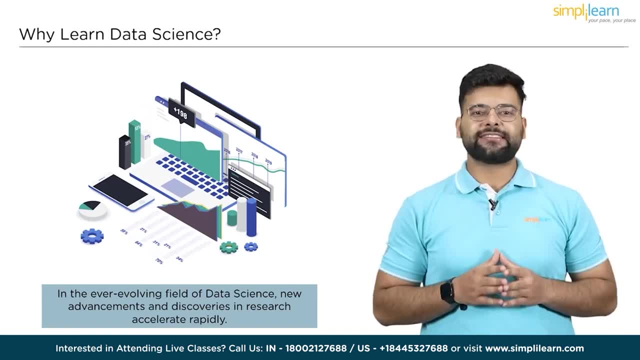 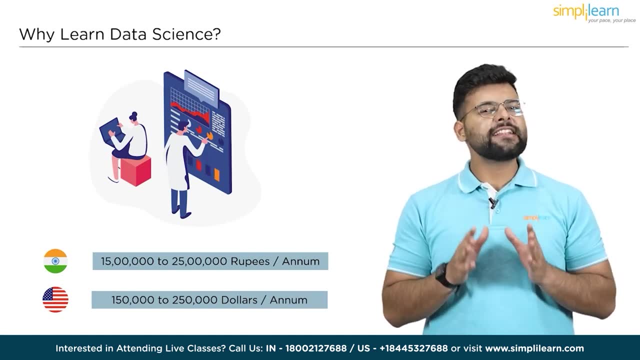 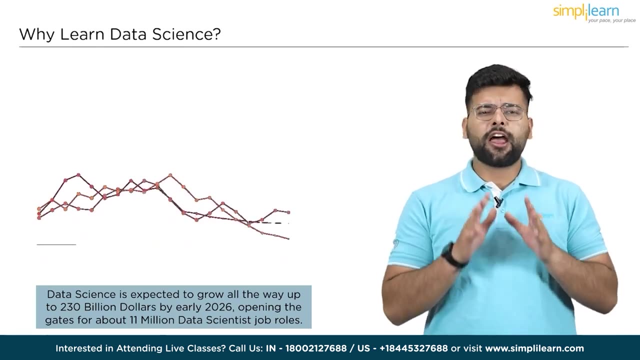 quite endlessly, giving you a competitive edge with knowledge and expertise. the salary of a data scientist in India ranges from 15 to 25 lakhs per annum, and in the United States of America the salaries range from 150 000 to 250 000 per annum. depicting the future of data science results in: 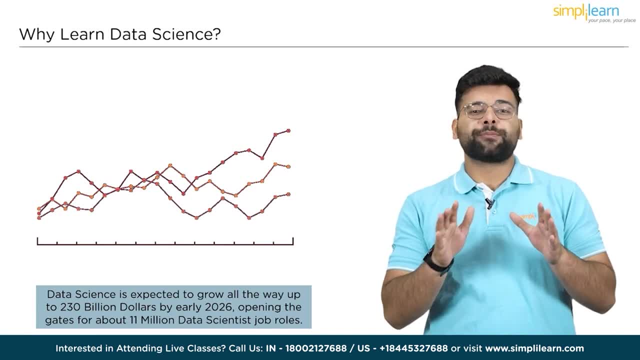 an unmatched potential to settle in a secure job role. as the field expands, more jobs should become available, as more data scientists are needed for analysis. individuals wishing to pursue a career in data science can look forward to bright future with data science. data science has a huge scope across. 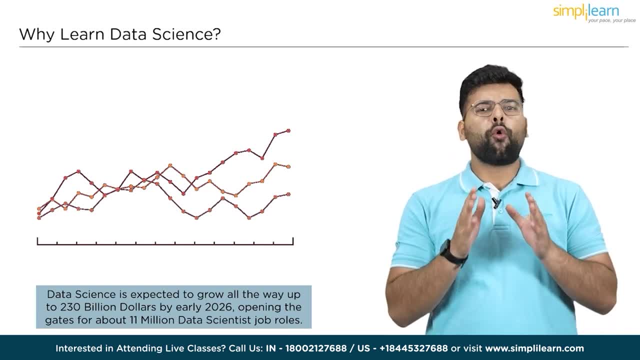 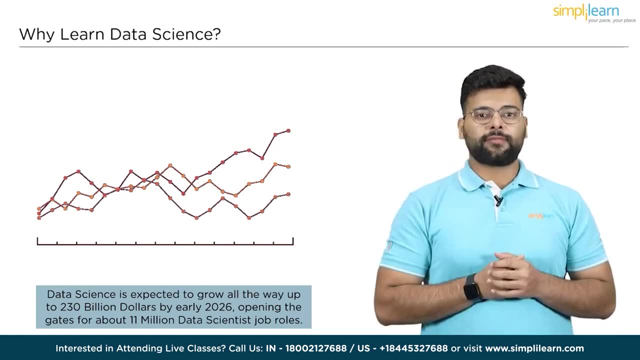 all industries. the global market for data science is expected to grow all the way up to 230 billion dollars by early 2026, opening the gates for about 11 million data scientists job roles. another important aspect of the future of data science is artificial intelligence. AI will likely to be most powerful. 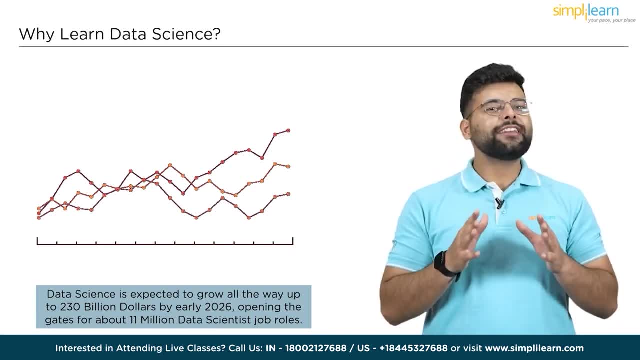 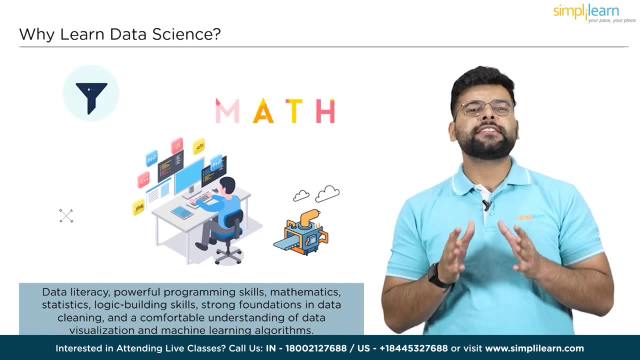 technology data scientists will have to deal with in the future. to put it another way, the future of data science will align itself to make it better in the long run. to become a data scientist, the professionals in the organizations need to have healthy data literacy, powerful programming skills. 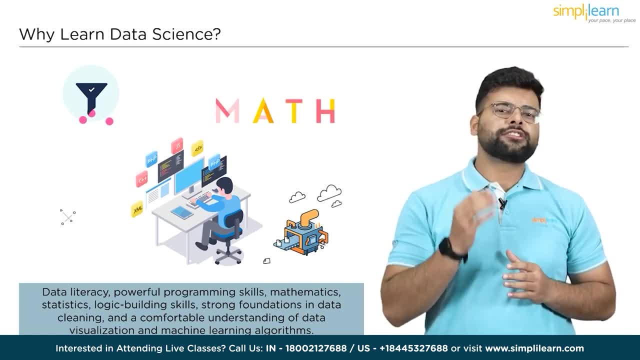 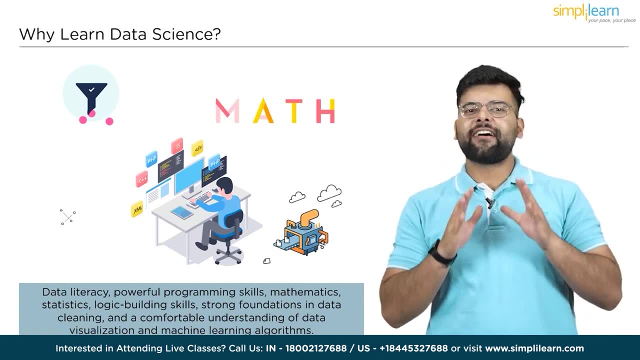 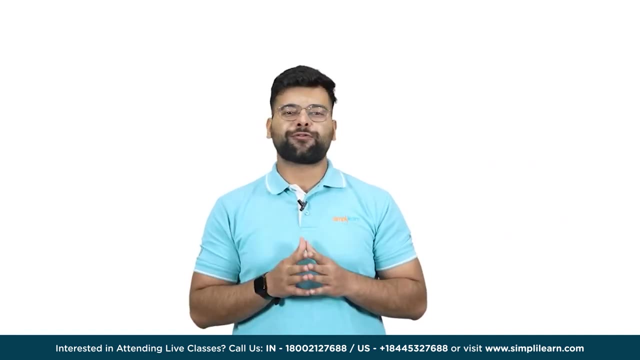 mathematics, statistics, logic building skills, strong Foundations in data cleaning and a comfortable understanding of data visualization and machine learning algorithms. handling all these are nothing less than herding cats. one skill gap could be the final nail in the coffin. if you are an aspiring data scientist looking for online training and certifications from prestigious 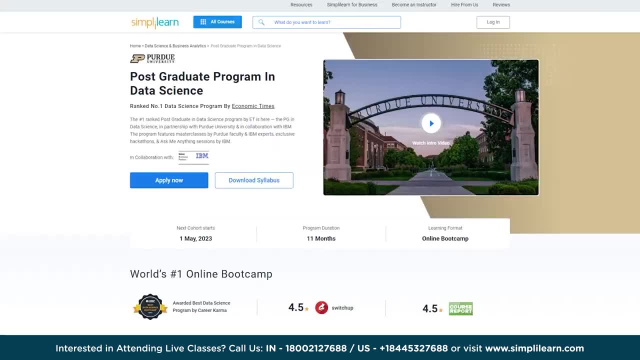 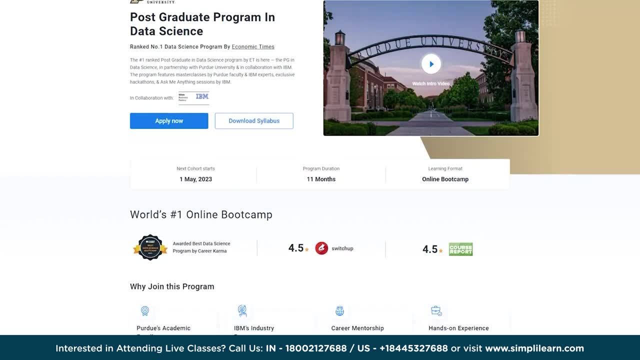 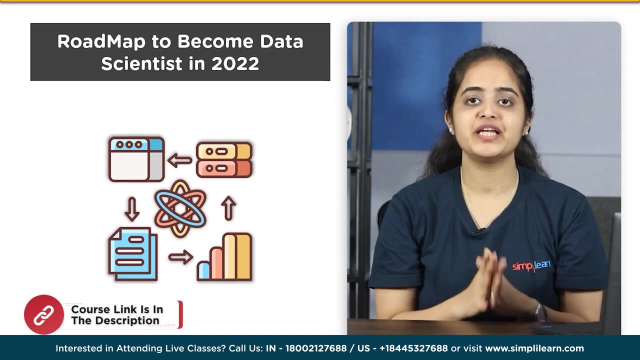 universities and in collaboration with leading experts. then search no more. just cap simply learns. postgraduate program in data science from Purdue University in collaboration with IBM. that should use the link given in the description box below. Google had gathered five exabytes of data between the beginning of time 2003. this amount of data started to be produced every two days in 2010. 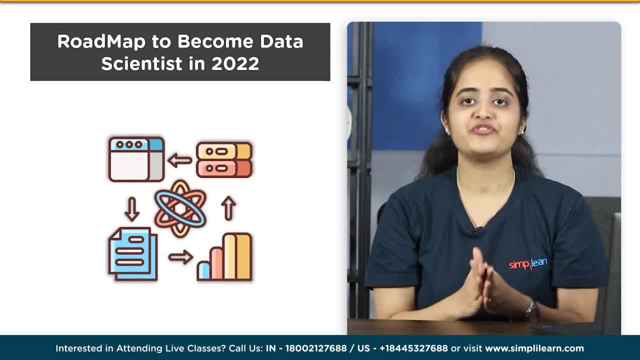 and every 40 minutes by 2021. the responsibility of a data scientist is to gather, clean and present data, and have a keen business sense and analytical abilities. let us have a discussion about it in the upcoming slides. how can you become a data scientist as a beginner? I 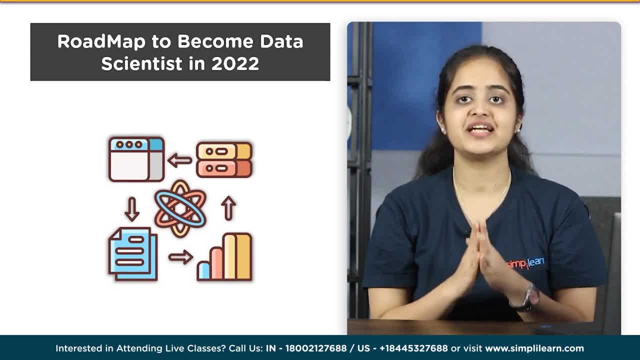 guarantee you, after watching this video, you will have a clear understanding on how to drive your career as a data scientist. hey guys, welcome to simply learn. before proceeding, please make sure you subscribe to simply learn's YouTube channel and press the bell icon to never miss any updates. 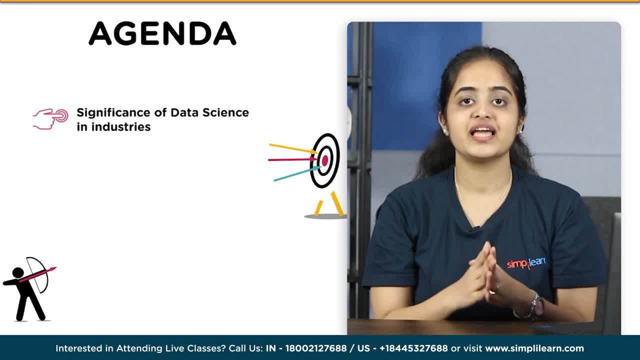 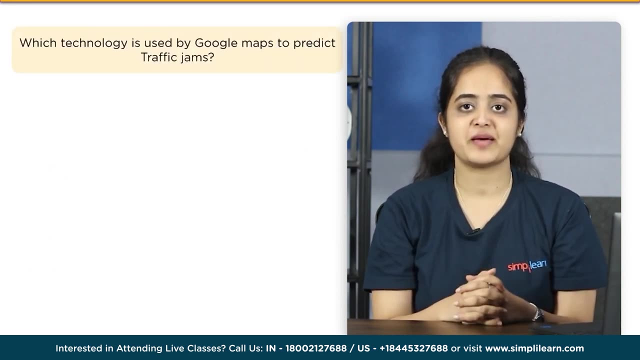 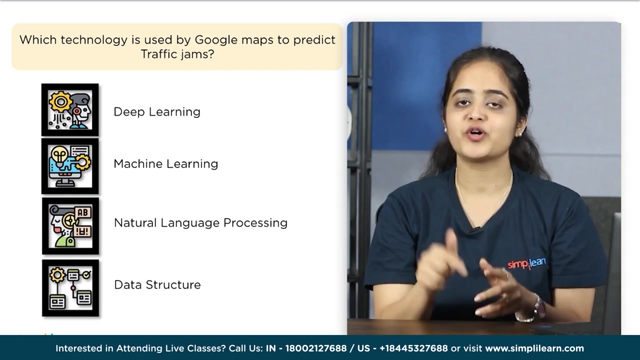 today we are going to cover significance of data scientists in Industries. after that, prerequisites and Technologies required for a data scientist and, finally, salary of a data scientist. I have a query for you: which technology is used by Google Maps to predict traffic jams? deep learning, machine learning, natural language, processing data structure? please leave the answer in the comment section. 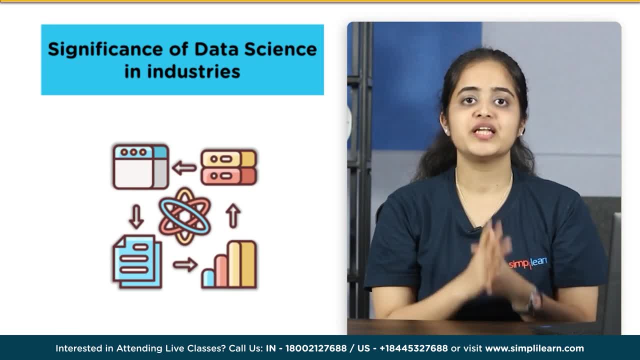 below and stay tuned to get the answer significance. now we will see how top Industries are involved in the field of data science. by 2025, the data science industry is anticipated to grow to a value of 16 billion dollars. there is an abundance of data science jobs. 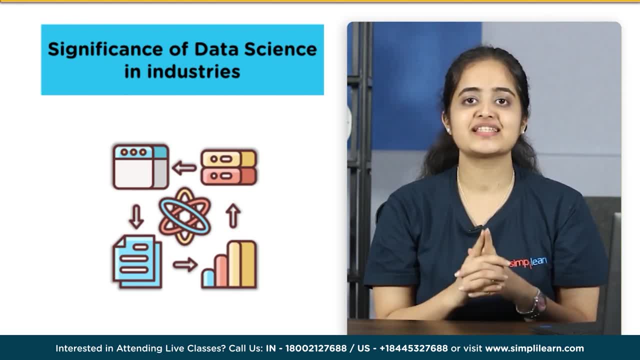 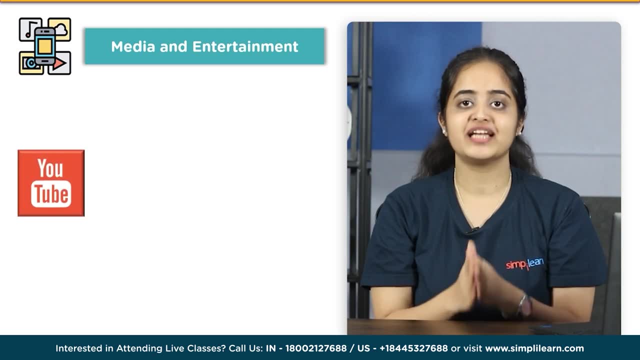 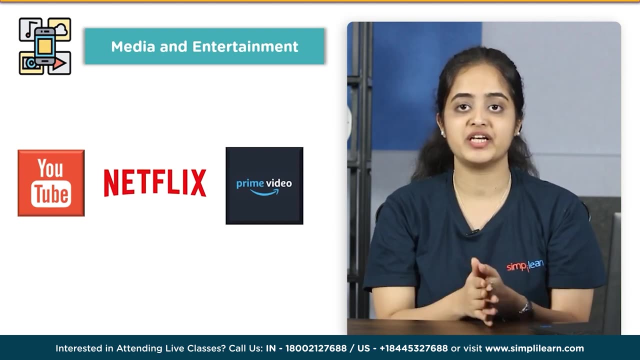 all over the world. now let's list out crucial areas where data science is used: media and entertainment: the major player in the media and entertainment sector, such as YouTube, Netflix, hot star, Etc. have begun to use data science to better understand their audience and provide them with recommendations. 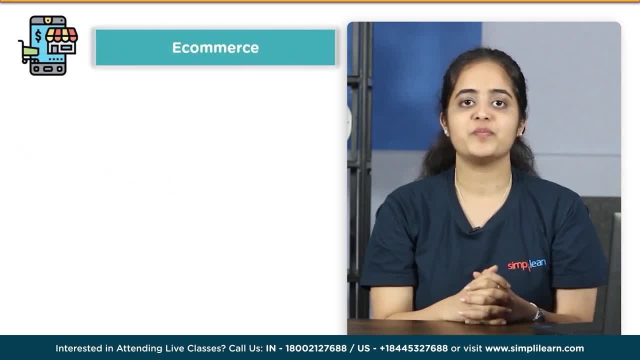 that are both relevant and personalized. e-commerce data science has aided retail companies in better meeting their expectations, as they bring a unique combination of deep data knowledge, technology skills and statistical experience. data scientists are in high demand in the retail industry. top recruiters are Amazon, Flipkart, Walmart, Myntra, Etc. digital marketing. 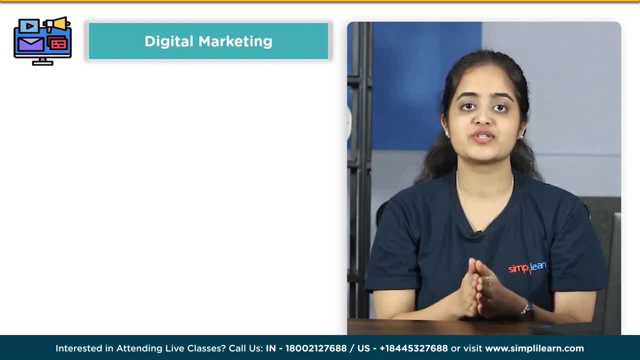 large volumes of data are currently being fetched from its users through search pages, social networks, online traffic display networks, movies, web pages, Etc. a high level of business intelligence is needed to analyze such large amount of data, and this can only be done with the proper use of data science approaches. top recruiters are 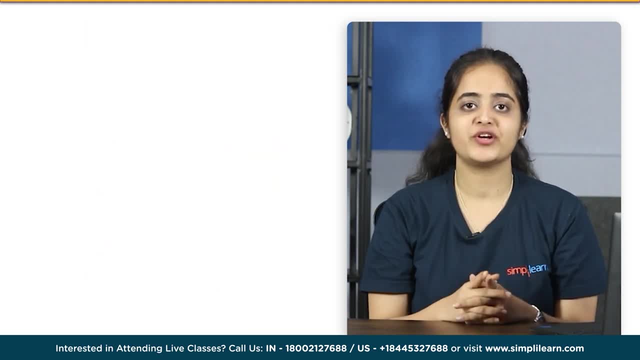 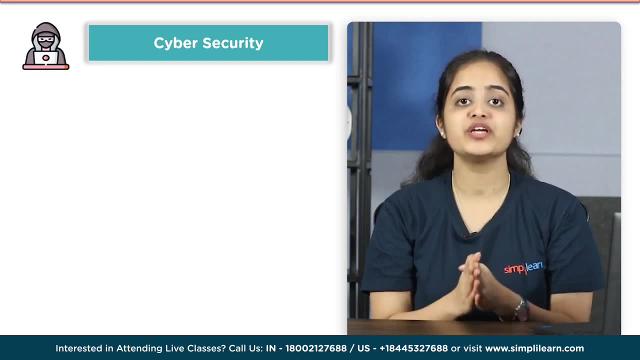 Amazon, Flipkart, Facebook, Google, Etc. cyber security, data science and AI are now being used by the cyber security industry to prevent the growing usage of algorithms for harmful purposes. top recruiters includes IBM, Microsoft, Accenture, Cisco and many more. before moving forward, what is the response to the Google map question? 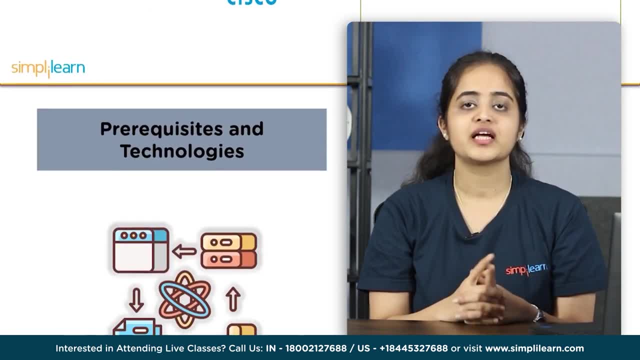 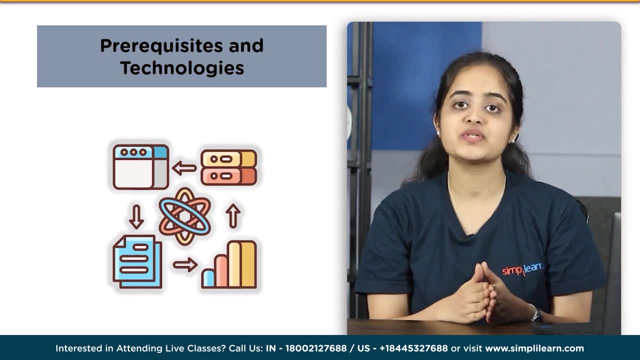 that I asked. answer: is machine learning coming to prerequisites? now that we know significance of data science in Industries, let us explore the prerequisites and Technologies required for a data scientist. seeing the demand of data scientists in every industry, it is obvious that the scope of a data scientist is very high. so how to start? there is no necessity that you should be knowing any. 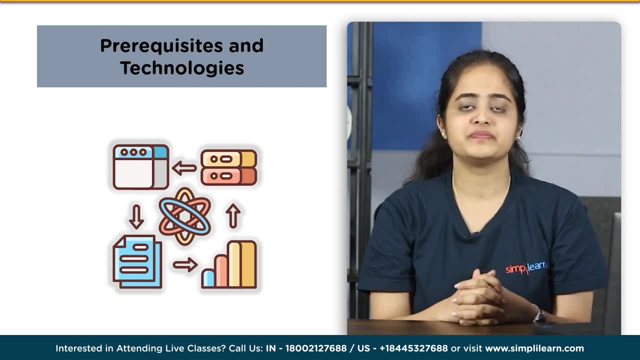 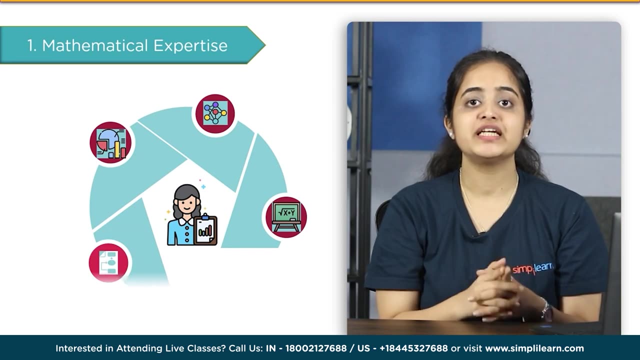 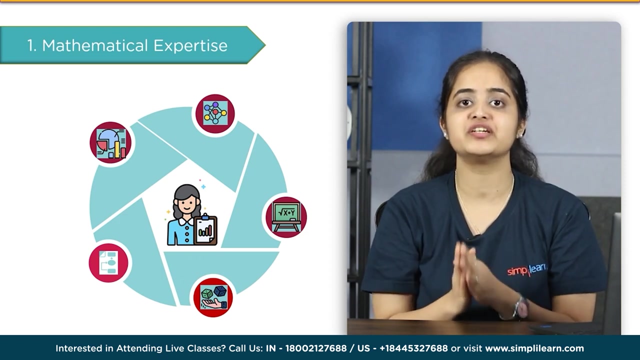 technology or programming language. you can be a layman too. data scientists typically have a variety of educational and professional experiences. most should be proficient in four crucial areas. important skill is mathematical expertise. three concepts like linear algebra, multivariable calculus and optimization technique are crucial because they aid in our understanding of numerous machine learning algorithms that are crucial to 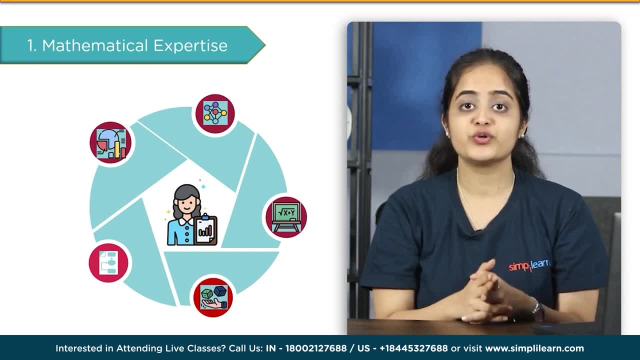 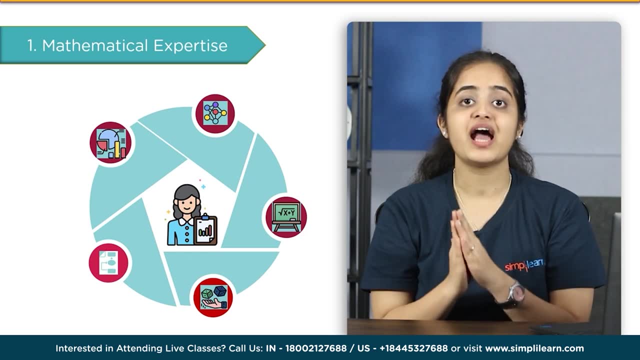 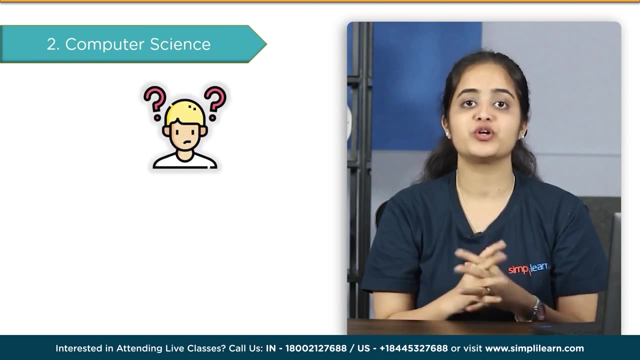 data science similar to that. knowing statistics is crucial because they are used in data analysis. additionally important to statistics, probability is regarded as a must offer. mastering machine learning. next is computer science. in the field of computer science, there is a lot to learn, but one of the key inquiries that arises in relation to programming is R or python language. there are 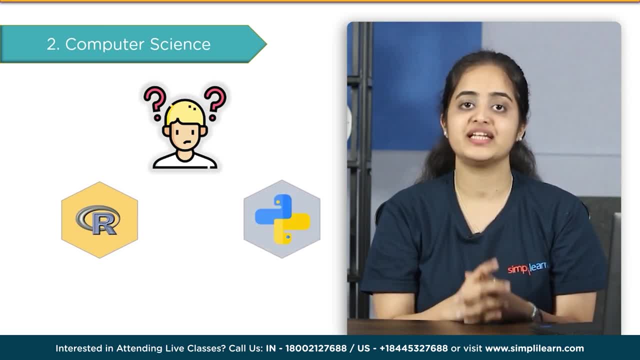 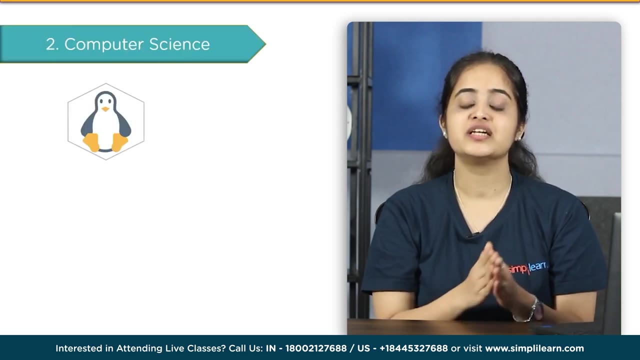 many factors to consider when deciding which language to choose for data science, because both have a comprehensive collection of libraries to implement complex machine learning algorithms. in addition to learning a programming language, you should learn the following computer science skill: fundamentals of algorithm and data structures. distributed computing, machine learning- deep. 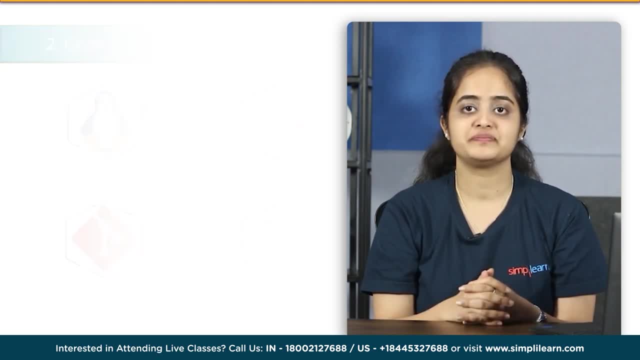 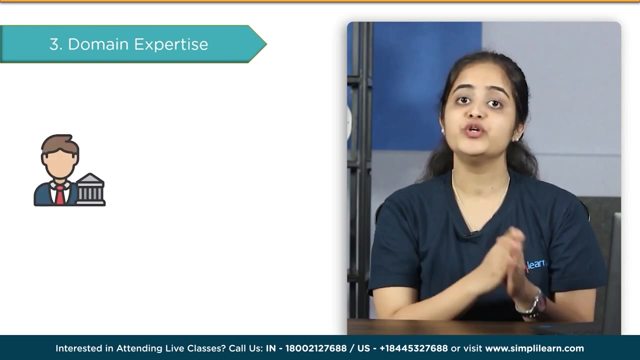 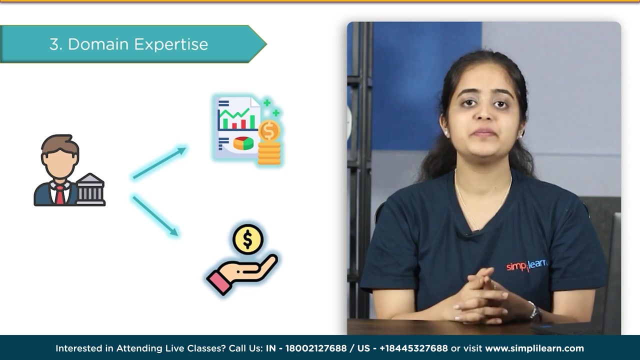 learning, Linux, SQL, MongoDB, Etc. domain expertise. most individuals strongly believe that domain expertise is not crucial to data science, yet it is. consider the following scenario: if you are interested in working as a data scientist in a banking Industries and you already know a lot about it- for instance, you are knowledgeable about stock trading, Finance, Etc. this will be very advantages. 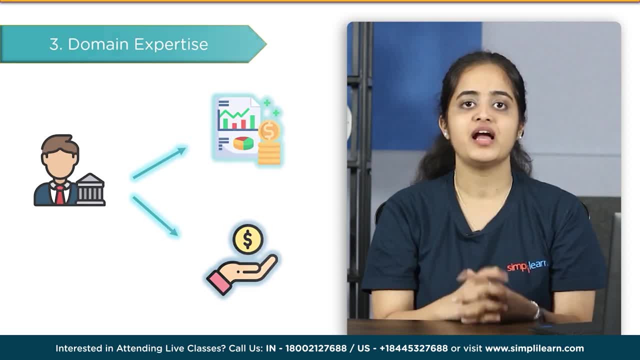 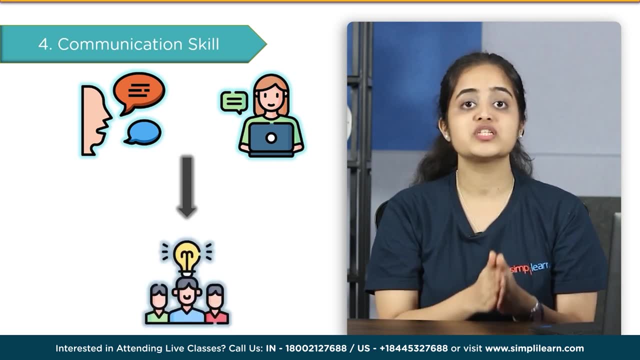 for you and the bank itself will favor you over other applicants. and finally, communication skill. it covers both spoken and written communication in a data science project. the project must be explained to others when finding from the analysis have been reached. this can occasionally be a report that you provide to your team or employer at work. sometimes it might be a blog entry. it is frequently. 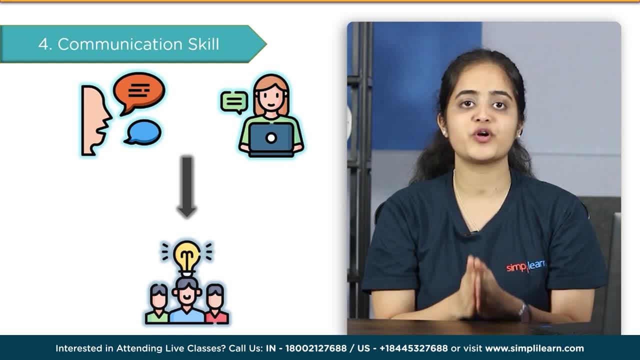 a presentation to a group of co-workers. regardless, a data science project always involves some form of communication of the project's findings. therefore, having a good communication skill is a requirement for being a data scientist. apart from all this, practicing is very important. keep using different tools. also, start reading blocks on data science. start building projects on data science. 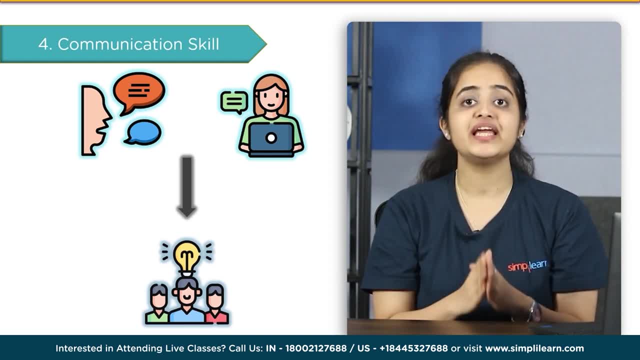 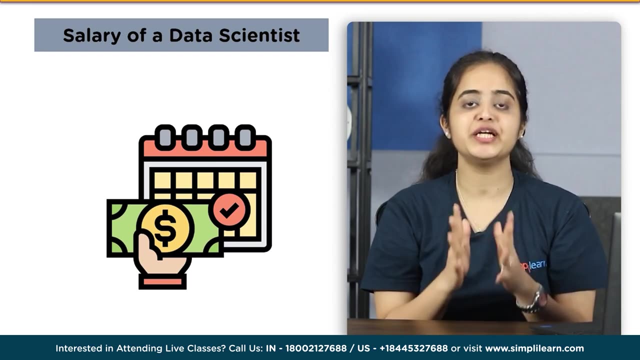 which can be added to your resume. also, you can find many interesting courses on data science by yourself. salary reward is the result of good work. now we shall discuss salaries that a data scientist will get. it should come as no surprise that data scientists may add significantly to a business. 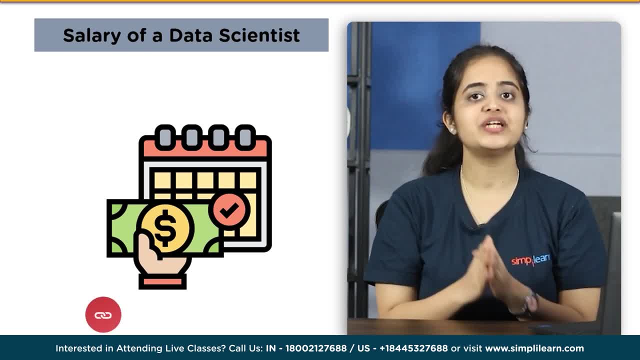 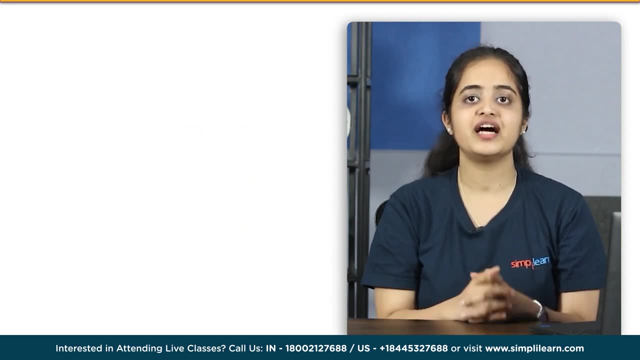 every step of the process, from data processing to data cleansing, requires persistence, a lot of arithmetic and statistics, as well as scattering of engineering skills. one of the most important factors in a data scientist salary is experience at the beginner level. a data scientist can make ninety five thousand dollars annually, the typical annual compensation for a 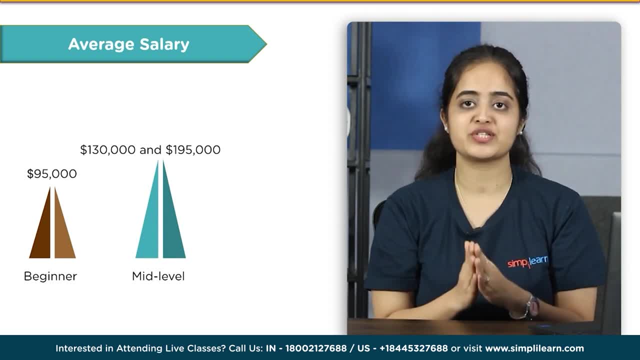 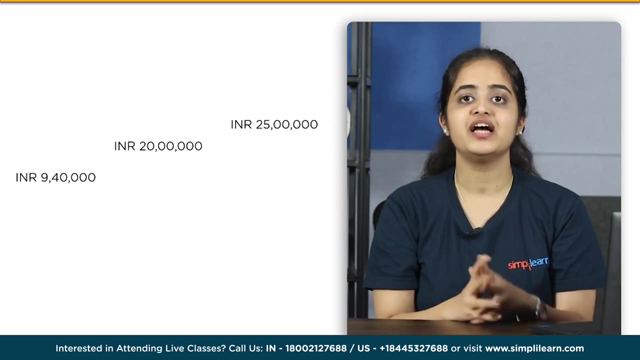 mid-level data scientist is between one hundred thirty thousand dollars and one ninety five thousand dollars. a seasoned data scientist typically earns between one sixty five thousand dollars and two hundred fifty thousand dollars per year. in India, at the beginner level, a data scientist can make nine lakh forty thousand rupees on average per year. at mid-level data. 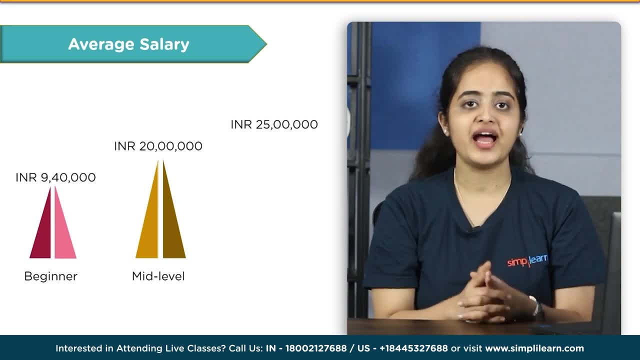 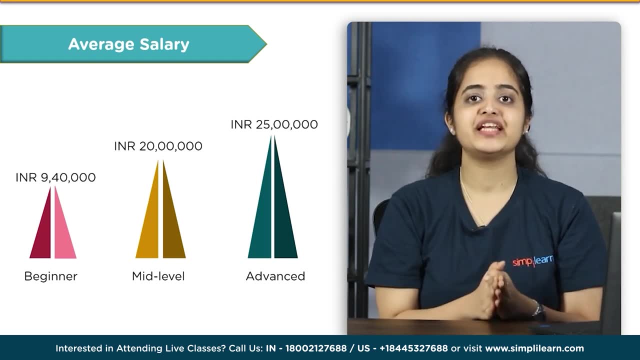 scientist will get twenty lakhs rupees per annum, and if you are at the advanced level, you will get paid an average of rupees twenty five lakhs annually. this salary will vary in different countries. the top hiring businesses in the US that provide the highest salaries for data scientist are: 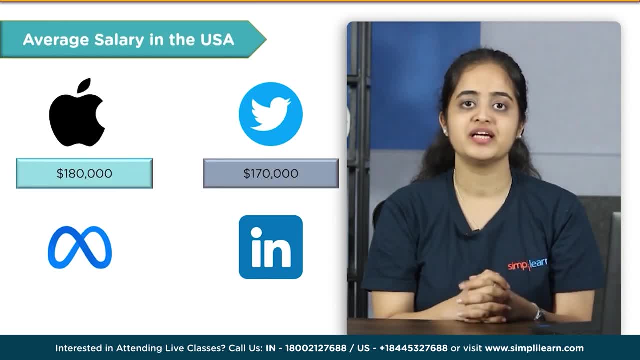 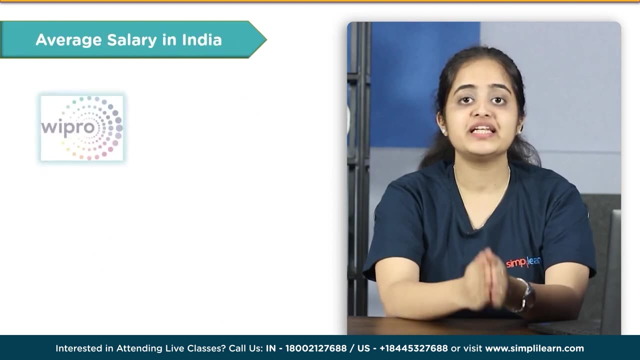 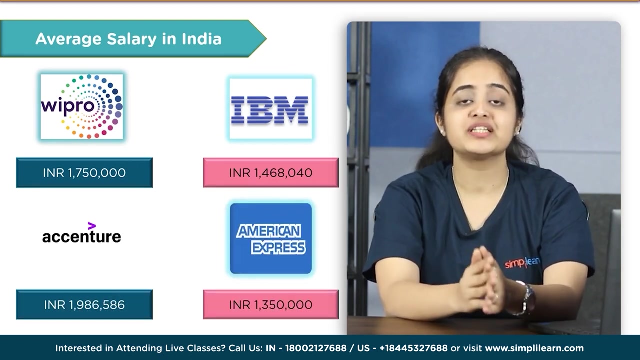 Apple, with one hundred eighty thousand dollars per annum. next is Twitter, with one hundred seventy thousand dollars per annum. Fipro technology provides 17 lakh fifty thousand per annum, IBM provides 14 lakhs per annum and Accenture will provide you with 19 lakhs per annum. and finally, 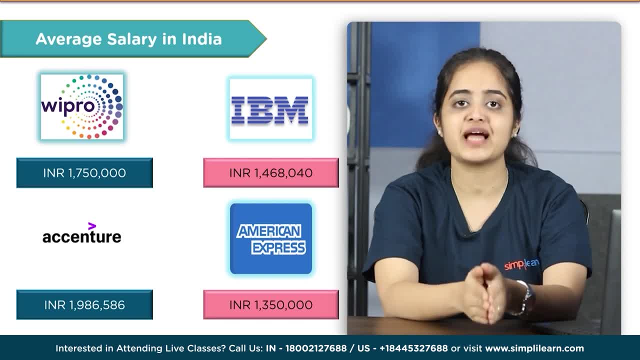 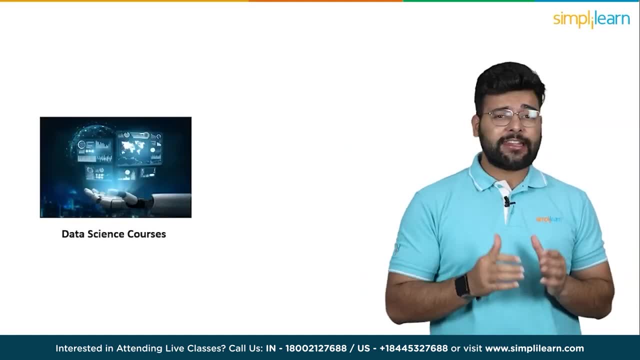 American Express will provide on average of 13 lakhs per annum. no matter if you are recently graduated, have experience in the IT field or are seeking a career change, these courses in data science will provide you with the necessary foundation to pursue a successful career in data. 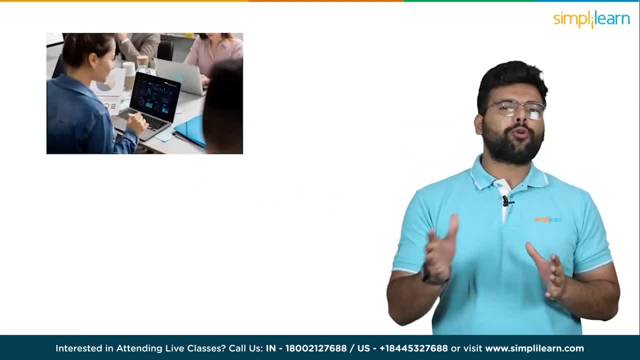 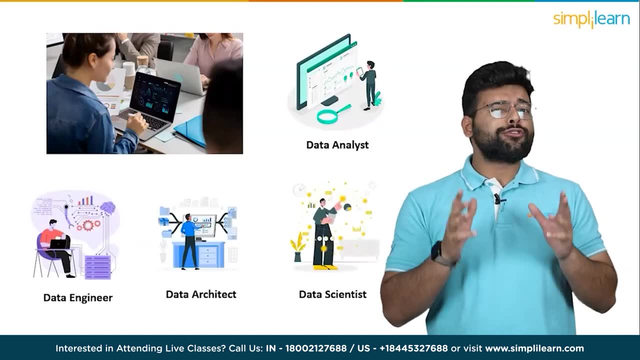 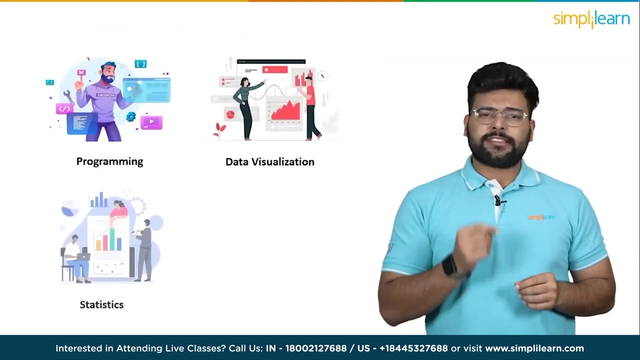 science. obtaining an education in data science can open doors to various job opportunities, such as data analyst, data engineer, data architect or data scientist. your specific path in data science will depend on your skills and interests. however, all these career paths require a certain level of proficiency in programming, data visualization, statistics and machine learning. data engineers: and data architects primarily work with coding databases and intricate queries, while data analysts and data scientists focus on analyzing, collecting and interpreting large data sets to aid in making informed business decisions. it is a rapidly expanding and financially rewarding career path, with data scientists reporting an average annual salary of 130 000 in the United. 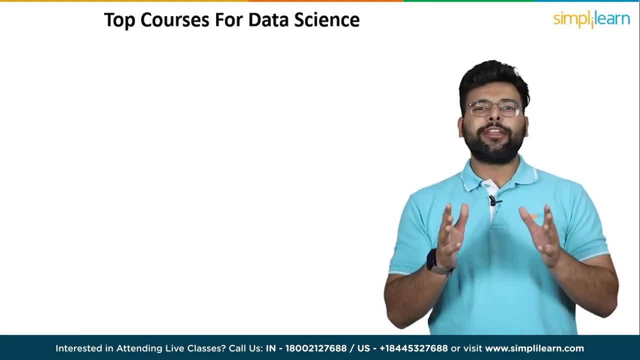 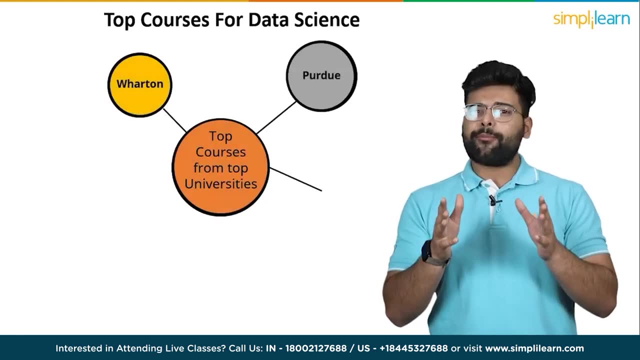 States and in India it is 12 lakhs per annum. in this simply learn video on top courses for data science, we will explore some of the top courses in data science, including Wharton, Purdue IT, Kanpur, Caltech and SPJMIR. these courses are at the forefront of data science education and research. 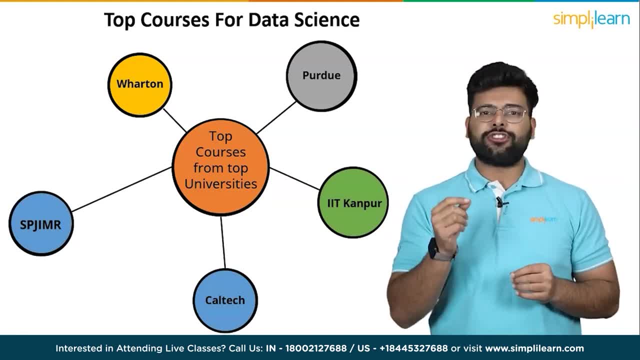 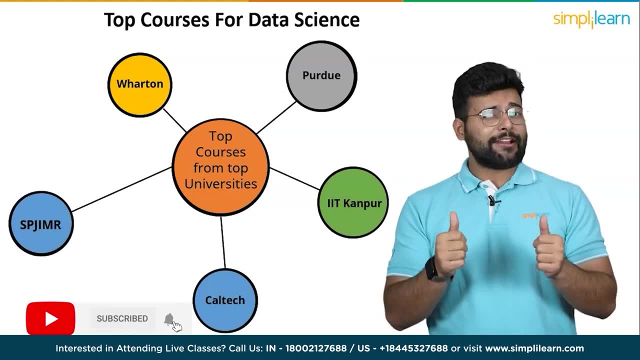 their programs are designed to equip students with the skills and knowledge needed to succeed in this exciting and rapidly evolving field. but before moving ahead, do subscribe to our YouTube channel and hit the bell icon to get all the updates from simply learn. so let's get started. first one on the list is Caltech, the California 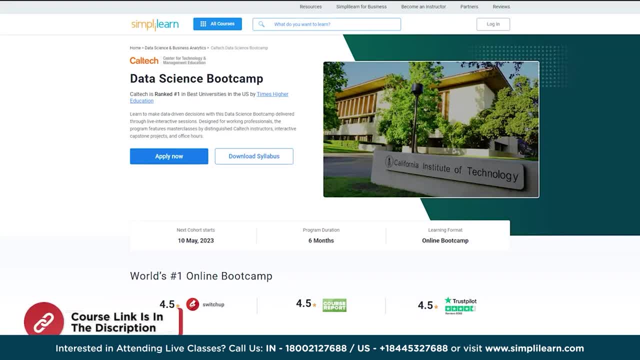 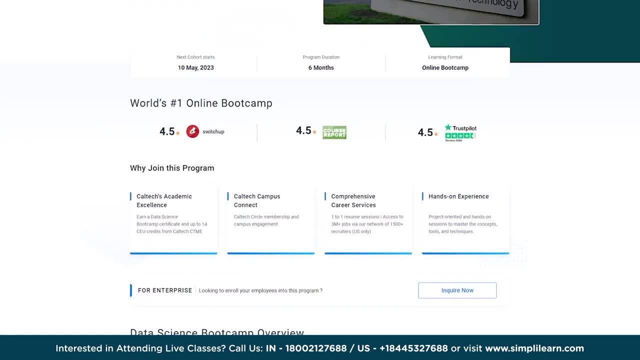 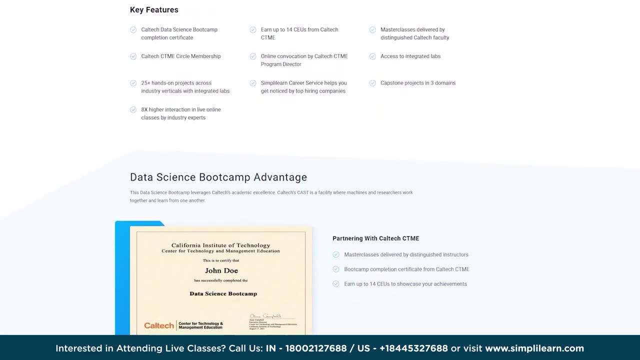 Institute of Technology, known as Caltech, is a private research University in Pasadena, California. the university's division of engineering and applied sciences over data science courses. this data science course curriculum emphasizes hands-on learning and encourage students to explore projects that have real world applications. that's why simply learn has collaborated with. 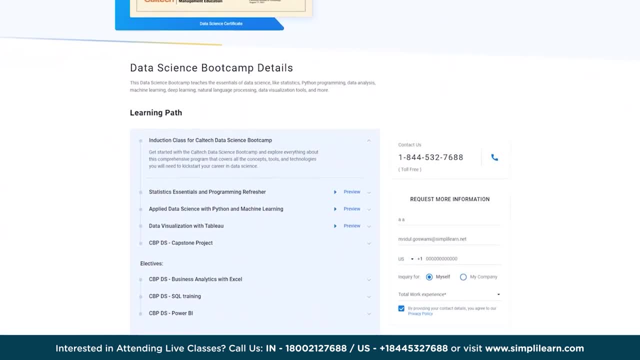 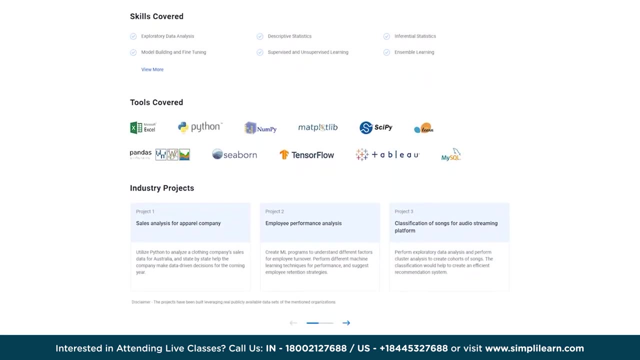 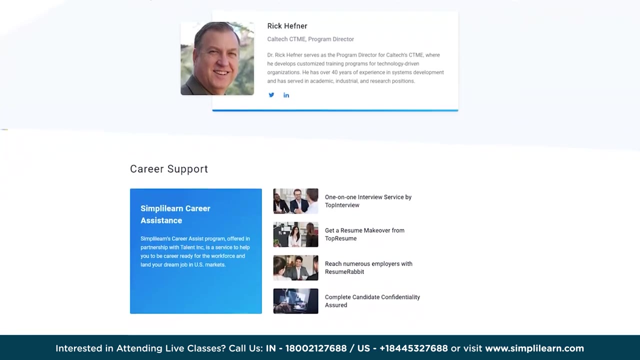 Caltech to create a data science course that leverages the superiority of Caltech's academic minions. this data science course course critical data science topics like python programming, R programming, machine learning, deep learning and data visualization tools through an interactive learning model with live sessions by Global practitioners and practical labs. this course 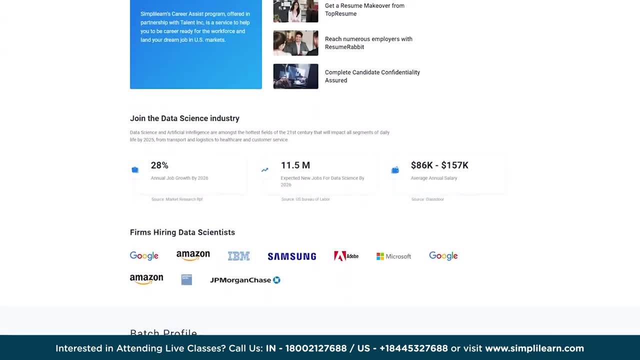 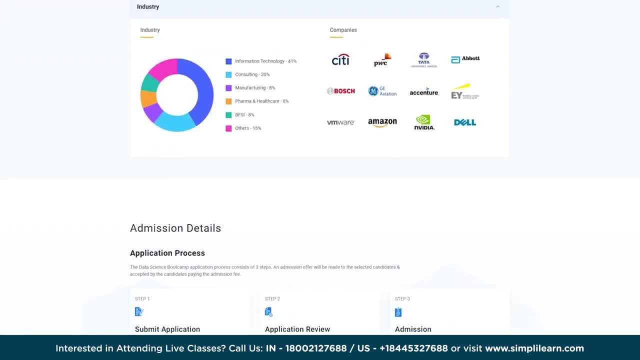 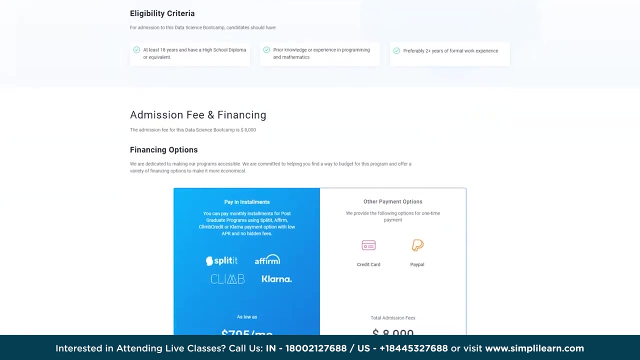 also provides a program certificate with up to 14 cu credits from Caltech CTME and a course completion. we will also earn membership to the Caltech CTME circle and an online convocation by the Caltech program director. and, last but not least, thanks on experience with tools like numpy, pandas, R python and 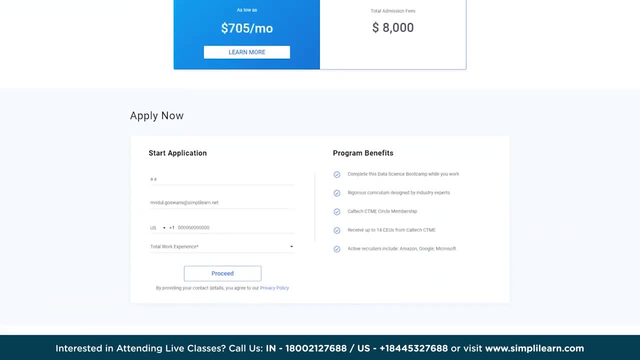 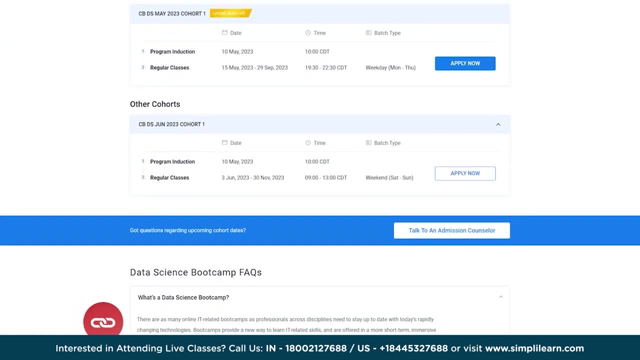 sci-fi, with 25 plus industrial element projects from the likes of Walmart, Amazon, Uber, Mercedes Benz and many more. interested in this course, then do check out the link to this course in the description. the second one on the list is Purdue University. Purdue is a public research University. 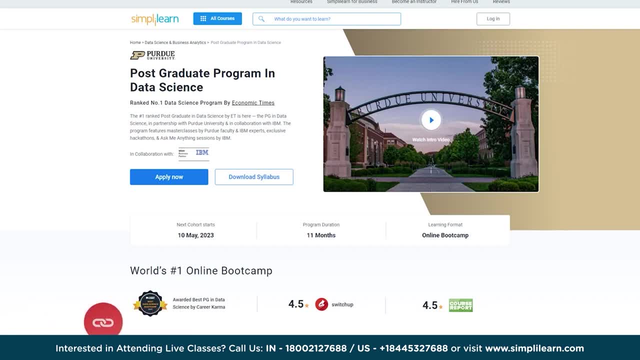 in Atlanta. the university's Department of computer science offers a data science program covering data mining, machine learning and statistical modeling. well with simpliness, postgraduate program in data science in partnership with Purdue University and in collaboration with IPM. you can have the opportunity to take the advantage of master classes by Purdue faculty and IBM experts. 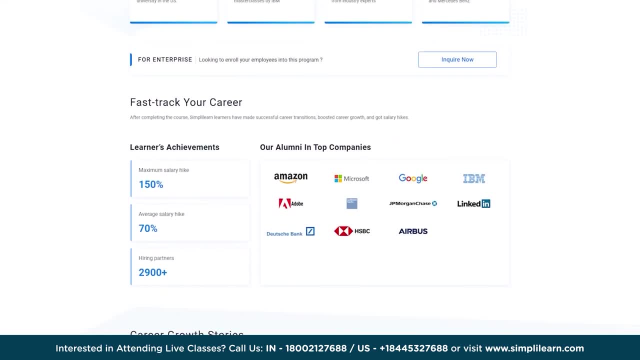 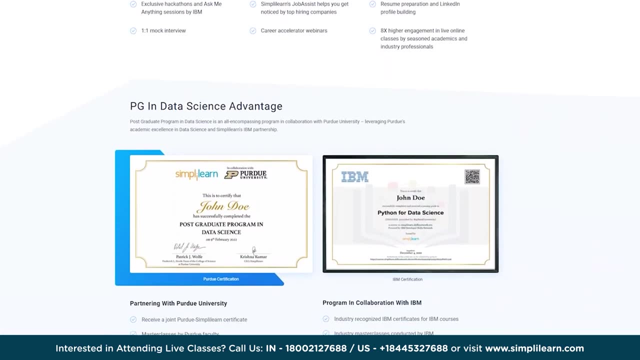 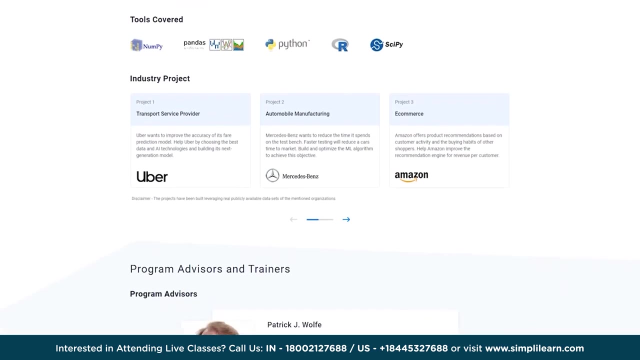 exclusive hackathons and ask me anything- sessions by IBM. this program in data science is perfect for working professionals and it focuses on essential job skills like R and python programming, machine learning, NLP and data visualization with tableau to prepare for the job market. you will learn all this through live sessions with experts, hands-on labs, IBM hackathons and corporate projects. 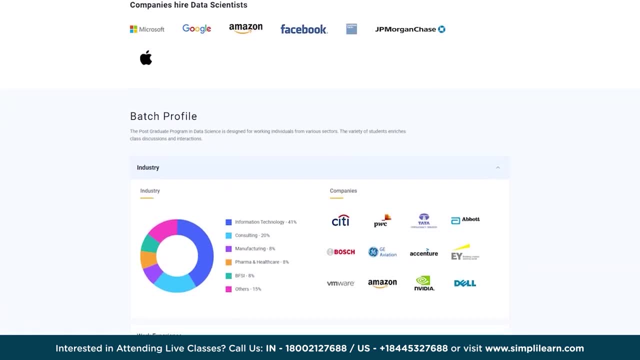 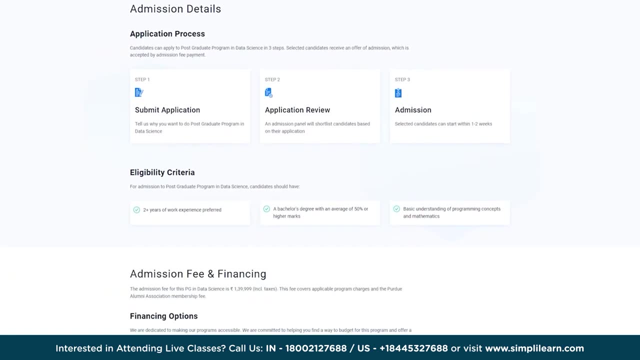 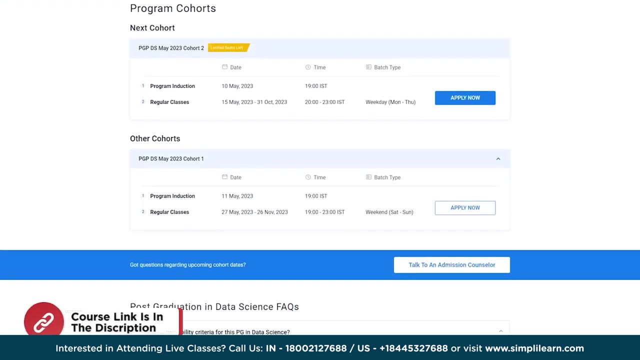 this course will also provide you with the data science certificate from Purdue, the eighth most innovative University in the US, along with IBM certificates from IBM courses. with this, you will also get a chance to build your resume and prepare your interviews with valuable insights from industry experts and 25 plus industry relevant projects from Amazon, Walmart, Uber and Mercedes. 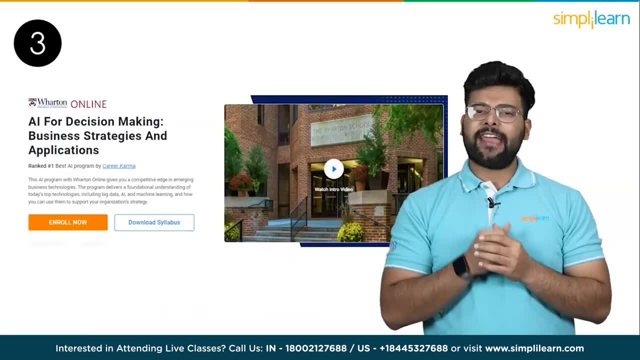 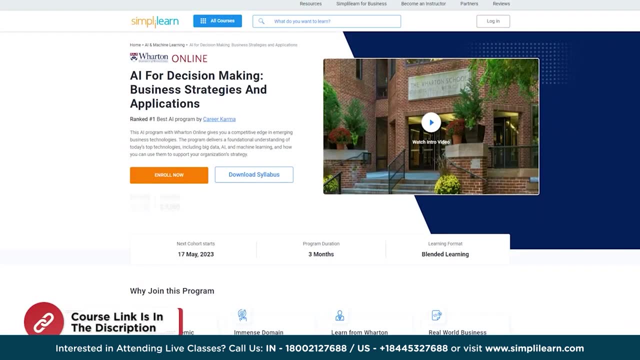 Mercedes-Benz- you can find a link to this course in the description box- and the third one, Warton. Warton is a global technology company that has been a leader in the data science field for decades. in addition to offering a range of data science solutions and tools, Wharton also provides: 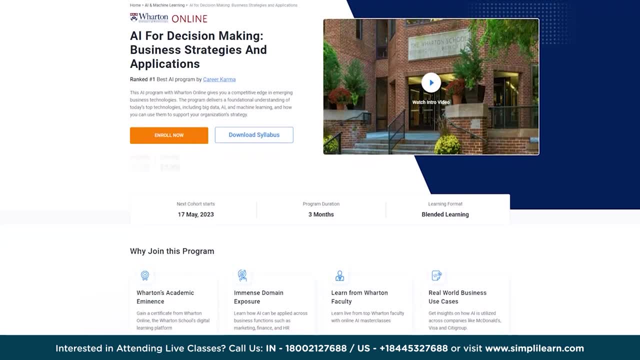 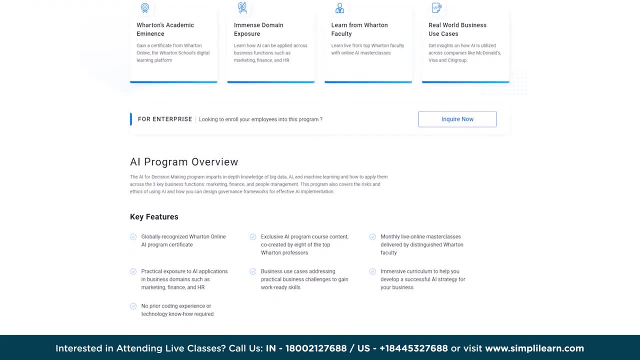 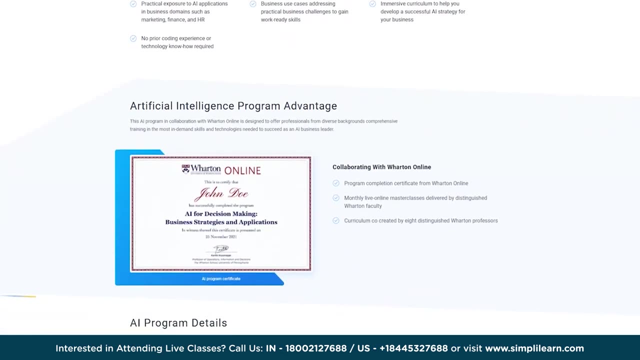 training and education in data science. this AI program, in collaboration with Wharton, impacts in-depth knowledge of big data, AI and machine learning and how to apply them across the three key business functions: marketing, finance and people management. this program also covers the risks and ethics using AI and how you can design governance frameworks for effective AI implementation. 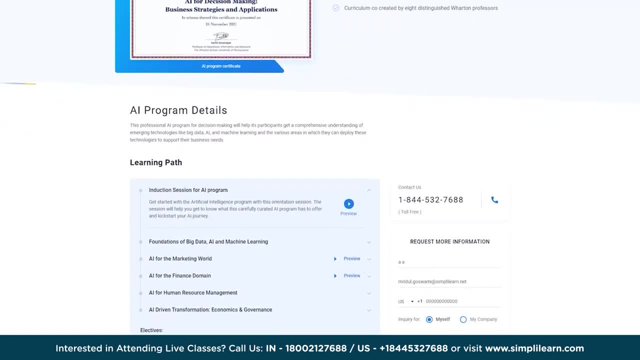 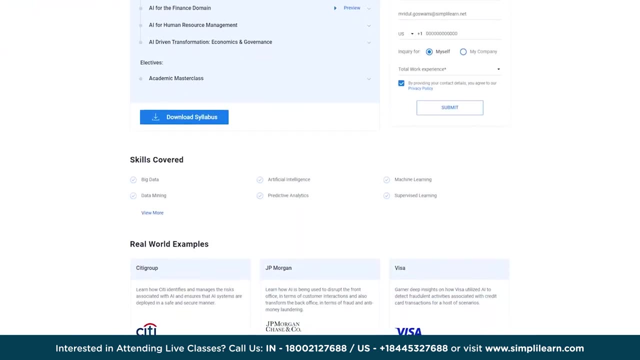 apart from this, you will get a certificate from Wharton online, the Wharton school's digital learning platform, and you will learn how AI can be applied across business functions such as marketing, finance, HR, and you will also be having live master classes from top Wharton faculty and. 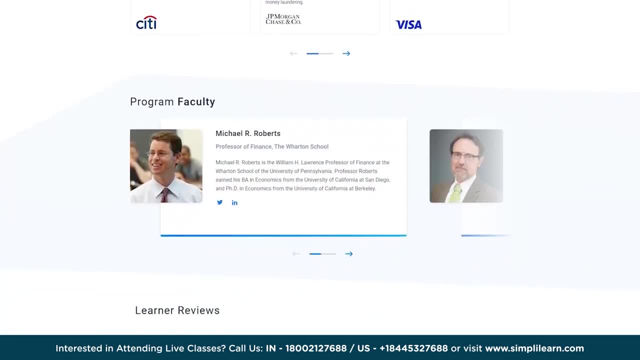 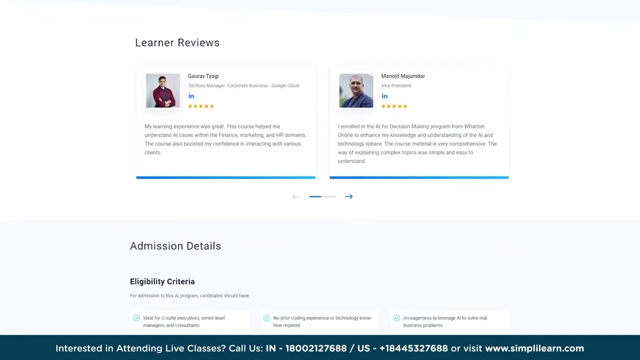 get insights on how AI is utilized across companies like McDonald's, Visa and Citigroup. this program is designed to equip students with the skills and knowledge needed to succeed in this fast-growing field and become a data scientist by diving deep into the nuances of data interpretation mastering. 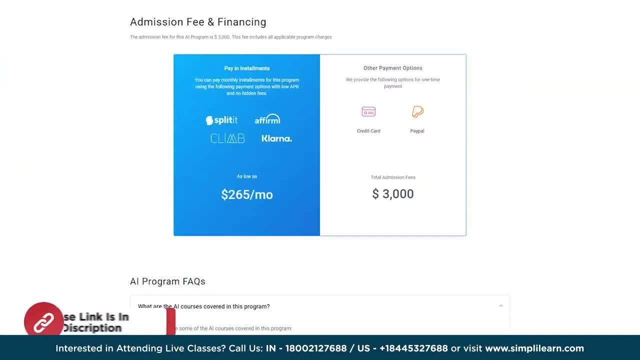 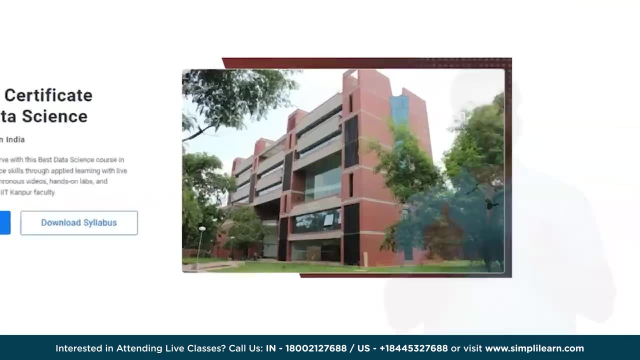 Technologies like machine learning and mastering powerful programming skills to take your career in data science to the next level. also, the link for this course is mentioned in the description box. following that, we have IIT Kanpur, the Indian Institute of Technology Kanpur is one of the top. 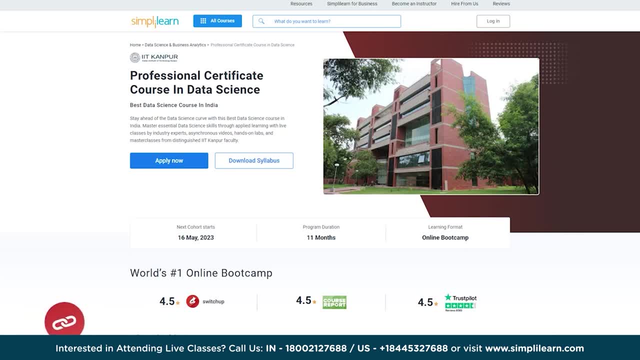 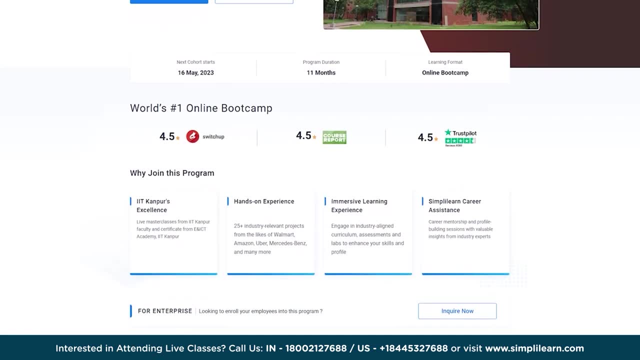 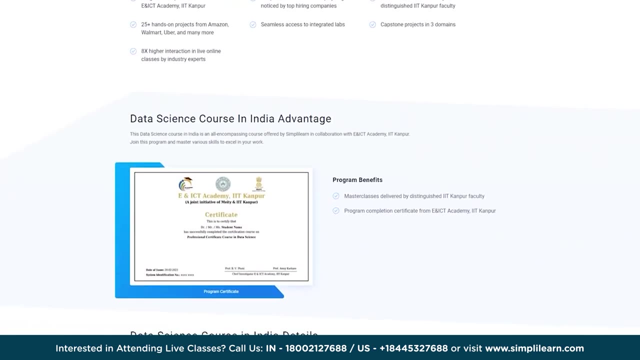 engineering schools in India, known for its strong focus on research and Innovation. the Institute's Department of computer science and engineering is one of the most popular universities offering data science. taking advantage of such resourceful alumni simply learn. provides a professional certificate course in data science in collaboration with IIT Kanpur, mastering essential data science. 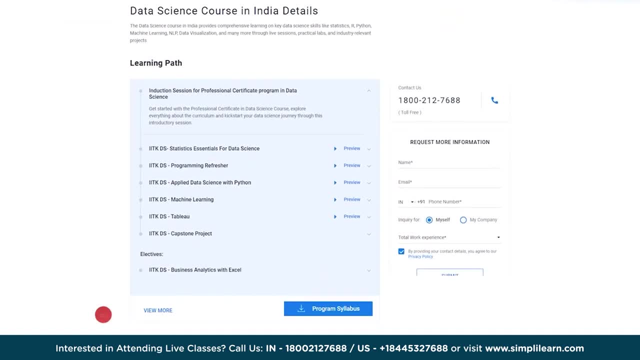 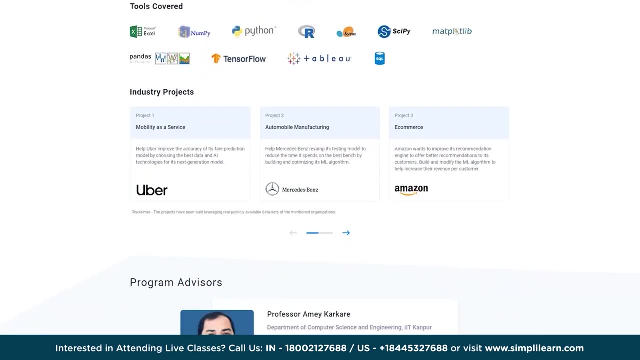 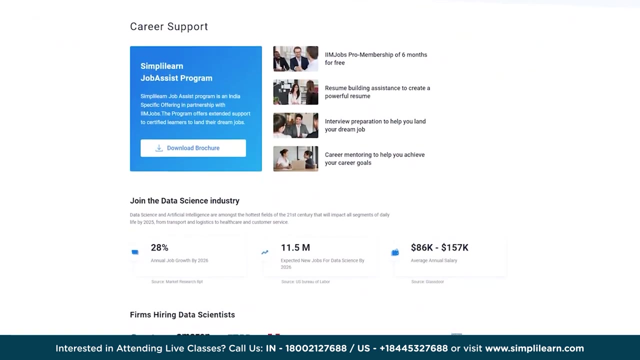 skills through applied learning with live classes, industry experts, asynchronous videos, hands-on labs and master classes from distinguished IIT Kanpur faculty. along with that, you will get hands-on experience on 25 plus industry relevant projects from the likes of Walmart, Amazon, Uber, Mercedes Benz and many more, along with career mentorship and profile building sessions with valuable insights from. 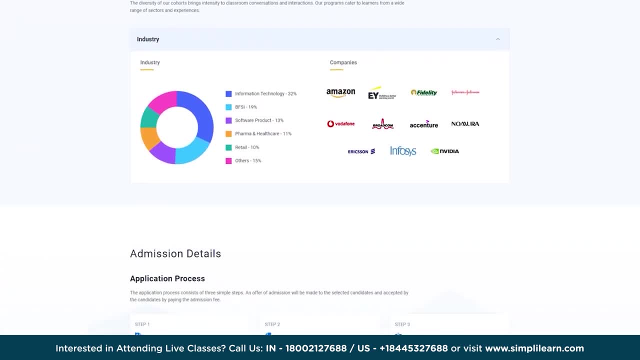 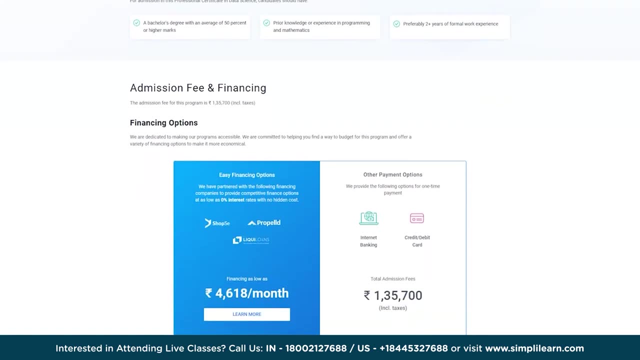 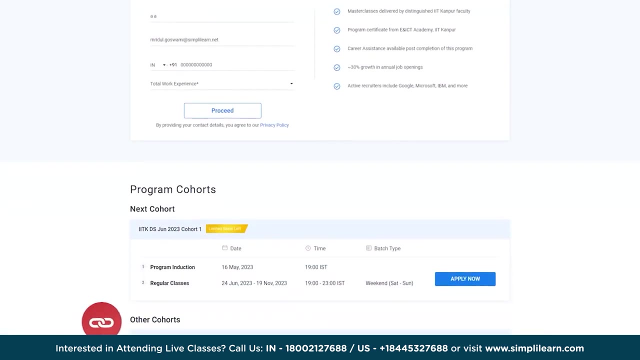 data experts. this course is designed with a carefully curated curriculum that includes critical topics like python, machine learning, NLP and data visualization, delivered using hands-on labs and industry relevant projects to help you advance your career trajectory. this data science course in India aims to domestic data science. the link is mentioned in the description box and the 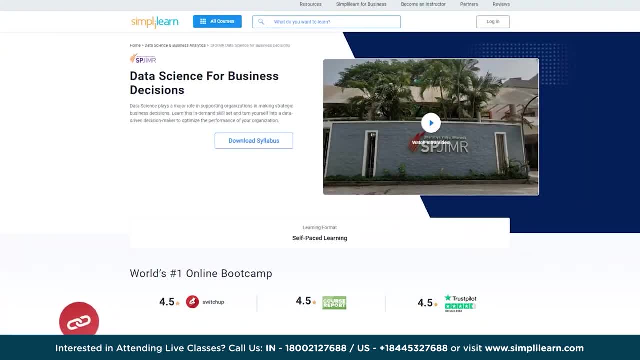 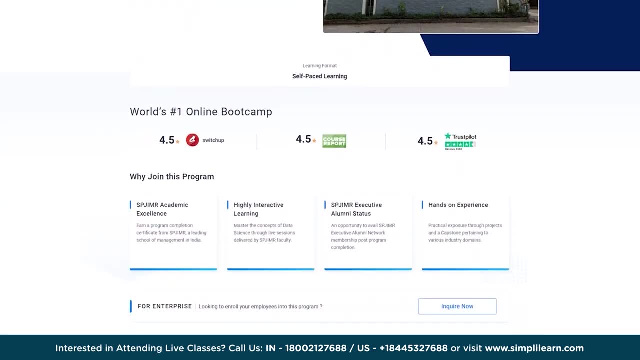 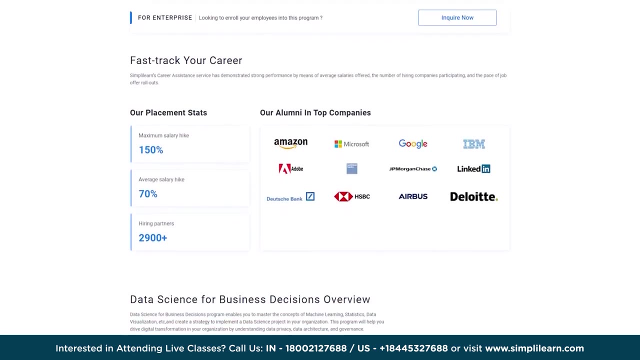 last one is spjmir. spjn Institute of management and research is a leading business schools located in Mumbai, India. the Institute's business intelligence and analytics program is designed to provide a strong foundation in data science, analytics and business intelligence. therefore, simply learn has collaborated with spgmir to design the data science for business decisions program. that will help you. 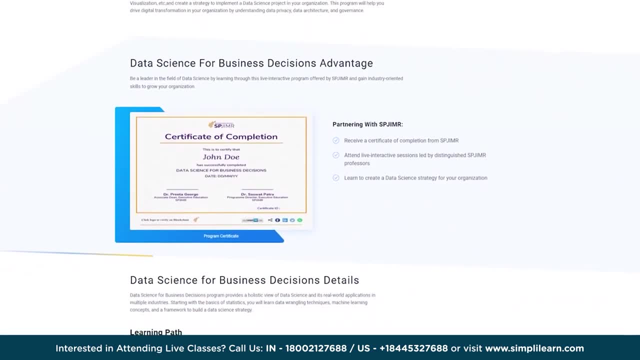 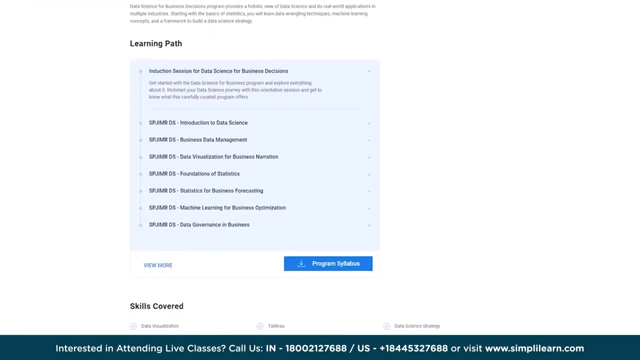 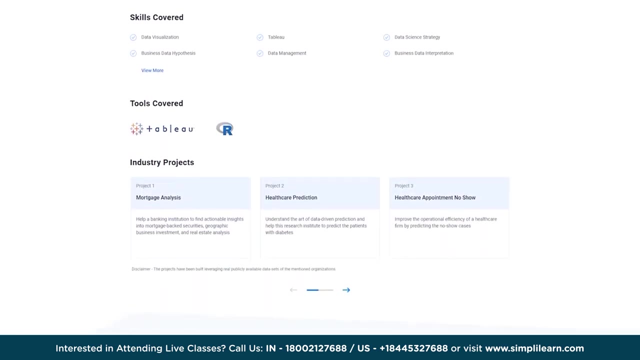 learn this in-demand skill set and turn yourself into a data-driven decision maker to optimize your organization's performance. this program enables you to master the concepts of machine learning, statistics, data visualization, Etc. and create a strategy to implement a data science project in your organization. this program will help you drive digital transformation in your 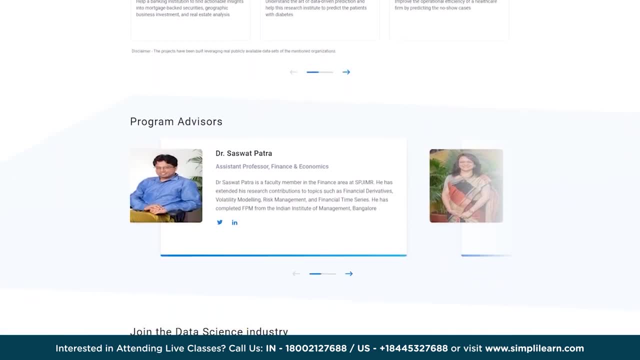 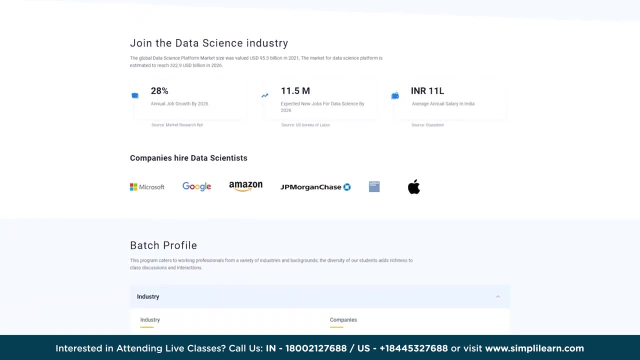 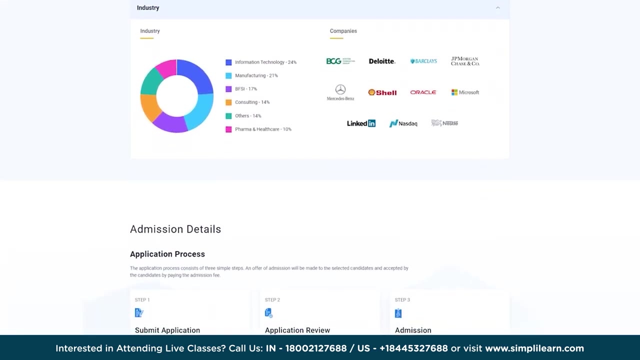 organization by understanding data privacy, data architecture and governance. you will also earn a program completion certification from spgmir, a leading school of management in India, and master the concept of data science through live sessions delivered by spgmir faculty. you will also bag an opportunity to avail of spgmir executive alumni Network membership post program completion. hence. 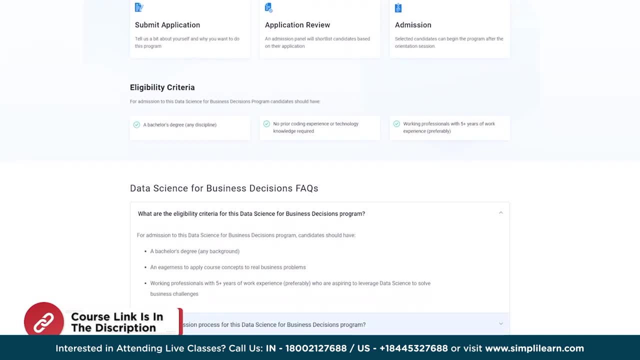 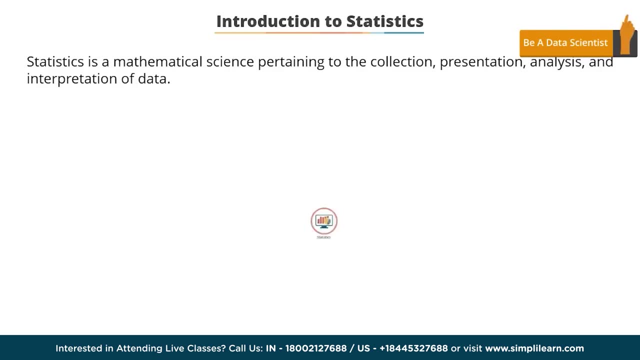 an experience on multiple projects and a capstone pertaining to various industry domains. the link is mentioned below in the description. let's begin this lesson by using the term statistics. statistics is a mathematical science pertaining to the collection, presentation, analysis and interpretation of data. it's widely used to understand the complex 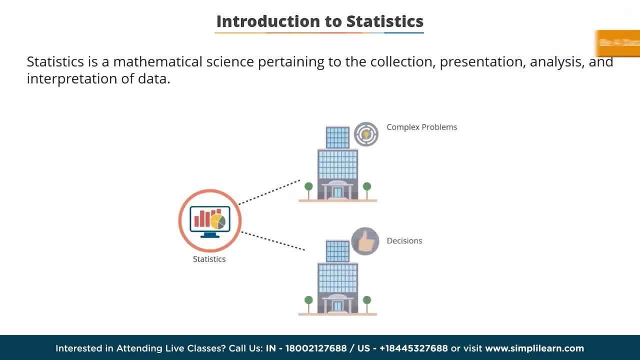 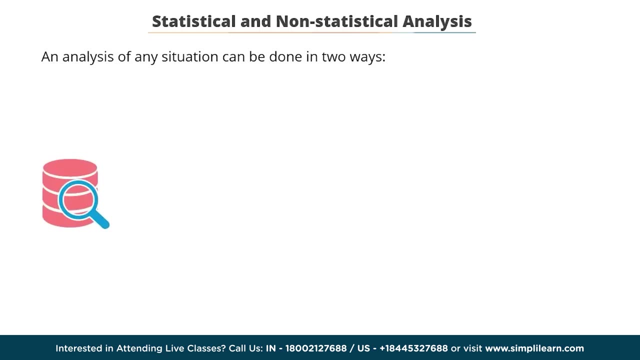 problems of the real world and simplify them to make well-informed decisions. several statistical principles, functions and algorithms can be used to analyze primary data, build a statistical model and predict the outcomes. an analysis of any situation done in two ways: statistical analysis or a non statistical analysis. statistical- 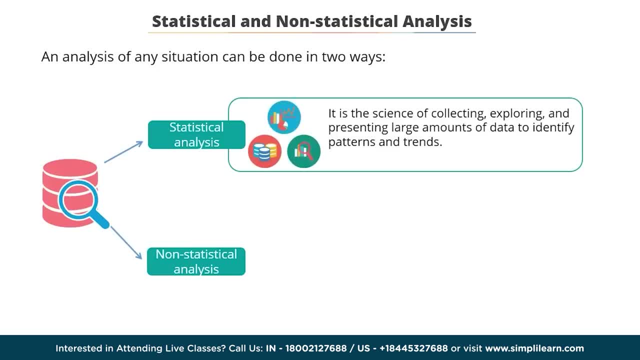 analysis is the science of collecting, exploring and presenting large amounts of data to identify the patterns and trends. statistical analysis is also called quantitative analysis. non statistical analysis provides generic information and includes text, sound still images and moving images. non statistical analysis is also called qualitative analysis. although both forms 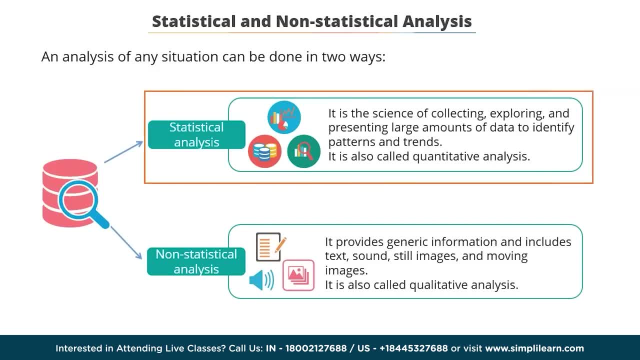 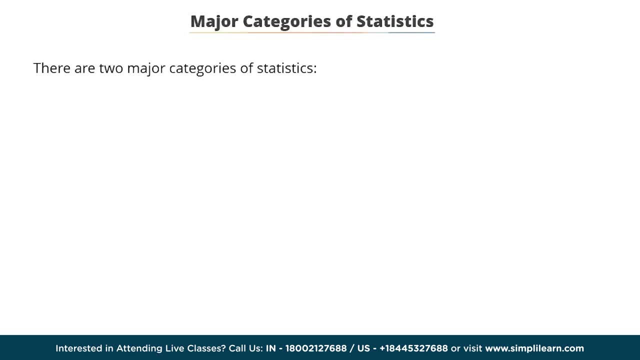 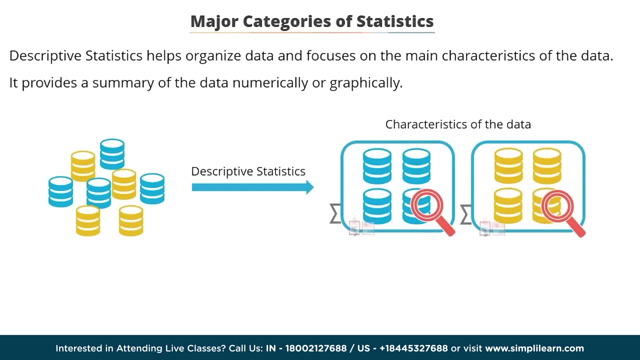 of analysis provide results. statistical analysis gives more insight and a clearer picture, a feature that makes it vital for businesses. there are two major categories of statistics: descriptive statistics and inferential statistics. descriptive statistics helps organize data and focuses on the main characteristics of the data. it provides a summary of the data numerically. 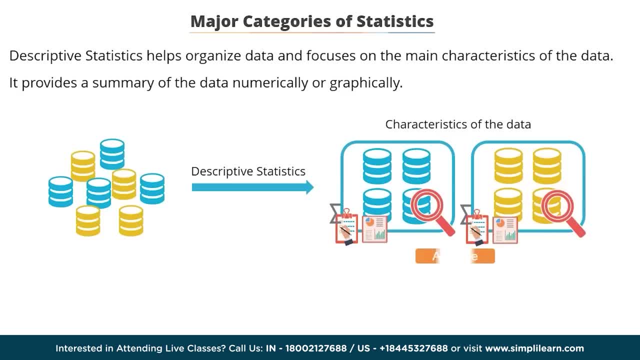 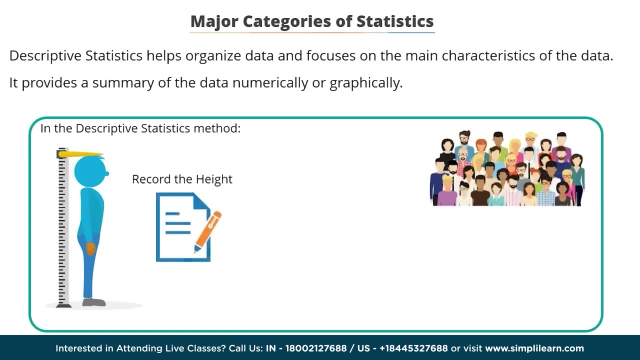 or graphically. numerical measures such as average mode, standard deviation or SD, and correlation are used to describe the features of a data set. suppose you want to study the height of students in a classroom. in the descriptive statistics you would record the height of every person in the classroom and then find. 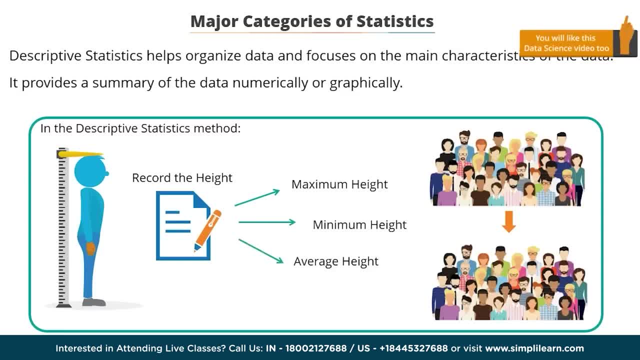 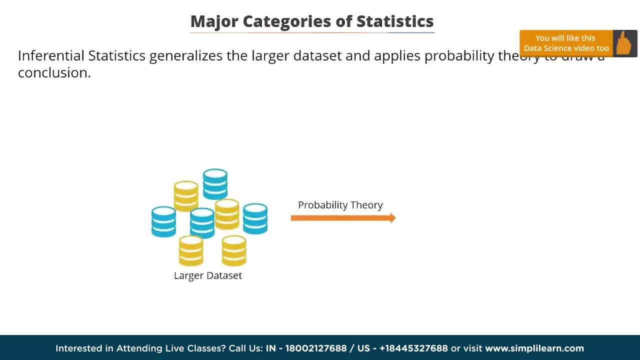 out the maximum height, minimum height and average height of the population. inferential statistics generalizes the larger data set and applies probability theory. to draw a conclusion, it allows you to infer population parameters based on the sample statistics and to model relationships within the data. modeling allows you to develop mathematical equations which describe the inner 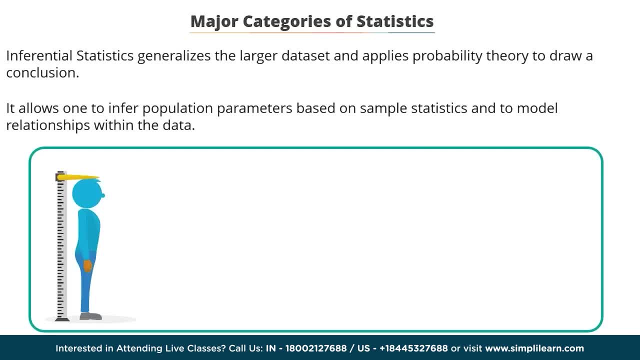 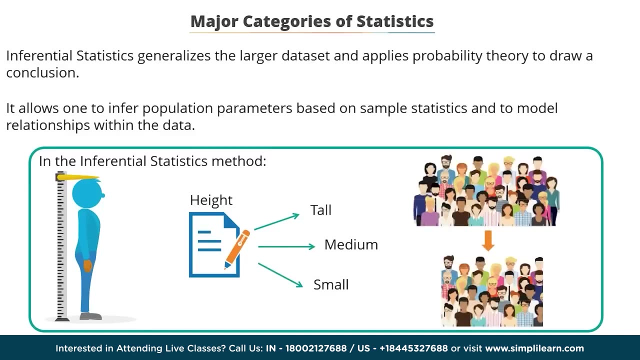 relationships between two or more variables. consider the same example of calculating the height of students in the classroom. in inferential statistics you would categorize height as tall, medium and small and then take only a small sample from the population to study the height of students in the classroom. the field of statistics. 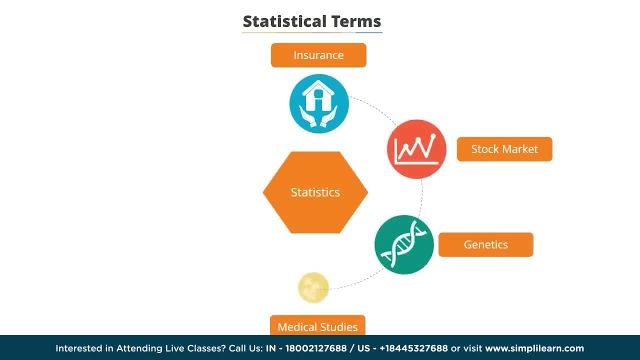 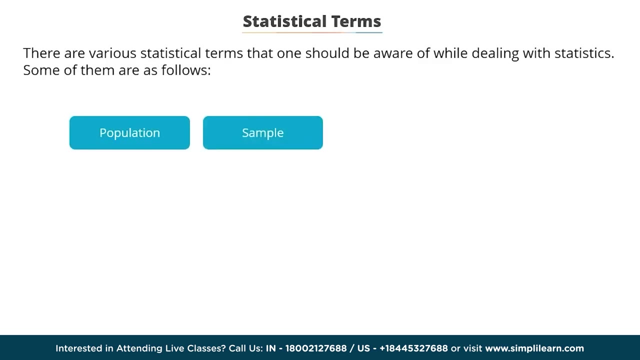 touches our lives in many ways, from the daily routines in our homes to the business of making the greatest cities run, the effect of statistics are everywhere. there are various statistical terms that one should be aware of while dealing with statistics: population sample variable, quantitative variable, qualitative variable, discrete variable, continuous variable. 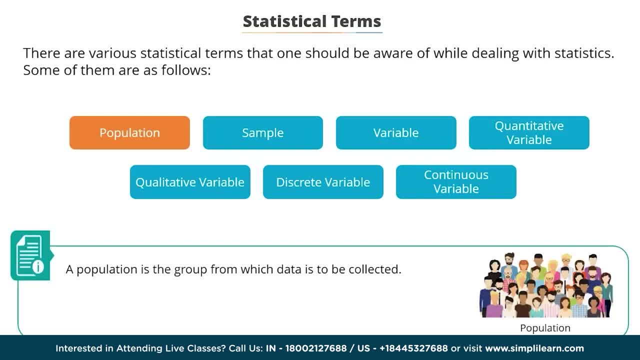 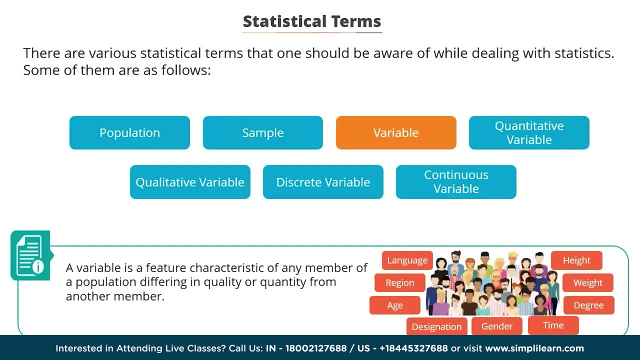 a population is the group from which data is to be collected. a sample is a subset of a population. a variable is a feature that is characteristic of any member of the population, differing in quality or quantity from another member. a variable differing in quantity is called a quantitative variable. for example, the 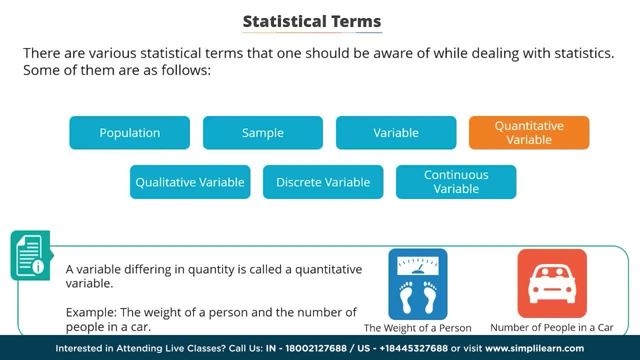 weight of a person, number of people in a car. a variable differing in quality is called a qualitative variable or attribute, for example color, the degree of damage of a car in an accident. a discrete variable is one which no value can be assumed between the two given values, for example the number of 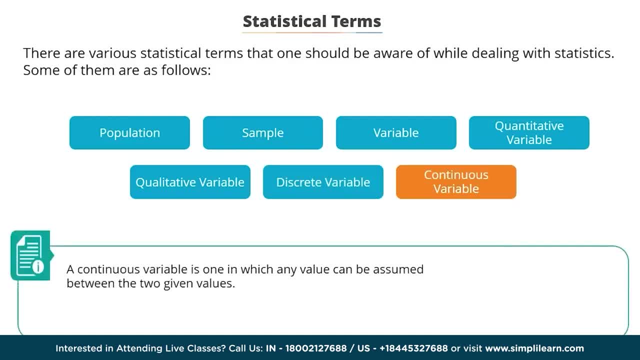 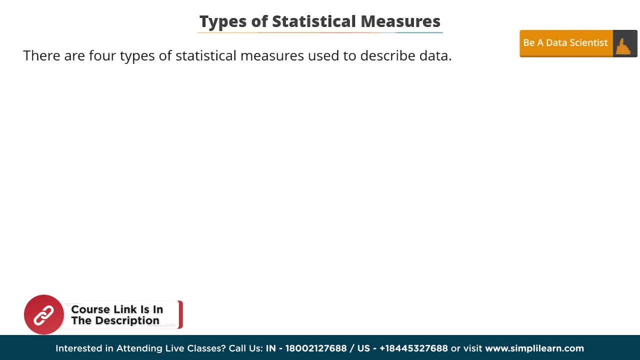 children in a family. a continuous variable is one in which any value can be assumed between the two given values, for example, the time taken for a 100 meter run. typically, there are four types of statistical measures used to describe the data. they are: measures of frequency, measures of central tendency, measures of spread, measures of position. let's learn. 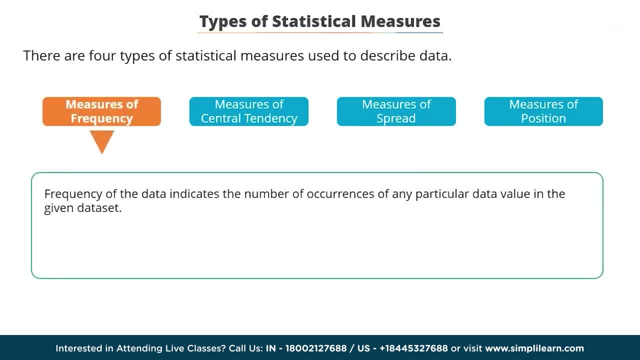 each in detail. frequency of the data indicates the number of times a particular data value occurs in the given data set. the measures of frequency are number and percentage. central tendency indicates whether the data values tend to accumulate in the middle of the distribution or toward the end. the measures of central tendency are mean, median and mode. spread describes: 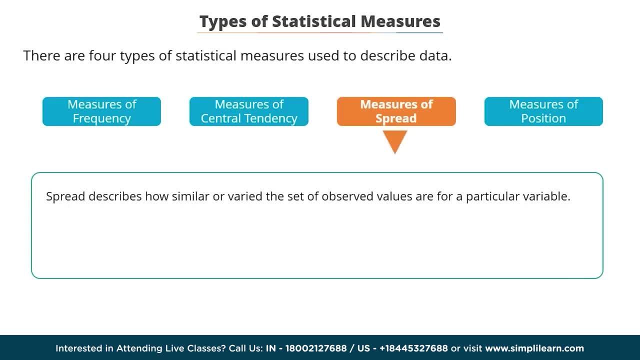 how similar or buried the set of observed values are for a particular variable. the measures of spread, our standard deviation, variance and quartiles. the measure of spread are also called measures of dispersion. position identifies the exact location of a particular data value in the given data set. the measures of position are percentiles. 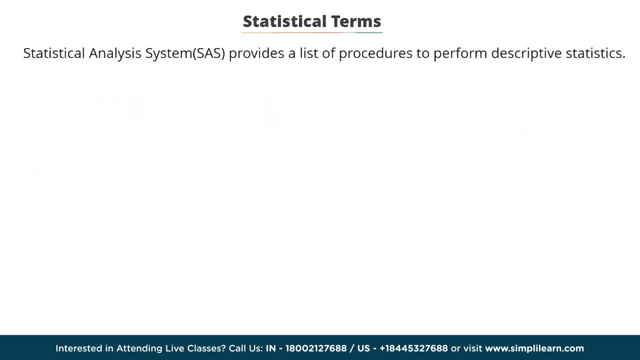 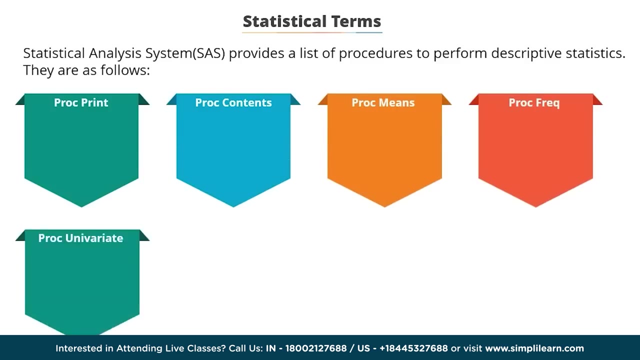 quartiles and standard scores. statistical analysis system, or SAS, provides a list of procedures to perform descriptive statistics. they are as follows: proc print proc contents. proc means proc frequency, proc univariate proc g chart, proc boxplot proc. gplot proc print. it prints all the variables in 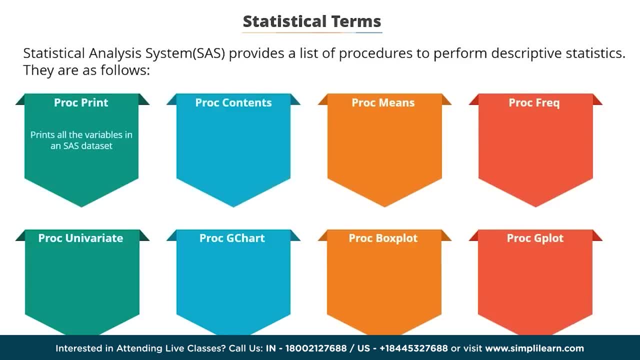 a SAS data set proc contents: it describes the structure of a data set proc means: it provides data summarization tools to compute descriptive statistics for variables across all observations and within the groups of observations. proc frequency: it produces one way to in way frequency and cross tabulation tables. frequencies can: 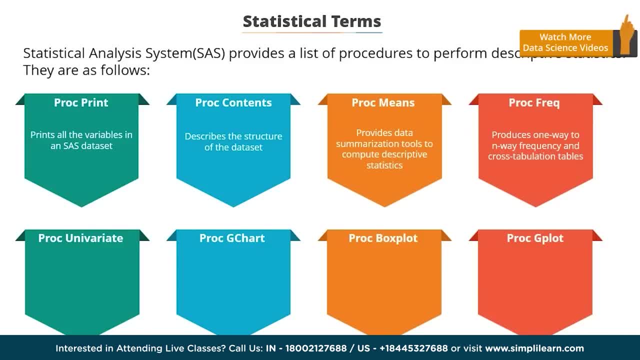 also be an output of a SAS data set, proc univariate. it goes beyond the problem. 덜пол proc gcharưởng. hight of k, t, s, k, p. can it windows, p, nd, nd, numeric or character PROC? BOXPLOT: The boxplot procedure creates side-by-side. 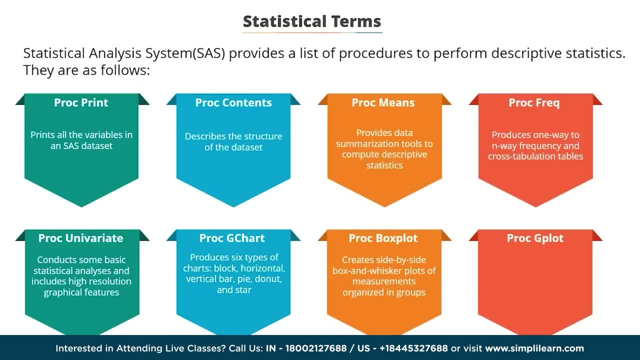 box-and-whisker plots of measurements organized in groups. A box-and-whisker plot displays the mean, quartiles and minimum and maximum observations for a group. PROC GPLOT- Gplot procedure creates two-dimensional graphs including simple scatterplots. overlay plots in which multiple sets of data points are. 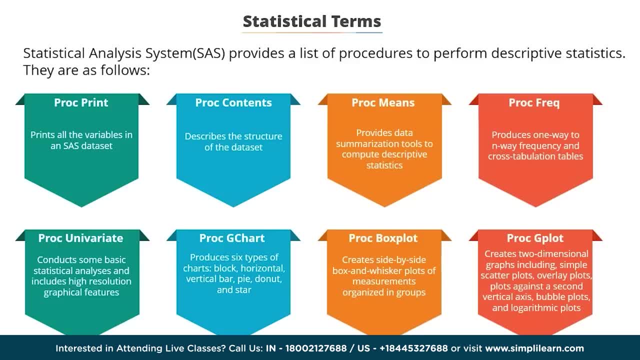 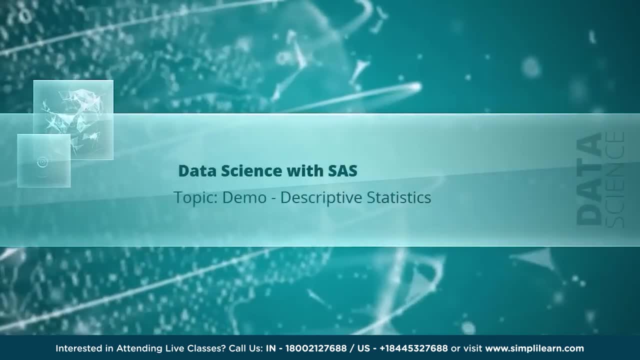 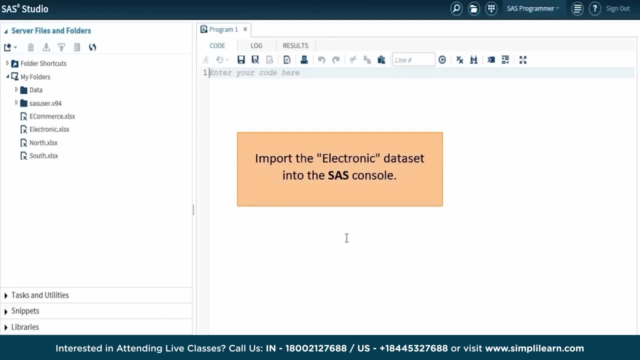 displayed on one set of axes plots against a second vertical axis, bubble plots and logarithmic plots. In this demo you'll learn how to use descriptive statistics to analyze the mean from the electronic dataset. Let's import the electronic dataset into the SAS console. 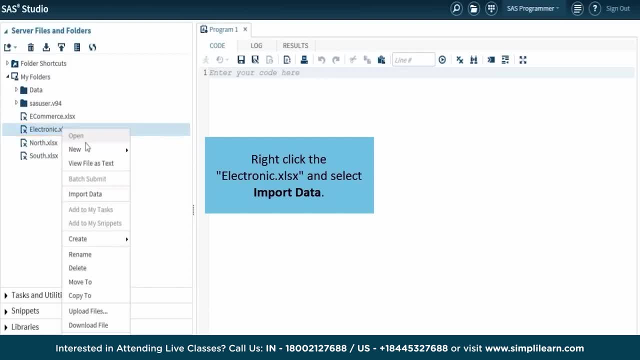 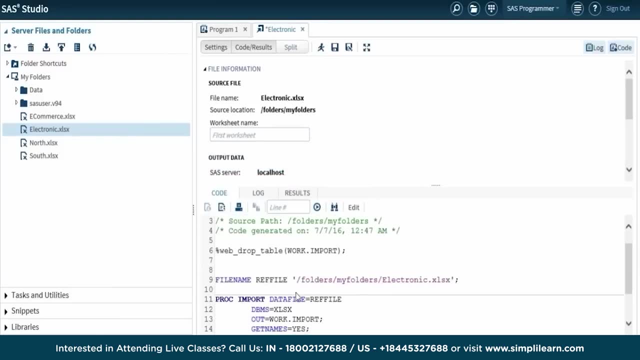 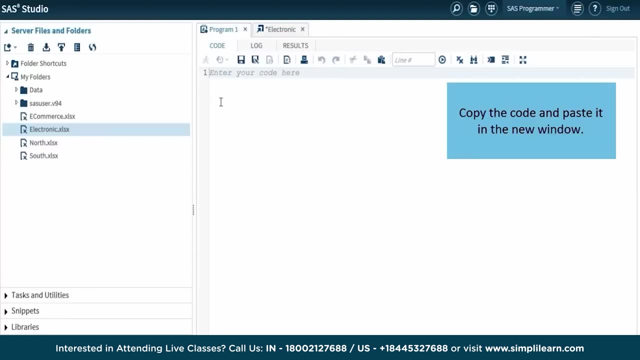 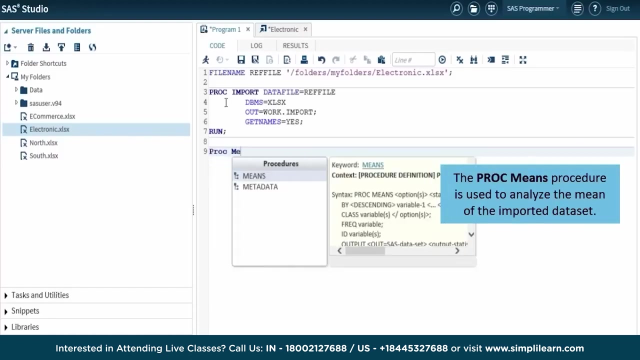 In the left plane, right-click the electronicxlsx dataset and click Import Data. The code to import the data generates automatically. Copy the code and paste it in the new window. The PROC MEANS procedure is used to analyze the mean of the imported dataset. 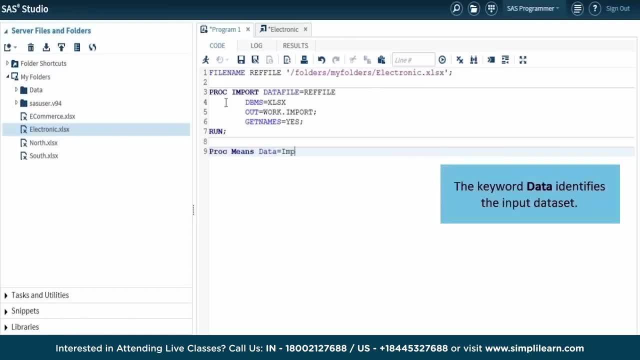 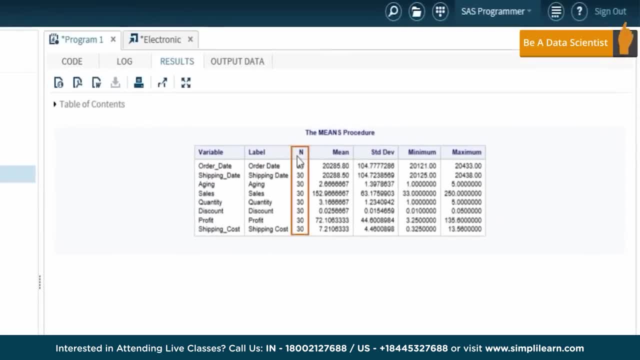 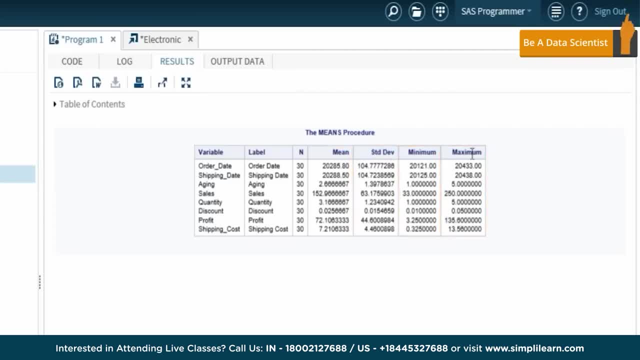 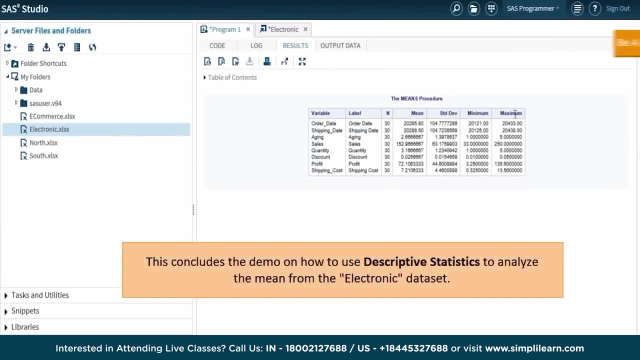 Note that the number of observations, mean, standard deviation and maximum and minimum values of the electronic dataset are obtained. This concludes the demo on how to use descriptive statistics to analyze the mean from the electronic dataset. This concludes the demo on how to use descriptive statistics to analyze the mean from the electronic 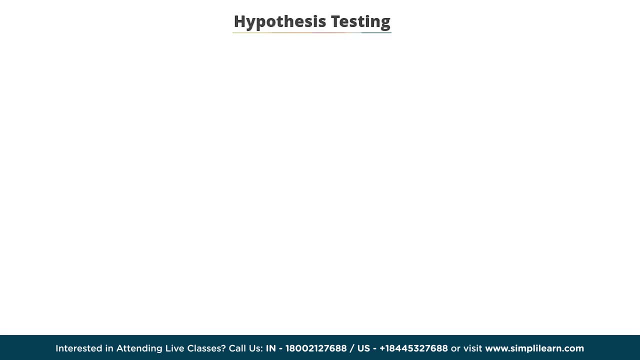 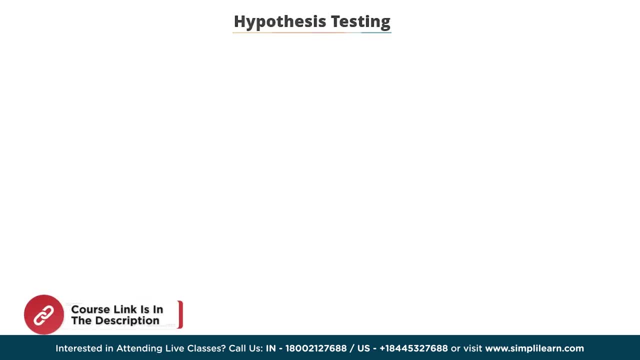 dataset. So far you have learned about descriptive statistics. Let's now learn about inferential statistics. Hypothesis testing is an inferential statistical technique to determine whether there is enough evidence in a data sample to infer that a certain condition holds true for the entire. 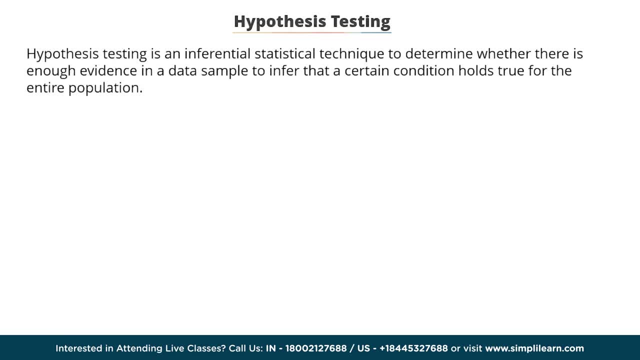 population. Hypothesis testing is an inferential statistical technique to determine whether there is enough evidence in a data sample to infer that a certain condition holds true for the entire population. To understand the characteristics of the general population, we take a random sample and analyze the properties of the sample. 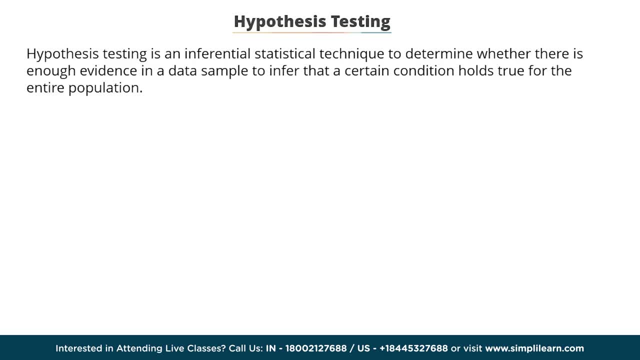 To understand the characteristics of the general population, we take a random sample and analyze the properties of the sample. We then test whether or not the identified conclusions correctly represent the population as a whole. To understand the characteristics of the general population, we take a random sample and analyze 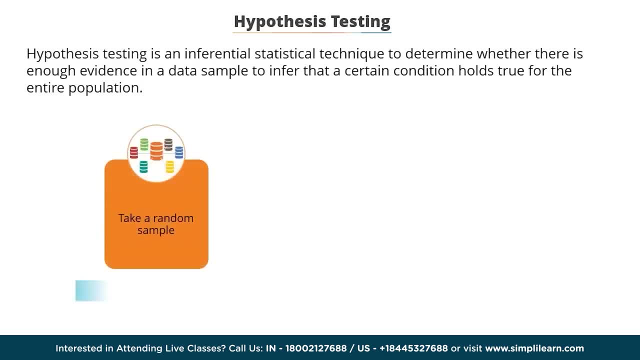 the properties of the sample. We then test whether or not the identified conclusions correctly represent the population as a whole. We then test whether or not the identified conclusions correctly represent the population as a whole. The population of hypothesis testing is to choose between two competing hypotheses about. 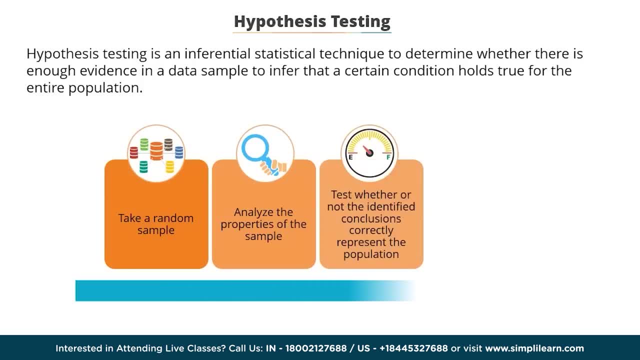 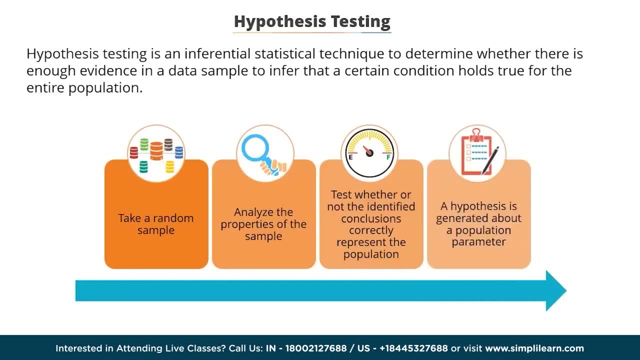 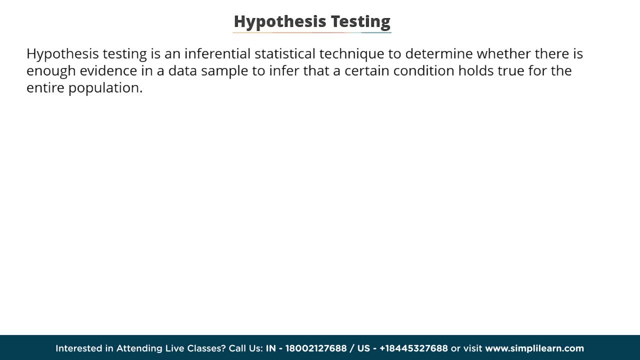 the value of a population parameter. The population of hypothesis testing is to choose between two competing hypotheses about the value of a population parameter. For example, one hypothesis might claim that the wages of men and women are equal, while the other might claim that women make more than men. 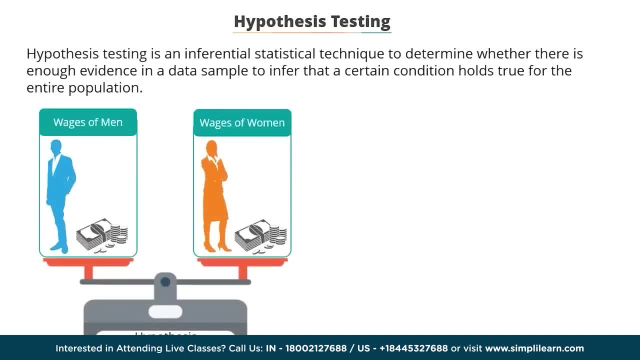 For example, one hypothesis might claim that the wages of men and women are equal, while the other might claim that women make more than men. For example, one hypothesis might claim that the wages of men and women are equal, while the other might claim that women make more than men. 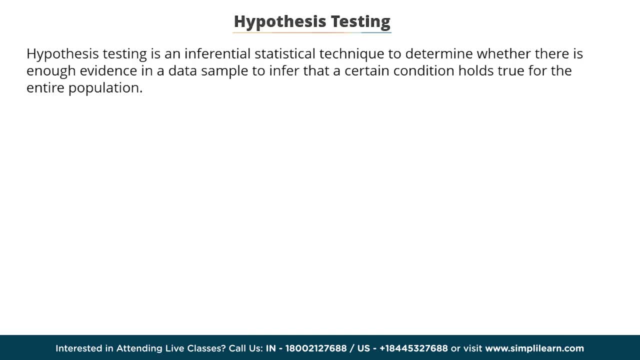 For example, one hypothesis might claim that the wages of men and women are equal, while the other might claim that women make more than men. 2- There is a rule in the Verbatim karena in�� a testa, Edinburgh Summa, There is a law in the Verbatim: karma and optimise a testa to get a得erata of Body. 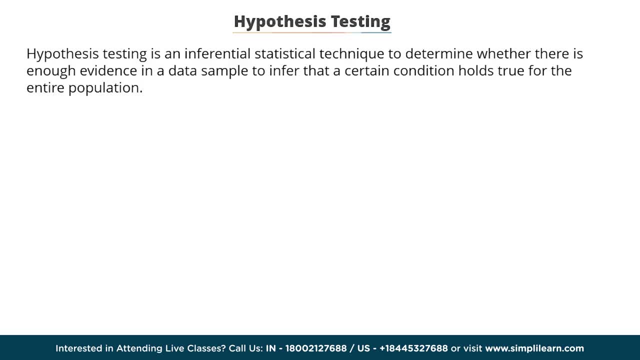 254이ŚmũXũnũťnũnũnũũ and 246iŚbũũnũwũũţũnũũnũũnũũnũnũũũnũũnũũnũũũũnũnũũnũũnũŬnũnũũnũsũũũnũũũsũ. 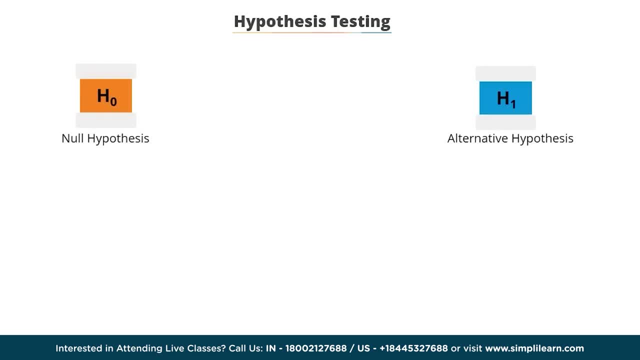 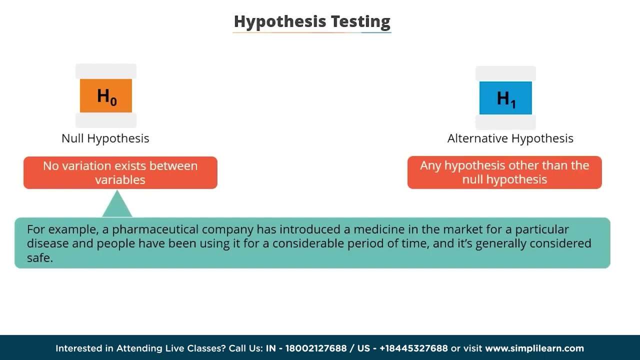 and alternative hypothesis using a general example. null hypothesis attempts to show that no variation exists between variables, and alternative hypothesis is any hypothesis other than the null. for example say, a pharmaceutical company has introduced a medicine in the market for a particular disease and people have been using it for a considerable period of time and it's generally considered. 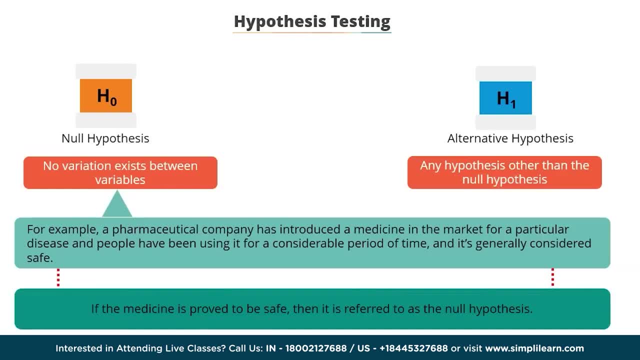 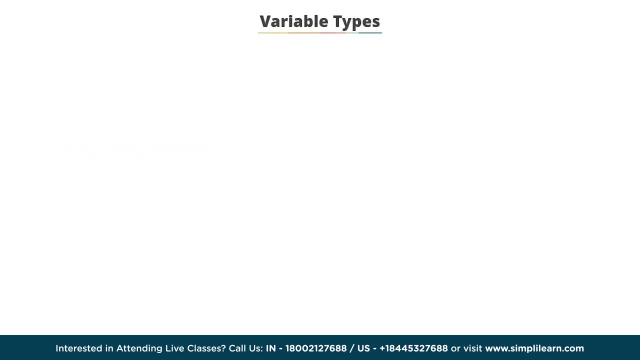 safe. if the medicine is proved to be safe, then it is referred to as null hypothesis. to reject null hypothesis, we should prove that the medicine is unsafe. if the null hypothesis is rejected, then the alternative hypothesis is used. before you perform any statistical tests with variables, it's 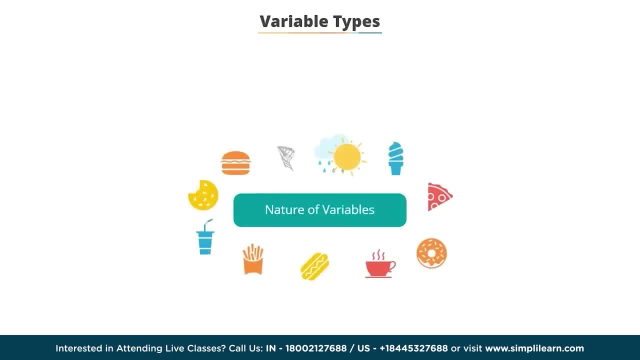 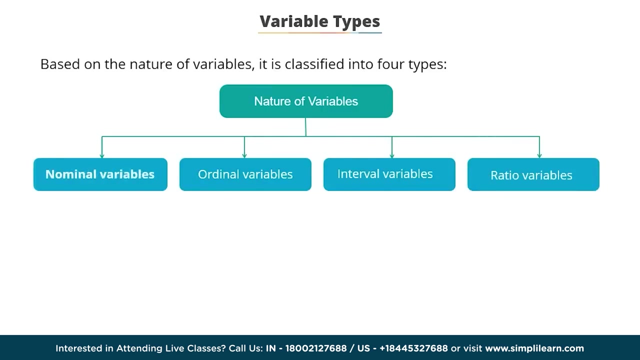 significant to recognize the nature of the variables involved. based on the nature of the variables, it's classified into four types. they are categorical or nominal variables, ordinal variables, interval variables and ratio variables. nominal variables are ones which have two or more categories and it's impossible to order the values. examples: 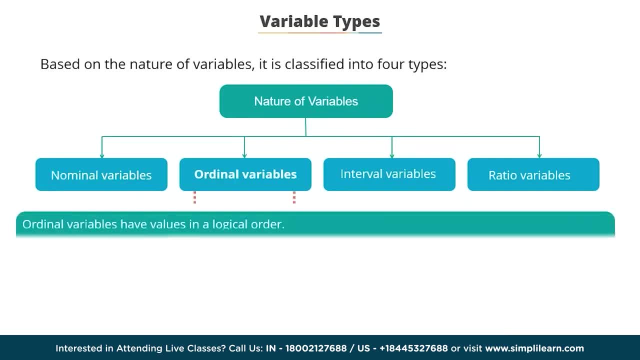 of nominal variables include gender and blood group. ordinal variables have values ordered logically. however, the relative distance between two data values is not clear. examples of ordinal variables include considering the size of a coffee cup- large, medium and small- and considering the ratings of a product- bad, good and best. interval variables are similar to ordinal variables, except 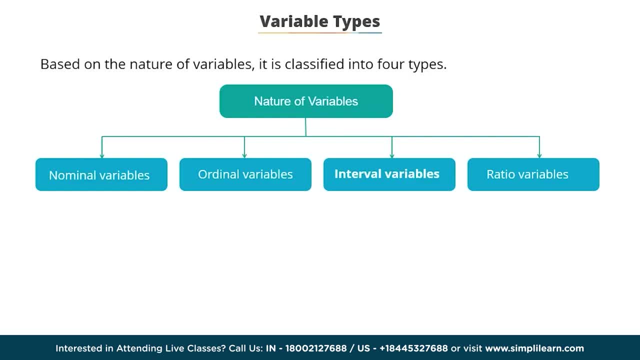 that the values are measured in a way where their differences are meaningful. with an interval scale, equal differences between scale values do have equal quantitative meaning. for this reason, an interval scale provides more quantitative information than the ordinal scale. the interval scale does not have a true zero point. a true zero point means that a value of zero on the scale 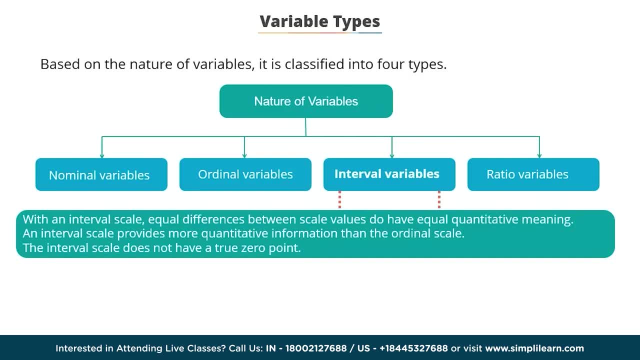 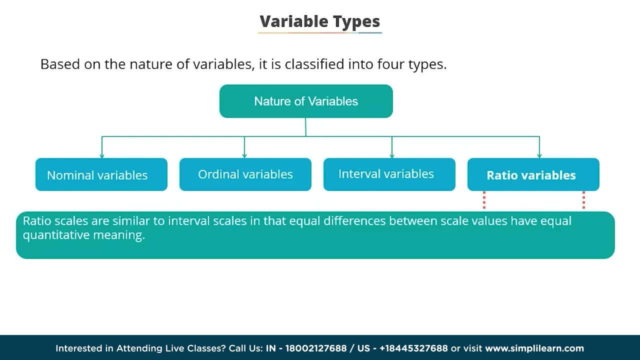 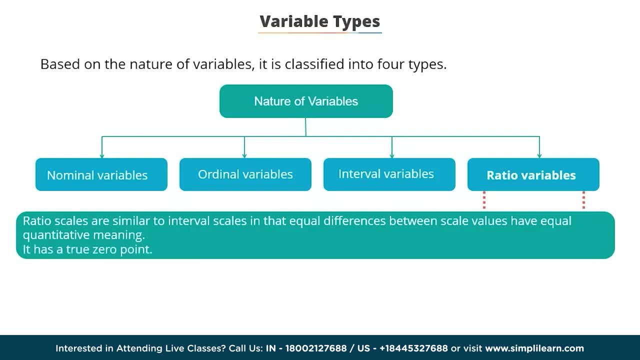 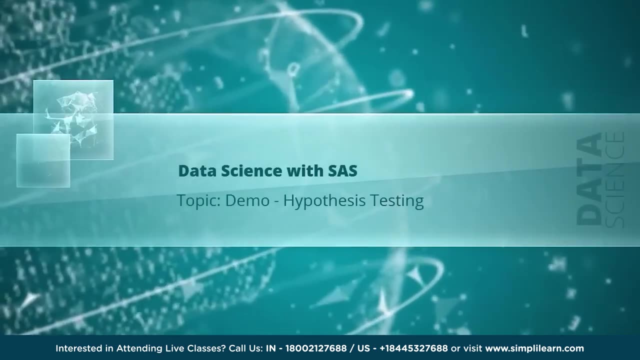 minus H, we get a derivative correct. these are related by the distance zero quantity of the construct being assessed. examples of interval variables include of a ratio scale. There is a true zero point because zero inches does in fact indicate a complete absence of length. In this demo, you'll learn how to perform the hypothesis testing using SAS. 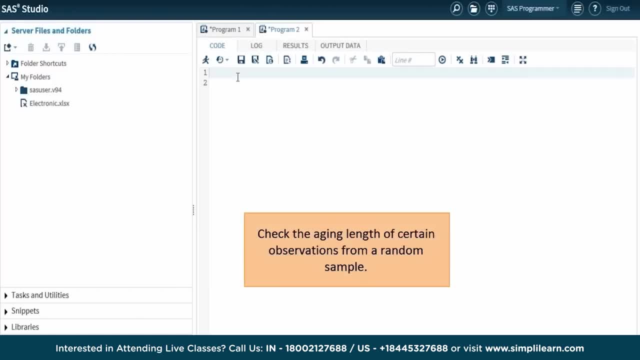 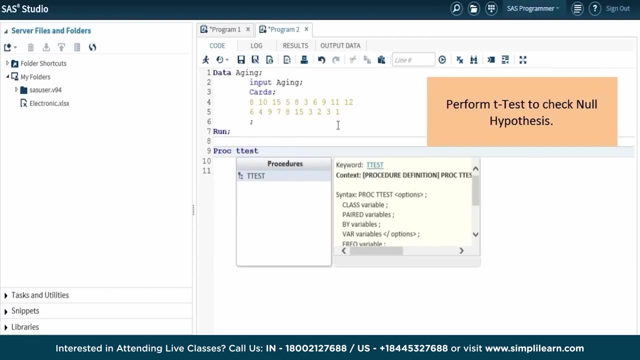 In this example, let's check against the length of certain observations from a random sample. The keyword data identifies the input dataset, The input statement is used to declare the aging variable and cards to read data into SAS. Let's perform a t-test to check the null hypothesis. 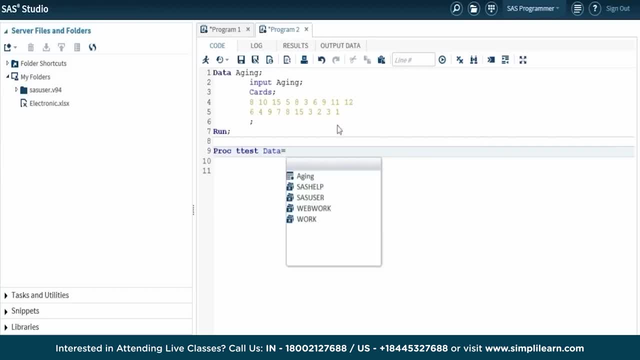 Let's assume that the null hypothesis is true. Let's set the null hypothesis to be that the mean days to deliver a product is 6 days, So null hypothesis equals 6.. Alpha value is the probability of making an error, which is 5% standard, and hence alpha equals 0.05.. 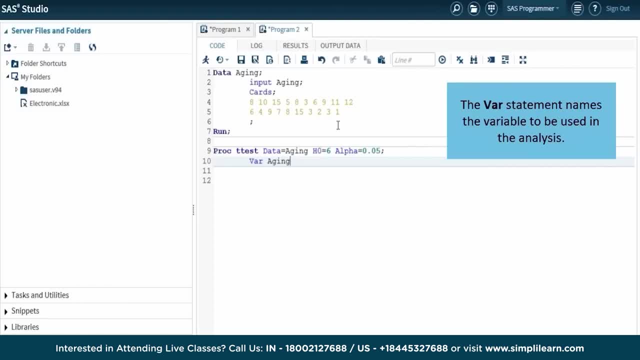 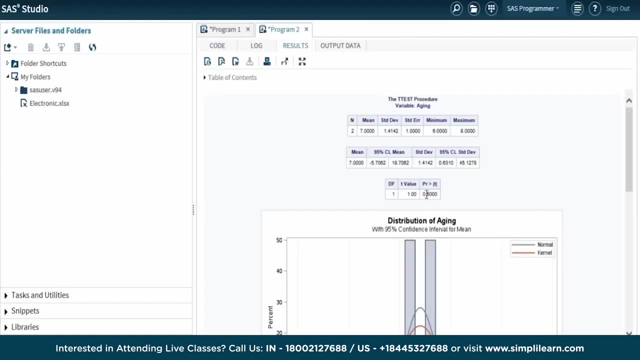 The variable statement names the variable to be used in the analysis. The output is shown on the screen. Note that the p-value is greater than the alpha value, which is 0.05.. Therefore, we fail to reject the null hypothesis. This concludes the demo on how to perform the hypothesis testing using SAS. 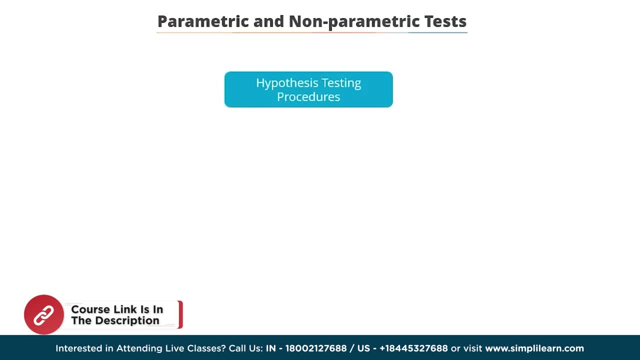 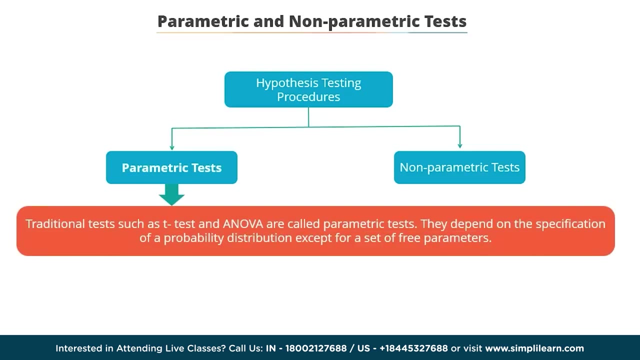 Let's now learn about hypothesis testing for SAS. For hypothesis testing procedures, there are two types of hypothesis testing procedures. They are parametric tests and nonparametric tests. In statistical inference or hypothesis testing, the traditional tests, such as t-test and ANOVA, are called parametric tests. 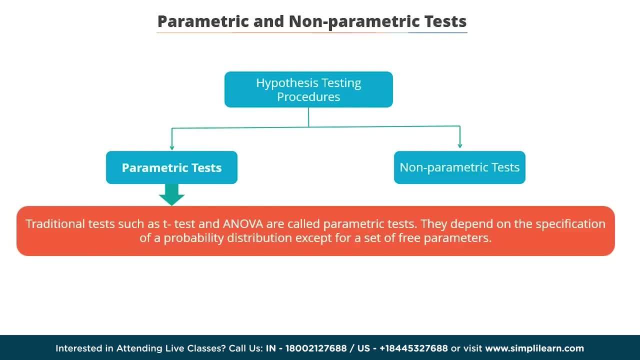 They depend on the specification of a probability distribution, except for a set of free parameters. In simple words, you can say that if the population information is known completely by its parameter, then it is called a parametric test. If the population or parameter information is not known and you are still required to test the hypothesis of the population, 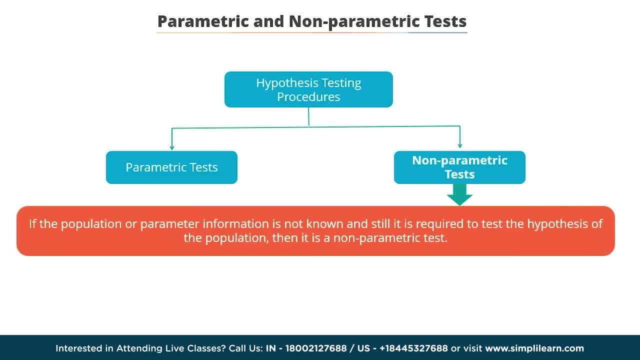 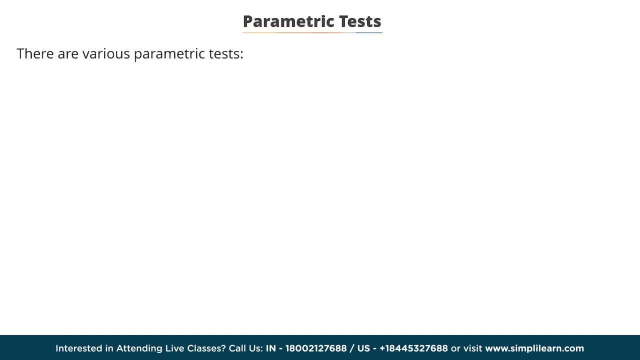 then it is called a nonparametric test. Nonparametric tests do not require any strict distributional assumptions. There are various parametric tests. They are as follows: t-test, ANOVA, chi-squared, linear regression. Let's understand them in detail. 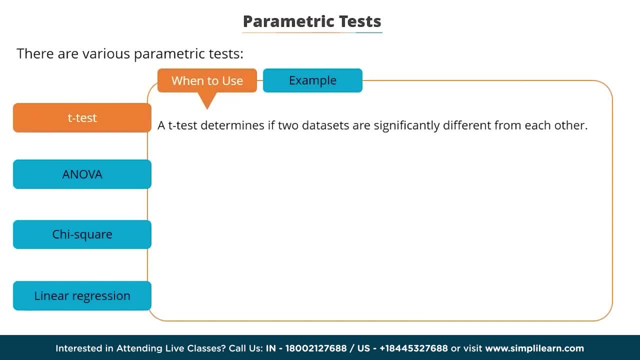 t-test. A t-test determines if two sets of data are significantly different from each other. The t-test is used in the following situations: To test if the mean is significantly different than a hypothesized value. To test if the mean for two independent groups is significantly different. 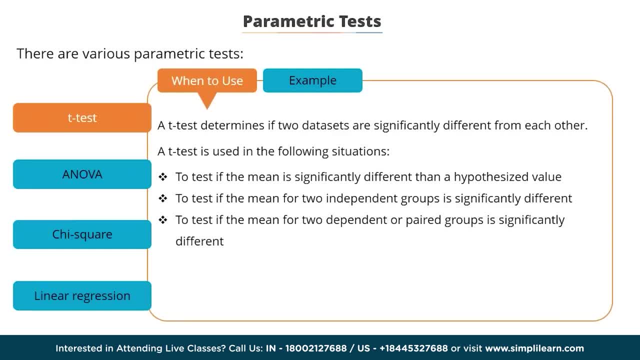 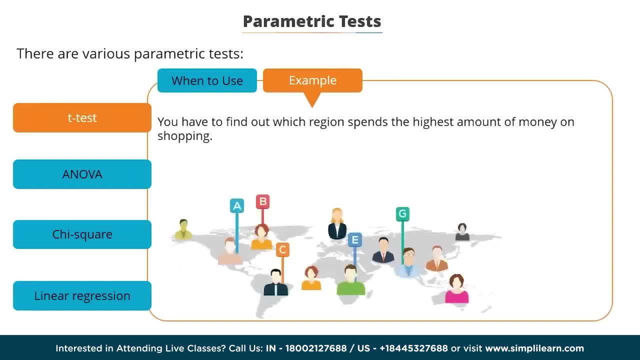 To test if the mean for two dependent or paired groups is significantly different. For example, let's say you have to find out which region spends the highest amount of money on shopping. It's impractical to ask everyone in the different regions about their shopping expenditure. 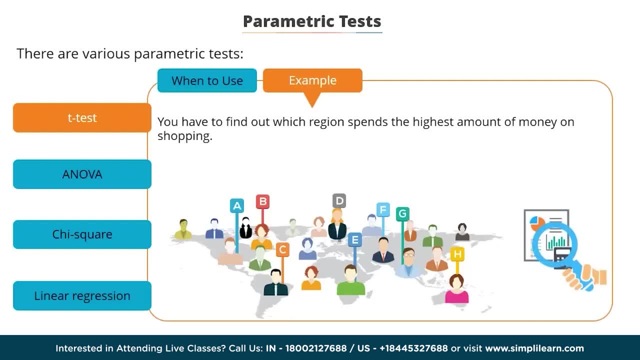 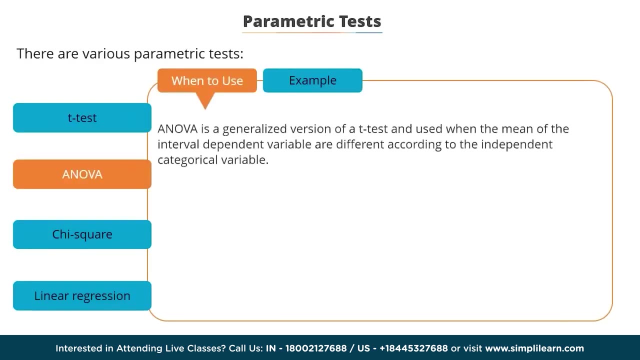 In this case, you can calculate the highest shopping expenditure by collecting sample observations from each region. With the help of the t-test, you can check if the difference between the regions are significant or a statistical fluke. ANOVA- ANOVA is a generalized version of the t-test and used when the mean of the interval dependent variable is different to the categorical independent variable. 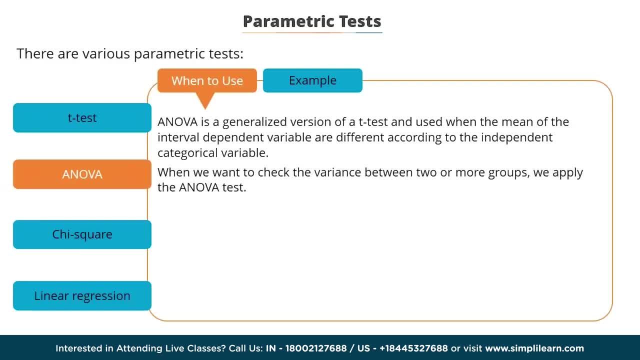 When we want to check variance between two or more groups, we apply the ANOVA test. For example, let's look at the same example of the t-test example. Now you want to check how much people in various regions spend every month on shopping. 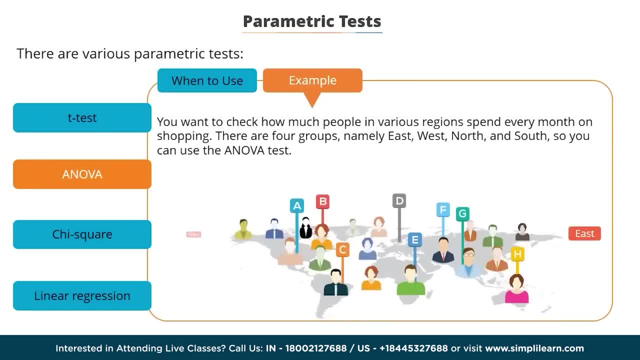 In this case, there are four groups, Namely East, West, North and South. With the help of the ANOVA test, you can check if the difference between the regions is significant or a statistical fluke- CHI-SQUARE. 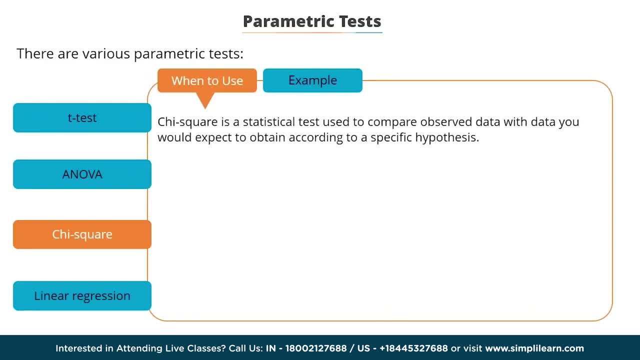 CHI-SQUARE is a statistical test used to compare observed data with data you would expect to obtain according to a specific hypothesis. Let's understand the CHI-SQUARE test through an example. You have a data set of male shoppers and female shoppers. 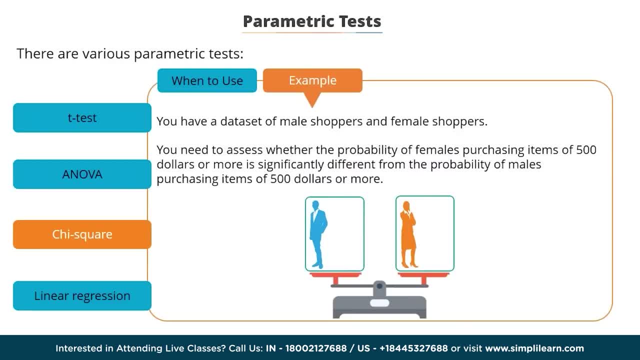 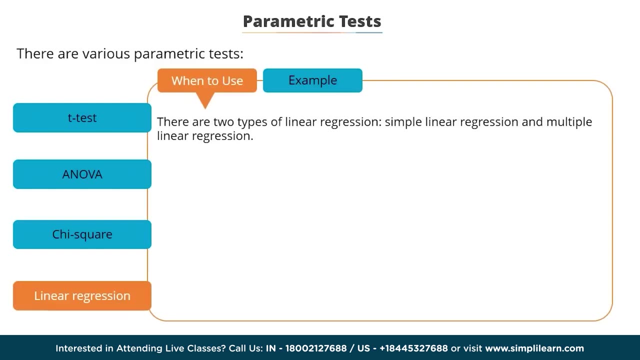 Let's say you need to assess whether the probability of females purchasing items of $500 or more is significantly different from the probability of males purchasing items of $500 or more. LINEAR REGRESSION: There are two types of linear regression: Simple linear regression and multiple linear regression. 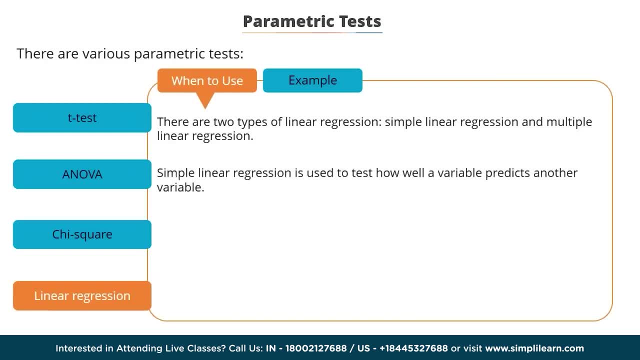 Simple linear regression is used when one wants to test how well a variable predicts another variable. Multiple linear regression allows one to test how well multiple variables or independent variables predict a variable of interest. When using multiple linear regression, we additionally assume the predictor variables are independent. 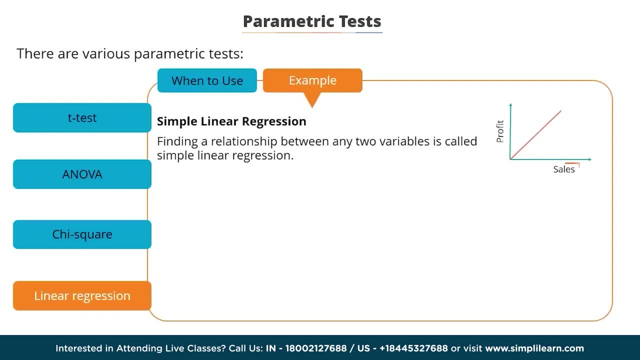 For example, finding relationship between any two variables, say sales and profit, is called simple linear regression. Finding relationship between any three variables, say sales, cost and telemarketing, is called multiple linear regression. In this case, my thanks to my websearchpad. 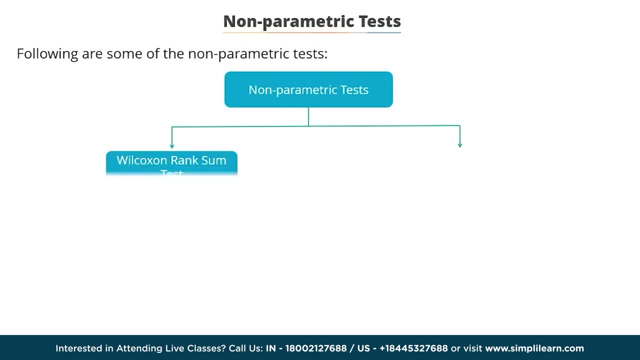 Some of the nonparametric tests Are Wilcoxon ranked sum test and Kruskal Wallace mask mark mark test. Will Coxen Ranks Sum Test. The Wilcoxon Signed Rank test is a nonparametric statistical hypothesis test used to compare two related samples or matched samples to assess whether or not their population mean ranks differ. 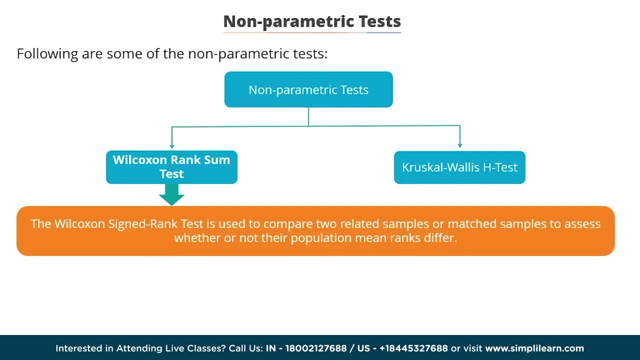 It is used by several models. differences of how well a variable predicts how many plus a variable is likely to believe. In Wilcoxon Rank Sum Test, you can test the null hypothesis hypothesis on the basis of the ranks of the observations. Kruskal-Wallis H-test: Kruskal-Wallis H-test is a 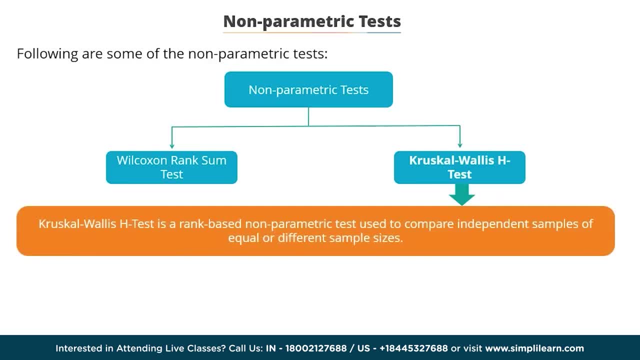 rank-based non-parametric test used to compare independent samples of equal or different sample sizes. In this test, you can test the null hypothesis on the basis of the ranks of the independent samples. Hello everyone, Welcome to this video on R4 Data Science. 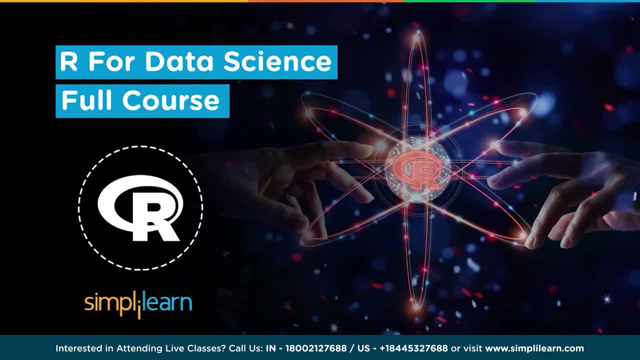 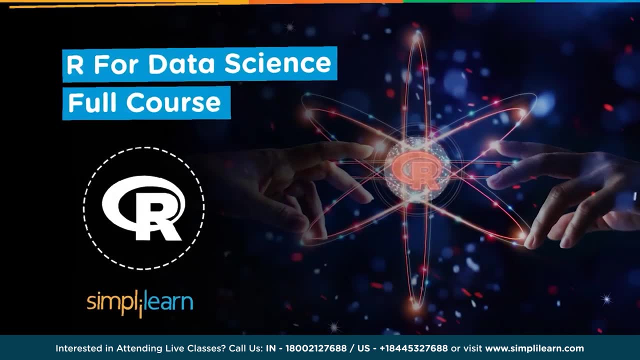 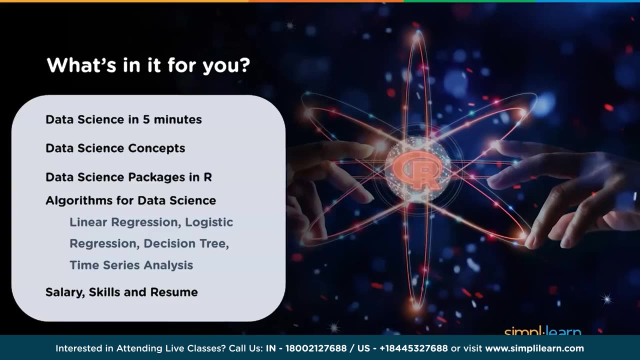 Full Course. Today we have our experience instructors, Richard Ajay and Pete Ferrari, who will help us learn everything from basics to advanced and master data science in R. We will start by learning data science from an animated video. You will then learn the essential concepts in data science and understand the important packages. 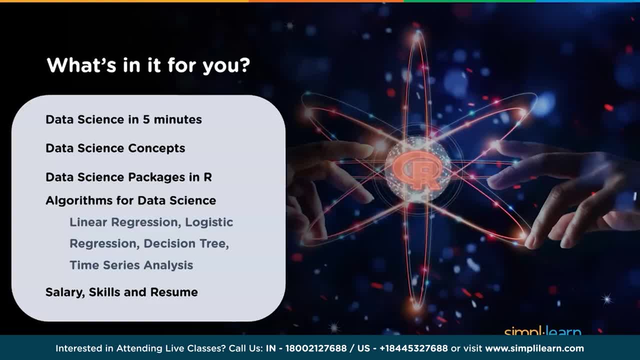 in R for data science, such as dplyr and tidyr. You will look at some of the widely used data science algorithms, such as linear regression, logistic regression, decision trees, random forests, including time series analysis. Finally, you will get an idea about the salary structure. 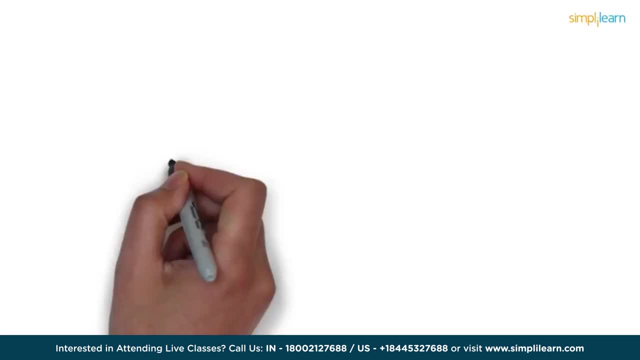 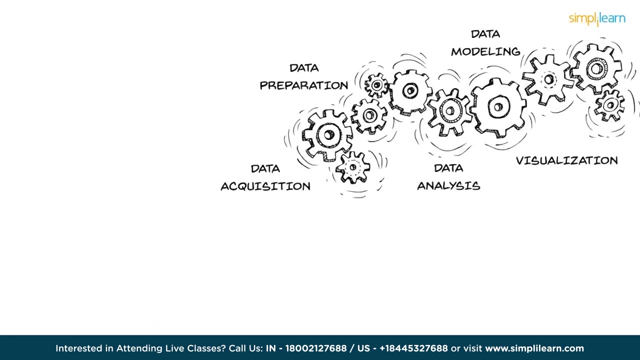 skills, jobs and resume of a data scientist. Are you one of the many who dreams of becoming a data scientist? Keep watching this video if you are passionate about data science, because we will tell you how does it really work? under the hood, Emma is a data scientist. Let's see how. 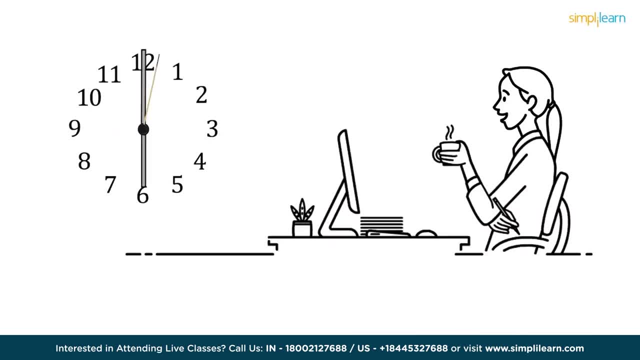 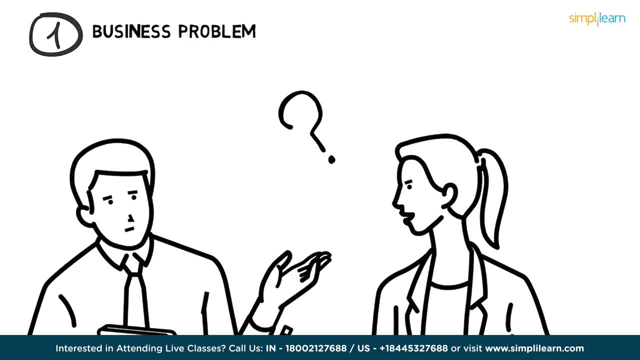 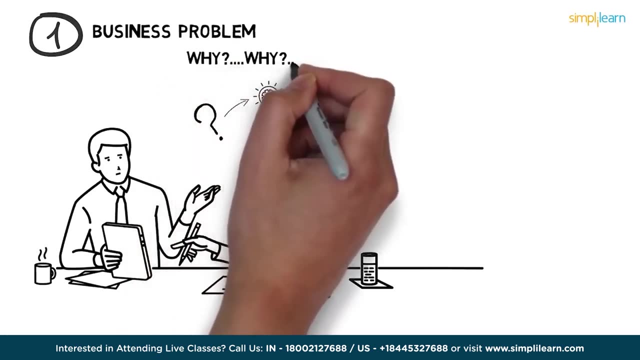 a day in her life goes while she is working on a data science project. Well, it is very important to understand the business problem first. In our meeting with the clients, Emma asked relevant questions, understands and defines objectives for the problem that needs to be tackled. She is a curious soul who. 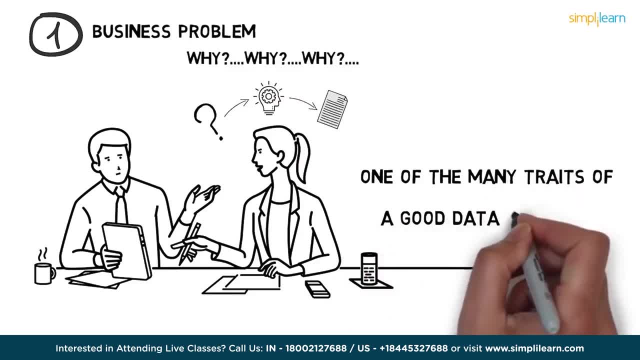 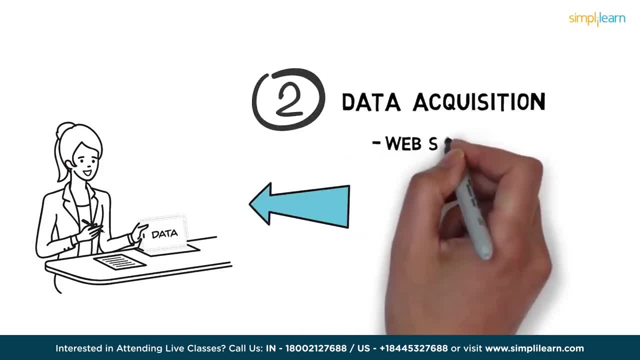 asks a lot of questions, One of the many traits of a good data scientist. Now she gears up for data acquisition, To gather and scrape data from multiple sources like web servers, logs, databases, APIs and online repositories. Oh, it seems like. 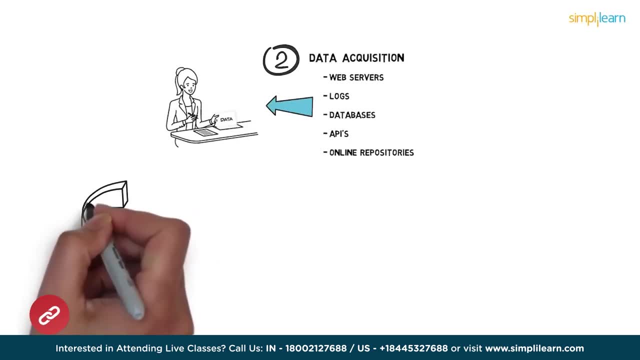 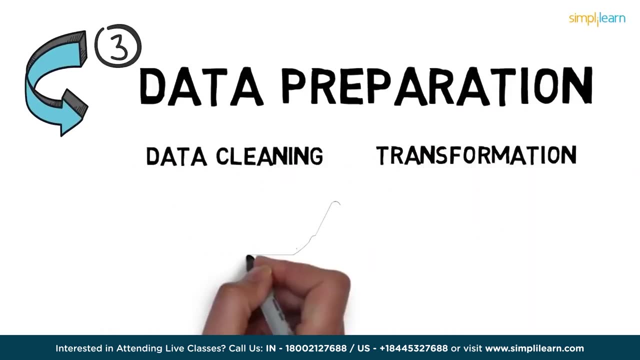 finding the right data takes both time and effort. After the data is gathered comes data preparation. This step involves data cleaning and data transformation. Data cleaning is the most time consuming process, as it involves handling many complex scenarios. Here Emma deals with inconsistent data types, misspelled attributes. 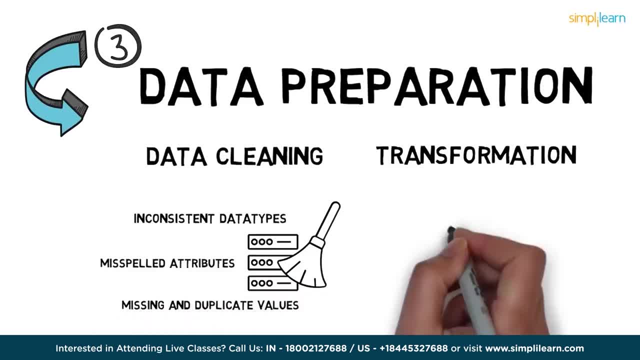 missing values, duplicate values and what not? Then in data transformation, she modifies the data based on defined mapping rules. In her project, ETL, tools like Talent and Informatica are used to perform complex transformations. that helps the team to understand the data structure better, Then understanding what you actually. 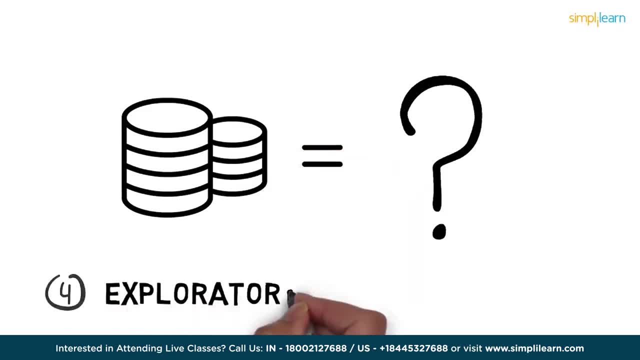 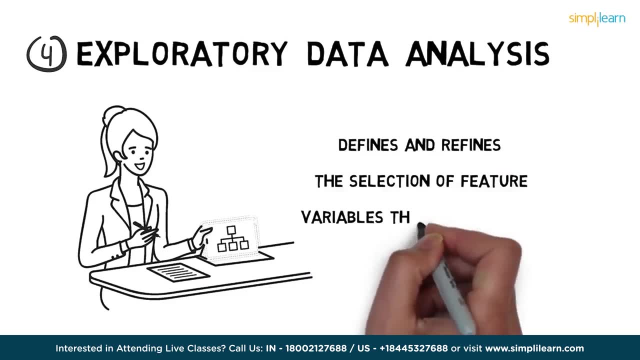 can do with your data is very crucial. For that, Emma does exploratory data analysis. With the help of EDA, she defines and refines the selection of feature variables that will be used in the model development. But what if Emma skips this step? She might end up choosing. 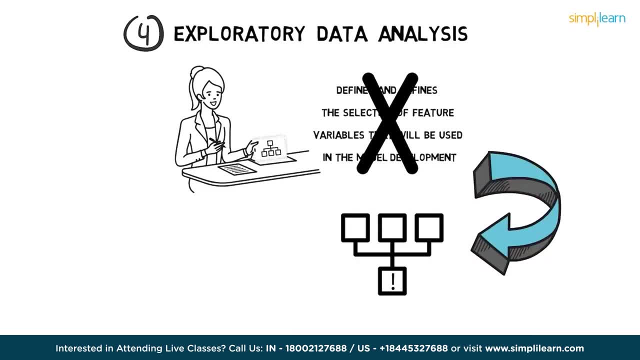 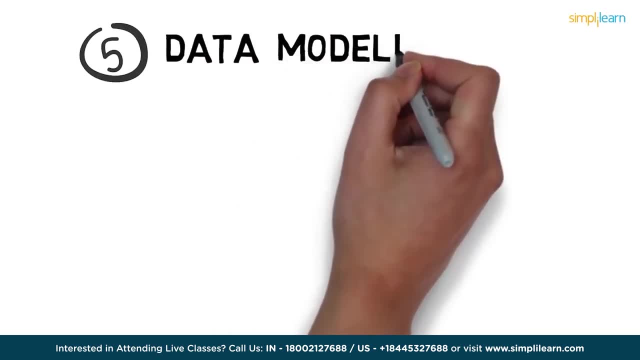 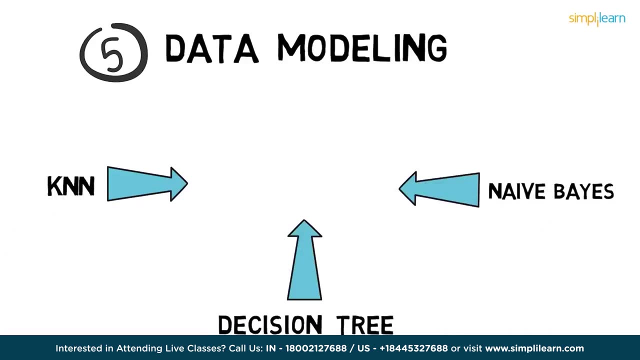 the wrong variables, which will produce an inaccurate model. Thus exploratory data analysis becomes the most important step. Now she proceeds to the core activity of a data science project, which is data modeling. She repetitively applies diverse machine learning techniques, like KNN, Decision Tree, KnifeBase, to the data. 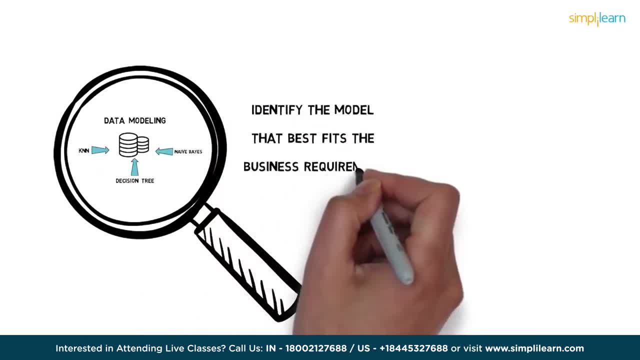 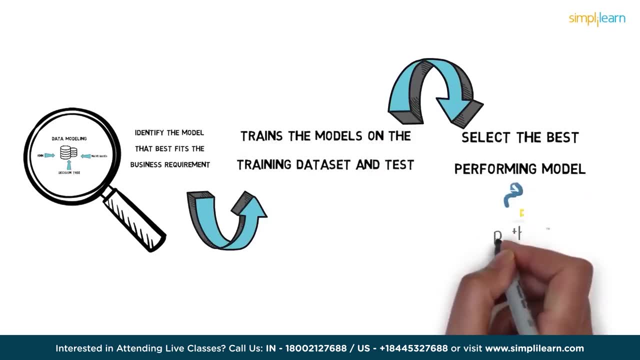 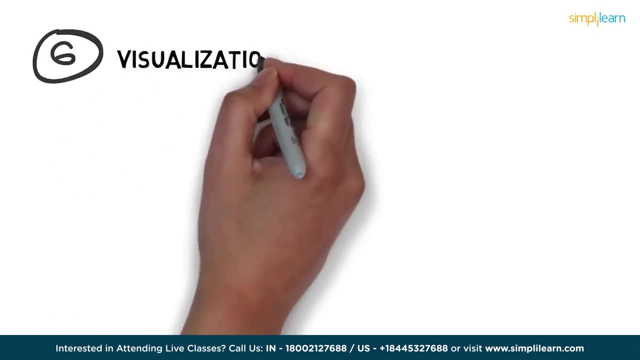 to identify the model that best fits the business requirement. She trains the models on the training dataset and tests them to select the best performing model. Emma prefers Python for modeling the data. However, it can also be done using R and SAS. Well, the trickiest part is not yet over. 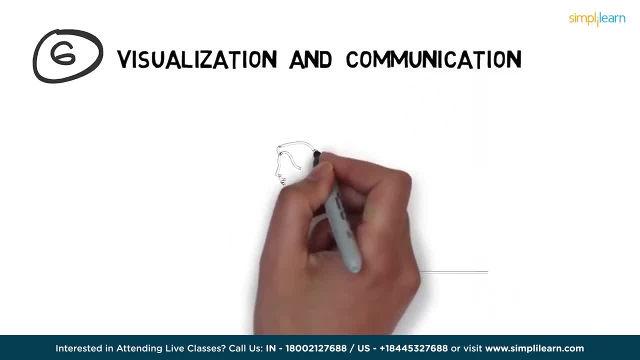 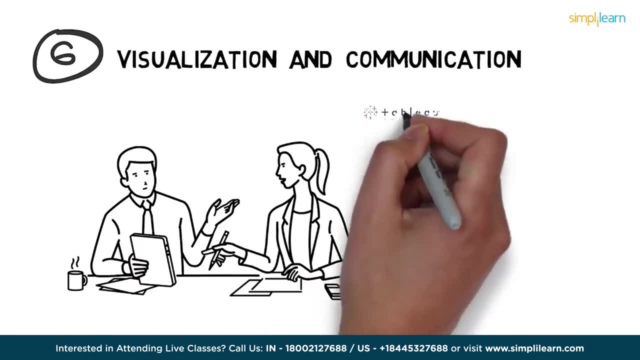 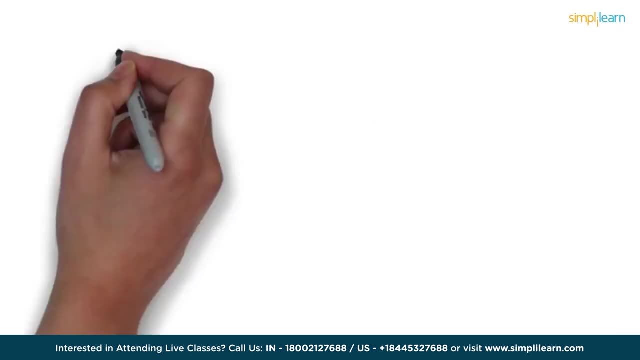 Visualization and communication. Emma meets the clients again to communicate the business findings in a simple and effective manner to convince the stakeholders, She uses tools like Tableau, Power BI and QlikView that can help her in creating powerful reports and dashboards. And then, finally, she deploys and maintains. 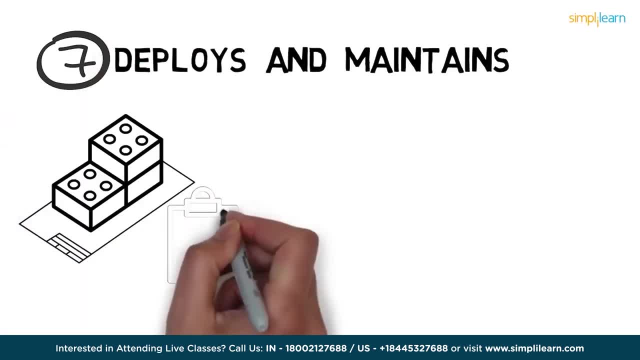 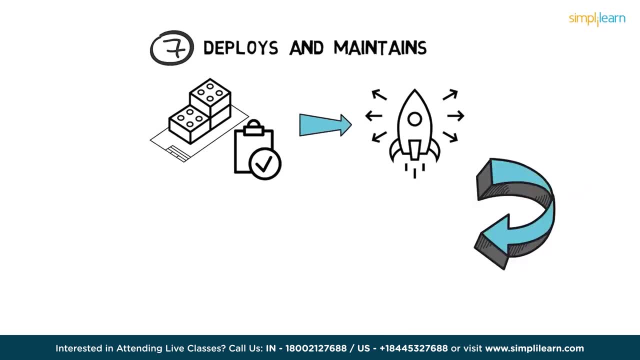 the model. She tests the selected model in a pre-production environment before deploying it in the production environment, which is the best practice. right After successfully deploying it, she uses reports and dashboards to get real-time analytics. Further, she also monitors and maintains the project's performance. Well, that's how. 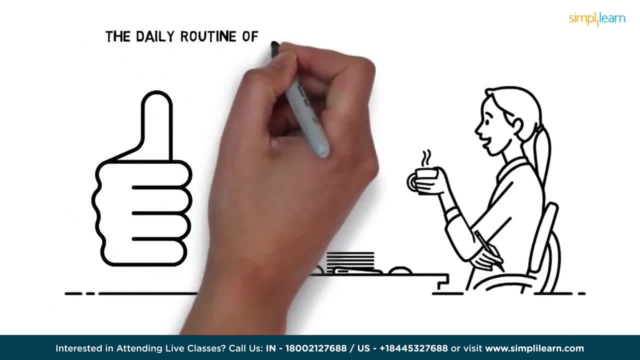 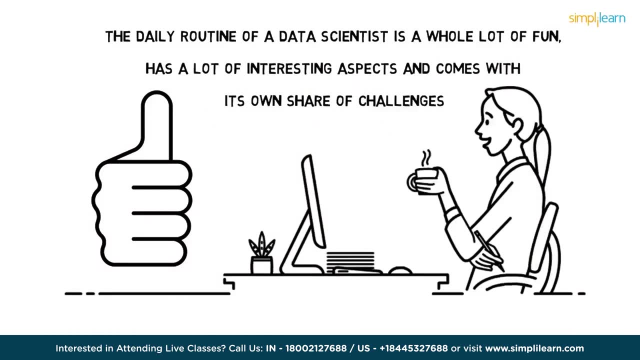 Emma completes the data science project We have seen the daily routine of a data scientist is a whole lot of fun, has a lot of interesting aspects and comes with its own share of challenges. Now let's see how data science is changing the world. Data science techniques, along with 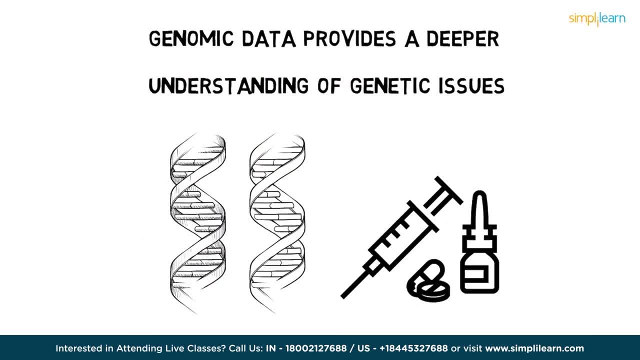 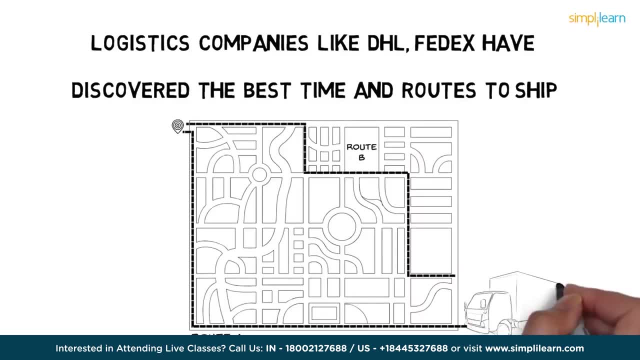 genomic data provides a deeper understanding of genetic issues and reaction to particular drugs and diseases. Logistic companies like DHL, FedEx have discovered the best routes to ship, the best suited time to deliver, the best mode of transport to choose, thus leading to cost efficiency. With data science, it is possible. 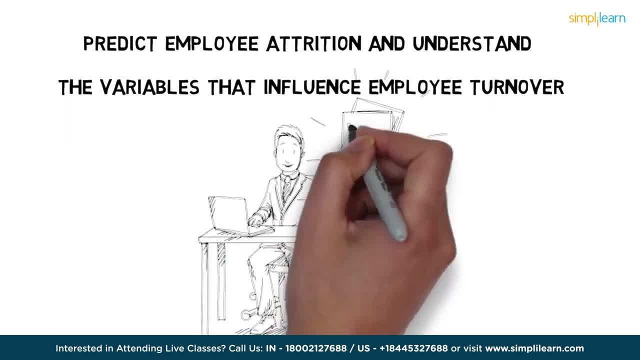 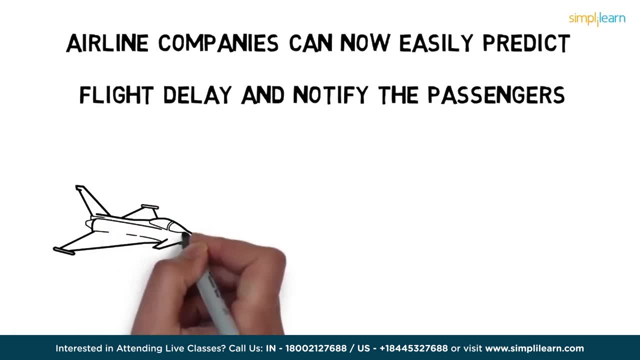 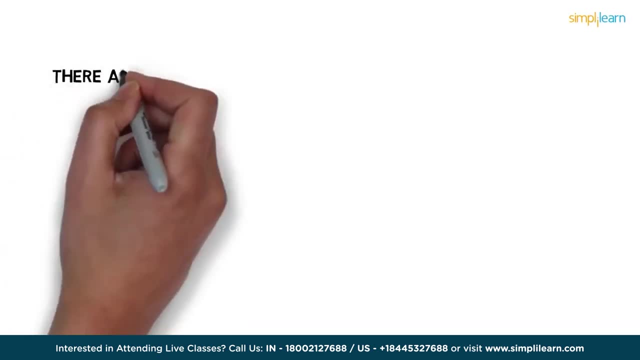 to not only predict employee attrition, but to also understand the key variables that influence data science. Also, the airline companies can now easily predict flight delay and notify the passengers beforehand to enhance their travel experience. Well, if you're wondering, there are. 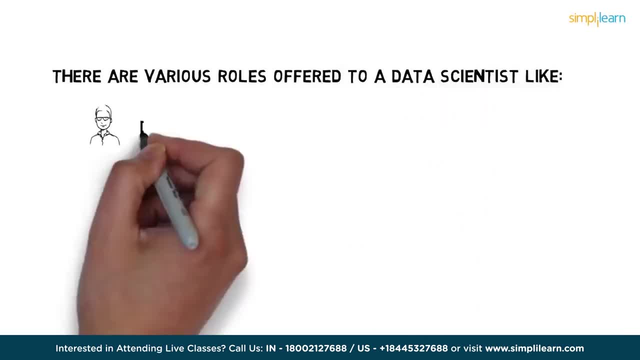 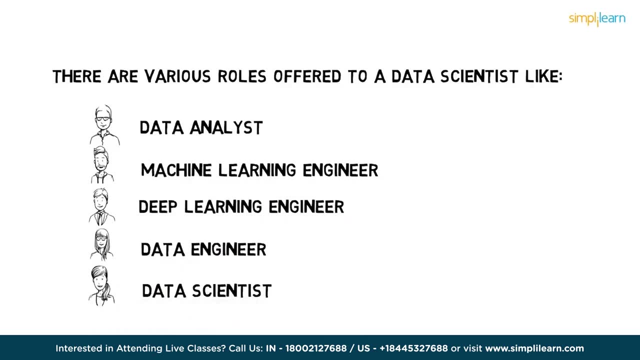 various roles offered to a data scientist, like data analyst, machine learning engineer, deep learning engineer, data engineer and, of course, data scientist. The median base salaries of a data scientist can range from $95,000 to $165,000.. 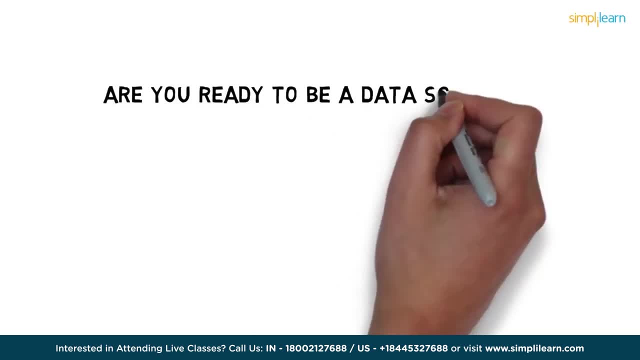 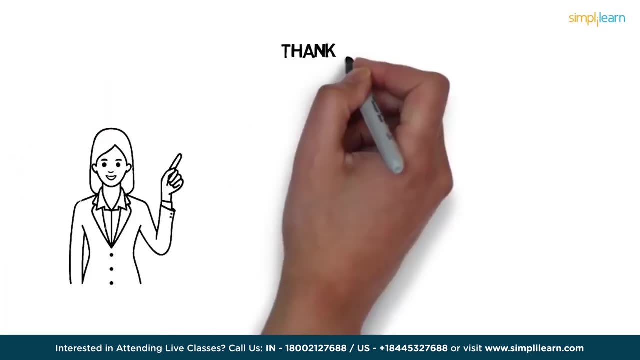 So that was about the data science. Are you ready to be a data scientist? If yes, then start today. The world of data needs you. That's all from my side today. Thank you for watching Comment below the next topic that you want to learn and subscribe to SimplyLearn to get the latest. 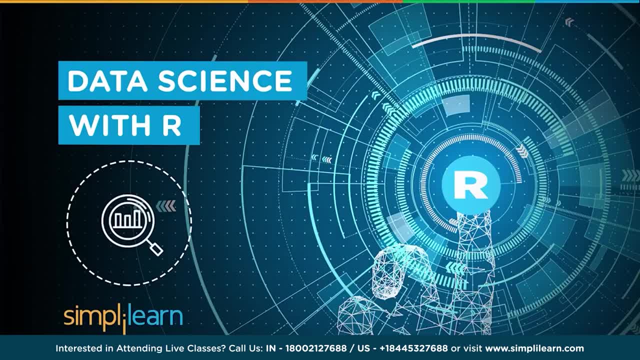 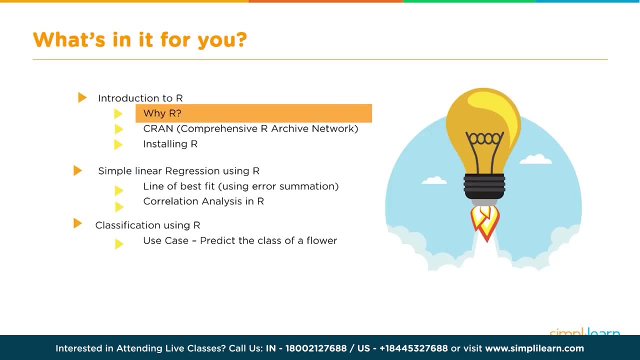 updates on more such interesting videos. What's in it for you? We're going to go through an introduction to R, YR, CRAN, comprehensive R archive network, and cover installing R. Then we'll get into simple linear regression using R line of best fit, using error summation. 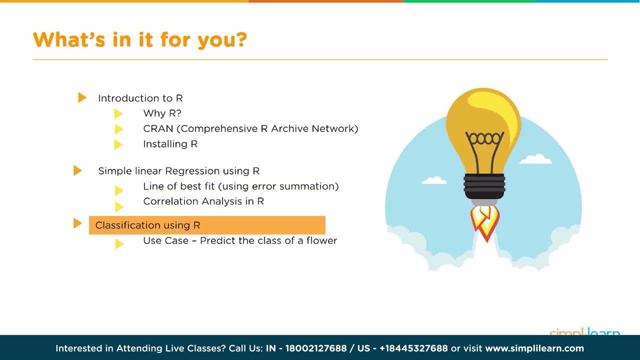 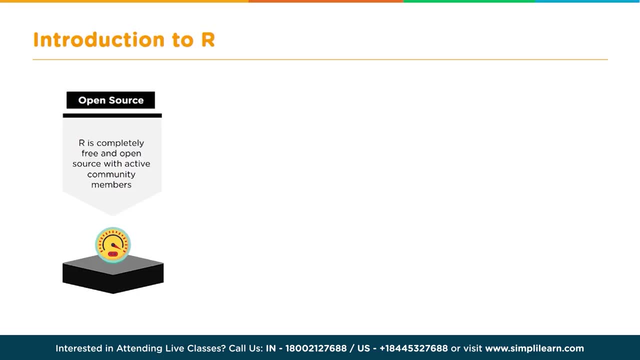 correlation analysis in R and then we'll get into classification using R. Use case: predict the class of a flower. Let's start with an introduction to R First. it's an open source. R is completely free and open source, with active community members Extensible. 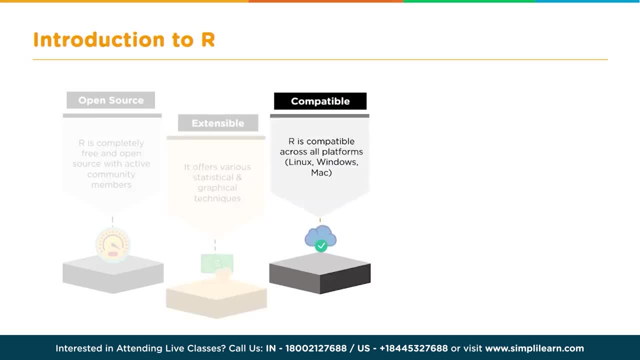 It offers various statistical and graphical techniques. Compatible: R is compatible across all platforms: Linux, Windows and Mac. Library R has an extensive library of packages for machine learning. Easy integration: It can be easily integrated with popular softwares like Tableau, SQL Server, etc. 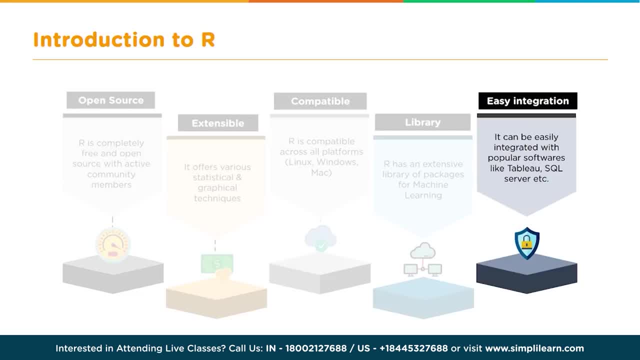 This only touches a little bit on these different aspects of R. The fact that it's a free: it's very extensive. It probably has one of the most extensive set of data analysis packages currently out. It has a compatibility that is continually growing, So it's integrated with everything. 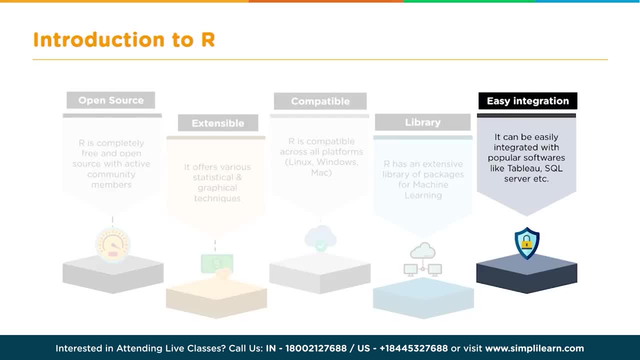 from cluster computing to Python. integration, which is now coming out, And it's extensive libraries, allows you to import the different libraries to use for whatever your needs are, Makes it a very diverse and easy to use coding source for analyzing data. R is more than just a. 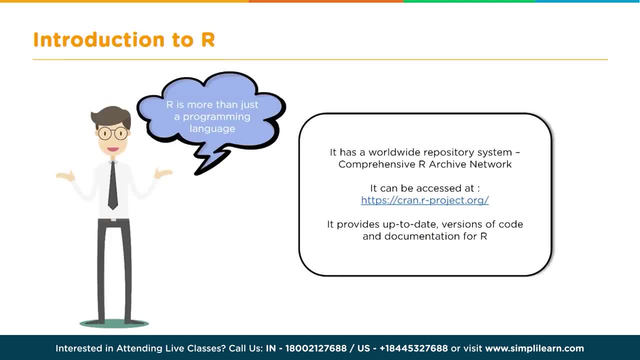 programming language. As I just touched upon it. it has a worldwide repository system, Comprehensive R archive network, And it can be accessed at https//cranrprojectorg. It provides up-to-date versions of code and documentation for R. Cran hosts around 10,000 packages of R. That is a 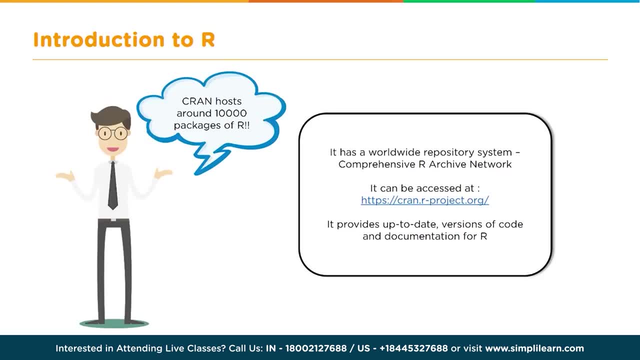 huge repository focused on just data analytics. Let's install R to get started. You can easily download the executable file for R and install it from Cran website If you go under the downloads. in this case, since I'm on a Windows machine, we'll walk through it from. 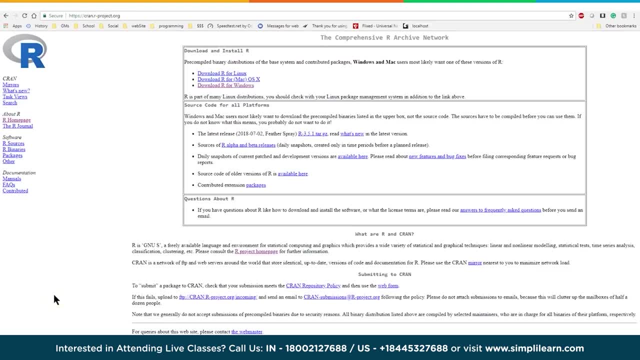 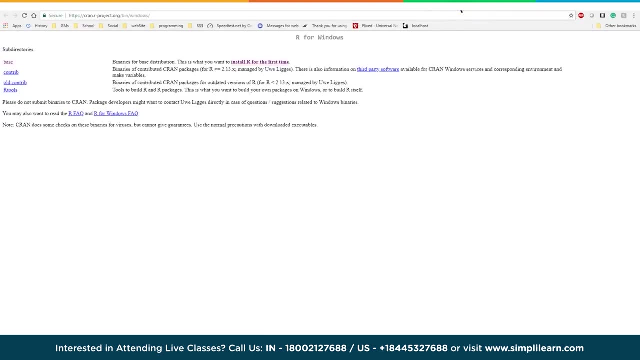 the R 3.5 version for Windows. So here we are at https//cranr-projectorg And you can see down here we have the different options for the downloads. If we go under Windows, which is I'm on a Windows machine, If you're on a Mac machine, you can do the Mac or Linux. 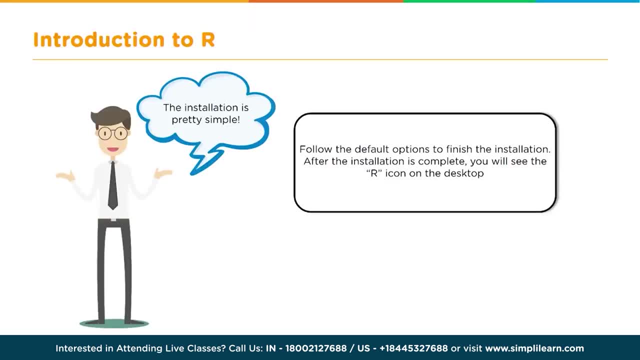 There's install R for the first time. Just click on that and open and run it. The installation is pretty simple. Follow the default options to finish the installation. After the installation is complete, you'll see the R icon on your desktop. Alternatively, there are mirror sites And so we can go into. 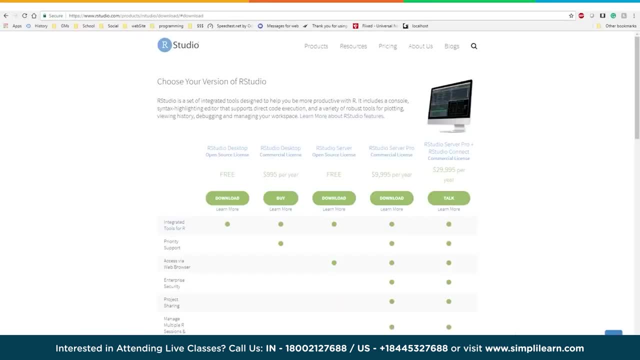 RStudio. Let's just take a quick look at that. If you're on the RStudio website, that's wwwrstudiocom, You can go down under products and RStudio download. You'll see a number of options here. The first one is the RStudio desktop open. 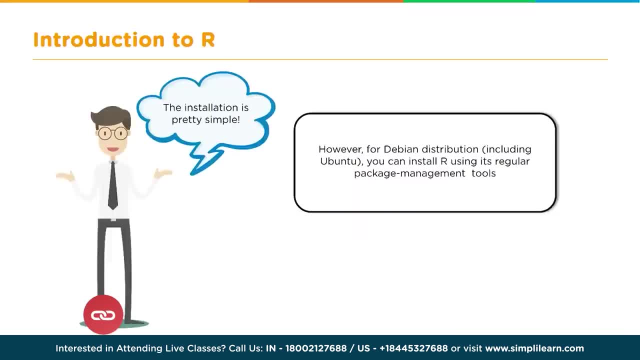 source license. That's the same thing you just downloaded, including Ubuntu. You can install R using its regular package management tools, And when you're using a Linux system, that is preferred because then it registers it properly on the setup system. Let's go ahead and open up our RStudio and take a look. Here we are. 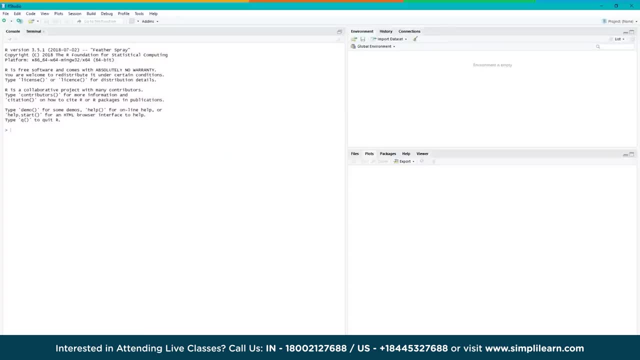 and I've opened this up in the RStudio version, which automatically opens up some extra windows, which is nice. Let's go ahead and take a look at that. We have our console on the left. This is your main workspace. So if I go in here, 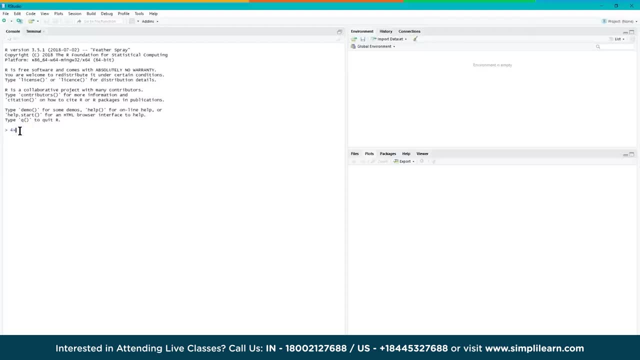 and I click the mouse and I do a 4 plus 4, it'll come up and say the answer is 8. And you have some environmental information and over on the right you have plots. Usually when you're working in here, let's do a script. We'll go up here to the plus sign in the 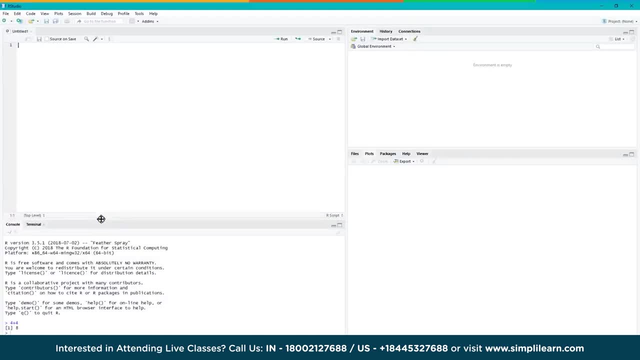 upper left hand corner and just add some script in here. In this case it showed up on the top, but you can move these windows around. And let's say I do: Y equals 3 plus 4.. X equals Y plus 2.. And then I'm going to do just X. 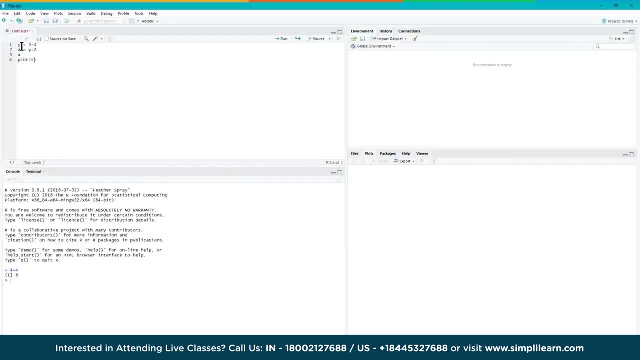 And let's do a plot. We'll throw a plot in there. C- C is a notation that these are going to be Cartesian points. So we've got 1 comma, 2 comma 3.. That would be like your X And then Y, 3 comma, 4 comma, 5, for just a standard call scatter. 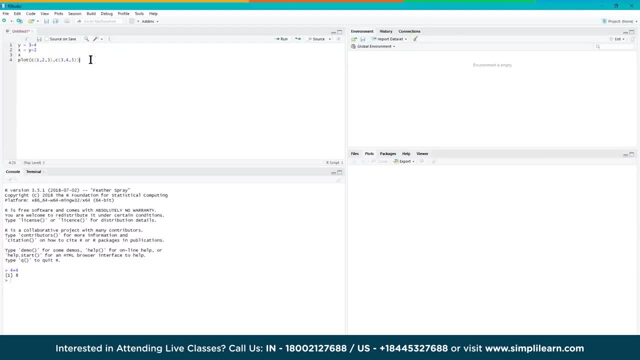 plot. We don't have to memorize this. We'll go into some of this later on And then I can take all of this If I go under code, since I'm working in the code console And I go down to run. 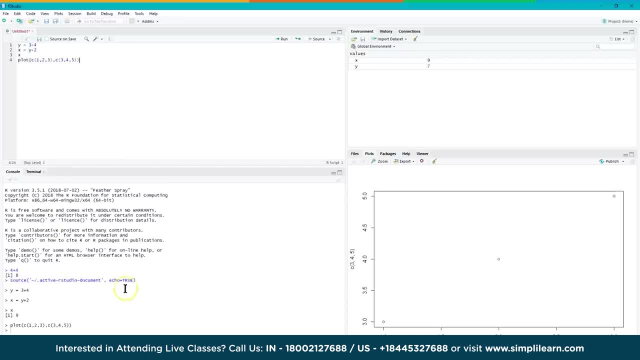 Region and just run all It. takes this code and just runs it through my console And you can see down here it's executed. Y equals 3 plus 4.. X equals X plus 2.. And if you add 3 plus 4, 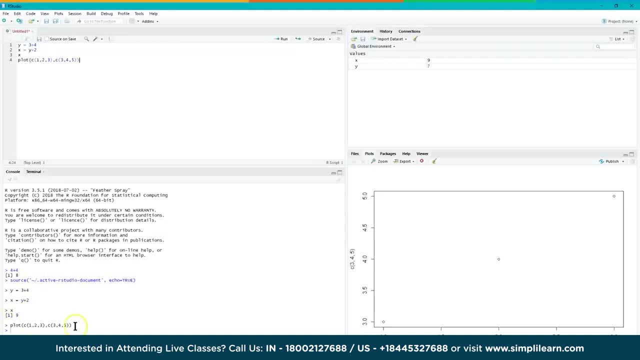 plus 2, you get 9.. That's what the X does. And then I did a plot. I threw the plot in there. I'm plotting 1, 2, 3,, 3,, 4,, 5.. And if you use, 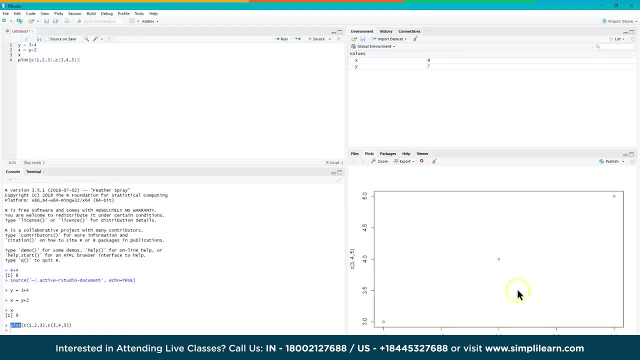 just a straight plot. it's a scatter plot And you can see that this appears on the bottom right where you have your plots coming in. So it's a very quick way to show data, And that's one of the wonderful things about R is it's very easy and quick. 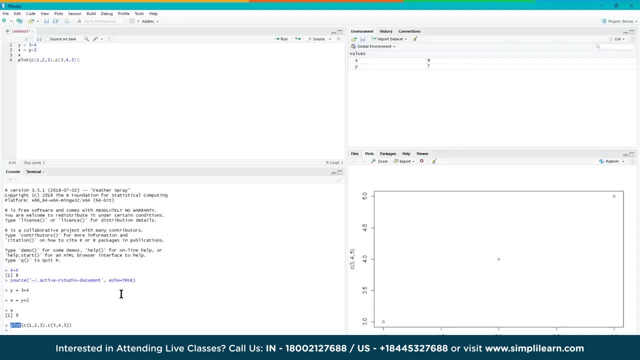 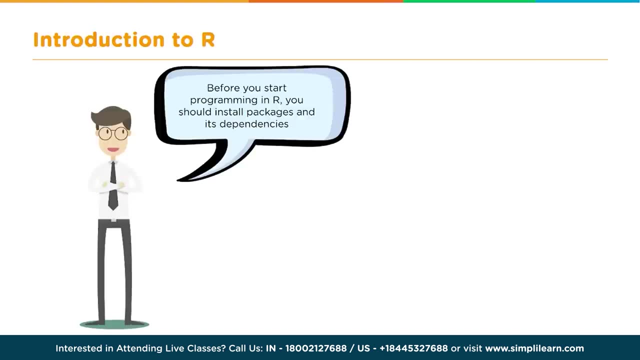 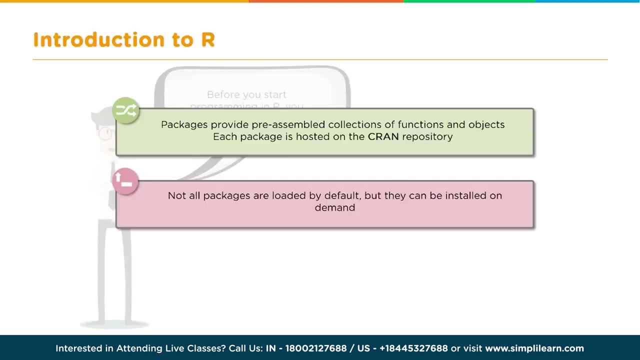 to go through and do different functions on the data and analyze it, So it's a very popular package. Before you start programming in R, you should install packages and its dependencies. Packages provide preassembled collections of functions and objects. Each package is hosted on the CRAN repository- Not all. 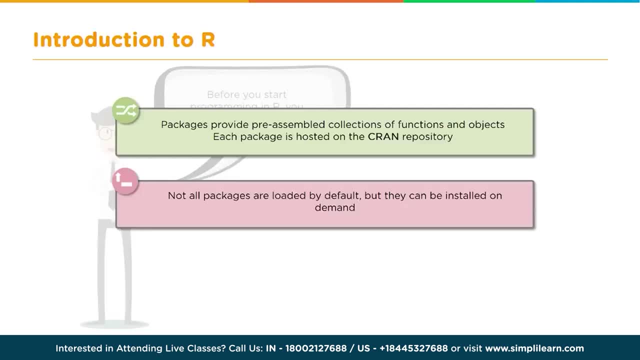 packages are loaded by default, but they can be installed on demand. Remember earlier we were talking about all the different packages available. You don't want to install everything from R. It would just be a huge waste of space. You want to just install those packages you need. So to install. 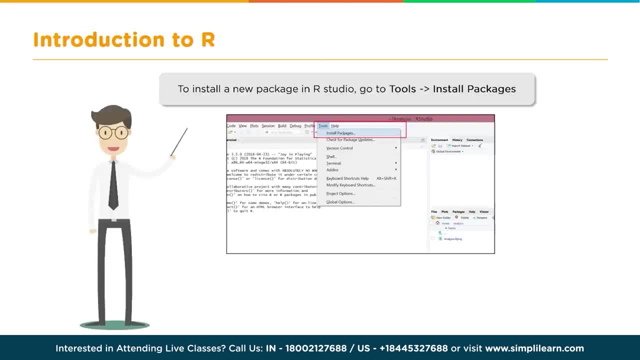 packages. in RStudio you go under tools and install packages. If you click on the install packages you'll get a dialog box. You'll see where it has the repository CRAN, because there's other repositories and you can even download and install your own. 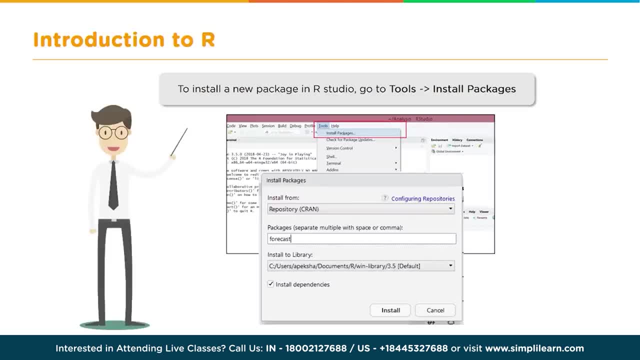 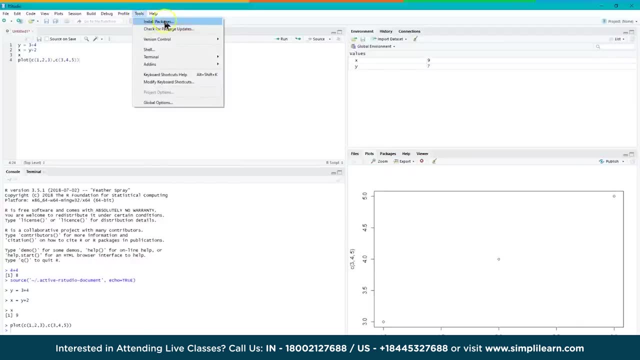 packages you can build And then you'll pick out the packages you want and separate multiple with spaces or commas So you can install numerous packages at the same time. In this case we're installing the forecast package And you can see down here. I just type in: 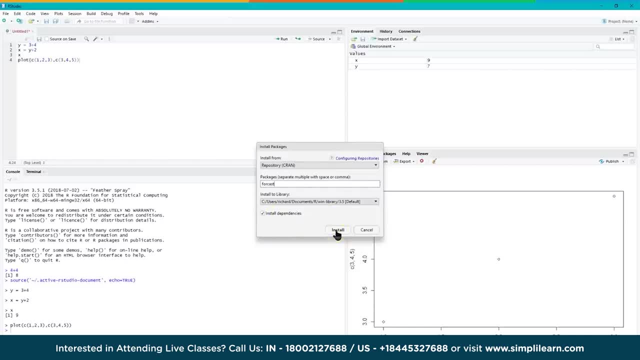 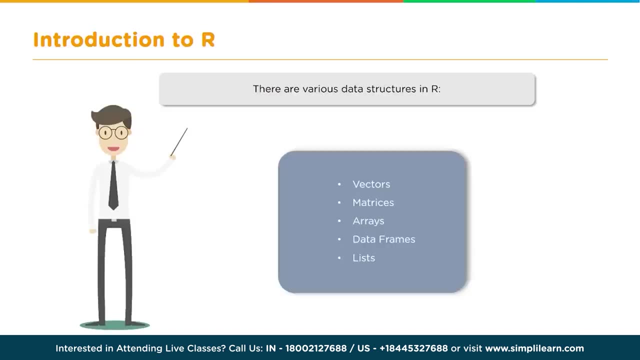 forecast Install all the dependencies It uses other packages to build on. It has those. Then just click on install And it's done. Before we cover the basic linear regression model, let's just take a quick look at some of the different parts of R. 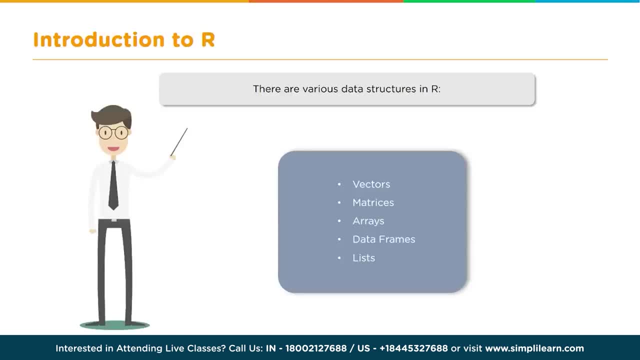 or parts of programming you'll need, or scripting First you need to know there are various data structures in R. We have vectors, we have matrices, we have arrays, data frames and lists. Vectors is the most basic data structure, If you remember, vectors are a location and a direction. 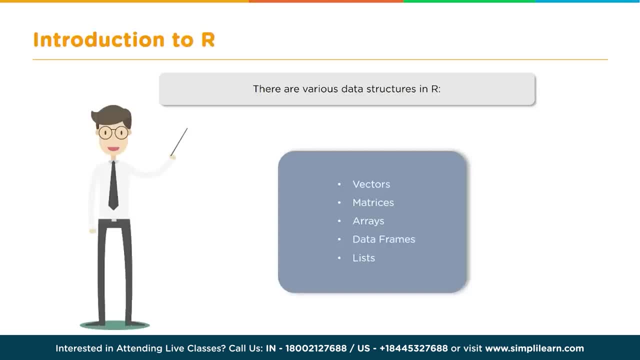 They're generally defined, Although vectors- when you're talking about scripting- can contain numerous different values. You could have vectors with 4,, 5,, 6,, 7, 8 different values in it. For example, a picture on the computer might have. 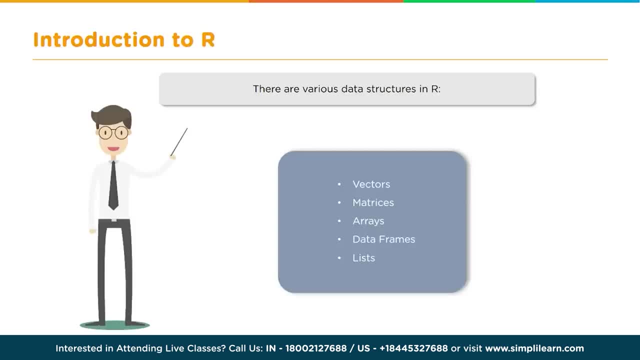 the location of the pixel and the number for the red hue and the green hue and the blue hue. So now you have something with 5 different numbers in it, consisting of that. vector Matrixes allow you to move stuff around, So you might have a 2x3 matrix that you switch to. 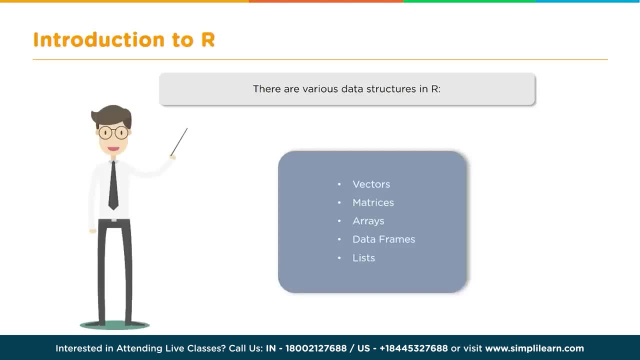 a 3x2.. We looked at an xy plot earlier. It might be that you have 10 different numbers and each one has two values- xy, and you need to switch that matrix. So then you have two arrays of 5 numbers. Arrays are just that: a collection. 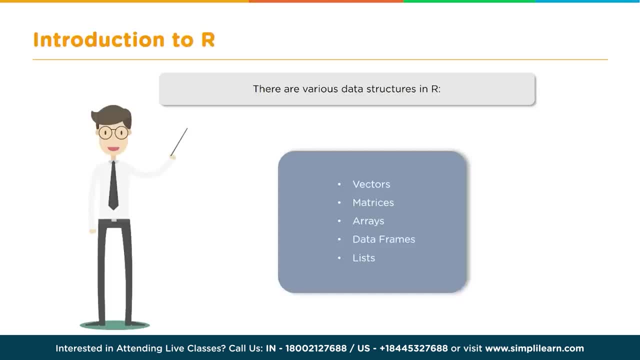 and you can have arrays of arrays of arrays. Data frames have labels on them, which makes them easier to use. So usually we use a lot of data frames when we're working with data because they're just easy. You can have a column and you can have a row, So think of rows and columns. 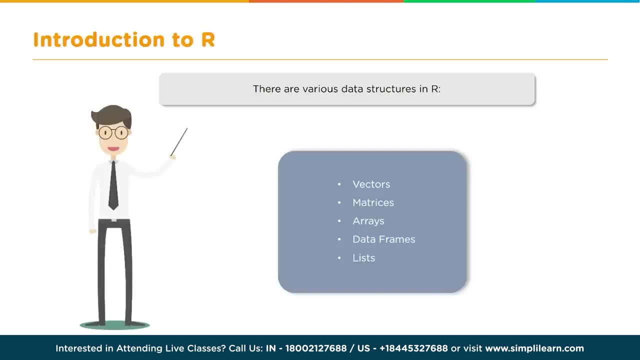 when you see the term data frames And then lists are usually homogenous groups, So in R you're usually looking at similar data that's connected in the list. So the first thing we do, before we're even importing the data, you should have the data ready So we need to look at 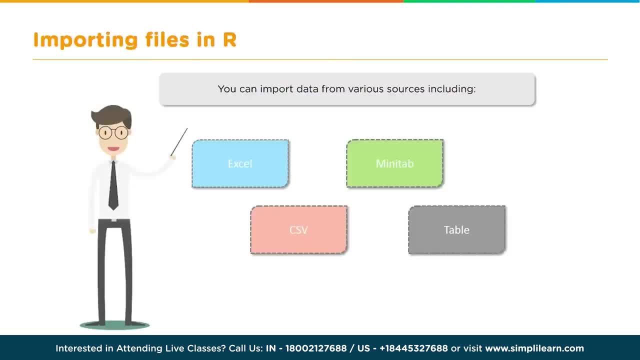 the data and see what's going on. You can import data from various sources, including Excel, Minitab, CSV, Table text files. CSV is usually a text file. comma separated variables, tab separated variables- There's all kinds of different options here- And importing the 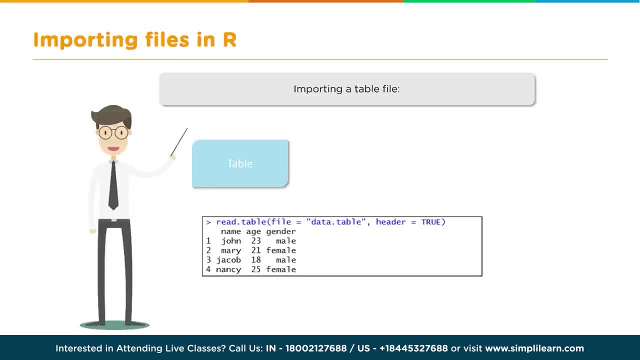 table is very simple. We have table read. table file equals data, table header equals true. And let's just take a closer look at what we're talking about here. Scratch the closer look. I didn't realize it was just, for example, 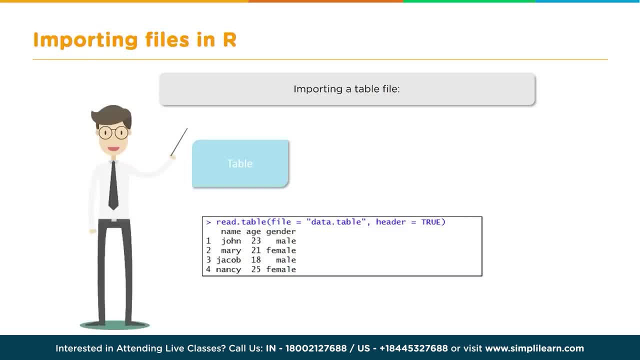 So importing a table file is pretty simple. You read: dot table file equals data, dot table. So whatever the name of the file is, comma, header equals true. So if there's a header to it In this quick flash, they have name age. 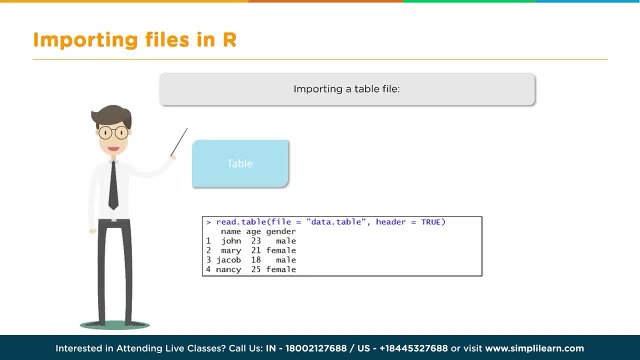 gender. We'll actually do this in R with another data set in just a minute, But you can see it's very easy to read. A lot of people use R, even in other programming languages, so they can quickly look at the data before they even start analyzing it. 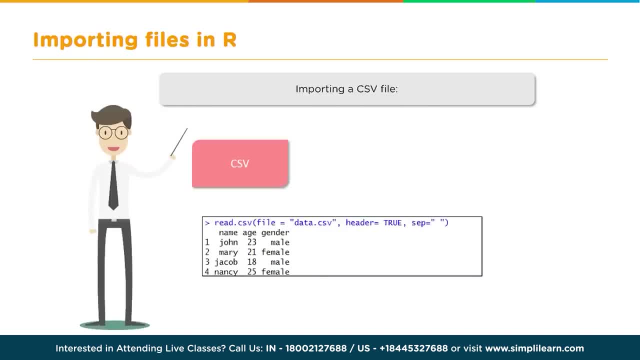 CSV file same thing. Read dot: CSV File equals data, CSV Header equals true Separation equals space. So in this case, even though CSV stands for comma separated variable, this one is separated by spaces And they have the header name, age, gender. 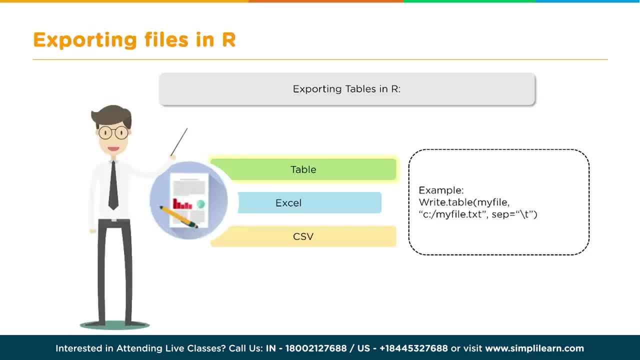 So it's the same file saved as the CSV file, And there's also Excel. Excel has its own issues as far as making sure you know what the tables are and the headers are, But you can see that each one of these is easy to import. 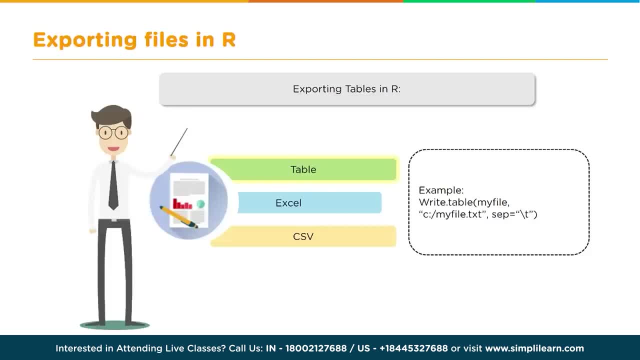 So just like it's easy to import the data, you can also export tables in R. So you can see here: write dot table my file: see my file. dot text comma separated And the scoop T just means it's tab separated. So if you're using tabbed files on there, 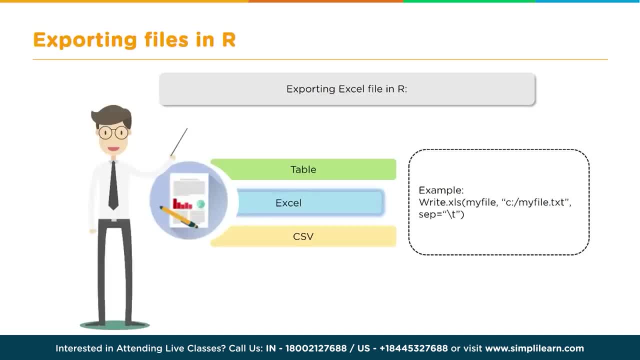 Example: Excel, So you can write a dot XLS to my file. In this case they did a text Separation equals scoop T, So it's a tab separated for an Excel file. CSV: same thing. Very easy to write a CSV file to your computer once you've changed. 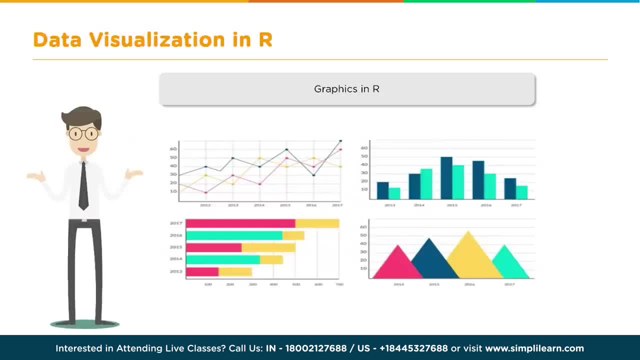 the data or altered it, depending on what you're doing with it, And once we have our data imported and we can save it afterwards and export it. graphing Visualization in R is very powerful and it's quick. Love doing this before even exploring the data. Sometimes you just want to graph it to see. 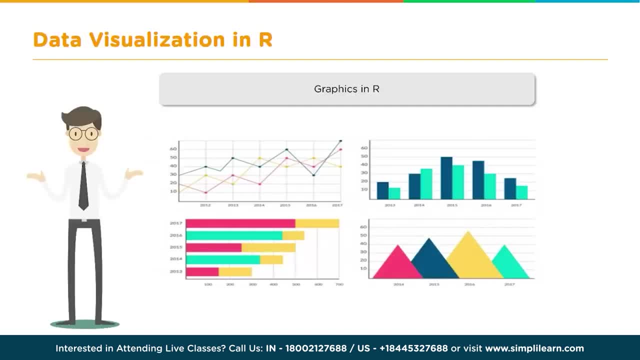 what it is there. So you have an idea of what you're looking for. So graphics in R cover a huge amount of different things. R includes a powerful package of graphics that help in data visualization. These graphics can be viewed on screen, saved in various formats, including PDF. 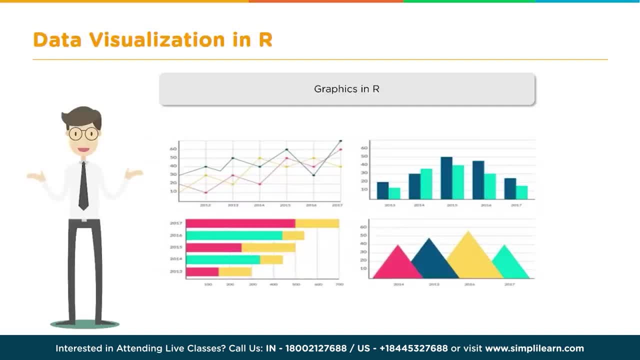 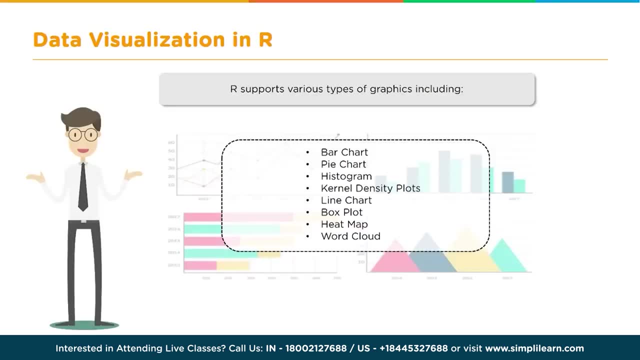 PNG, JPEG, WMF and PS Can be customized according to varied graphic needs. You can copy and paste in Word or PowerPoint files. R supports various types of graphics, including bar chart, pie chart, histogram, kernel density plots, line chart. 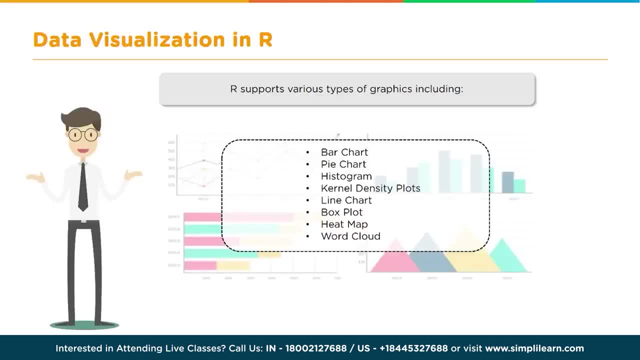 box, plot, heat map, word cloud. There's even some more obscure ones, But these are the main ones that most people use. I know I use a lot of heat maps, But word clouds are a lot of fun if you're doing websites. 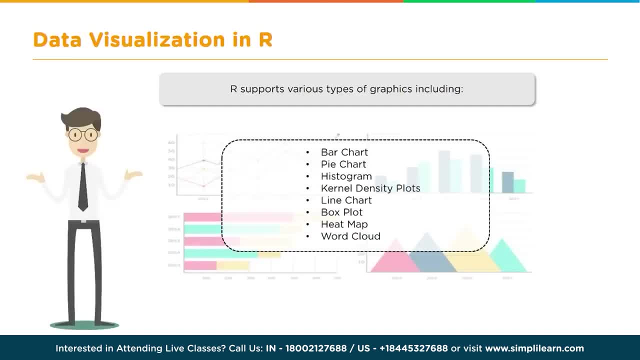 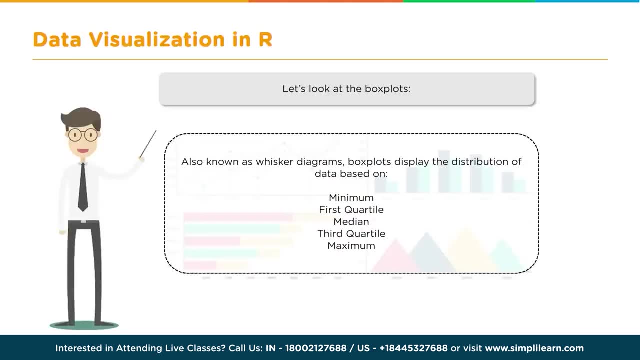 and word analysis And histogram is very popular. All of these are very widely used. Let's look at the box plots, Also known as whisker diagrams. box plots display the distribution of data based on minimum, first quartile, medium, third quartile and maximum. So right off the bat we can use a box. 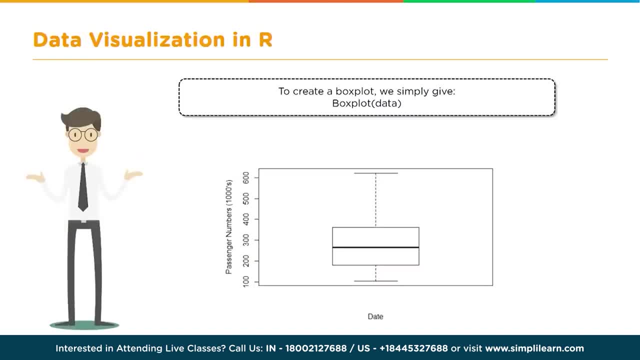 plot to explore our data with very little work To create a box plot. we simply give a box plot and the data Very straightforward So we might have passenger numbers in the thousands. I guess this is exploring data dealing with airplanes And you can see here they just have a simple 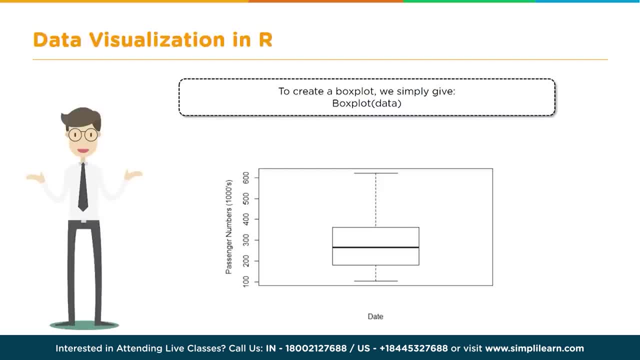 plot. If you break it down, you have your. if we go back one, you'll notice we have a minimum, a maximum, our medium first quartile and third quartile. Let's just break that apart. You can see the line on the bottom is your minimum. Your line on the top is: 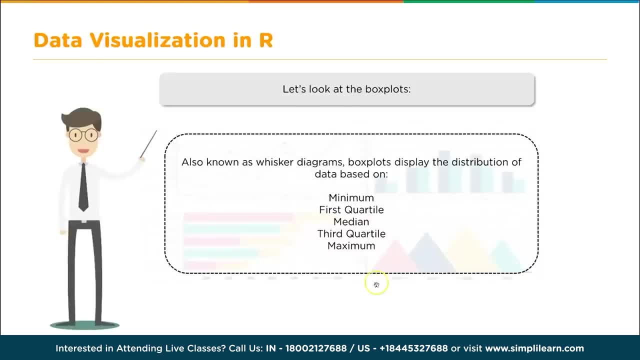 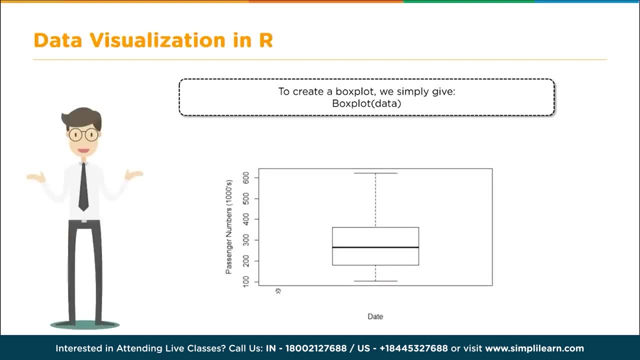 the maximum. You have your medium and your first quartile right there, First quartile and third quartile, And the way a lot of times you read this is things that are above the box are outliers and things below the box are outliers And what's in the middle of the box? 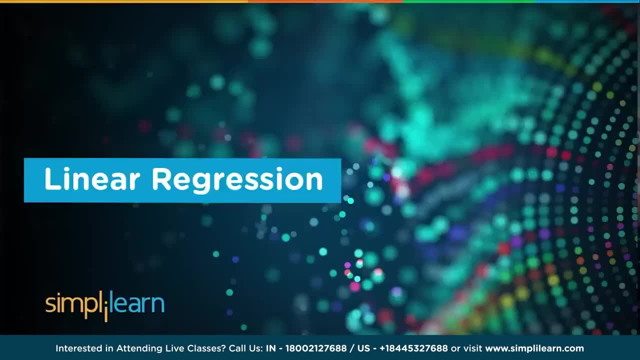 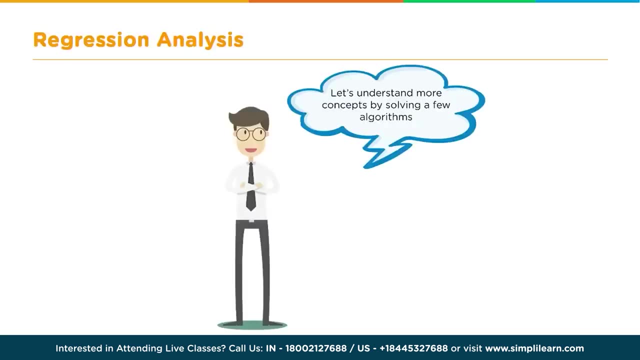 is usually the data you're looking at. Linear regression. Now we have a few tools of what R can do. Let's look at the theory behind linear regression and how that applies to what we're going to use in R. Let's understand more concepts. 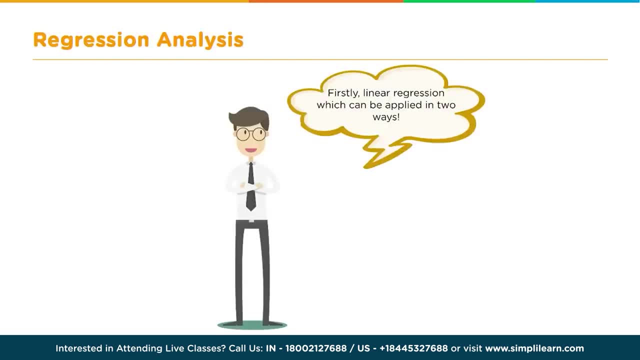 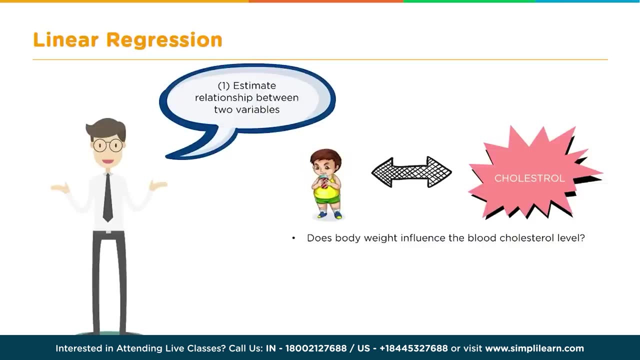 by solving a few algorithms. Firstly, linear regression, which can be applied in two ways. One: we can estimate the relationship between two variables: Does body weight influence the blood cholesterol level? So we just want to know if it's even a valid connection or not. 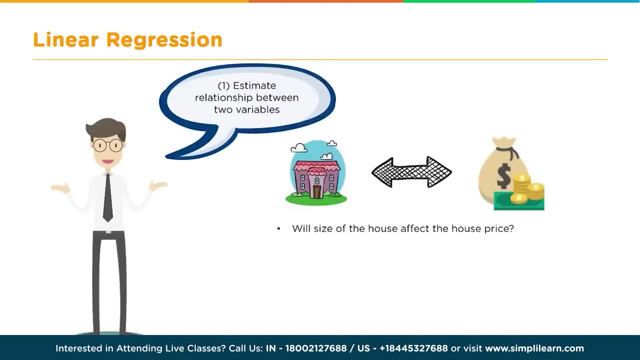 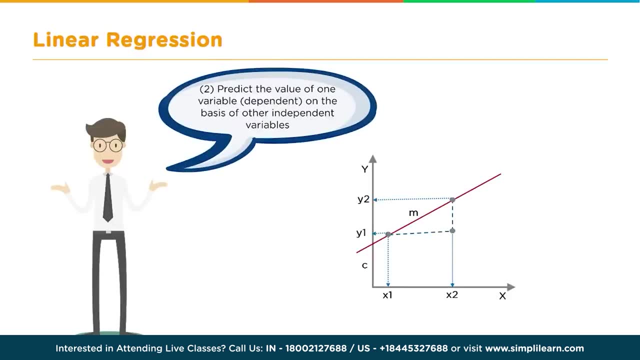 Will the size of the house affect the house price? So we can estimate the relationship between two variables also, And then we can predict the value of one variable dependent on the basis of other independent variables. So once we know they're connected, we want to use that to go ahead. 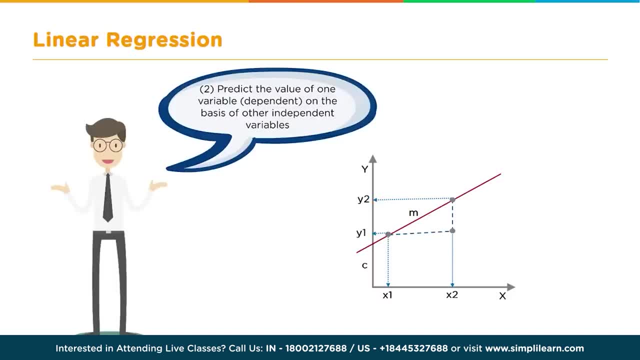 and predict it. In the cases above maybe the body weight versus cholesterol. So the more, the higher the body weight is probably the higher cholesterol. So first we explore: is there a connection? And if there is, can we actually apply that? 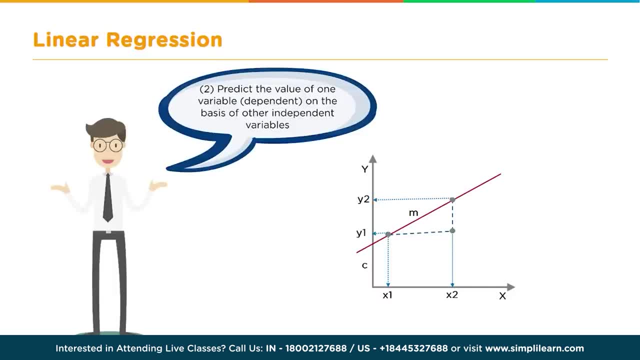 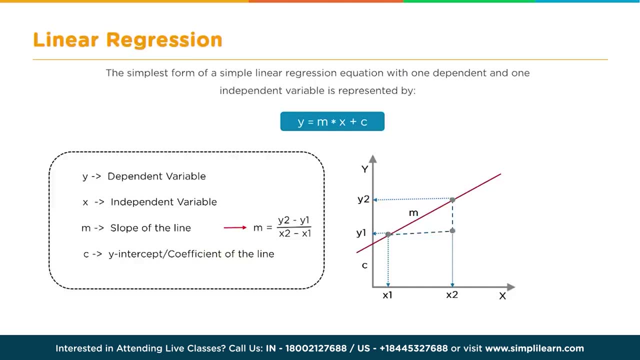 to a linear regression model where we can see how they're connected. Same thing with house pricing. The simplest form of a simple linear regression equation with one dependent and one independent variable is represented by: y equals m times x plus c, y being the dependent. 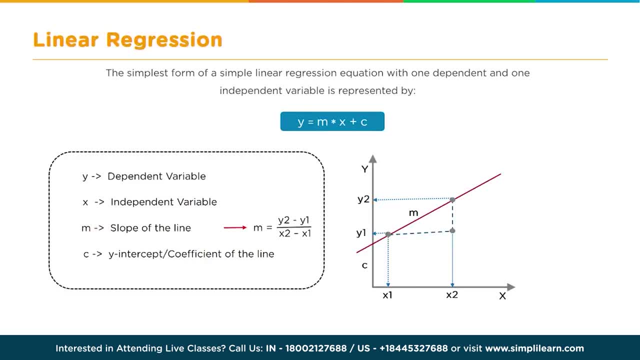 variable, x being the independent variable, m being the slope of the line which you can see over here on our graph, equals y2 minus y1 over x2 minus x1, and c being the intercept or the coefficient of the line. Now you don't have to memorize all the formulas. 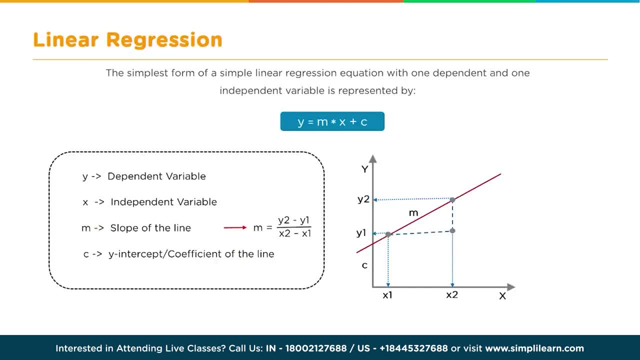 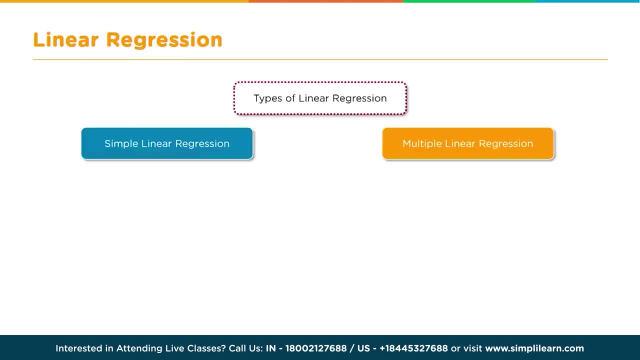 we're going to go in here because most of R does this for you, But you do need to know what's going on in the back end so that you can understand if it's working or it's not working where the problem lies. Types of linear regression. 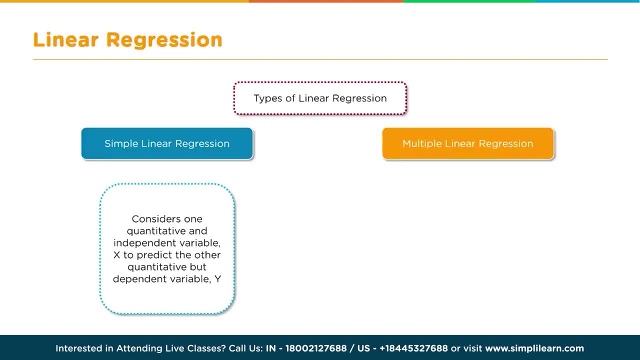 there's simple linear regression: considers one quantitative and independent variable, x, to predict the other quantitative but dependent variable, y. And that's the formula we just saw: y equals m times x plus c. And then we have multiple linear regression. 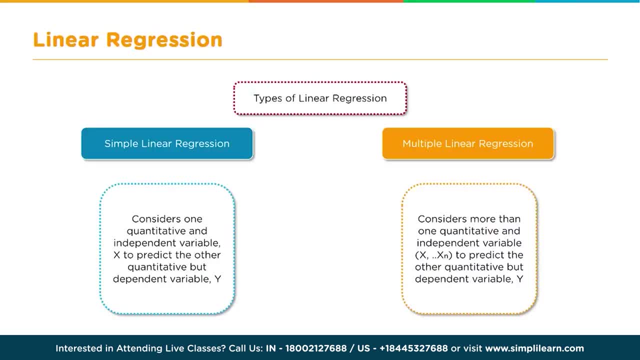 considers more than one quantitative and independent variable. So instead of having just x, you have x of y equals m times x plus c. So instead of looking at just body mass, we might also look at height. So you have body mass and height would be two independent variables. 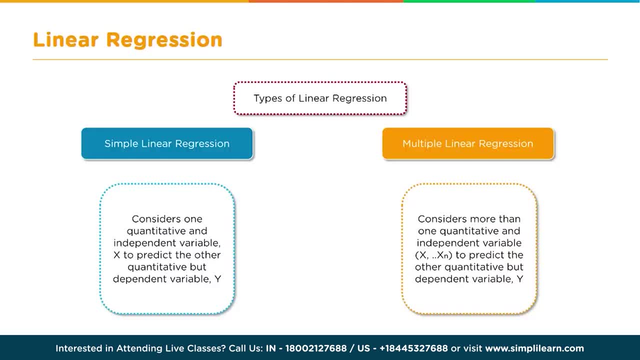 Housing prices might have to do with the distance to a certain area, So location might be one of the variables, along with the size of the house. Let's consider a sample data set with five rows and find out how to draw the regression line. 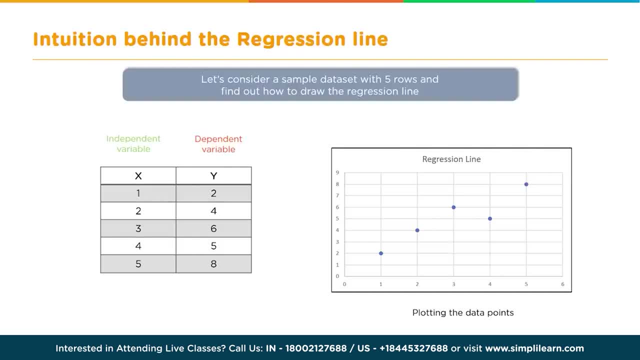 So in here you can see we have independent variable y. so in here you can see we have independent variable and our dependent variable, where we've taken some random data. In this case we have 1,, 2,, 3,, 4, 5 for x. 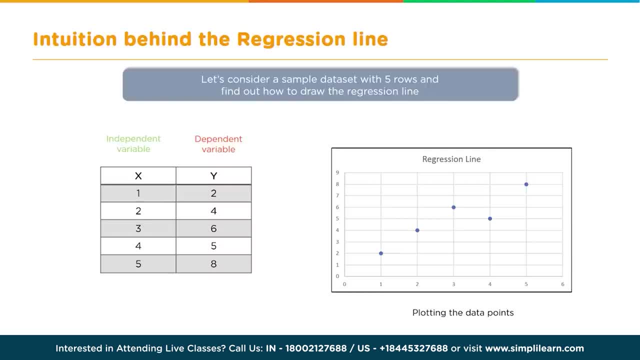 and we have 2,, 4,, 6,, 5,, 8 for y And the first thing we do is we might plot it. If you look at the plot you can see that it has a nice line through it. Just eyeballing it you can guess that there's probably a linear 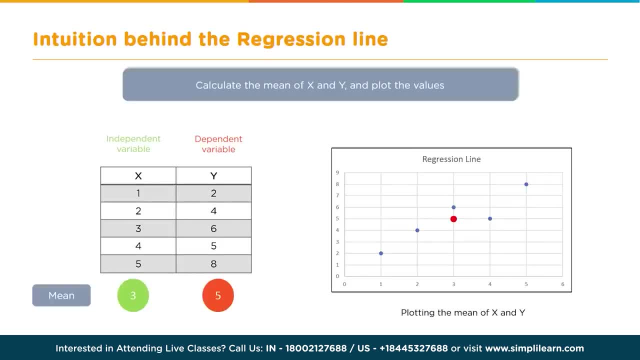 regression model that will fit this data. Then we go ahead and calculate the mean. We calculate the mean of x and the mean of y And you can see that we plotted that on there. 3, 5 for this particular data set. 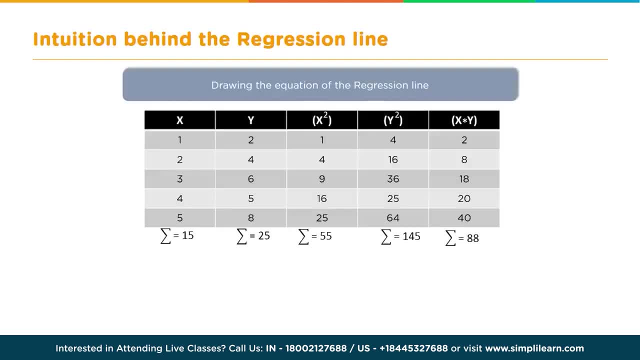 And so, drawing the equation of the regression line, we'll go ahead and take a summation of x, a summation of y, take a summation of x squared and a summation of y squared, and then x times y. This is why it's so nice for the computer to do this work for you. 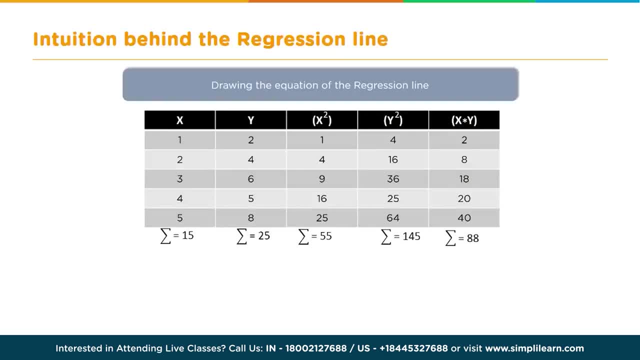 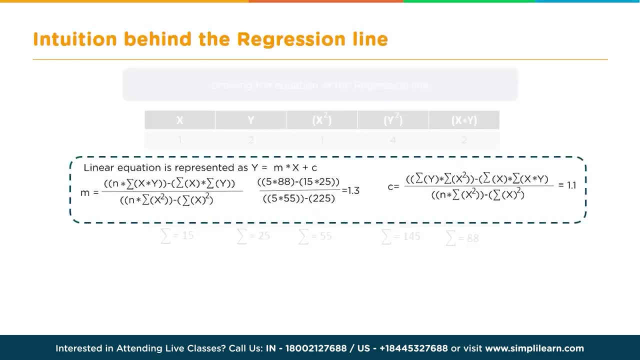 because I don't know about you. I hate sitting there with a calculator and if you have just five variables that would be very long, not a big deal. but if you're doing hundreds of variables it's definitely much easier to let the computer do it all. So the intuition behind the regression: 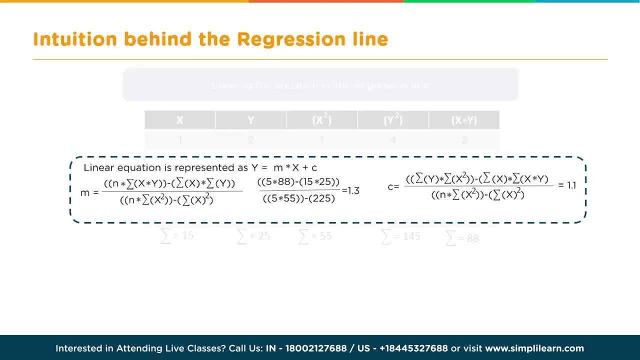 line breaks down to the linear equation, which is represented as: y equals m times x plus c. In this case, m equals this very lengthy formula where you have your summations. So all the values that we've already computed fit right into this equation, And so you have n being the number. 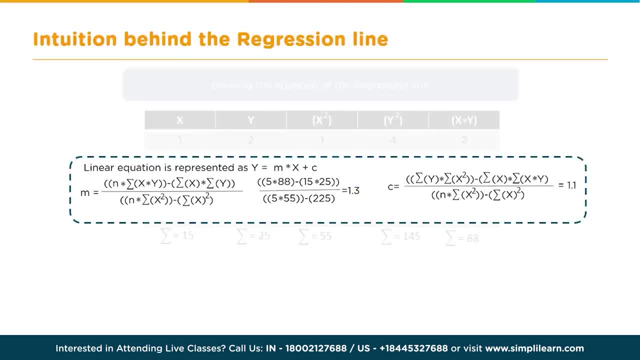 of variables. that's what the n stands for: Your x times y. we computed the sum of x sum of y over the number of variables times the sum of x squared, minus the sum of x squared, and then, of course, we have you put the numbers in and you get a value of 1.3. 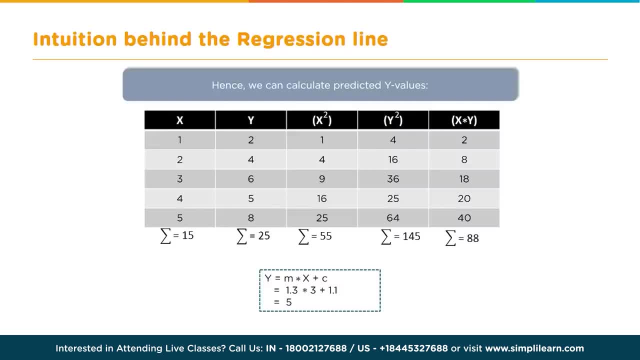 and you find out that your c is equal to 1.1.. Once we have this formula, we can easily compute the y values. y equals m times x plus c equals 1.3 times 3 plus 1.1 equals 5.. And this would be the example of 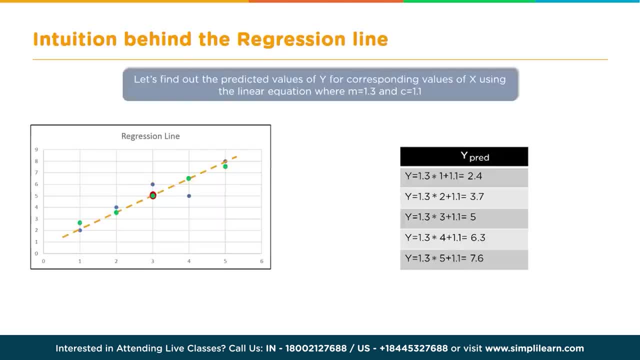 x equals 3,. you could also put in x equals 6,, an unknown value. Let's find out the predicted values of y for corresponding values of x using the linear equation, where m equals 1.3 and c equals 1.1.. 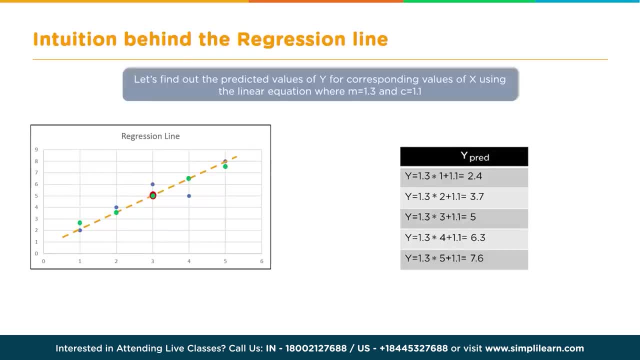 So here's our regression line and then you can see if we put in all the numbers 1,, 2,, 3,, 4, 5, we don't get the exact prediction because it's a line. through the data You'll see that it's ever so slightly off: 2.4, 3.7,. 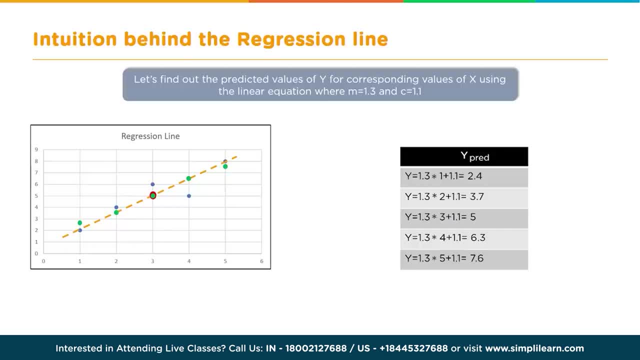 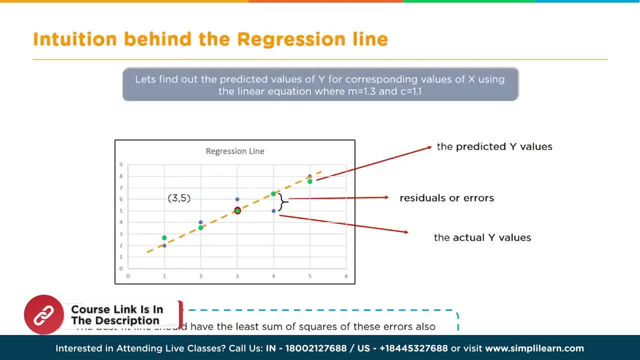 5,, 6.3, 7.6.. But it is a good estimate of what the data is going to generate. Let's find out the predicted values of y for corresponding values of x using the linear equation, where m equals 1.3 and c equals 1.1.. The best fit. 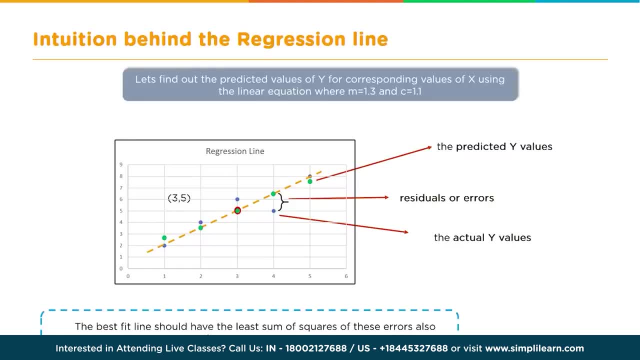 line should have the least sum of squares of these errors, also known as e-square, The predicted y value, residuals of errors, the actual y values. So one of the things we're looking at when we put this information together is we want these distances to be. 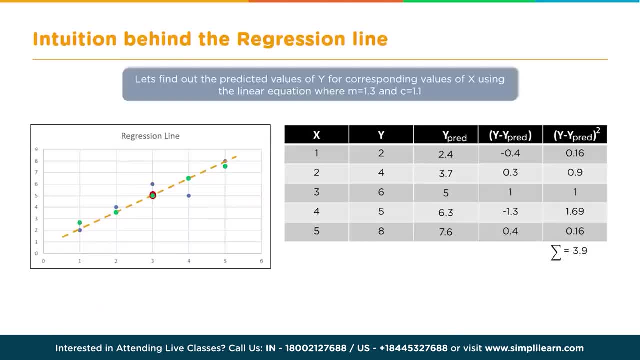 minimized, So it has the smallest amount of error possible. Let's find out the predicted values of y for corresponding values of x using the linear equation, where m equals 1.3 and c equals 1.1.. And here you can see we've done. 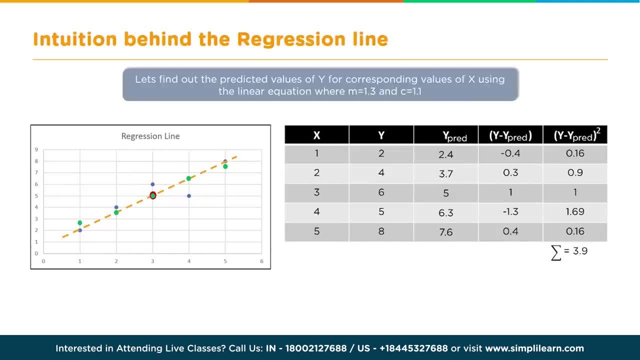 the same kind of chart. We have our y predicted and then we have the actual y minus the y predicted, Because we are looking for the error squared or the e-squared values. The sum of the squared errors for this regression line is 3.9.. We check this error. 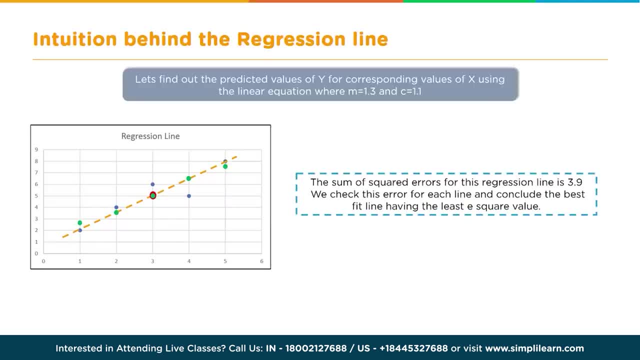 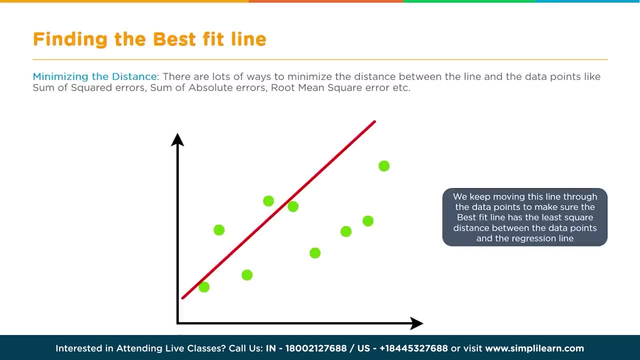 for each line and conclude the best fit line having the least e-square values. Minimizing the distance: there are lots of ways to minimize the distance between the line and the data points, Like sum of squared errors, sum of absolute errors, root mean square error, etc. And no matter. 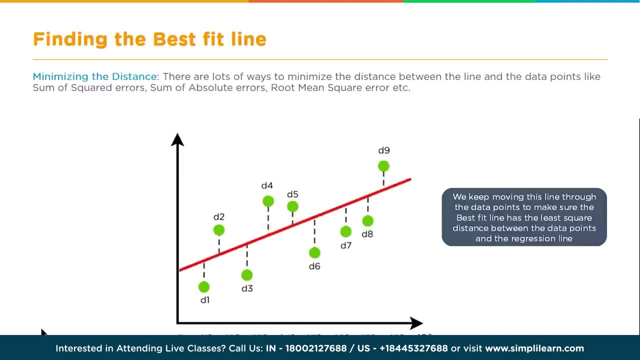 how you compute the errors you can see here. this is what it's basically going through. It's taking the line and slowly adjusts it until it has the minimal error available, the minimal distance between the line and the different data points. Use case. 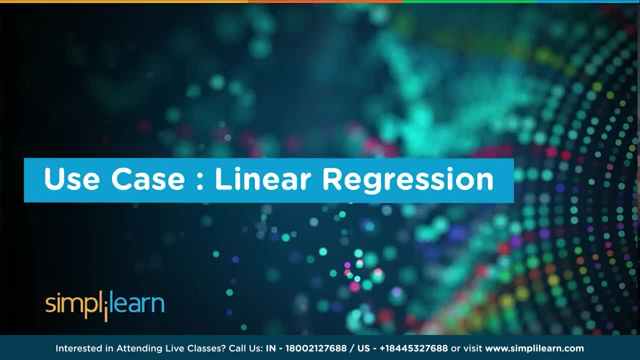 We'll start with linear regression and then we'll jump in and also do a decision tree so you can see how they are same and how they differ and the way they function and what they're used for. And while we're going through the use case, you can 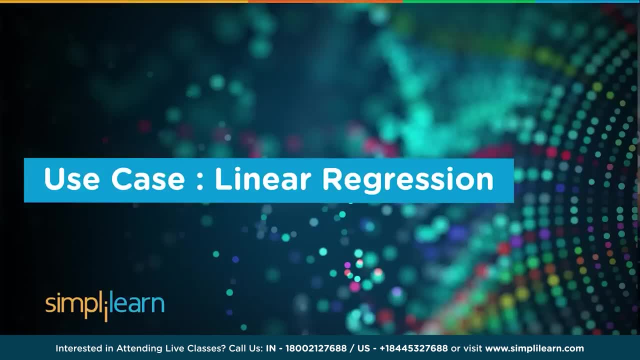 start linking the theory behind it connected to the actual use. And as you connect those dots you can see that by making changes in the model based on the theory, you can also fine tune it. We'll talk about that briefly as we go through this For this. 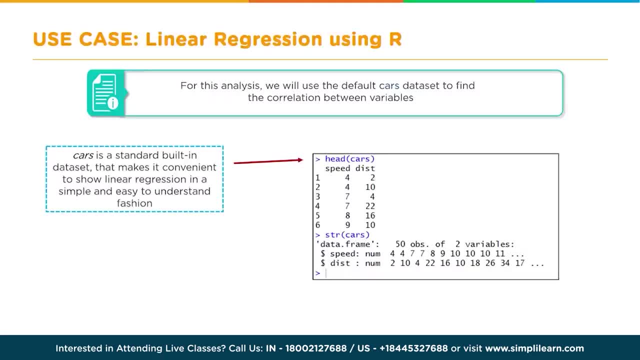 analysis, we'll use the default CARS dataset to find the correlation between variables. CARS is a standard built-in dataset that makes it convenient to show linear regression in a simple and easy to understand fashion, And we'll start with head cars and string cars Now. 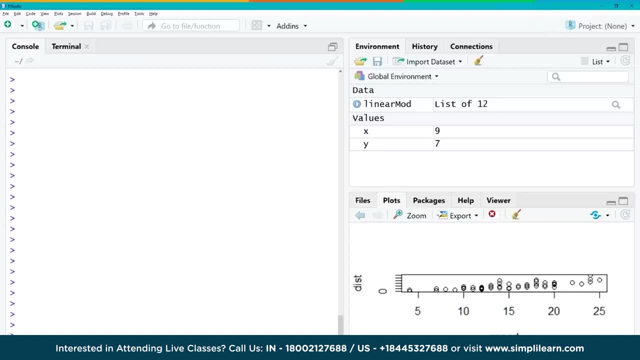 I've gone ahead and removed the script on here to make this easier to see And we don't have to do any kind of importing of data because it's already in there. I'm just going to type in head and cars and hit enter, And what you're going to notice is it's going to. 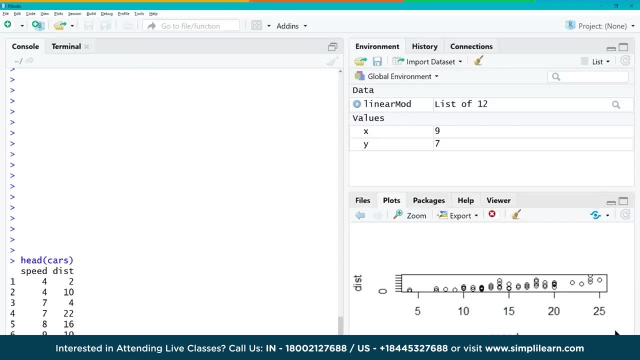 display the first six rows- 1,, 2,, 3,, 4,, 5,, 6, and you'll see speed and distance. Now this is a little bit like a spreadsheet, so if you're using an Excel spreadsheet it should look the same. And this is a standard data frame, kind of. 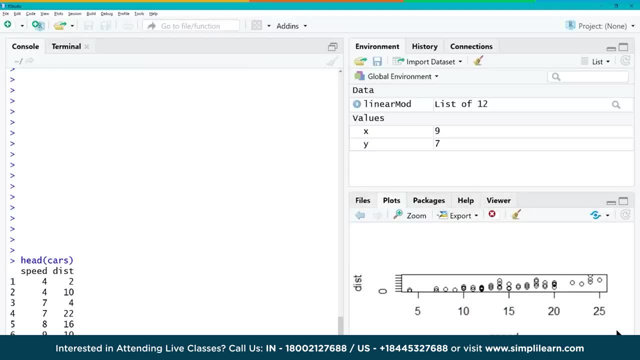 setup. In this case, whenever you say head, it usually lists the first number of rows, depending on your package. In R it starts with 1 and then it does the first six rows String. when we do string of cars, it's going to break it down and show us that it's a data frame. 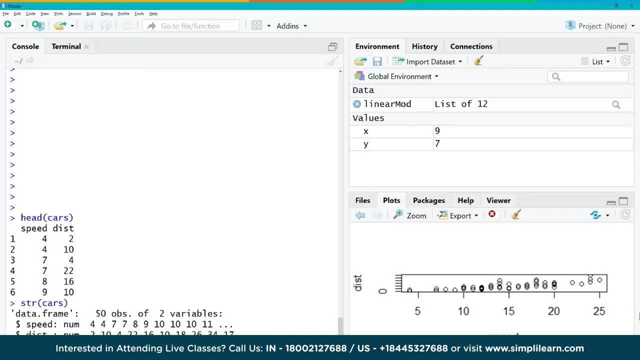 It has 50 objects, that's with the 50 OBS of two variables. And then we have speed. the first variable is going to be a number. that's what NUM stands for: 4,, 4,, 7, 7,. it just starts listing the data there. 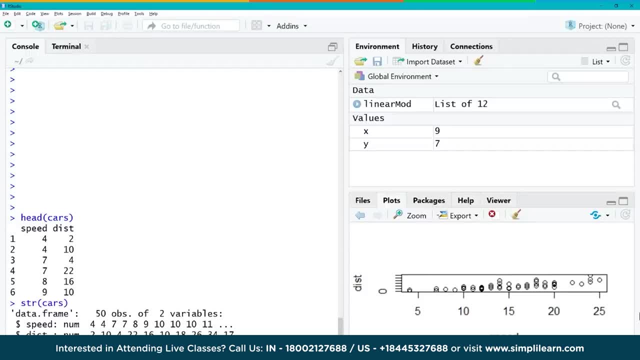 And distance. Now I'm assuming the speed is the speed of the engine. Otherwise, if it's the speed of the car, then the distance should always be the same, and that would be kind of silly. But this is the speed of the engine and based on the speed of the engine, can we correlate? 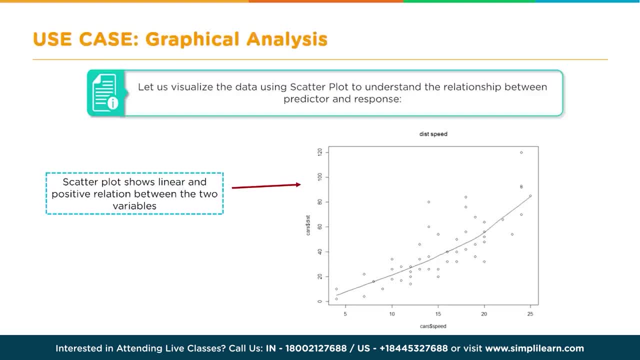 that to the distance. Let us visualize the data using scatterplot to understand the relationship between predictor and response, And I want you to notice that in this slide, a line has been drawn through the data. Now, when we first start with data, you don't have that line. So as we plot it, I want you. 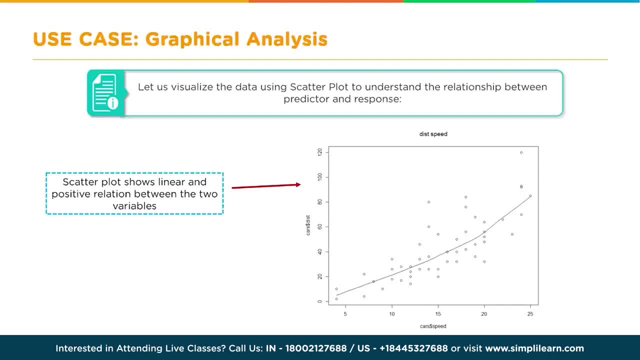 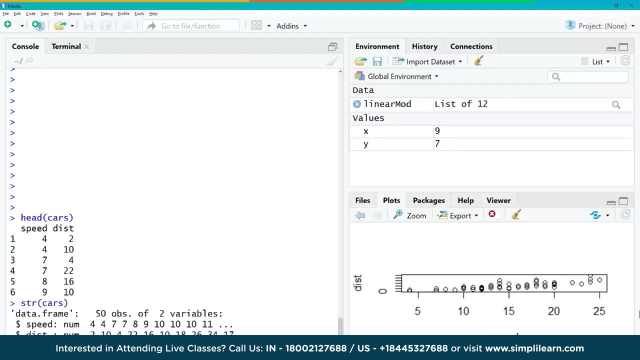 to kind of visualize that line there and just kind of say, hey, does this stuff kind of scatter around a line or not, before we actually create the model And we simply do plot, and I'm going to do a shorthand here- cars and I hit enter. 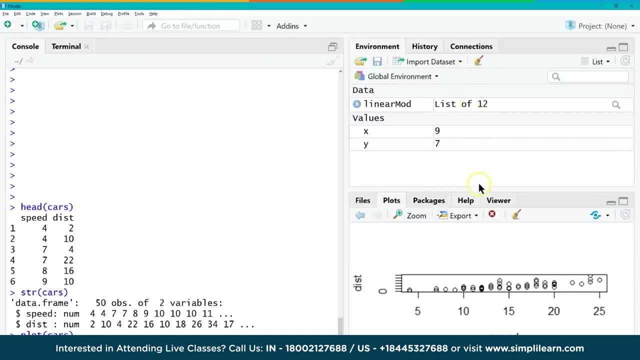 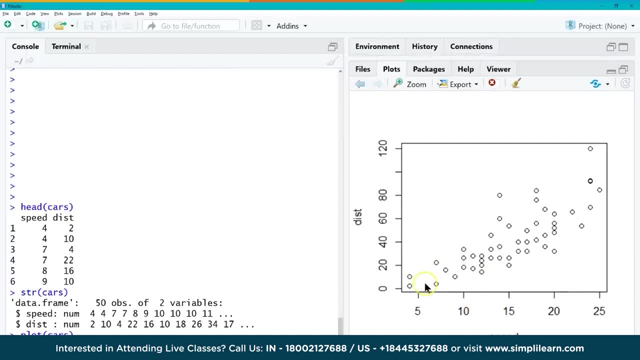 and it comes over here to the right and plots our data for us. Now, because there's only two variables, I don't have to do anything special. I'm going to expand this over environment so we can see it And you can see. you can just visualize a line right through the data. 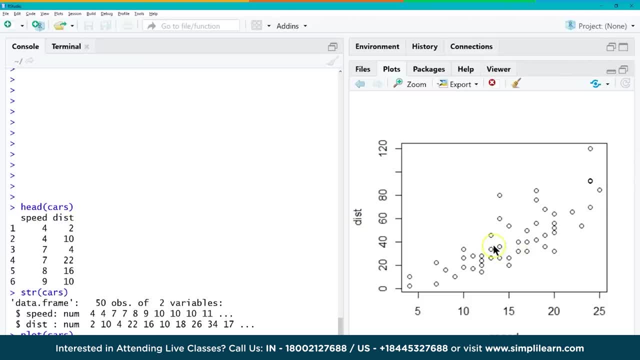 and it's all clumped along that line, which makes it really nice for doing a linear regression model. Now I did something a little tricky here because I'm very lazy. I typed in plot cars A lot of times. you don't want to do that. 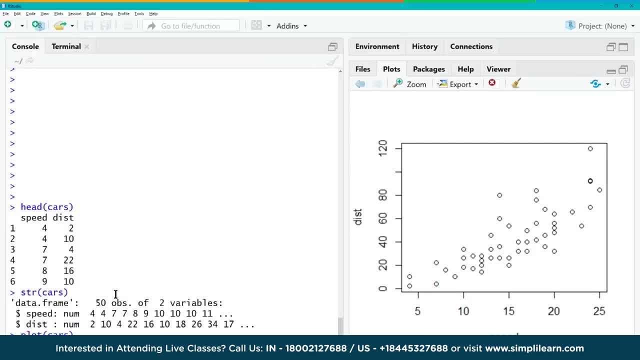 because you don't want to plot all the data. We can do. plot, in this case, cars dollar sign speed, the first variable, cars dollar sign distance. When I do that, I get the same plot. All I'm doing is telling it to use just these two columns of data. 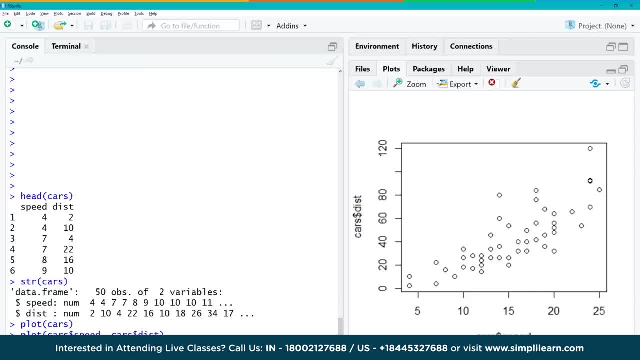 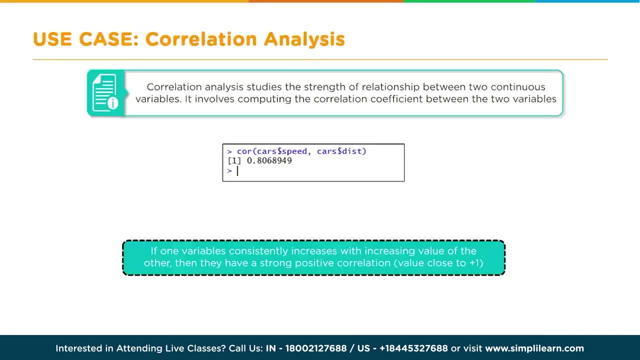 And although the first one is quick and easy if you only have two columns of data, the second one is what you really want to do when you're plotting data like this. You want to control which columns you're using, And then we want to do a correlation. 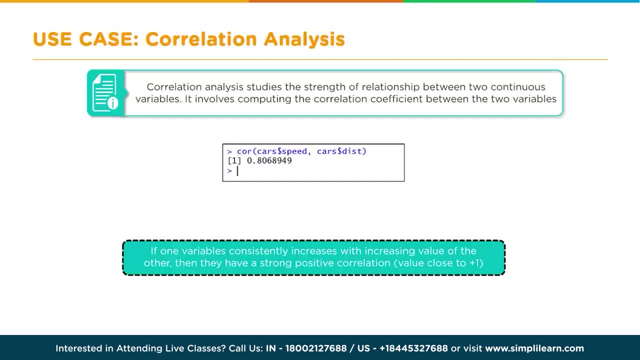 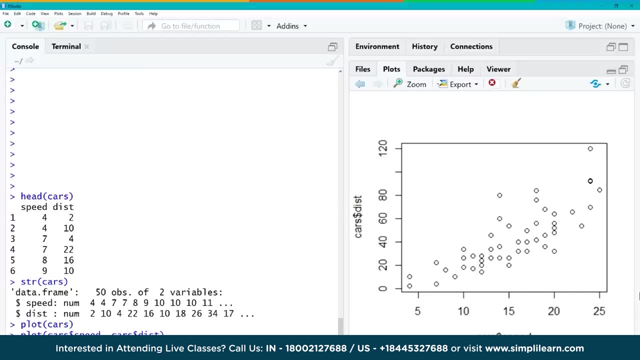 Correlation analysis studies the strength of relationship between two continuous variables. It involves computing the correlation coefficient between the two variables. If one variable consistently increases with increasing value of the other, then they have a strong positive correlation, a value close to one. And again I can just type in correlation cars. 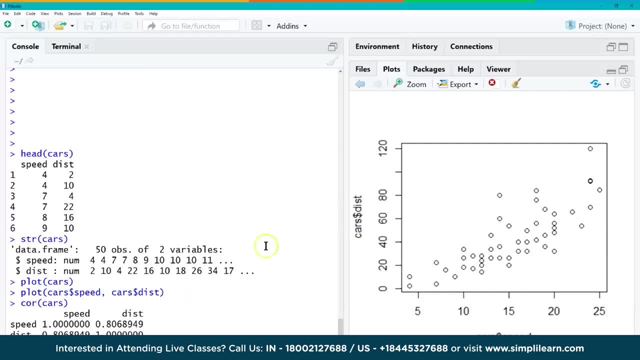 the short form, and we can see we have a nice correlation going on there between the two. What we really want to do, though, is we want to correlate cars, and then we're going to do the speed cars and the distance, And so, when you look at this, I actually hit the enter. 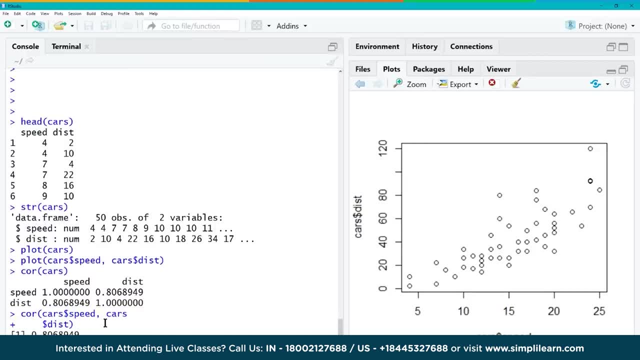 key in the middle of that, which is fine. You can, in R, do it line by line. So if you're trying to do a bunch of different columns, you might want to do that to make it easier to read. And you can see, here I get the .806894.. 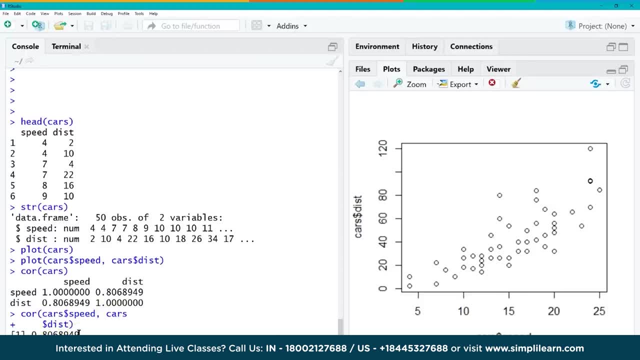 The closer this is to one, the more these correlate. So I'm saying there's a pretty good correlation, positive correlation, between the two variables And if you look at it, when I did just cars, which did the correlation over all the variables, 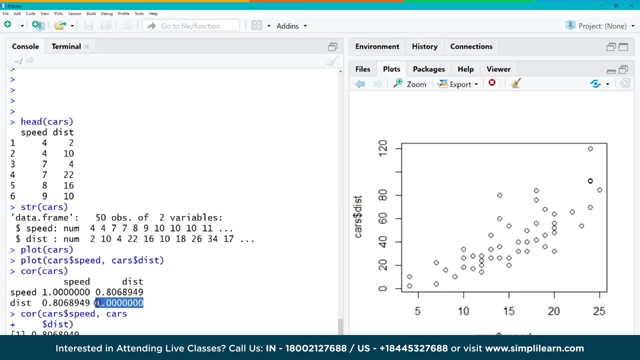 you'll see that speed correlates with speed 100%, because they're the same. That's just the nature of that. But when you look at speed versus distance, we get the .806894.. And if you do distance to distance, you get also one, since they're. 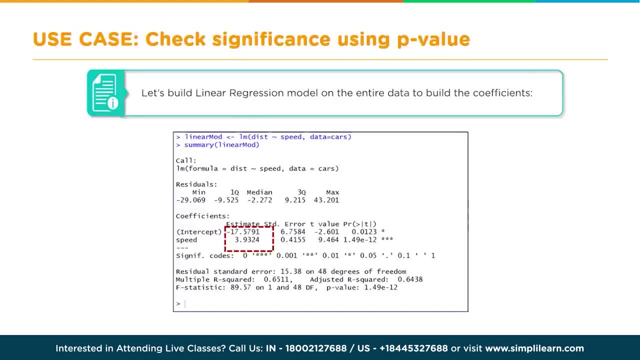 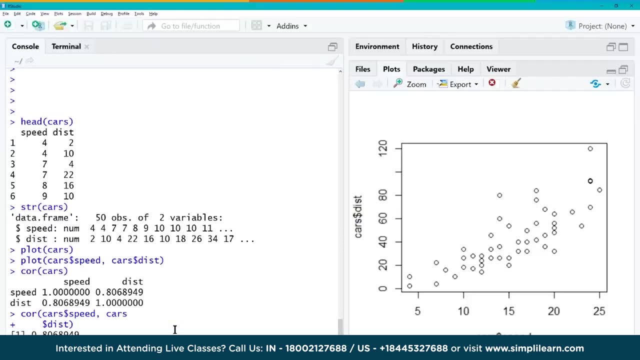 identical variables. So now it's time to build our linear regression model on the entire data set, to build the coefficients. Let's just take a look and see what that looks like Back in our console. I'm going to type in linear mod and in R we want to do: 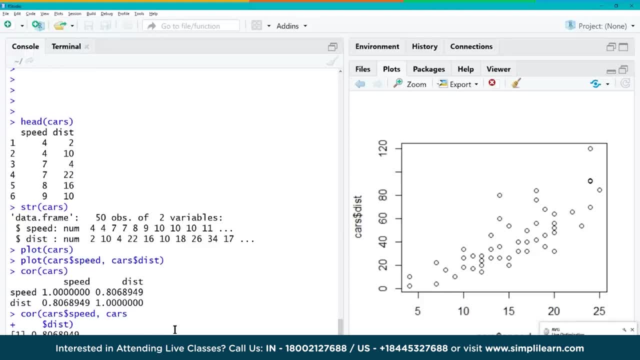 the arrow, kind of like an arrow on a line, or, in this case, the less than minus sign. That's the same as assigning whatever we're going to put after it to this variable. So we're creating the linear variable. LM stands for linear module. 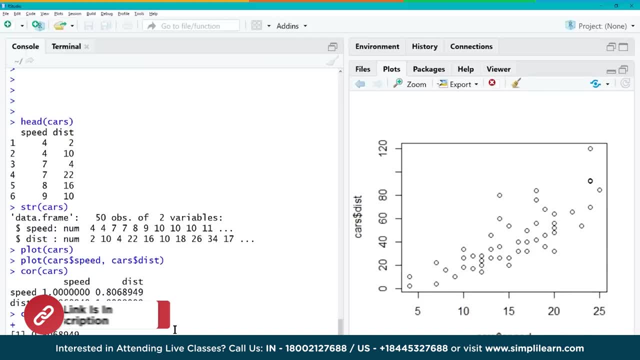 And we're going to look at speed and distance. So we put the little squiggly bracket between them. This lets R know we're going to deal with these two columns. comma data equals cars And when I hit enter on here, we've generated our linear mod. Now we want to go ahead. 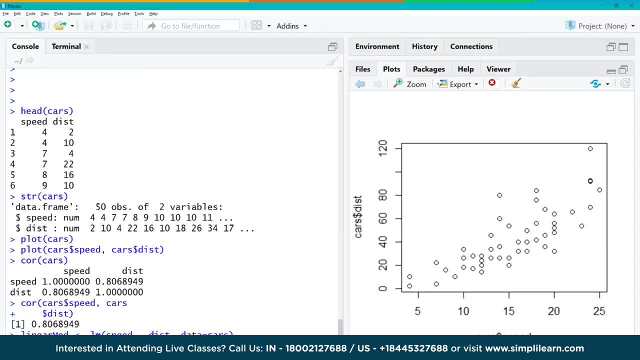 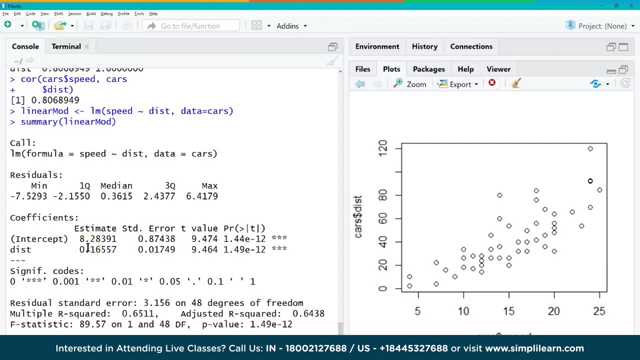 and summarize it And we simply do a summary and then brackets linear mod and it generates all kinds of information on our model So we can explore just how well this model is fitting the data we have right now. Now, if you've done linear regression and other packages and scripts you're going to 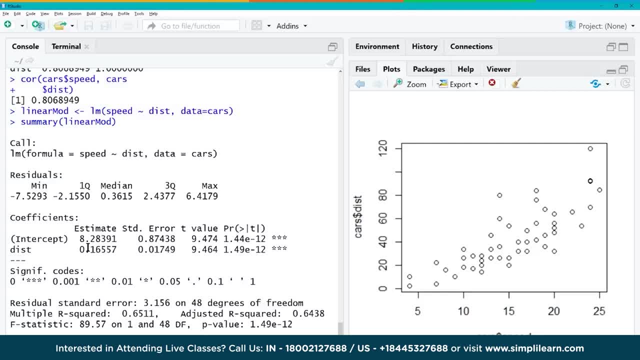 see that this is so easy to explore data in R. So even somebody who's working in, say, Python or Spark Hadoop, coming back to the R console to do some basic exploration of the data is very beneficial. And if you use just R, R goes into all kinds of different. 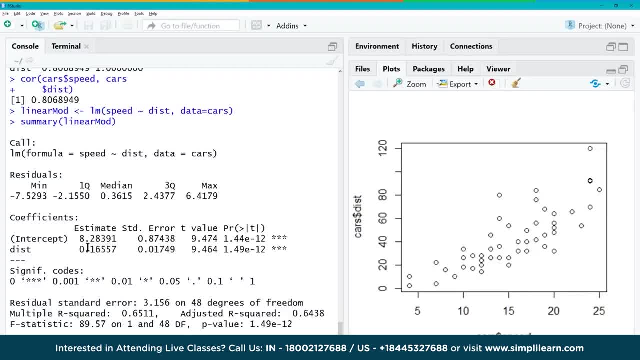 packages, and you can even do cluster computations through H2OR. There's a lot of cool things. This is what makes R so wonderful is how easily we can summarize something like a linear model. And to explore this data, let's go back to the slide And we'll see here where it says the residuals, the 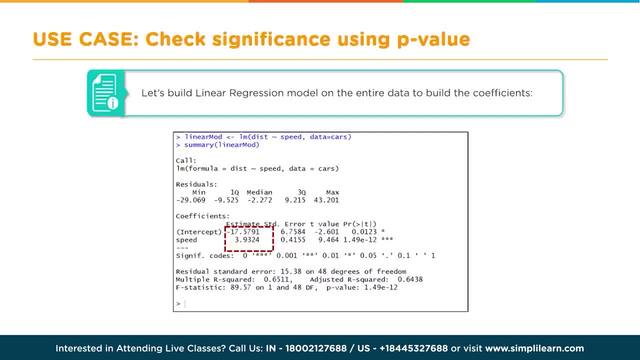 one Q stands for first quadrant median, third quadrant max coefficients, And what we first want to do is look at the estimate standard deviation on here And you'll see the intercept is at minus 17.5791, and speed 3.9324.. 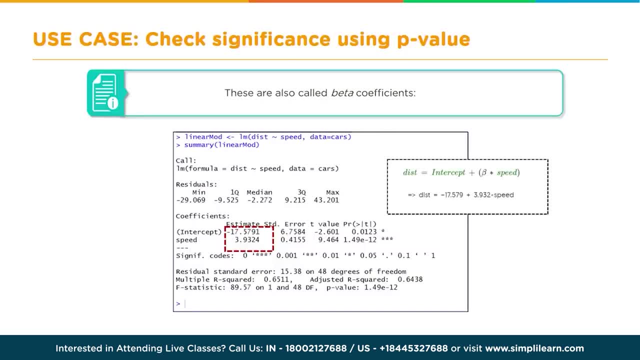 So we can compute: the distance equals to the intercept plus the beta times the speed, which just means that we can assign a distance equal to minus 17.579 plus the 3.932 times the speed. The value of p should be less than .05 for the. 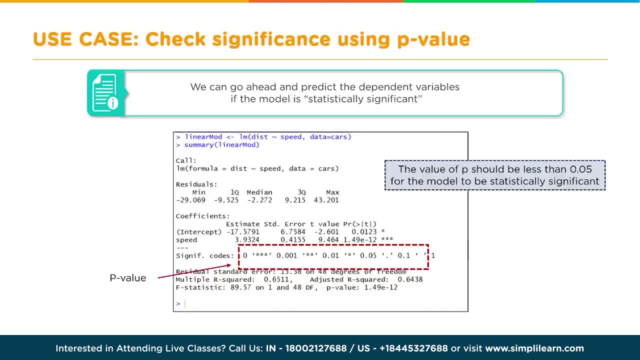 model to be statistically significant. And this is one of the things I love about R. You can see right down here we punched in the numbers and it even tells you the significant codes. So if you're trying to guess or remember, it tells you right away: hey, this 1.49 to the 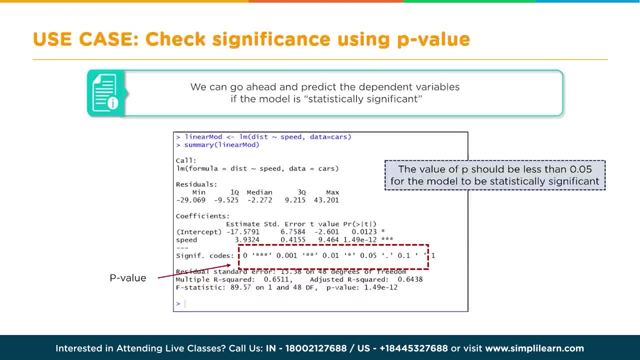 minus 12th is way below .001 on there, And it even puts three stars next to it. so you can see that that is a very high correlation. And you can see the .0123 gets one star because it is greater than the .05, or it's less than the .05.. So this: 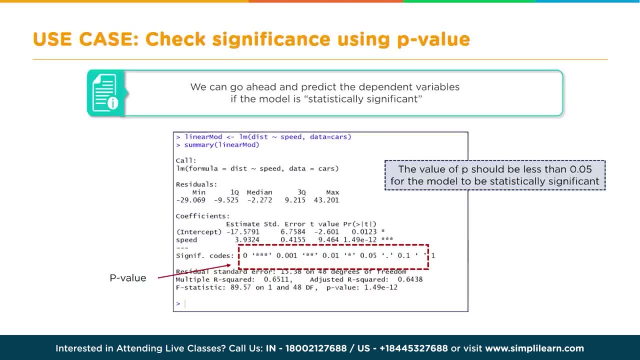 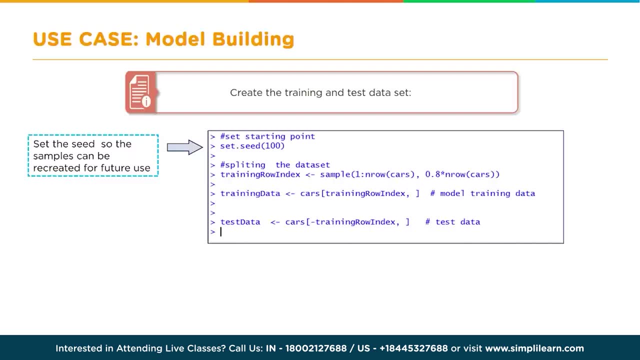 shows that there's a very high correlation. statistically is very significant. So now we're going to go ahead and create a training and a test dataset And the first thing we want to do is we want to set the seed so the sample can be recreated for future use. Remember, in all these different regression, 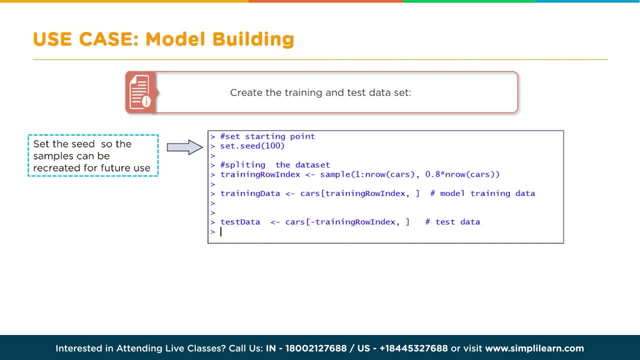 models. they usually have some randomization going on in the back to kind of fit it and guess where it's going to go. And if you want everything to match, you want to start with the same seed in that randomizer. That way it recreates it identical every time. 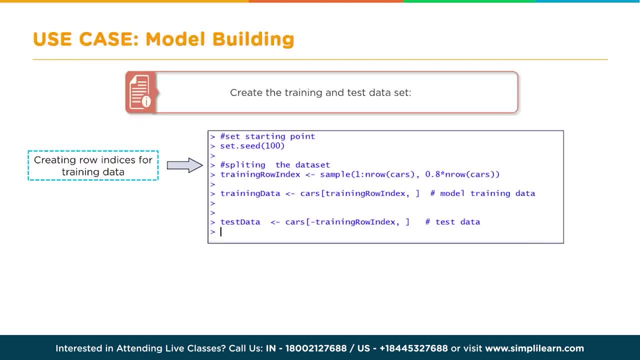 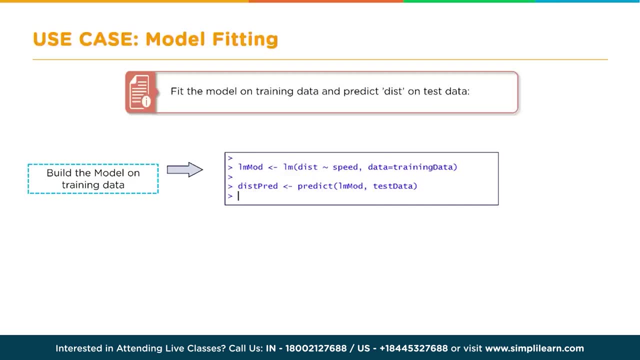 you run it on a different computer And just like working with data in any package, we're going to create indices for the training data and we're going to model the training data and then we're also going to do the test data and build our model on the training data. And let's walk through that. 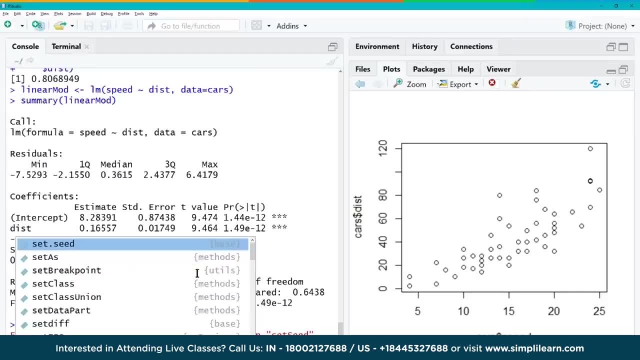 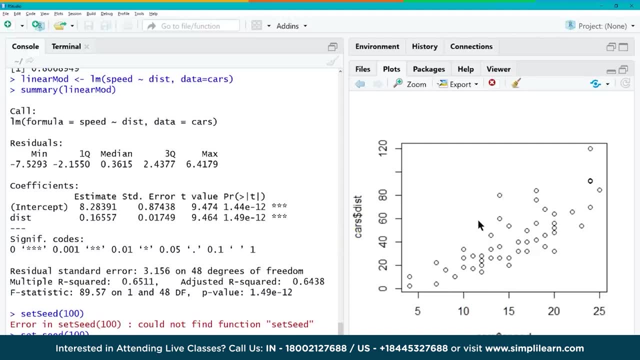 and see what that looks like in R- And I actually mistyped that one- Let's type in setseed to set our seed for the 100.. Let's go training row index and that's our name. we're making up for our variable And we're going to set that. 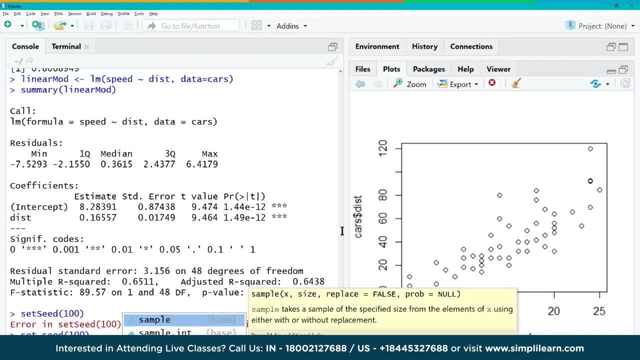 to sample. Now, sample is a command in R, so we're going to take a random sample of some of the data And then we're going to do 1 colon in rows- cars. So this is the number of rows in cars and we're. 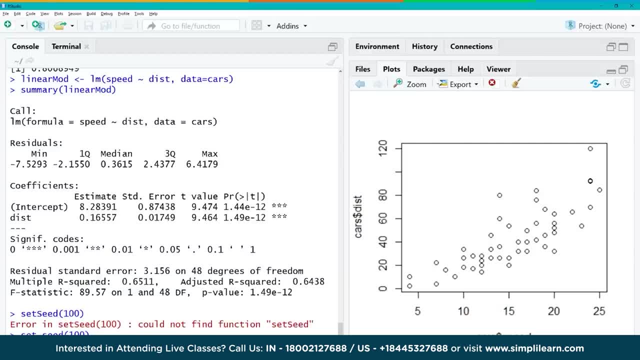 going to start with 1 and sample them. So, row 1 of the data, We're skipping any of the titles on the top And then in the sample it has two variables that go in. The first one is the in rows of cars. 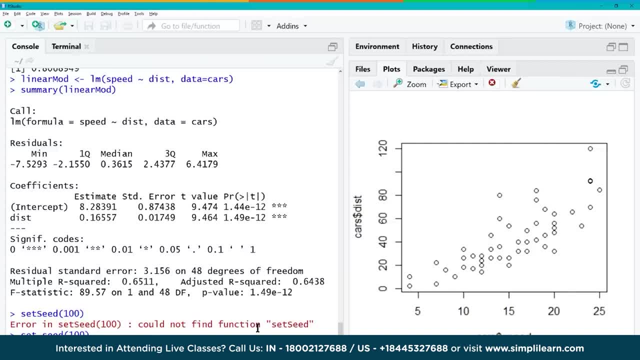 And then we want to do 0.8 times in rows of cars And this basically says that we're going to take 80% of all the rows in the cars sample, We'll hit enter to go ahead and run that. And we see here that I had an error And that is because 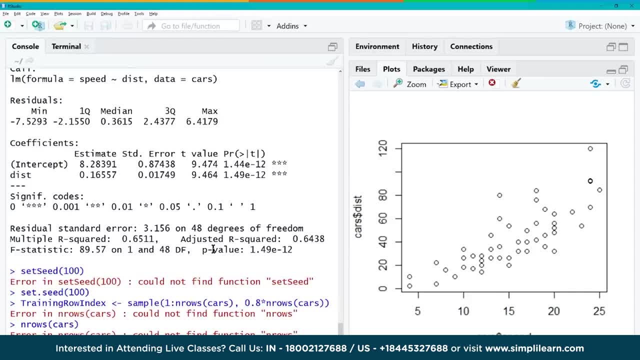 it's in row. I actually put an s on there. That's something I do a lot on. We'll just fix that real quick. It brings up a point that if you use your up down arrow, you can quickly paste through the last things you typed in and then you can reuse them. So 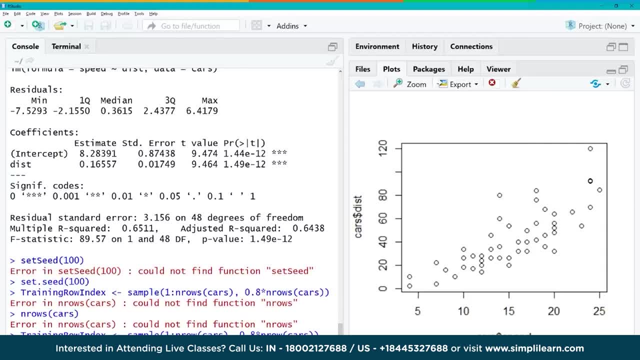 there we go. Now I have my training row index, which is basically a list of all the rows we're going to use, And now that we have a training row index, we'll go ahead and create our training data variable And we'll assign. 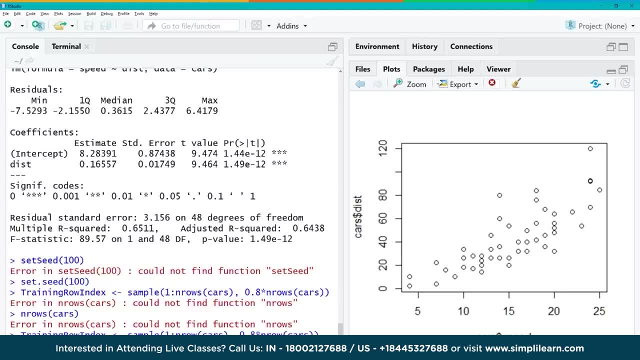 that cars, and we'll put that as training row index And this is supposed to be brackets because we're dealing with an array type format. We want to do the training row index comma because we just need the index of the row. And as far as the columns, we want all the columns. So here we have our. 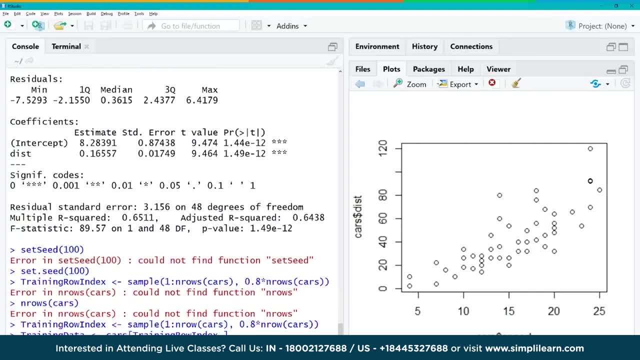 training data And now we set up a training data, We also need our test data And with our test data we'll assign that also to cars. And because we used the training row index and we used the sample to create it, we can simply do a minus sign. 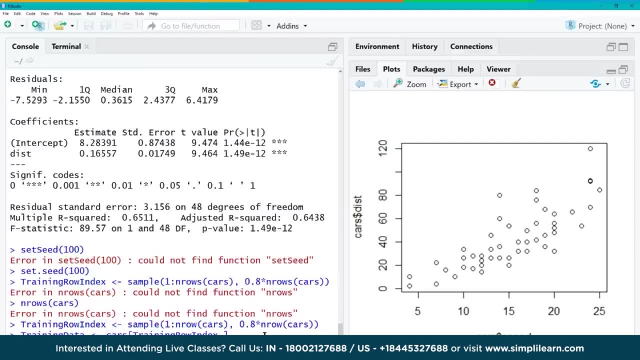 training index comma. So it's identical to the training data, but the test data is going to be the ones, the rows that were not included in the random sample of 80%. So it's going to be 20% of the data And of course it's 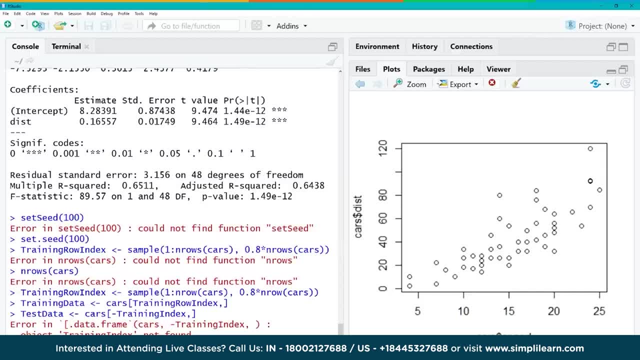 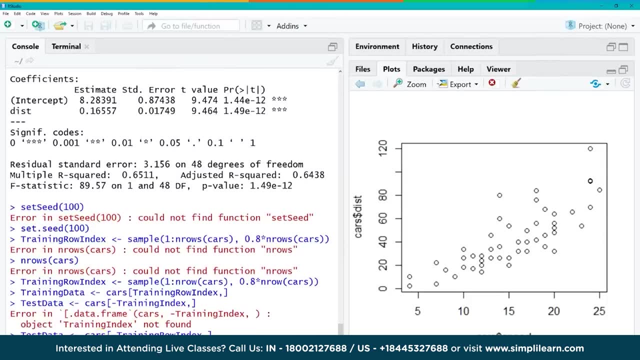 very easy to do mistakes on here, So we'll come back into this, bring back up the error, and then we have training into training index, training row index. There we go Very easy to correct errors in R. So now we have. 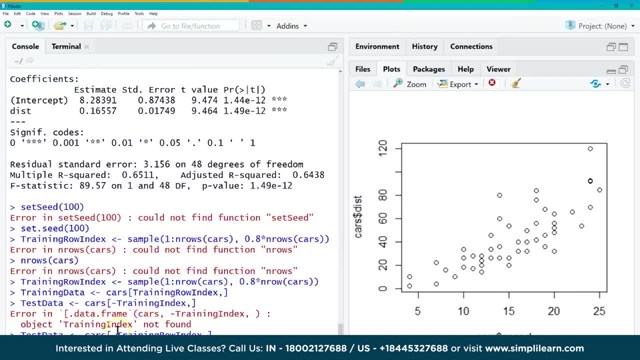 our training data and our test data. So we have 80% in training data and 20% in test data. And let's go ahead and create our model. We'll call it lm mod, And this is identical to what we did earlier. Here's our linear model We're going to. 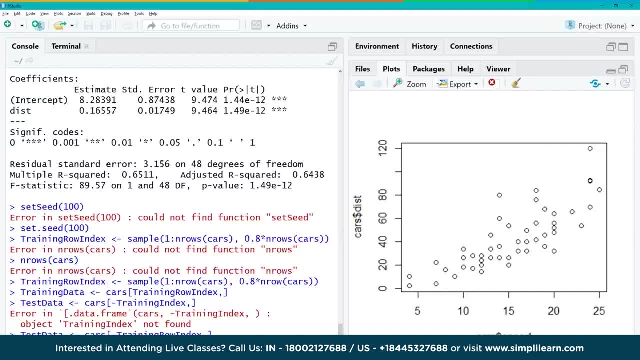 have our two different columns. If you remember above, we had to tell it which columns we wanted. I'm going to do distance and speed and then the data We're going to set equal to training data. So, as opposed to doing all of cars, we want to use just 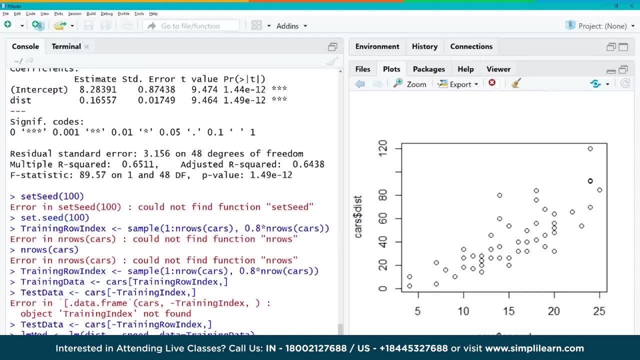 the training data on here And now that we've created a model off of the training data, we need to go ahead and run our prediction off of our test data. We want to see how the test data- which has nothing to do with the model- 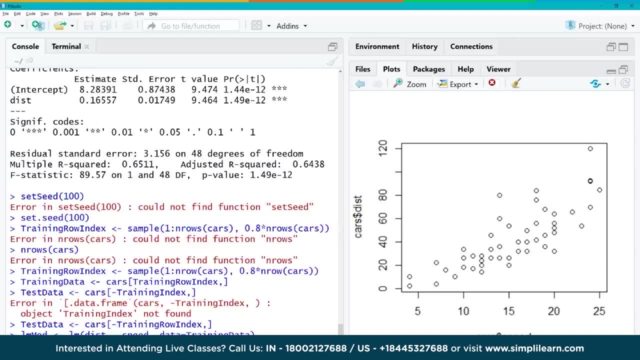 so far how well it fits, And we'll go ahead and call it distance predict. There's our assignment, So we're going to assign the value to it, And with R we type in predict and then we call our model. We go ahead and pull up our model, lm mod, And so we're going to 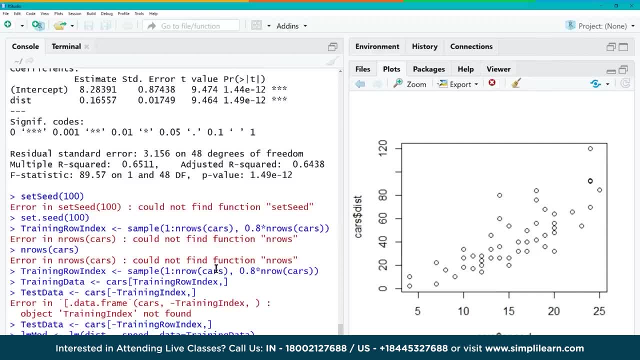 use that model and then we want to put in the test data. Here's our test data. And so now we're creating the distance predict variable and we're going to put all the information as far as predicting on our test data And we'll run that. Just hit the enter key And then, if you remember from before, 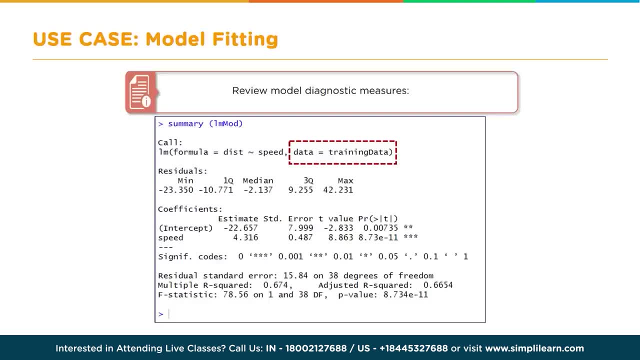 we want to review the model diagnostic measures, And so we're going to go in here and do a summary, And you'll see, in here we have a couple different things going on, But let's go ahead and take a summary of this and just walk through what this means. 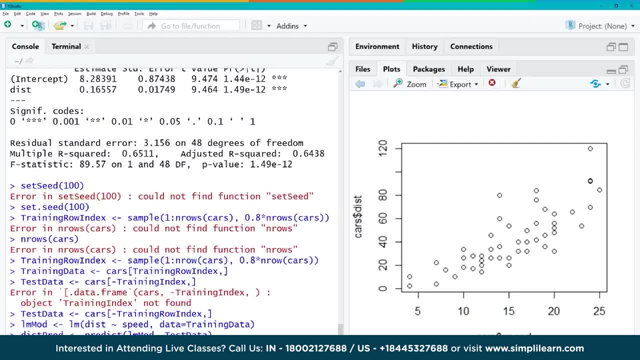 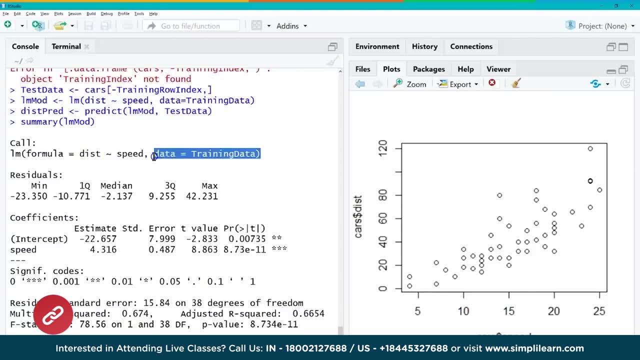 So summary, and then we call it lm mod And we hit enter and it pulls it up And we have a nice summary of our lm mod And the first thing we're going to note is that the data that's right now in our lm mod, that we're summarizing, is our training data. 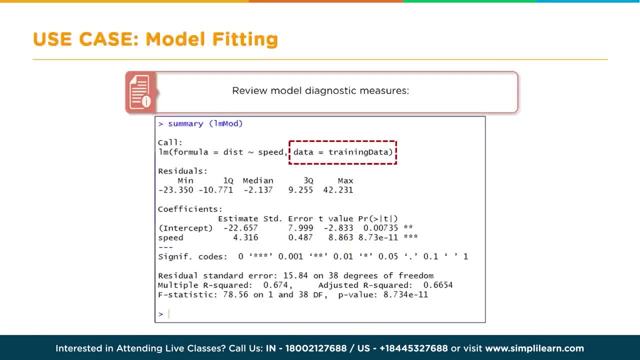 And let's go back to the slide and highlight this. So the data equals the training data. That's where the lm mod comes in. Residuals we have our minimum, our first quarter, medium, third quarter, and the max, Or quadrant. 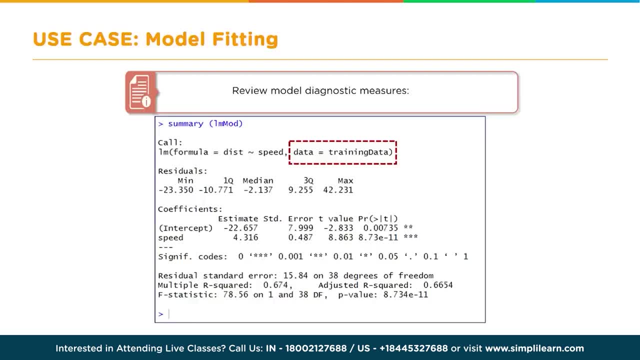 not quarter. You'd think I was doing business analysis as opposed to end of the year taxes and first quarter versus quadrant. We look at our coefficient, We can see where our intercept is and our speed is And we note over here our significance codes so they all match up. 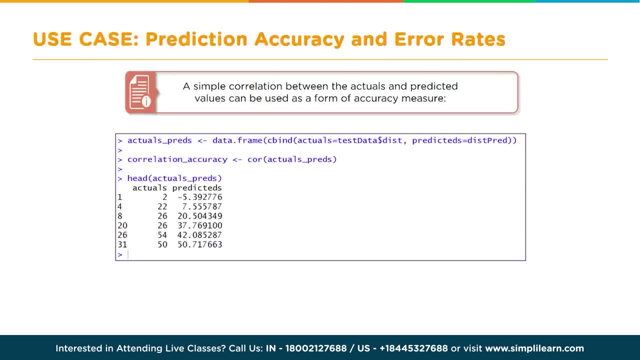 So a simple correlation between the actuals and the predicted values can be used as a form of accuracy measurement. So we took a look at the model we created and now we need to take our predictions and just see how accurate it is on the data that we didn't use to program the linear model. 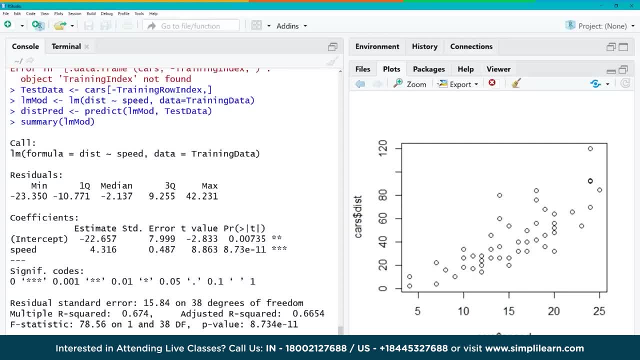 So let's create a variable called actuals- underscore- predicts- and assign it data frame. This is how we create a data frame: is we just assign data dot frame and we'll do a cbind and in our cbind we're going to take our data. 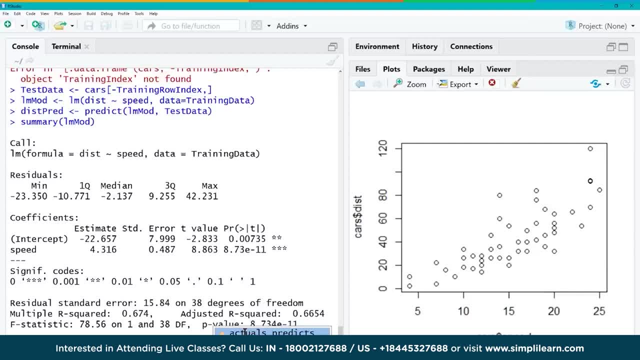 and we're going to create a column called actuals. So this is our choice: the name actuals. This is going to equal test data and we're going to use a dollar sign and distance, And we're running out of a little room there. 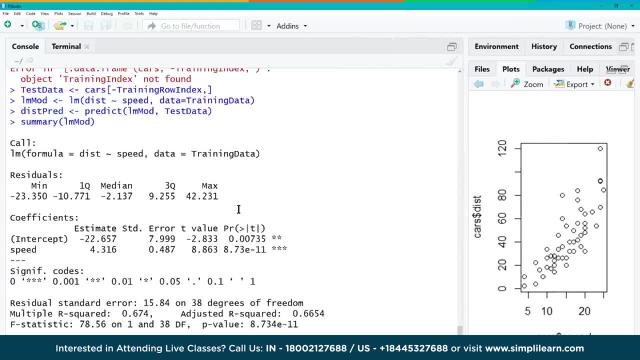 so let me pull this over so we can see it better. There we go, distance, And then we also want to take and compare that to what we predicted for the other data And we'll call this column predicteds, and that's going to equal our distance predict And remember, distance predict. 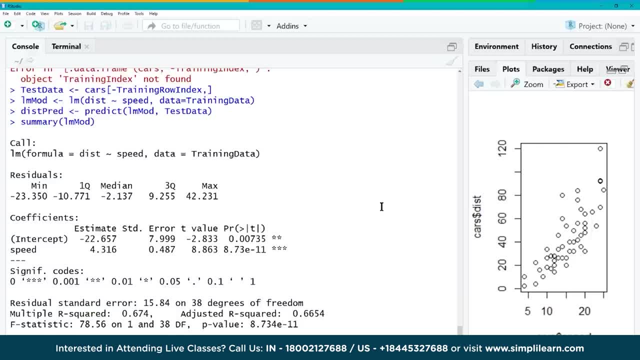 is set to the predicted values of our test data. So what this is is we're saying, hey, here's our test data, the actual data and the distance, and then we have what we predicted that distance to be And we'll go ahead and assign that And we can do a quick head. 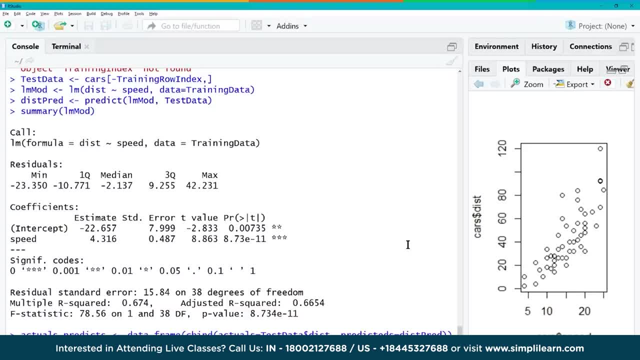 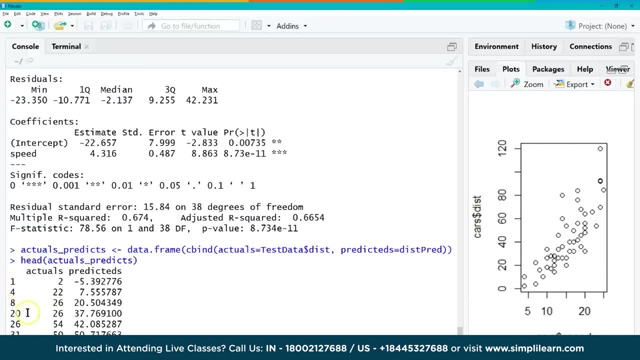 actuals predicts. there we go And remember. head shows us. it's a data frame, So it's going to show us the labels and the first set of data. In this case, you'll notice that the rows have a different count. They're not 1,, 2,, 3,. 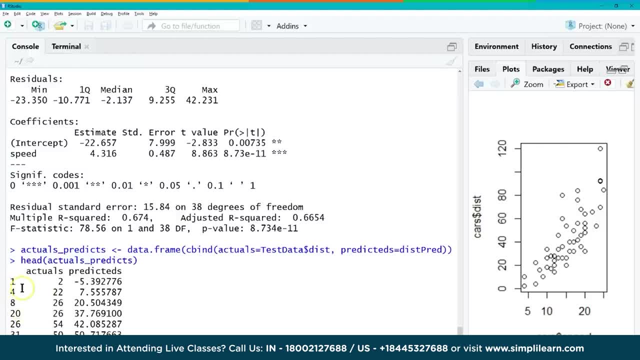 4,, 5,, 6.. Well, we randomly picked 20% of the data, So this is the first 6 rows of that random selection, which comes out as 1,, 4,, 8,, 20,, 26,, 31.. And we have the actuals. So the actual value is: 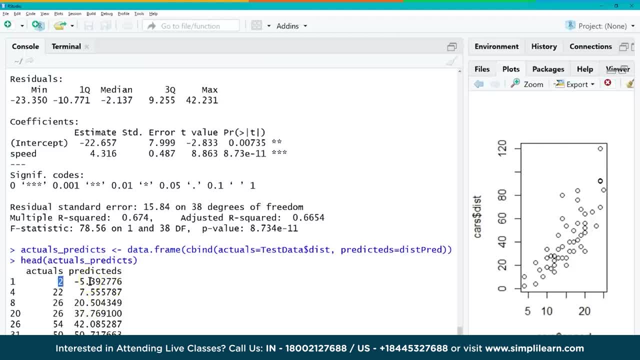 2 and the predicted value on this first one is minus 5.. So they're way off: 22,, 7,, 26,, 20,, 26,, 37,, 54 to 42,, 50 to 50,. 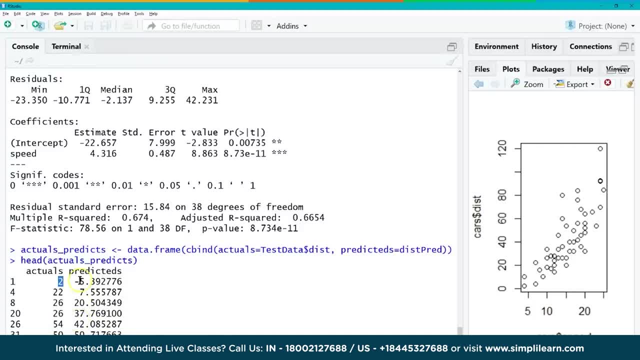 so one of these is actually pretty right on where a lot of them are really off at the beginning. Let's just see what that looks like, though, Because just eyeballing the first 6 rows does not tell us what's really going on, So let's create another variable correlation. 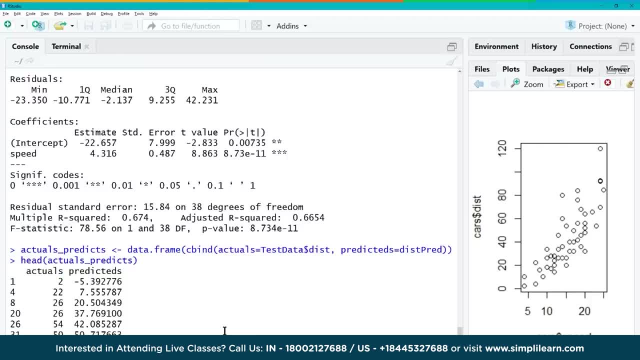 accuracy And we're going to assign this correlation COR. Remember, we do a COR And we have our actual predictions. So let's just see how our actual values versus the predictions correlate with each other And we assign that one actuals. 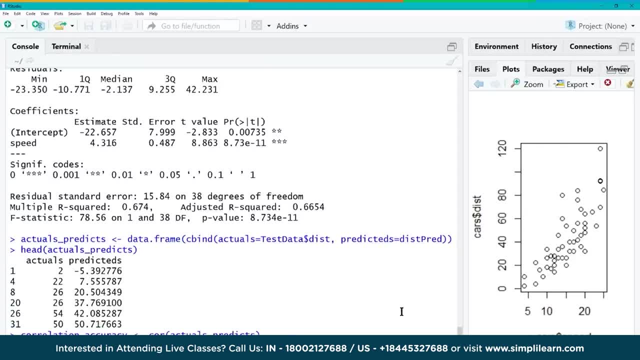 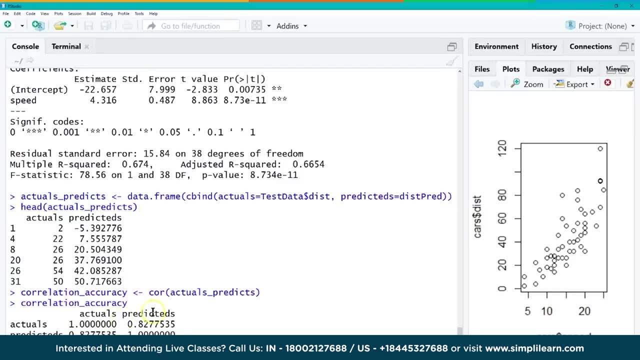 underscore predicts. There we go, Let it auto finish for me, And we can just go ahead and type in correlation accuracy and see what that looks like. So we have an actuals 1, a predicts 0.8.. And you can see how they kind of correlate. We have the 0.82.. And if you remember, 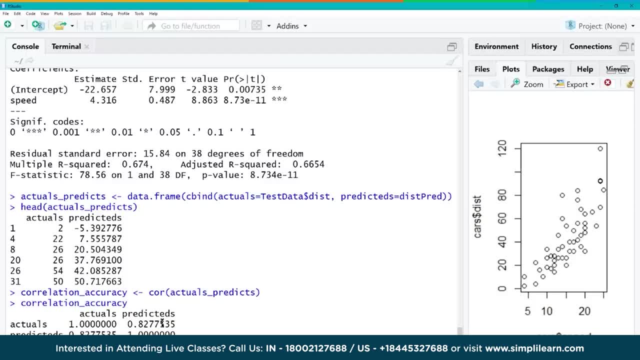 from before. we're looking for either 0.001, 0.01, 0.05, 0.1.. That is the p-value, which we're not looking at here. This is not based on the p-value. This is based on what we looked at earlier with correlation: that the closer 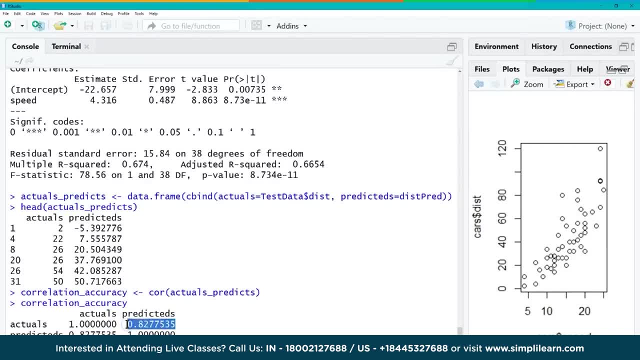 to 1, the closer the values are, And so 0.82 gets upwards of 1.. So you see that there's a normal, pretty much a correlation in here. But we want to dig a little deeper, because this doesn't really tell us how accurate it is. 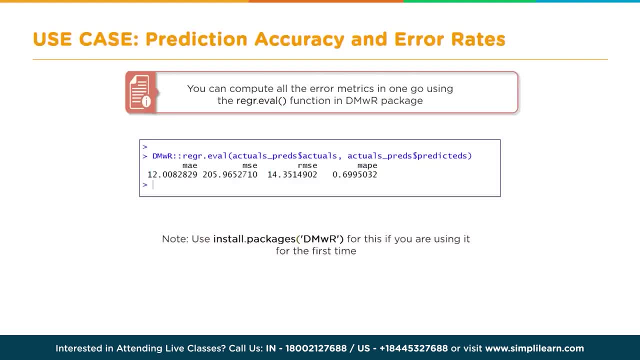 For that we're going to use another tool. For that we're going to calculate the min-max accuracy and MAPE. And the min-max accuracy equals the mean value of the minimal actuals and predicts over the max value of the actuals and predicts. 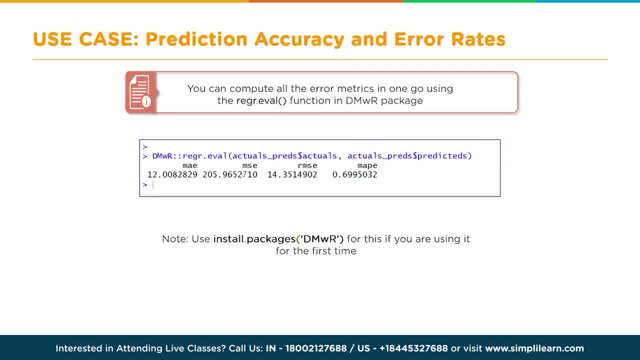 And then the mean absolute percentage error, or MAPE as it's called, equals the mean of the absolutes predicteds minus actuals over the actuals. That's a lot to follow as far as remembering all these different math and theory behind it. Cool thing, though, is it's all done. 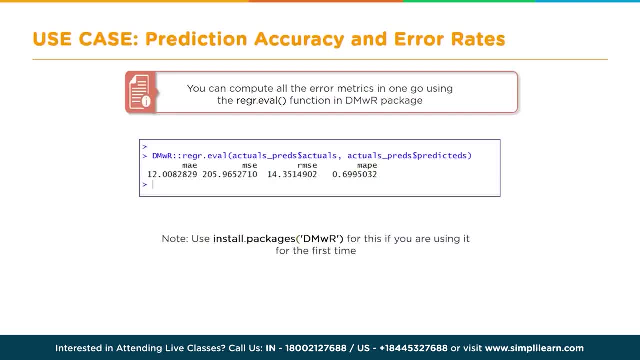 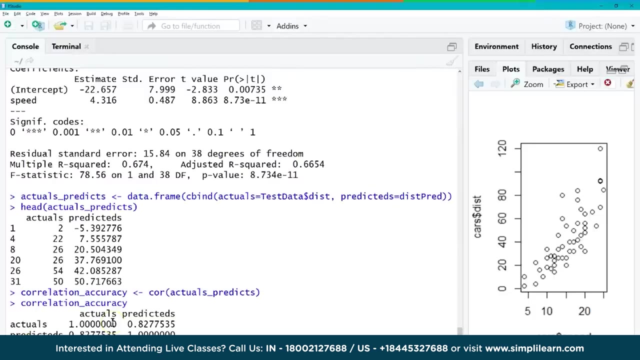 pretty much for you, So you can compute all the error matrices in one go using the regress eval function in DMWR package. Since this is the first time I've used this install, I'm going to have to install the DMWR package So we can actually install it two different ways. If you remember, we talked about 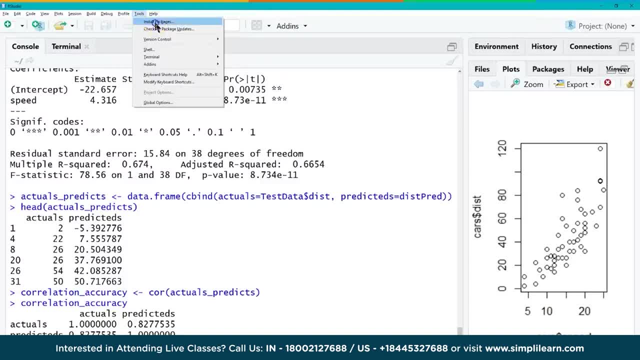 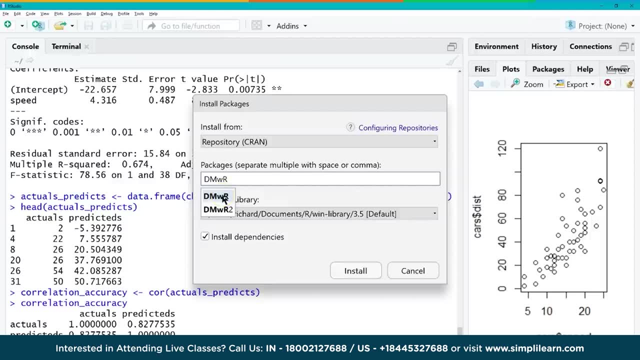 installing package earlier where you can go under tools and install packages, and I certainly could type in DMWR. It even comes up and lets me know that's one of the main packages up there. Well, that's a tool of the RStudio setup. You can also install this using the console. 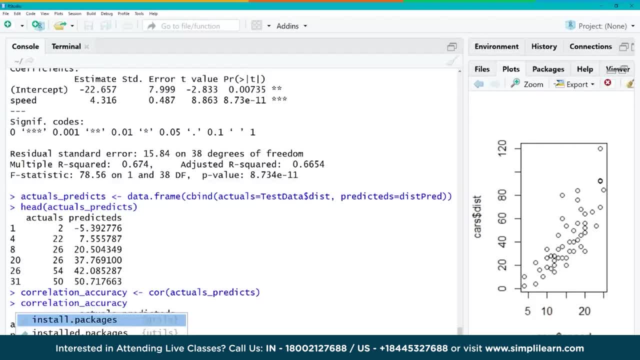 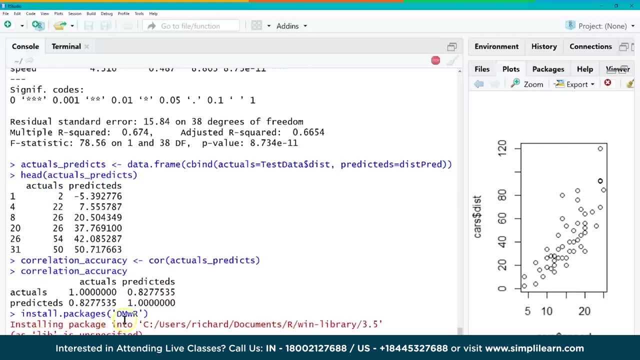 We simply type in install dot. you can even see here it comes up install packages and then DMWR. And when I hit enter it should do the same thing as the other one does. It goes through and installs the DMWR package. It takes just a moment to zip through. 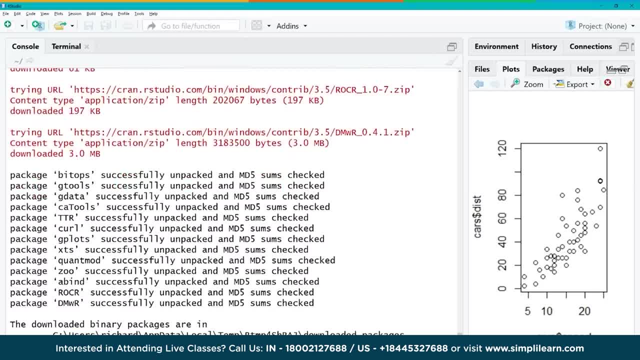 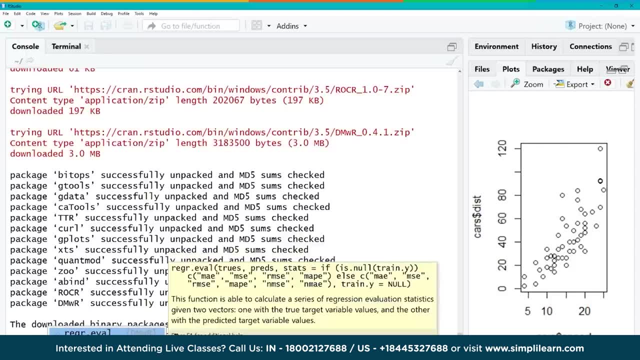 all the different package setup And then the format for DMWR is DMWR. We're going to go colon, colon. We are specifically looking at the regression dot eval, And then we're going to do actuals underscore predicts And we'll go ahead and put in the individual columns on this one. 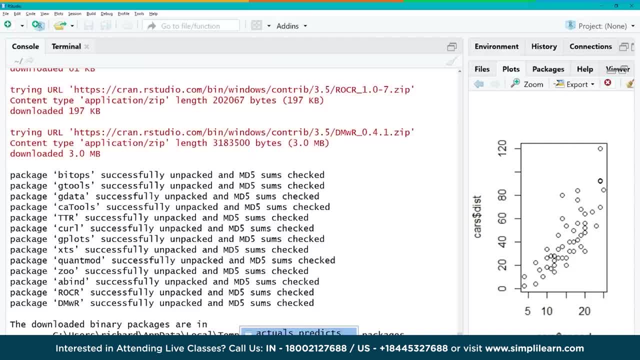 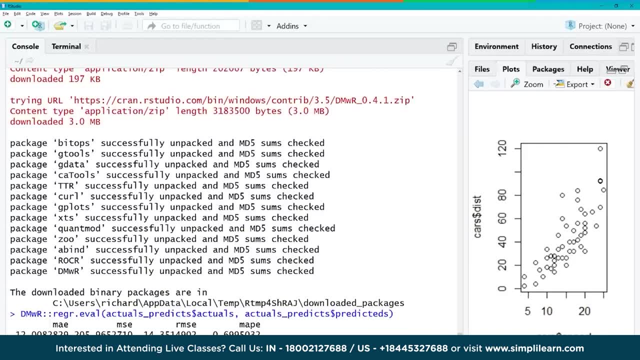 So we have actuals Love the auto typing, And then again actuals predicts, And this time we want to do it against the predicteds. We'll go ahead and hit enter on here And you'll see in here it comes up with. 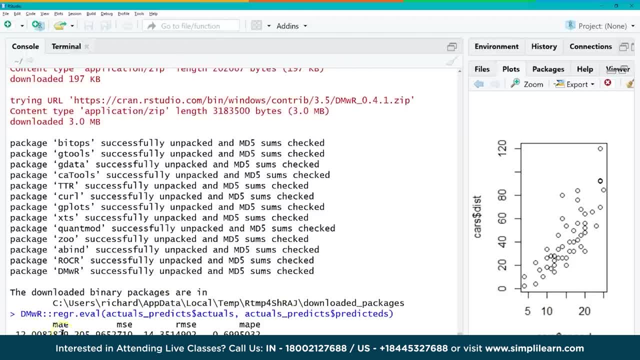 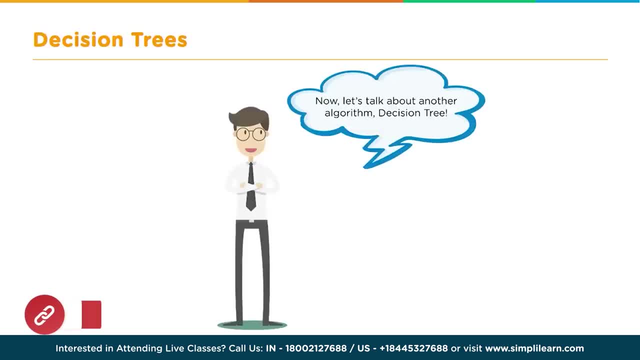 our MAE, MSE, RMSE and the MAPE values. So we looked at the linear regression model. Let's go ahead and take a look at the decision trees. So let's go ahead and talk about another algorithm: Decision tree. Decision tree is a tree shaped algorithm used to determine. 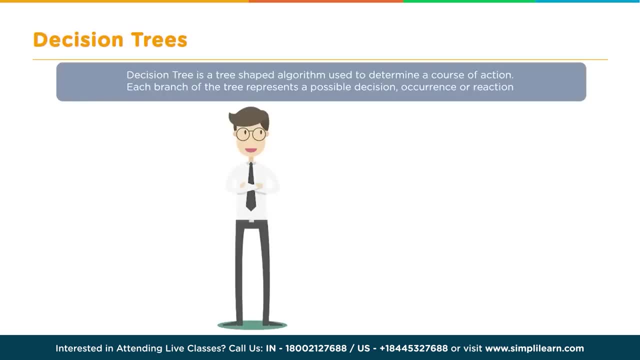 a course of action. Each branch of the tree represents a possible decision, occurrence or reaction. It's a tree which helps us by assisting us in decision making. Let's look at the basic terminologies to understand decision trees. We have our root node. We have a splitting, We have decision node- decision node. 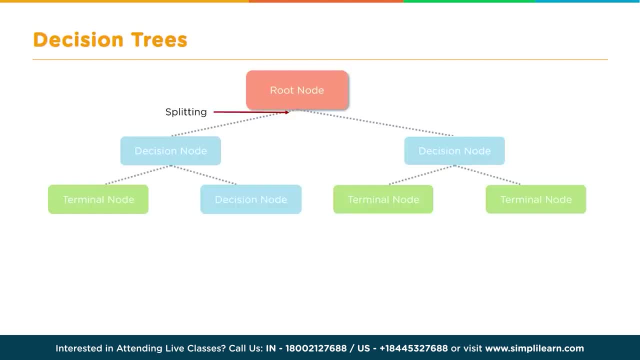 and then those split into terminal node, decision node, terminal node, terminal node And each decision node has a split. The decision node continues to split until it ends in a terminal node. Note A is the parent node of B and C. Also note we call the terminal nodes. 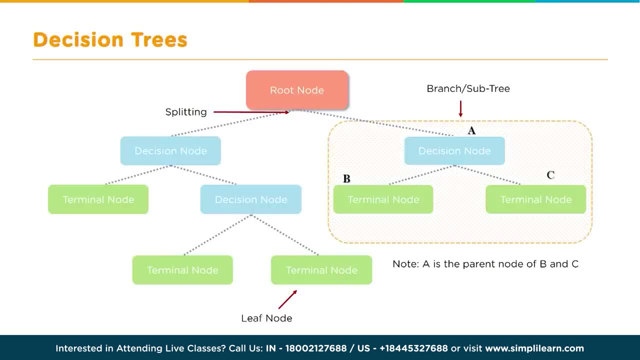 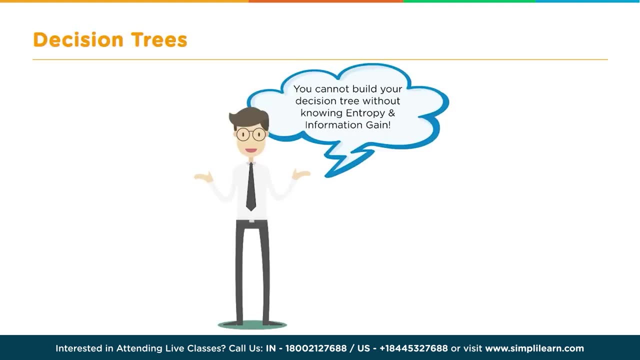 leaf nodes, You can also see that we have a branch or a subtree. So when you have a split, everything under that split, under one side, is called a subtree. You cannot build your decision tree without knowing entropy and information gain Entropy. Entropy is the measure. 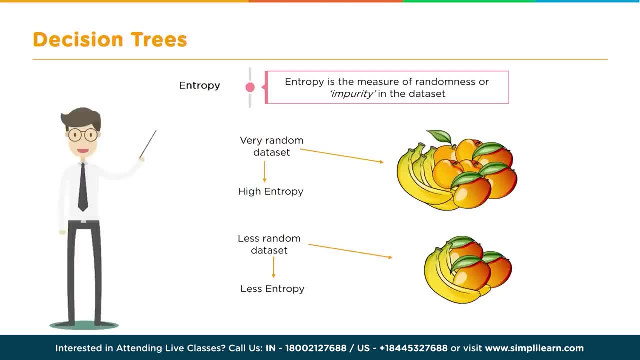 of randomness, of impurity in the data set. So we have here a fruit and you can see we have. it looks like apples, oranges and bananas. It's very chaotic, So it's a very random data set. It has a very 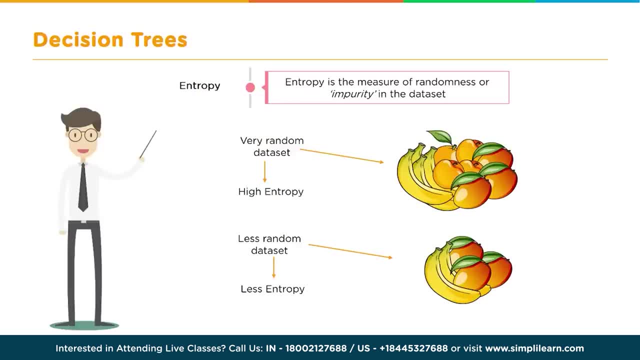 high entropy And if we take out one group- let's say we take out the apples- it's a little less random. Now we only have bananas and oranges, So it's a less random data set and we have lower amount of entropy. Entropy is: 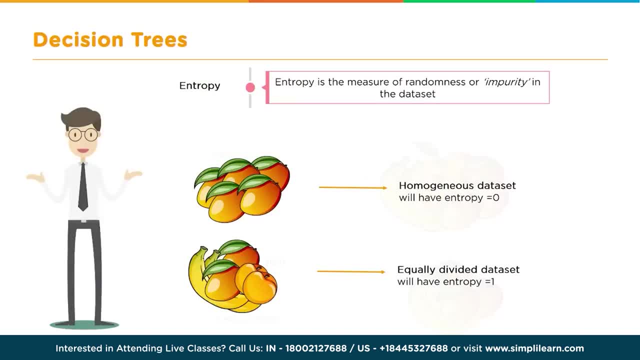 the measure of randomness or impurity in the data set. So when you have a homogenous data set we will have entropy equals zero. And here you can see it's all oranges. An equal divided data set will have an entropy equal to one. So here we have half or 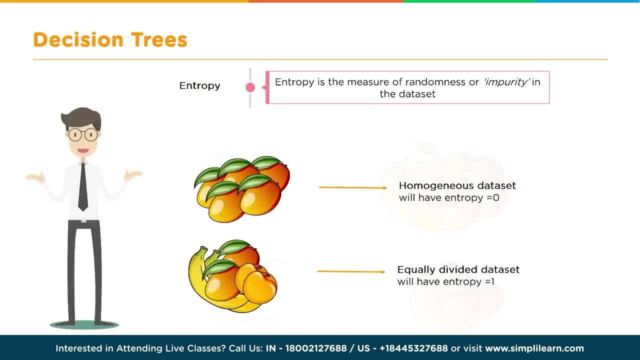 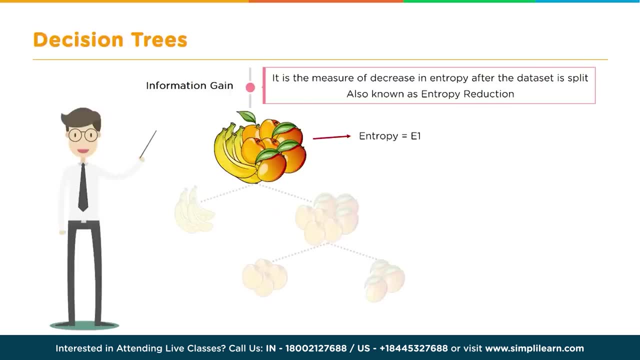 what is it? It looks like a couple bananas, a couple oranges and a couple apples, So everything is equal. So we have an entropy of one on there, since there's two of everything: Information gain: It is a measure of decrease in entropy after the data set. 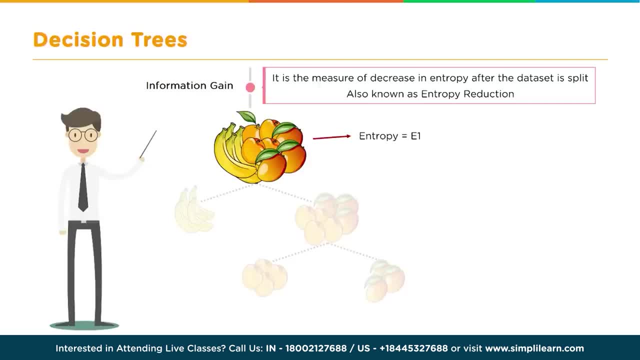 is split, Also known as entropy reduction. So we look over here and we have an entropy equals E1. And the information gain. we split the bananas out, the size becomes smaller and you'll see that E1 is going to be greater than E2. Or we measure E2. 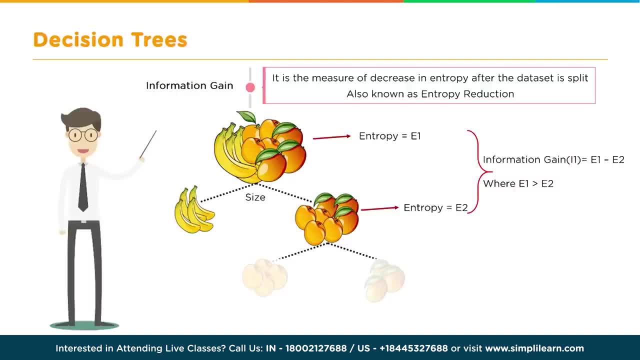 of the apples and oranges in this case. If you love your fruit, it's probably getting you hungry right about now. And then the information gain from our level two equals E2 minus E1, where E2 is greater than E3. And as we come down here, we'll see that the E3 is now the third level where we split. 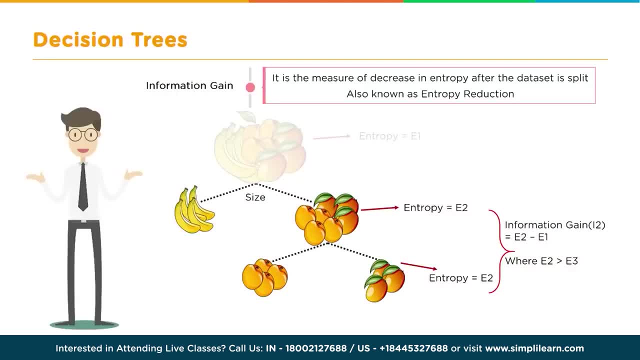 the oranges and apples out, And each time that entropy becomes less and less, until, in this case, we have an entropy of zero, since they're all homogenous in their order: All oranges, all apples, all bananas. So let's take a look at the use case decision tree and actually put this into code and see what that looks like. 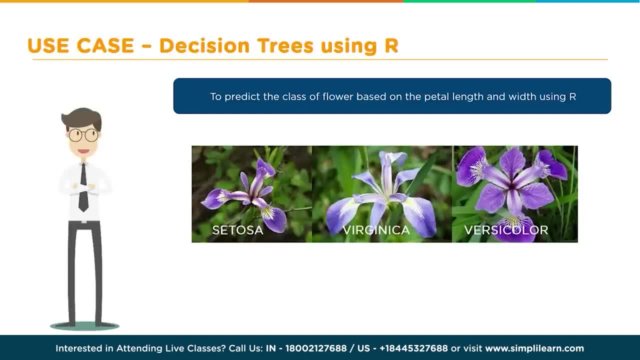 as we go from theory to script And to predict the class of flower based on the petal length and width, using R, And you'll see, here we have these beautiful irises, Probably the most popular data set for beginning data analysis and statistics. We have the 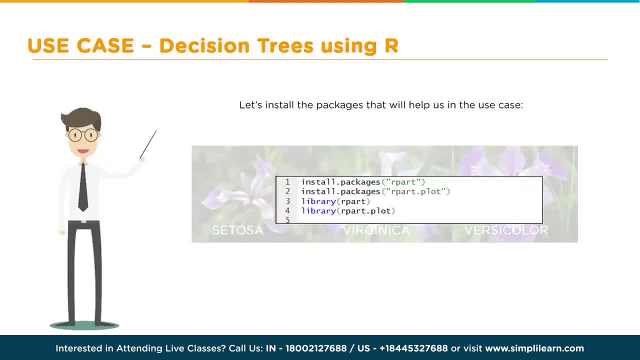 setosa, the virginica and the versicolor. Let's install the packages that will help us in the use case. So, because we're doing decision tree, we have rpart, rpartplot, and then we have the library rpart and the library rpartplot. 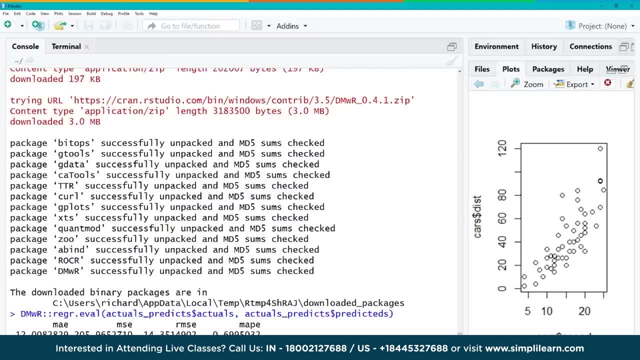 Let's go ahead and take a look at that. And, if you remember, we have two ways of installing it. We can do the install packages. We did that earlier. Here we go: install packages, using my up error to get to it, Or we can go up to tools. 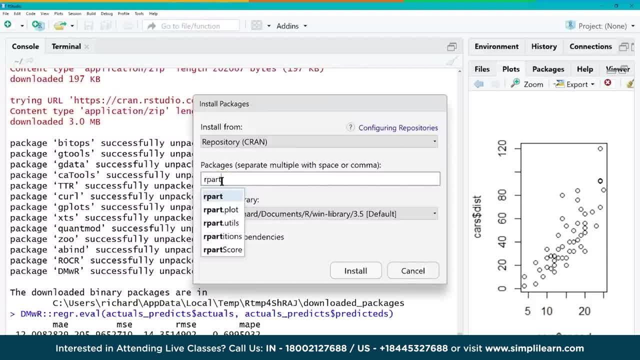 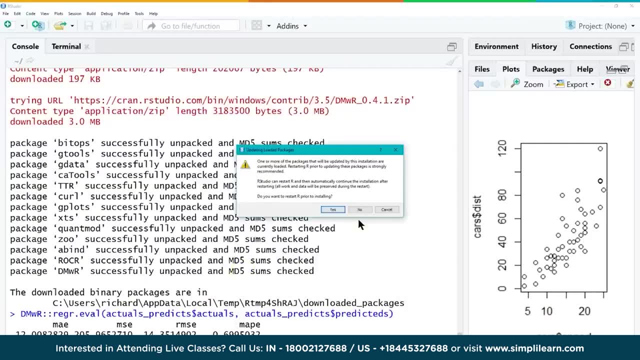 install packages and I can do rpart and rpartplot and then go ahead and hit the install. It will be updated as they are currently loaded. Oh, looks like some of them are already loaded. That's fine, We'll just go ahead and update those And once we have those, 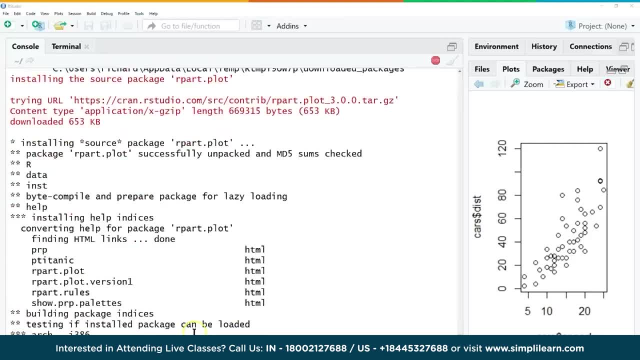 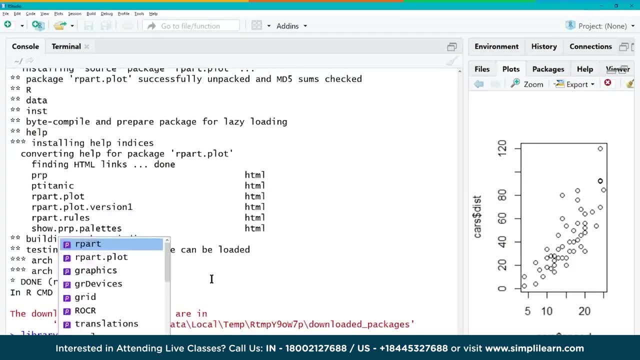 updated. let's take a look and see what we have going on here. Oops, still loading. Let's go ahead and type in library rpart and library rpartplot. So we want to bring it into our console that we're working in. So up until now we just downloaded the packages, and now 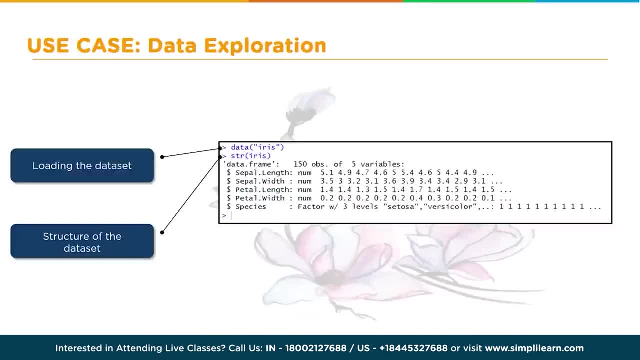 we want those libraries available to what we're doing. So the iris, although it's built into the rpackage download, on the basic download we actually have to install the data or bring the data in. So we're going to do the data iris and then we're going to do the string iris And let's just flip back on over. 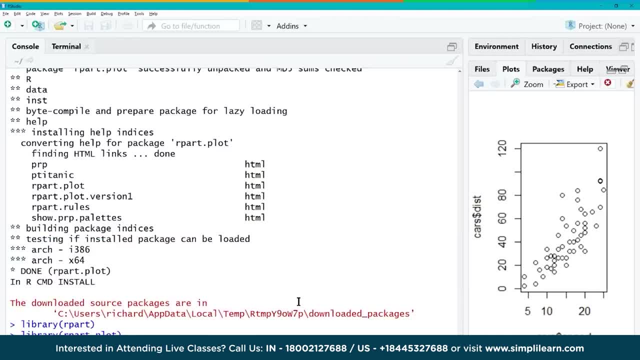 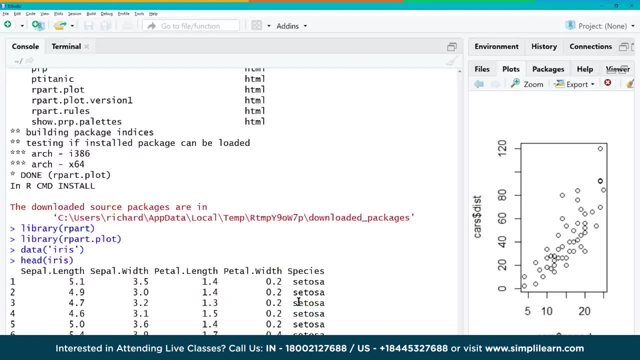 to our RStudio and set up our data iris and then we're going to do string. Before we do that, let's do head head iris. There we go And you can see the head has sepal length, sepal width, petal length, petal width, species. In this case, the top part's all setosa. 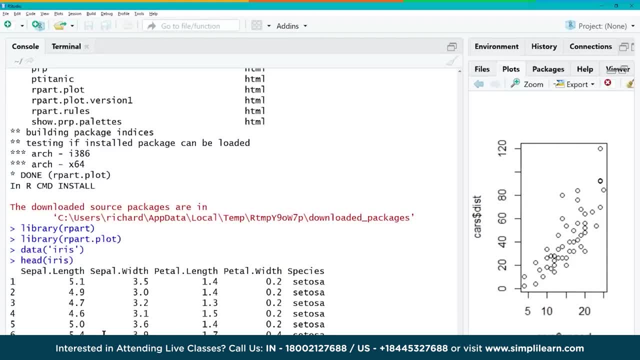 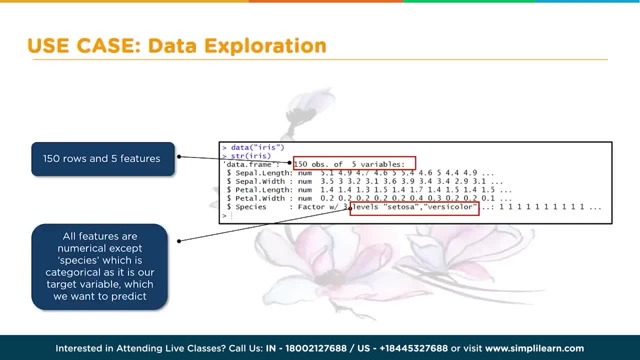 and each row gets a number. And then we did the string iris and that comes up with information. And if we flip back to our slide, you can see here the structure of the database. under string is: it's a data frame. It has 150 objects, 5 variables each, so each one. 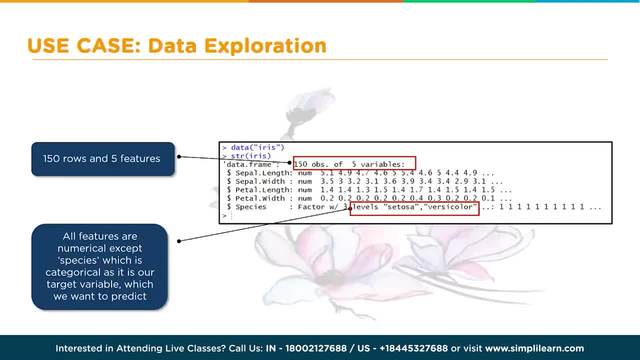 has 5 variables. All features are numerical except species, which is categorical as it is our target variable, which we want to predict. So we want to predict whether it's going to be a varicosa versicolor setosa. So you can see, here we want to predict, all the features are numerical. 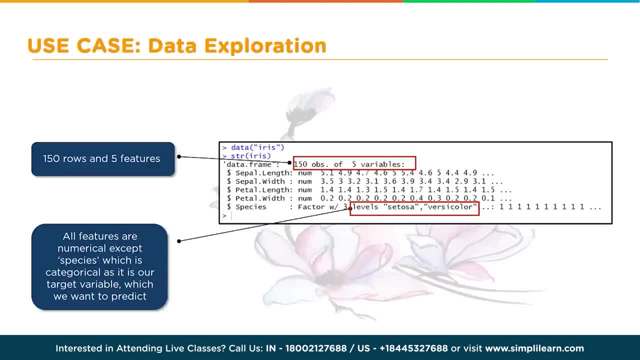 except species, which is categorical. It is our target variable which we want to predict, And you can remember that's the setosa, the versicolor, the virginica, the three different categories we saw earlier in the beautiful pictures of the flower, And so we're going to go ahead and use the set seed to 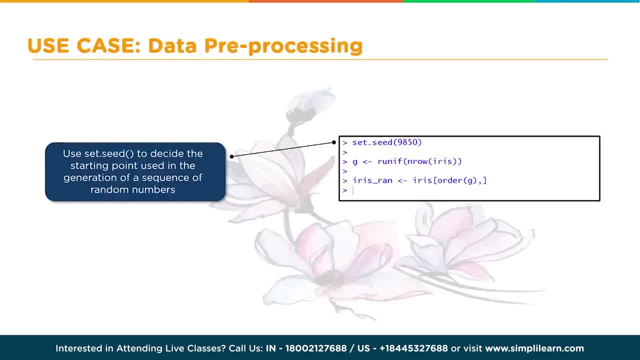 decide the starting point used in the generation of sequence of random numbers. Remember, we set the seed so that if we ever want to reproduce what we're doing, it will reproduce the same thing each time. because it's using the same randomizer seed, It brings slightly different results. 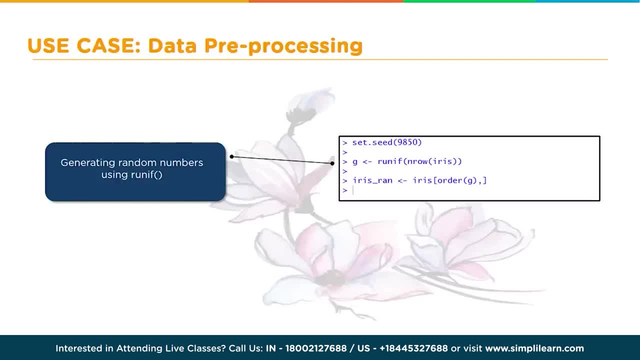 depending on what you need it for. And then we're going to generate random numbers using runif. And the question is, why do we want to create random numbers on here? It's kind of an unusual thing to do for in rows, iris, And let's go back and just take a quick look here. 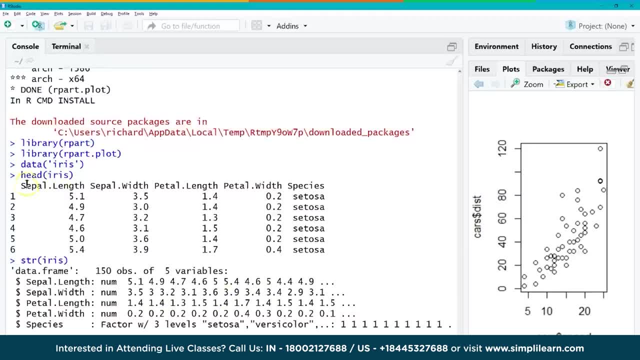 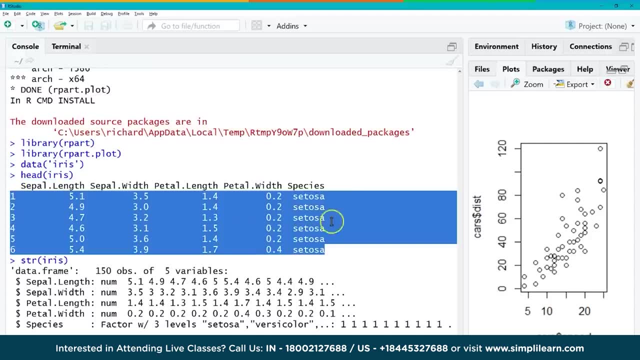 Actually, we want to go back to our R studio And you're going to notice, when I did the head of iris, what did I have? I had setosa, setosa, setosa, setosa, setosa. So the data is organized by species. 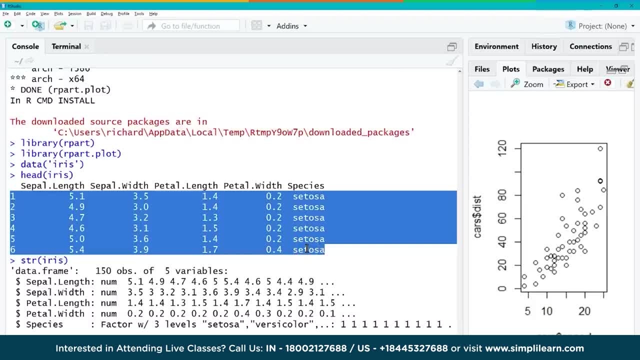 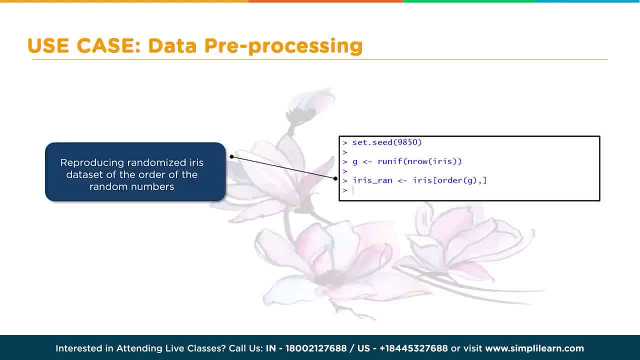 And it's already grouped them together in the data set. Well, we want to randomize that so that doesn't affect our output, And then we'll go ahead and take and create our iris ran, where we recreate the data frame based on a random order instead of setosa all being grouped together. Let's go ahead and put that into our. 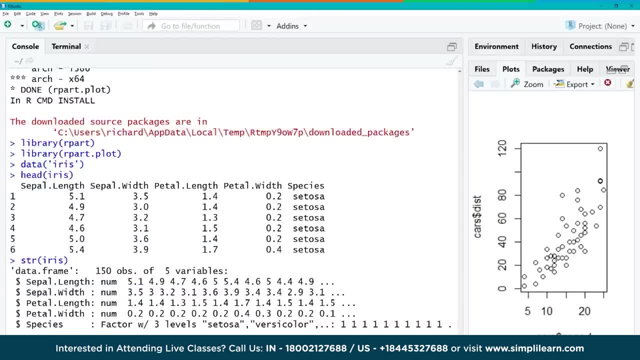 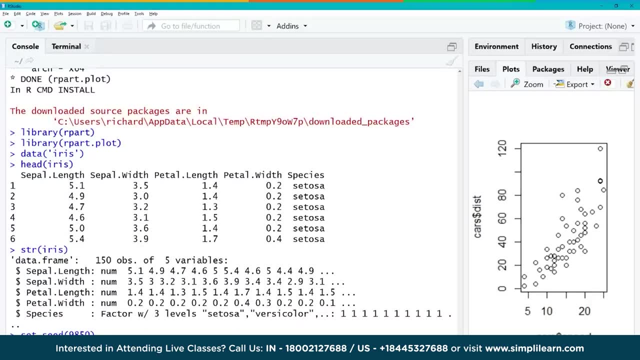 R studio And setseed and we'll match their number. It's 9850.. This way we'll have identical results to what they're doing on the slides. Then we're going to set the variable g equal to runif and base this on in row of iris. And finally, 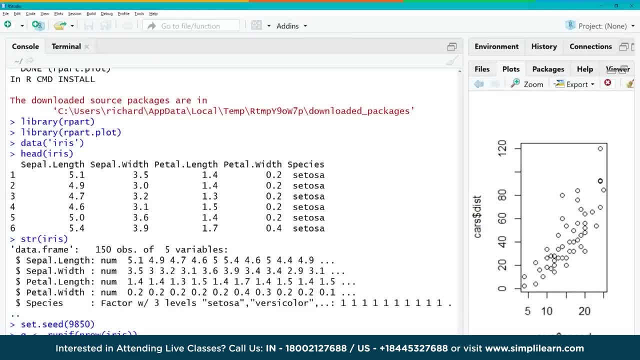 we're going to create iris underscore ran and we're going to assign our variable. we're creating iris underscore ran And we'll set that equal to. We're going to do that to the original database. We're going to set that equal to iris And we need brackets because we're assigning the. 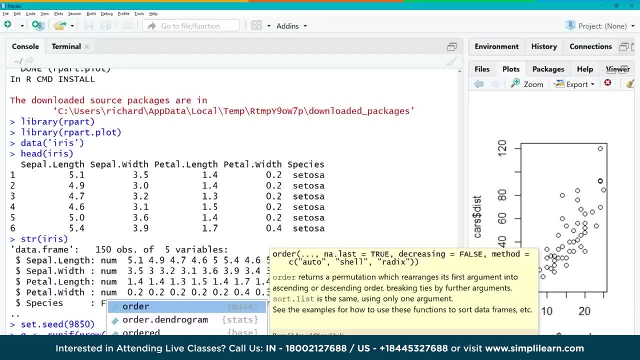 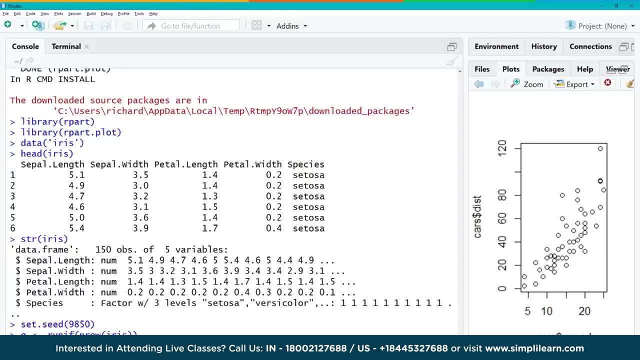 variables And we want to change the order. So there's an actual command order we can do. It's going to be order g, So this means all the rows in the order that g is. So we just randomized all those rows. And then we want to keep all the columns, So we'll just put a comma and we'll leave it. 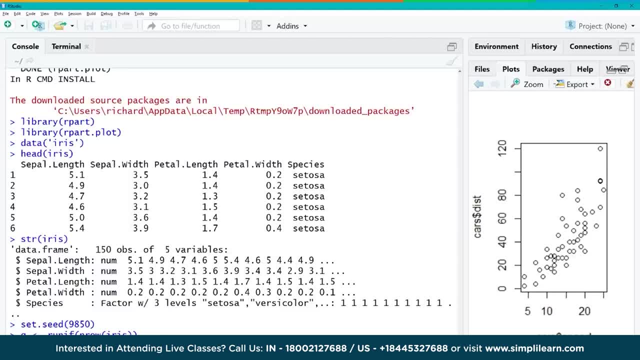 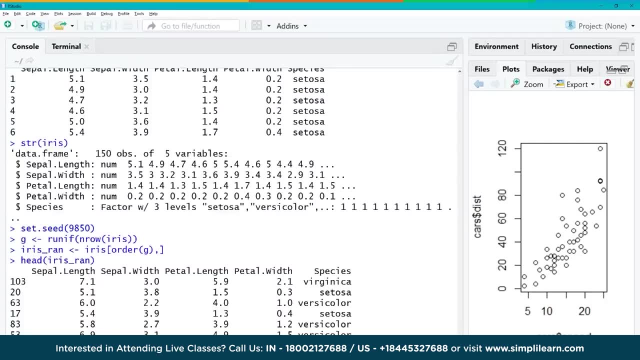 blank for the columns. So now iris ran will have some randomized rows coming in And if we do head, Let's just do this real quick. Iris ran, We can see that it's no longer satosa satosa. We now have virginica satosa versicolor. 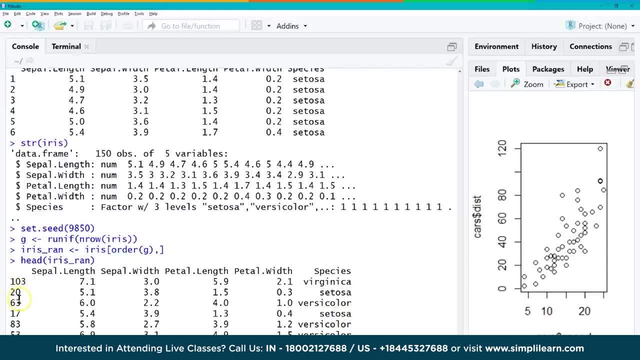 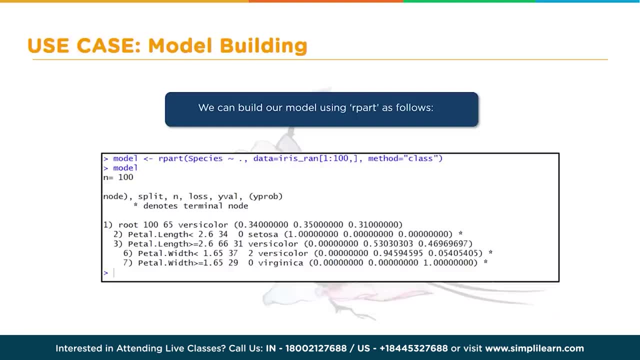 satosa And you can see the row numbers at the beginning. We have 103,, 20,, 63,, 17.. So they're randomized on there pretty well. Now that we've done a little data manipulation, We can go ahead and build our model using our part. 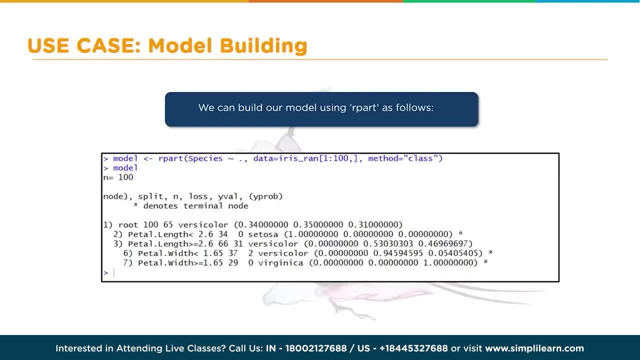 as follows, And one of the things I want you to notice here is we're going to build our model for our R part on the first 100.. Because our data equals, iris ran 1 to 100.. There's 150 objects, So we're keeping a third of them off to the side. That way, we have our 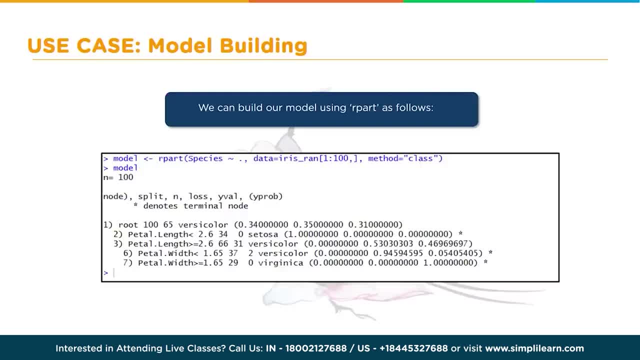 training set and our test set already pre-built because we randomized the rows going in from the beginning And then, once we've done that, we want to go ahead and print our model out and take a look at it. Let's go ahead and put this into our R studio and take a look. 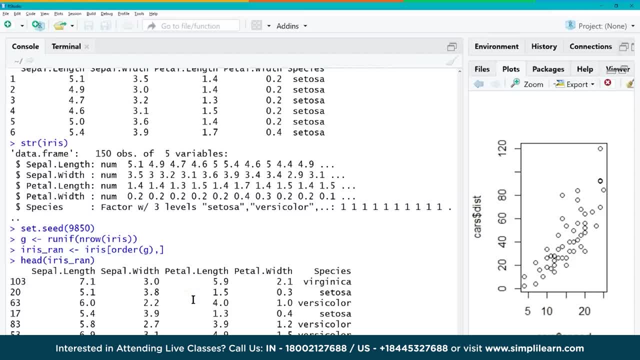 And so we have our model. We're going to call it model, That's our variable name that we're giving it. We're going to assign that our part, and in brackets we'll start with species And we want to correlate species to all the other columns. So how do we do that? 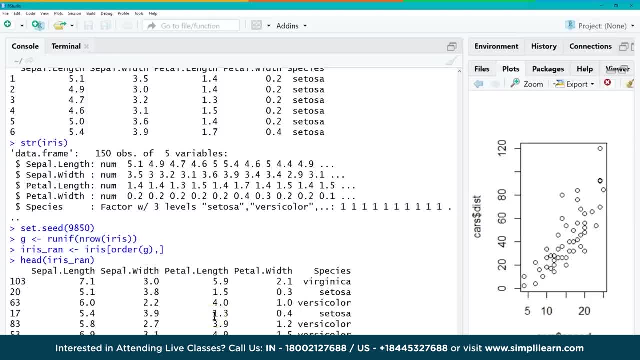 And the shorthand is just to put a period there And then we're going to put a comma And we want to set our data equal to iris ran. That's the data we put in there. And remember I said we're going to do just the first 100 rows. 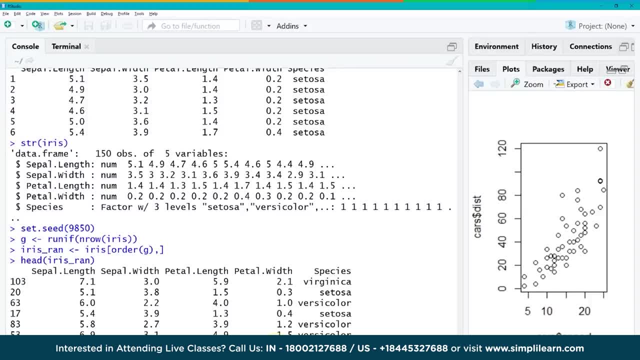 So we can save the last 50 for testing. So we can do that simply by doing row 1 to 100.. So in R you start with 1 for your rows And because we want all the columns, we just put a comma And that denotes that we're going to use all the columns in here. 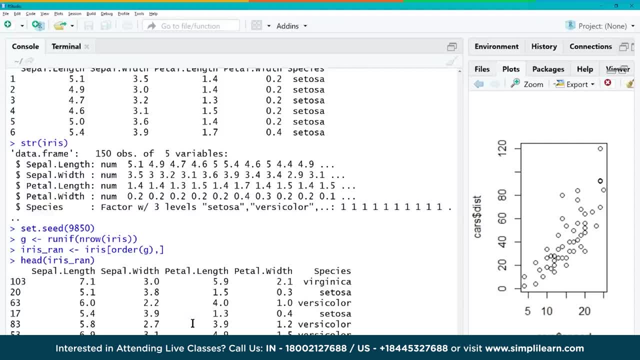 And in the R part there's different methodologies. We're using the method equals class, And you realize that we're doing a classification between the three different types of flowers, And so this is what we want to go ahead and set up our model with. 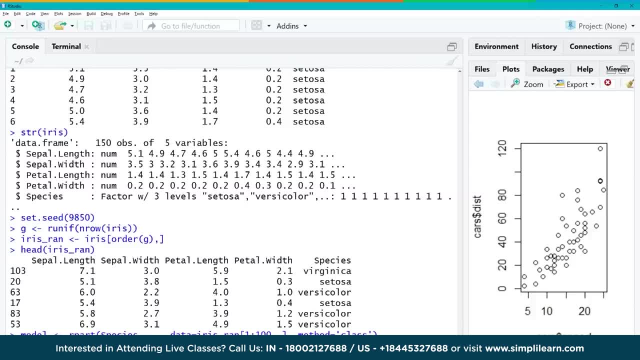 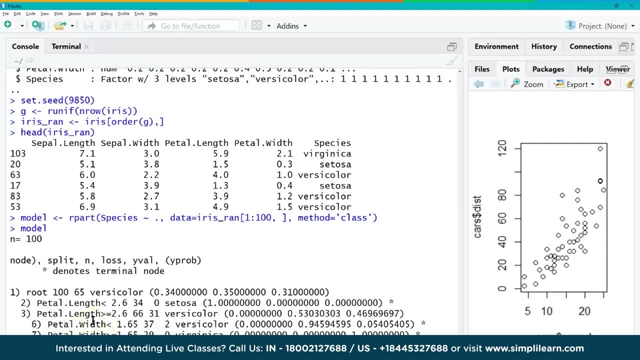 And when we run that we've now created a nice model for us. We can go ahead and just type in model, Hit enter And you'll see it'll print out a bunch of information about our model. So let us know what's going on in there And let's just break that down and see what that 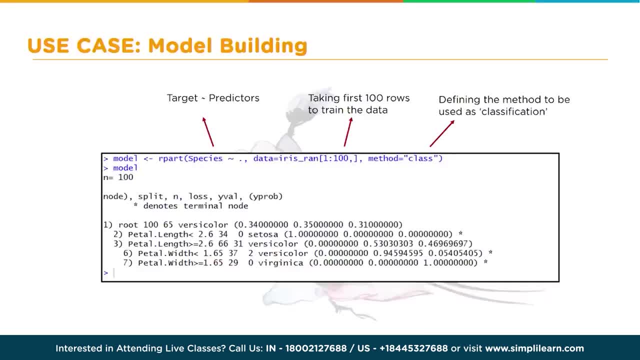 looks like. So we have our target, our predictors, That's species And it's going to relate to. we used a period to denote all the columns. We're going to take the first 100 rows to train the data And we have the defining method to be used. 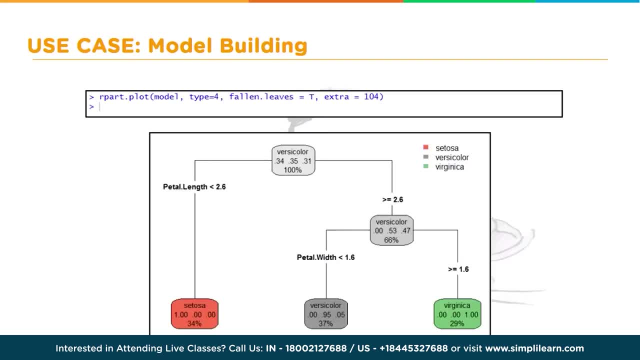 as classification. That's what the method equals class is, And what we want to do next is we're going to do a plot And take a look and see what this actually looks like. A little visual here, which is nice. We can simply do that with rplot. 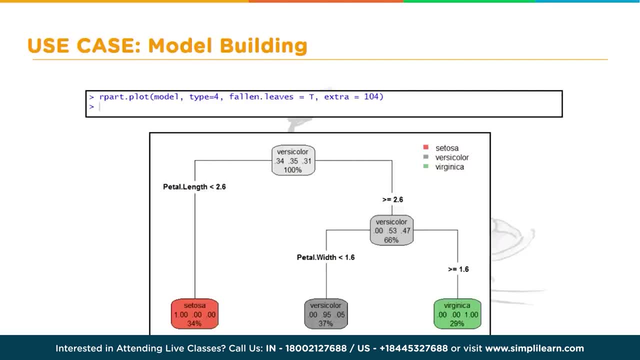 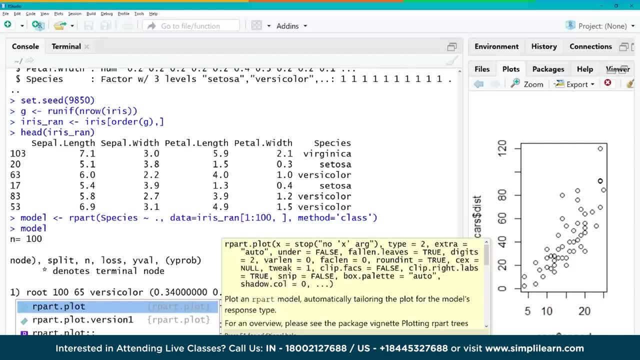 for the model And let's break this down a little bit and see what that looks like in the R setup. When we do this rpartplot A little bit of a mouthful there, sometimes That's part of the rpart package or module. So when you 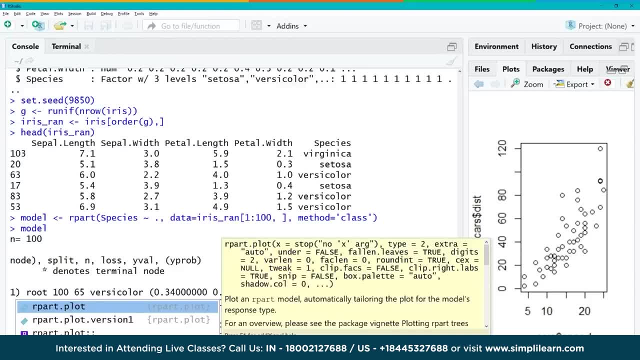 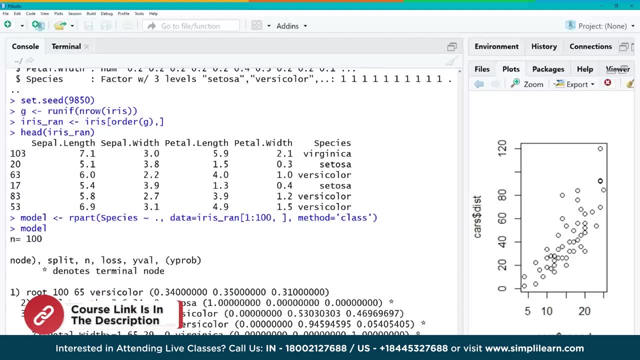 imported this in. it also included its own plotting format. We're going to send it our variable model And there are actually a number of types of plots listed for rpart, But we're just going to do type equals 4, fallen dot leaves equals t and. 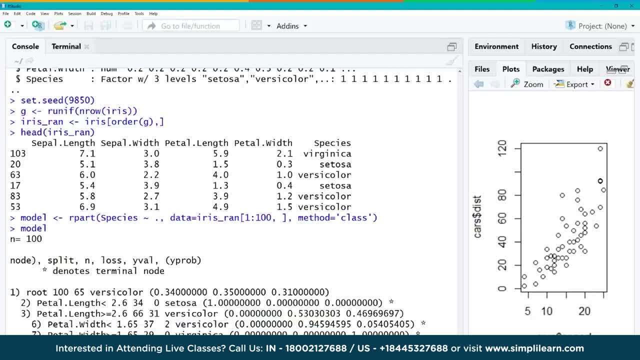 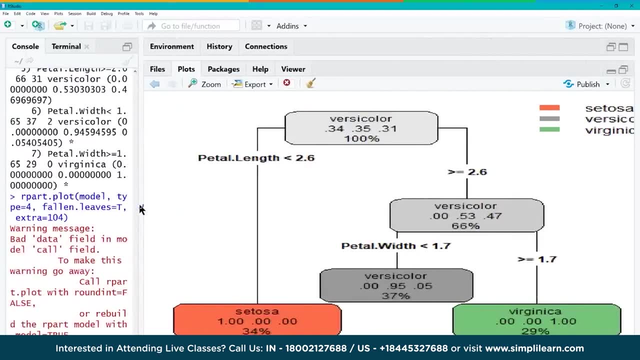 extra equals 104.. Let's go ahead and hit enter on there And you'll see, right over here on the right hand side, it goes into our plots. We just enlarge that. We have our versicolor, our setosa versicolor, virginica. 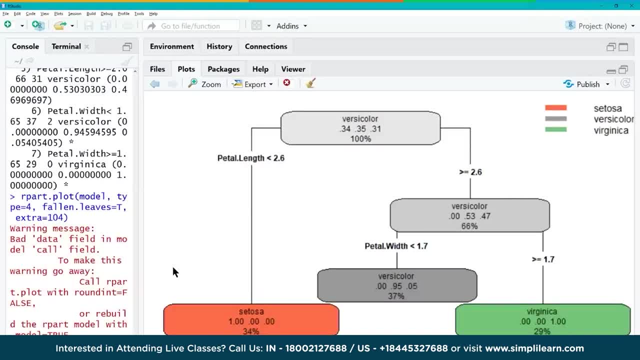 And let's go ahead and break that down. As you can see down here, it represents a tree. as it splits, It looks at it and says, hey, if the petal dot length is less than 2.6, it's going to be a setosa. So 34% of them fall into. 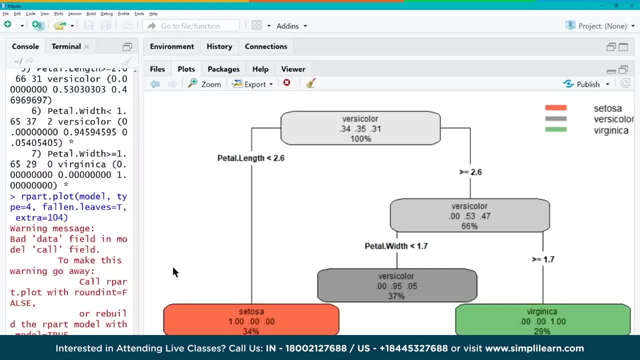 that category And if the petal length is greater than 2.6, then it looks at that and says, okay, now I have three different variables, We're going to split it again. Petal width is less than 1.7.. 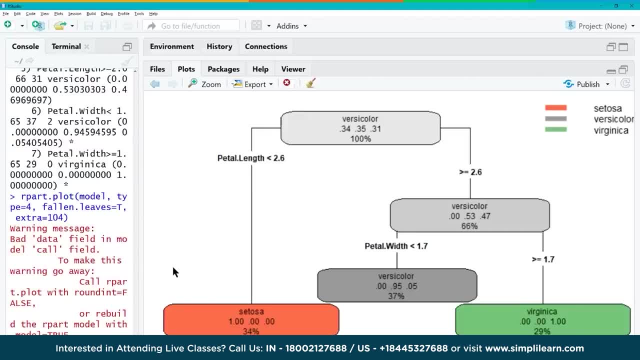 It's going to be a versicolor And if it's greater than 1.7, it's a virginica. And so you can see here it's a very simple tree it forms. It's only got a couple levels. You can see a branch off to the right. Very nice. 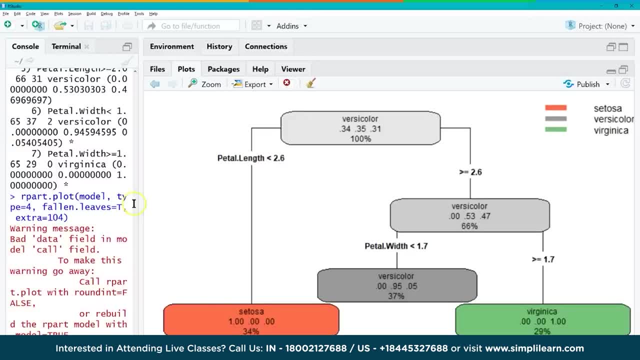 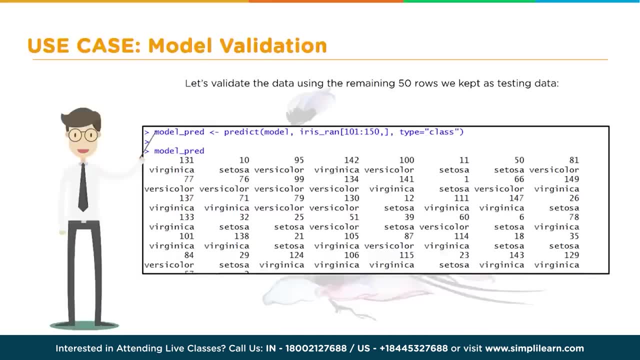 depiction of what's going on as far as the model, now that it's created. But once we create the model, we need to figure out: is this model any good? So let me go back over here. Let's go back to our slides And the first thing we're going to do is we're going to 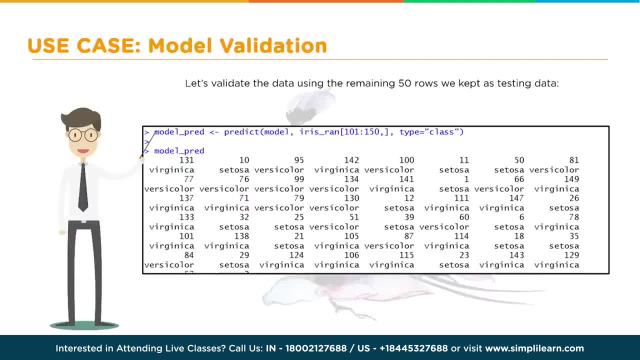 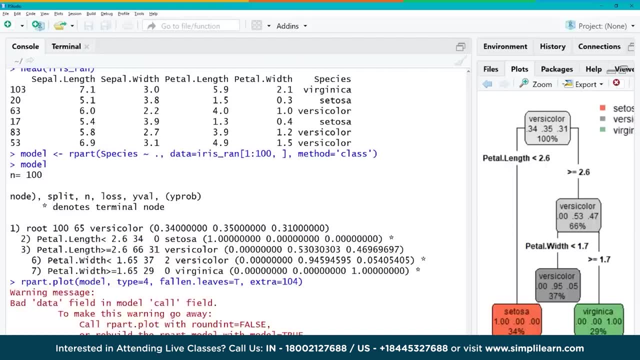 take our test data. Remember we saved 50 rows for the end to go ahead and run a predict on there. So let's go ahead and run that prediction. So we'll call it model underscore predict And we're going to hit a wrong. 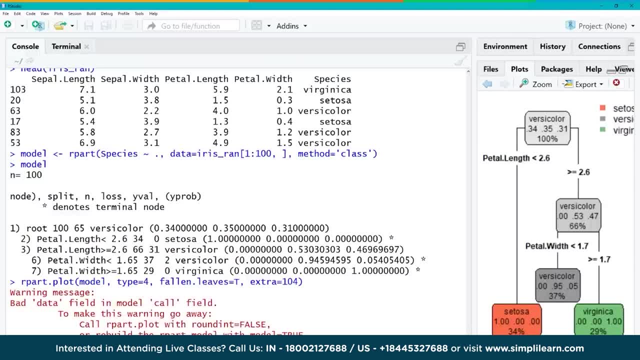 button there to predict. And what are we going to predict? We're going to predict our initial model And we need to send the data. So data equals And we don't actually have to put the data part in, We just put in iris underscore. 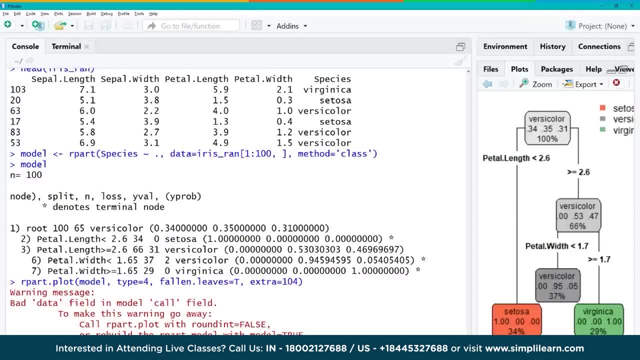 ran, And then we want to do just the last 50 rows And we denote that by 101, colon, 150 and then comma, And we'll leave that part blank, since we want all the columns to show up. And then, finally, this is a classification, So 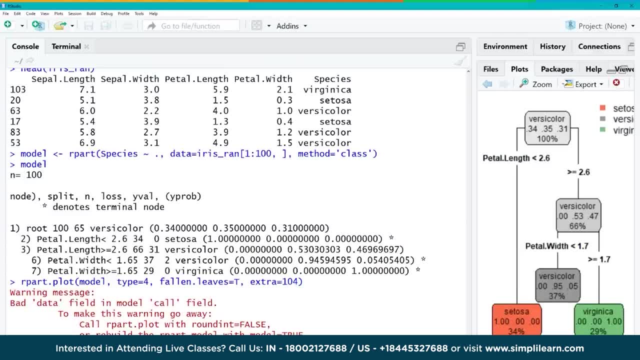 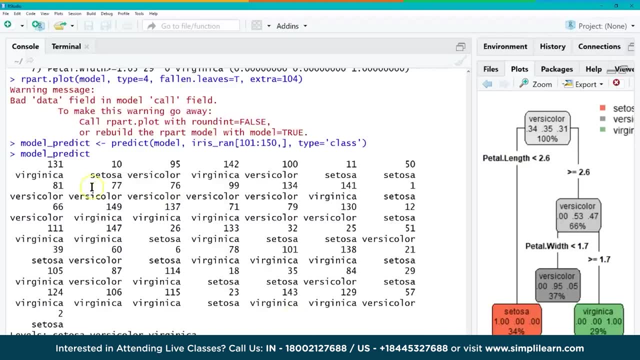 we need to let it know that type equals class. There we go, And let's just see what that looks like. Model predict, And so this is what the data is put out, as It says whatever this is. 131 is a virginica Number. 10 is a setosa Line number. 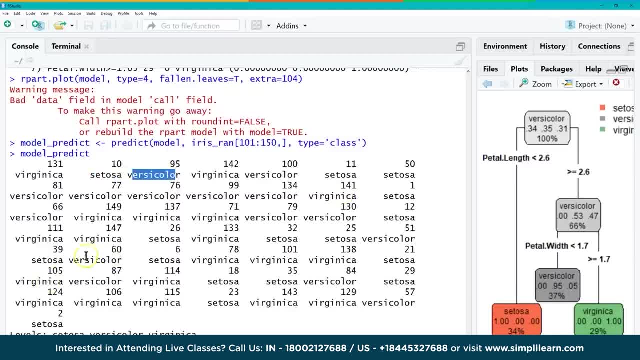 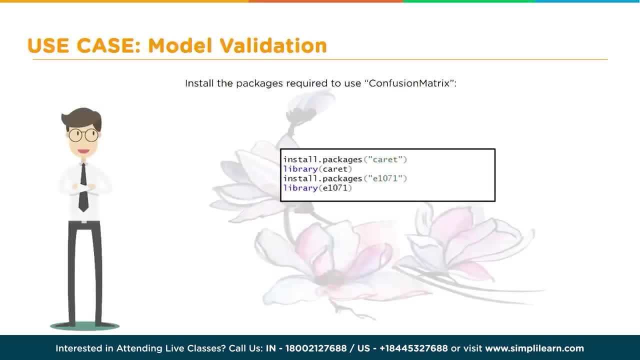 95 is a versicolor, And so on all the way through. What we really want to know is how good our model is, So we're going to go ahead and install a couple more packages. We're going to install the packages required to use the. 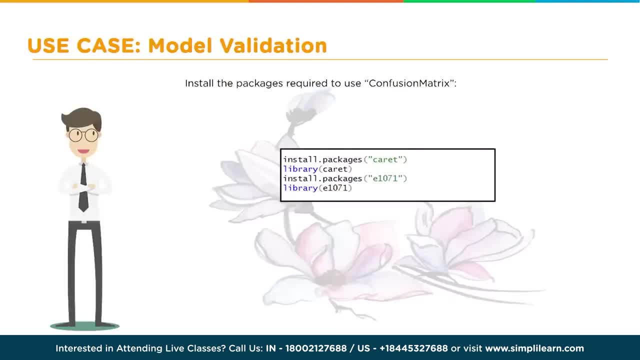 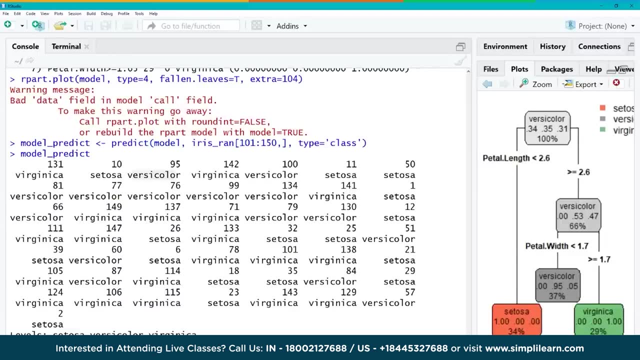 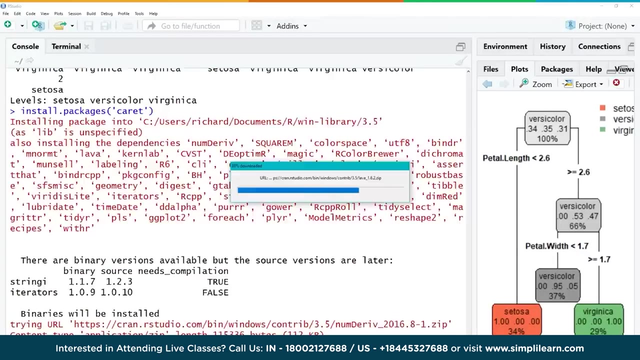 confusion matrix, And to do that we're going to install caret and e1071.. And then of course, we want to set them to our project by using the library command, And so we can simply install packages. And we want caret, And we'll go ahead and just do that. right there There's caret installed And we went ahead. 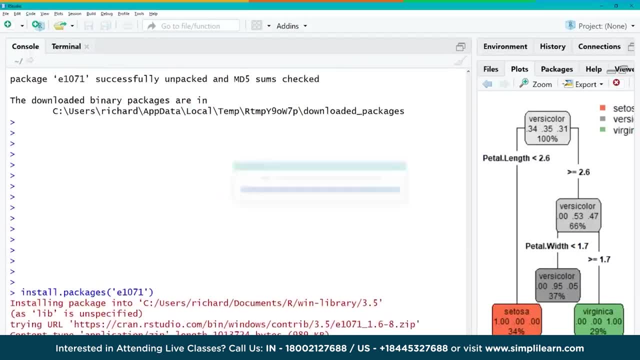 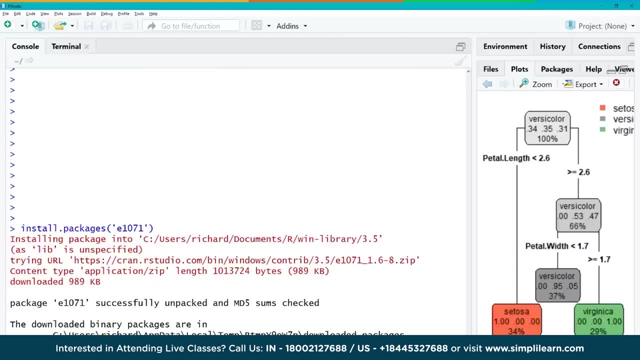 and did the install for packages e1071.. See, it goes through there. It's a really quick install compared to the caret. And then, once we've installed the packages, we need to load it into our workspace. So there's our library caret. Oops, I should load it in there. There it goes. 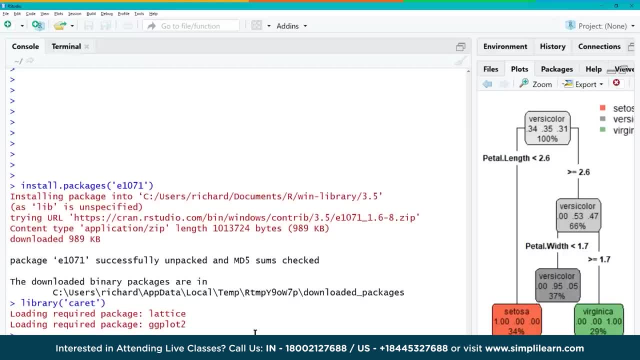 And once that's loaded we'll go ahead and also load the or set the library to the e1071, so that we have both those libraries available to us. And here we go, library, And then this one is e1071. And now these two libraries are fully available to. 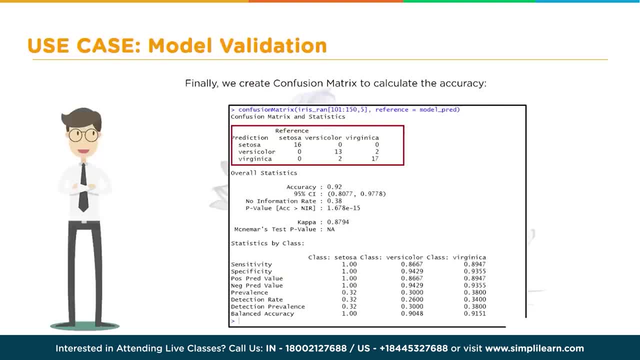 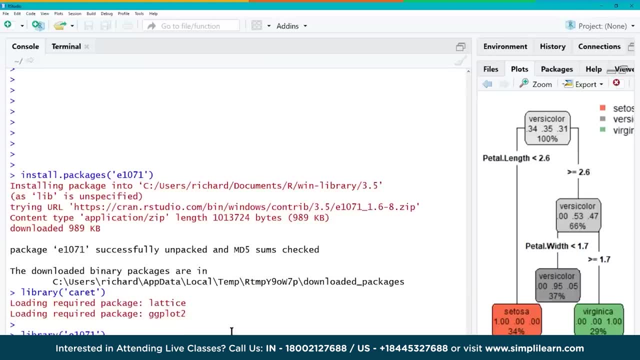 us, And then we're going to use these tools to create the confusion matrix And this one confusion matrix, This is the iris ran, And then we'll go ahead and put the brackets here, And we're only going to do 101 to. 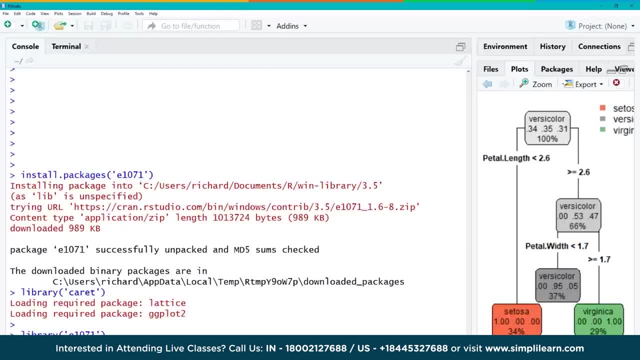 150.. And then we only want the first five columns, Not the last five columns. The first five columns, So five in there And we'll set that to our model predict And then when we hit enter, it's going to head and just print out all this information. So right here we're looking. 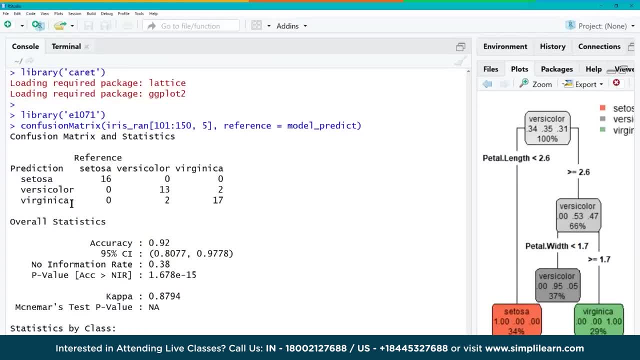 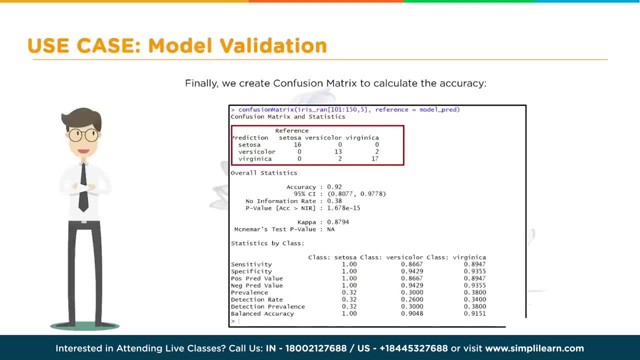 at our confusion matrix to see how everything kind of balances out. Let's go over that and see a little closer what that actually means. So the first part we see is a reference, And in here we have our prediction, because that's what we call. 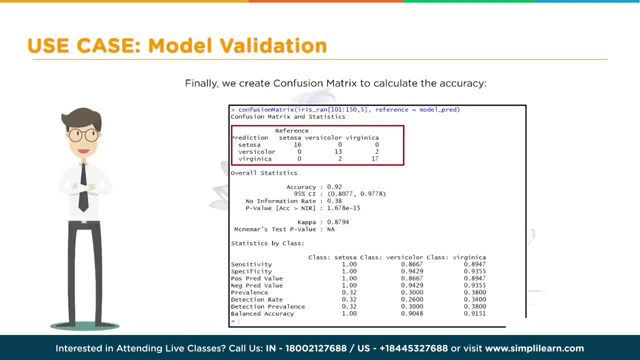 the column, if you remember correctly, And we have it for setosa versicolor virginica, And then we have setosa versicolor virginica going down each side, And the way you read this is, if you look at this, we predicted. 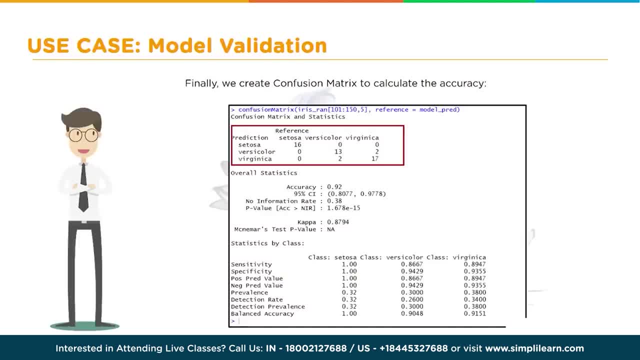 16 out of 16, setosa And then versicolor. we predicted 13 of the versicolor And then two of those we predicted as virginica. So we were wrong on two of those And with the virginica we predicted 17 correct and we had two wrong that were versicolor. So we look at: 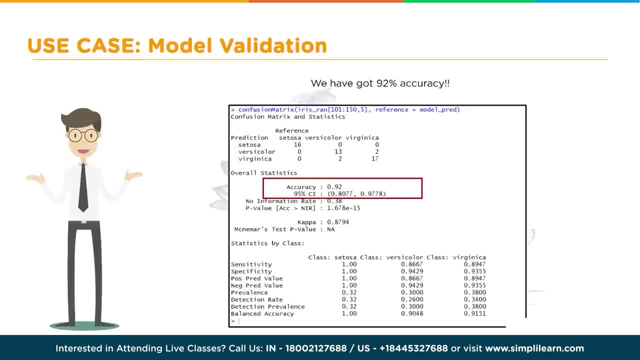 the overall statistics on here And we have an accuracy of .92 and a 95% CI. That's pretty good. as we're going through here, Those are good deals on that And there's a lot more information as you go down this. 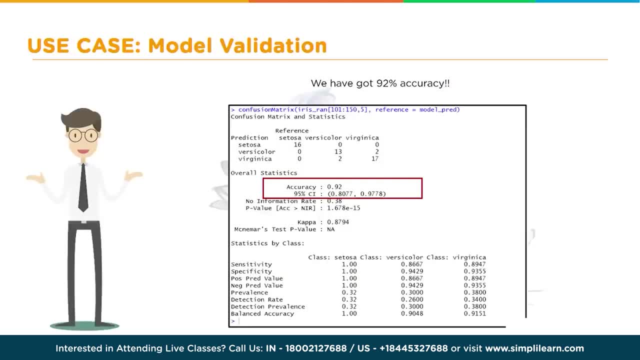 The one thing I want to remind you on this, as we're looking at these predictions- and this is also true for the linear regression model we looked at earlier- When we talk about the accuracy, that is the accuracy on this data- And we say that as a programmer, to make that a very clear distinction, Because if 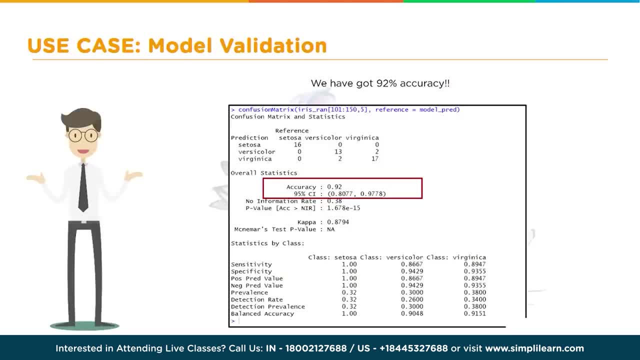 you're in data analysis, you should cringe if I say this is a 95% accurate model without that put in there, Because bad data in, bad data out. We won't go into detail right now on that, but that is very. 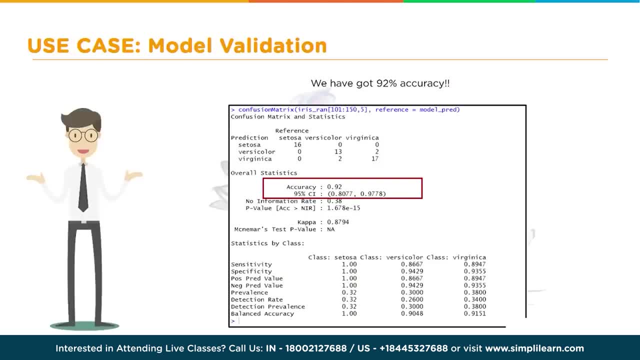 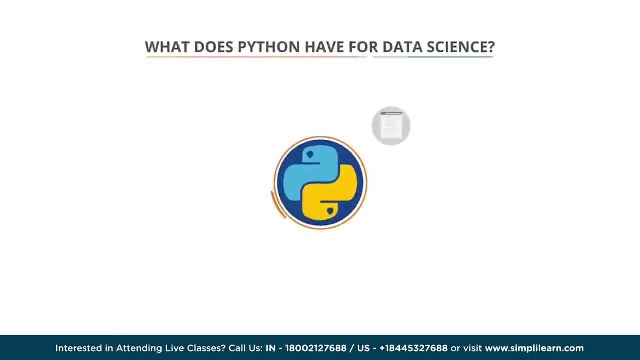 important to note that whenever you quote any of the accuracies on here or you discuss any of these values that come up. So what does Python have for data science? Python is an interpreted, dynamically typed language with a precise and efficient syntax and is renowned for its ease of use to analyze. 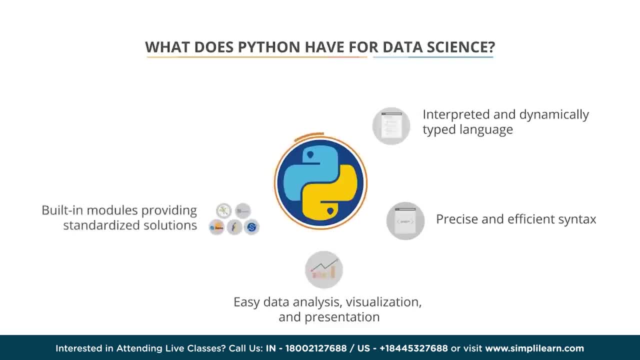 visualize and present data. Python has an extensive library with built-in modules providing easy access to system functionalities, which not only improves accessibility, but also provides standardized solutions for everyday programming challenges By taking away platform specific requirements and replacing them with platform neutral APIs. modules in Python libraries encourage 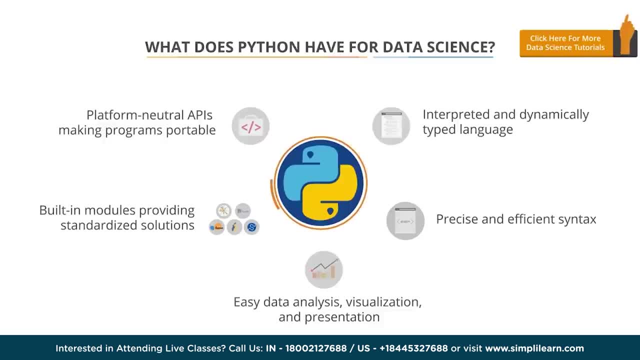 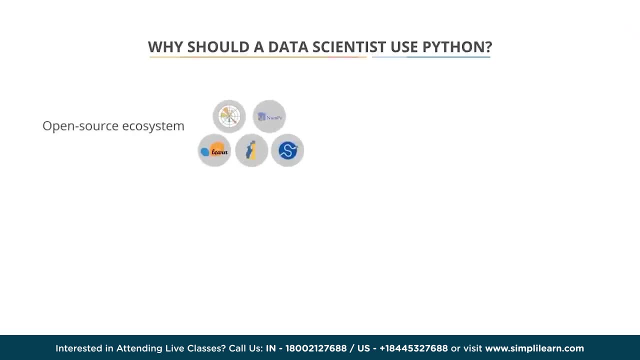 users to make programs portable. Why should a data scientist use Python? Apart from being an open source ecosystem, Python and most of its incredible libraries are platform independent, so you can run this notebook on Windows, Linux or OS 10 without a change. Python is part of the winning formula. 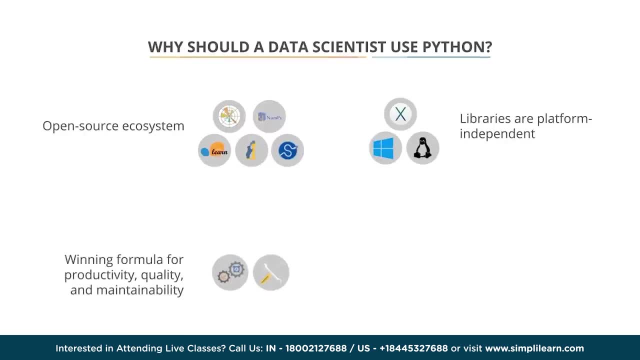 for productivity, software quality and maintainability at many companies and institutions around the world. Python is one of the leading technologies used widely in academic circles and industries because of its flat learning curve. Still not sold on Python? Then here's some proof. 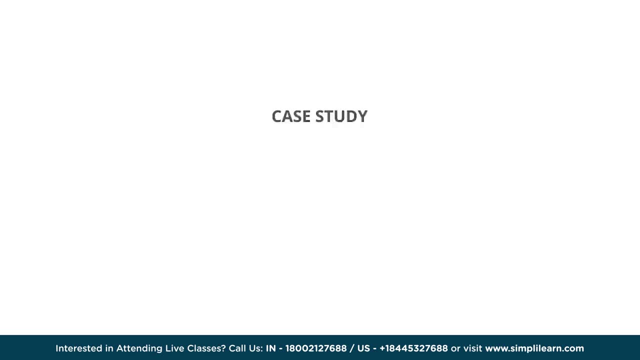 Case Study: Forestwatchcom, a weather report accuracy rating service, is a 100% Python solution, using it in all its components: the front end, back end, as well as the performance critical portions. Python was chosen to develop this solution because it comes with many standard libraries useful in collecting. 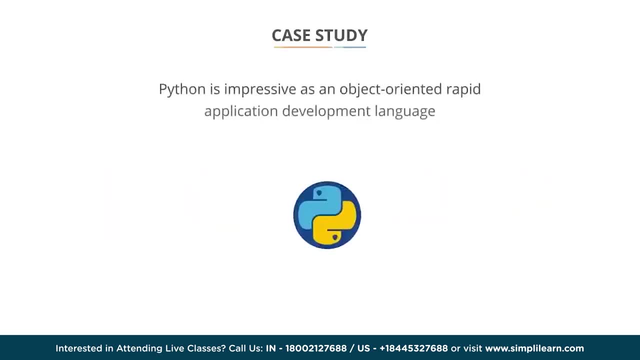 parsing and storing data from the web. Python is impressive as an object-oriented, rapid application development language. One of Python's key strengths lies in its ability to produce results quickly without sacrificing maintainability of the resulting code Because of the clean design of the language. 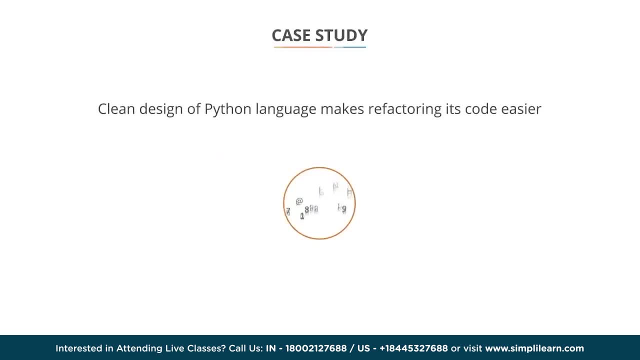 refactoring the Python code was also much easier than in other languages. Moving code from one language to another around simply requires less effort. Forecastwatchcom was made possible because of the ease of programming complex tasks in Python. the rapid development that Python allows the ease to analyze and represent data in a simple 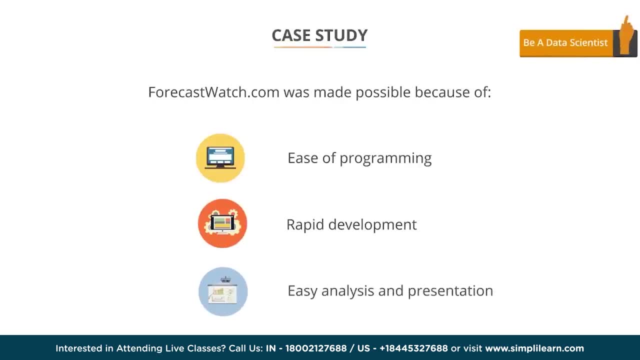 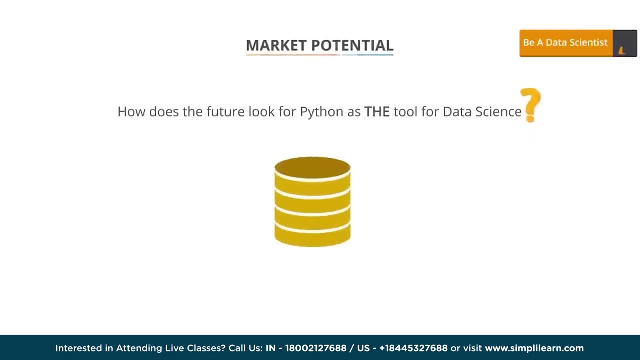 and visually appealing style Market Potential. So how does the future look for Python as the tool for data science? According to Katie Nuggets, 46% of all the data science jobs list Python as the skill required, second only to SQL. According to a survey by the Association for Computing, 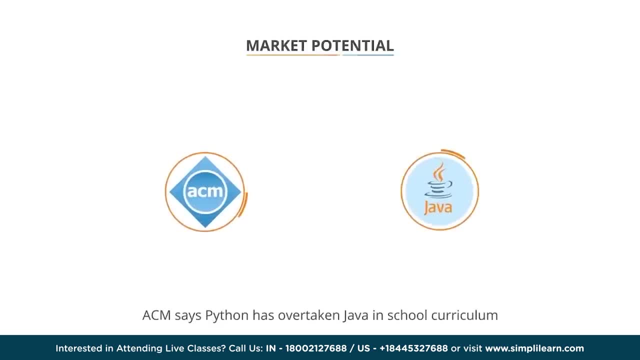 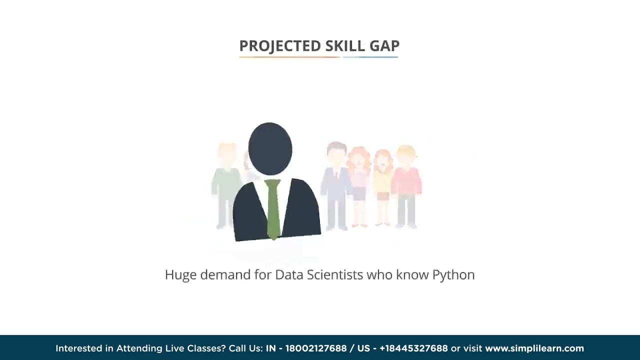 Machinery ACM, posted on javaworldcom. Python has surpassed Java as the top language used to introduce US students to programming and computer science. Projected Skill Gap. There is also going to be a huge demand for data scientists who know Python. McKinsey & Company- a trusted advisor. 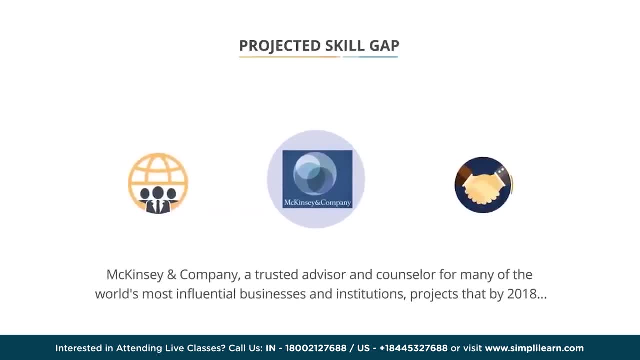 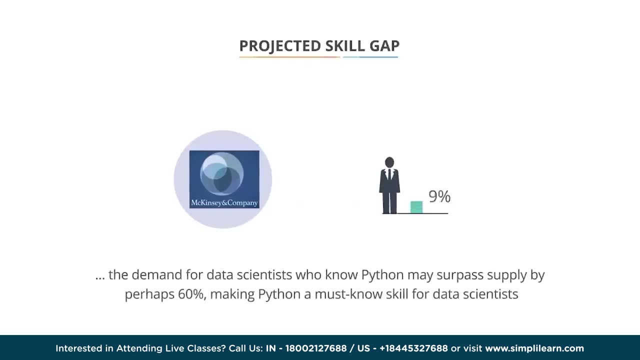 and counselor for many of the world's most influential businesses and institutions, projects that by 2018, the demand for data scientists who know Python may surpass supply by perhaps 60%, making Python a must-know skill for data scientists. Forbescom mentions that the 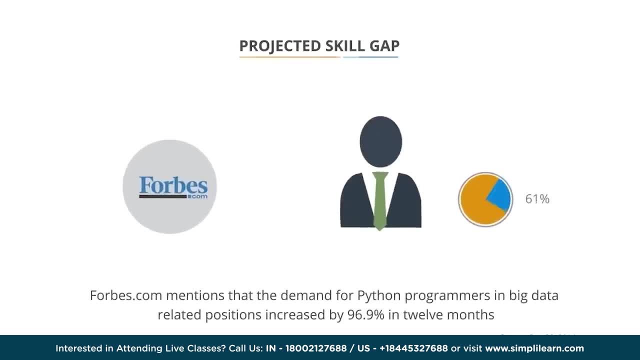 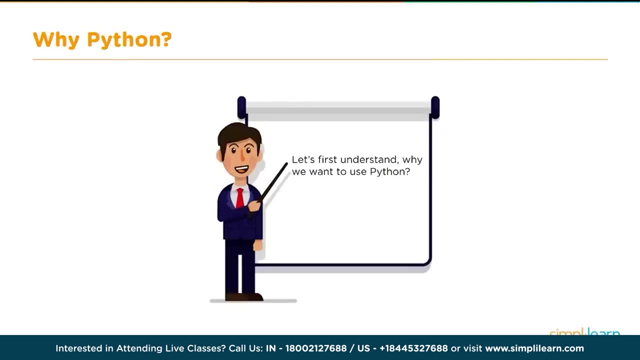 demand for Python programmers in big data related positions increased by 96.9% in 12 months. Now let's talk about Python. For doing data science, we need some kind of a programming language or a tool, and so on. So this session will be about Python. There are other tools like 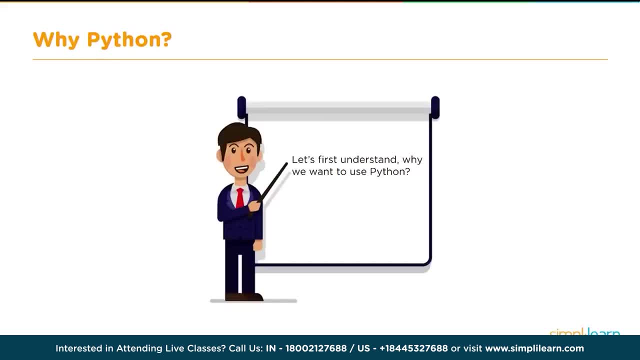 for example, R, and we will probably do a separate video on that. But this session is on Python And you must have already heard. Python is really becoming very popular. Everybody is talking about Python, Not only data science, in IOT and AI and many other places, So it's a very popular. 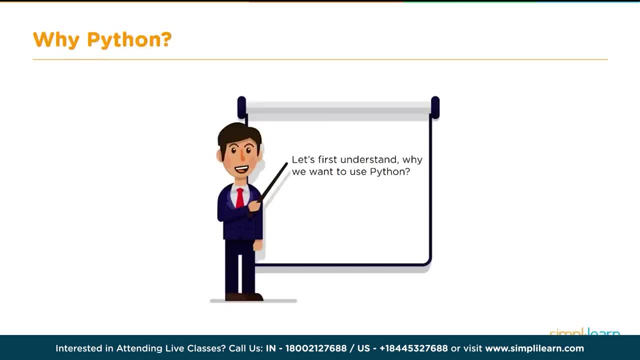 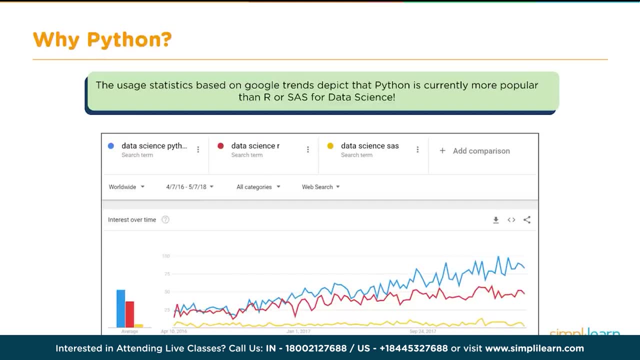 getting very popular. So if you are not yet familiar with Python, this may be a good time to get started with it. So why do we want to use Python? So, basically, Python is used as a programming language, because it is for data science, because it has 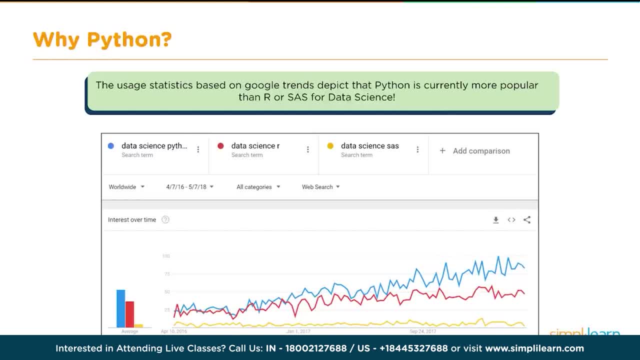 some rich tools. from a mathematics and from a statistical perspective, It has some rich tools. So that is one of the reasons why we use Python And if you see some of the trends- if you are probably tracking some of the trends- you will see that over the last few years Python has become 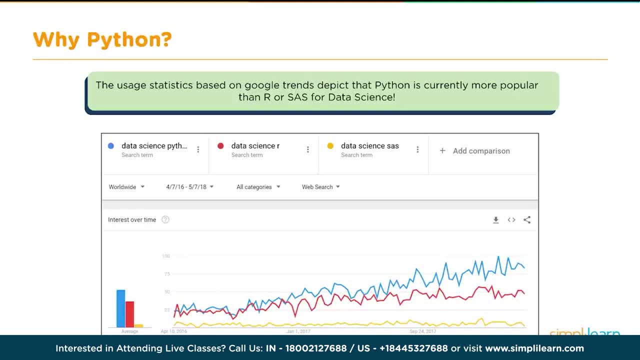 programming language of choice, And especially for data science. SAS was earlier one of the most popular tools, But now, increasingly, Python is being used for doing data science and, of course, as well as R. One of the reasons, of course, is that Python and R are open. 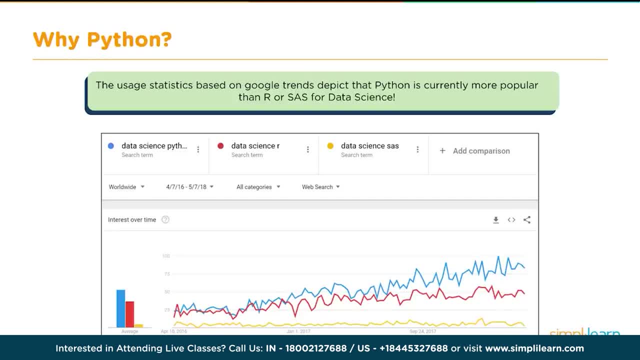 source, compared to SAS, which is a commercial product. So that could definitely be one explanation, But beyond that, I think it is the ease of understanding this language, the ease of using this language, which is also making it very popular, In addition to the availability of fantastic libraries for 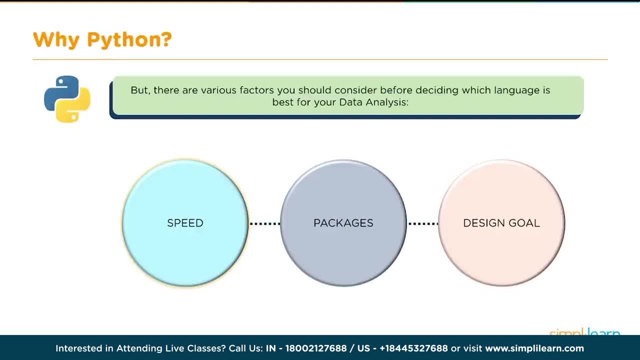 performing data science. What are the other factors? There are speed, then there are availability of number of packages and then, of course, the design goal. Alright, so what are each of these design goals? Primarily, the syntax rules in Python are relatively intuitive and easy to understand. Thereby it helps. 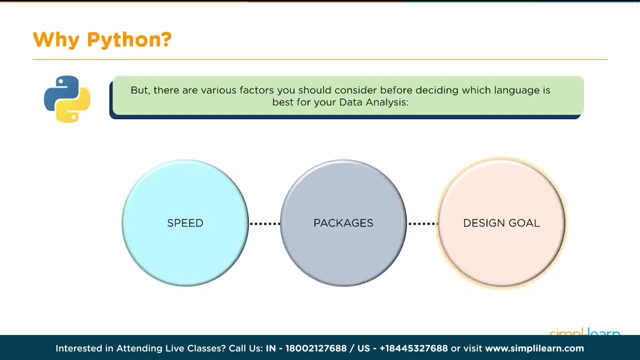 in building applications with concise and readable code base, So with a few lines of code you can really achieve a lot of stuff. And then there are a lot of packages that are available, that have been developed by other people, which can be reused, So we don't have to reinvent the wheel. 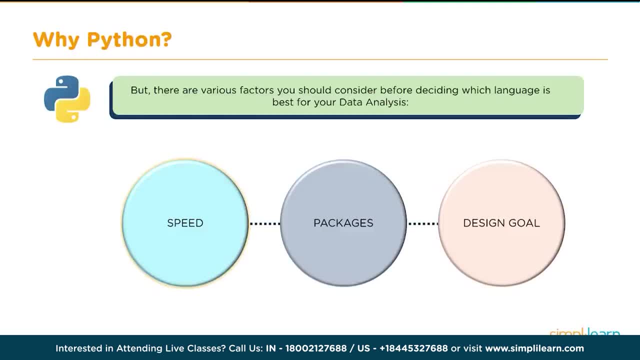 And last but not least, speed. So Python is a relatively faster language. Of course it is not as fast as, let's say, C or C++, but then relatively it is still faster. So these are the three factors which make Python the programming language of choice. 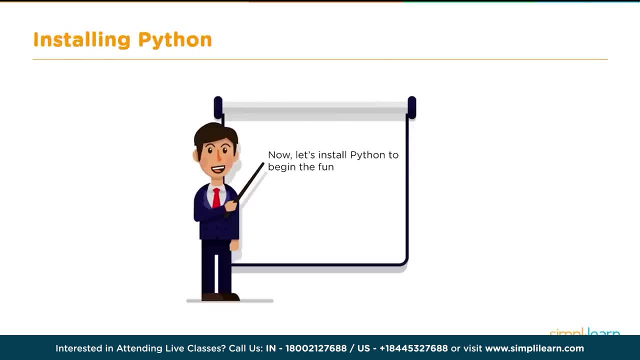 So if you want to get started with Python, the first thing obviously is to install Python. So there is some documentation, There are some steps that you need to follow, So we will try to briefly touch upon that. Otherwise, of course, there is a lot of material available on how to install Python and so on. 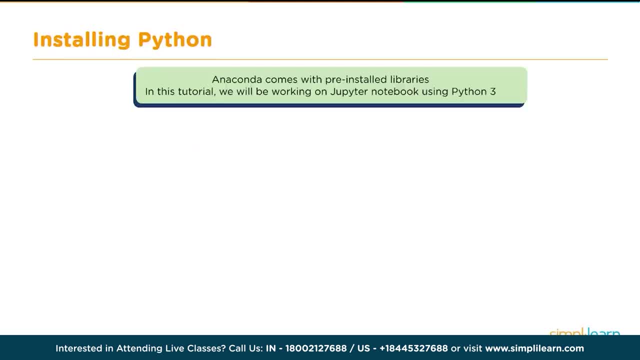 You can always look around, But this is one of the. again, there are different ways in which you can also install Python, So we will use the Anaconda path. There is a packaging tool called Anaconda, So we will use that path. You can also directly. 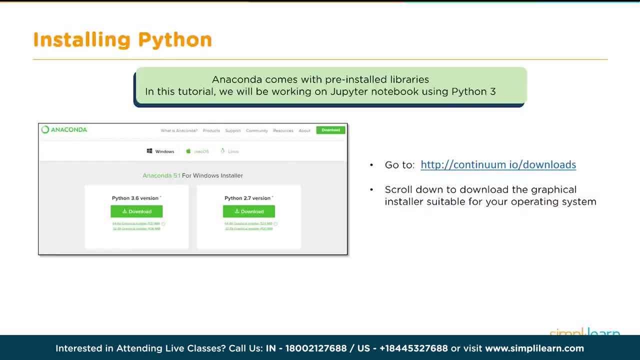 install Python, But in our session we will use the Anaconda route. So the first thing you need to do is download Anaconda, And this is the path for that, And once you click on this you will come to a page somewhat like this- And download. you can do the corresponding download. 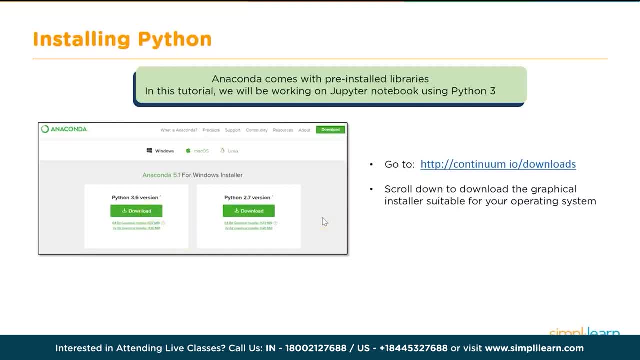 based on whether you have a Windows or Ubuntu. There is also a download possible for a package available for Ubuntu if you are doing something on Ubuntu. So based on which operating system? In fact, this page will automatically detect which operating system you are having and it will. 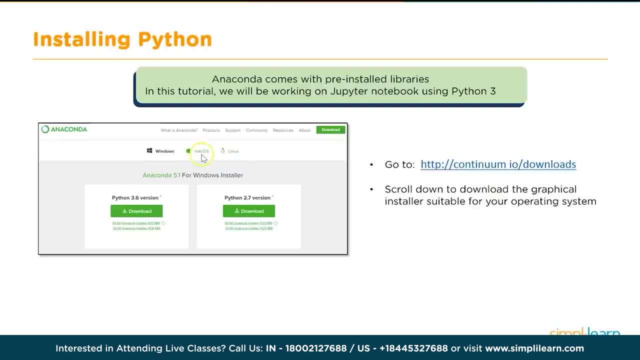 actually suggest. So, for example, you see here, if you are running Mac OS, then it will automatically detect that you have Macs and the corresponding installers will be displayed here. Similarly, if you are on some flavor of Linux, like Ubuntu or any other, Then you will. 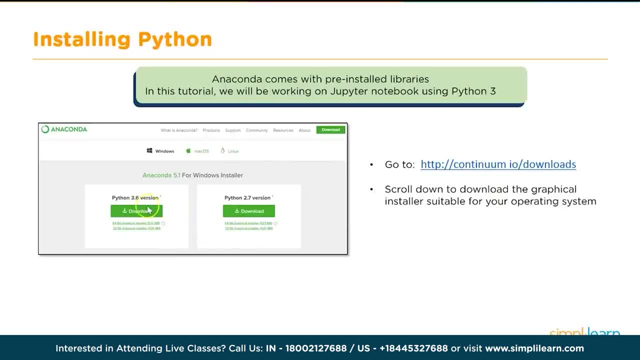 get the corresponding download links here And then, beyond that, you can also select which version of Python you want to install. Of course, the latest version is in the 3.x range at the time of recording. This. 3.6 is one of the latest versions, But some of you 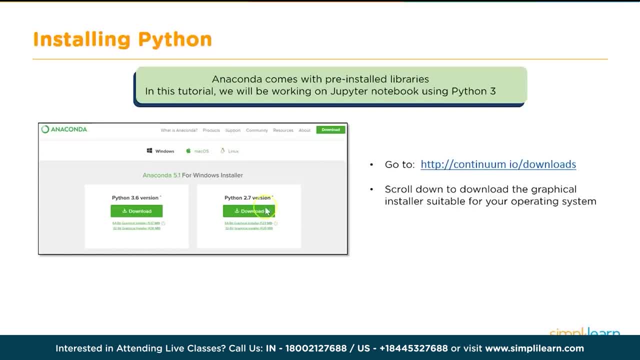 may want to do or start with the earlier version, which is Python 2.7,, 2.x, And you can download that as well. If you don't have anything installed, then my suggestion is to start with Python 3.6.. Alright, so once you do that, you will. 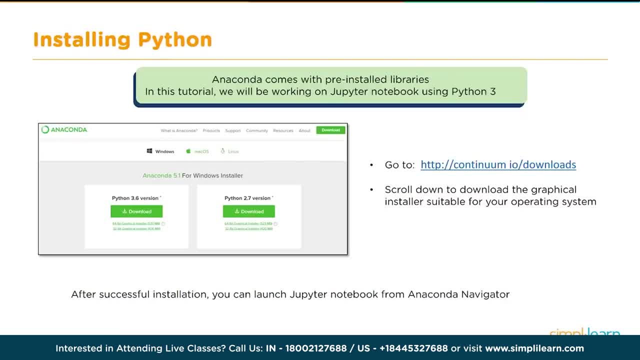 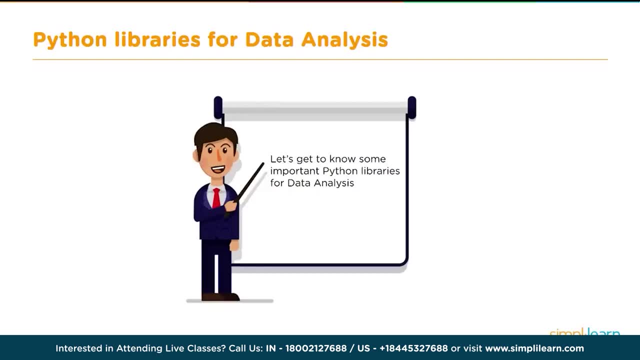 be able to install Python and you will be able to run Jupyter Notebook. Okay, so, now that you know how to install Python, and if you have installed Python, let's take a look at what are the various libraries that are available. So Python is a very easy language to learn and there are some basic. 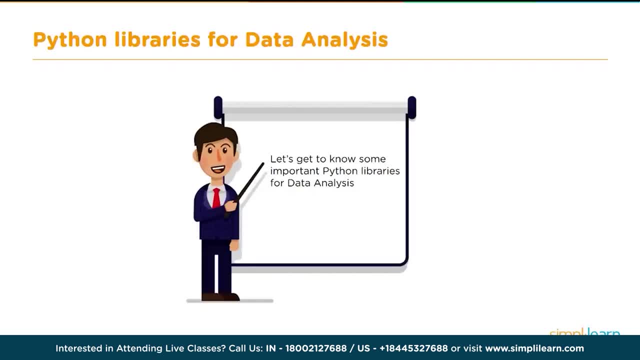 stuff that you can do, For example, adding or printing a single word statement and so on, without importing any specific libraries. But if you want to perform data analysis, you need to include or import some specific libraries. So we are going to talk about those as we move forward. So Pandas, for example. 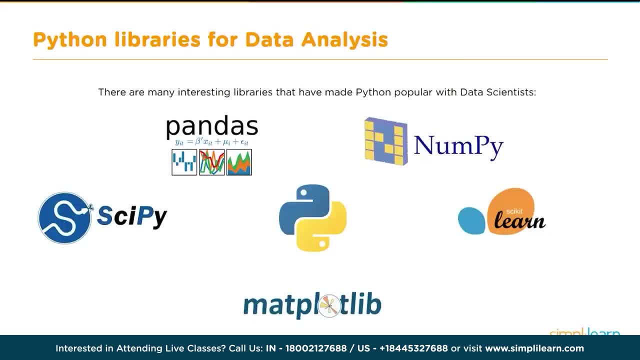 is used for structured data operations. So if you, let's say, are performing something on a CSV file, you import a CSV file, create a data frame and then you can do a lot of stuff like data munging and data preparation, before you do any other stuff like 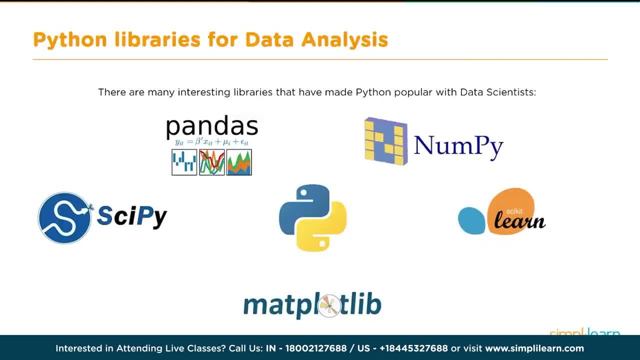 for example machine learning or so on. So that's Pandas SciPy, as the name suggests it is kind of. it provides more scientific capabilities, like, for example, it has linear algebra, it has Fourier transform, and so on and so forth. Then you have NumPy, which is a very powerful 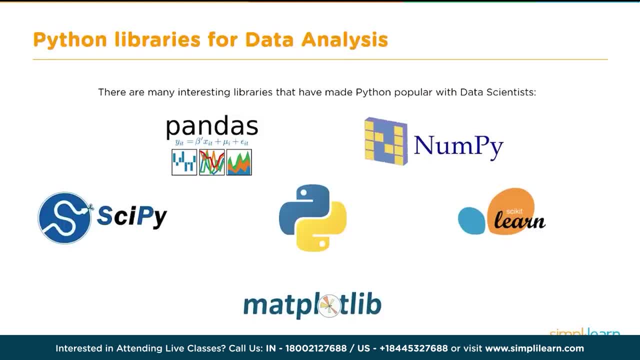 library for performing n-dimensional or creating n-dimensional arrays, and it also has some of the stuff that is there in SciPy, like for example linear algebra and Fourier transform and so on and so forth. Then you have Matplotlib, which is primarily for visualization purpose. It has again very powerful. 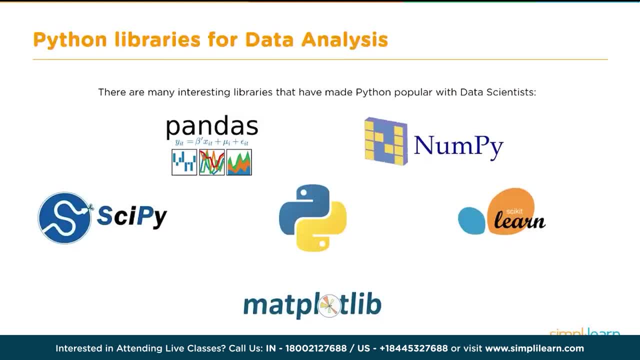 features for visualizing your data, for doing the initial, what is known as exploratory data analysis, for doing univariate analysis, bivariate analysis. So this is extremely useful for visualizing the data, And then Scikit-learn is used for performing. 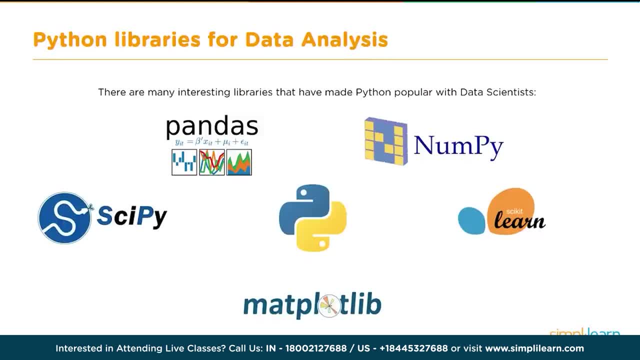 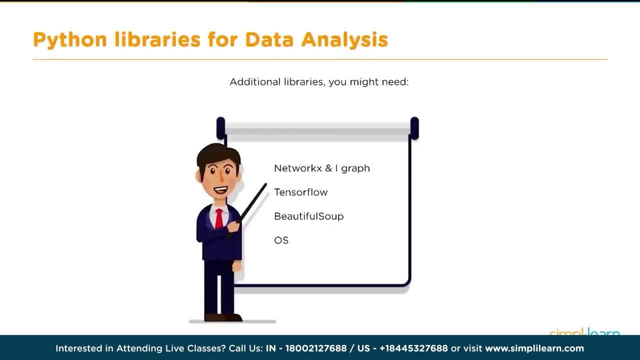 all the machine learning activities. If you want to do anything like linear regression, classification or any of this stuff, then the Scikit-learn library will be extremely helpful. In addition to that, there are few other libraries, for example Networks and iGraph, Then, of course, a. 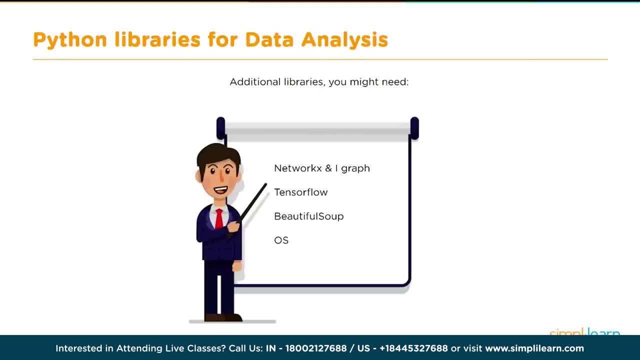 very important one is TensorFlow. So if you are interested in doing some deep learning or AI related stuff, then it would be a good idea to learn about TensorFlow, and TensorFlow is one of the libraries. There is a separate video on TensorFlow. you can look for that, and this is 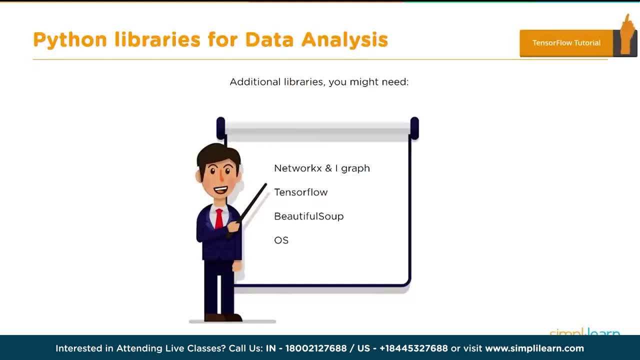 one of the libraries created by Google open source library. So once you are familiar with machine learning, data analysis, machine learning- then that may be the next step to go to deep learning and AI. So that's where TensorFlow will be used. Then you have Beautiful Soup, which is primarily used for web scraping. 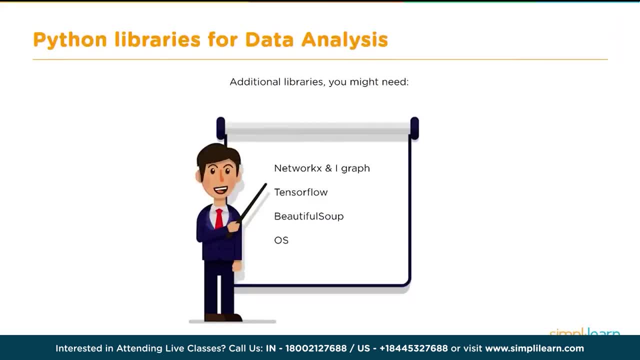 and then you take that data and then analyze and so on, Then OS library is a very common library. as the name suggests, it is for operating system. So if you want to do something on creating directories or folders and things like that, that's when you would use. 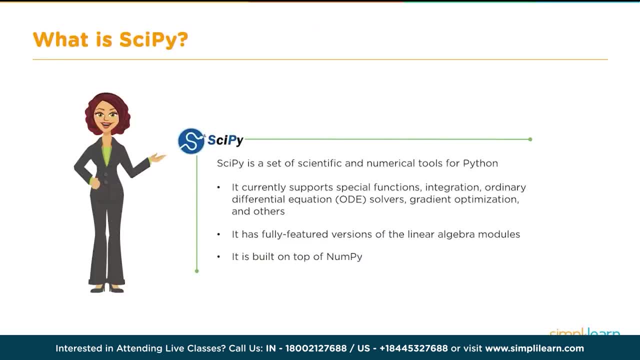 OS. Alright, so moving on, Let's talk in little bit more detail about each of these libraries. So SciPy, as the name suggests, is a scientific library and it very specifically it has some special functions for integration and for ordinary differential equations. So, as you can see, these are mathematical. 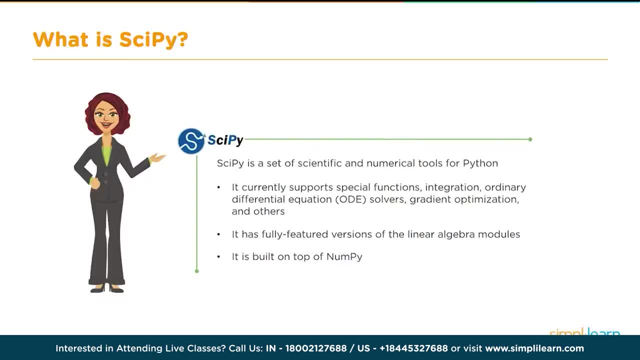 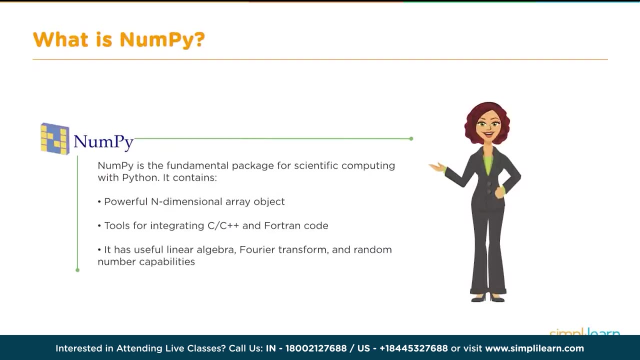 operations or mathematical functions, So these are readily available in this library. And it has linear algebra modules and it is built on top of numpy, So we will see what is there in numpy. So this is again, as the name suggests, that num comes from numbers, So it is a 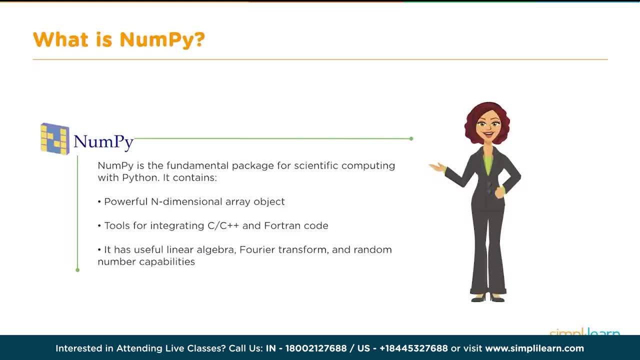 mathematical library, and one of its key features is availability of an n-dimensional array object. That is a very powerful object and we will see how to use this, And then, of course, you can create other, let's say, objects and so on, And it has tools for integrating. 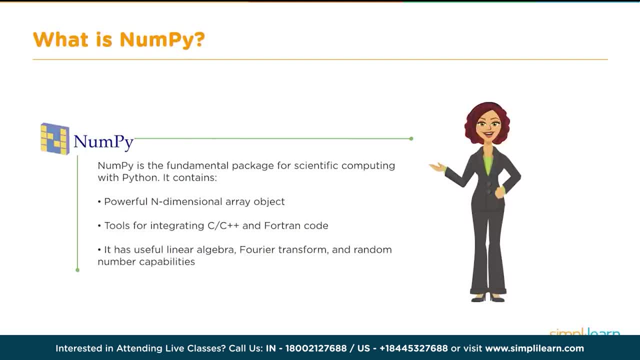 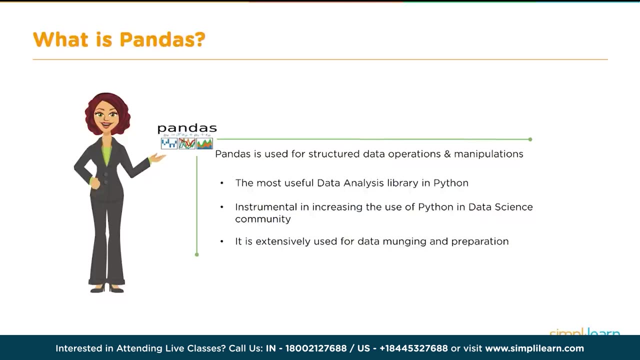 with C, C++ and also Fortran code, And then it of course also has linear algebra and Fourier transformation and so on. All these scientific capabilities, Okay, what else? Pandas is another very powerful library, primarily for data manipulation. So if you are importing any files, you will. 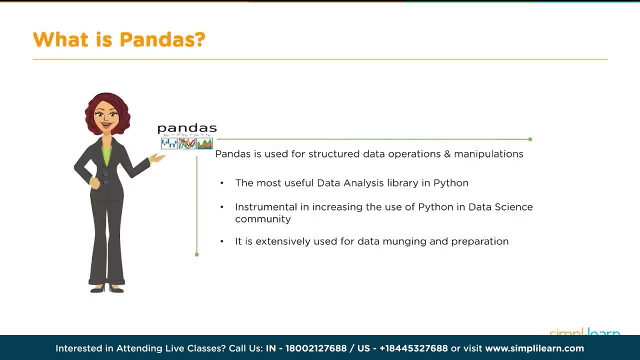 want to create it like a table, So you will create what is known as data frames. These are very powerful data structures that are used in Python programming, So Pandas library provides this capability, and once you import a data into data frame, you can pretty much do whatever you are doing, like in. 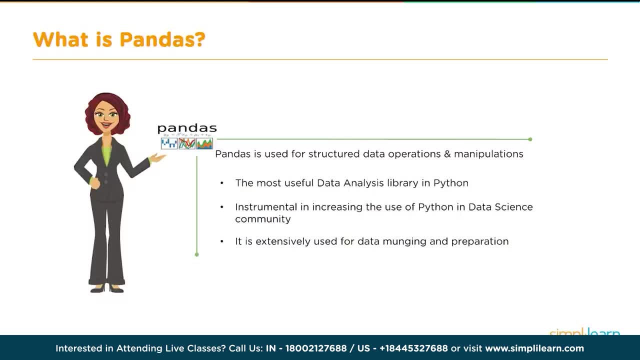 a regular database. So people who are coming from a database background or SQL background would really like this because it is very they will feel very much at home because it feels like you are using, you are viewing a table or using a table and you can do a lot of stuff. 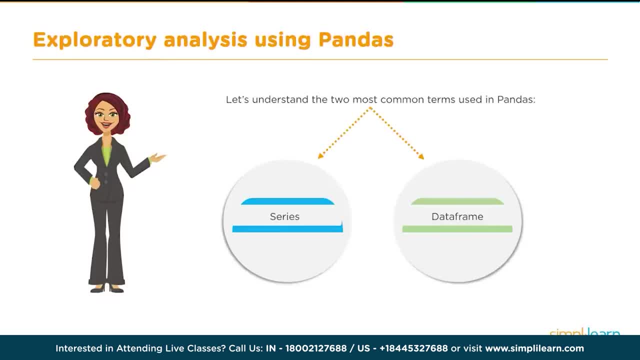 using the Pandas library. Now, there are two important terms or components in Pandas: series and the data frame. I was just talking about the data frame, So let's take a look at what are series and what is data frame. So, within, 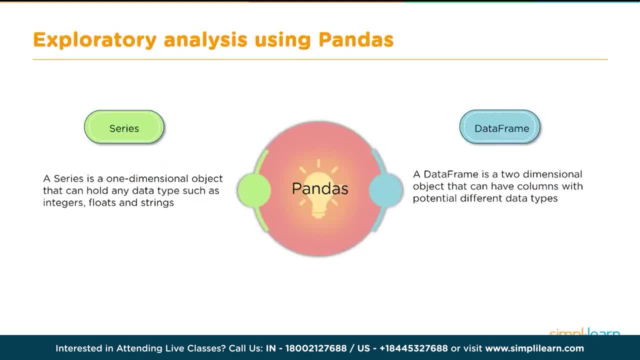 Pandas. we have series and data frame. So series is primarily- some of you may also be knowing this- as, let's say, an array, So it's a one dimensional structure, data structure, if you will. So in some other languages we may call it as an array, or maybe some others probably. 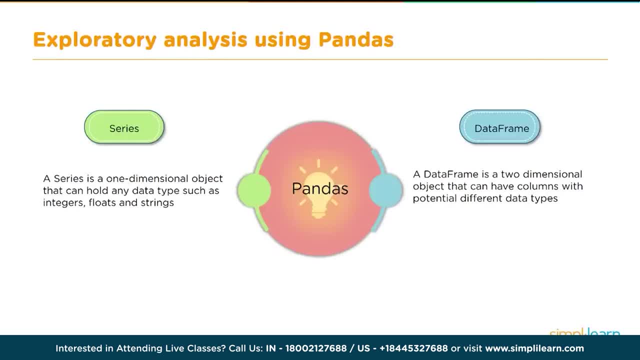 an equivalent of a list. Perhaps I am not very sure on that aspect, but yes, So this is like a one dimensional storage of information, So that is what is series, Whereas data frame is like a table. So you have a two dimensional structure: You have rows and you have columns, and this is very 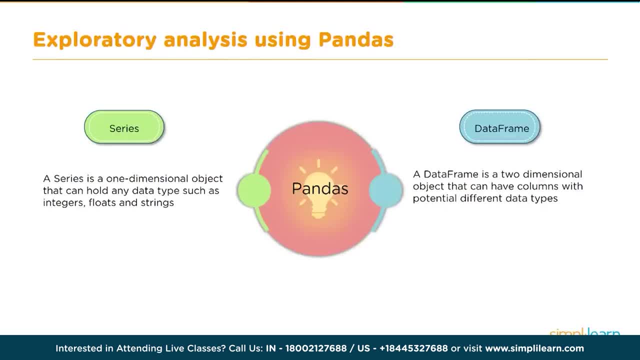 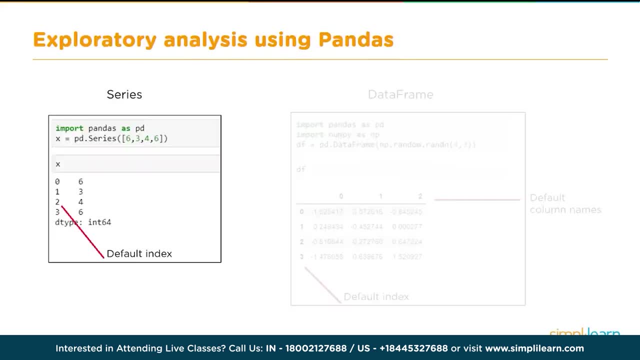 people, as I said, who are familiar with SQL and databases will be able to relate to this very quickly. So you have like a table, you have rows and columns and then you can manipulate the data. So, if you want to create a series, this is how you would create a code snippet And, as you can see, the 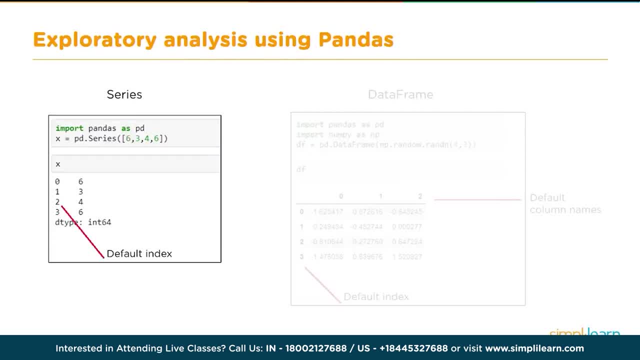 programming in Python is very simple. There are no major overheads. You just need to import some libraries, which are essential, and then start creating objects, So you don't have to do additional declaration of variables and things like that. So that is, I think, one key difference. 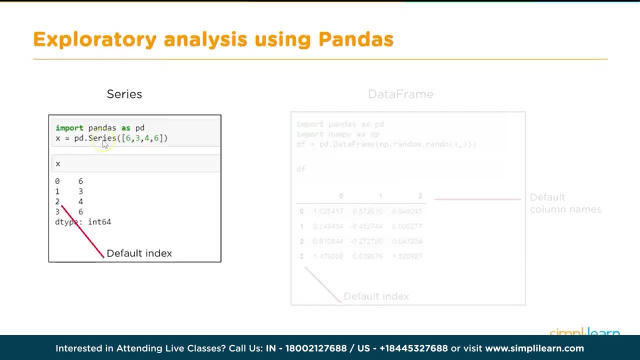 between Python and other programming languages. And what does this series contain? It has to contain these numbers: 6346 and x is my object, consisting of the series. So if you display, if you just say x, it will display the contents of x and you. 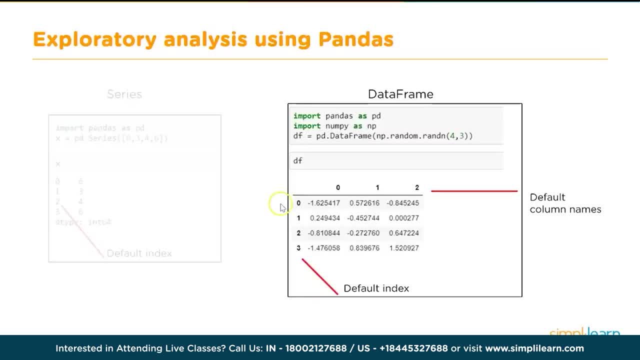 will see here that it creates a default index. then you have data frame. So if you want to create a data frame, as you can see, the series is like a one dimensional structure. There is just like a row, one row of items, Whereas a data frame looks somewhat like this: It is a two dimensional structure. 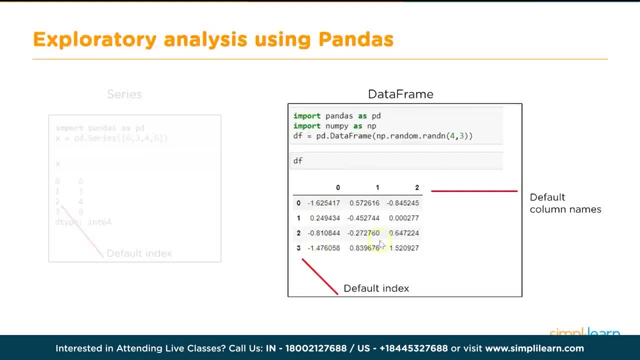 So you have columns in one dimension and then you have rows in the other dimension. How do you create a data frame? You need to create, you need to, rather, import pandas and then you import. in this case, we are basically creating our own data. So that is the reason we are importing numpy, which is 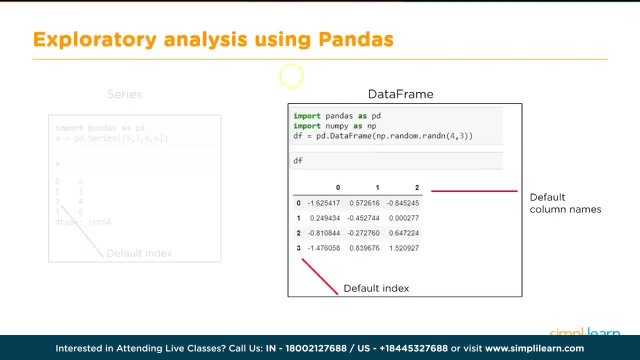 one of the libraries we just referred to little bit before. So we are using one of the functionalities within numpy to create some random numbers. Otherwise this is not really mandatory. You probably will be importing the data from outside, Maybe some csv file and import into the. 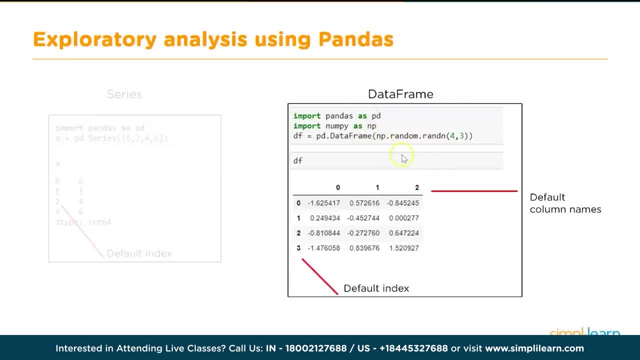 data frame. So that is what we are doing here. So in this case we are creating our own test data. That is the reason we are importing numpy as np, and then I create a data frame saying pd dot data frame. So this is the keyword here. 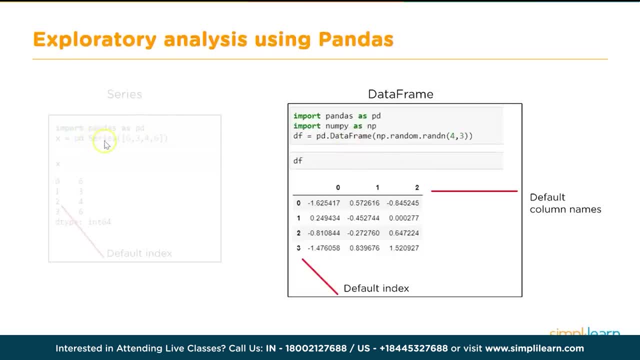 Similarly here. in this case, while creating series, we said pd dot series and then you pass the values. Similarly, here you are saying pd dot data frame. Now, in order to create the data frame, it needs the values in each of these cells. What are the values in the rows and what are the values in the columns, So that 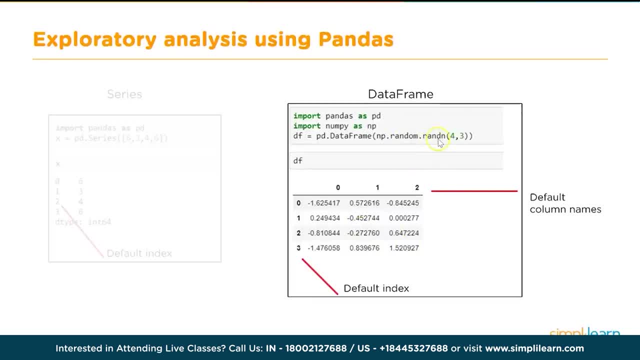 in our example we are providing using this random number generator. So np dot. random is like a class or a method that is available in numpy and then you are saying, ok, generate some random numbers in the form of a 4 by 3 matrix or 4 by 3. 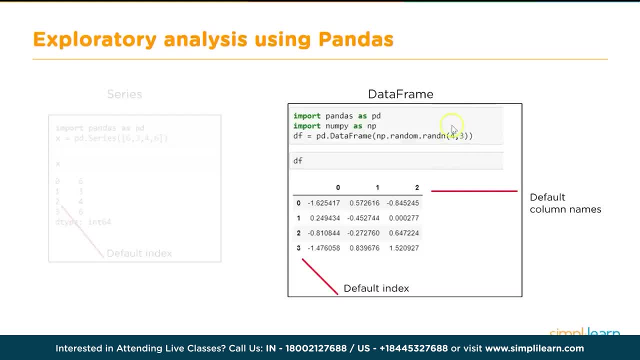 data frame. The 4 here indicates the number of rows and the 3 here indicates the number of columns. So these are the columns: 0,, 1,, 2 are the columns and these are the rows Here: 0, this is 1,, this is 2,, this is 3.. And 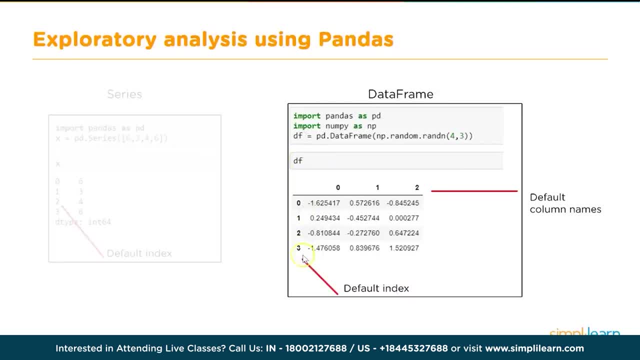 once again, it will. when you display df, it will give us a default index. There are ways to omit that, but at this point we will just keep it simple. So it will display the default index and then the actual values in each of these rows and columns. So this is the way you create. 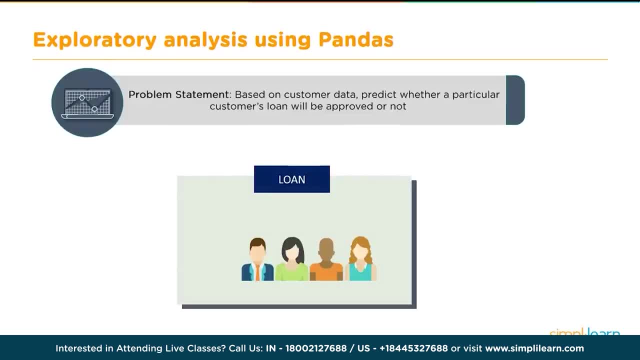 a data frame. So now that we have learnt some of the basics of pandas, let us take a quick look at how we use this in real life. So let us assume we have a situation where we have some customer data and we want to kind of predict whether a customer's loan 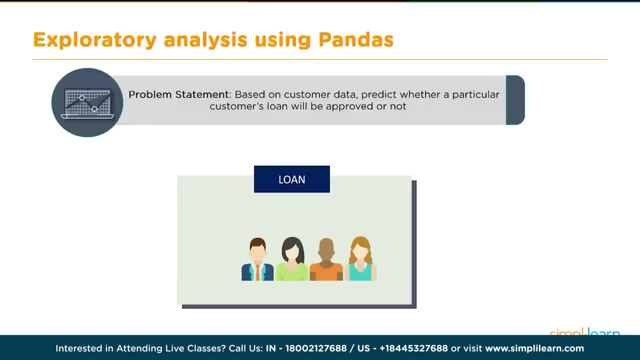 will be approved or not. So we have some historical data about the loans and about the customers and using that we will try to come up with a way to maybe predict whether loan will be approved or not. So let us see how we can do that. So this is part of exploratory analysis. 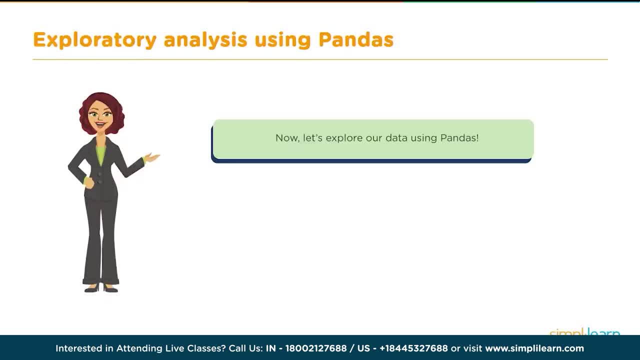 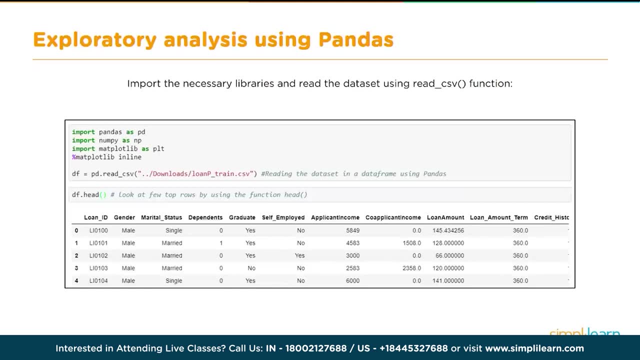 So we will first start with exploratory analysis. We will try to see how the data is looking. So what kind of data? So we will, of course, I will take you into the Jupyter Notebook and give you a quick live demo, But before that, let us quickly walk through some of the pieces of this. 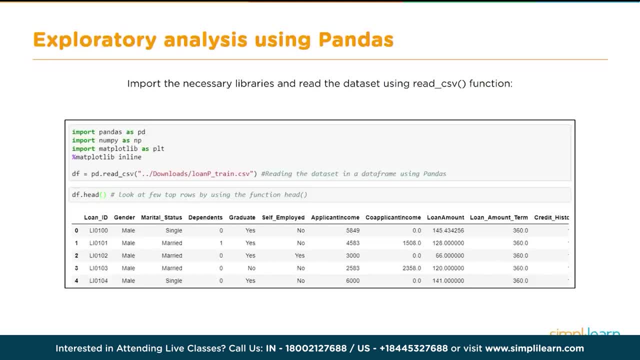 program in slides and then I will take you actually into the actual code and do a demo of that. So the Python program structure looks somewhat like this: The first step is to import your all the required libraries. Now, of course it is not necessary that you have to import all your libraries right at the top of the code. 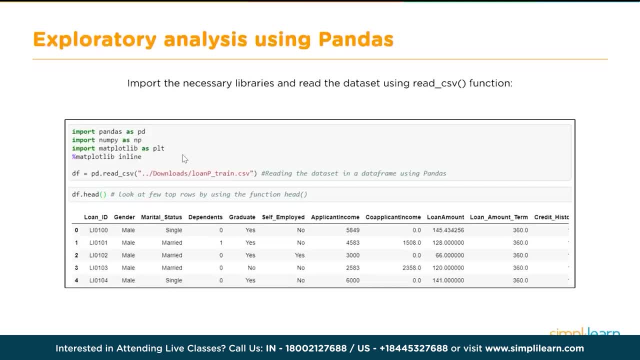 but it is a good practice. So if you know you are going to need a certain set of libraries, it may be a good idea to put from a readability perspective. it is a good practice to put all the libraries that you are importing at the beginning of your code. However, it is not. 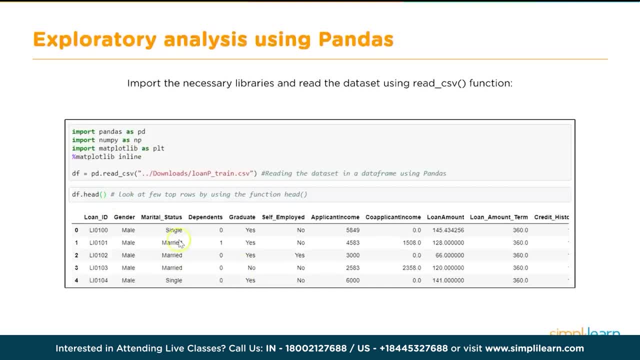 mandatory. So in the middle of the code somewhere, if you feel that you need a particular library, you can import that library and then start using it in the middle of the code. So that is also perfectly fine. It will not give any errors or anything. However, as I said, it is not such 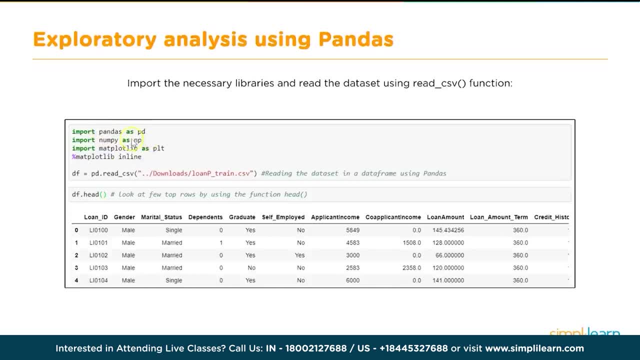 a good practice. So we will import all the required libraries. In this case, we are importing pandas, numpy and matplotlib and, in addition, if we include this piece of code- percentage matplotlib- inline, what will happen is all the graphs that we are going to create, the visualizations that we are going to create. 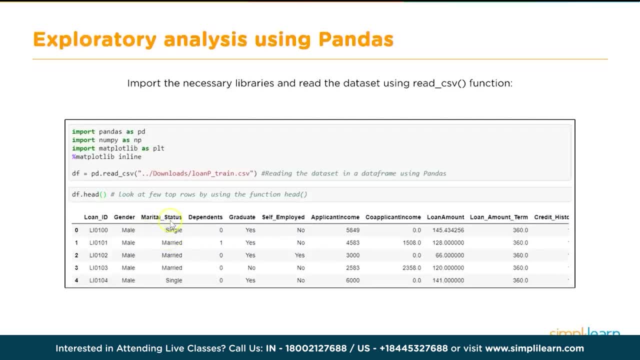 will be displayed within the Notebook. So if you want to have that kind of a provision, you need to have this line. So it is always a good idea when you are starting off, I think it is a good idea to just include this line so that your graphs are shown inline. So these are 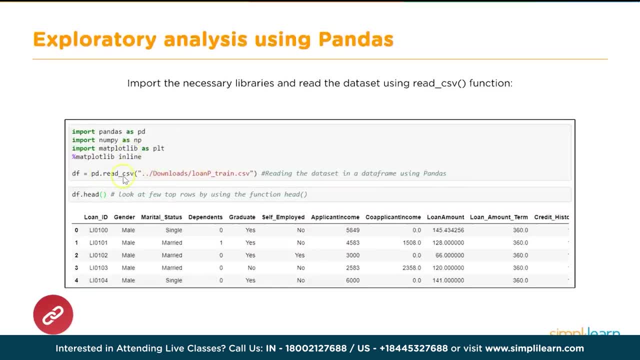 the four. we will start with these four lines of code. Then the next step is to import your data. So in our case, there is a training data for loans by the name loanpe__traincsv and we are reading this data. So in this case, you see here, unlike 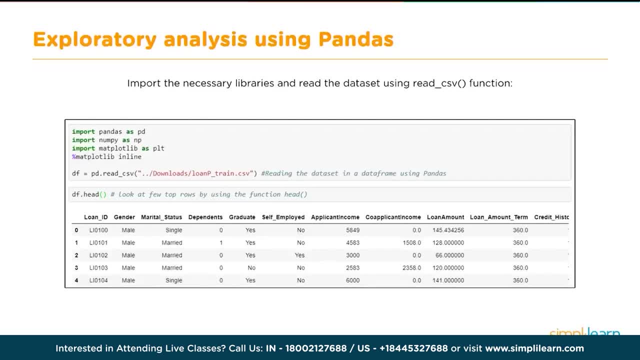 the previous example, where we created a data frame with some data that we created ourselves. Here we are actually creating a data frame using some external data and the method is very, very straight forward. So you use the read underscore csv method and it is a very intuitive function name. 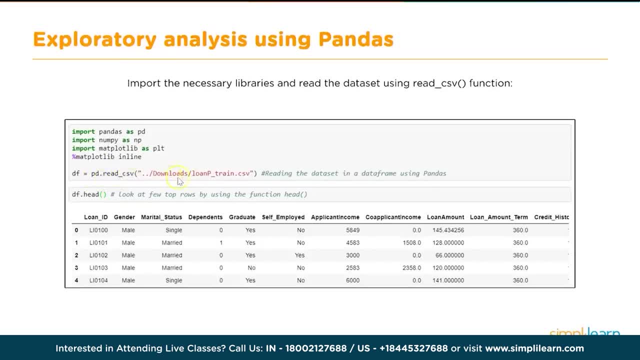 and you say pdread, underscore csv and give the path of the file, csv. file, That is about it and then that is read into the data frame df. This can be any name We are calling it df. you can call xyz anything. This is just the name of the object. 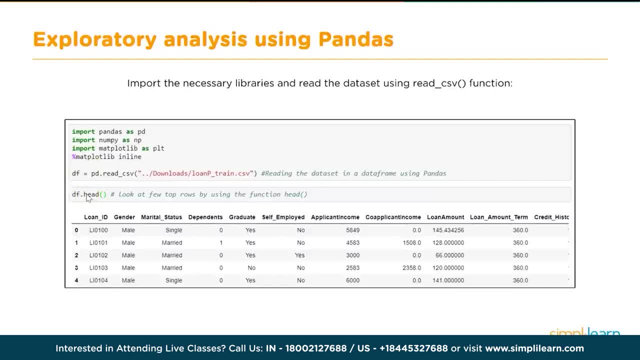 So head is one of the methods within the data frame and it will give us the first five. So this is just to take a quick look. Now you have imported the data, You want to initially have a quick look how your data is looking. What are the values in some of the columns, and so on and so forth. 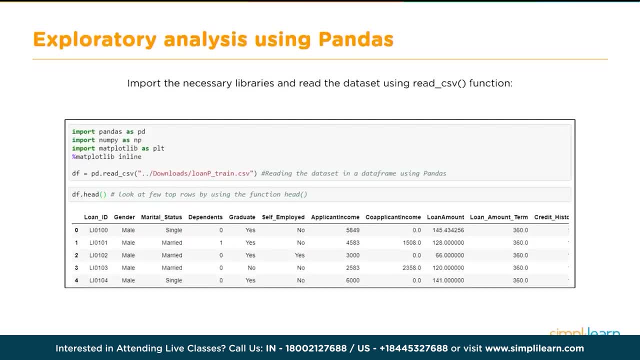 So typically you would do a head dfhead to get the sample of, let's say, the first few lines of your data. So that's what has happened here, So it displays the first few lines and then you can see what are the columns within that and 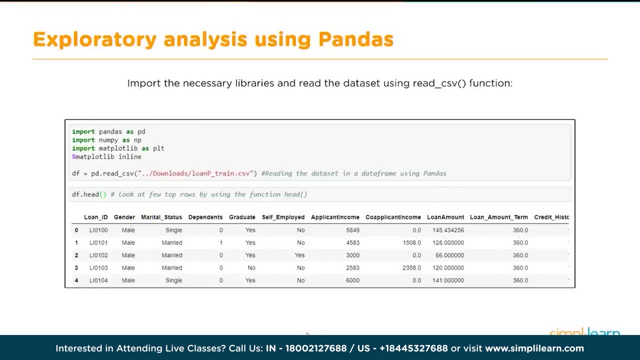 what are the values in each of these cells, and so on and so forth. You can also, typically you would like to see if there are any null values, or are there any? is the data, for whatever reason, is invalid or looking dirty for whatever reason, some unnecessary character? 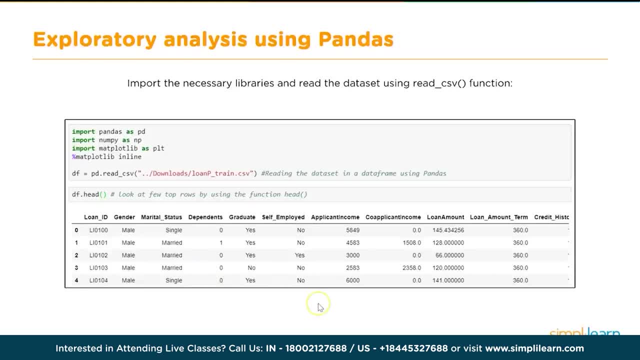 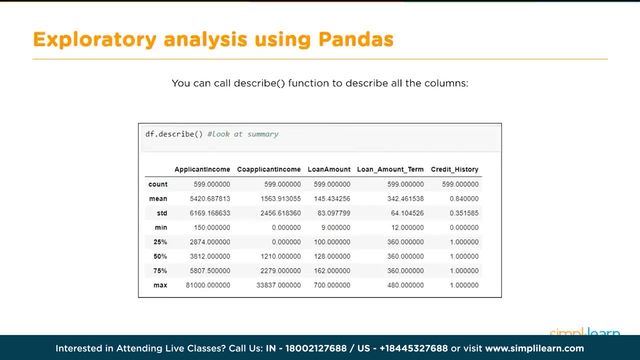 So this will give a quick view of that. So in this case pretty much everything looks okay. Then the next step is to understand the data a little bit overall. for each of the columns, What is the information? So the describe function will basically give us a summary of the data. What else can we do, Pandas? 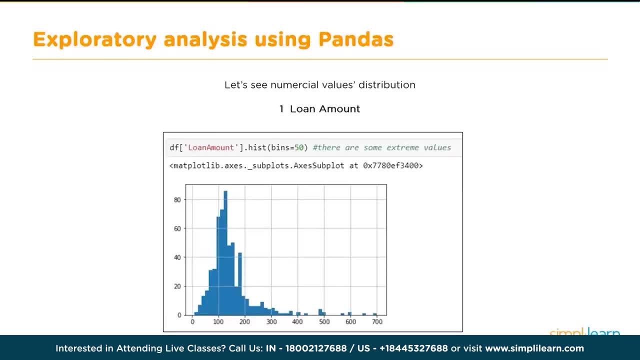 also allows us to visualize the data and this is more like a part of what we call it as univariate analysis. That means each and every column. you can take and do some plots and visualization to understand data in each of the columns. So, for example, 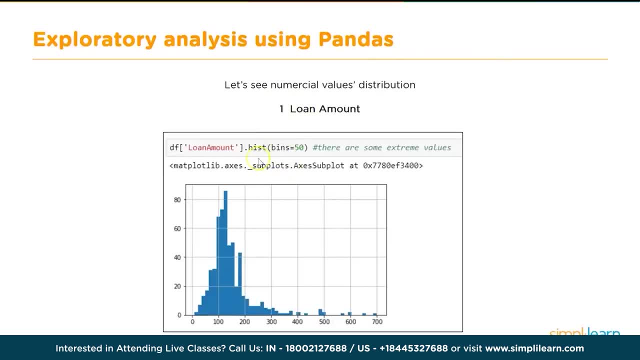 here the loan amount column we can take, and then the HIST. basically HIST method will create a histogram. So you take all the values from one column, which is loan amount, and you create a histogram to see how the data is distributed. So that's what is happening here. 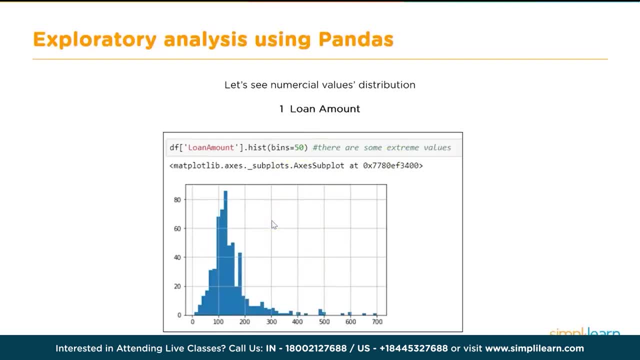 and, as you can see, there are some extreme values. So this is again to identify. do we have to do some data preparation? because if the data is in a completely haphazard way the analysis may be difficult. So these are the initial or exploratory data. analysis is primarily done to understand. 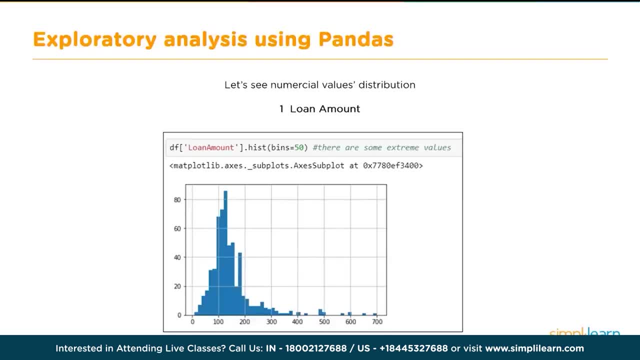 that and see if we need to do some data preparation before we get into the other steps like machine learning and statistical modeling and so on. So in this case we will see that here. by plotting this histogram we see that there are some extreme values. So there are some values, a lot of it is around 100 range. 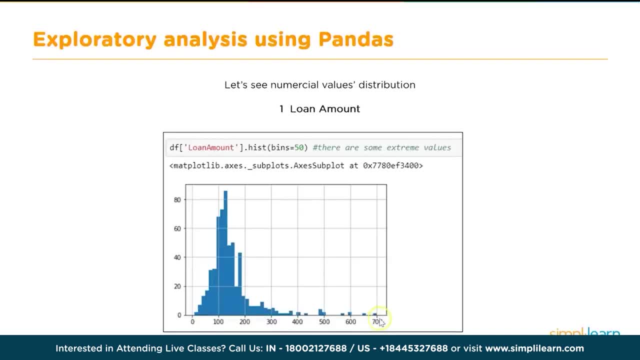 but there is also something 1 or 2 observations in the 700 range, so it's pretty scattered in that sense, or they are not really scattered, distributedly scattered, but it is randomly scattered, So the range is really huge. So what can we do about this? So there are some steps that we need. 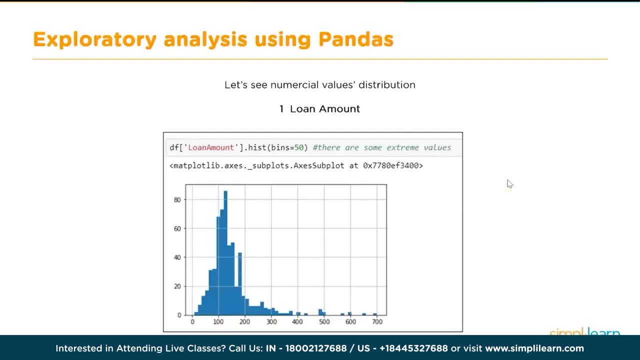 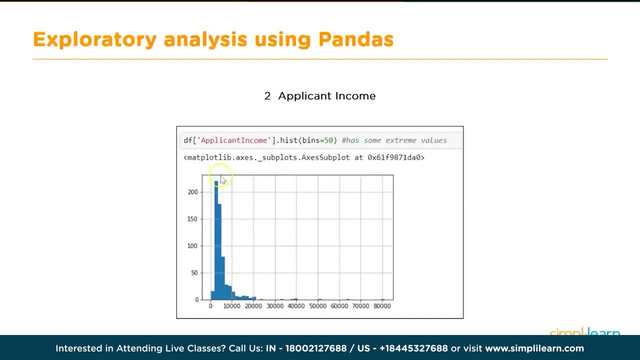 to do normalization and so on. So we will see that in a bit. So this is for one of the columns. Let's take another column, which is applicant income. Similar kind of similar situation. you have most of your observations in this range, but there are also some which are far off from where most of the observations. 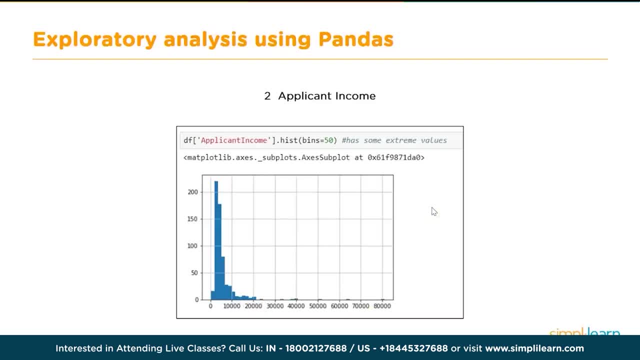 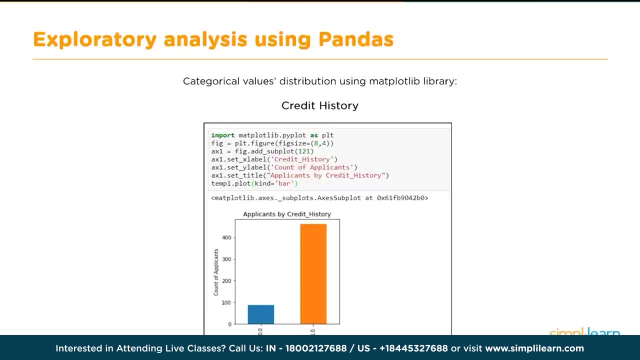 are, So this is also pretty. this also has some extreme values, So we will have to see what can be done. Credit history is the binary value, So some people have a 0 value and some will have credit history of 1.. This is just like a flag, So 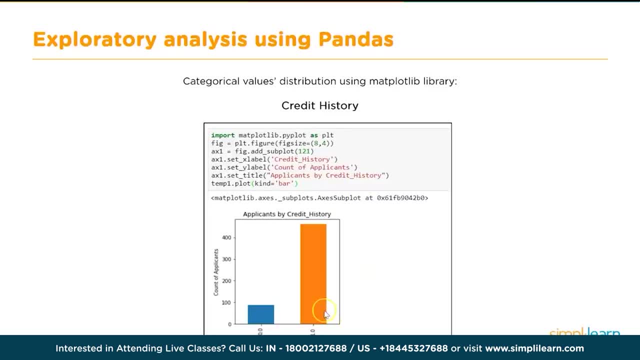 this basically is telling us how many people have a 1 and how many people have 0. So looks like majority of them have a value of 1 and a few- about 100 of them- have a value of 0. Okay, what else can we do? So we now understood a little bit about the data. so 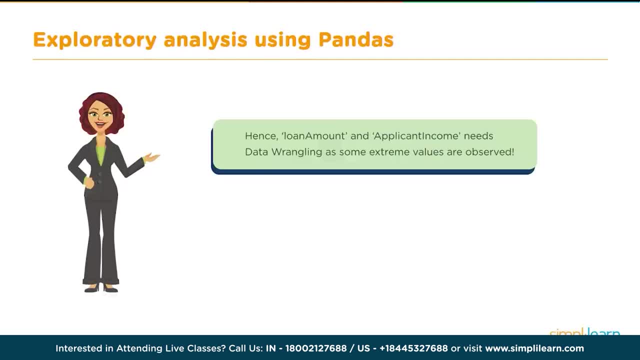 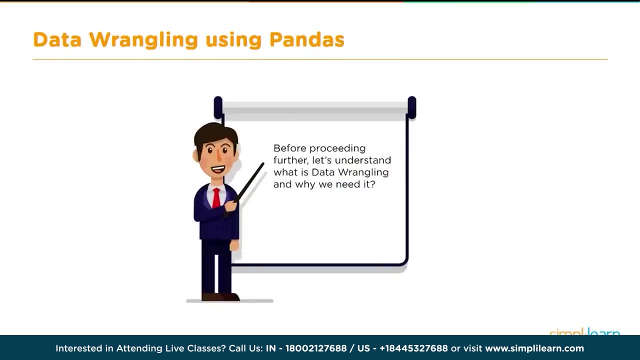 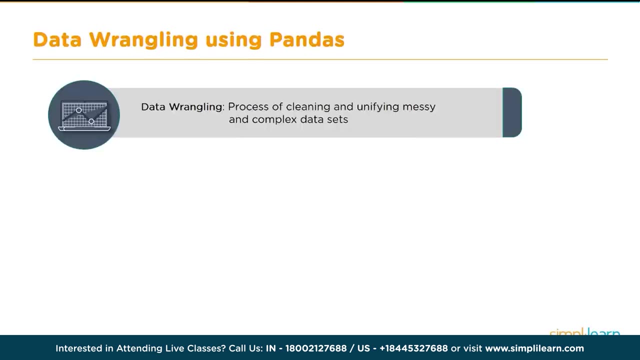 we need to do some data wrangling or data munging and see if we can some bring in some kind of normalization of all this data, and we will kind of try to understand what is data wrangling and before we actually go into it. So data wrangling is nothing but a process of cleaning the data. 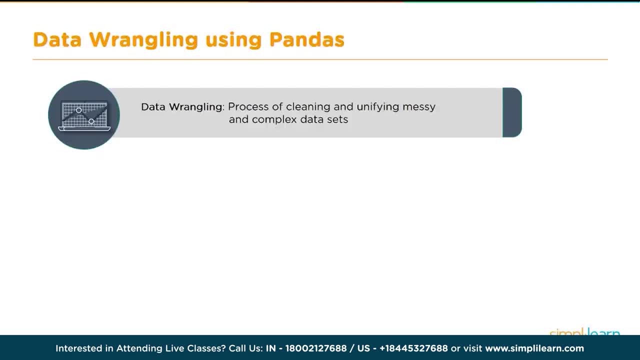 if, let's say, there are multiple things that can happen. In this particular example there were no missing values, but typically when you get some data, very often it will so happen that a lot of values are missing. Either they are null values or there are a lot of 0s. 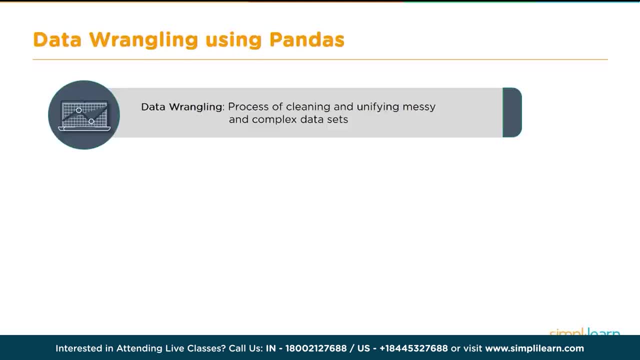 Now you cannot use such data as it is to perform some, let's say, predictive analysis, or perform some machine learning activities and so on. So that is one part of it. So you need to clean the data. The other is unifying the data. Now these ranges of this data are: 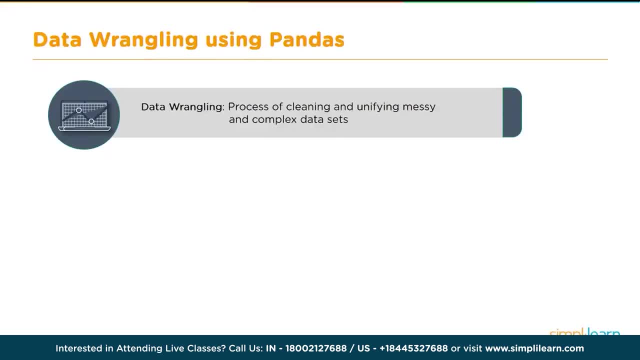 very huge. Some of them are going from. some columns are going from 0 to 100,000, and some columns are just between 10 to 20 and so on. These will affect the accuracy of the analysis, So we need to do some kind of unifying. 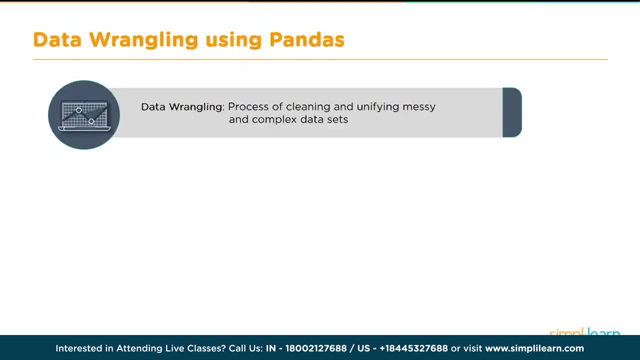 the data and so on. So that is what data wrangling is all about. So before we actually perform any analysis, we need to bring the data to some kind of a shape so that we can perform additional analysis, actual analysis on this and get some. 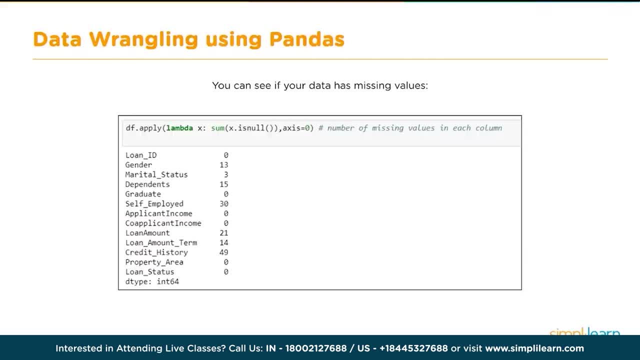 insights. Now, how do we deal with missing values? This is a very common issue when we take data or when we get data from the business, When a data scientist gets the data from the business. So we should never assume that all our data will be clean and all. 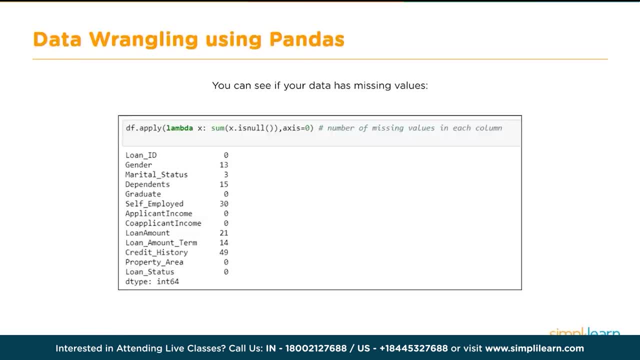 the values filled up and so on, because in real life very often there will be the data will be dirty. So data wrangling is the process where you kind of clean up the data: First of all identify whether the data is dirty and then clean up. So how do we find? 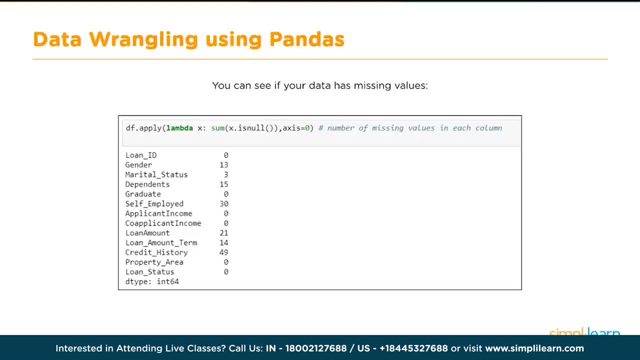 some data is missing. So there are a few ways You can write a small piece of code which will identify if, for a given column or for a given row, any of the observations are null. primarily So this line of code, for example, is doing that. It is trying to identify. 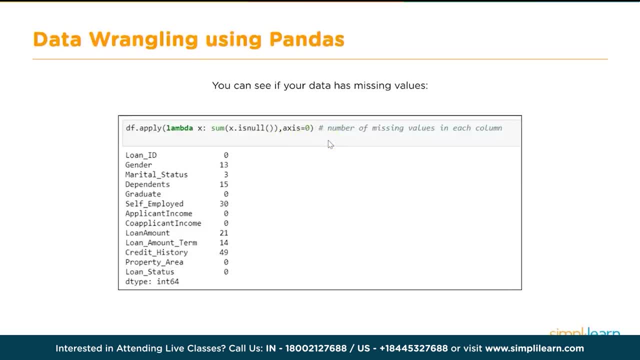 how many null values or missing values are there for each of the columns. So this is a lambda function and what we are saying is find out if a value is null, and then you add all of them. How many observations are there where this particular column is? 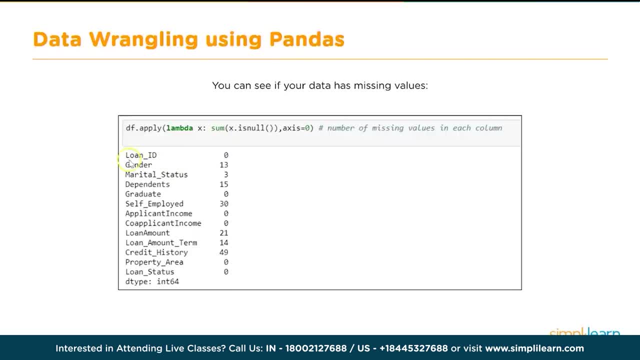 null. So it does that for all the columns. So here you will see that for loan id, obviously it is an id. so there are no null values or missing values. Gender has about 13 observations where the values are missing. Similarly, marital status has 3, and so on and so forth. So we will see here. 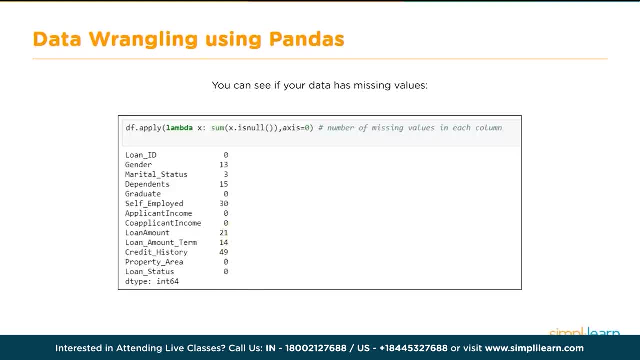 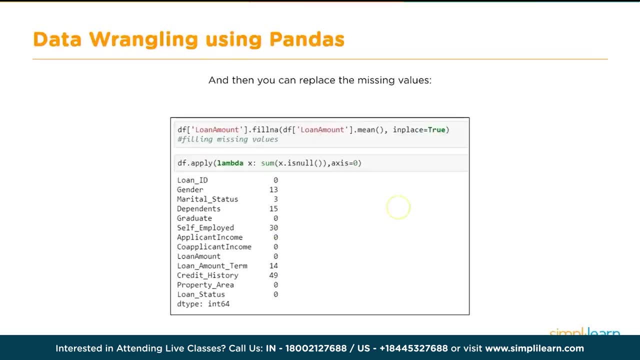 for example, loan amount has 21 observations. where the values are missing, Loan amount term has 14 observations, and so on. So we will see how to handle this: missing values. So there are multiple ways in which you can handle missing values. If the number of observations 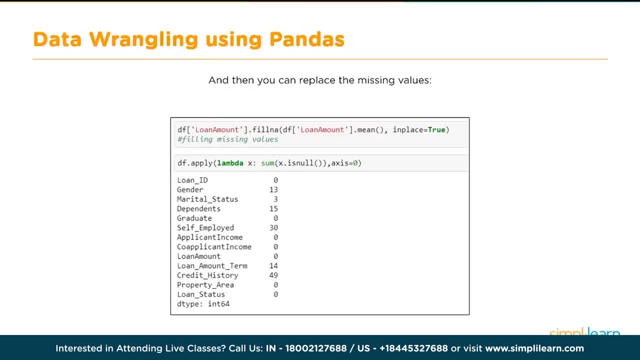 are very small compared to the total number of observations, then sometimes one of the easy ways is to completely remove that data or delete that record, exclude that record. So that is one way of doing it. So if there are, let's say, a million records, 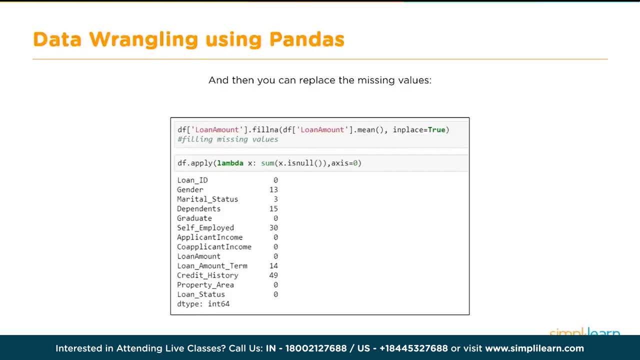 and maybe 10 records are having missing values, it may not be worth doing something to fill up those values. It may be better off to get rid of those observations. So that is, the missing values are proportionately very small. But if there are relatively large number of missing values, 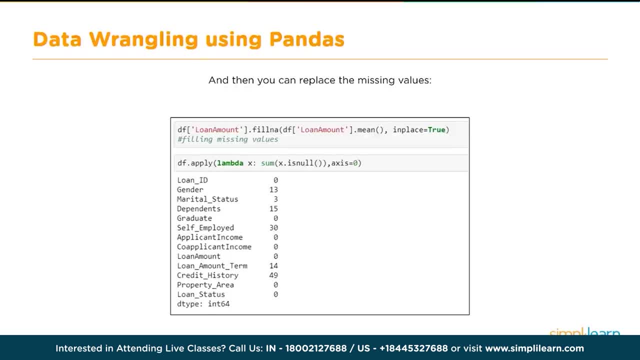 if you exclude those observations then your accuracy may not be that very good. So the other way of doing it is we can take a mean value for a particular column and fill up wherever there are missing values. fill up those observations or cells with the mean value. 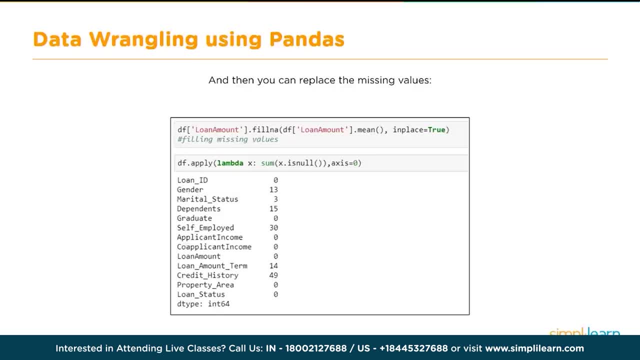 So that way, what happens is you don't give some value which is too high or too low and it somehow fits within the range of the observations that we are seeing. So this is one technique Again there are. it can be case to case and you may have to take a call based on 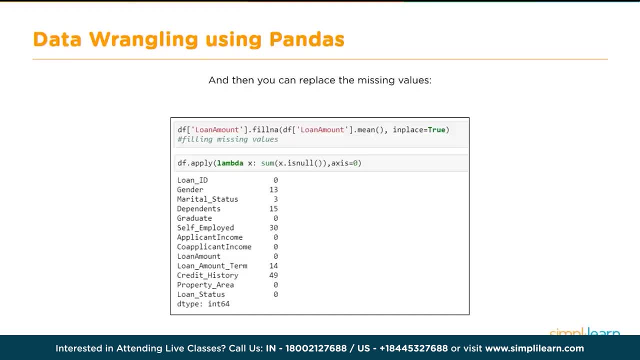 your specific situation, but these are some of the common methods. If you see, in the previous case loan amount had 21 and now we went ahead and filled all of those with the mean value. So now there are zero with missing values. So this is one part of a data wrangling. 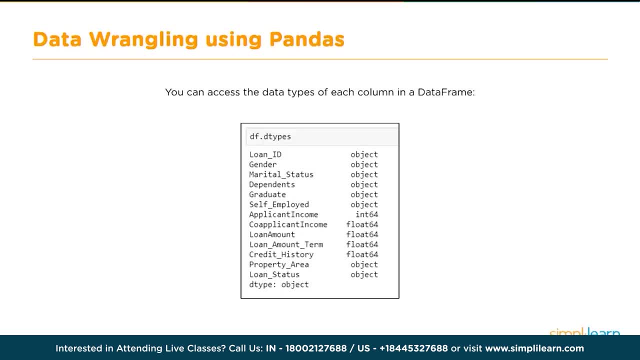 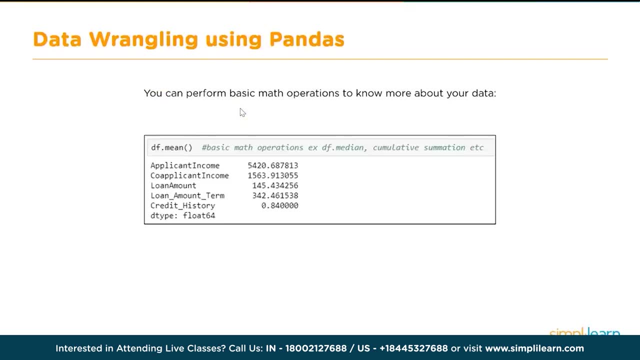 activity, What else you can do. you can also check what are the types of the data. So df, dot, d types will give us what are the various data types. So you can also perform some basic mathematical observations. We have already seen that mean we found out. So similarly, 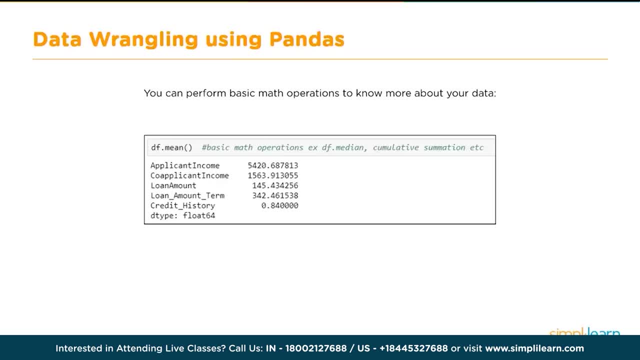 if you do call the mean method for the data frame object, it will actually perform or display or calculate the mean for pretty much all the numerical columns that are available in this. So for example here, applicant income, co-applicant income and all these are numerical values, So it will display the mean. 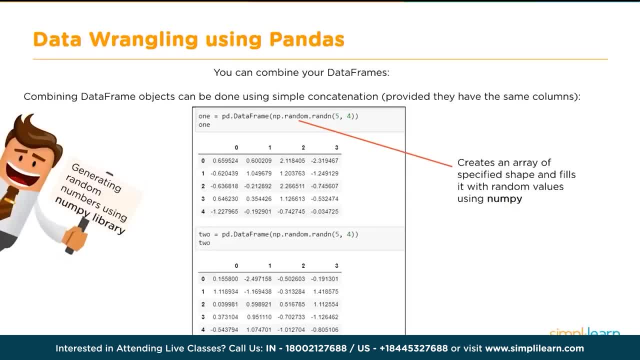 values of all of those. Now, another thing that you can do is you can actually also combine data frames. So let's say, you import data from one CSV file into one data frame and another CSV file into another data frame, and then you want to merge these because you want to do. 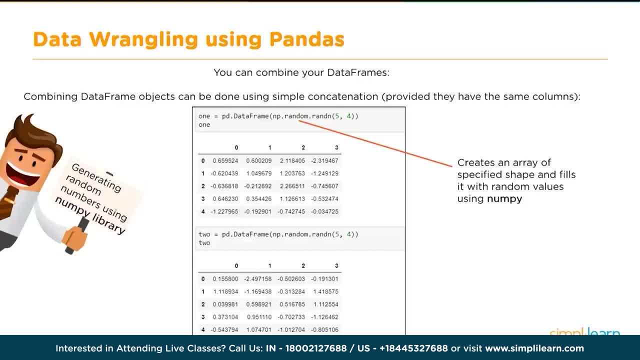 an analysis on the entire data. Okay, one example could be that you have data in the form of CSV files, one CSV file for each month of the year: January, February, March. each of these are in a different, So you can import them into, let's say, 12 data frames and 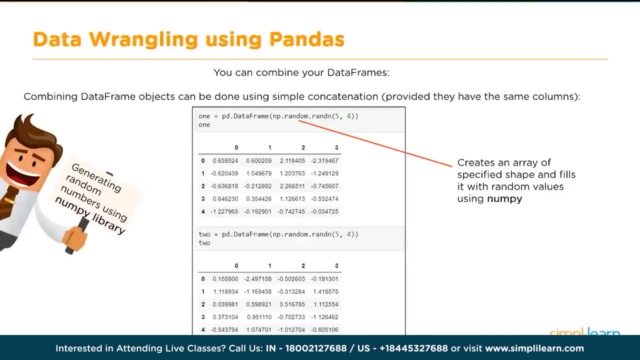 then you can merge them together as a single data frame and then you perform your analysis on the entire data frame or the entire data for the year. So that is one example. So how do we do that? This is how we do. Again, in this case, we are not importing. 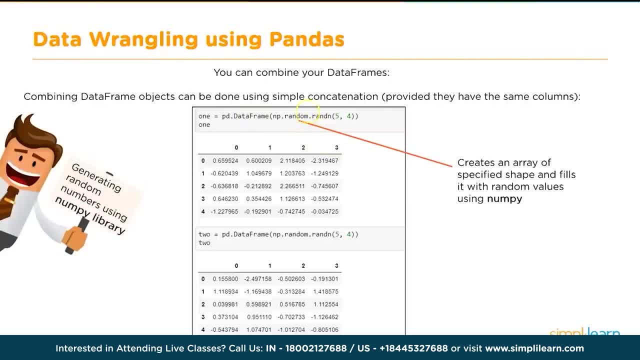 any data. We are just creating some random values or using some random values. So let's assume I have a data frame which is by the name 1 and I assign some random values here, which is a 5 by 4 format. So there are 5 rows and 4 columns. 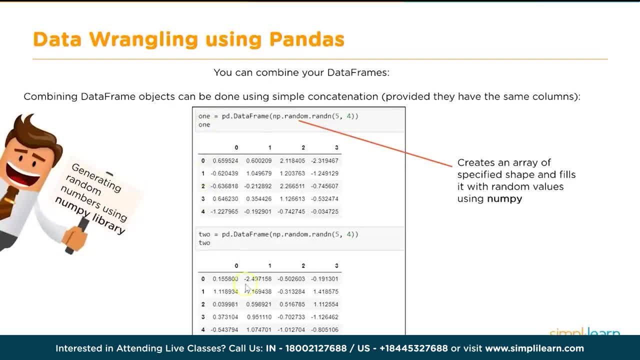 and this is how my data frame 1 looks. and then I create another data frame, which is data frame 2, again random numbers of the format 5 by 4, and I have something like this. Now I want to combine these two. How do I combine these two? 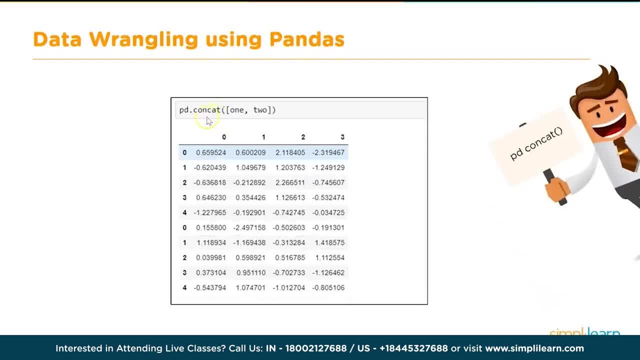 I can use the concatenate or concat method and I can combine these two. So pdconcat, and it takes the data frames 1 and 2. If you have more of them, you can provide them and it will just simply add all of them, merge all. 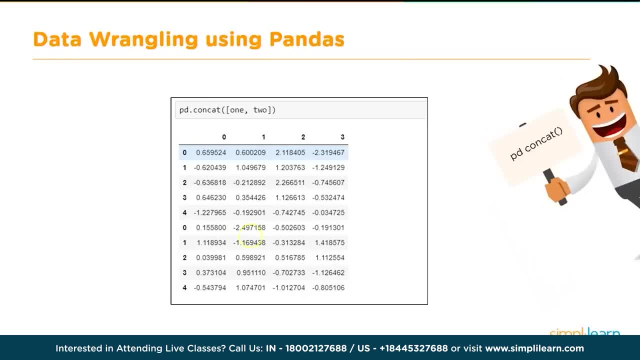 of them or concatenate whatever you call, whichever term you call. So of course, we have to make sure that the structure remains the same. Like I said, this could be, let's say, sales data coming for 12 different months, but each of the files has the same structure. so now you can. 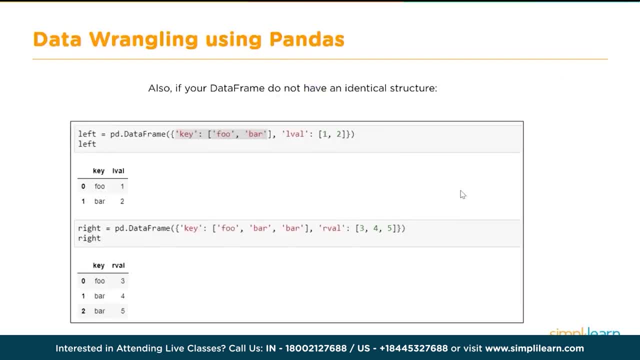 combine all of them, merge all of them using the concat method. If we have, let's say, structure is not identical, then what will happen? Let's say we have these two data frames: One has a column by the name key and the second column is lval. 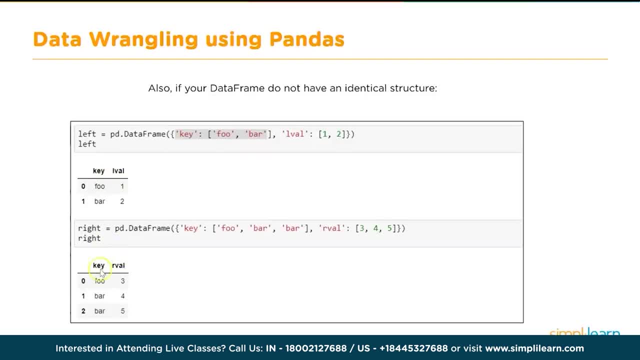 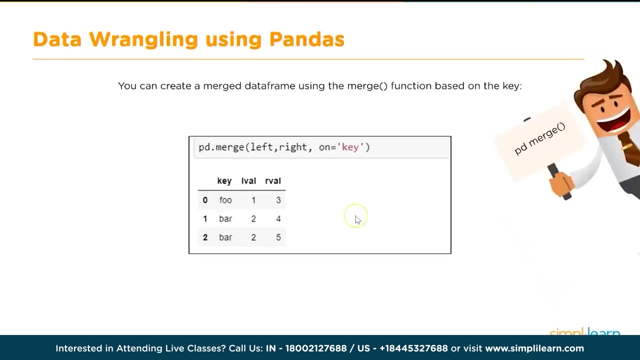 and a second data frame which has a column by the name key, but the second column by the name rval, not lval. So you see, here the structure is not identical. So you can still combine them, but then the way they get combined or merged is somewhat like. 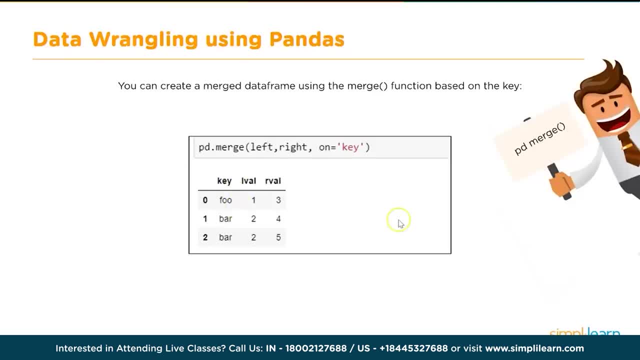 this, So it takes the key as a common parameter between them. Some common column has to be there, otherwise this will not work, and then we have to use merge instead of concatenate, and when we do a merge then we get the result will be in this format What it does. 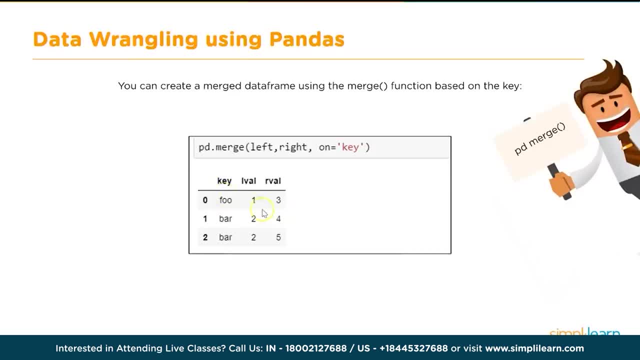 is, it uses the key as a common thread between them and then it kind of populates the values accordingly. So if you see here the first one had foo and bar for key and then it had l values of 1 and 2, right? So if we go back foo and bar, 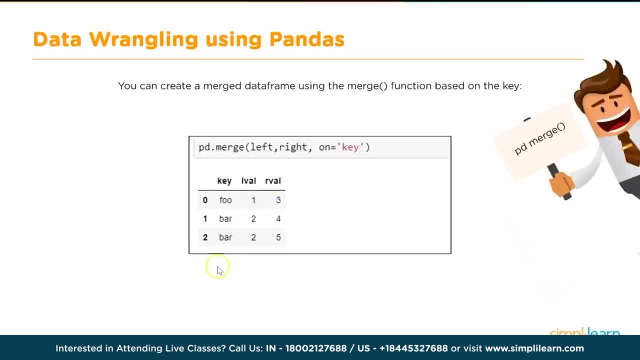 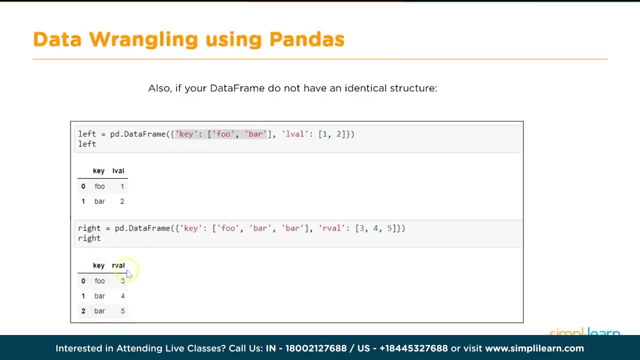 had 1 and 2 l values. So that's what we see here: 1 and 2.. Whereas in the right data frame we had foo, bar and bar as a second time, and then r values are 3, 4 and 5.. So what it has done for foo, it has put for the existing. 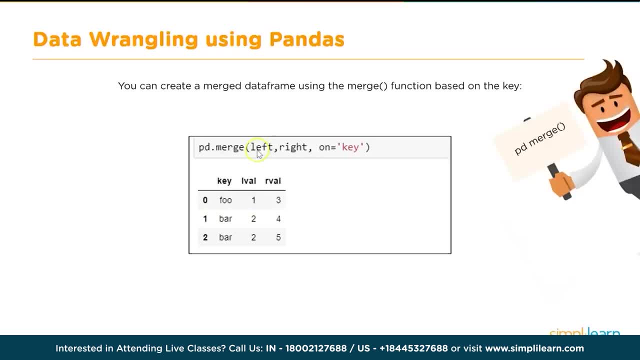 right For foo is already existing. right For foo is already existing because it has come from left. So it will just put the value of r? val here, which is 3.. Similarly, it will put 4 here, because for bar, if you go back for bar, it is the value. 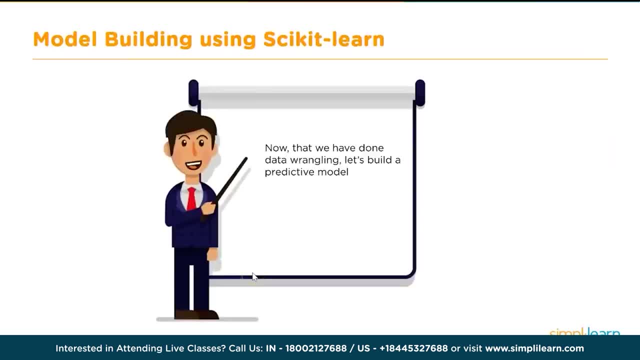 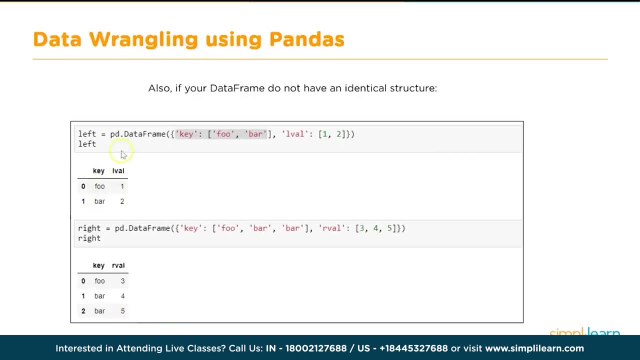 is 4, and since it has one more value of bar, it will go and add this 5 as well. The only thing here is that this one had, for example, left had only 2 values and only 1 value for bar, but since we are appending or 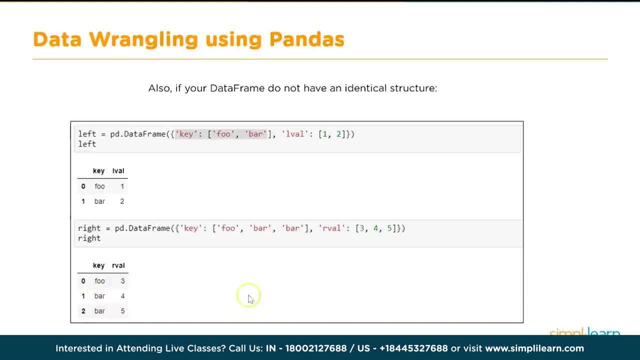 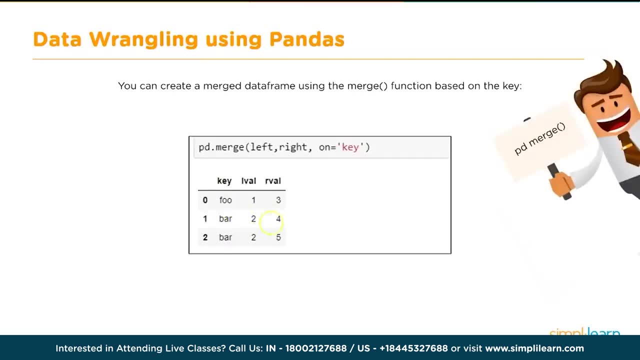 merging and there are 2 key values with bar. therefore it will kind of repeat the value of l val here. So that's what we are seeing in this case, right? So l value appears twice, the number 2 appears twice, but that is because r value there are. 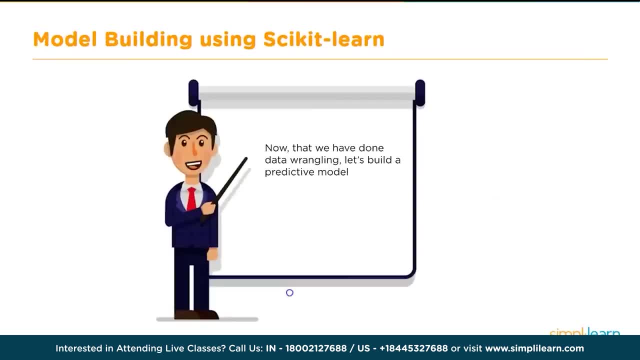 2 of them. Alright, so that is how, when you don't have identical structure, that is how you merge. Now we will talk a little bit about scikit learn. So scikit learn is a library which is used for doing machine learning or for performing machine. 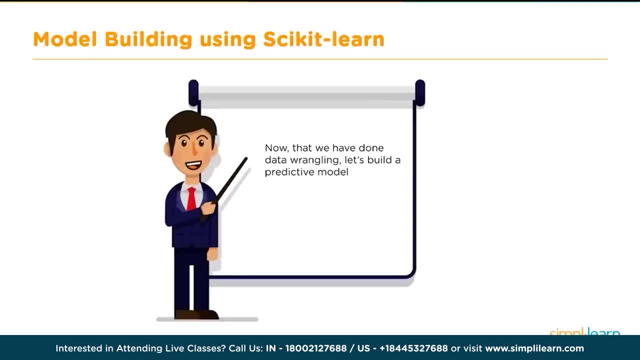 learning activities. So if you want to do linear regression, logistic regression and so on, there are easily usable APIs that you can call. and that's the advantage of scikit learn And it provides a bunch of algorithms. so I think that is the good part about this library. So if you want to use scikit learn, 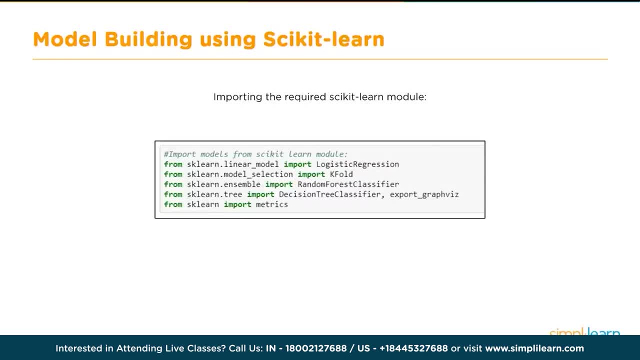 obviously you need to import these modules and also there are some sub modules you may have to import based on what you are trying to use. For example, we know we want to use logistic regression- Again, people who are probably not very familiar with machine learning. there is a separate module for machine learning. you may want to take a look at that. 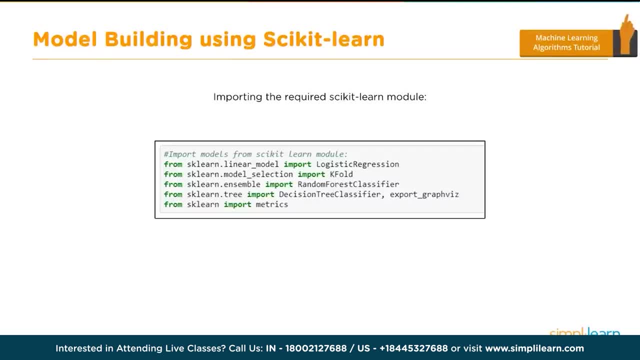 But we will just touch upon the basics here. So machine learning has some algorithms like linear regression, logistic regression and random forest classification and so on. So that is what we are talking about here. So those algorithms are available and if you want to use some, 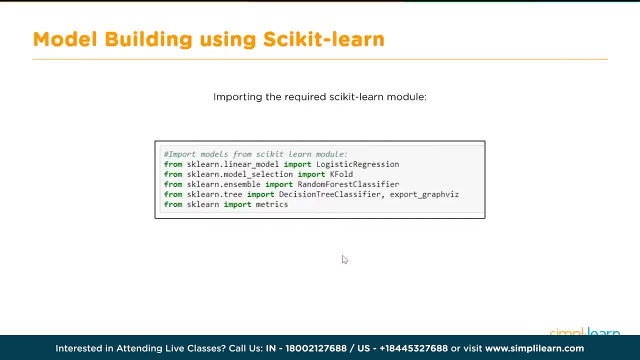 of them. you need to import them and from the scikit learn library. So scikit learn is the top level library, which is basically sklearn and then it has kind of sub parts in it. You need to import those based on what exactly you will be or which. 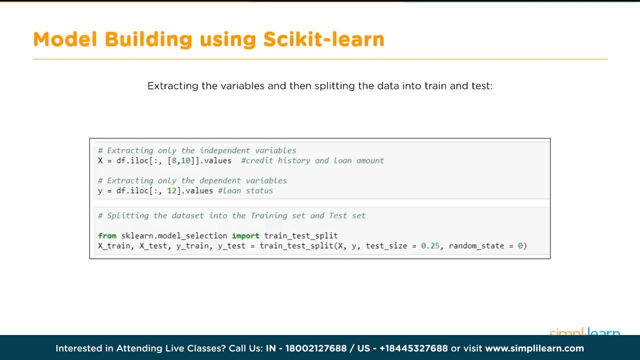 algorithm you will be using. So let's take an example. as we move- and we will see that Whenever we perform some machine learning activity- those of you who are familiar with machine learning will already know this- We split our labeled data into two parts: Training and test. Now there are multiple. 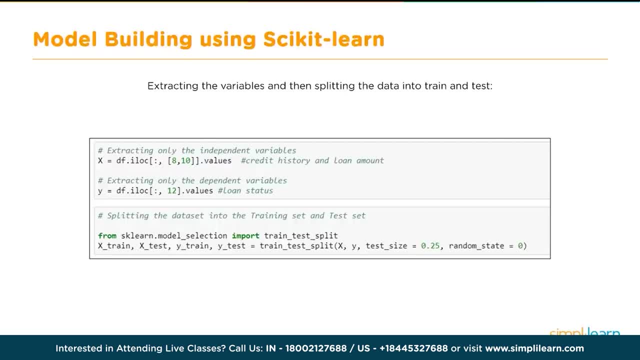 ways of splitting this data. How do we either? some people do it like 50-50,, some people do it 80-20, which is training is 80 and test is 20, and so on. So it is an individual preference. There are no hard and fast rules. By and large, we have seen that training. 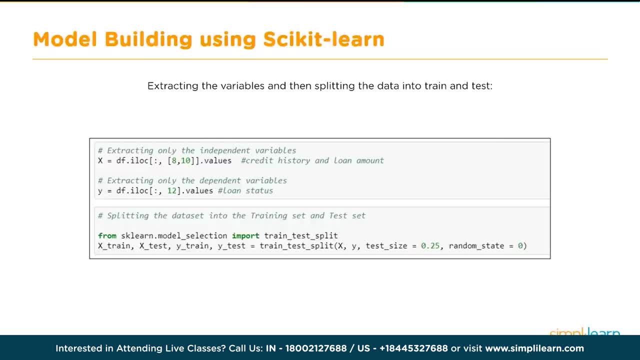 data set is larger than the test data set and again, we will probably not go into details of why do we do this At this point, but that's one of the steps in machine learning. So scikit learn offers a readily available method to do this, which is train test split. So in this example, 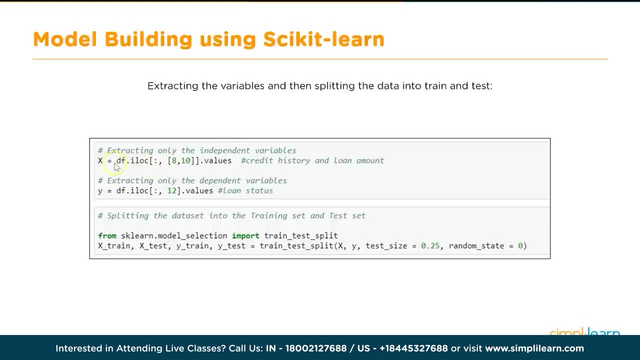 let's say we are taking the values x and y are our values, X is the independent variables and y is our dependent variable, And we are using these two, and then I want to split this into train and test data. So what do we do? We import the. 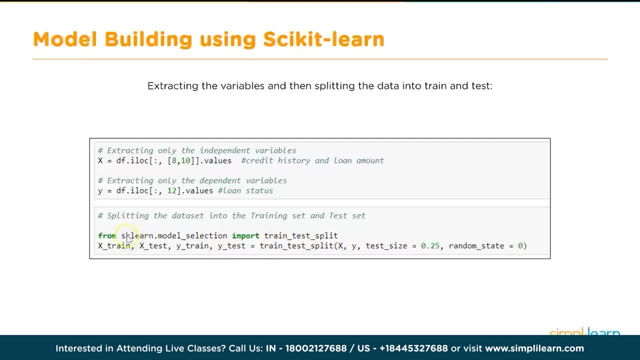 train test split submodule from within scikit learn, which is sklearn. So within that we import train test split and then you call this train test split method or function or whatever you call it, and pass the data. So x is the, all the values of the independent variables and y is our labels. 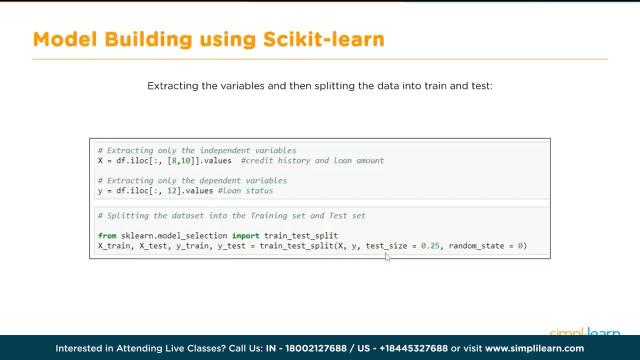 So you pass x and y and then you specify what should be your size of the test data. So only one you need to specify. So if you say test size is 0.25, it is understood that train size will be 0.75.. 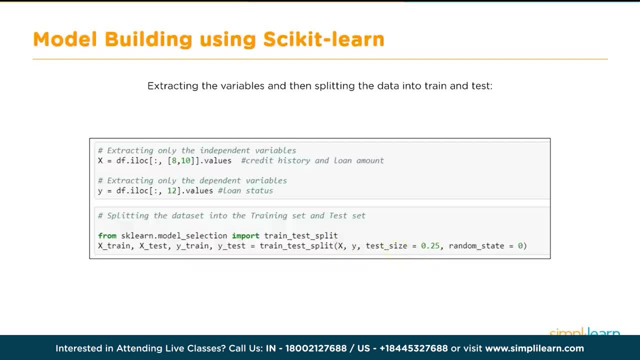 So you are telling what should be the ratio of the split. So technically nothing prevents you from giving whatever you like here. So you can give test as 80 and train as 20. so whichever way, but then the normal practices you will have, the training data set would be larger. 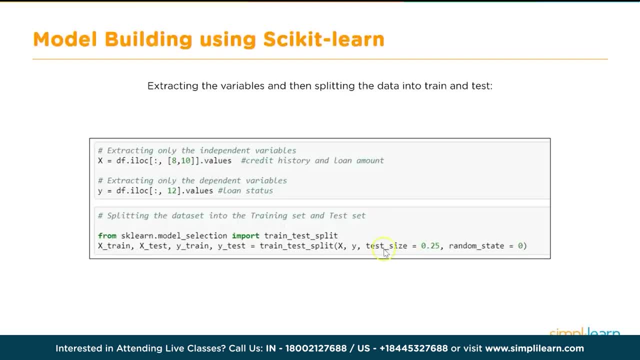 than the test data set, and typically it would be 80, 20, 75, 25 or 65, 35, something like that. So that is the second parameter, And this is just to say that you know the data has to be randomly split, So it shouldn't be like you take the first 75% and put it in. 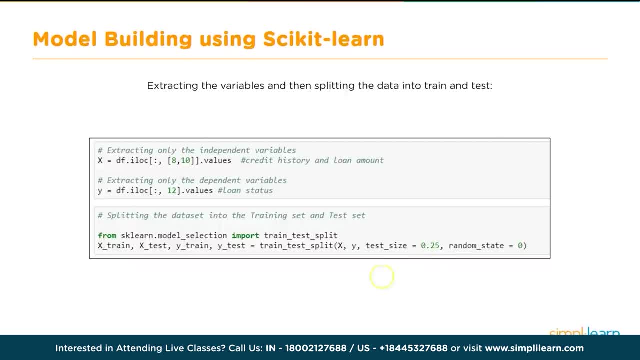 training and then the next 25% and put it in test so that. so such a thing shouldn't happen. So we first set the state random state, so that the the splitting is done in a very random way, So if they are randomly picked up, 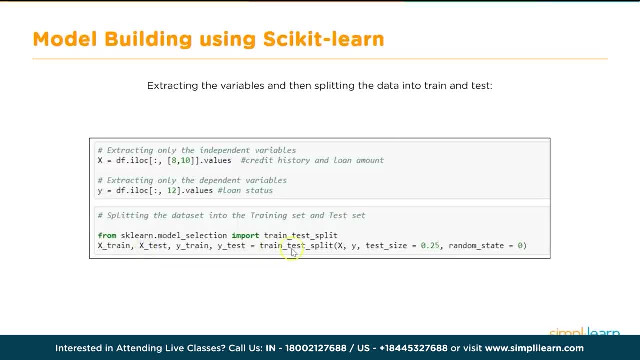 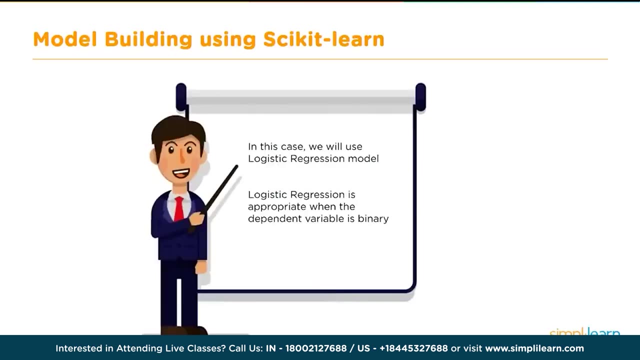 the data and then put it into training and test, and then this results in these four data frames, So x- train and x test and y- train and y test. So that is basically the result it will return. Now that the splitting is done, let's see how to implement or execute. 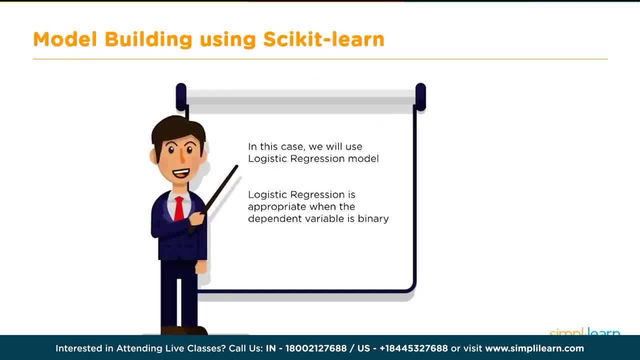 logistic regression. So in logistic regression, what we try to do is try to develop a model which will classify the data. Logistic regression is an algorithm for supervised learning, for performing classification. So logistic regression is for classification and usually it is binary classification. So binary classification. 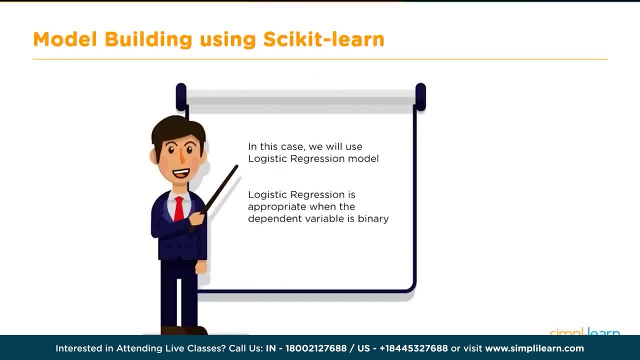 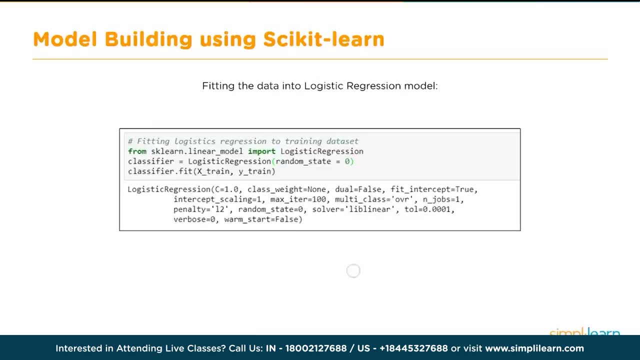 means there are two classes. So either like a yes, no or, for example, customer will buy or will not buy. So that is a binary classification. So that's where we use logistic regression. So let's take a look at the code: how to implement something like that using scikit-learn. So the first thing is to import. 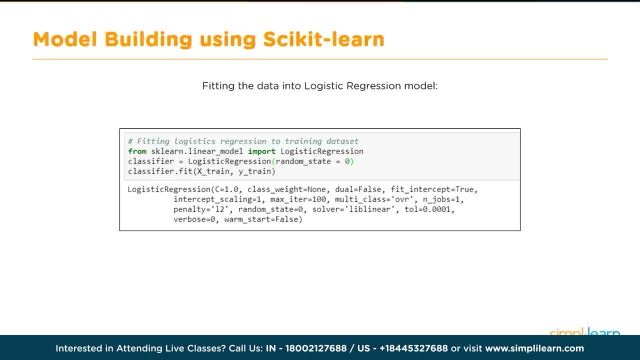 this logistic regression, submodule or subclass, whatever you call it, and then create an instance of that. So our object is classifier. So we are creating an object by the name. This is a name, by the way, You can give any name. In our case, we are saying classifier. We say classifier is equal to logistic. 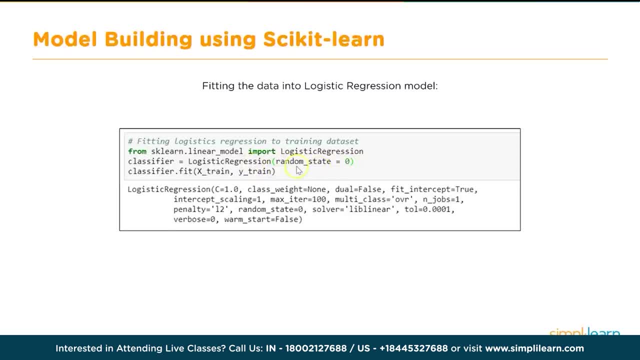 regression. So we are creating an instance of the logistic regression variable or class or whatever, And you can pass a variable or a parameter rather, which is the random state is equal to 0. And once you create the object, which in our case is named classifier, you can then train the object by calling. 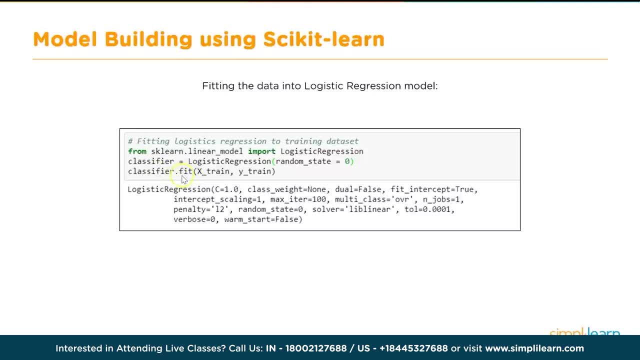 the method fit. So this is important to note- We don't call any. there is no method like train here, but we call what is known, as there is a method called fit. So you are basically, by calling the fit method, you are training this model And in order to 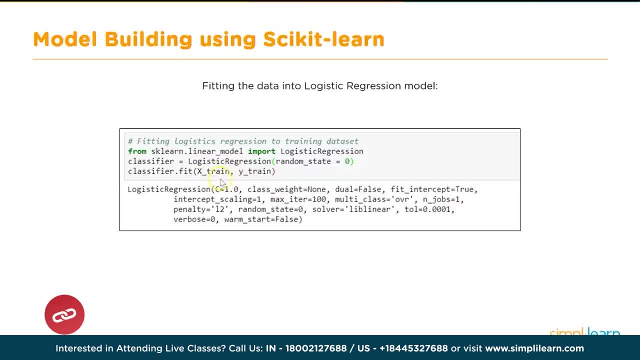 train the model, you need to pass the training data set. So x underscore train is your independent variables, The set of independent variables, and y underscore train is your dependent variable or the label. So you pass both of these and call the fit function or fit method. 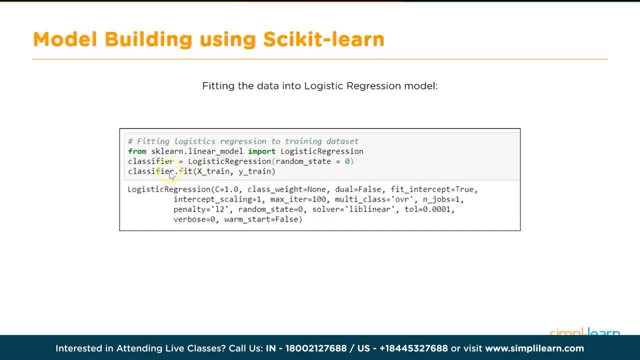 which will actually result in the training of this model classifier. Now this is basically showing what are the possible parameters that can be passed or initiated when we are calling the logistic or the instance of logistic regression. So this is, but you can also look up the help file if you have installed Python. So some 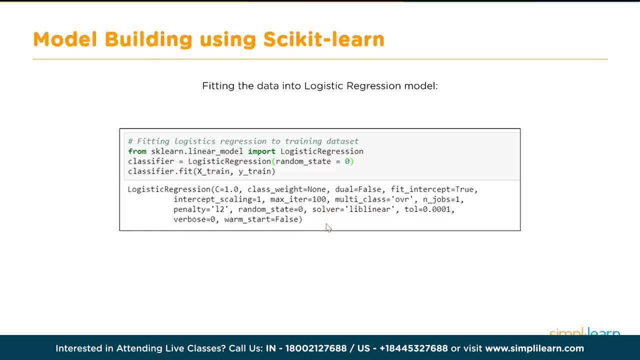 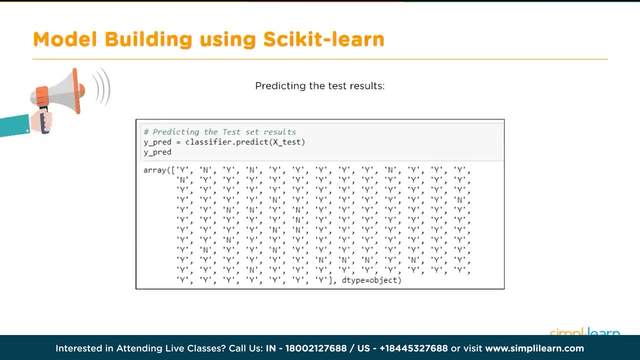 of these are very intuitive, but some you may want to take a look at the details of what exactly they do. Alright, so moving on. once we train the model by calling fit, then the next step is to test our model. So this is where we will use the test data You need. 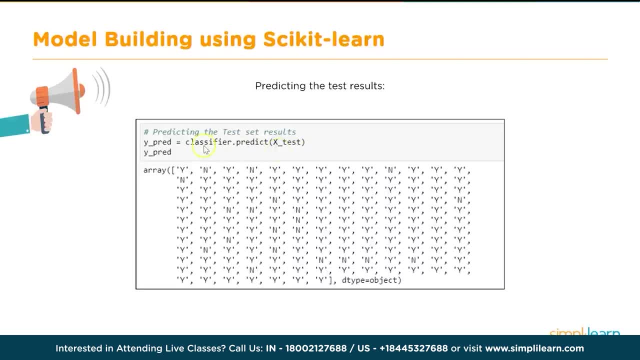 to pay attention here. Here I am calling. so there are two things. One is, in order to test our data, we have to actually call what is known as the method, known as predict. So here, this is where, so the training is done. Now is the time for inference, Isn't it? So we have the model. 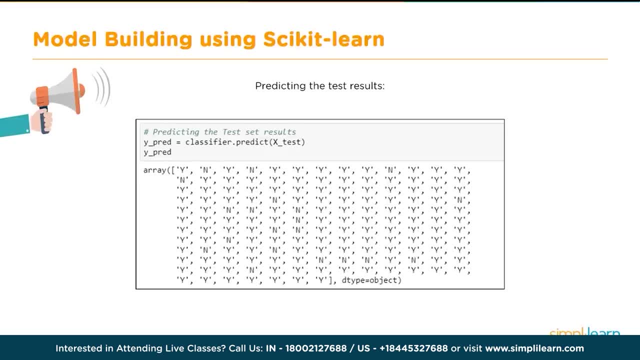 now we want to check whether our model is working or not. So what do you do? You have your test data, Remember? we split it. 25% of our data was stored here, Right? We split it into test and training, So that 25% of the data we pass. 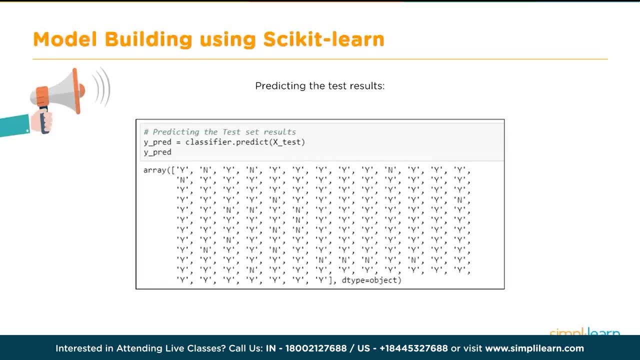 to and call the method predict, so that the model will now predict the values for y Right. So that's why here we are calling it as y underscore predict, And if we display here, as I said, this is the logistic regression, which is basically binary classification, So it gives us the results. 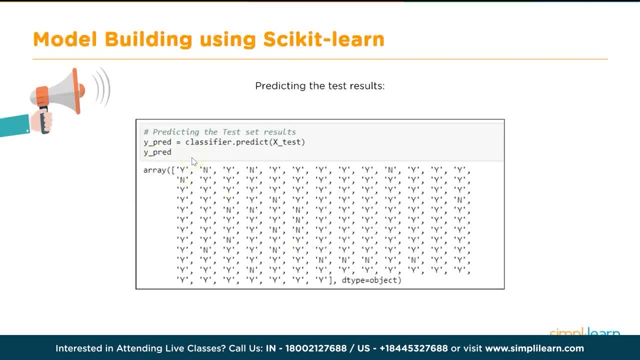 like yes or no in this particular case, And then you can. so this is what the model has predicted or model has classified Now. but we also know we already have the labels for this. So we need to compare with the existing labels, with the known labels, whether 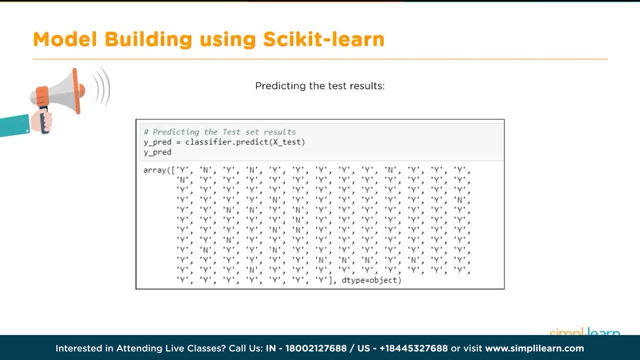 this classification is correct or not. So that is, where is the next step, which is basically calculating the accuracy and so on, will come into play. Okay, So in this case, the first thing, most important thing to note, is we do the prediction using predict, and here we are passing x underscore. 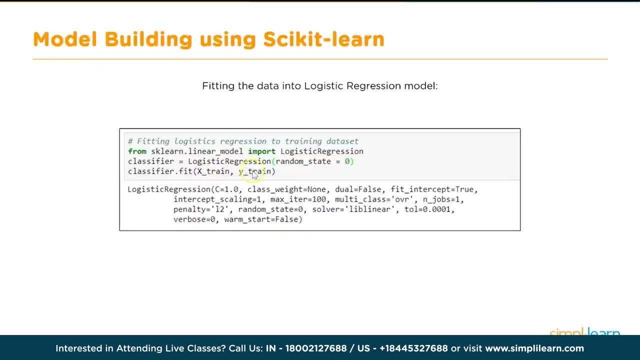 test and not train. Right, In this case we did x and y train. So again one more point to be noted here: In case of training, we will pass both the independent variables and also the dependent variables, because the system has to, internally, it has to verify. 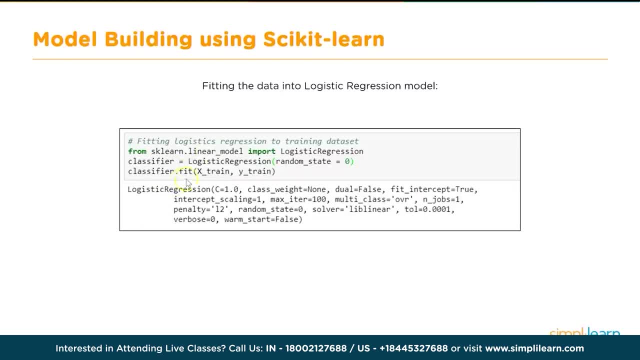 that is what is the training process. So what it will do. it will take the x values. It will try to come up with the y value and compare with the actual y value, Right? So that is what is the training method. So that's why. 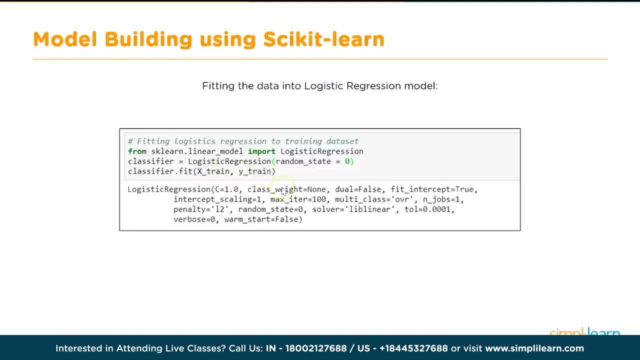 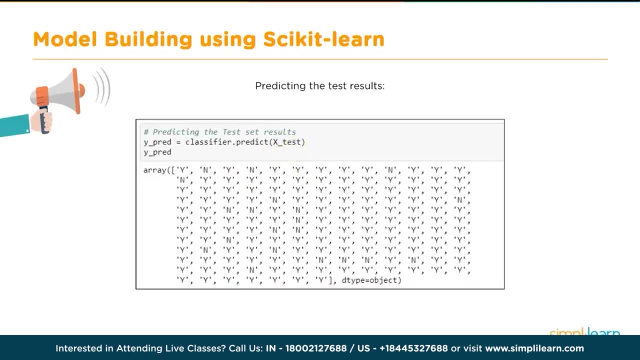 we have to pass both, x as well as y, Whereas in case of predict we don't pass both. We only pass because we are pretending as if this is the actual data. So in actual data you will not have the labels, Isn't it? So we are just passing the independent variables. 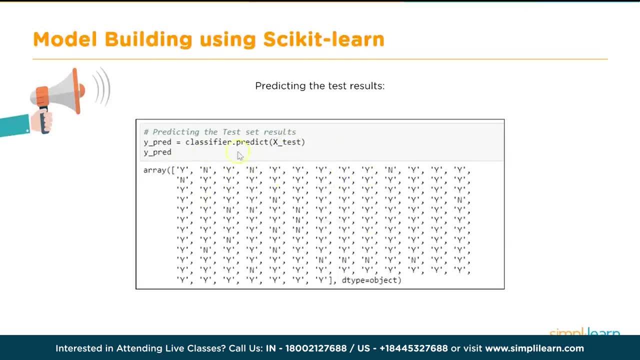 and the system will then come up with the y values, which we will then- okay, remember, we also know the actual value. So we will compare this with the actual values and we will find out whether, how accurate the model is. So how do we do that? 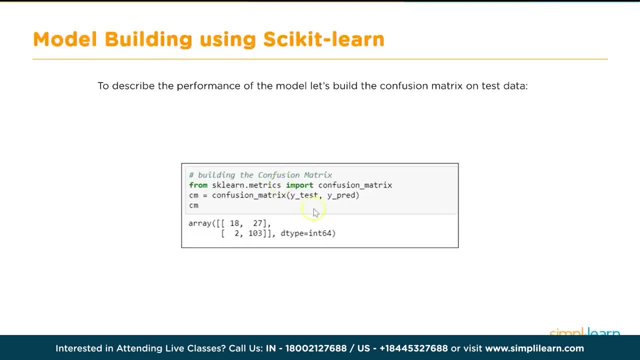 We use what is known as a confusion matrix. So this is also readily available in the python library. So we import this confusion matrix and some of you who already know machine learning will find this familiar. But those who are new to machine learning, this confusion matrix is nothing but this matrix, This kind of a matrix. 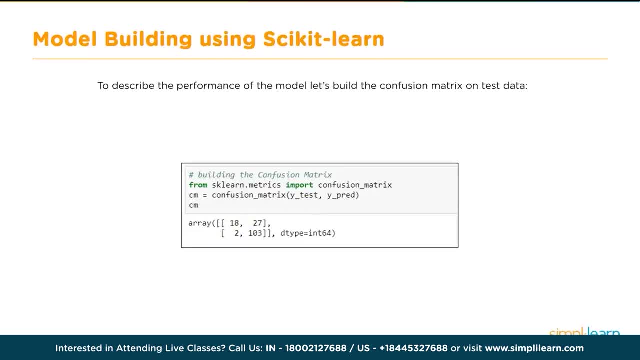 which basically tells how many of them are correctly predicted and how many of them are incorrectly predicted. So some of the characteristics. let's quickly spend some time on this confusion matrix itself. This the total numbers out here. These are just the numbers. These are like number of observations. 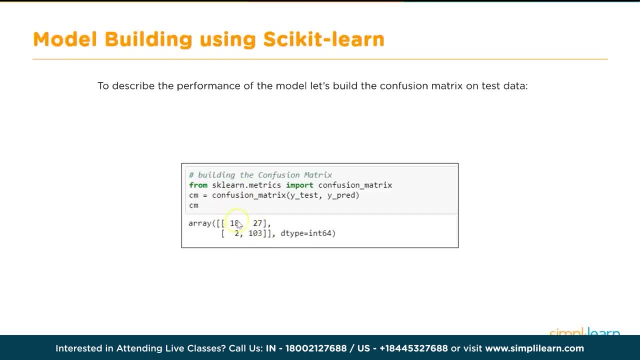 Then the accuracy is considered to be highest when the numbers, or the sum of the numbers across the diagonals is maximum, Okay, and the numbers outside of the diagonals should be minimum. So, which means that if this model was 100% accurate, then the sum of these two, There would have been only numbers in these two. 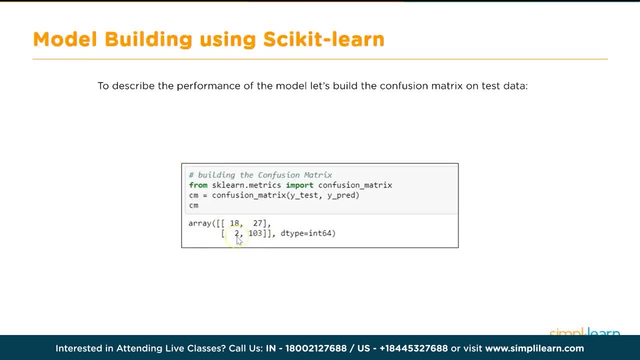 along the diagonal, This would have been 0 and this would have been 0. So that is like a 100% accurate model. That is very rare, but just that you are aware. So just to give an idea. So once you have, 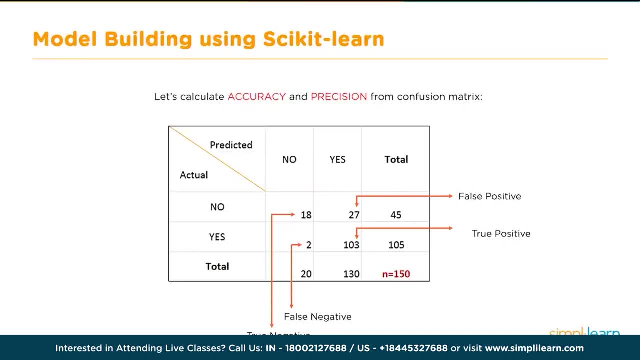 the confusion matrix. you then try to calculate the accuracy, which is in a percentage. So there are two things that we can do from a confusion matrix or that we can calculate from a confusion matrix. One is the accuracy and the other is the precision. What is the accuracy? Accuracy is basically. 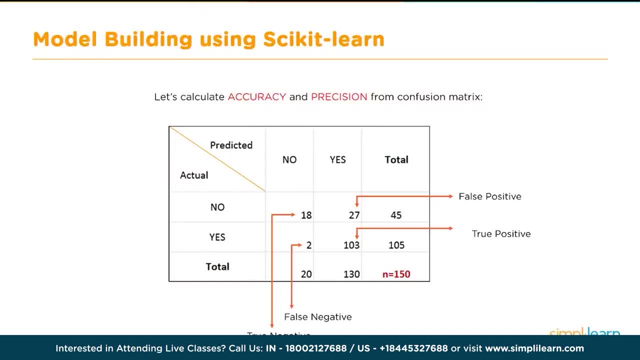 a measure of how many of the observations have been correctly predicted. So let us say this is a little bit more detailed view of the confusion matrix. It looks very similar like as we saw in this case. So this is a 2 by 2 matrix. That is what we are seeing here. 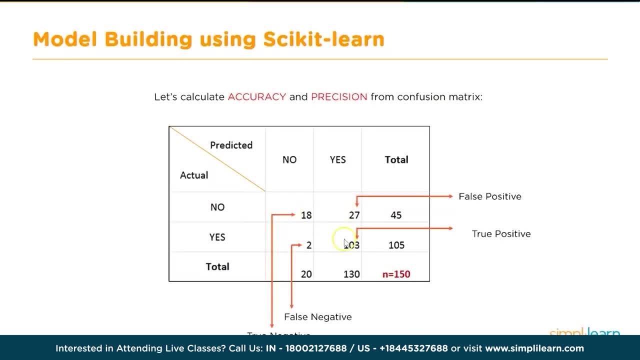 18, 27,, 2,, 1,, 0, 3.. So 18, 27,, 2,, 1,, 0, 3.. Now, but what are these values? That is what is kind of the labels are. 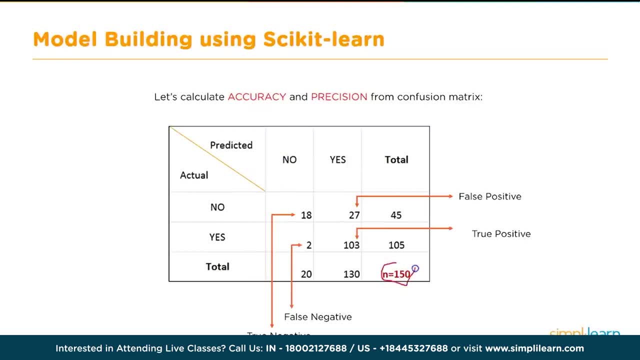 shown here in this. So there are altogether 150 observations. So, as I said, the sum of all these four, 18 plus 27 plus 1,, 0,, 3 plus 2- is equal to 150.. That is the first thing we have to observe. The sum of all these. 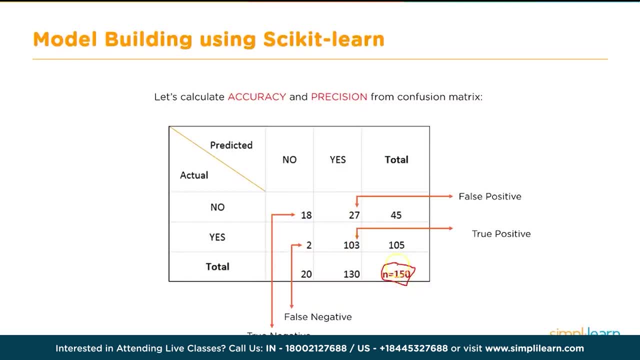 values will be equal to the sum of test observations. Number of test observations: We have 150 test observations Because remember we had about 500. We split that into 25, 75. So that is why we have 150 here and, I think, 350 in the training data set. 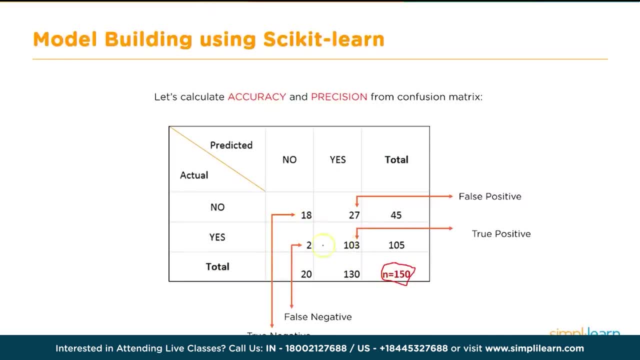 So that we get the numbers correct. So that is the first thing. Now the next thing is: let us take a look at the actual values. This view is the actual view, So there are actually right in the actual data. we have labels, yes and no. So, as per the 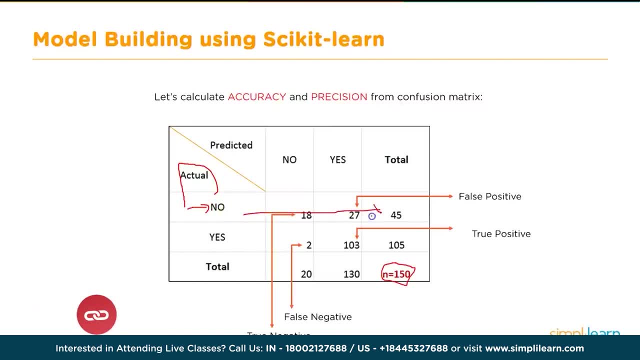 actual data: there are 45 observations tagged as no And similarly, there are 105 observations that are tagged as yes or labeled as yes. Now I know for the first time when you are seeing this. it may be a little confusing, but just stay with me. So this is the actual part of it. 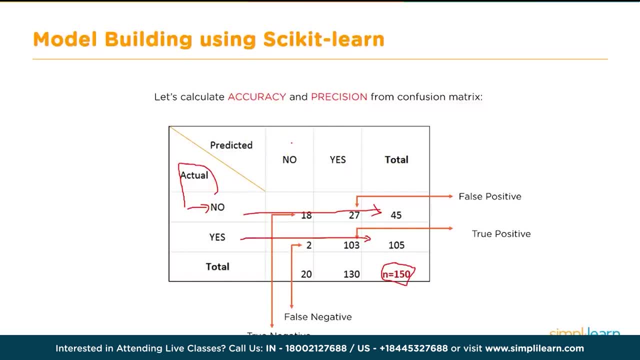 And this side tells us the predicted part of it. So our model has predicted- and it has totally predicted- 20 of them as no. So that is what this is: Totally 20 of them. it has predicted as no And it has predicted 130 of them as yes. 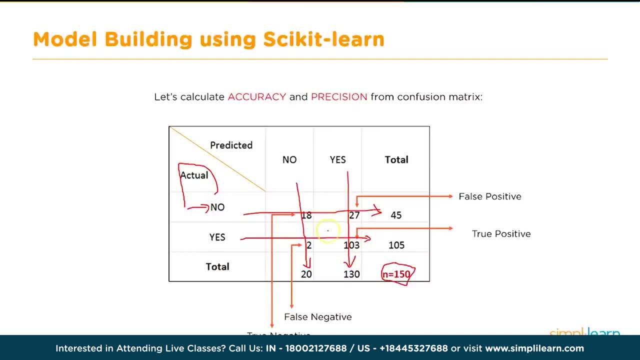 I hope this part is clear. So before we go into the middle part, let us first understand what exactly are these numbers So, actually tagged as no, there are 45 total. Actually tagged as yes, there are 105.. And predicted no, there are 20.. Predicted as: 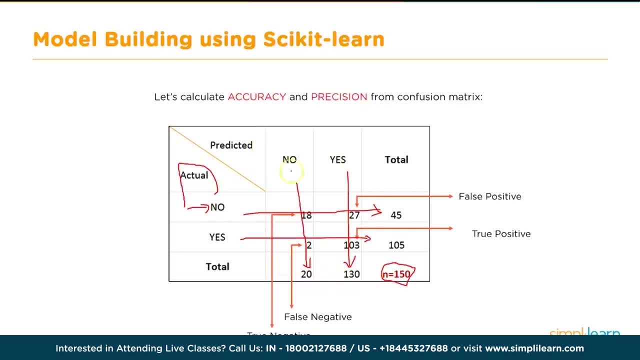 yes, there are 130.. This is the result from our model And this is the actual value, which we already know Because this is our labeled data. That is the first thing. Now let us take a look at each of these individually. Now, what are the options we have? 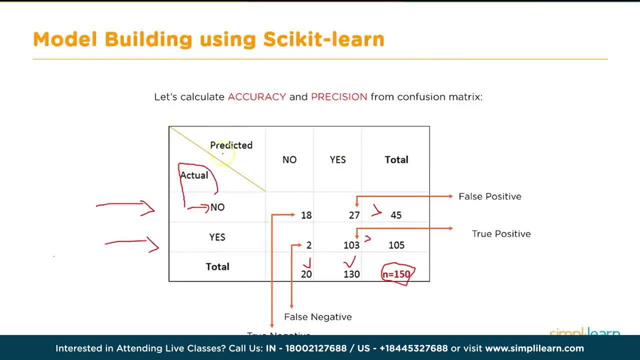 once again. So now, what is happening here? let us look at these values. This 18 says that these are actually tagged as no and the model is also predicted as no, which means this is what is known as a true positive right or true negative, sorry, right. 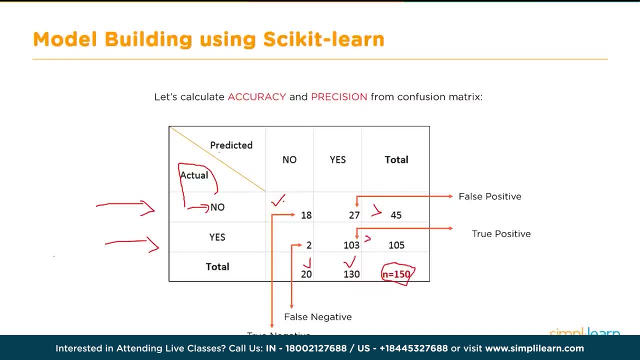 which means that our model, as predicted, is it correctly? it is negative because it says no, So, and it is also predicted no, so it is known as what is known as true, negative. okay, Now let's come to this side of it. that way, we are talking about the diagonal. 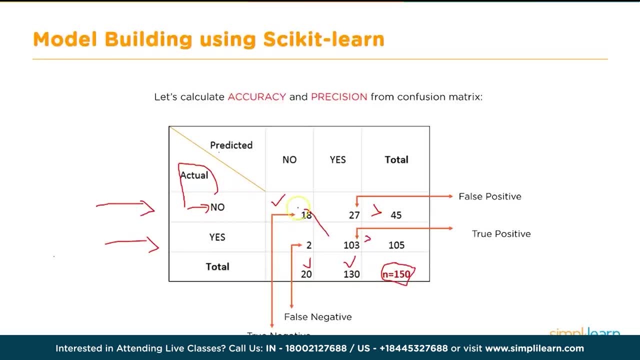 Remember I said most of the value should be in the diagonal. okay, So that means these 18 are correctly tagged. they are labeled as no and our model is predicted as no, So these are correctly tagged and these are known as true negative. okay. 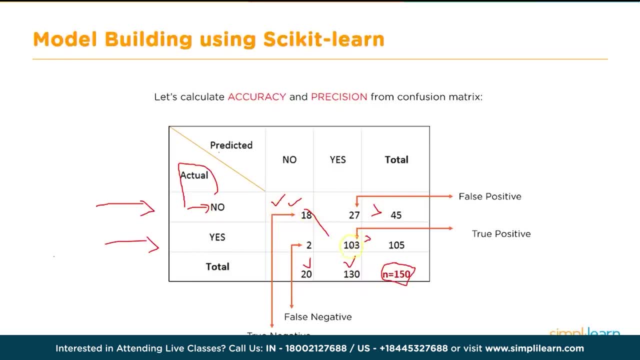 Similarly, if we come diagonally down, there are 103 observations which are labeled as yes, actual value is yes and our model is also predicted as yes, and these are known as true positive values. positive because of this: yes, okay, right. 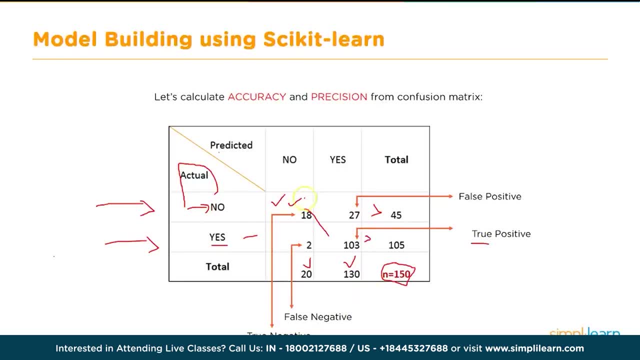 So what is important is- this is true, This is also true. So we have to make sure that the maximum number of values are in the true section. okay, True positive and true negative. That's the reason I said the sum along the diagonal should be maximum. 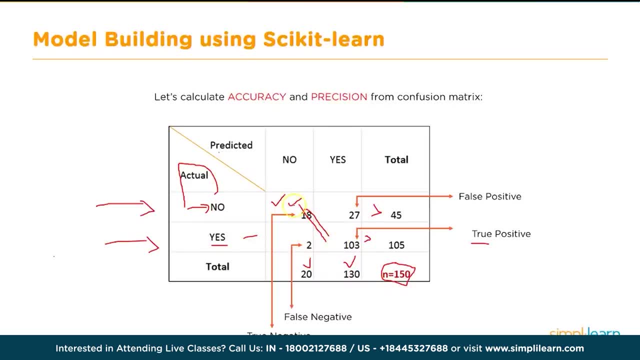 Now let's say our model was hundred percent accurate. this some. in this case it is only 103 plus 103 plus 18, which is 121, but if our model was accurate, the sum of these two would have been 150.. 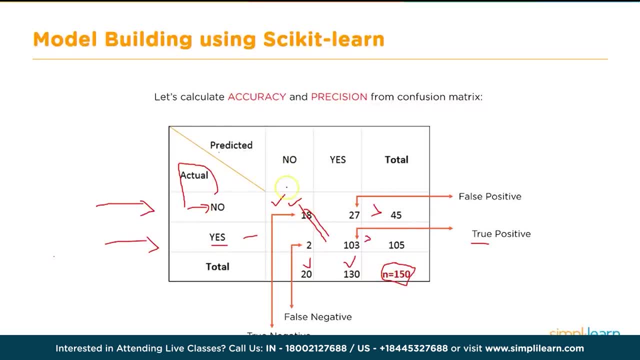 that means it's a perfect model. okay, all right. now what else? since we covered these two, let's also cover these two. so here, this says that 27 of them were actually labeled no, but our model has predicted as yes. that means this is wrong, right? similarly, these are two of them where 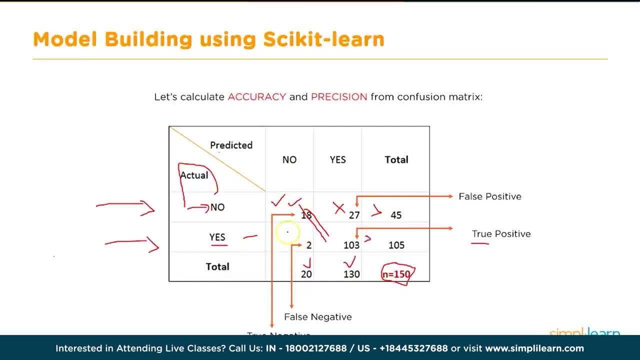 the actual value is yes, but our model has predicted as no, that means it's a wrong prediction. so you get the point. so, therefore, along the diagonals are the correct values, whereas in other places it is all wrong values or wrong predictions. okay, now how do we calculate accuracy? 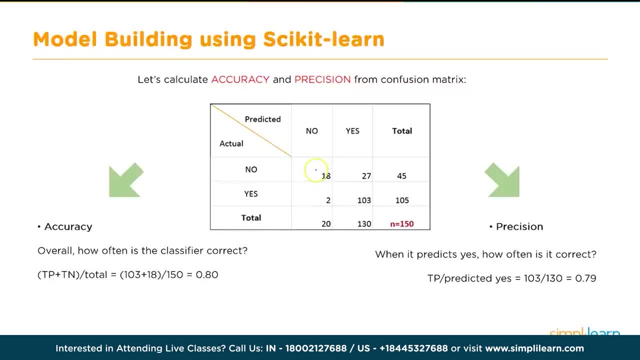 from this information. so the way to calculate accuracy is: so we'd say: okay, there are, total observations are 150, and what are the correctly predicted values? these are the correctly predicted values, which is 18 plus 103. so this will give us our accuracy. so 103 plus 18, which is 121. 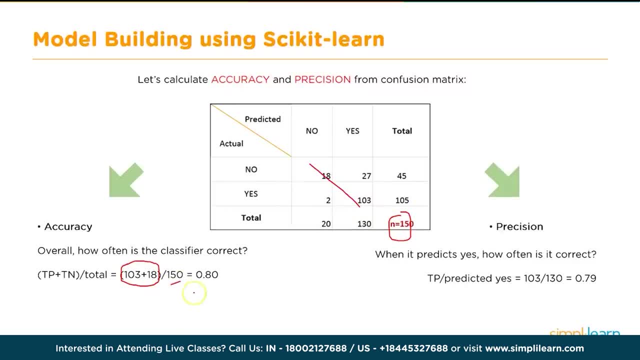 divided by our total observations, which is 150, is our accuracy, which is 0.8, or we can say it is 80 percent. okay, now there is another concept called precision. so precision is given by the formula true positives divided by the predicted positives, totally predicted positives, okay, what do we mean by that? which are the true positives here? 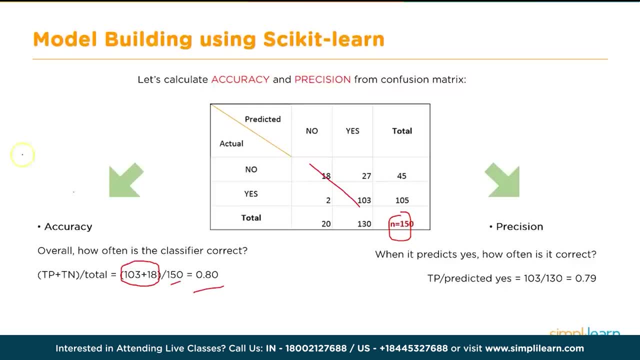 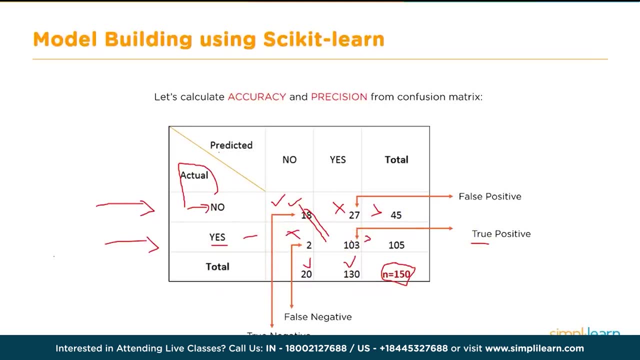 remember which are the true positives. we just recall, we just talked in the previous slide which are the true positives you see here. so this 103 are the true positives, which means that the value is positive, actual value is positive, predicted value is also positive. so that's. 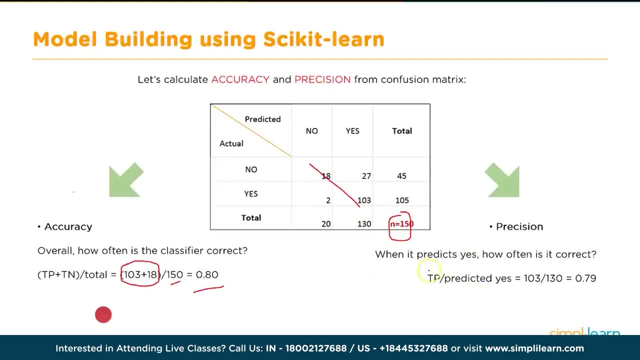 why it's called a true positive. so 103 divided by: so that is our true positive: 103 divided by totally predicted as yes. now, what is totally predicted as yes? remember, 130 of them have all together been predicted as yes. not that they are correctly predicted. only 103 have been correctly. 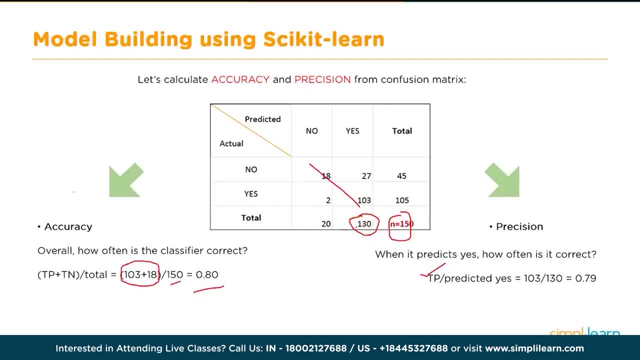 predicted, but 130 of them have been predicted as yes. so precision is basically the ratio of these two out of the totally predicted. how many of them are actually true? that ratio, so 103 by 130, which is again about 80 percent, is the precision. that's how you calculate precision. so this is just a simple. 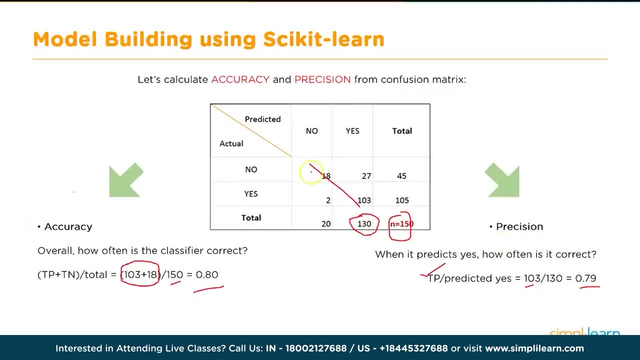 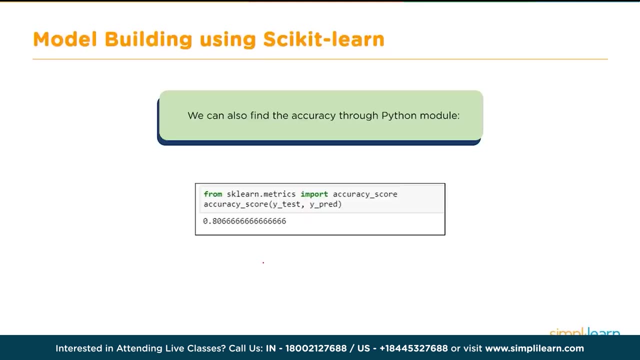 formula and the term that you need to remember. so accuracy is: you need to take total of true positive and true negative divided by the total number of observations, whereas precision is true positives divided by the totally predicted positives. okay, so that is our accuracy and precision. now, what we did, the accuracy calculation was manual, but we can also use some libraries. 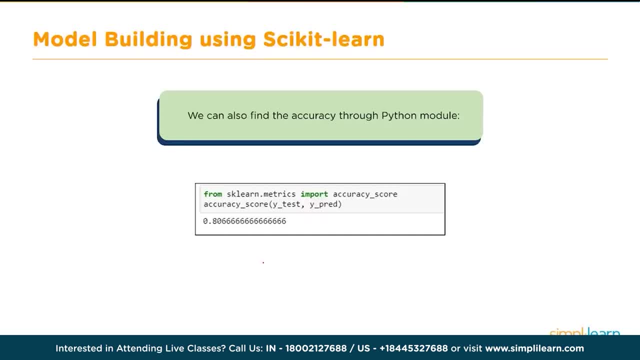 which are already existing and the functions within that library. So scikit-learn provides one such method. So, for example, accuracy underscore score is one such method. So if you use that and pass your test and predicted values, only the y you need to pass. 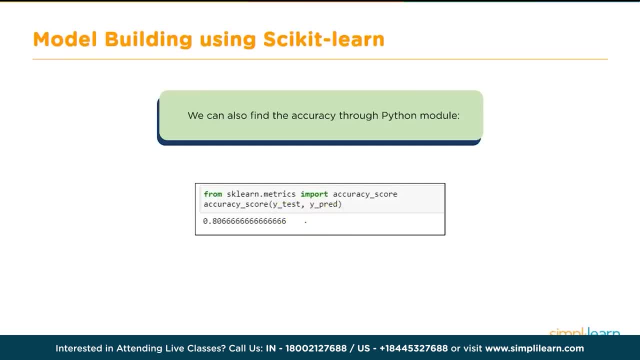 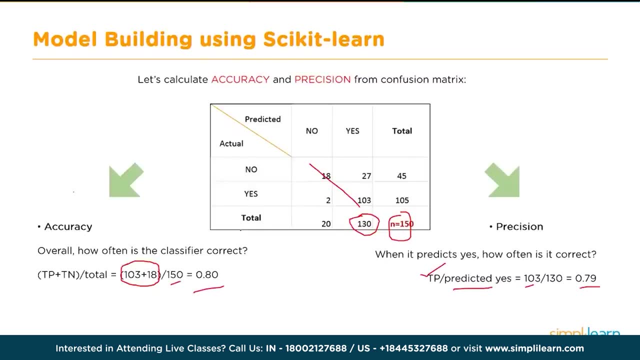 right, the dependent variable values. So if you pass that, it will calculate it for you. So in this case again, as you can see, it still calculates the same, which is 80%, which we have seen here as well. Okay, so this can be done using the method. 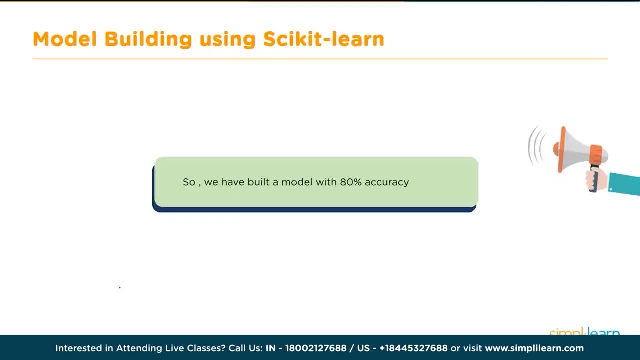 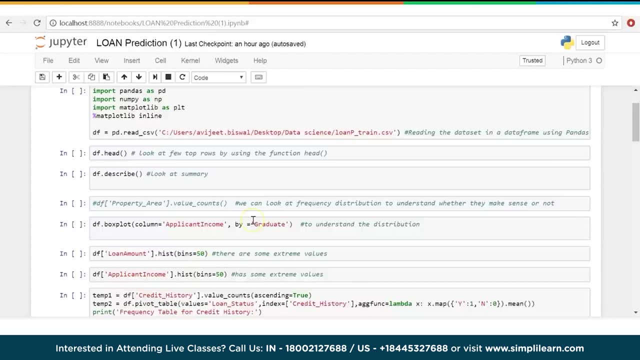 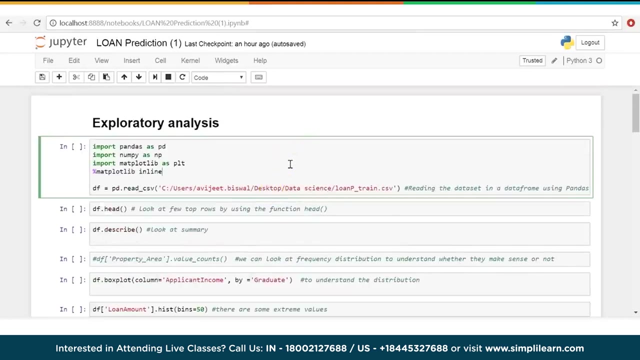 Great. So that's pretty much what we have done here. Before we conclude, let me take you into the code and show you how it actually looks. Okay, so this is our code. Let me run it. Okay, one by one. we have already seen most of the steps and slides. 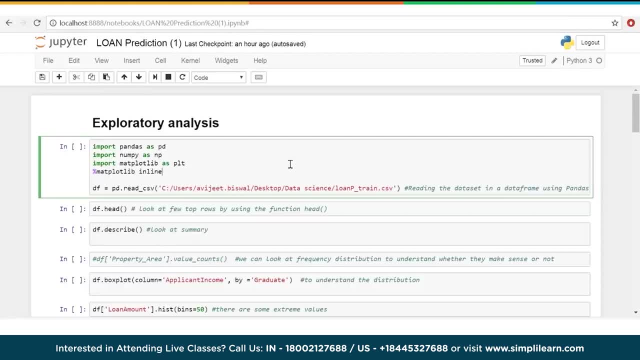 So I will, but I will run this in the action: Actual Jupyter Notebook. Some of you, if you're not yet familiar with Jupyter Notebook, again, there are other videos we created on how to install Jupyter Notebook and how to set up Jupyter Notebook and so 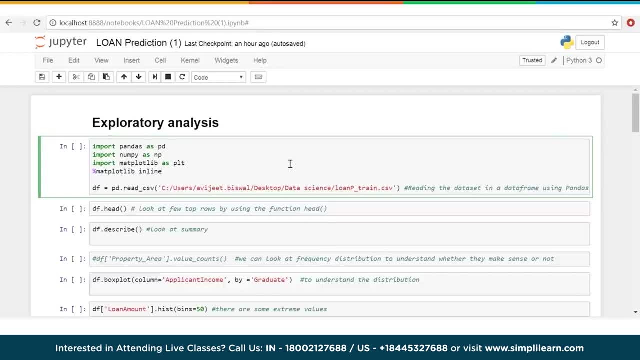 on In this tutorial also, we there was one slide on how to install Python and Jupyter Notebook. If you have not yet done, please do that, so that then you can actually walk through this code while you're watching this. Okay, so what are we doing here? we are importing the libraries required libraries, recall here. 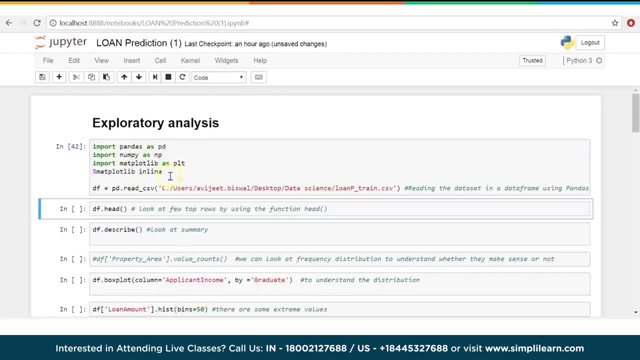 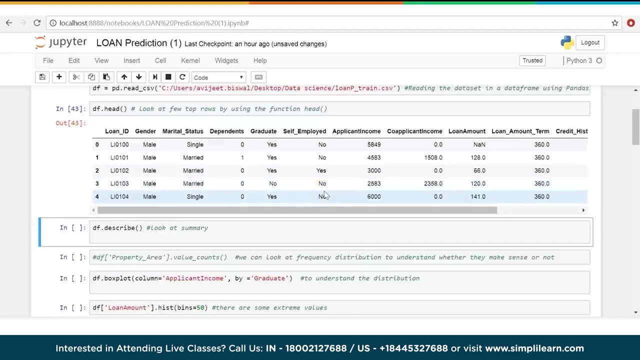 we have pandas, We have NumPy and for visualization we have matplotlib, And this line is basically reading the CSV file. So we have the CSV file locally on our local drive And this is where I'm checking the data, just so that I'm starting with my exploratory analysis. 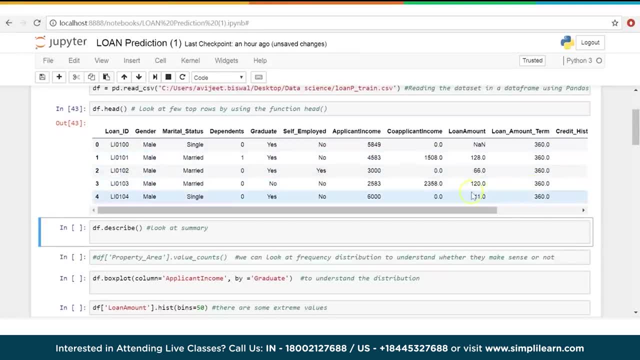 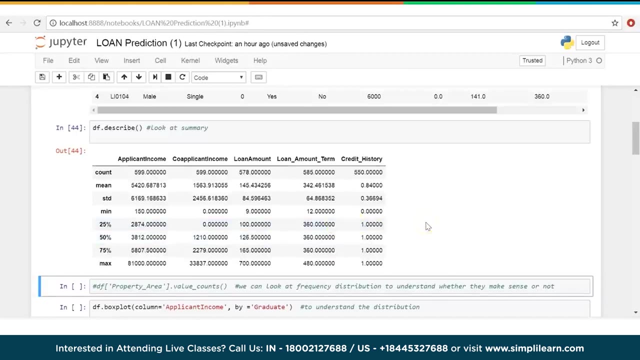 how the data is looking. So it looks good. There are no major missing values or anything like that. So it will display all the columns and it will show me the first five rows. if, when I'm using this Head function And then I want to see a kind of a summary of all the each of the numerical columns, 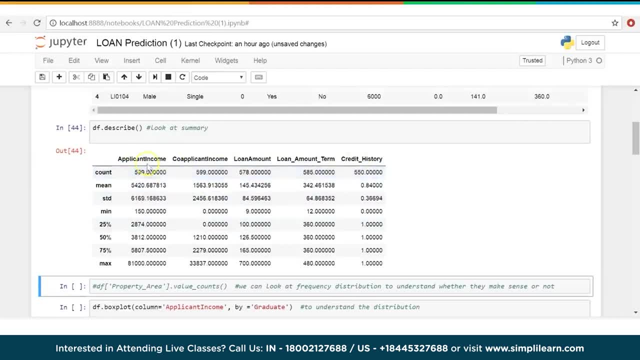 So that's what I'm doing here. So these are the numerical columns and it gives a summary like: how many observations are there, What is the mean- standard deviation, minimum, maximum, and so on and so forth for each of them, And then you can do some visualization. 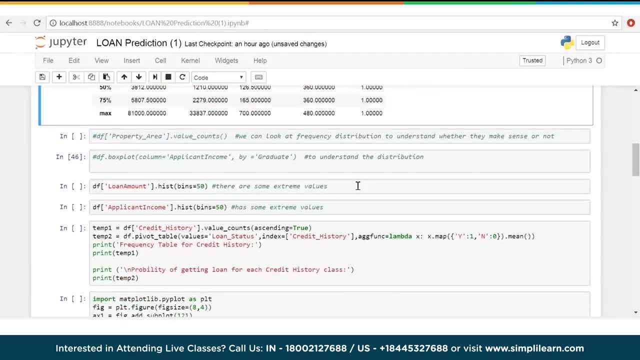 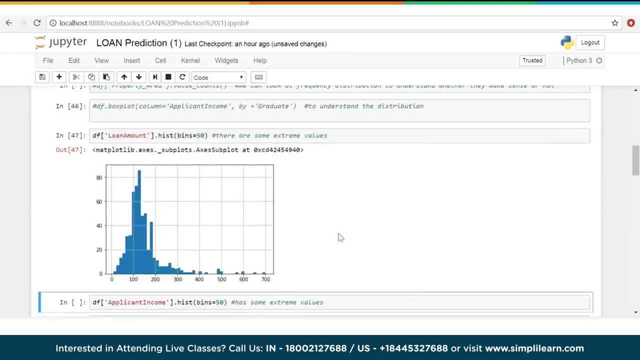 So this is the visualization for this. Okay, the next step is to view the data data visualization, And we will do that Using a histogram for a couple of these columns. So in this case, I'm taking a look at the loan amount. 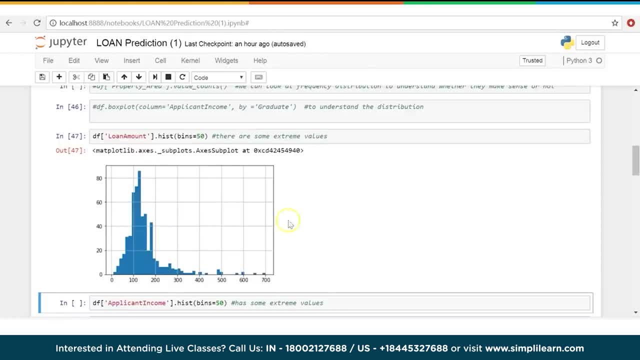 And if I create the histogram, it displays the data here in the form of a histogram, One thing that we gather from this, as I mentioned in the slides, as well as how the data is kind of scattered. So, while most of the values are in this range- zero to 300 range- there are a few extreme. 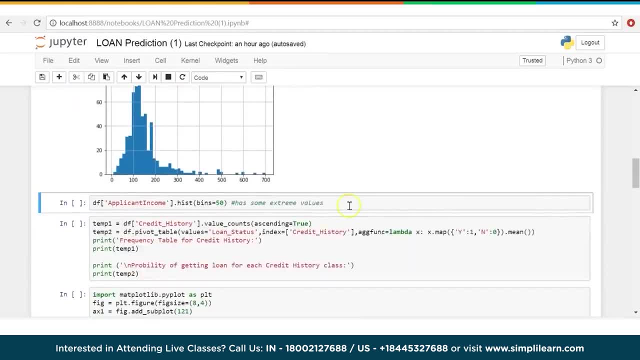 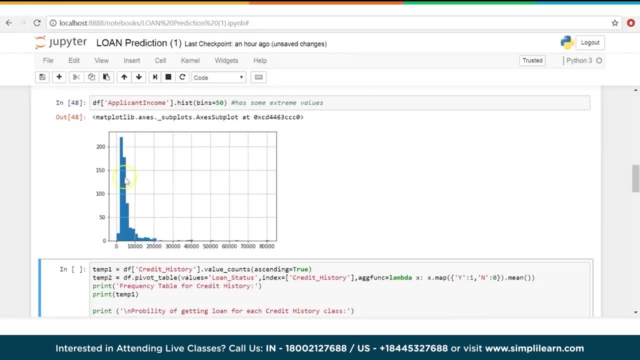 values around the 700 range. So that is one information we get from this histogram. Similarly So for the applicant income. if we draw a histogram, something similar, we can see that while most of the values are in this range, zero to 20,000 range, there are a few. 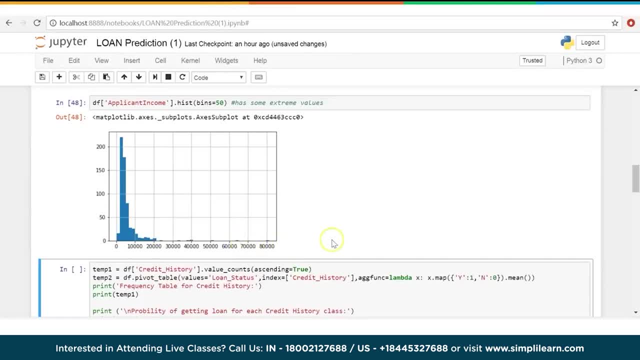 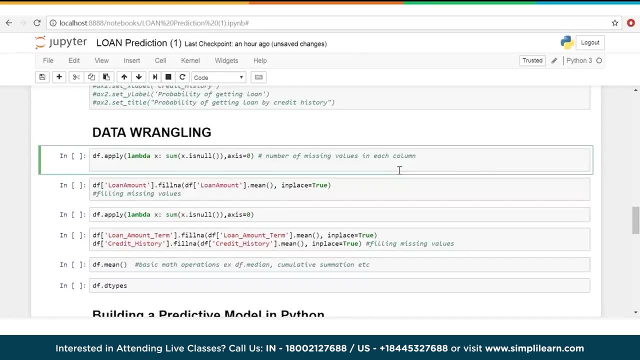 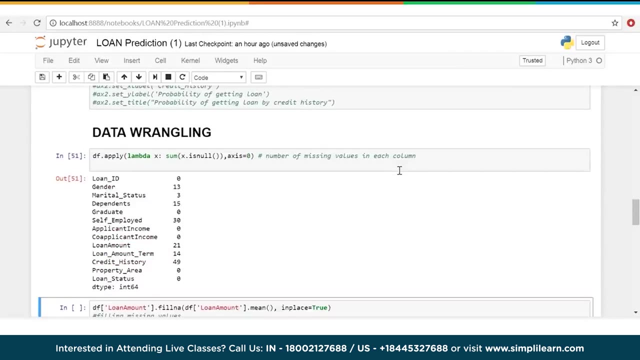 in the range of 80,000 and probably 65,000, and so on. Okay, so the next step is to perform data wrangling, where we will check if any data is missing and how to fill those missing values and so on. So in this case, we will just check for all the columns how many data or how many entries. 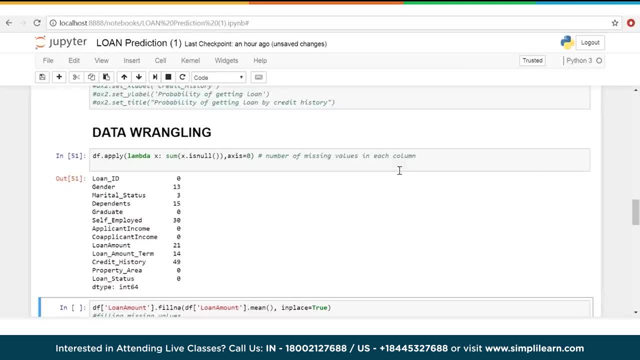 are there with missing values. So this is the result. The results: the loan ID has all the columns or all the cells filled. Gender has 13 missing values. Marital Status has three missing values, and so on and so forth. Loan amount has 21.. 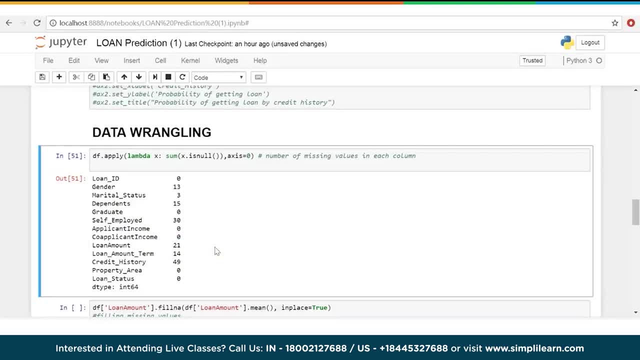 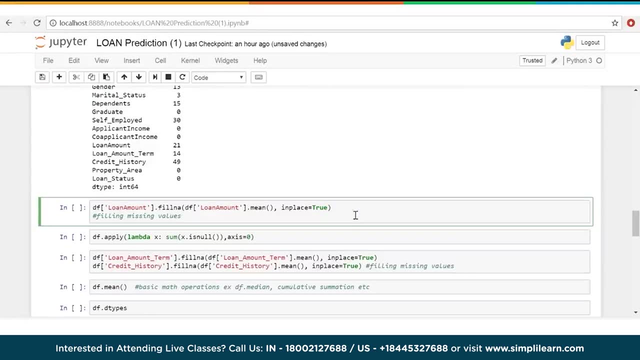 And this is what we are going to show you: how to remove these missing values. So when you have missing values, as I mentioned in the during the slides, there are a couple of ways of handling that. One is you can completely remove those or you fill in with some meaningful value. 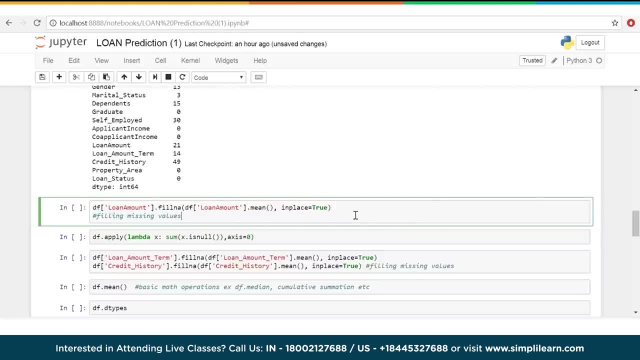 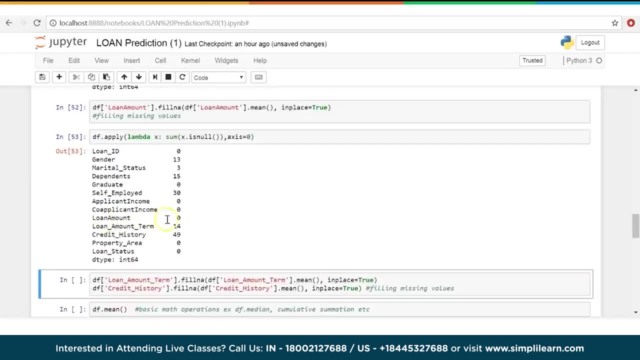 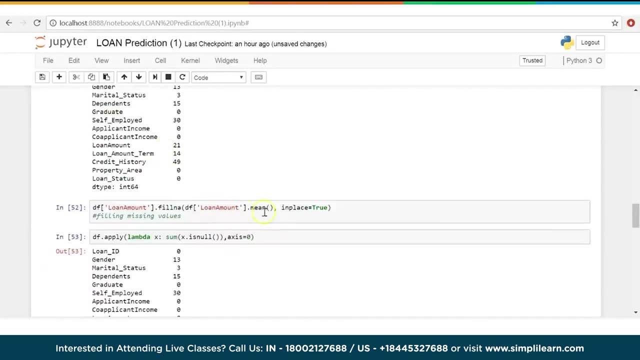 So in this case, we will fill the missing values with the mean value of the loan amount. So let's go ahead and do that. and now, if we check here now, loan amount number of missing values is zero, because what we did was, for all these 21 cells where the values were missing, we filled. 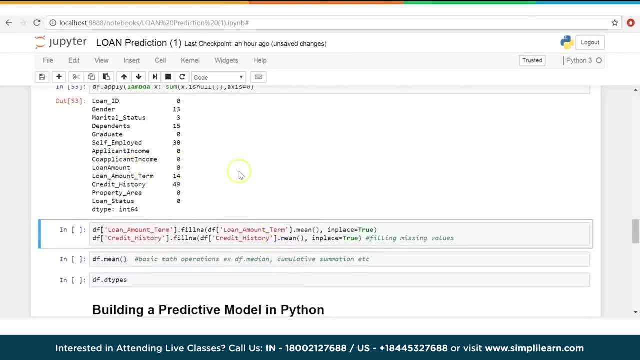 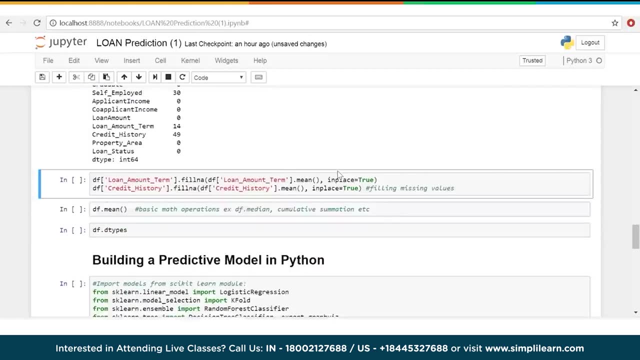 with the mean value of the loan amount. So now there are no more missing values for loan amount. We can do this for other columns as well, but this was just one example, so we have shown it here. Okay, so we will run this for credit history and loan amount term as well, and then, if we calculate, 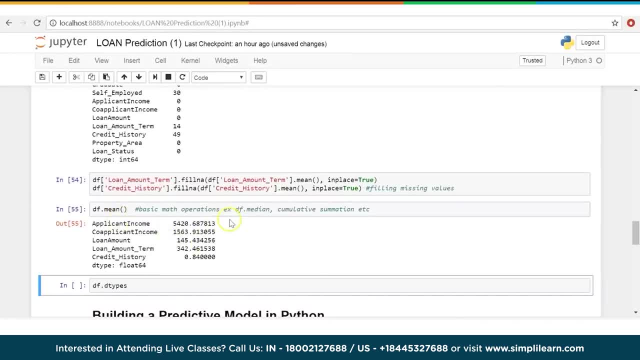 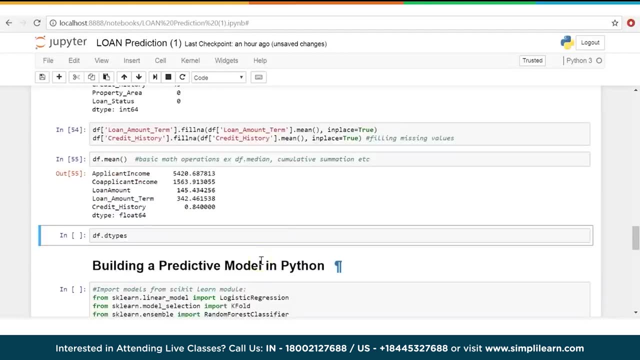 the mean of pretty much all the numerical columns. that's the method call So dfmean will give us the mean of all the numerical values. and another thing that we can do is we want to find out what are the data types of each of these columns. So you can call dfdtypes and get the data types. 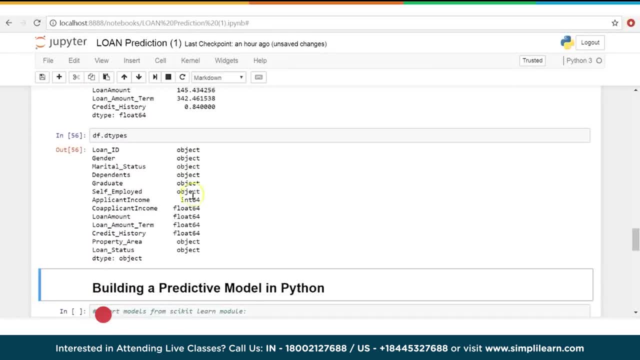 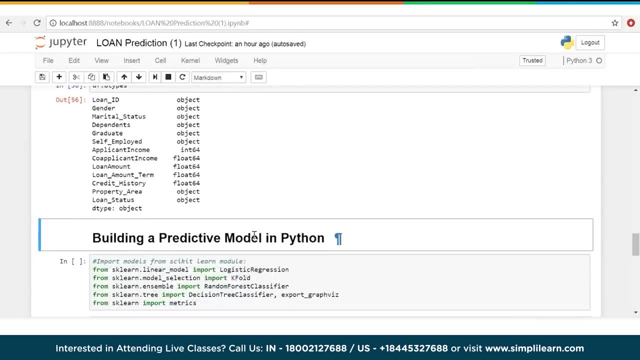 Of course it may not be that very useful. Most of the cases this is an object, but for example, this one: it shows as int 64 and there are float 64 and so on and so forth. Now, in addition to doing the exploratory data analysis, we can do some machine. 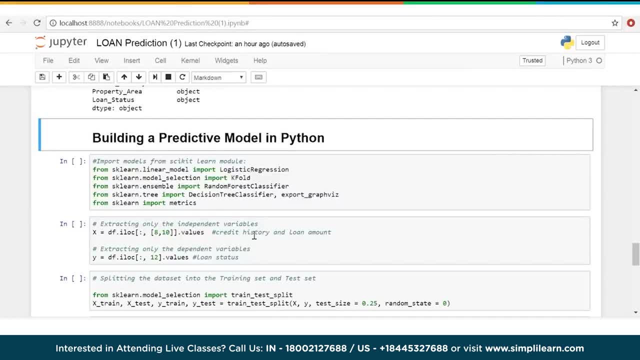 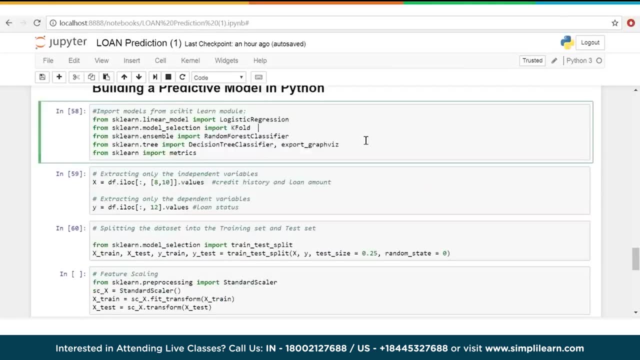 learning activity as well. So in this case we are going to do logistic regression. So this is the example that I have shown you in the slides as well. This is the actual code for that. All right, so the first step here is to import the libraries, and then the next step is to separate the 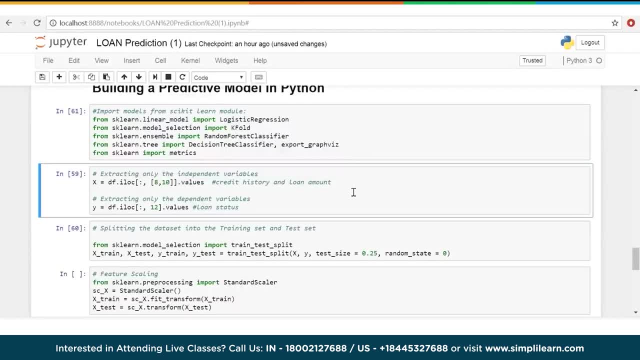 independent libraries. So the first step is to import the libraries and then the next step is to import the independent variables and the dependent variables. So x is our independent variable and y is our dependent variable. So we separate the data into two parts and this will be our target as well. 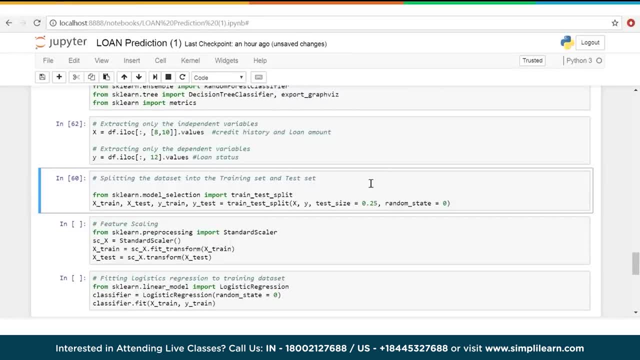 right, So that's how we separate it. Now we have to split the data into training and test data sets. As I mentioned in the during the slides, we use the train test split method and when we call this and pass the independent variables and the dependent variables, 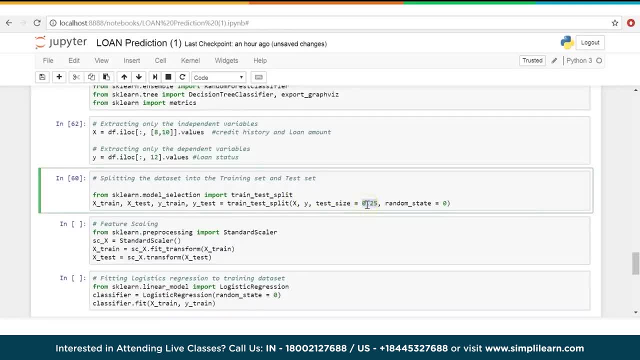 And we specify the test size to be 0.25, which means the training size will be 0.75, which is nothing. but you split the data into training data set, which is 75 percent, and test data set, in which is 25 percent. Okay, So once you split that, you will have all your independent variables data in. 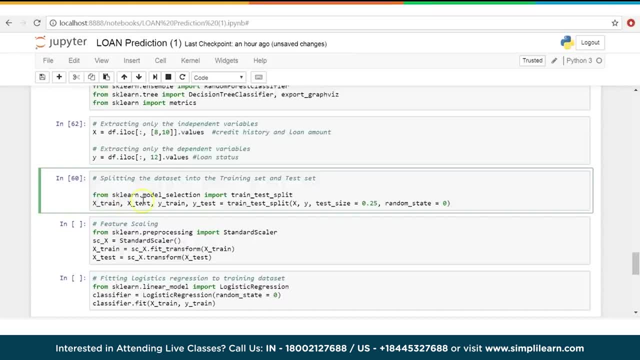 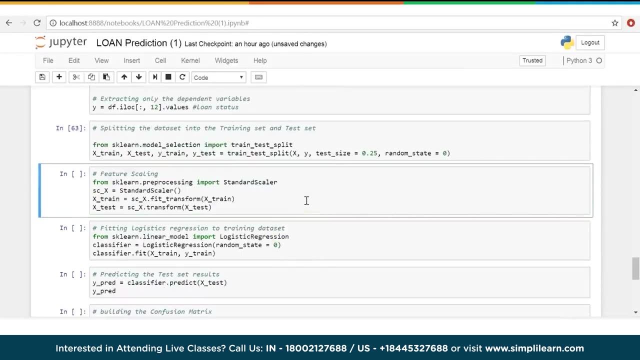 x train, the training data, which is 75 percent of it. Similarly, independent variables for test will be in x underscore test And dependent variables train will be in y underscore train and dependent variable test will be y underscore test. Once we do this, we have to do a small exercise for scaling. Remember we had some data. 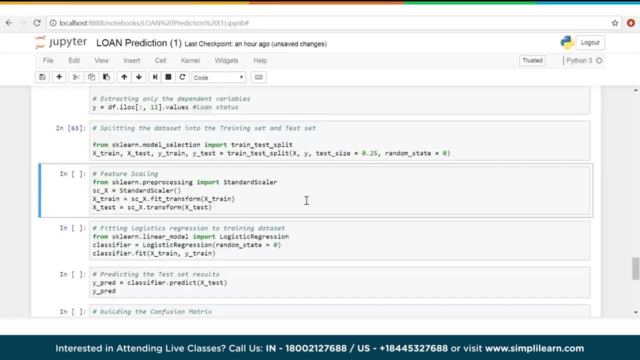 which was kind of very scattered. There were some extreme values and so on. So this will take care of that, so that the data is normalized, so that, before we pass to our algorithm, the data is normalized, so that the performance will be much better. The next step is to create the training data set. 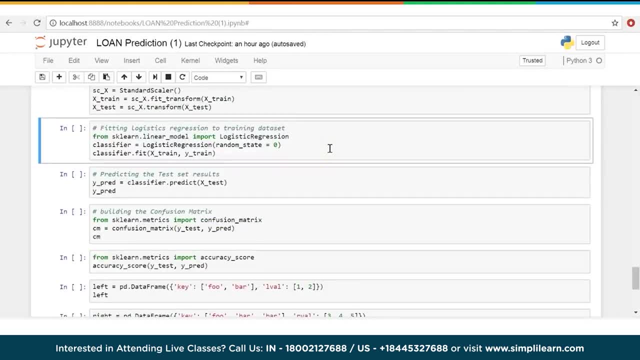 So we have to create the instance of logistic regression object. So that's what we are doing here. So classifier is our logistic regression instance, Classifier is equal to logistic regression. we are saying: So one instance of logistic regression is created, and then we call: 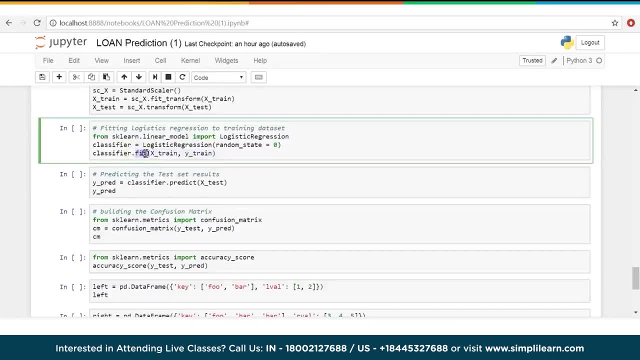 the training method. The name of the method actually is fit, But what it is doing is it is taking the training data. X is the training data or the independent variables, and y is the dependent variables. So we are taking both of these and the model gets trained. So the method. 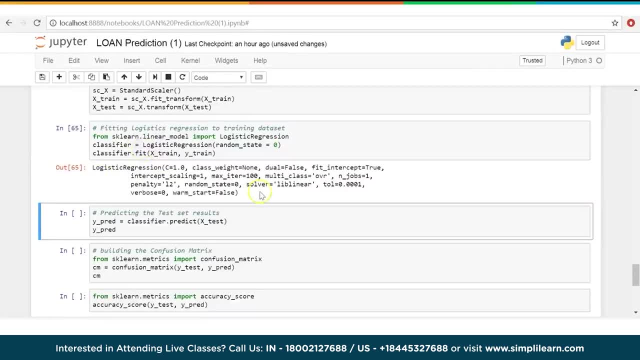 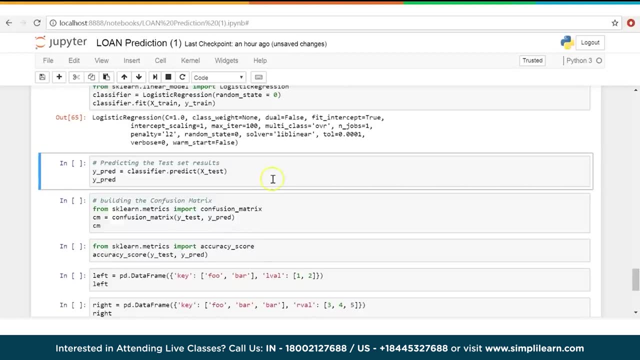 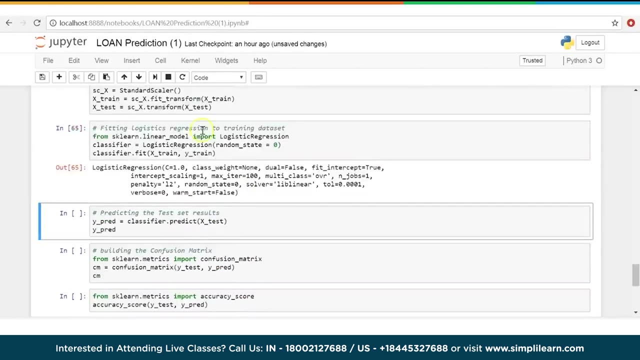 for calling the training is fit, Okay, so it gives us the output. and then, once we are done with the training, we do the testing. And once again, just to recall in the slides, when I was showing you the slides also, I mentioned we don't pass y here. while we are testing, While for training, we do. 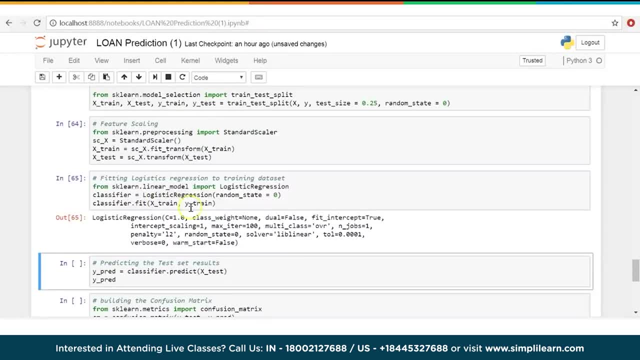 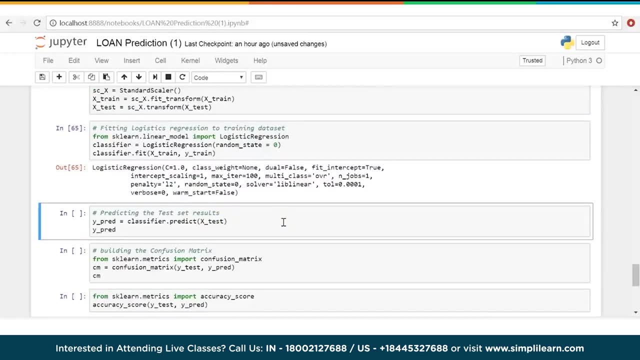 pass y. So for fit, we are passing X and Y, But for test we are only passing X, something you need to observe, because y will be calculated by the modelcsv vs login. anderer Has apost不了 wie C kann. des types wird im Absatz des learningetz werden entwickelt. 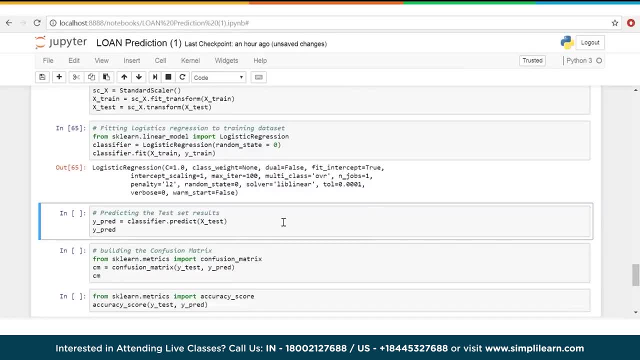 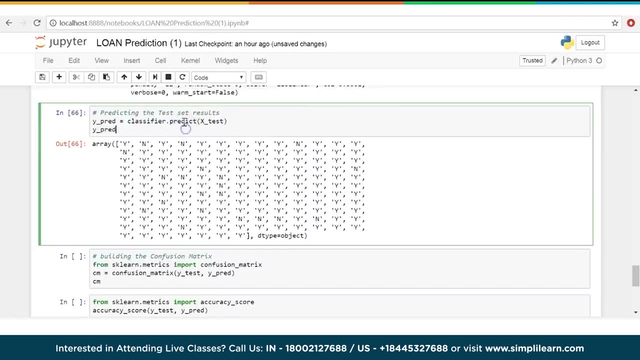 And we will then compare that with the known value of y to measure the accuracy. So that's what we will do here, And the method that is called here is predict. So this will basically create or predict the values of y. Now we have in this case a binary classification. 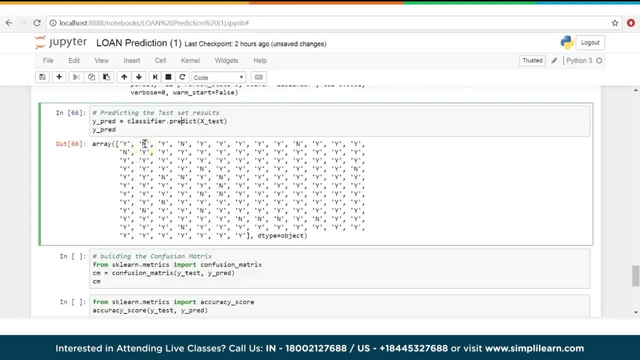 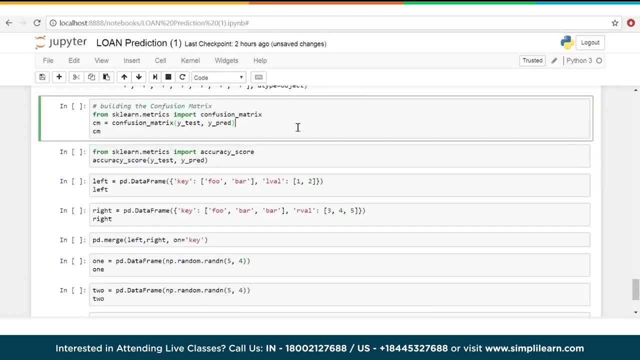 So the outputs are yes or no. Y indicates yes and n indicates no. So y or n is the output. Now, how do we measure the accuracy? As we have seen earlier, I described how confusion matrix works and how we can use confusion matrix for calculating the accuracy. 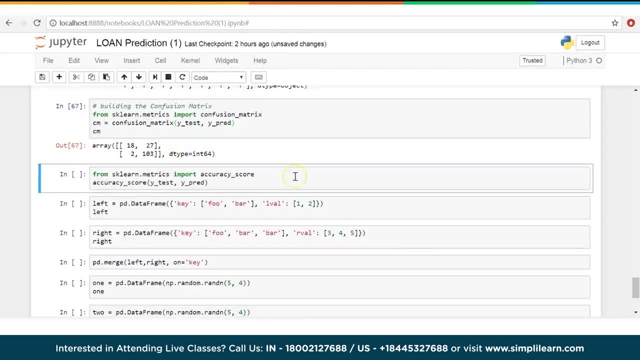 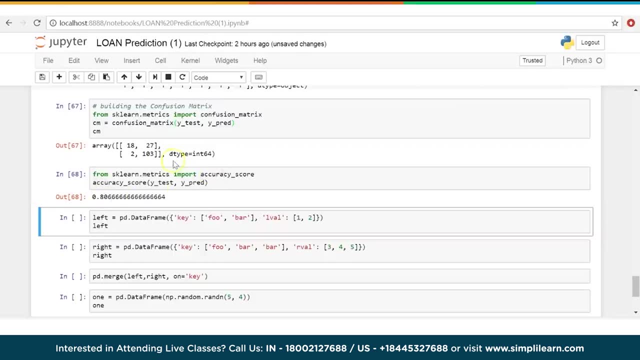 That's what we're seeing here. So this is the confusion matrix And then you want to do the measure, the accuracy. you can directly use this method and we find that it is 80%. So we in the slides we have seen, when we calculate manually as well, we get an accuracy of 80%. 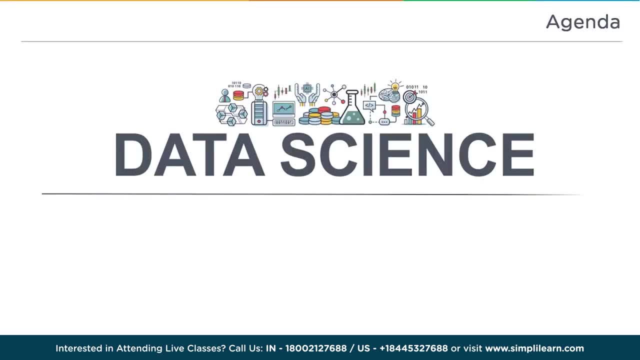 So we will be learning the data science algorithms today by going through the following docket: At first we will learn the logistic regression, And Then we will move ahead and know what is a decision tree. followed by that we will understand what is clustering. next we will learn divisive clustering, later the support vector machine. 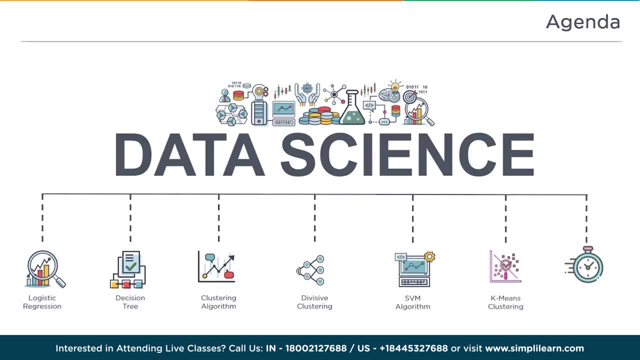 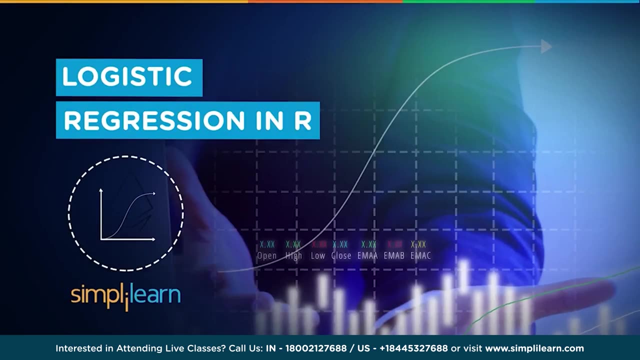 advancing ahead. We will have the key means, clustering And, lastly, we will wind up the session by learning time series analysis. I hope I made myself clear with the agenda now escalating over to our training experts. Hello and welcome to logistic regression in R. My name is Pete Ferrari. 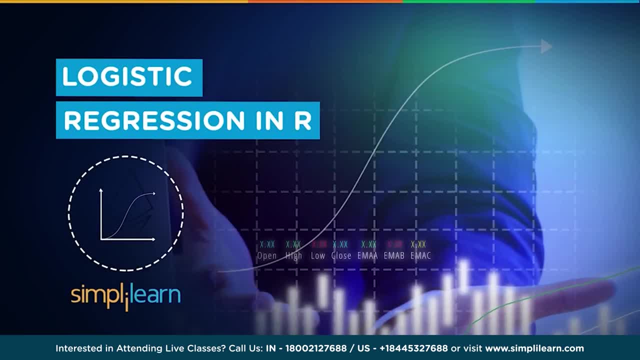 And I am with the Simply Learn team, and today we're going to cover logistic regression in the R programming language. Logistic regression is kind of a misnomer in that when most people think of regression they think of linear regression, which is a machine learning algorithm for continuous 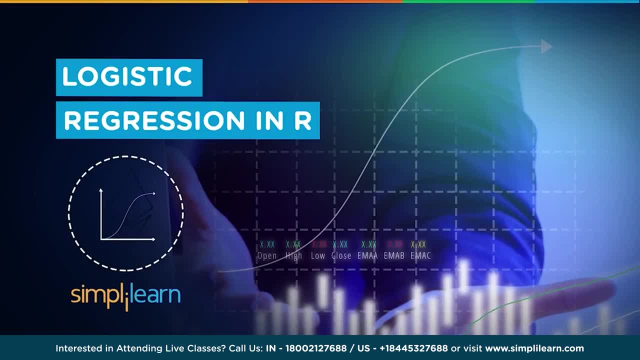 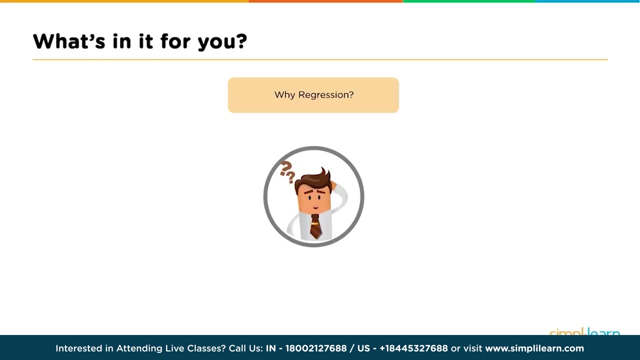 variables. However, logistic regression is a classification algorithm, not a continuous variable prediction algorithm. Logistic regression is also sometimes called logic regression. In This video, we are going to learn why we would use regression as a predictive algorithm. What is regression? 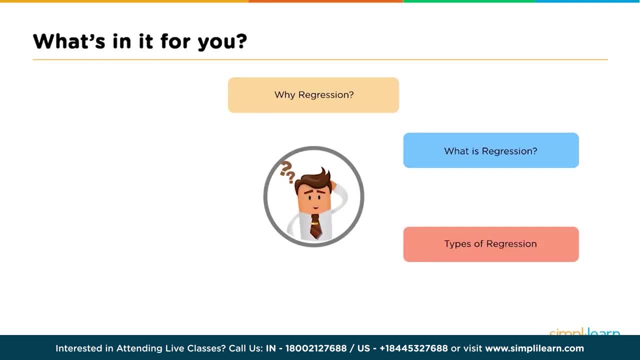 The different types of regression. as I've already mentioned, some regression algorithms are classification algorithms and some are continuous variable algorithms. Why use logistic regression? What is logistic regression? And then we'll look at a use case: a college admission using logistic regression. 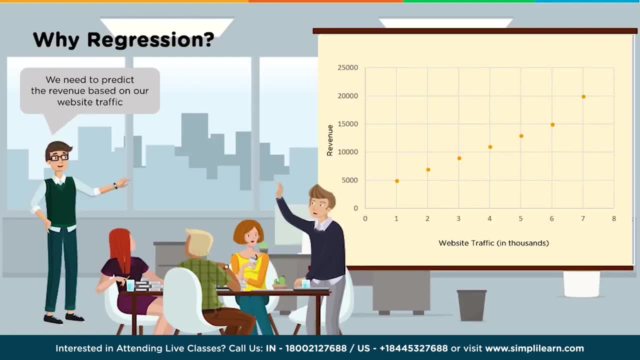 So why would we use logistic regression? Well, let's say we had a website and our revenue was based on the traffic that we could drive to that website, whether through R&D or marketing, and we wanted to predict the revenue based on site traffic. then the website traffic would be related to the revenue we 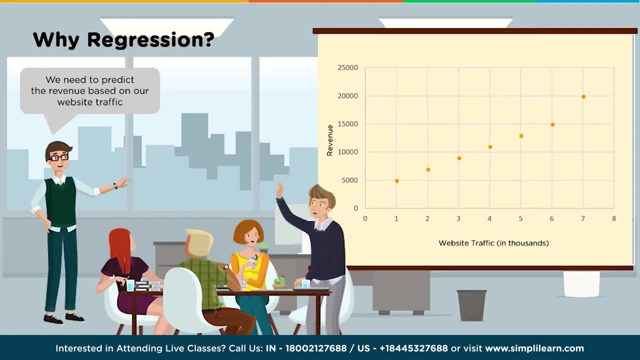 could generate. The more traffic driven to our website, then the higher our revenue, or at least that's what we would intuitively assume, And so we need to predict the revenue based on our website traffic. here we have the plot of revenue versus website traffic. 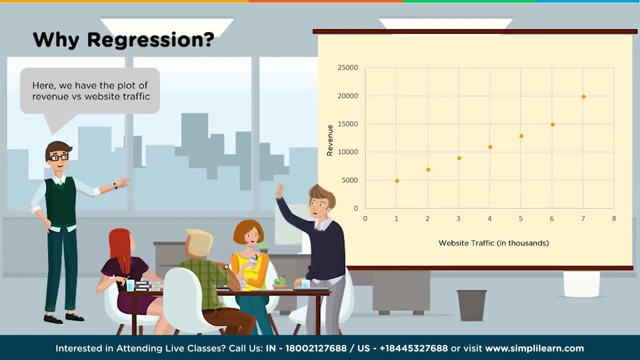 Traffic would be considered the independent variable and revenue would be the dependent variable. Often, the independent variable or variables- if we had more than one- could be called the explanatory variables and the dependent variable would be called the response variable. However, we typically refer to them as independent and dependent variables. 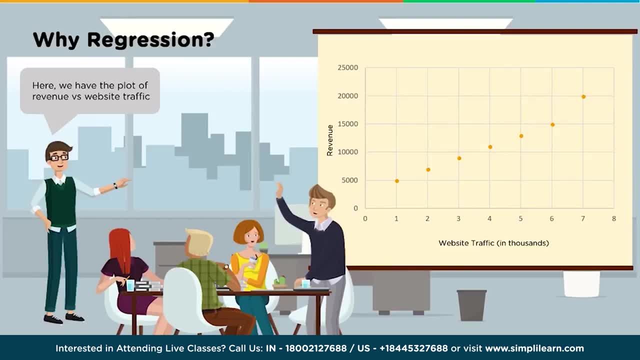 So our intuition tells us that the independent variable drives the dependent variable and if there is some relationship between them, the two variables, and we would say that there is a correlation between the two variables, and then we may be able to use the independent variable to make. 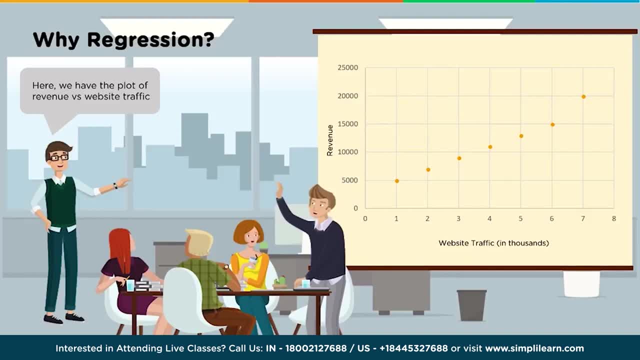 predictions about the dependent variable. if you look at the chart on the right, you'll see there is a clear trend between website traffic and revenue. as website traffic increases, the revenue increases, and we could draw a line to show that relationship and then we could use that line as a predictor line. so for 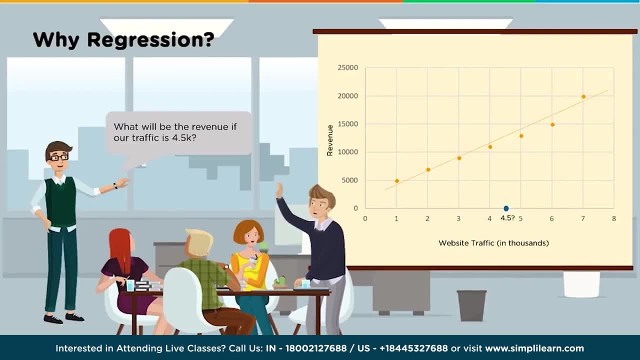 example, what will revenue be if our traffic is 4.5 K? we see that when the traffic is around 4,500 the revenue is around 13,000. and if we could draw perpendicular line from 4.5 K on the axis and the x axis, the traffic axis up? 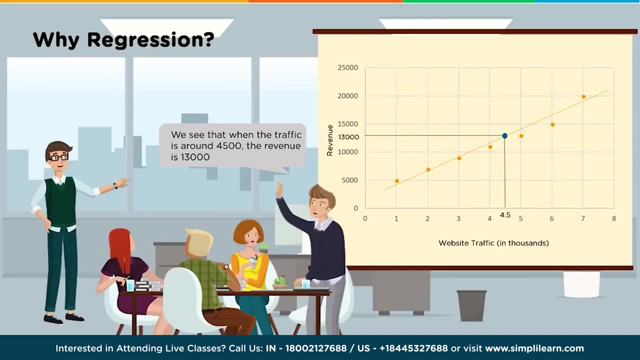 to the orange regression line, sometimes called the line of best fit. then we could draw another line over to the y axis, the revenue axis, and we could see where it lands and that would be the prediction. So in this example, when the traffic is around 45,000 hits, the predicted revenue is around 13,000. 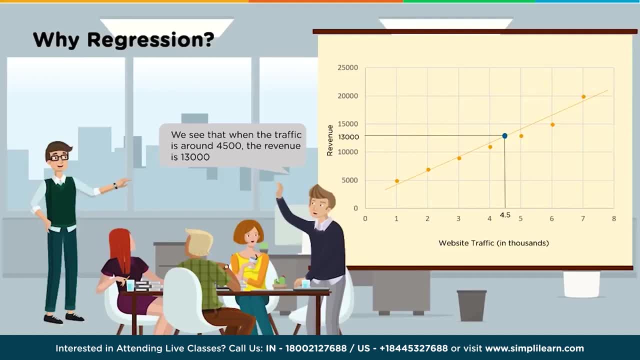 Normally we wouldn't actually draw those lines. We would generate an equation and we would call that equation a model and we could plug the independent variable into the equation to generate the dependent variable output which we would call our prediction. So what is regression? 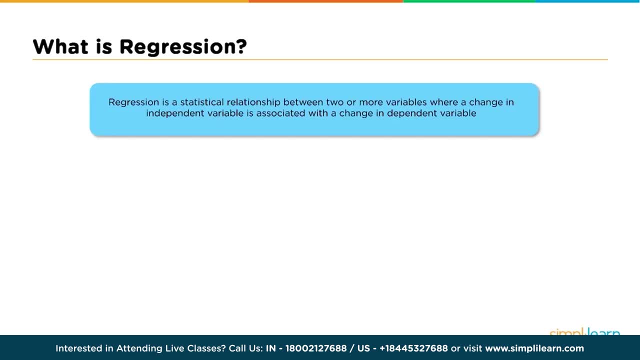 Regression is a statistical relationship between two or more variables, where a change in the independent variable is associated with a change in the dependent variable. It's important to note that not all variables are related to each other. For example, a person's favorite color may not be related to revenue from a website. 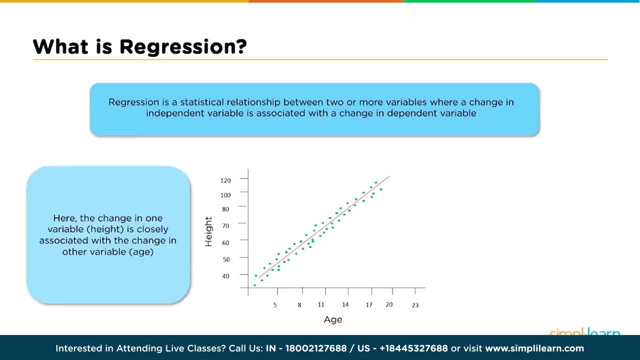 Here the change in one variable, height is closely associated with a change in the other variable, age. This makes intuitive sense: As you get older, from when you're born, you get taller, And it seems to make sense if we plot that data. 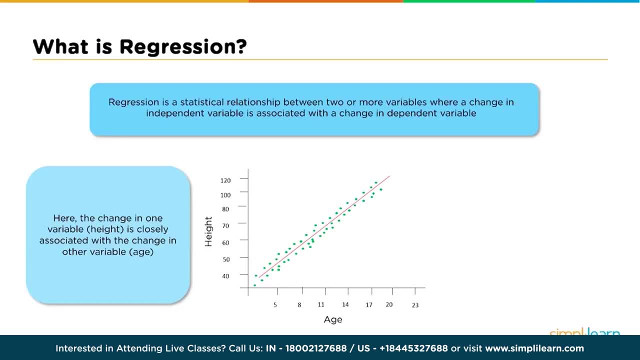 that we would see those green points on the graph up to some certain age where growth would taper off In the plot. in the middle of the screen we see the clear linear relationship between age and height, which is indicated by the solid red line. 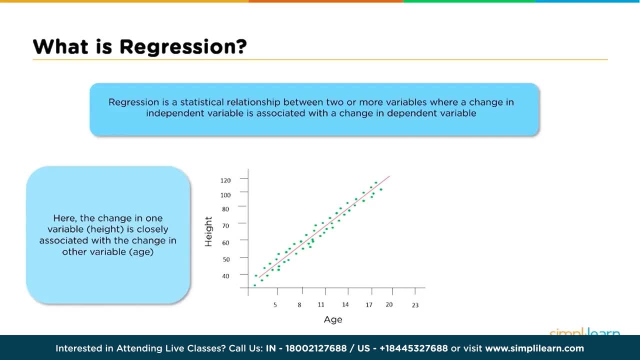 We sometimes call that line a trend line or a regression line or the line of best fit, And we see that the height is the dependent variable and age is the independent variable. Of course you might ask: doesn't height depend on other factors? 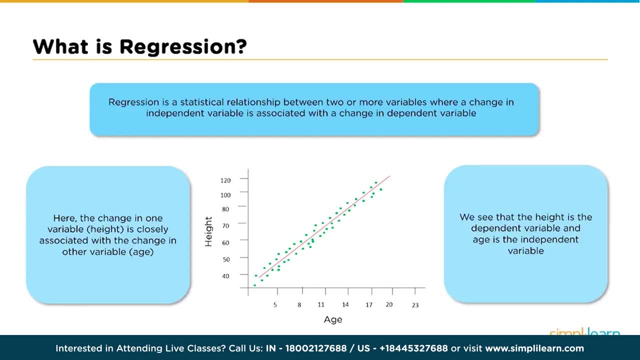 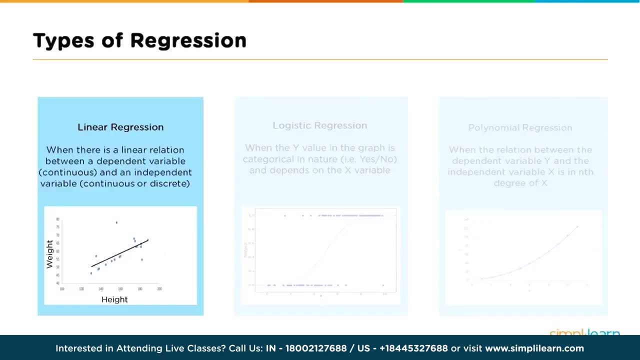 Of course It does, But here we're looking at the relationship between two variables, one independent and one dependent: age and height. There are various types of regression: Linear regression, logistic regression, multiple linear regression, polynomial regression, and there are others. 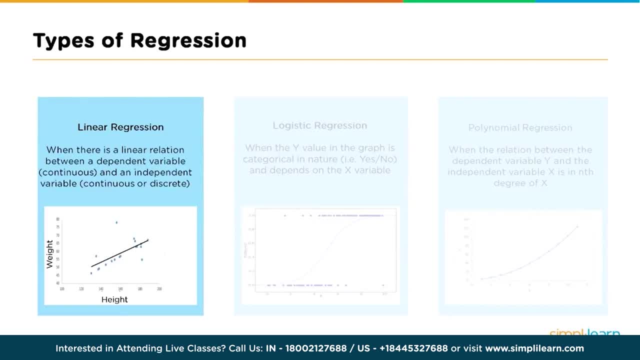 Decision, tree regression, random forest regression, But linear regression is probably the most well-known. By definition, when there is a linear relationship between a dependent variable which is continuous and an independent variable which is continuous or discrete, we would use linear regression. 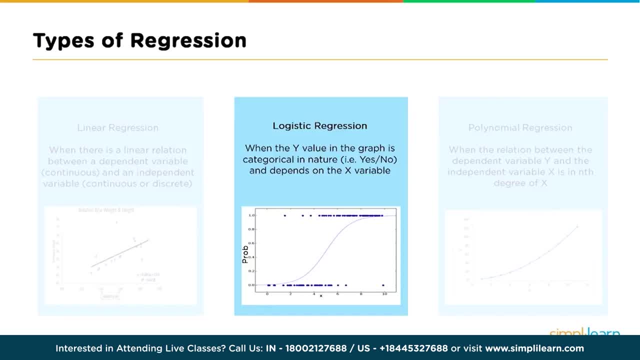 When the y-value in the graph is categorical, such as yes or no, true or false, they voted, they did not vote. they purchased something. they did not purchase something. it depends on the x-variable Logistic regression- is when the y-value in the graph is categorical in nature. for example: yes, no, purchased, don't purchase. voted, did not vote. 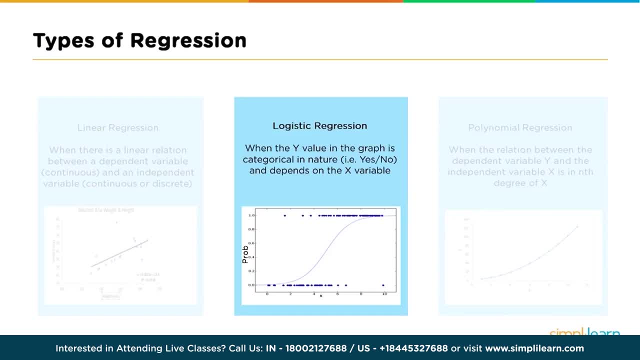 and it depends on the x-variable. Notice the trend line for a little bit Linear regression and the line for logistic regression. they're different- More on that later- And there's polynomial regression as well When the relation between the dependent variable y and the independent variable x is in the nth degree of x. 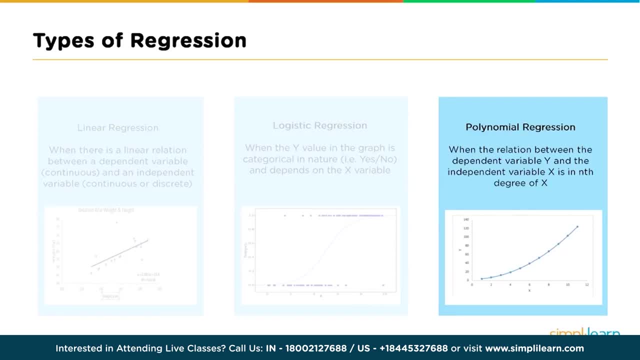 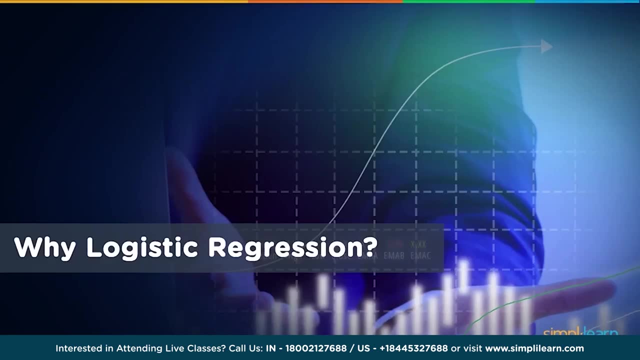 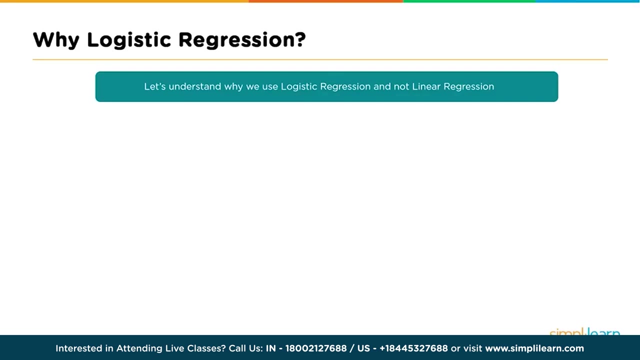 Sometimes we say an nth degree polynomial of x. In this picture you can see that the relationship is not linear. There's a curve to that best fit trend line. So why would we use logistic regression? And we need to understand why we would use logistic regression and not linear regression. 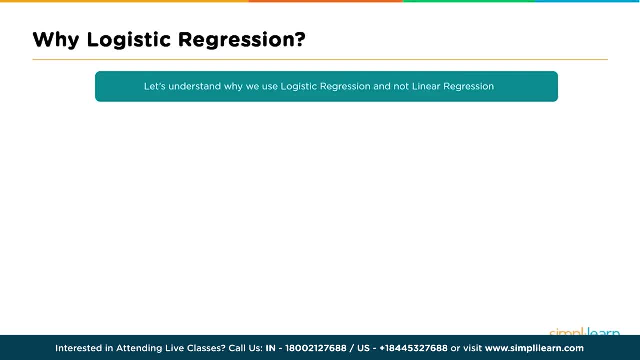 Picking the machine learning algorithm for your problem is no small task, and it really behooves us to understand the difference between these machine learning algorithms. Linear regression answers the question how much. So in our earlier example, if website traffic grows, then how much would revenue grow? 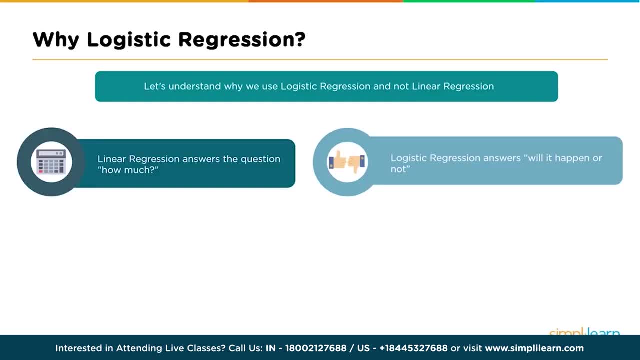 Whereas logistic regression would be how much would revenue grow, Logistic regression would answer what will happen or not happen. Linear regression in general is used to predict a continuous variable like height and weight. Logistic regression is used when a response variable only has two outcomes: yes or no, true or false. 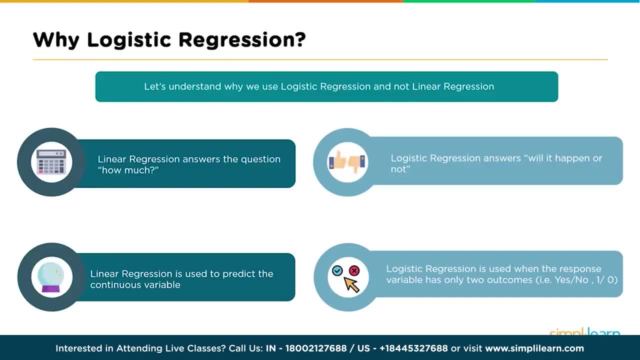 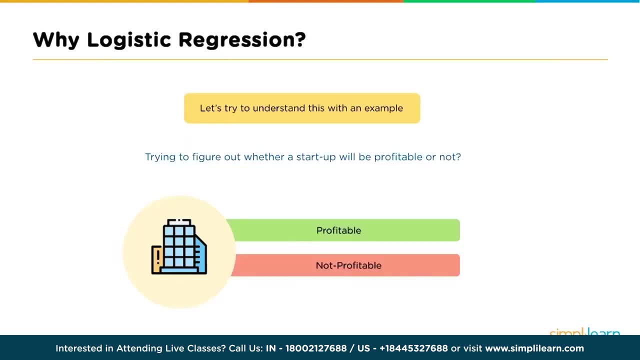 Often we refer to logistic regression as a binary classifier, since there are only two outcomes. So let's try to understand this with an example. Let's say we have a startup company and we are trying to figure out whether the startup company is profitable or not. 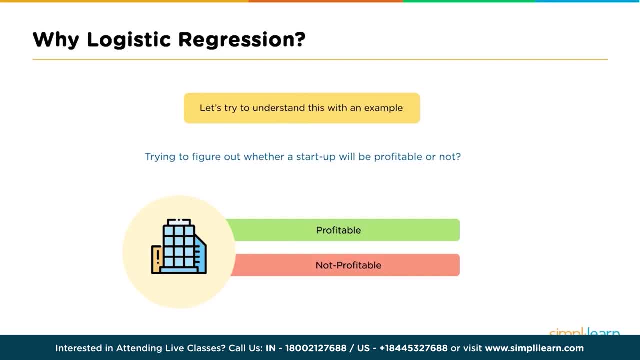 That's binary, with two possible outcomes- profitable or not profitable- And let's use initial funding to be the independent variable. Here we have a graph that shows funding versus profit, And it appears linear. Once again, our intuition tells us that the more funding a startup has, the more profitable. 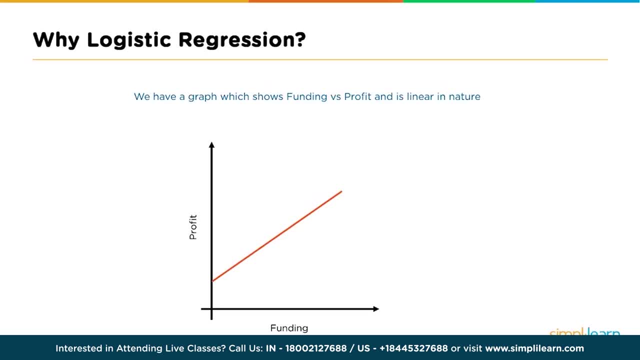 it will be. But of course data science doesn't depend upon intuition, it depends on data. But this graph does not tell whether the startup will be profitable, yes or no. It only states that with an increase in profit the startup will grow, and if it grows, the 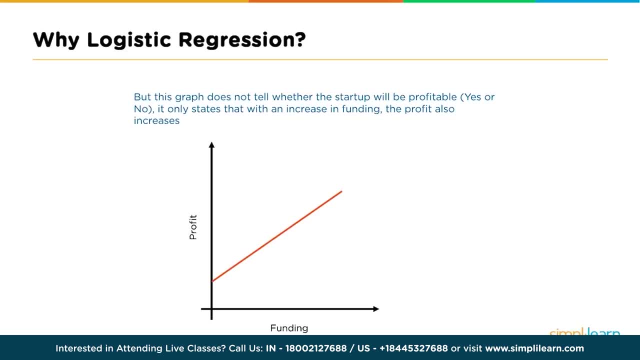 Deburger will not grow, But with an increase in funding, the profit also increases. That's not binary. If we wanted to predict how much profit, then linear regression would be useful, But that's not what we are being asked. Hence we need to make use of logistic regression, which has two outcomes, in our case, profitable. 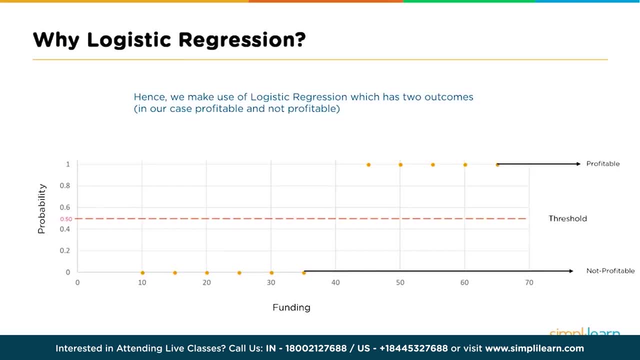 and not profitable. So let's draw a graph again: The x-axis will be our independent variable funding and the y-axis will no longer be the dependent variable profit, but it will be the probability of profit. For example, if you look at a company with a funding of, say, 40, then the probability 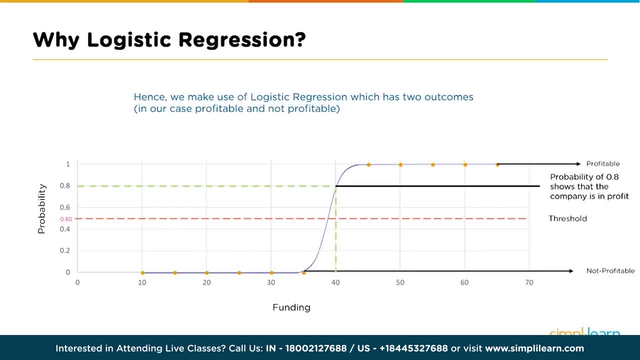 that that company will be profitable is around 0.8, or 80%, based on the best fit line called a sigmoid curve. In the example we plotted several companies, some with 10,, 15,, 20,, some with 50,, 60, or. 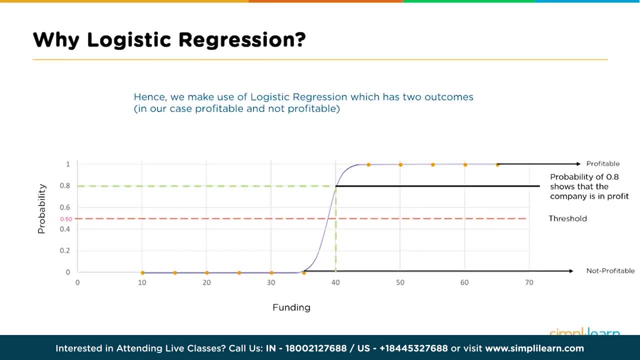 70, or 65.. And we indicated whether they were zero, A zero not profitable or a one profitable on the graph, And this is how we should think of logistic regression. In this example, given the amount of funding, we calculate the probability that a company 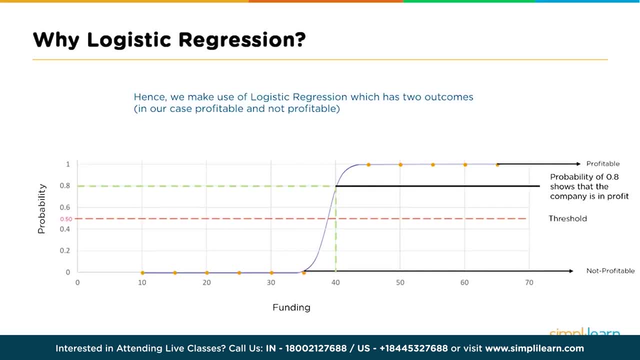 will be profitable or not profitable. And if we use the threshold line of 50%, then we have our classifier. If the probability is 50% or higher, the company is profitable. If the probability is lower than 50%, it's not profitable. 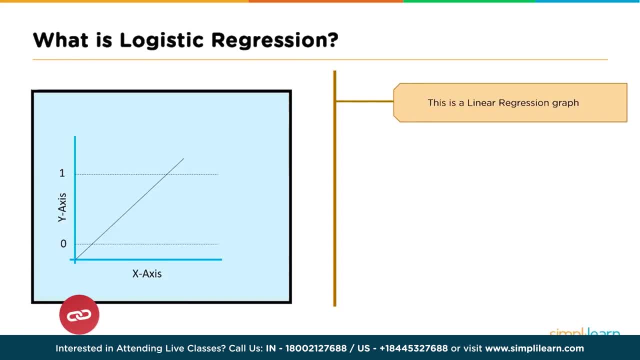 So what is logistic regression? This is a linear regression graph. So let's compare linear regression to logistic regression. So let's compare linear regression to logistic regression And take a look at the trend line that describes the model. It's a straight line, which is why we call it linear regression. 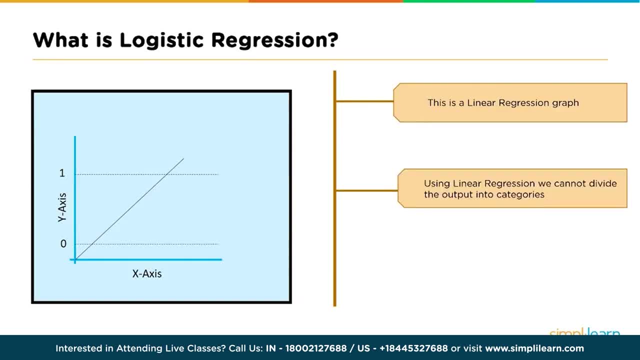 But using linear regression, we can't really divide the output into two distinct categories: yes or no. To divide our results into two categories, we would have to clip the line between zero and one. If you recall, probabilities can only be between zero and one. 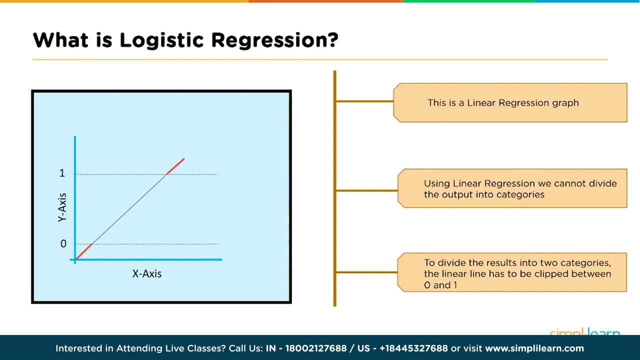 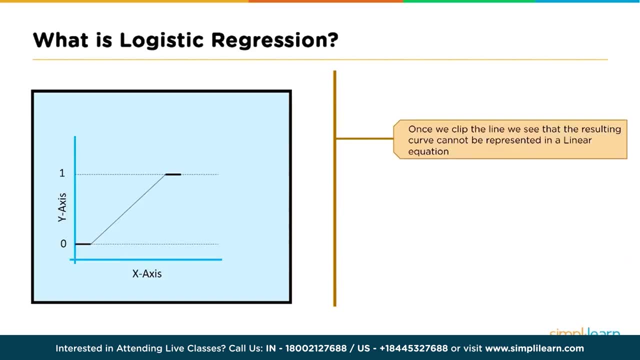 And if we're going to use probability on the y-axis, then we can't have anything that is below zero or above one. Thus we would have to clip the line, And once we clip the line, we see that the resulting curve cannot be represented in a 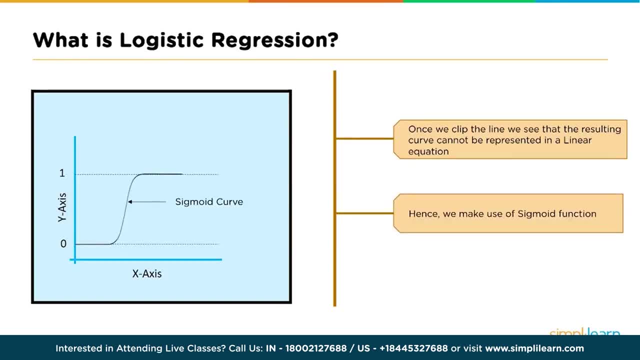 linear equation. So for logistic regression we will make use of a sigmoid function, and the sigmoid curve is the line of best fit. Notice that it's not linear, but it does satisfy our requirement of using a single line that does not need to be clipped. 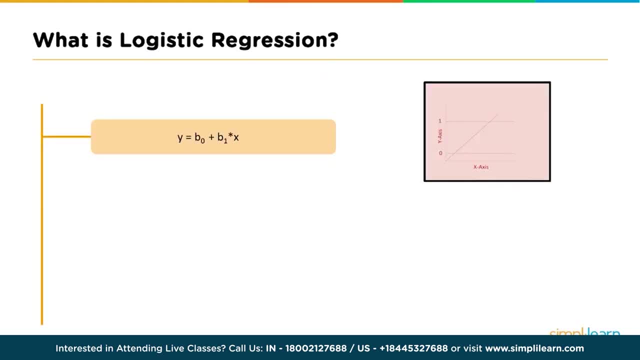 For linear regression, we would use an equation of a straight line: y equals b sub zero plus b sub one times x, x being the independent variable, y being the dependent variable. but, as we've said, we cannot use a linear equation for binary predictions, so we need to use the sigmoid. 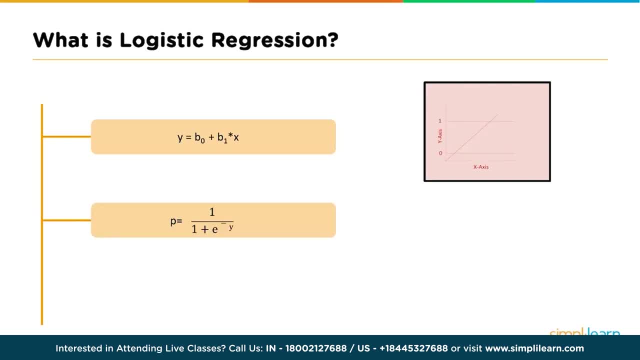 function which is represented by the equation p equals one divided by the quantity one plus e to the minus y, e being the base of the natural logs. Then, taking the log of both sides and solving, we get our sigmoid function. In graphing it, we get our logistic regression line of best fit. 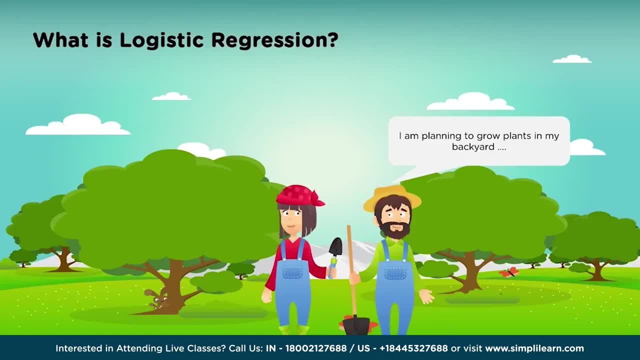 The applications form logistic regression are those above and beyond the limit of a are endless. Here we might have a couple of gardeners or farmers, and one farmer says: I am planning to grow plants in my backyard and I want to know whether my trees will get infested with bugs, which I'm sure is a huge problem. and these 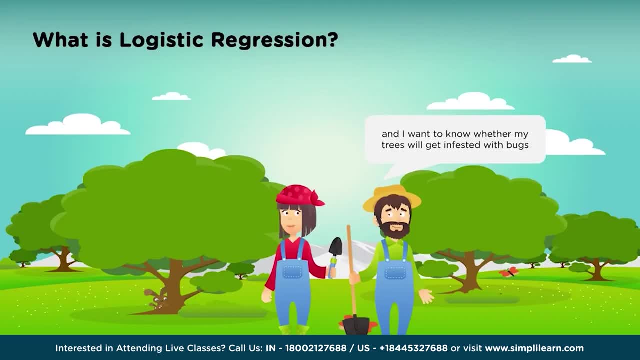 days. the fewer pesticides we use, the better off we are for health reasons. The young lady says: I can use logistic regression in a model to predict it for you. and the other farmer says: well, how is logistic regression going to help? but we know that healthy versus not healthy is a binary classification and we can. 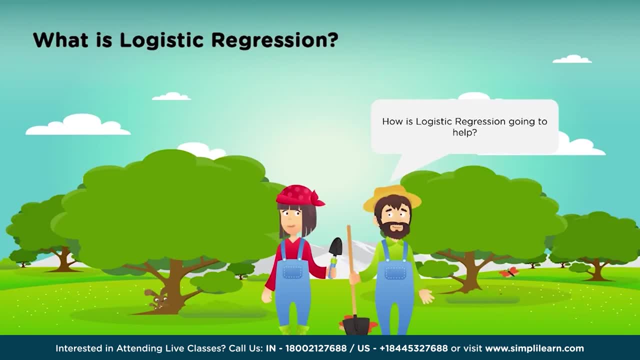 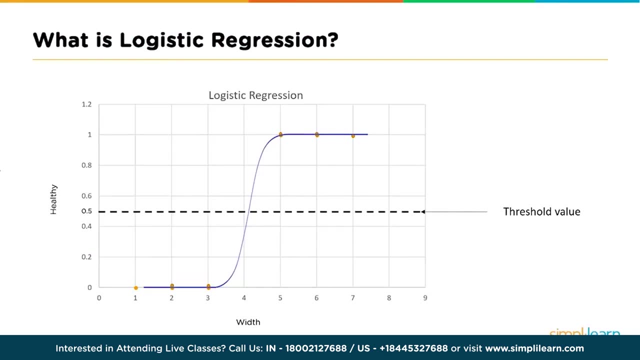 use a binary classifier, like logistic regression, to solve this problem, which is what the young lady has in mind. If we have the data, we can model the data and generate a sigmoid function that best fits our data and then use the probability of a healthy tree versus a not healthy tree or an infested tree. 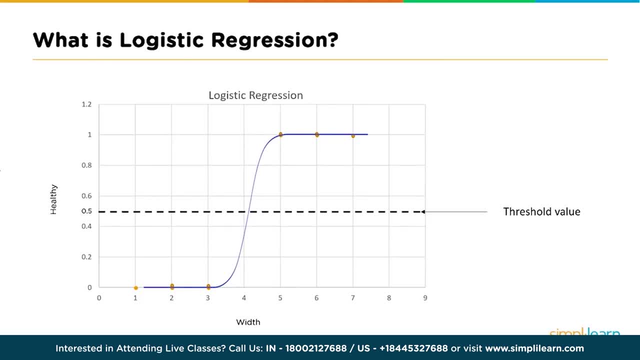 Once again, we see our sigmoid line of best fit and some points that represent a healthy tree versus a not healthy tree. We can use the data to predict the healthy trees and not healthy trees. Once again, we plot our sigmoid curve, scratch that and once again, once our sigmoid curve is plotted and our 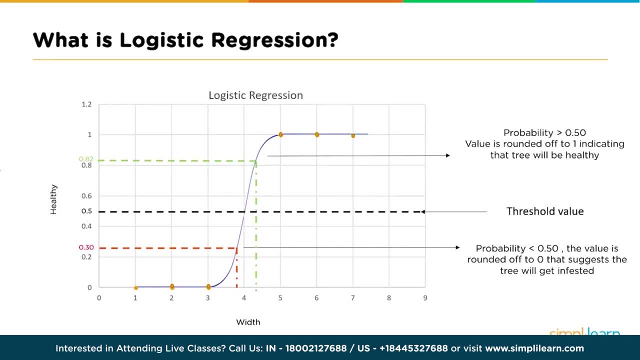 threshold is set almost always at 50%. we can use the sigmoid curve and calculate the probabilities and here the independent variable of width, which I assume is an application of pesticides or no pesticides, to determine whether or not the probability of healthy is greater than 50% the threshold or less than 50% the threshold. And now let's take 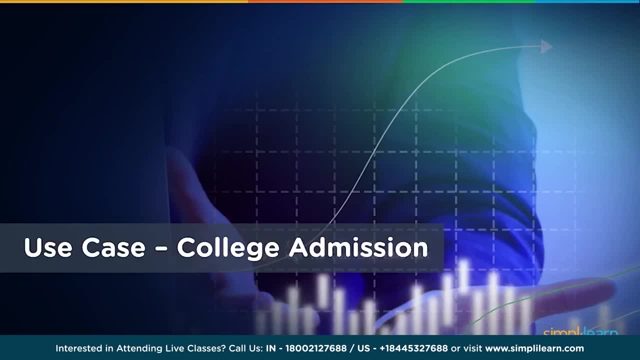 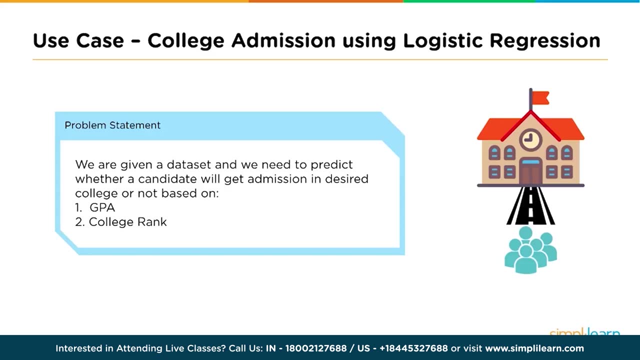 a use case of a college admission problem. Of course, we can't solve anything using data science if we don't know what the problem is. So we need a problem statement, and here the problem statement is simple: We are given a data set and we 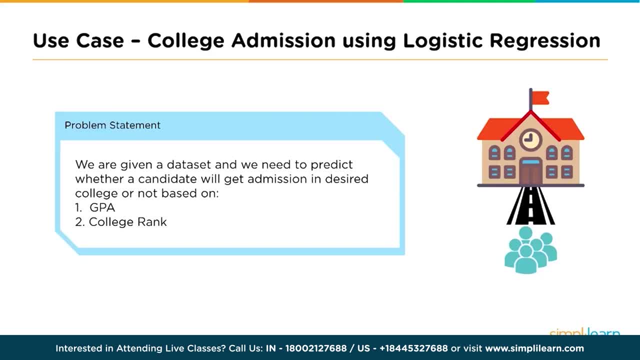 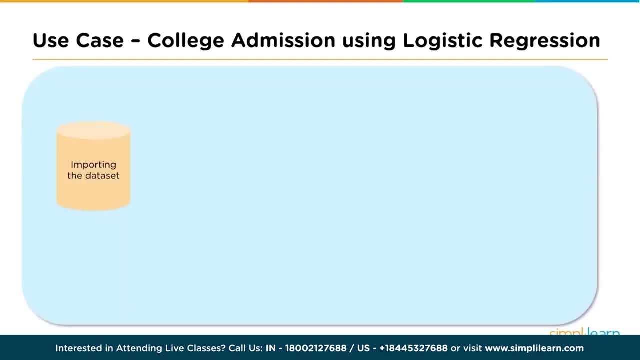 need to predict whether a candidate will get admission in a desired college or not, based on their GPA and college rank. So the very first thing we need to do is import the data set. If it's a small enough data set and it can fit into our computer memory, then we are. 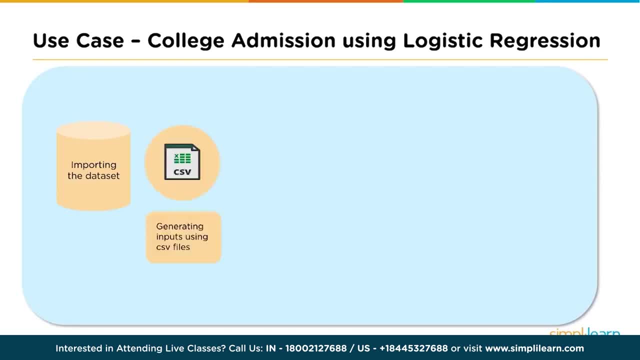 golden. Otherwise we have some work to do. The data set that we were given is in CSV format, comma separated values. CSV files are easily imported into our environment. Once we import the data, we next need to select and import the libraries that we will need. Although R is a great programming language, with a 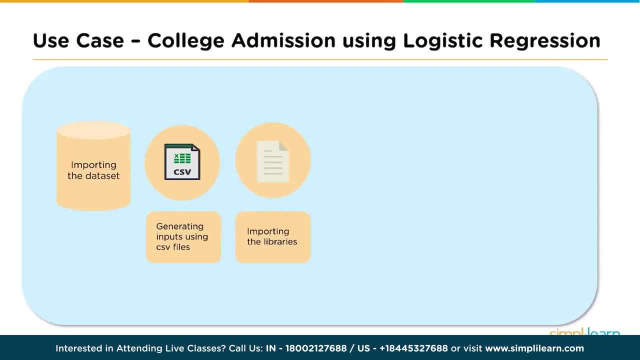 lot of built-in functions. it is easily and powerfully extended by the use of libraries and packages. Then we need to split the data set into a training set and a test set. It's important to note that the data set that we've imported, that we were given, has 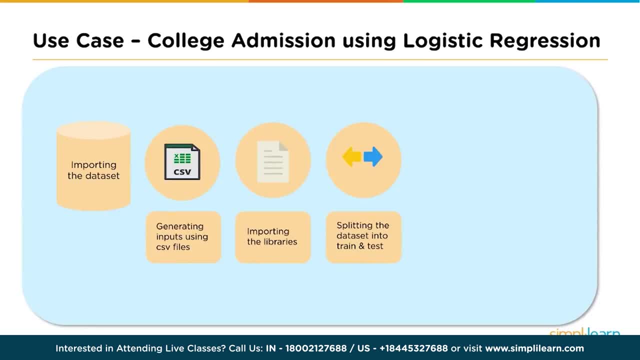 the GPA and college ranks for several students, but it also has a column that indicates whether those students were admitted or not. So what we're saying is that the data set has the answers and if you think about it, it must. How could we possibly train a model, have a model, learn, if we didn't know the answers? 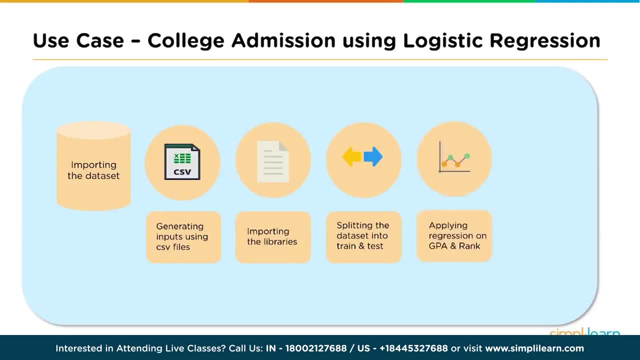 already. That's why it's called machine learning. So we train the model and then we test the model. Once we split the data into training and test sets, we will apply our regression on the two independent variables, GPA and rank, generate the model and then run the test set through the model. Once that is complete, we will 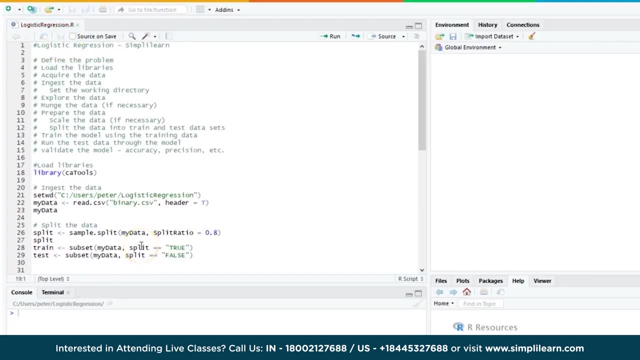 validate the model to see how well it performed. So now it's demo time. So here we have RStudio, my favorite IDE or integrated development environment, and I have a script already composed to run our RStudio. So let's just walk down the script before I run it and talk about the 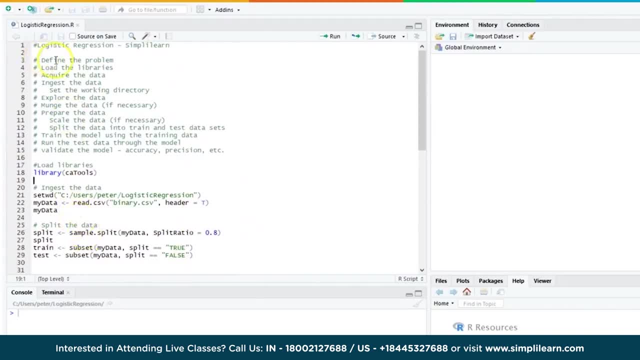 various points in the script. So first define the problem. Well, the problem was defined and you really can't do anything in data science without a clear problem definition. Once the problem is defined, you can load your libraries, acquire your data, set the working directory- in my case I'm on Windows- explore the data. 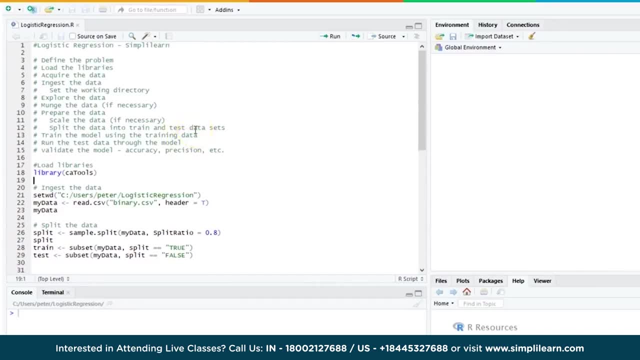 munch the data if necessary and then prepare the data, Scale the data if necessary, split the data into train and test data sets, then train the model using the training data and run the test data through the model and then validate the model for accuracy and precision, etc. So here we are going to. 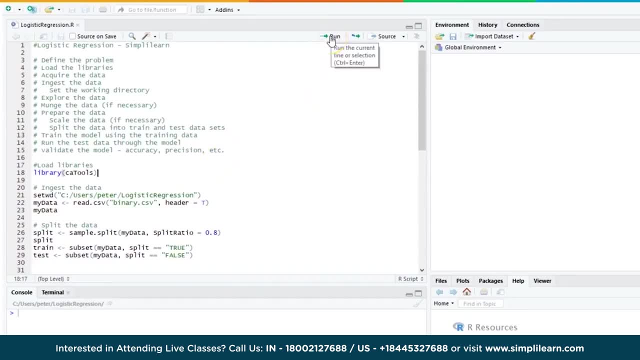 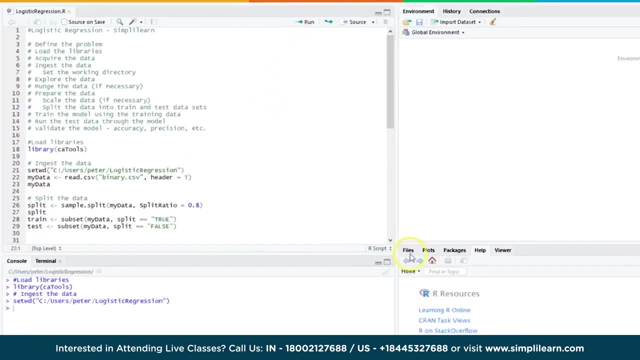 load our libraries. I'm going to use a package called CA tools and now that the library is loaded, I'm going to set my working directory, and if I come over here to the files tab, you'll see that there is my working directory In that. 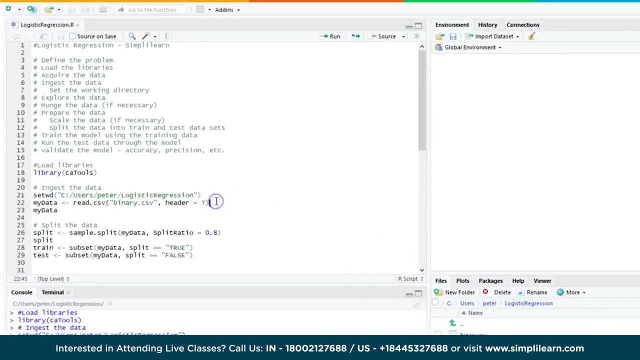 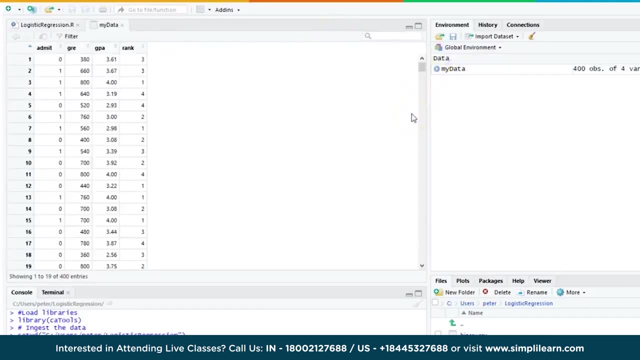 working directory there's a file called binarycsv and that's the CSV, the comma separated value file, that the college gave me. I'm going to adjust and then look at that data and, as you can see, it has four columns: GRE, GPA rank and then the answer column- admit- whether or not someone was admitted, which would be a 1. 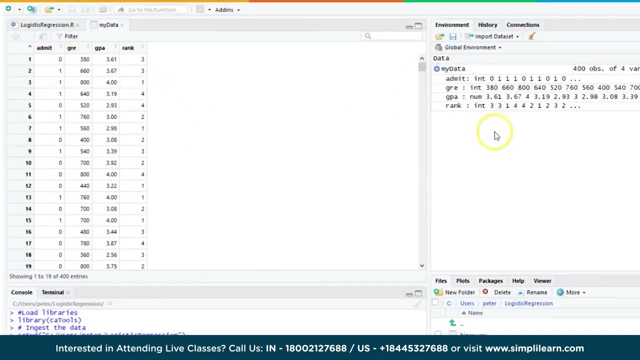 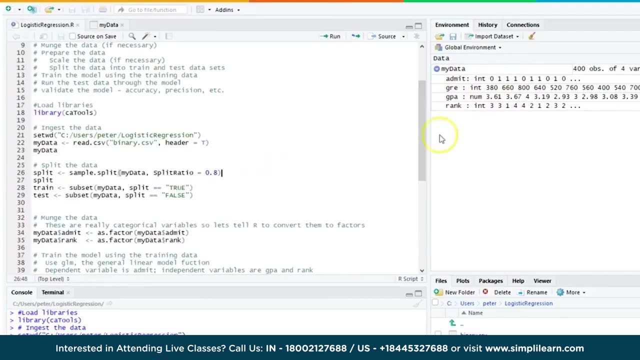 or not admitted, which would be a 0, and if we come over to the right, we can look and see some of the first few values of each of those four columns. Now let's split the data. We're going to take this, my data frame, and split it into two: a. 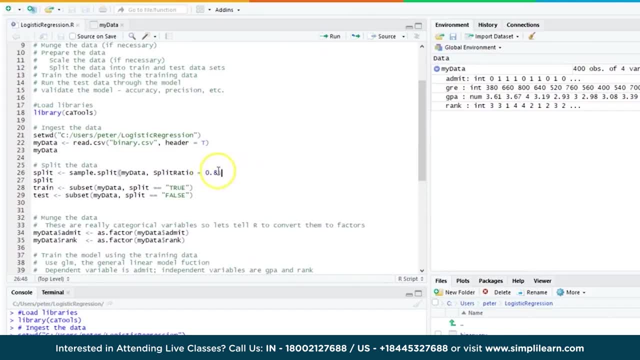 training set and a test set, and the ratio we're going to use is 80- 20. so 80% of the data will go into the training set and 20% will go into the test set. Now that ratio could be 60- 40, it could be 70- 30. typically it really depends on. 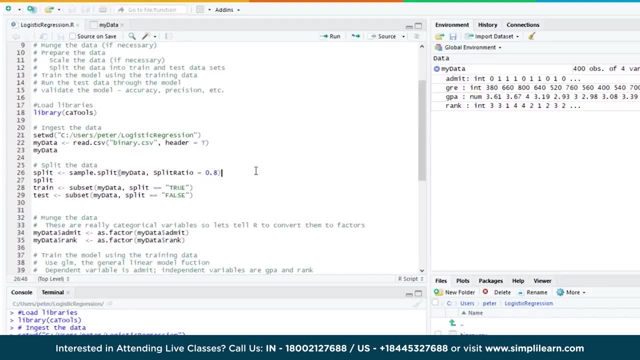 the size of your data, how much data you have. but this is for our example and for our purposes, 80- 20 is perfect. Next, we'll do a little data munging. in general, you munged the data early on after ingestion and you really have to. 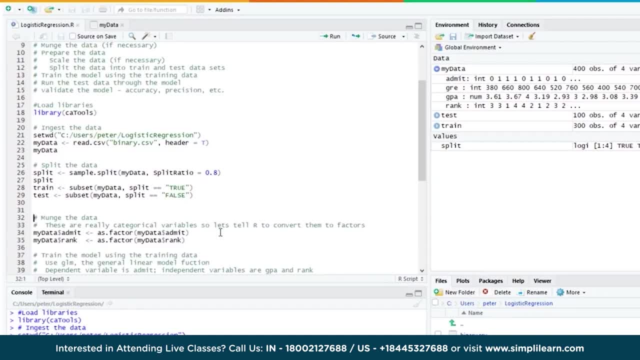 be careful in this case. we don't have any missing values. we don't have any real outliers. our data was pretty clean when we got it and ingested it. but in general that's not the case, and a lot of work and a lot of attention needs to be paid to the munging process. here we're just going to 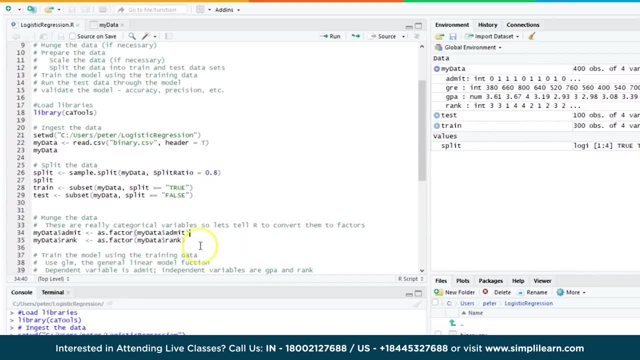 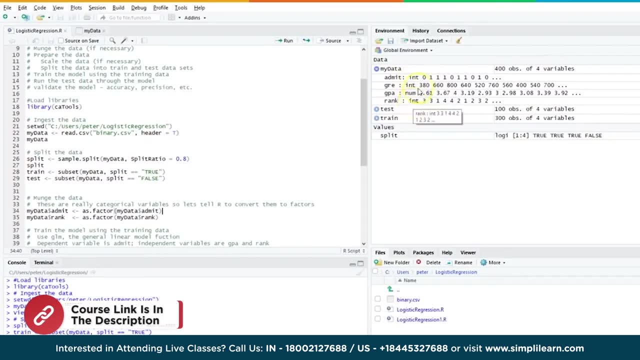 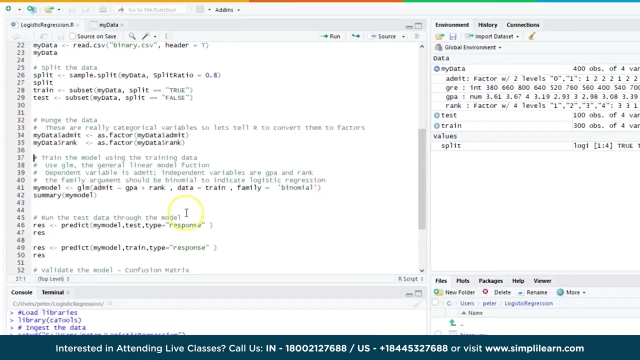 take our data- the admission column and the rank- and convert them to categorical variables. Right now they're integers, as you can see on the right hand side, and once I run these two lines they will be converted to factors. And now the fun stuff: we're going to use the GLM. 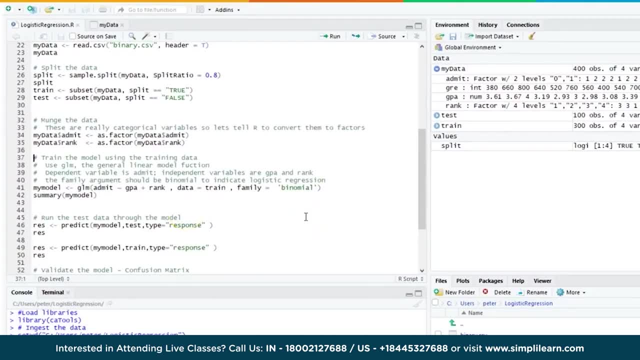 function, the general linear model function to train our logistic regression model, and the dependent variable is admit and the independent variables are GPA and rank and the little tilde sign here says the dependent variable will be a function of GPA and rank, the two independent variables. The data will be the training set and the family will be binomial and 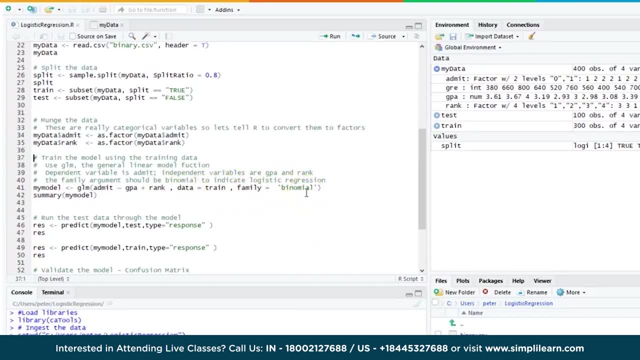 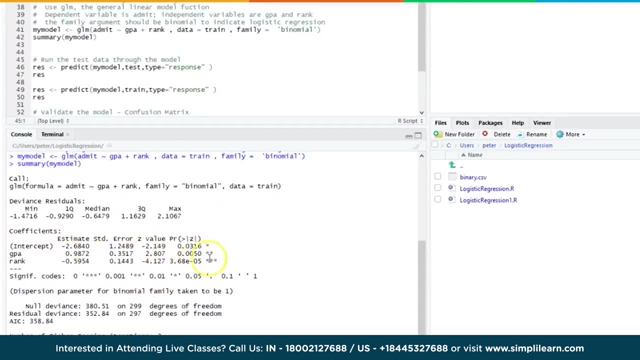 binomial indicates that it's a binary classifier. it's a logistic regression problem. There it is. we ran our model and there's a summary of our model. you can see that there is some statistical significance in GPA and in rank by the coefficient of GPA and rank. 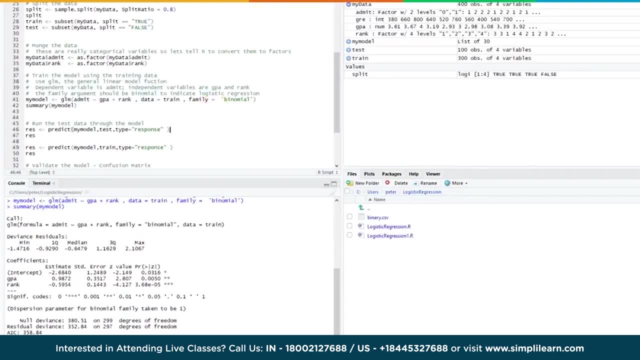 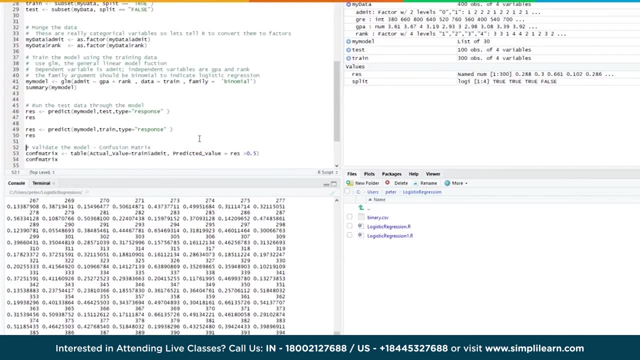 So next let's run the test data through the model and once we have done all that, we can now set up a confusion matrix and look at our predictions versus the actual values. Again, this is important: we had the answers and now we took and we predicted some answers, so hopefully our 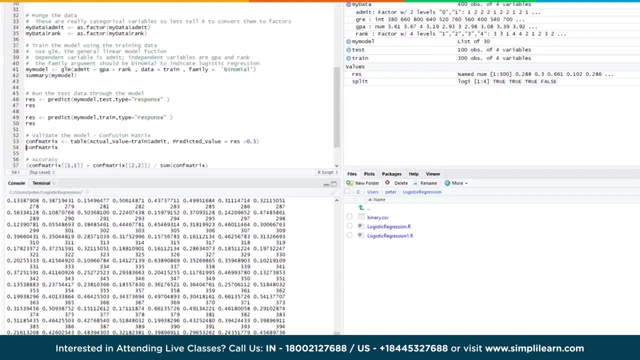 predicted answers match up with the actual answers. We'll run a confusion matrix, As you can see. we've got the answer, and we've got the answer, and we've got the answer, and we've got the answer, As you can see, the predicted values: 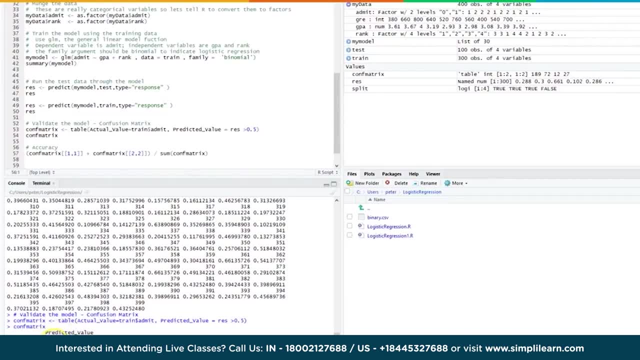 versus the actual values, and it's important here to note that if it was predicted false- and it was actually false, and we see 189- or if it was predicted true and it was actually true, which is 27, we did well on those, but there are few that were predicted incorrectly. some were predicted true, but 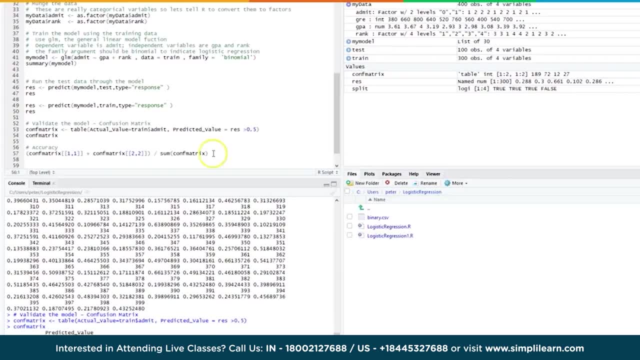 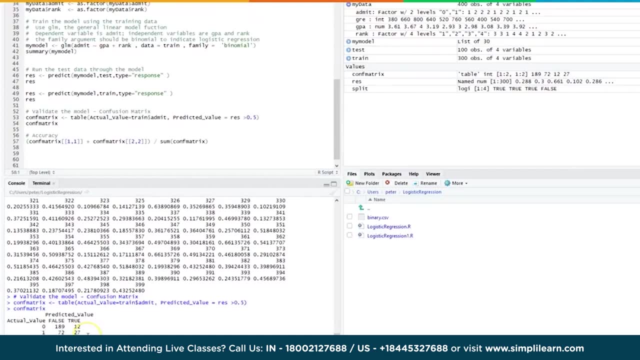 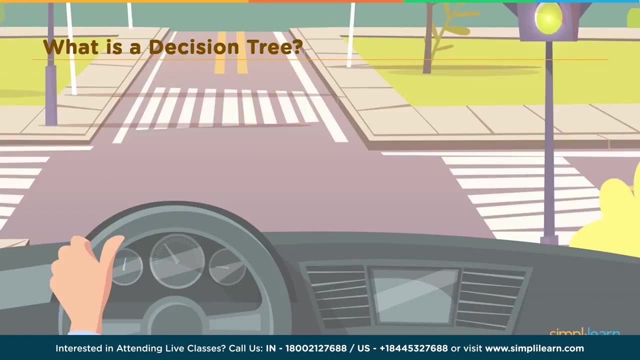 were actually false. some were predicted false. that were actually true and now we'll confirm what our percentage accuracy is: 72 percent, not bad, but we could probably do better. how? we'll leave that to another video. what is a decision tree? and here we have kind of a new looking front panel of a car driving. 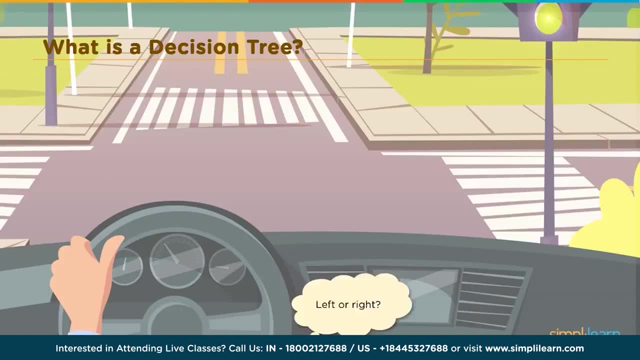 down the street and we have left or right. so you're coming to an intersection. you gotta decide which way to go. are you gonna go left or you're gonna go right, wait or go? so do you go right away? we have a green light, so probably want to go right away. after you check for cross-traffic, make sure no one. 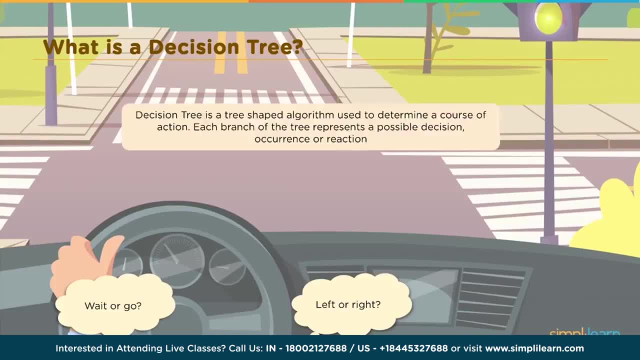 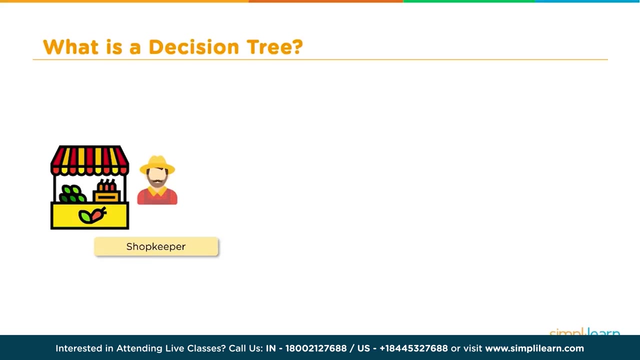 is asleep at the wheel or talking on their cell phone. decision tree is a tree-shaped algorithm used to determine a course of action. each branch of the tree represents a possible decision, occurrence or reaction. so another example is we have a shopkeeper, very nondescript shopkeeper, kind of little spooky without the eyes. so we have a. 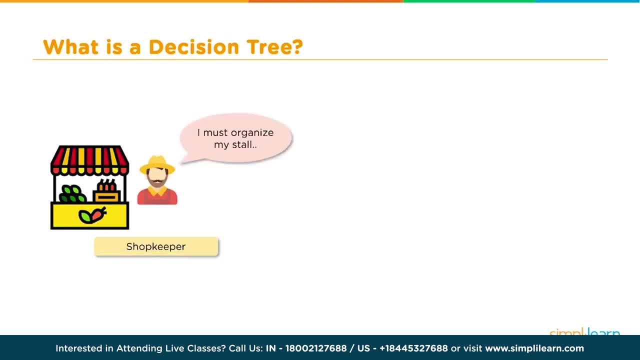 shopkeeper and he wants to organize his stall. so I must organize my stall. just looking around trying to figure out what the best way to stack all his goods are, and he has some broccoli, some oranges and some carrots. this is kind of a nice example, because we can see where some of the colors and shapes overlap. 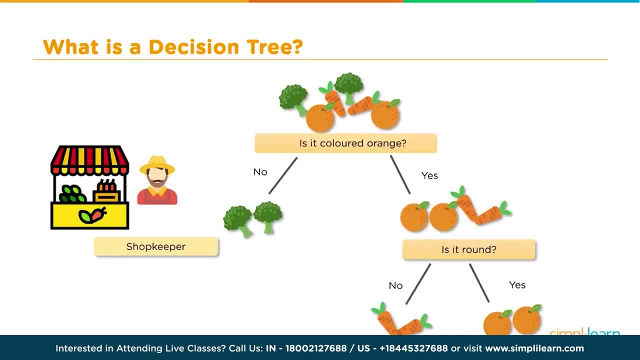 where others don't, and so you can create a tree out of this very easily say: is it colored orange? if it's not, what goes into one stack, well that happens to be all their broccoli. and if it is colored orange, then it goes into another stack and you're like, well, that's still kind of chaotic. you know people are. 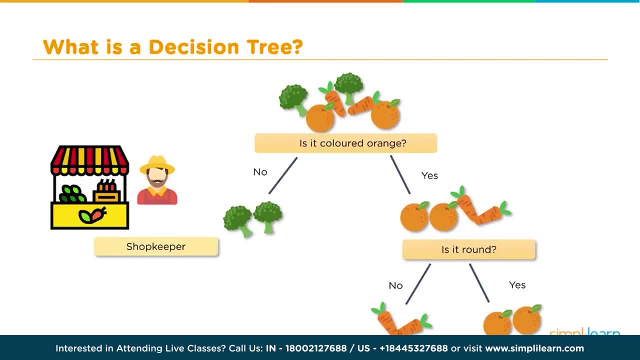 looking at carrots and oranges, a very strange combination to put in a box. so the next question might be: is it round? and if it is, then yes, you put the oranges into one box and no, that means it's carrots, we put it in the other box, and you can see that a lot of stuff we do in life. 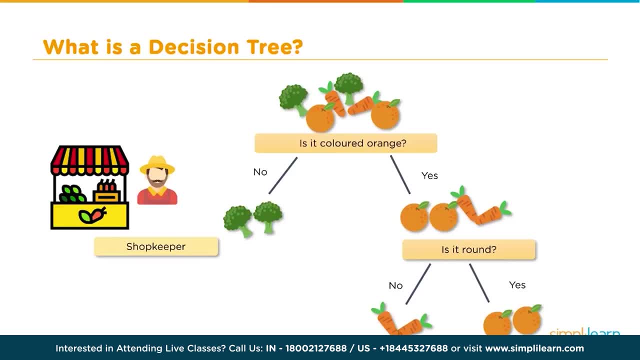 easily can fall into, like a decision tree. how do you decide something you know? does it go left, does it go right, yes or no? and even with this, we even have a number of different end choices: broccoli, carrots and oranges. so what kind of problems does this solve? what problems can be solved by using a? 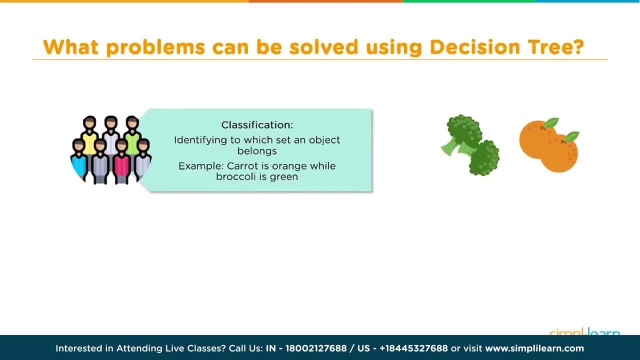 decision tree classification. we're dealing with the classification identifying to which set an object belongs and, from our example we just looked at, a carrot is orange while broccoli is green. I guess it's nondescript days without the faces. I love it. there's a lot of times you're looking at data. you. 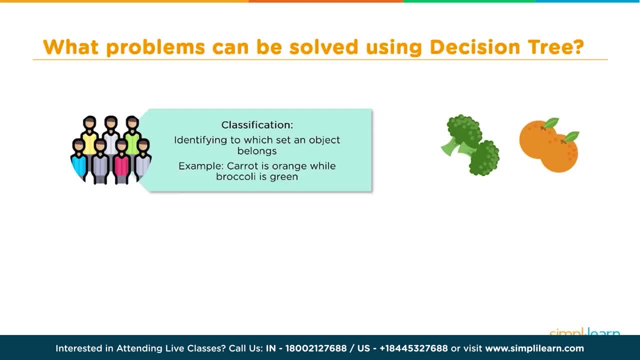 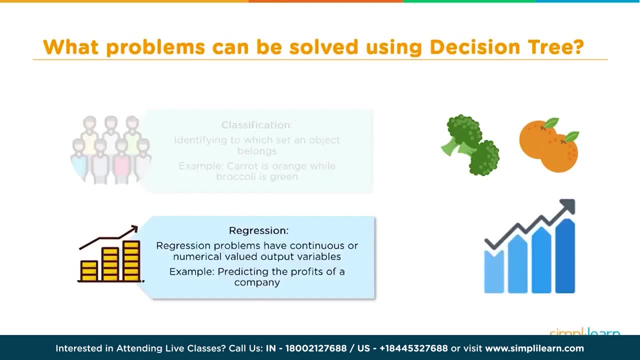 really don't want to know what exactly the data is, but you're sorting it so you know, like this kind of represents data that you really don't know exactly where it's coming from. just kind of a fun thing. regression: regression is another problem. the biggest can be solved. regression: 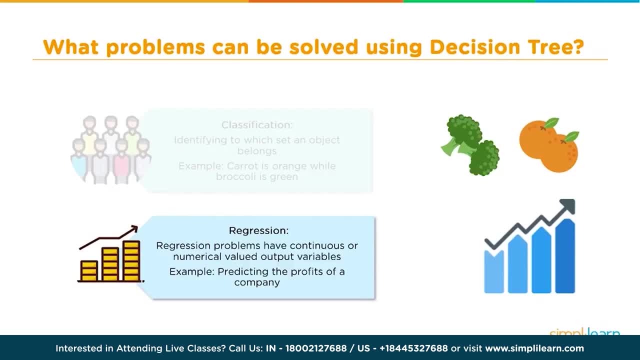 problems have continuous or numerical valued output variables, example: predicting the profits of a company. so we have two different primary problems we solve for. we solve for classification- is it green or is it orange- and we solve for regression, which is a continual number. so you know if you're. 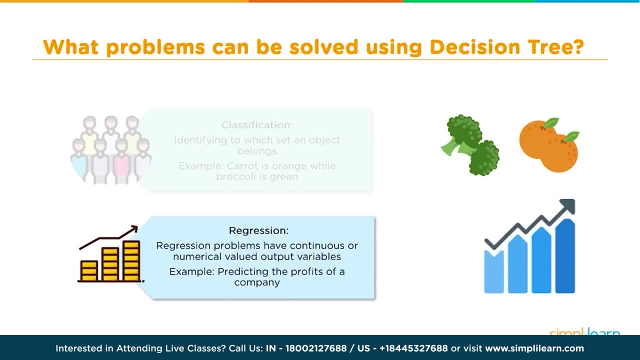 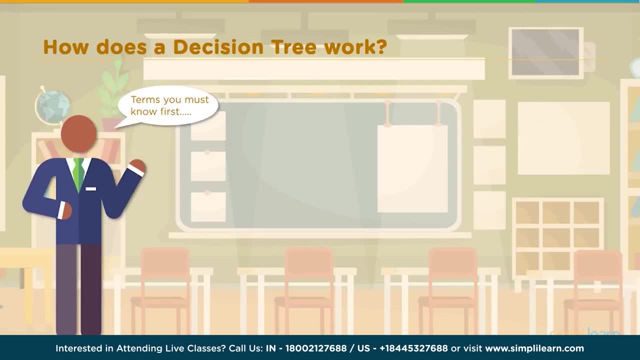 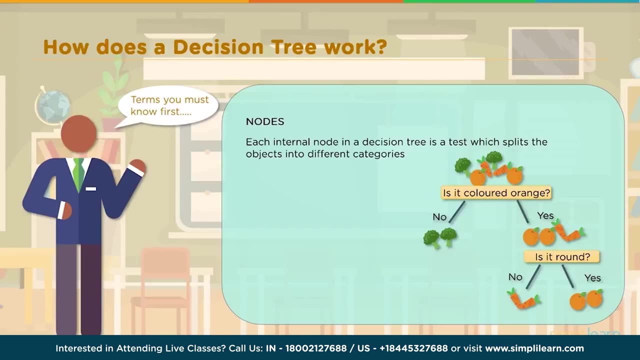 doing stocks just be a dollar value that ranges anywhere from zero to thousands of dollars. how does the decision tree work? terms you must know first. so before we dive into the decision tree, let's look at some of the terminology for the decision tree. we have notes. each internal node in a decision tree is a test which splits. 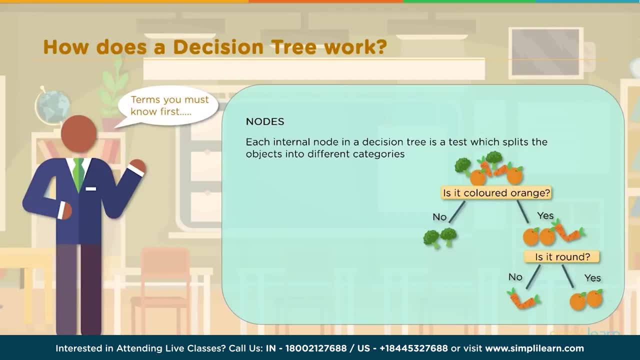 the objects into different categories and continuing with our vegetable stand example, we have broccoli- no, it's not orange- and oranges and carrots are, and so on. so you can see right there where it splits. that's a note- where the orange is split in, the carrot split into each of their own groups and each one of the 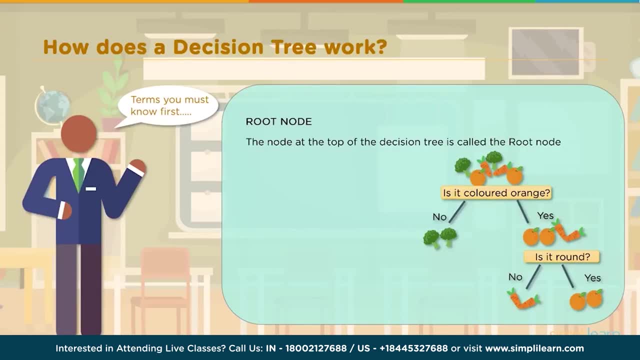 splits is a node. the very top node of the decision tree is called the root node. to the very first one we started off, where we split, it is a colored orange and you can see that point it out nice and neatly there. this is a root node at the top. each external node in a decision tree is called the leaf node. 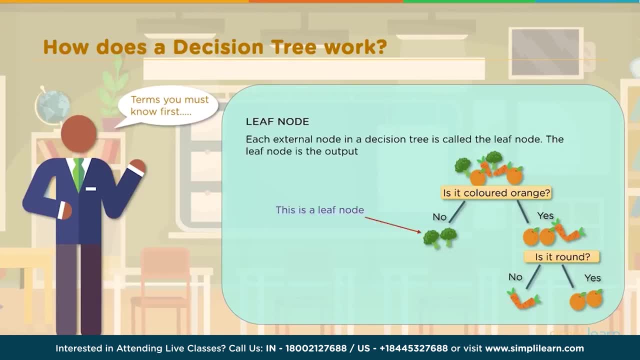 node. The leaf node is the output, and you can see down here. we have our broccoli and we have our carrots and our oranges. Each one of those is a leaf node. So, to quickly rehash our terms we have: anywhere there is a split, that's a node, and if it's at the very top of the tree, that's the root. 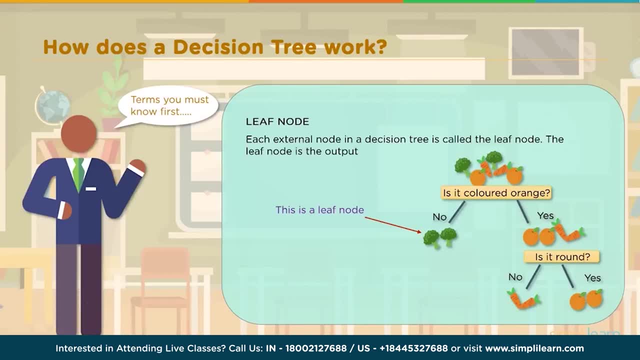 node and if you're at the very bottom of the tree, where you have a final answer, that is the leaf node. So you have a root node, a leaf node and then everything else is just a generic node. So one of the most important terms or concepts that powers a decision tree is entropy. Entropy is a measure. 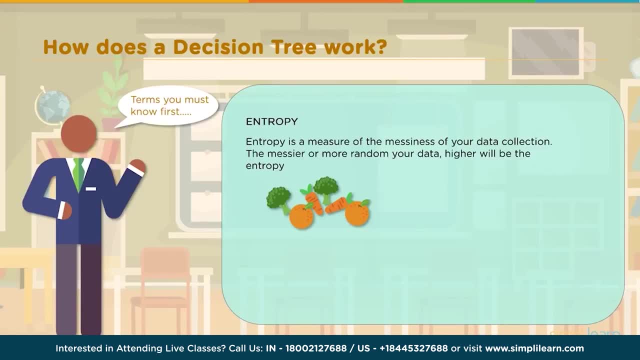 of the messiness of your data collection. The messier or more random your data, higher will be the entropy. So we can see: here we have broccoli, oranges and carrots are all mixed together and it's very chaotic And you could say this collection has high entropy. and if we sort out the carrots, 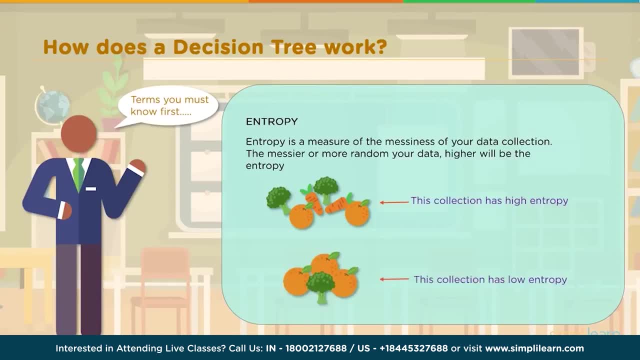 out of here and I guess just one of the broccoli. I don't know where the other broccoli went. you could say if you have just the oranges you have a high entropy, And if you have just the oranges you have a high entropy. And if we sort out the carrots out of here- and I guess just one of the- 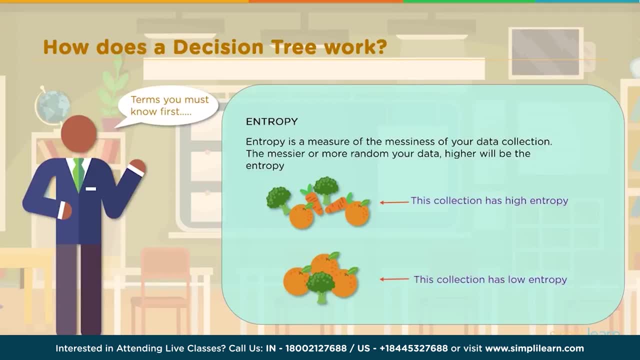 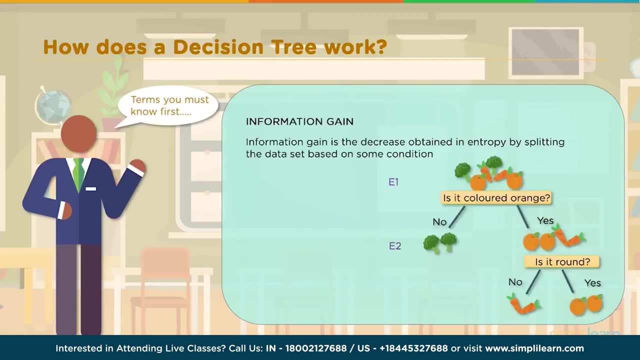 oranges and the broccoli. this is a lower entropy. They say this collection has low entropy, but really it's higher and lower. One is higher or lower than the other one And from entropy we get information gain. Information is the decrease obtained in entropy by splitting the data set. 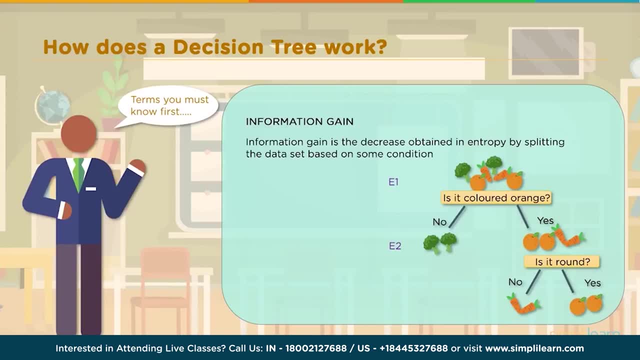 U based on some conditioning. So we have our information 1, which we can actually there's actual computations. And so we have our E1, which is put in there for our entropy value at the base node or root node, And we have E2, which is a leaf node, And so we can actually calculate there's. 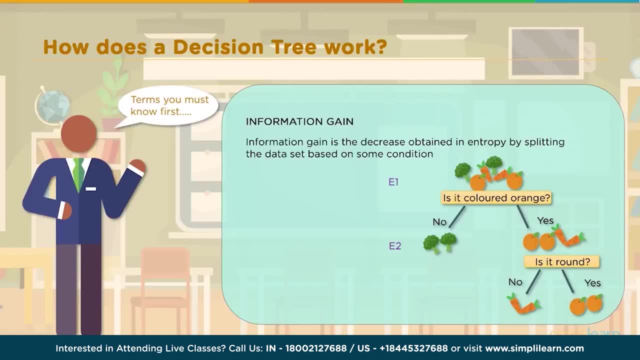 calculations for entropy And we actually look at those two values, the entropy- and we take that we have E1- is greater than E2.. Therefore the information gain equals E1 minus E2.. So here we have another example, and we're actually going to attach some values to this one in just a moment, So we're going to 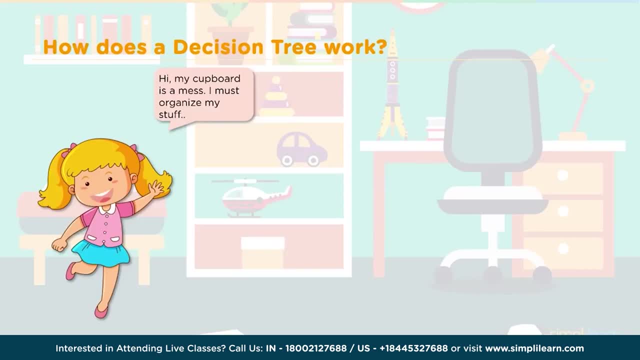 move away from the fruit and we're going to go to everybody's favorite thing: organizing a child's closet. And here we have a young lady waving at us: hi, my cupboard is a mess, I must organize my stuff. And we're going to classify the objects based on their 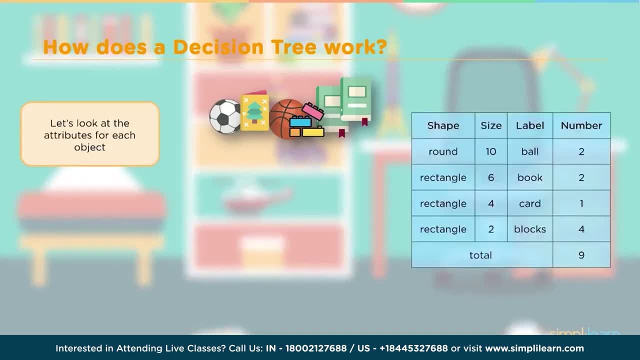 attribute set using a decision tree. We can look at it. we have a shape, a size and a label and a number. And I'm going to go ahead and look at the labels, because that's really what's key on this one is we have a couple balls in here, some books, cards and blocks- And if you look at that, when you have something that's a ball that's round, so it's a very different shape- the book card and block. 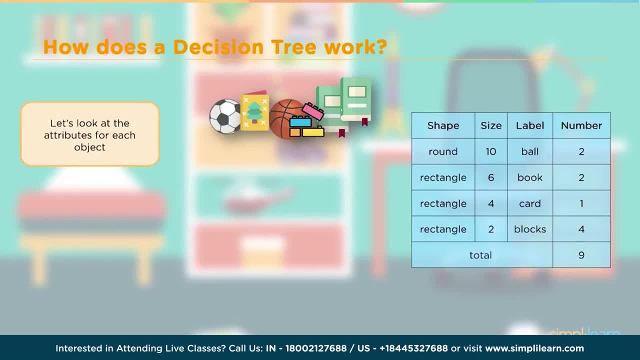 are all rectangular but the books are a different size. So the books have like a size six. I guess you think of them as very large. Cards are size four, so they're not quite as big, And the blocks are little Lego blocks. it looks like kind of fun to stack on there. And then we can actually quantify this and we can actually say, hey, we have different numbers. We have two balls, two books, one card, four blocks, And we split at each level based on certain conditions, on the attributes. So splitting aims at reducing the entropy And we're going to 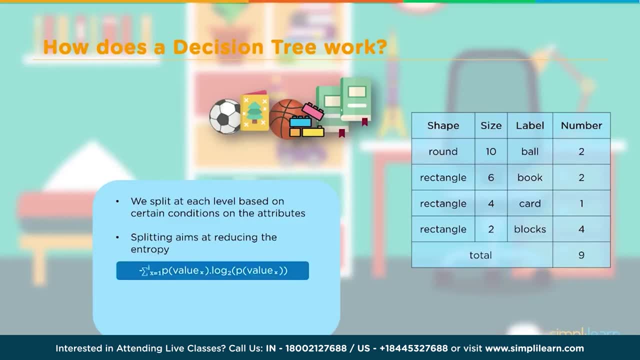 have a formula. our first actual formula that you'll see happens in the background when we're running these different modules in R And it looks a little complicated. but we can break that up and simplify that for you. So we see this formula: the negative sum of i of x equals the probability of one value of x times the log of two. probability value of x, The term probability value of x. it's probably easiest to understand if we go ahead and put the numbers in there so you can actually see what we're looking at, And so we plug the numbers in there we look at: 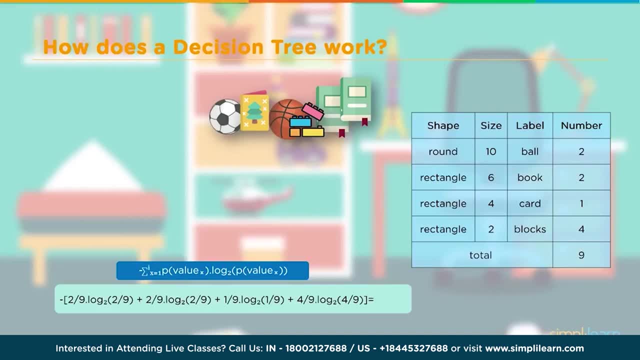 the probability of the value of x. Well, if we do the number of balls, there's two balls and the total number of items is nine. So we have a probability of any one object being two out of nine. So that's pretty straightforward math. when you look at the numbers, you can actually see that very easily, And so we can calculate our entropy of two over nine times the squared log of two over nine, plus one ninth, the log squared of one over nine, plus four over nine times the log squared of one over nine. 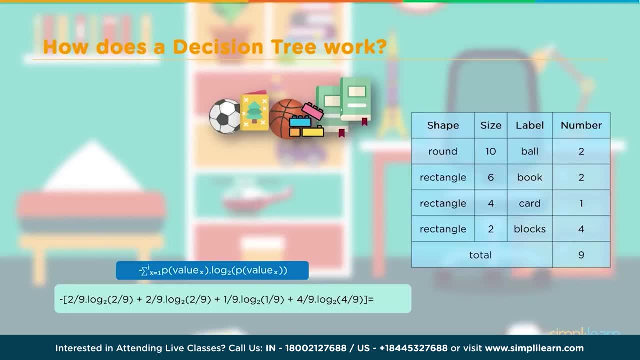 So our whole group is the sum of all the entropies. And so when we look at that, we have the entropy of the balls, which is the two over nine, rectangles two over nine, I mean books two over nine, cards one over nine, and the blocks four over nine, And we can just plug those numbers in there and we get an actual value of 1.8282.. So what the heck does a module do with that number? Well, now we must find the conditions for our split. Every split must give us the maximum of 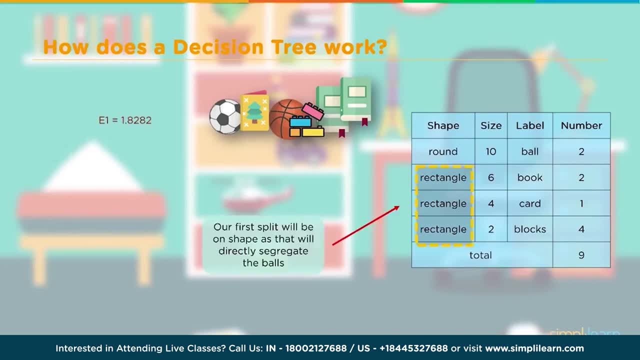 achievable information gain. And so we have our first entropy value: 1.8282.. And it turns out, when you compare all the different individual entropy values for the balls, for the books, for the cards, for the blocks, rectangles, you find out that the biggest split is going to be in the shape. And it's going to be our first split will be on the shape that will directly segregate the balls out, So they'll split up a huge group from one from the other, And so we compute that we end up 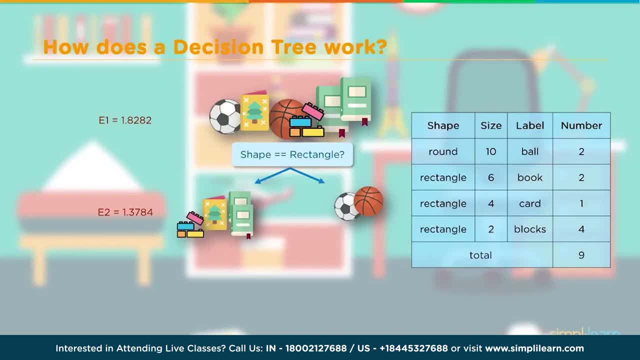 with E2, which is all of our rectangles, And then we have a leaf node which is the balls, And so with our E2, we see that 1.3784 is much less than the 1.8282.. And so our second split will be on the size is that will directly segregate the books, And so when we do that, we can see that if the size is greater than five, all the books go to one side, while the cards and the blocks go to the other, And again we have our E3, which equals 0.716, which is considerably less than 1.3784. 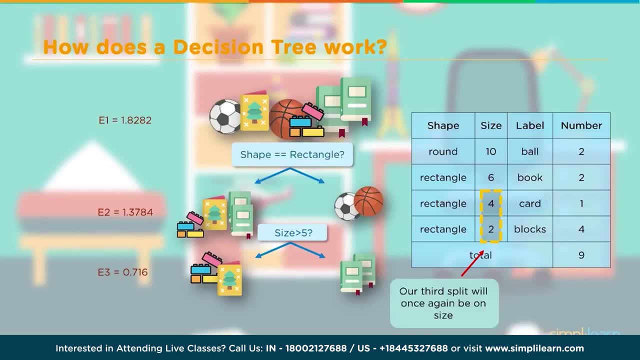 So our entropy is dropping each time we do a split And, of course, our third split. we look at and we'll see that we're left with size again. And we'd split it with four and two In this case. if it's greater than three, it's going to be a block, If it's less than three it's going to be a card, And at this point each of our objects is looped into similarity, So they all look the same And we end up with an entropy of zero. And so you can see, as we go down, the entropy continues to get less And because it hits zero, we can say all our objects 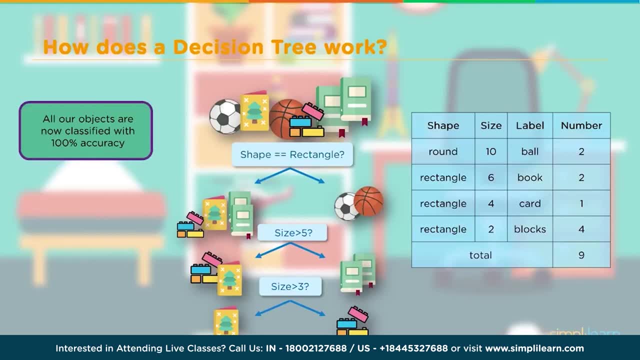 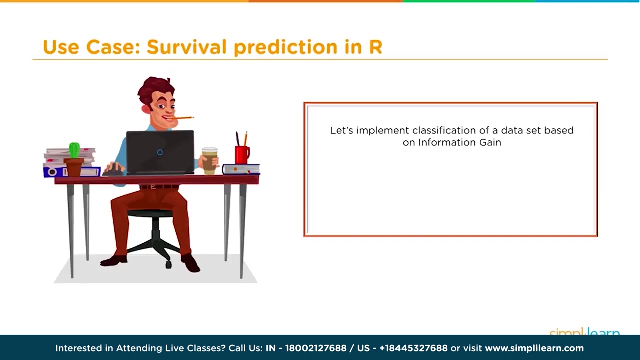 are now classified with 100% accuracy. if it was only that easy to clean the kids' closets And you can see, we have a nice drawing that shows you where all the leaf nodes are on this, in which case we have the balls, the books, the blocks and the cards are part of the leaf node And the root node is our first split, when we have all the objects and we're splitting them by a rectangle, by shape. So we're going to dive into the use case And in this case we're going to get a little morbid. There I am behind my desk. That's definitely not me. I don't have that big of a chin, But I do usually have a. 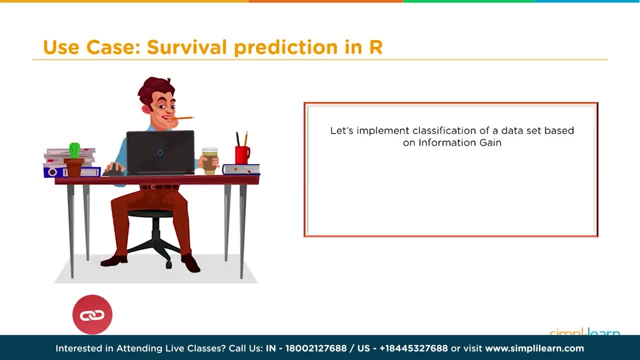 cup of coffee and it looks kind of like that It's sitting next to me on my desk. So the use case is going to be survival prediction in R And let's implement a classification of data set based on information gain. This is going to use the ID3 algorithm. Don't let that scare you. That's the most common algorithm they use to calculate the decision tree. There's a couple different ways they can calculate the entropy, but the formula is all the same behind it. So ID3 is most common in R And then we'll be using the RStudio. 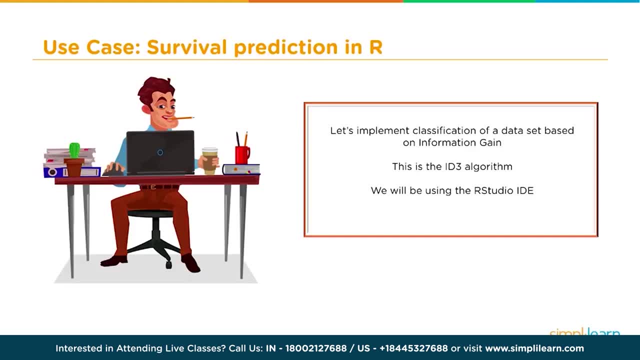 for our interface, for our IDE. So RStudio is free to download. There's the free version. Of course, there's an enterprise version and there's all kinds of different choices in there. But one of the wonderful things about R is that it's been an open source for a very long time and it's very 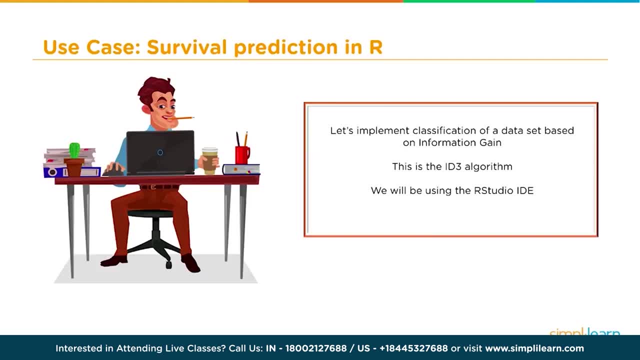 well developed. It's also very quick and easy to use on a lot of things. So this is going to be in the RStudio IDE. There's some other interfaces, but I would suggest using the RStudio. It's the most common one And, if you remember, I said this is going to be a little morbid because we're 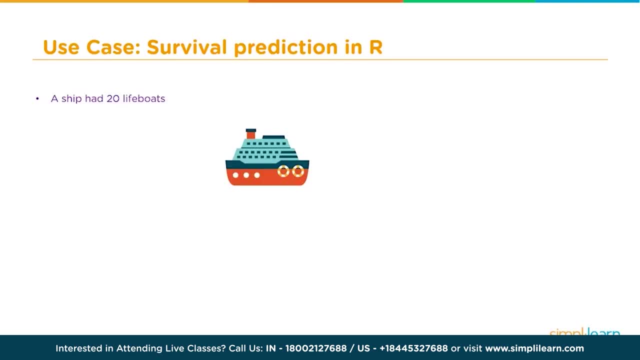 talking about how many people survived and died on these ships. So in this case we have a nice vacation cruise ship going on there. I'm not sure what that is with the tugboat. So we have a ship and it had 20 lifeboats. The lifeboats were distributed based on the class, gender and age. 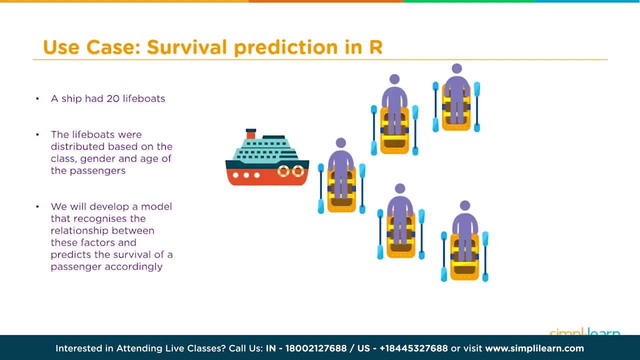 of the passengers. We will develop a model that recognizes the relationship between these factors and predicts the survival of a passenger accordingly. So we want to predict whether the person is going to survive or die in a shipwreck, And we'll be using a data set which. 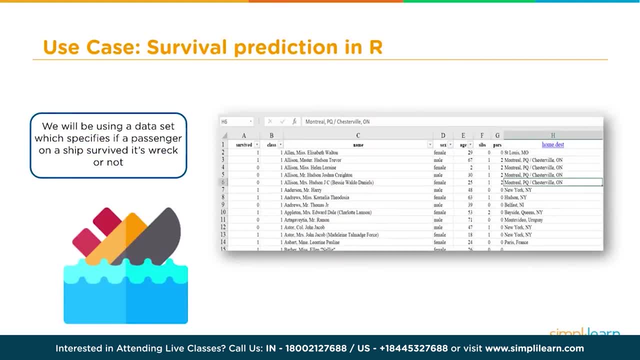 specifies if a passenger on a ship survived its wreck or not. So we're going to look at this data and if you open it up into a spreadsheet- and don't forget- you can always put a note on the YouTube video down below and we will be monitoring that. You can request the data set sent to you or 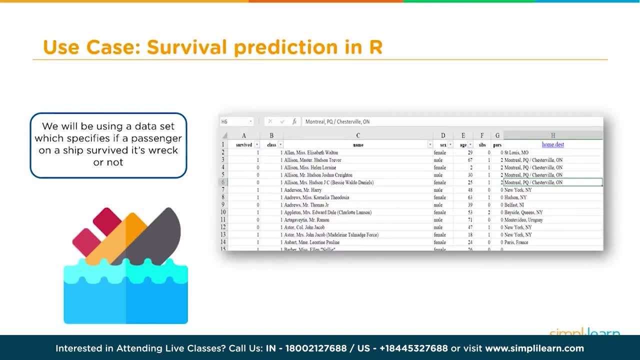 more correspondence. You can also go to wwwsimplylearncom and request this data set too. It's just a simple CSV file. we'll send out And you can see right here: we have survived. So one indicates a person survived the wreck and the other indicates a person survived the wreck. 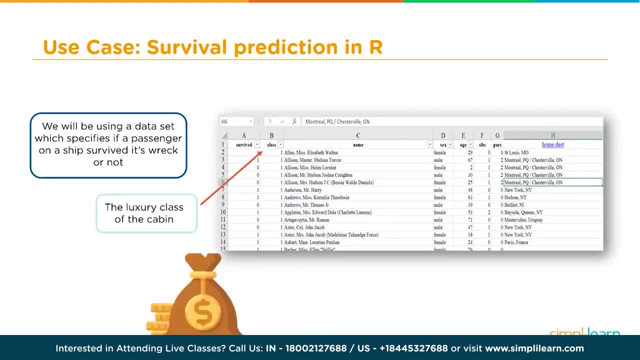 Zero. they didn't make it. They were under the water And the luxury class of the cabin. so if they were in, you know what value is like: 1,, 2,, 3, depending on what luxury class they were. And then we have. 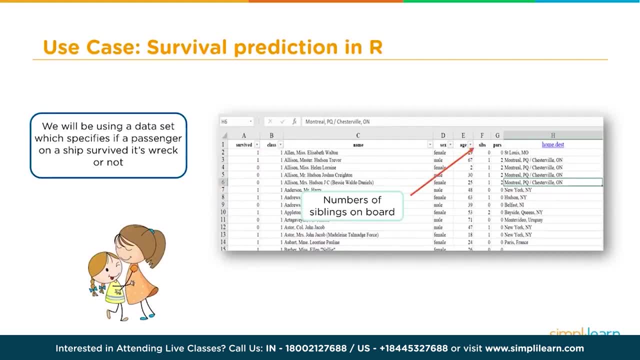 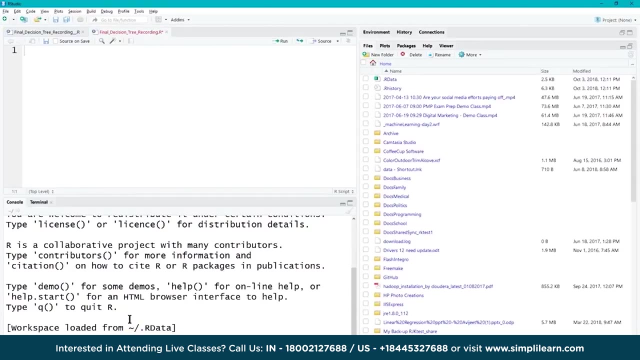 this is kind of interesting how many siblings they had. So it's kind of an interesting added statistic in there: Number of parents on board and disembark location, so where the destination is. So here we've opened up RStudio, and if this is your first time in RStudio you'll notice that it opens up standardly in three panes. So here we've opened up RStudio, and if this is your first time in RStudio, you'll notice that it opens up standardly in three panes. So here we've opened up RStudio, and if this is your first time in RStudio, you'll notice that it opens up standardly in three panes. 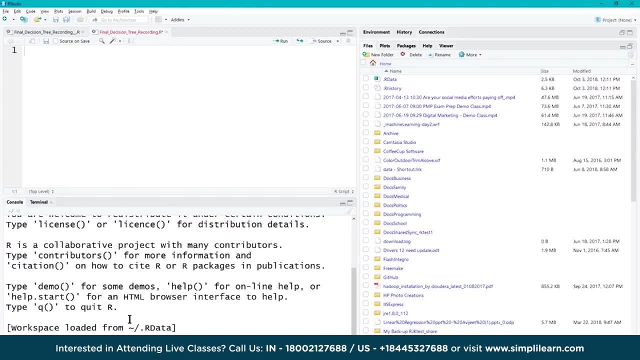 The upper left is for text documents you're bringing in, and then the bottom left is the actual commands as they're processed, And then on the right hand side you have your environment set up on there. Now I've zoomed in with my font a little oversized. In fact, we can even take that up one more size and see if we can get a larger setup view. 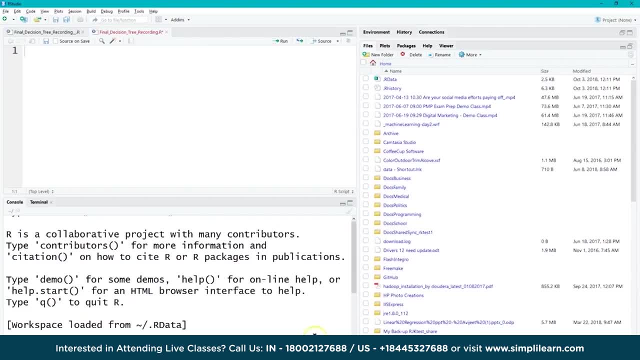 Here we go. So I've set the font for 18, probably a lot larger than you need to work on a project, And the first thing I'm going to do is, on the right hand panel, we're going to be working with plots. 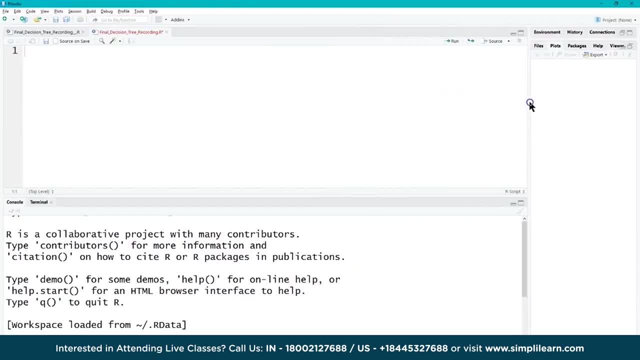 So I'm going to click on the little plot tab up there And I'm just going to collapse that over to the side for right now, And then I'm going to open up the bottom one And you'll see, on the top I actually have two different tabs. 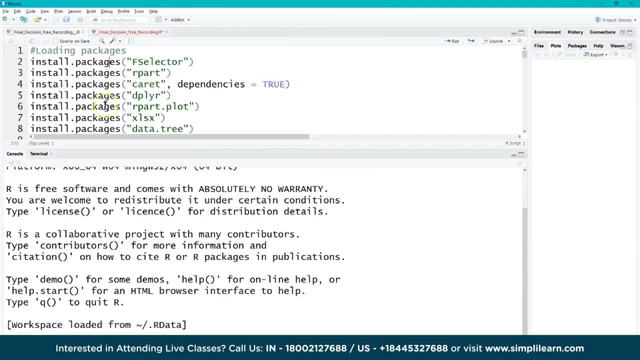 Team in the back was really nice to set up the whole package for what we're working on here, And we'll go through this line by line and then you'll see as we execute. the different lines are going to appear down below, So I'll be flipping between these two left panels. 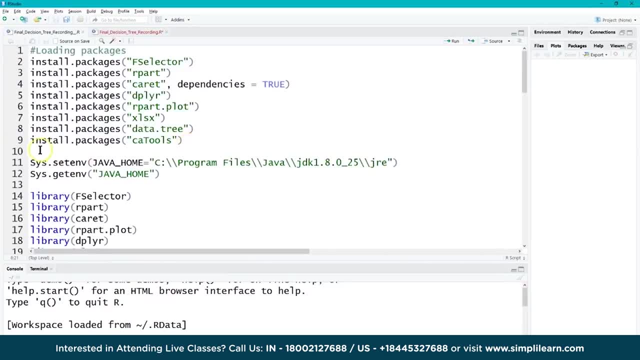 And let me go backwards just for a second here We're going to do this part. So let's take a look at the installs. And if you look at the installs- and I'm not going to actually run the installs because I've already run them on my computer- 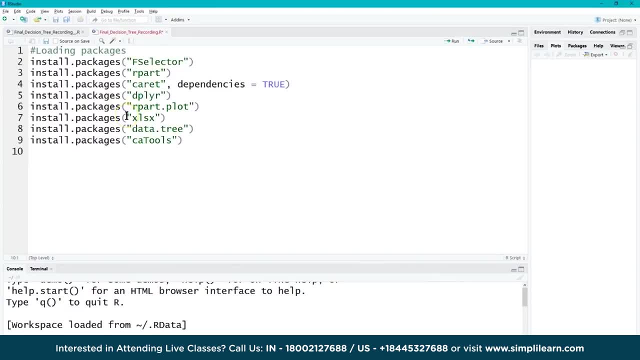 So these are already installed in my R packages and I don't have to rerun them. We have a number of packages we're bringing into R because that's how R functions, And the first number of packages are all part of our decision tree. 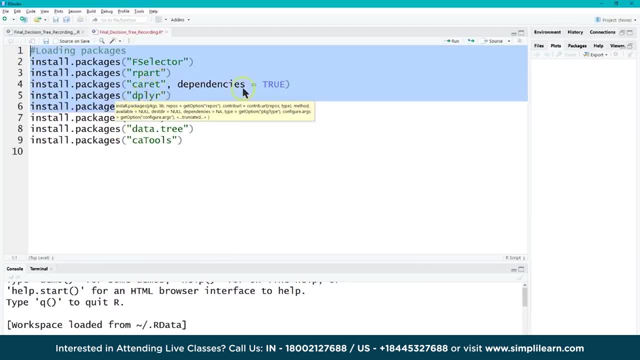 So our F selector, our R part, our caret, with the dependencies, equal, true- and our DPLYR and our R part, plot, Ooh, that's a mouthful. You'll need to import all of those, All of these, in your setup. 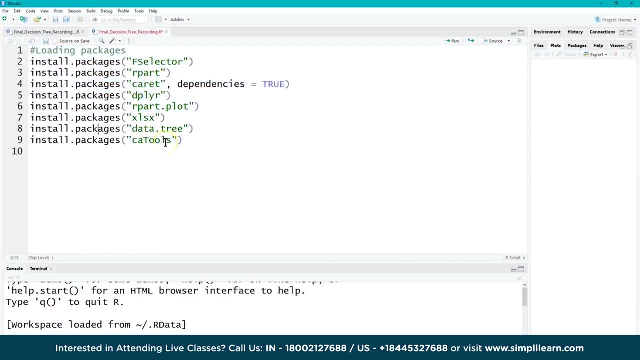 And the first one, which is your F selector, computes your chi, squared your information, gain your entropy. All of those formulas are a part of the F selector, So when you bring it in, that's what that package is. The R part is your partitioning of your decision tree. 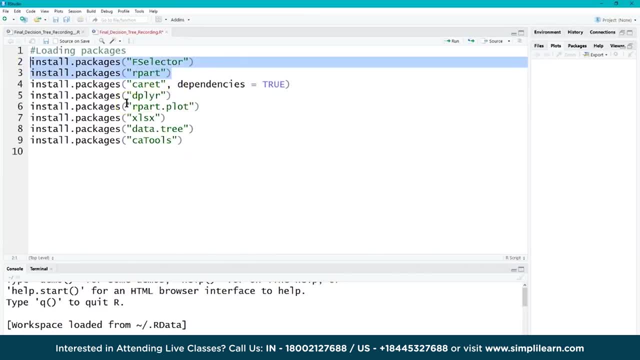 So these are your primary two decision tree modules that we're bringing in. The caret is a part for actually splitting apart the data, because we always want to do a test set, a train set, And then we also package caret to kind of handle all those. 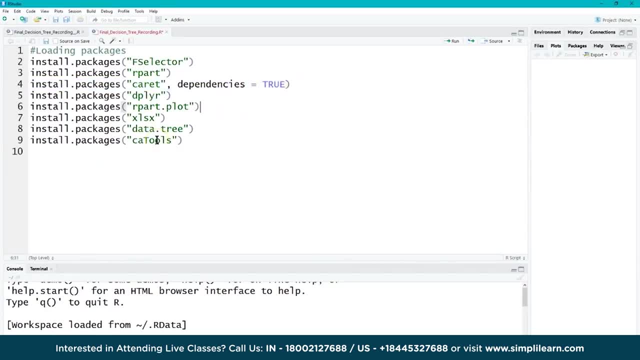 You'll see caret used in a lot of other machine learning packages when you're doing the R. The DPLYR is for mutating your data, so you can sum it, you can classify it, you can filter it. That's all part of the DPLYR. 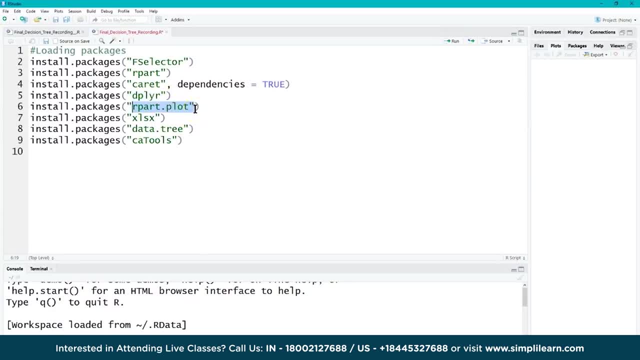 And then R part has another piece called plot, and that's for helping us plot the data as we sort out the tree, Because the R part creates the tree, but you still want to be able to plot it. And then we come down here and we have some additional tools. 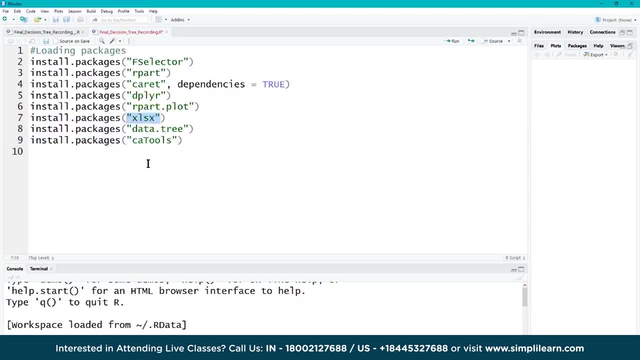 We're going to work with a spreadsheet. This is a Microsoft Access spreadsheet, so we're going to use the XLSX package to import it, And you might think that's a little outdated, because I know when I'm doing any new projects. 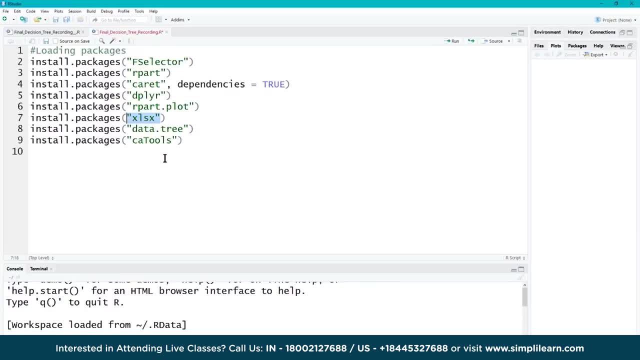 I try to save my data into a comma-separated variable file or something more standardized, But a lot of times you'll end up with these old databases where they're exporting data and their export comes in an Excel spreadsheet And guess what? This is a time saver. 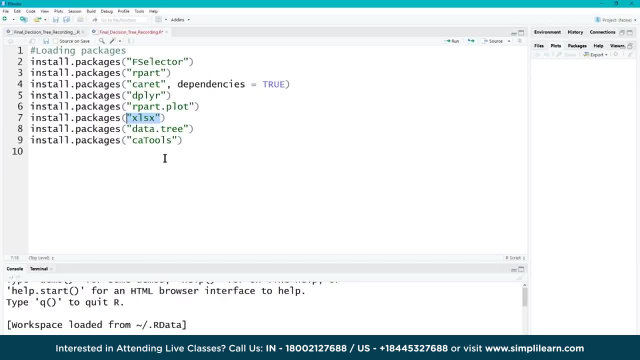 Instead of opening up the spreadsheet, instead of saving it as a comma-separated variable file, you can just open it right up in R, which is really nice. And then we have our data tree, which goes right along with displaying the data. So we have our rpartplot and we're going to put that into the data tree, so we have a nice visual. 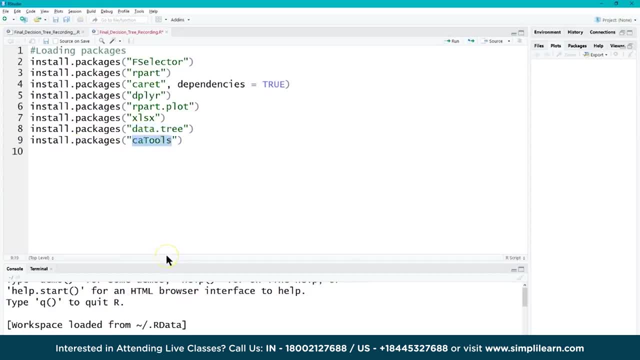 And finally, you need to install the package catools, And catools is another package used for general manipulation of your data and your vectors, So it also has a split function for training data. I know we have another package for that, but both those packages fit in there as far as working with the data. 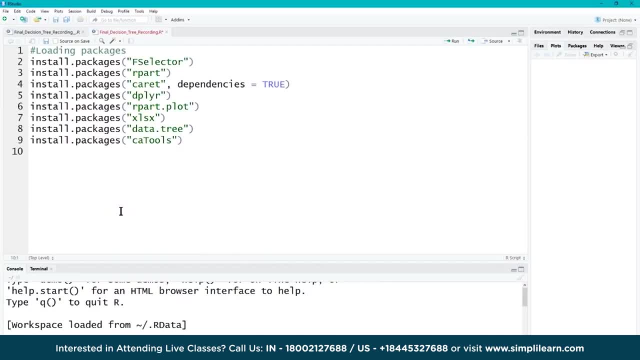 So a lot of times you'll see these loaded in there together And you'll see in a moment we'll import the elementary stat learn package also, which is very generic, working with data setup as far as statistics and data processing. Now, because my Java setup is a little different, because I use a developer package, 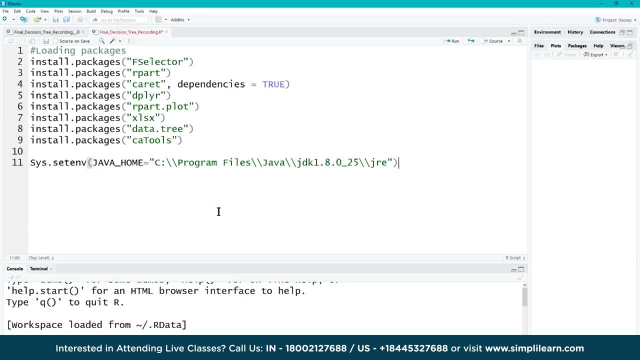 well, the latest update of the developer package and the R are struggling to see each other, So I need to go ahead and add this in. You don't need to worry about this, But if you do get an rjava error, you'll need to go ahead and add in a line to set your environment. 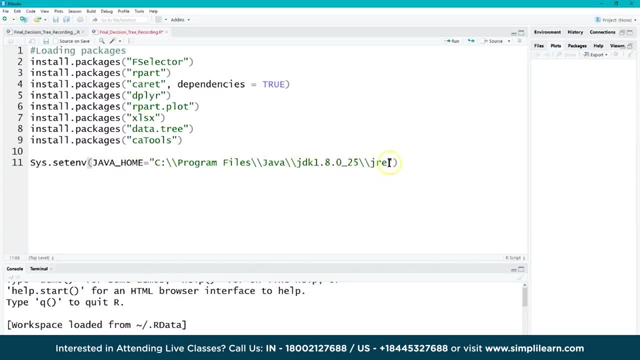 And I'm just going to set the Java home. I went ahead and looked up the last solid JRE folder And you'll see under Program Files, Java. you can look them all up to make sure it's the JRE and not the JDK. 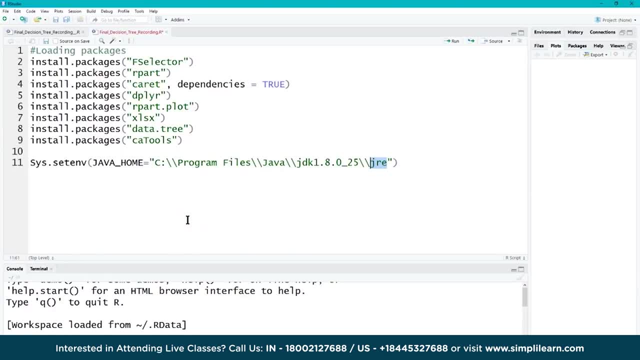 The difference between those is: one is a standard executable. That's a JRE folder. It is a folder, not an actual file, And the JDK deals more with developer side on things. And I'm going to go ahead and run this And if you're in R, you can run these lines individually by holding your control key down and hitting the enter button. 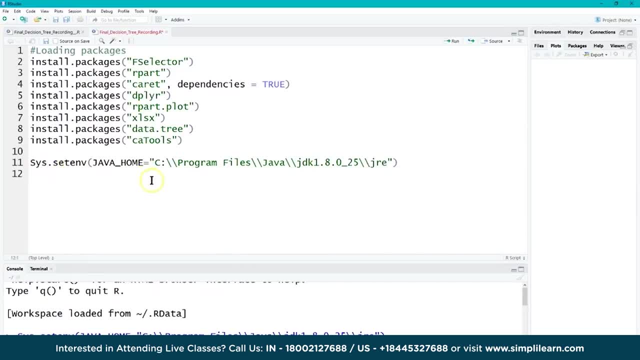 So I've now loaded my workspace and set my environment here And we can actually look and just make sure a systemget environment is the opposite one And I can just look real quick and say, hey, what's my Java home set to? 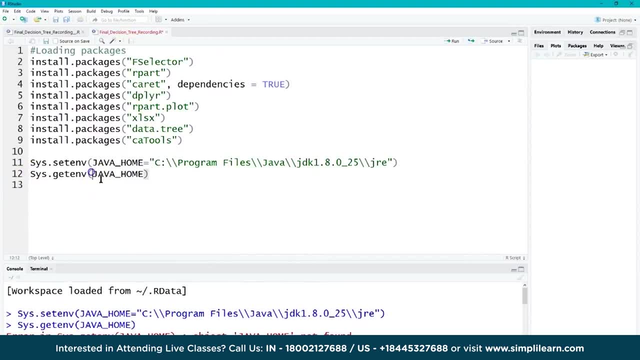 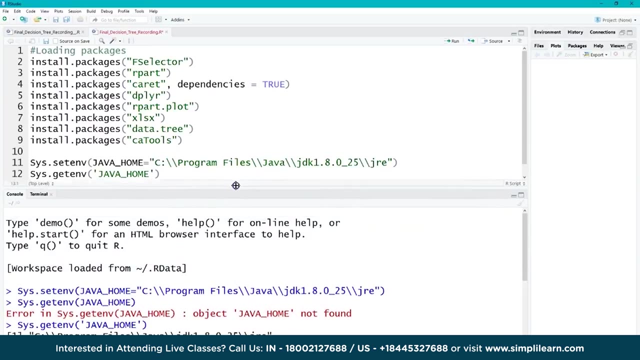 And if I run that- whoops, I forgot to put brackets around it. There we go. And if I do that, you'll see that it's set to the JDK18025.. And again we're looking at the split screen. 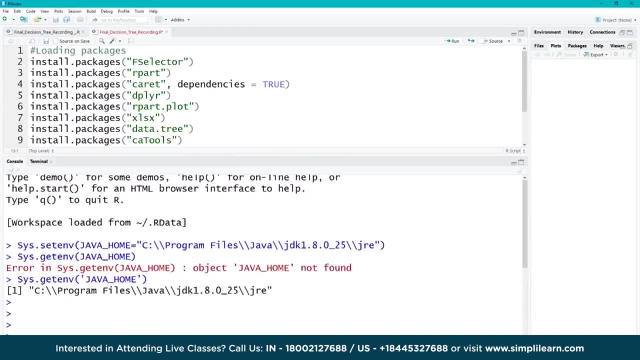 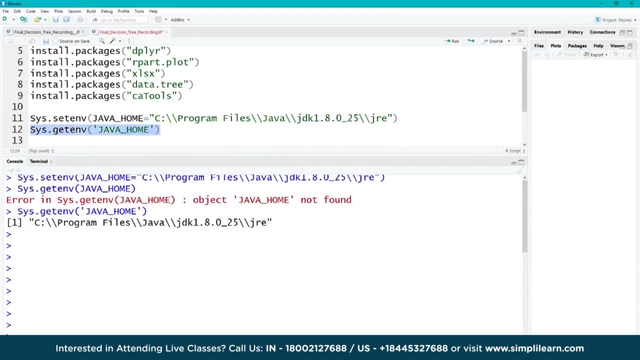 And let me just move this up here a little bit And let me hit the enter key a bunch of times so it comes up on the screen When I run it. and I'm running it line by line. the run text then appears down here. 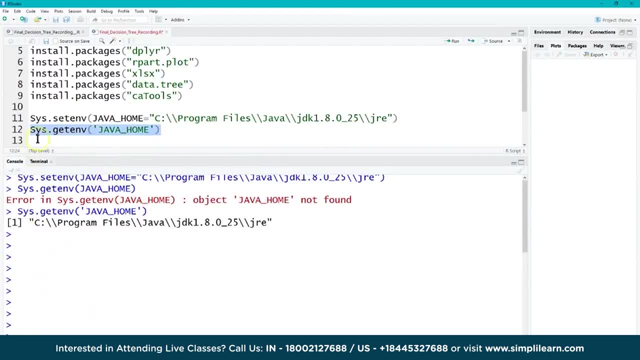 And this is what's actually being executed. So I could just as easily type it in down here as putting it in the JRE folder, As putting it up here on the top part, And that's just a little bit of RStudio and working with RStudio. 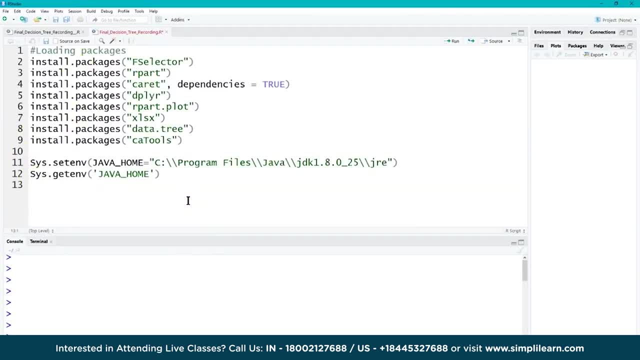 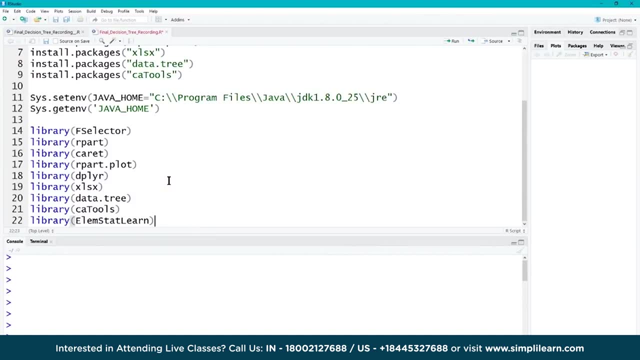 So I've shown you the installs And again, I've already installed it on my computer, so it takes a minute or two to install it. You need to go ahead and then bring those libraries in to work with. So basically we're going through all the different libraries we're using. 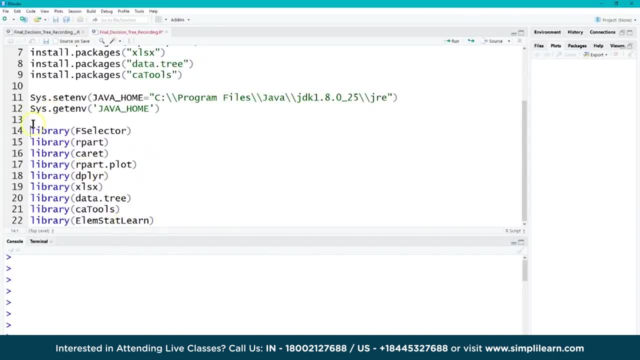 Elementslearn is a standard R library, so it should already be installed. You don't have to install that one, And I can just go right down them And you'll see, as I install them, that they show up on the bottom, And every time you go to run a new setup you need to go ahead and install these. 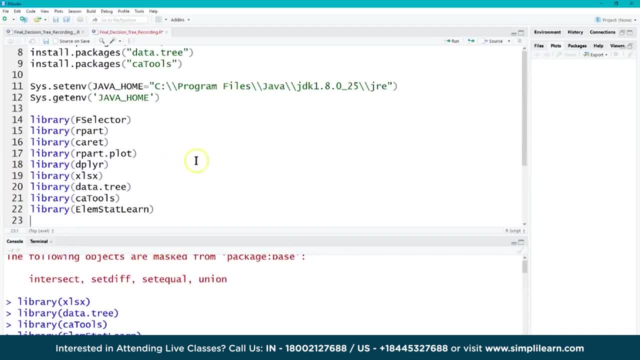 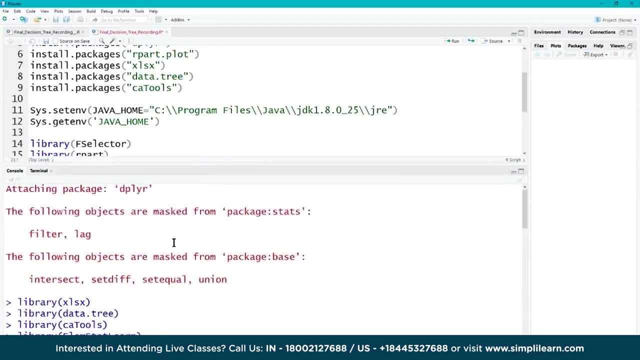 Pull the libraries in. You've got to tell your RStudio these are the libraries you're using And you can see right down here that as it executes them, it has all the different things. One of them had like a couple different parts to it. 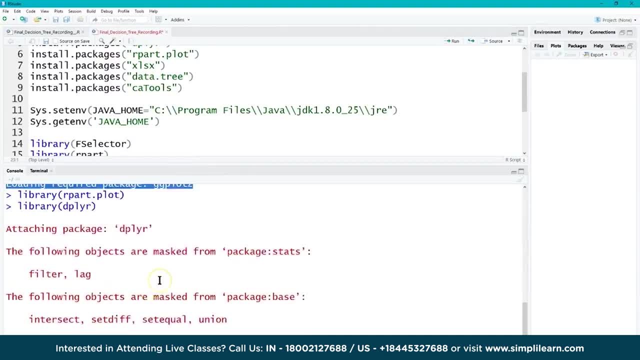 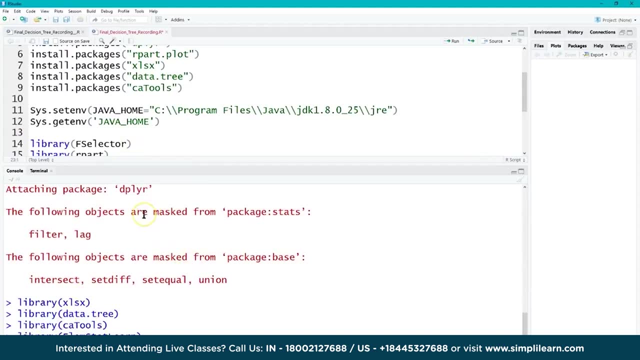 So it loaded the lattice and the ggplot2.. Really, nothing to worry too much unless you see errors down here. So if you start getting error codes then you might have to go troubleshoot and find out why it's not installing correctly. or did it install correctly? 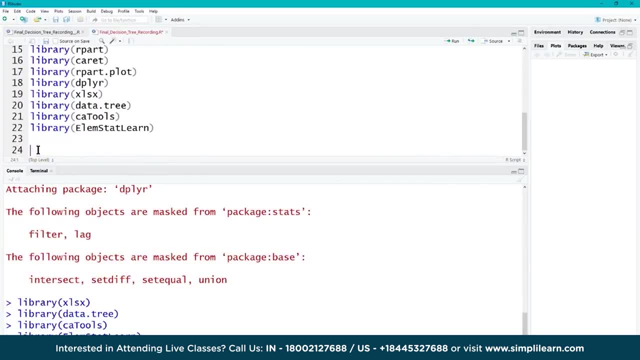 But it's pretty straightforward. We've covered all the libraries And again, if you want a copy of this code, simply let a comment down below on the YouTube video Or visit wwwsimplylearncom and they'll be happy to send you a copy of the base code. 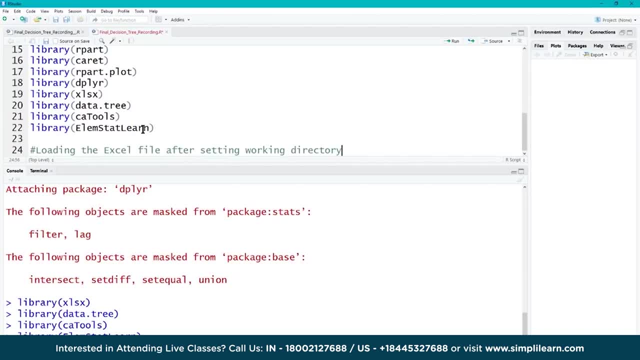 The next step is: we want to go ahead and load the Excel file after setting the working directory. So let's go ahead and set the working directory. SEWWD is the command for that in R. And then this is wherever you have downloaded your data to and your files to: 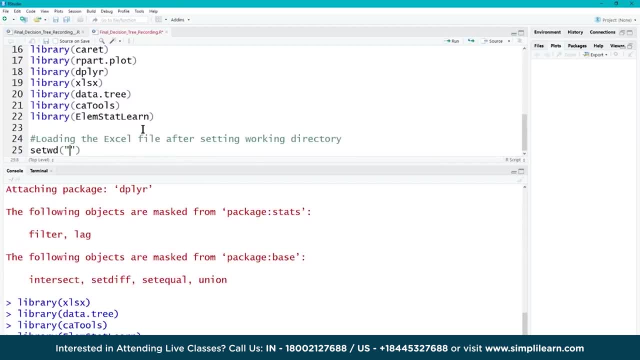 A lot of times, if you get the zipped framework sent to you, it will unzip all into one location And then you've got to look that location up and put that in here. A lot of times it automatically sets that for you if you're working in the same directory. 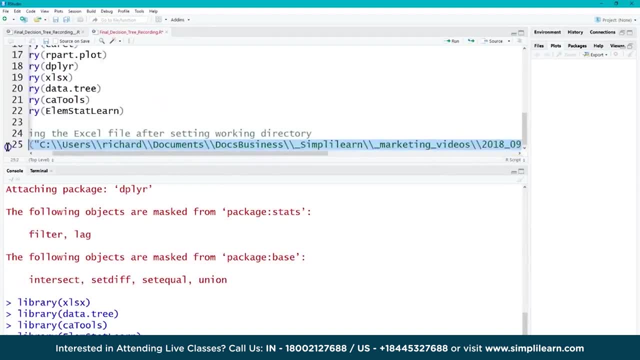 In this case you can see I've pasted in a very lengthy path because I have this as part of my documents, my business docs and Simply Learn and marketing videos and so on, And I'll go ahead and do the Control-Enter and run that. 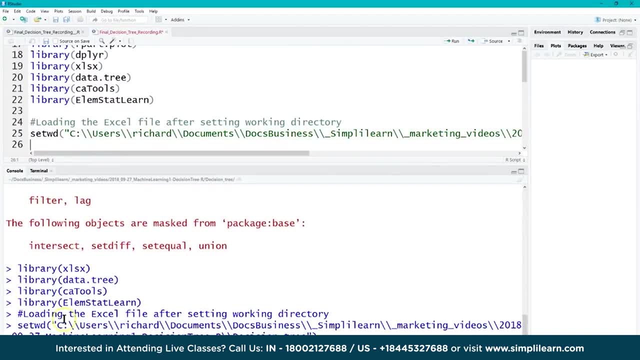 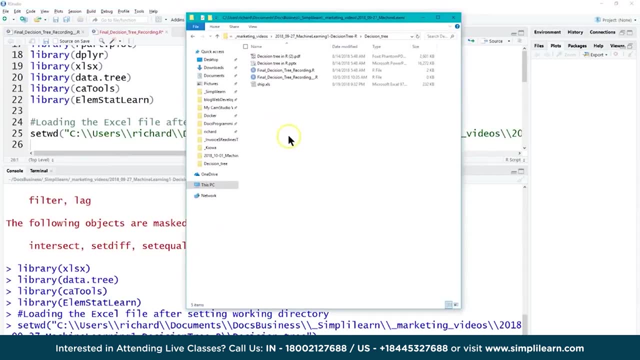 So now my working directory is set And you can see down below it's executed this on the console down here And if I open up that working directory you can see it's running. And in the working directory you can see I have a SHIPxls file. 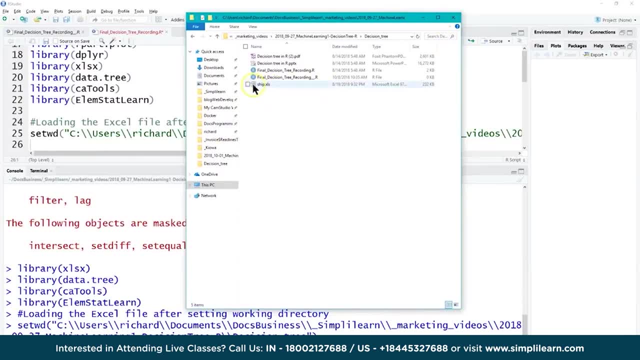 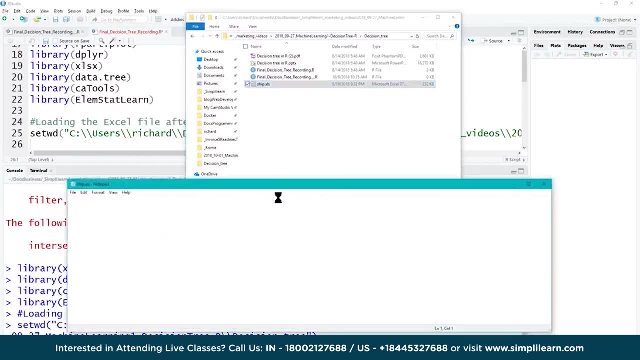 That's the data we're going to look at And we looked at that on the slide. You could also open this up, And I want to go ahead and open it up with a notepad. By default, it will open up as a spreadsheet. 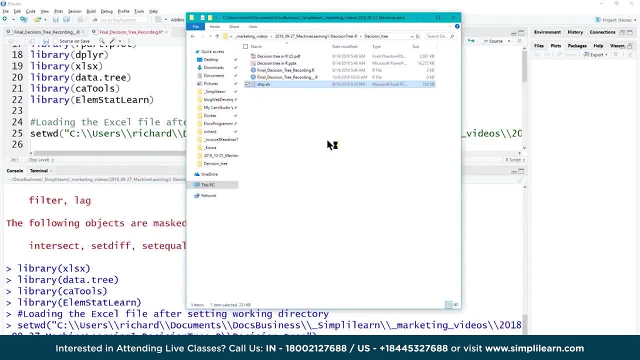 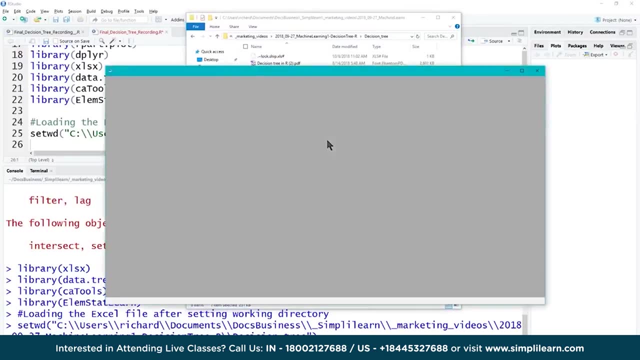 Oh, it is an Excel file, so I would have to open it up as an actual spreadsheet. Wasn't thinking that one through. This is one of the problems with saving stuff as a proprietary SHIP file, even as something as widely used as Microsoft. 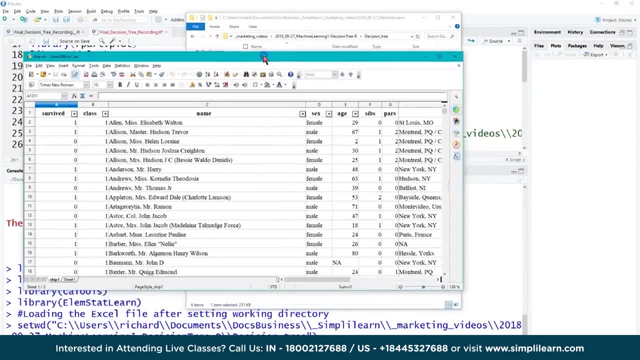 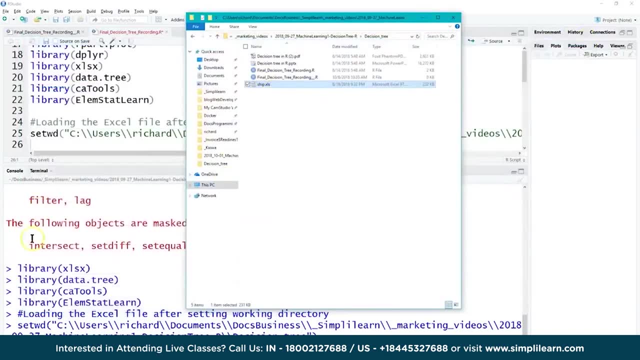 Excel spreadsheet. But when we open up the spreadsheet you can see here the same data we looked at before. This was coming up in this file, And so I take this file. We can go ahead and let's create a variable. We'll call it add. 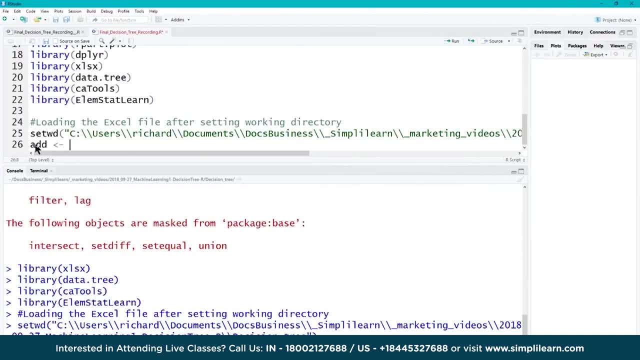 And we're going to assign it- That's what the lesser than dash means, if you've never used R before- And we're just going to assign it a SHIPxls, And then I'll do my Control-Enter And you'll see it run down here. 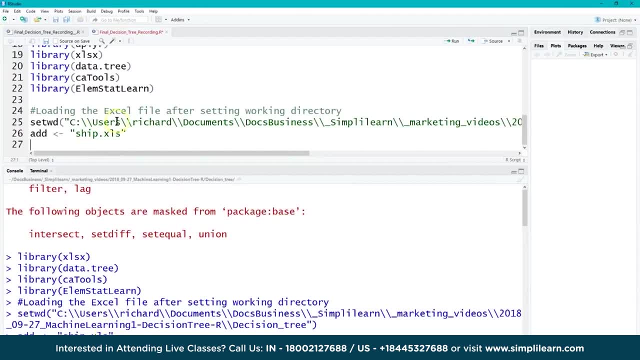 SHIP Add is assigned SHIPxls- Our Excel spreadsheet on there. And then let's have another variable. We'll call it df for data frame And we're going to assign this readxlsx. And that's from the library slxx that we just imported. 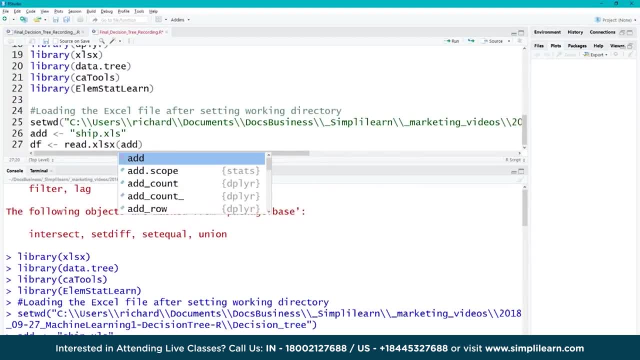 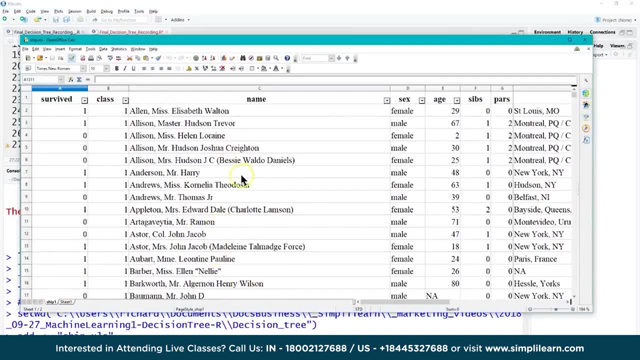 And we want to read the file add, Because we just created that variable with the SHIPxls And I didn't catch this right away. But you'll see when we open it up in a spreadsheet It might be hard to see in your video screen. 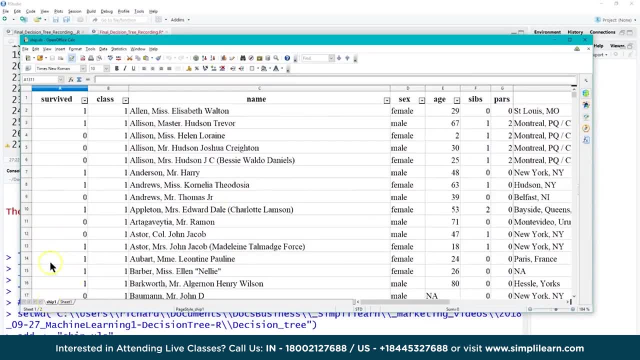 The first sheet is called SHIP1.. So this data is on the page SHIP1 in the Excel spreadsheet And we've got to make sure that we tell the reader to look for that, And so we can simply do that in our command line. 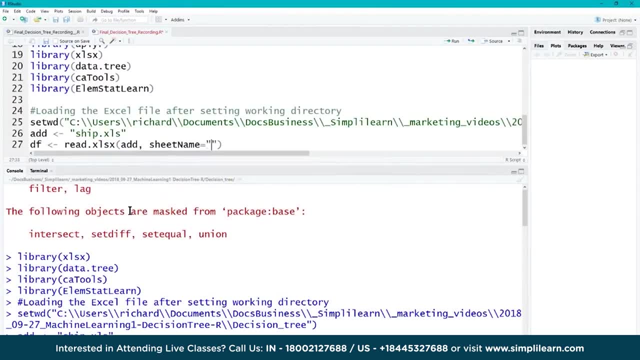 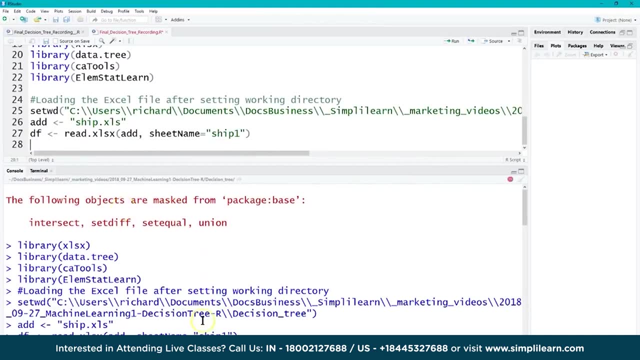 Sheet name equals And it was SHIP1 on there. So we go ahead and hit the control, enter and run this line And it brings it down below and executes it. It's now reading in that data from that spreadsheet. That's what's going on. 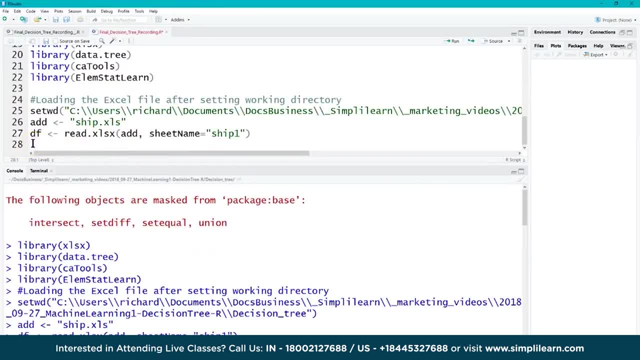 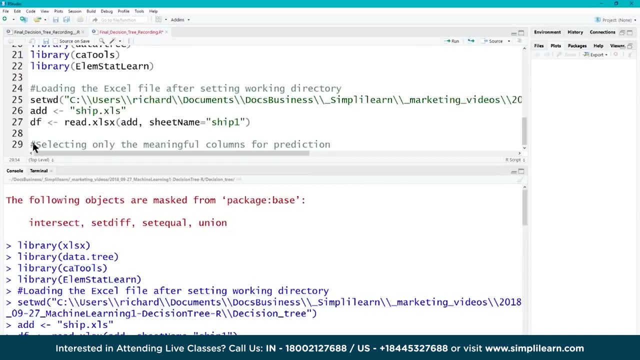 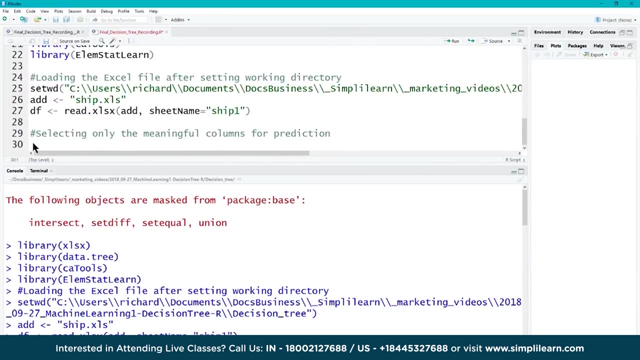 And it takes it just a moment to go ahead and read it in, And then with any data processing, We need to select the meaningful columns for the prediction. So this is important: that we sort through our data And set it correctly so that whatever we're feeding it into can read it correctly. 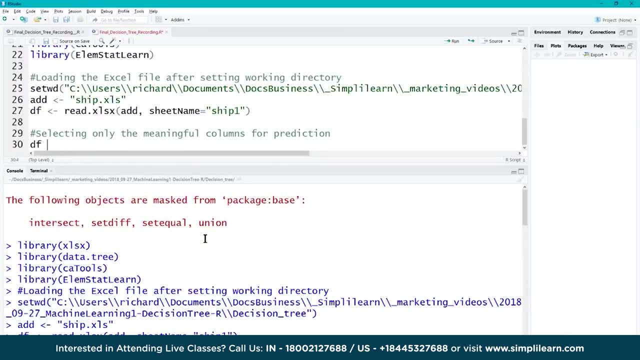 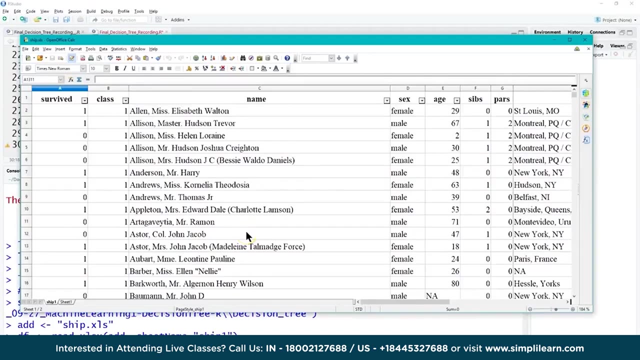 We can do this with DF. We're going to reassign it And we're going to select, And from there we're going to select DF as our main data frame going in And then list the columns that we want. And if we look at the data, 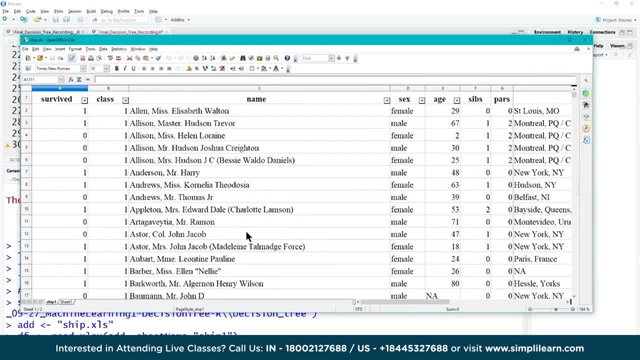 We have survived. We have a class, We have a name, Sex and age, And then there's siblings and parents. We really don't want to know the name, Because we don't need the name to write, Because we don't need the name to run this on here. 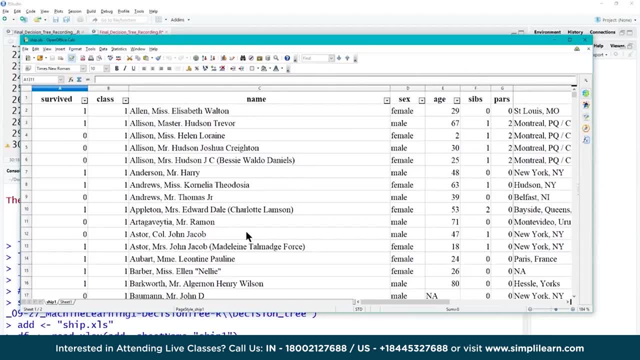 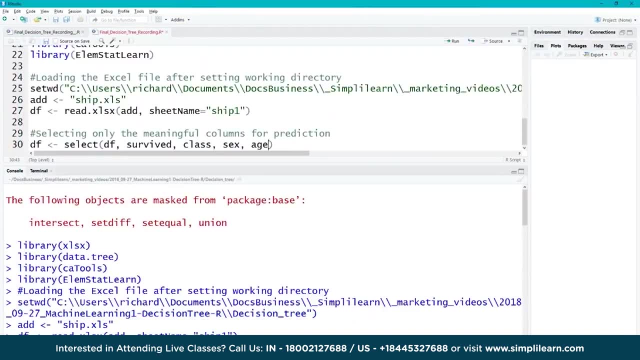 And then we've got to decide which one of these we want to work with, And the guys in the back played with the data a little bit And they came up with the following columns: Survived, Which we need definitely, Because that's what we're actually trying to figure out is whether we're going to survive or not. 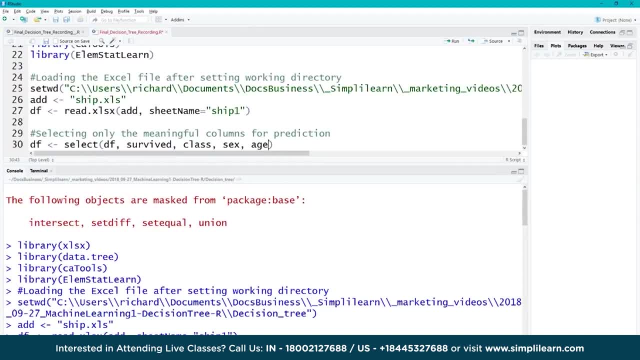 What class, Which class of the boat they're riding in Their first class, Second class, Sex and age, And we went ahead and dropped the rest of them, At least for this example, And then go ahead and do my control enter. 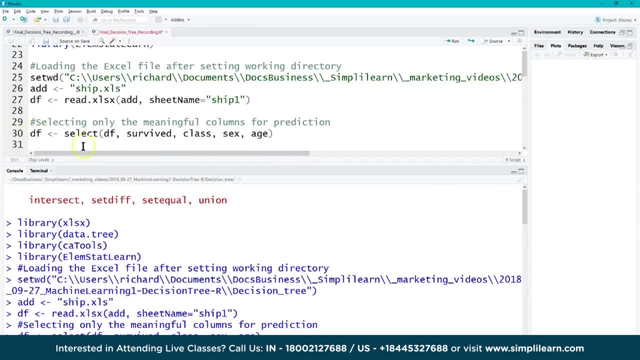 And you'll see it execute down below. And now, df equals these three columns Or four columns Plus. our answer is one of those. So I always think of it as three columns plus one, But it is four columns. And then for the next step, 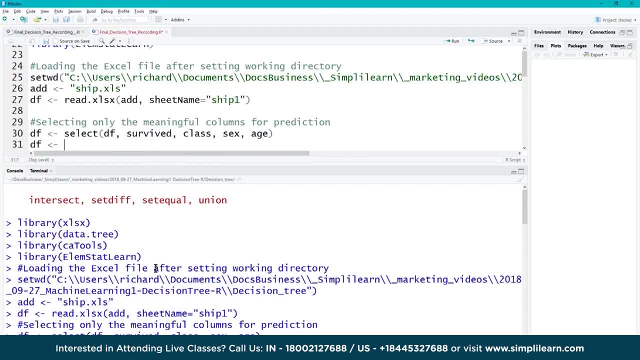 We want to make sure the data is in the right format. So again, I'm going to resign the df And we're going to mutate the data, And that means we're going to take each one of these columns And we're going to let it know what kind of data that is. 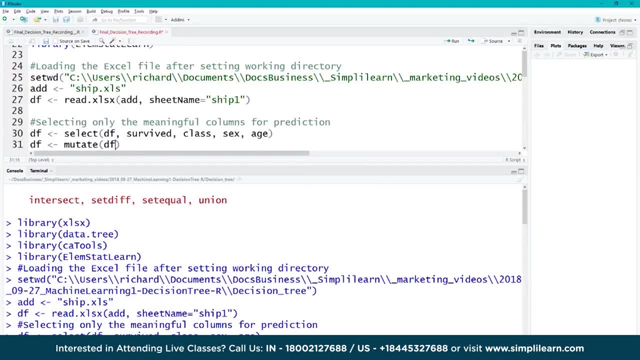 So our first one is: I'm going to put the database in, Or the data frame in there, Df, And then we want to go ahead and do: survived equals a factor of survived. So this is a yes. no, It's letting us know that this is a zero or a one on here. 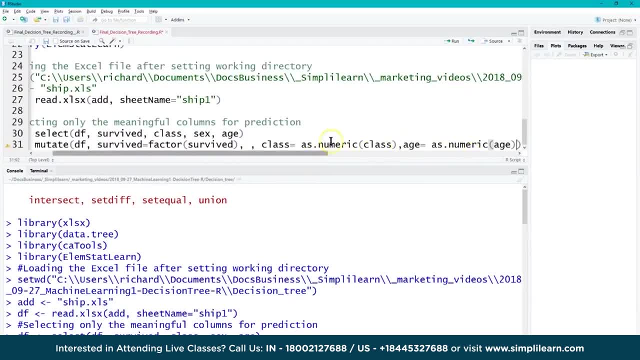 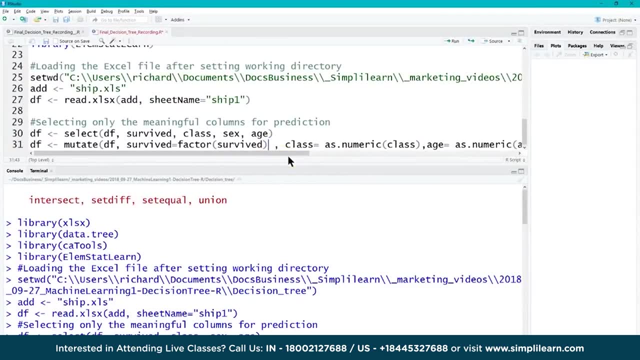 And then for the class and the age, Those are as numeric. There are other ways to process class, Since it is a very restricted number on there, But for this we're just going to do it as a numeric value. Same thing with age. 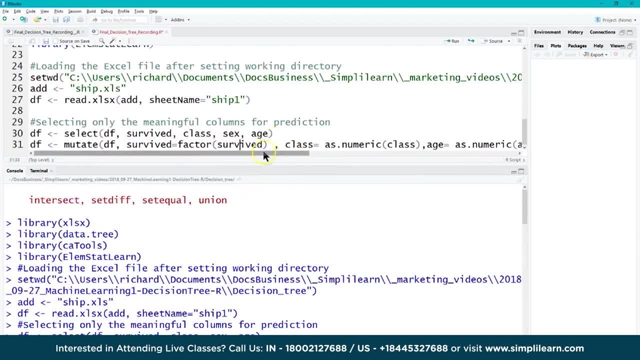 And you see, we didn't do anything with sex. We're just going to leave that as male or female, And that's fine for this, Because it will pick up on that when we run the decision tree And we'll do our control enter. 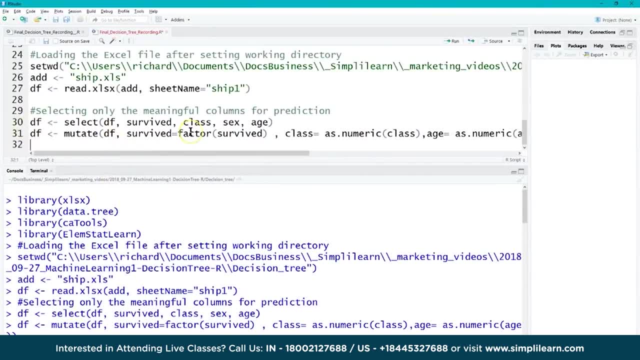 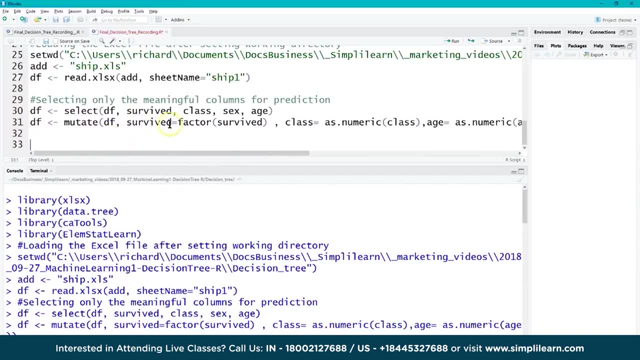 So now I've assigned the new df And you can see it comes down below As we run it on there. So this is now loaded And df now is a mutated data frame that we started with And we've set it up with our specific columns. 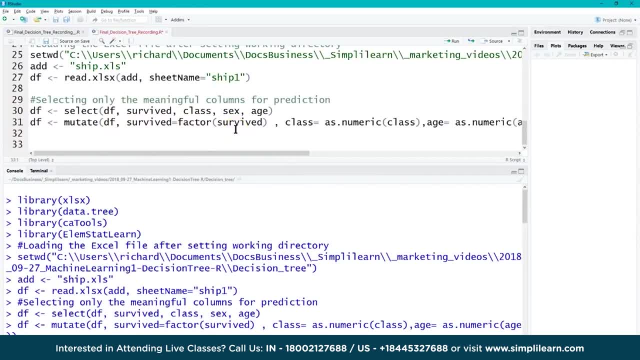 We want to work with, In this case survived class, sex and age. And we've formatted three of those columns to a new setup, So one of them is factor. That's what we use for survive. So it knows it's a zero and one. 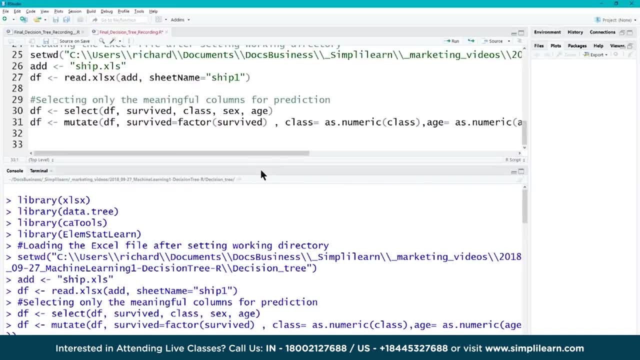 And then we switched class and age to make sure that it knows that those are numeric values. Now that we have our data formatted, We need to go ahead and split the data into a training and testing data set And by now, if you've done any of our other machine learning tutorials, 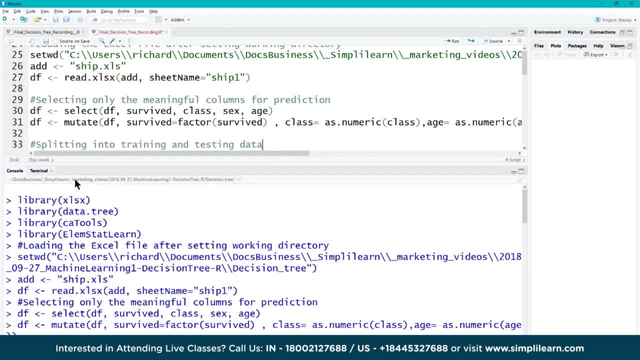 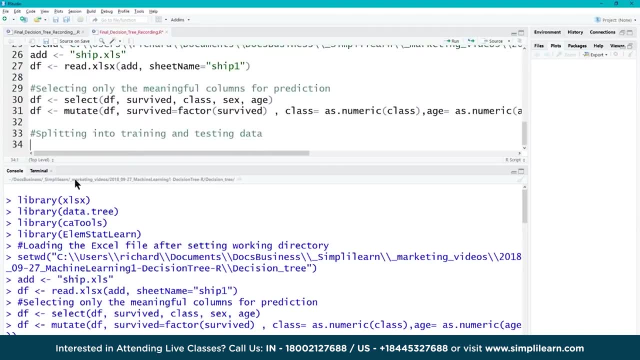 You know this is standard. You need to have your data that we train it with, And then you've got to make sure it works on data that it hasn't trained on. So we'll go ahead and do the splitting. Let's take a look and see what that looks like. 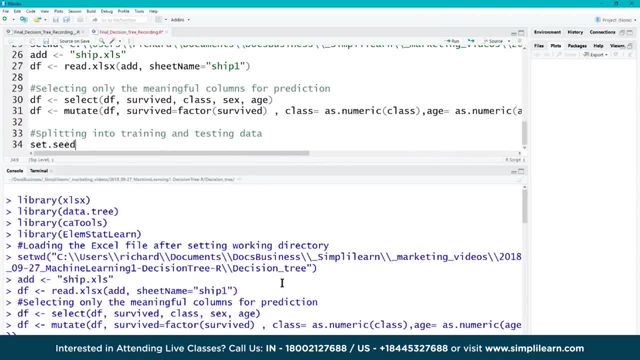 And when you're dealing with splitting the data, We're doing a little randomness, So we'll just go ahead and set the seed to 123.. You can set that to whatever number you want. That's just setting the random variable seed And we'll go ahead and hit enter on there. 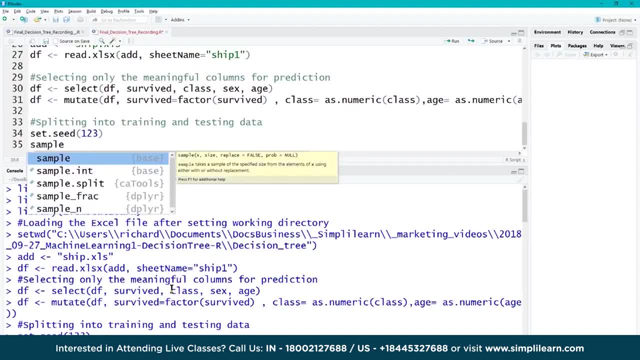 And to do this, we're going to create sample And we're going to go equals Sample dot split. So we're splitting up the data. This is actually creating a whole new column- Trues and falses- And it's all stored in sample. 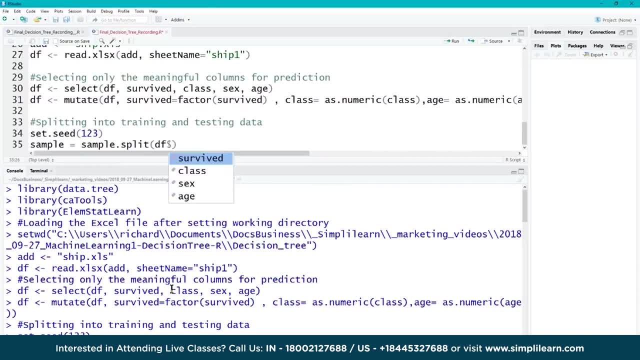 And we want our data frame And we use a dollar sign to denote That we're going to be working with One of the different columns. A nice thing you can do in R And it actually shows my survived, So DF survived. 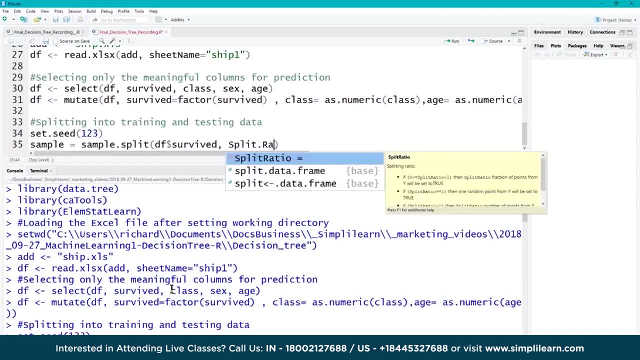 And then our split Ratio. split ratio- I want to add a period in there Which it doesn't have. Our split ratio is going to be equal to, And we'll do 0.70.. So we're going to take 70% of the data. 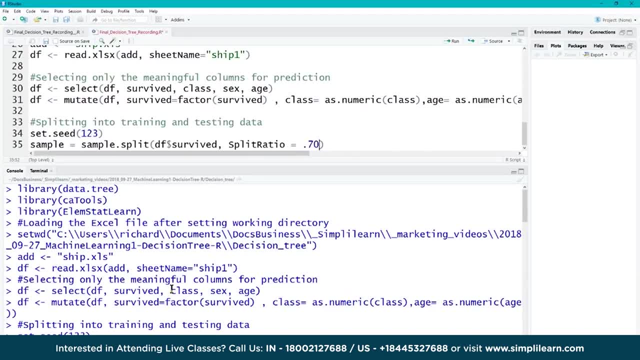 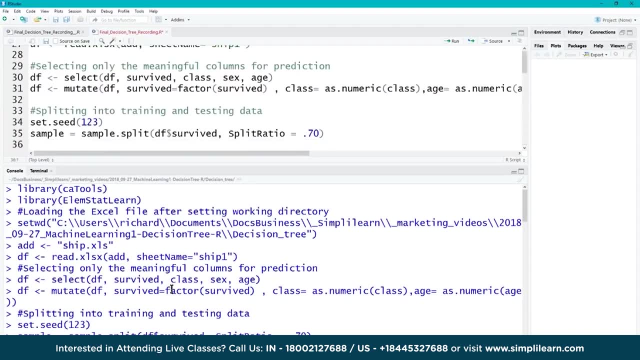 Of those that have survived And we're going to just randomly select Which one of those we're going to use for training And which one we're going to use For testing it out later And we'll hit our enter And load that sample in there. 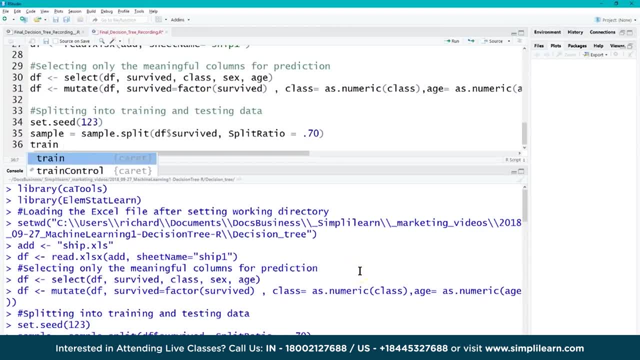 And then we'll go ahead And create our train and our test data sets. I'm going to set train equal to- And this is where it kind of gets interesting, Because we're going to do subset And then we're going to do: 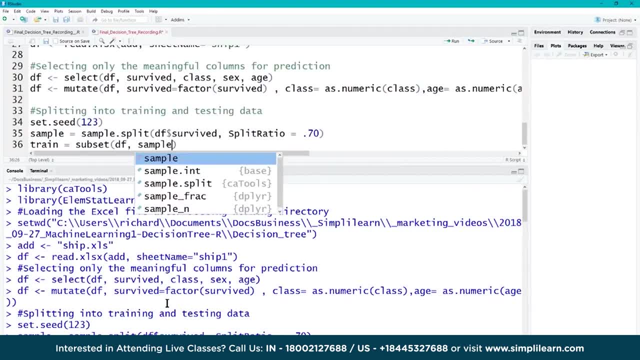 A subset of our DF Where sample, And then we're going to use equals, Since this is a logic gate. So wherever it says sample equal to true, We're going to use that line in DF, And this is, of course, R. 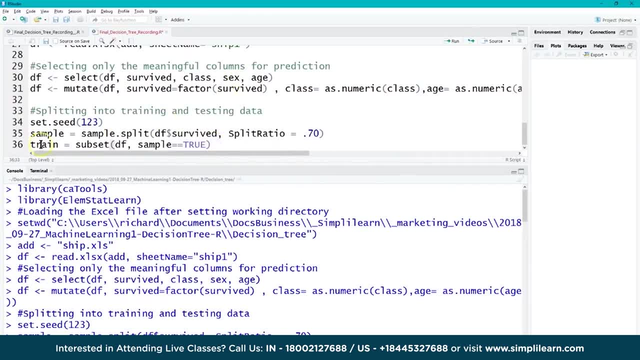 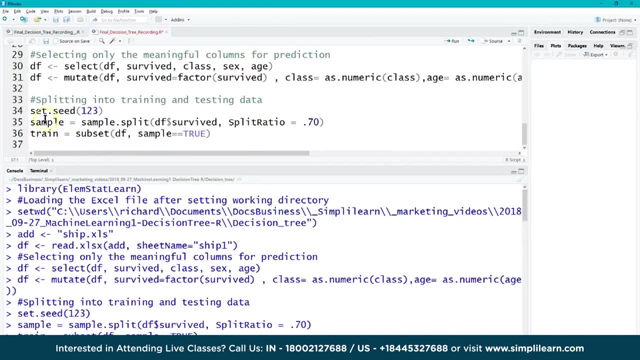 So it's all capitalized And we're going to use true. So here's our train data frame we're creating. So when I execute this And it shows up down below, It goes up and says: hey, this sample Created a whole bunch of trues and false. 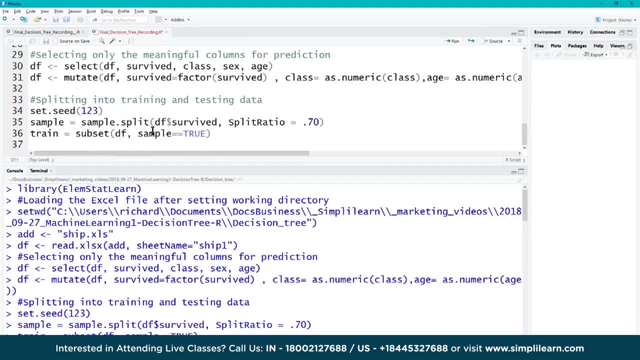 And we're going to take those trues and falses And wherever we've created a true, Which is 70% of the data randomly selected, That's what we're going to train the data with, And then we need our test set. 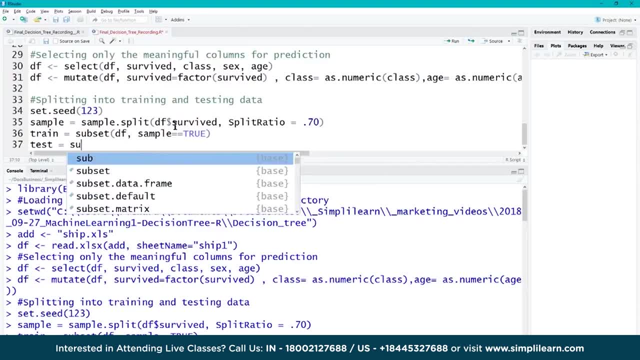 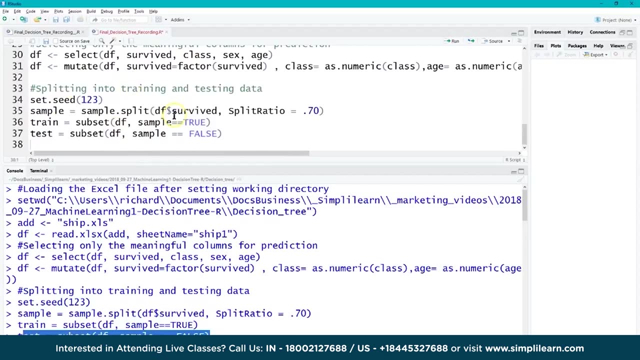 And that's a subset, Just the same thing we just did. And we need our data frame Where the sample equals False. And again, when I hit control enter, It goes down this line of code And it runs it down here in our terminal window. 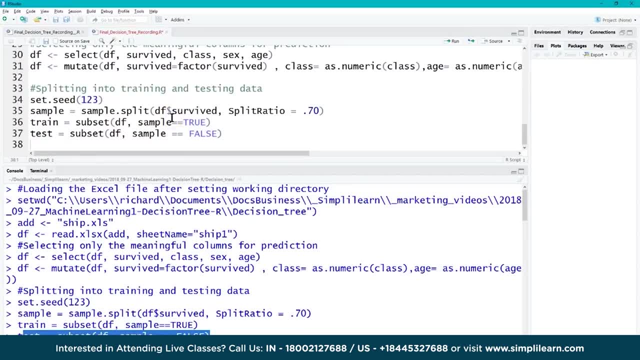 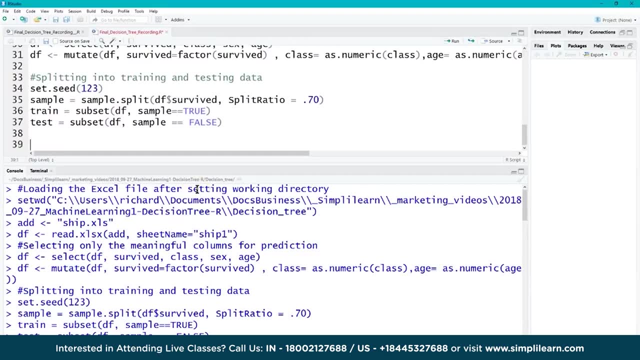 So now we've nicely split our data. We have our training data set And our test data set, And this is, of course, where we get to the point Of what we're actually trying to do, Which is create our decision tree, And we're going to do that by training the decision tree. 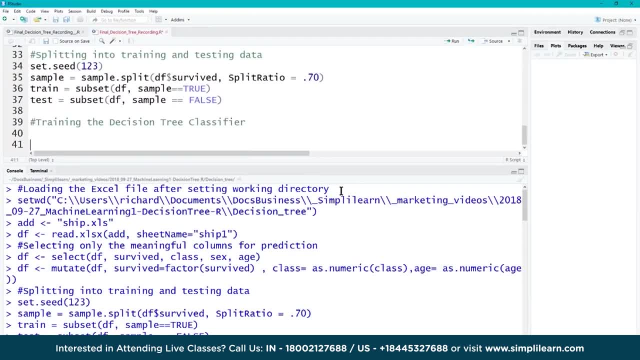 As a classifier. This always gets me. You spend all this work Sorting through the data, Reformatting it- In this case, mutating it- And filtering it, And creating a train set And a test set. So we're going to go ahead and create our tree. 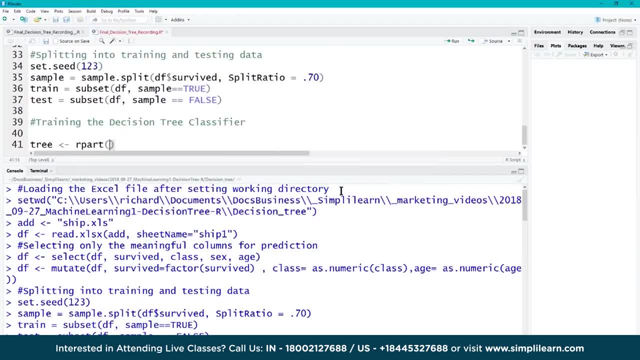 And we're going to assign to it The R part. That's the module we imported, And for the R part We need to go ahead And do what's called a survived, And this is kind of a little complicated to look at. 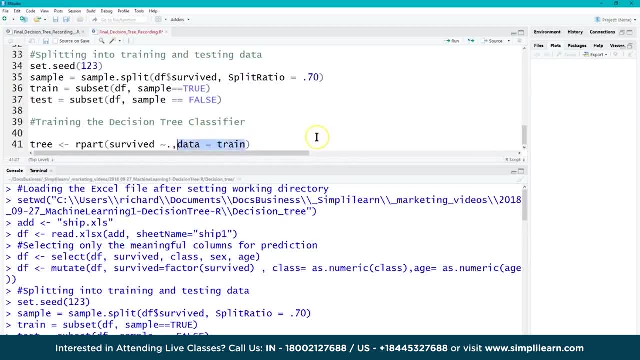 So let's just take a quick look at this. So the R part Is we're importing the data, So data equals train, And then what we want to know is: who survived? So the first part we put in here Is the column we're looking for is survived. 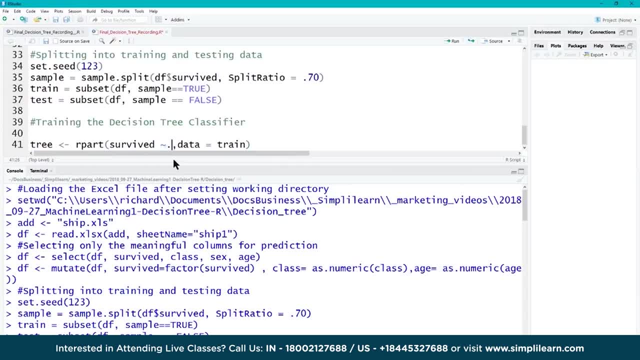 And you'll see that we have Out of the squiggly mark in the period, Because we're looking just for this prediction. We just want to know who survived On these boats For programming our decision tree, And I'll go ahead and hit control enter. 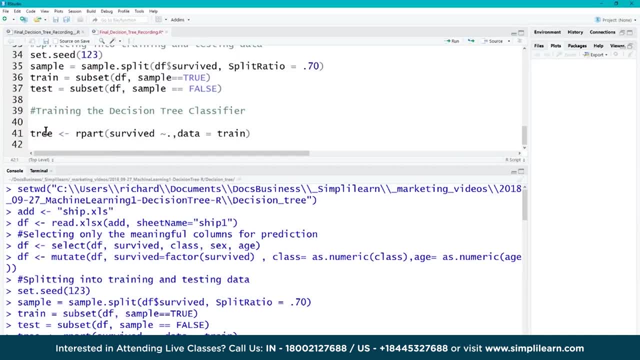 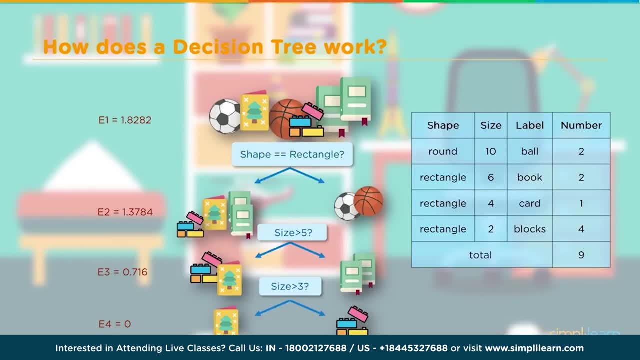 And we've now created the tree. That tree With all those values is now in there And if you remember, from before, We've taken, from when we did, the closet Full of clutter. We've done the same thing Where we have our entropy. 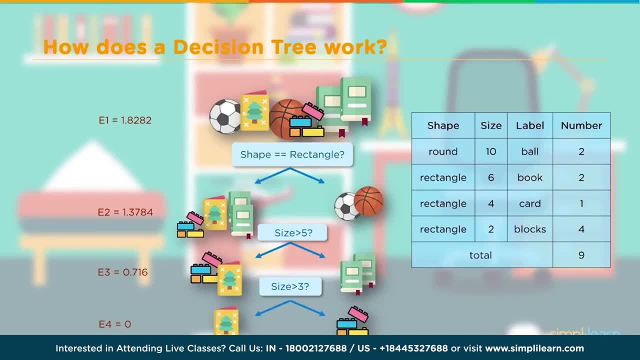 And that one line computes the entropy And the increase in information And it brings the entropy down to zero. So it's the same thing, But instead of applying it here, as we did visually To the closet, It's now applied it to the data on the ship. 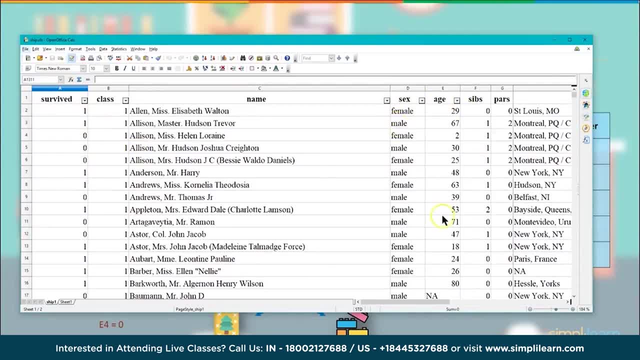 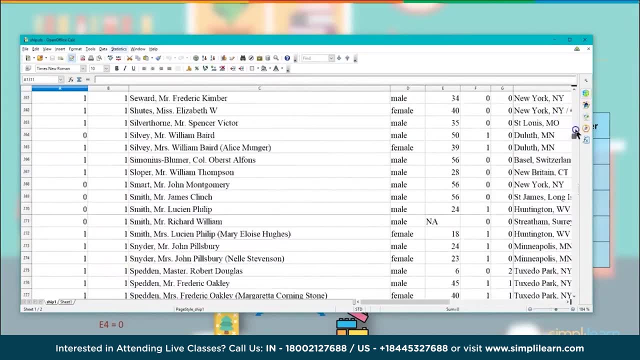 It's now looked at the survival of zero or one, Based on female, male, And what class they are, Where the best split of the age is And what class they were in. You can see we have first class If we go down there. 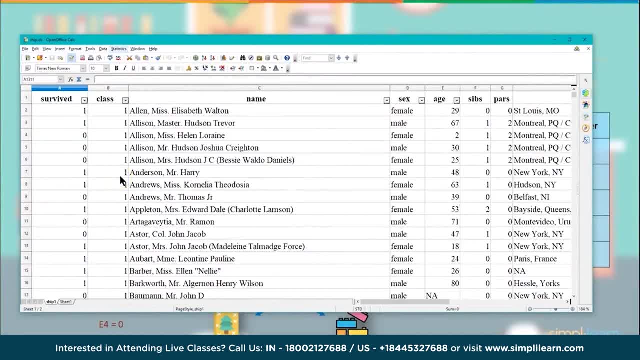 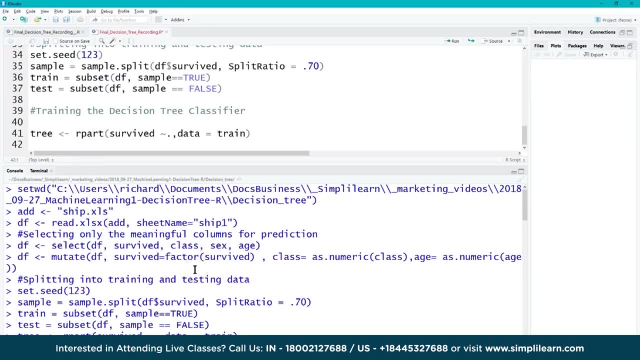 I think there's third, Yeah, third, Second, So I guess it's class one, two and three. But you can see that's how we split it up. So it's used these different variables To minimize the entropy And maximize the information gain. 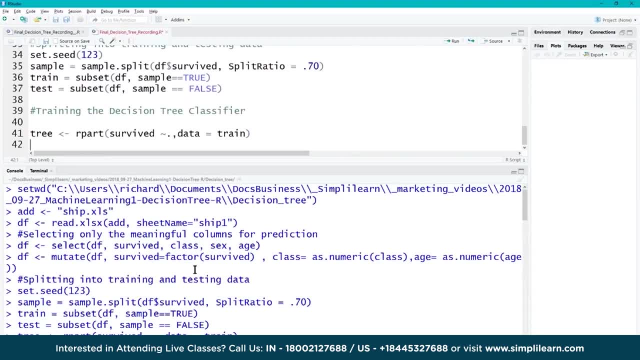 And that's all done in that one line of code. Boy, we worked on all that theory Because as they make changes to these, Or if you add special settings on it, You have to know what they're doing. But in this case you can see that once we get it formatted. 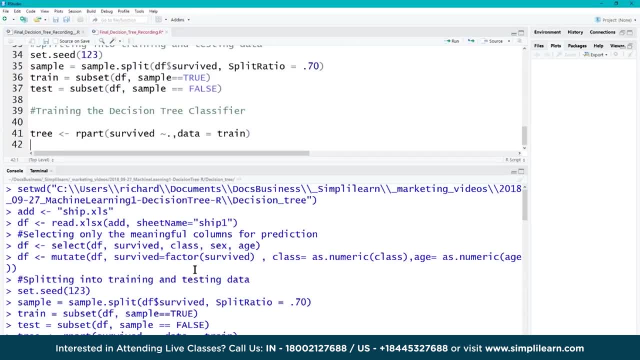 The computer does all the heavy lifting for us, And it never ceases to amaze me Just how advanced Machine learning has become these days And how easy it is For people to get into it And learn the basic setups And be able to compute your different machine learning models. 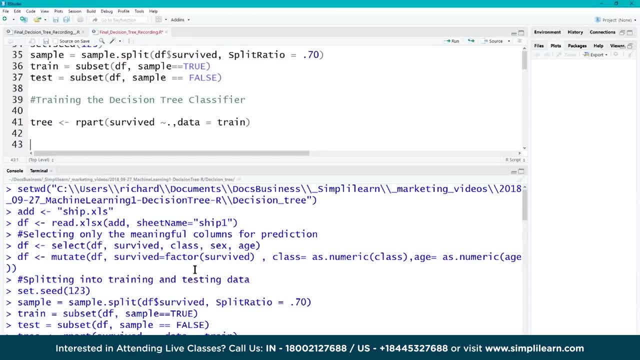 Once we've computed our decision tree And we've built it on there, We want to go ahead and start doing predictions with it. And what are we going to predict? Well, you remember that we created our data With the train and test. 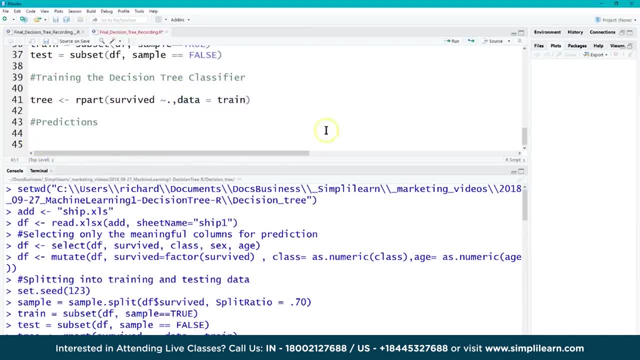 So we have our training data, Which we programmed the tree for. Now we want to see what it does with the test data. So let's see what that looks like And we can wrap that into Tree dot- Survived dot- predicted. 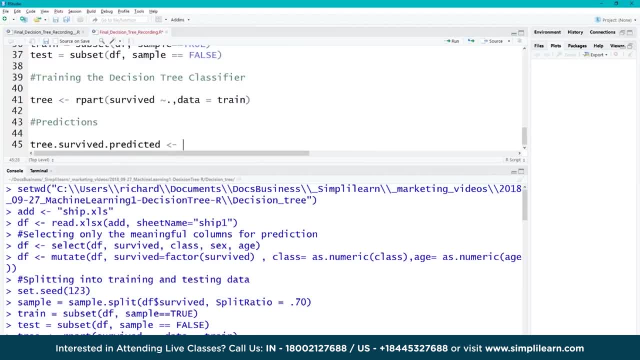 We'll assign that To our prediction And this is nice Because we have the command predict From one of the modules, The rpart module that we brought in, And I can simply put in here That we're going to use the tree. 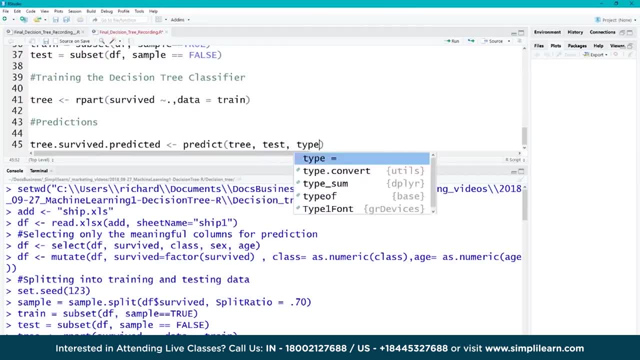 We have our test data And type And this happens to be classification Or class. And this would also be If you were to distribute this tree. You could save the tree And send it someplace else to be used on new data. 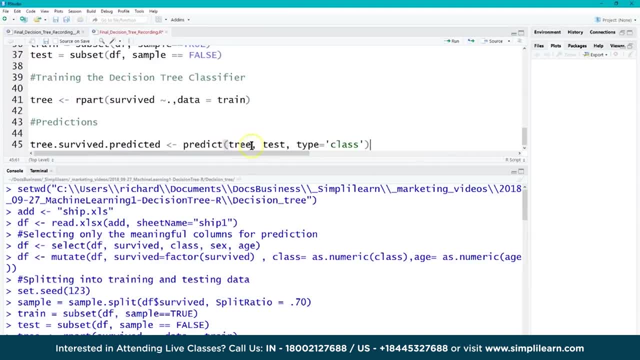 This would be the command line You would use to predict on here. You have your tree saved, You have whatever data you're putting through And you let it know it's doing a classification on the tree And we'll go ahead and run that. 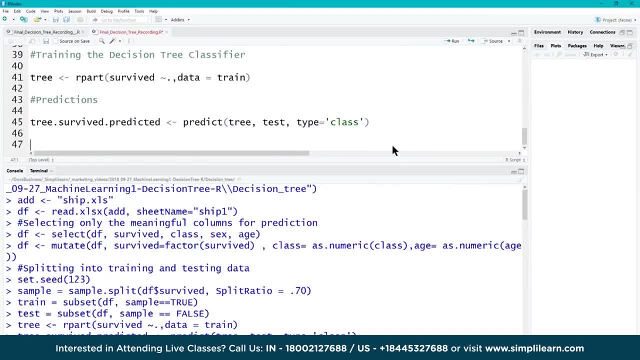 So now that's loaded up And now that we've gone through, We've trained our tree, We've run a prediction on our test data. Remember, the tree had never seen the test data till now, So we've already built the tree. 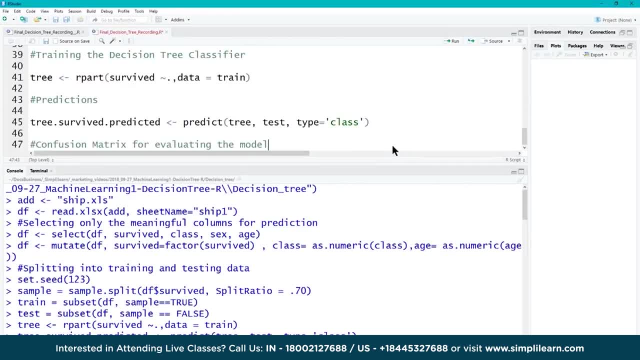 And we're just testing it out, And to do that, we're going to use a confusion matrix For evaluating the model. And let's see what that looks like: Simply confusion Matrix. So, once we have the confusion matrix Which came in from our carrot, 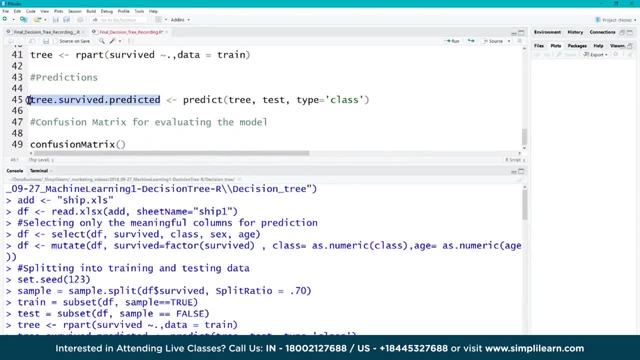 We need to compare the two different pieces of data, And the first one's going to be The value we generated up here. We have tree dot survived, dot predicted, So I'm just going to copy that And paste it down here. And then the second one is the tree. 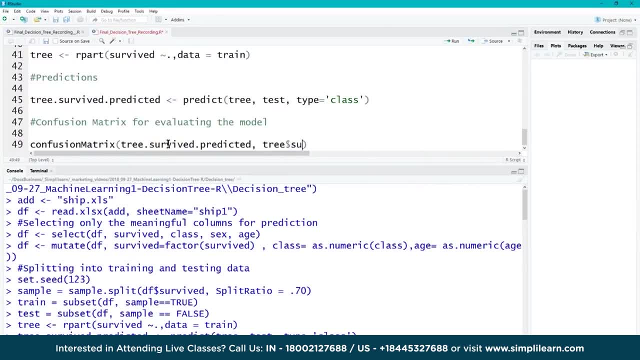 We're comparing that to Let's see Survived, But it's not the tree, So it's easy to get confused sometimes When you're moving these things around. We're going to compare it to test The test group of data. 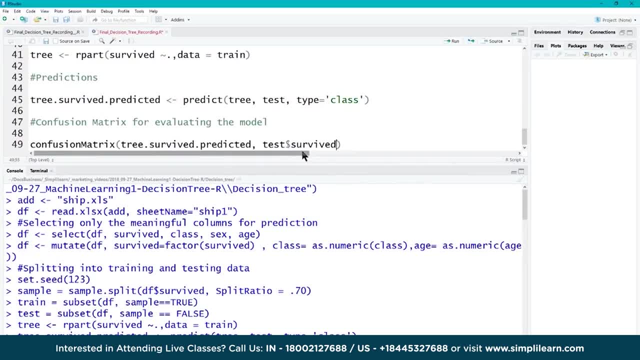 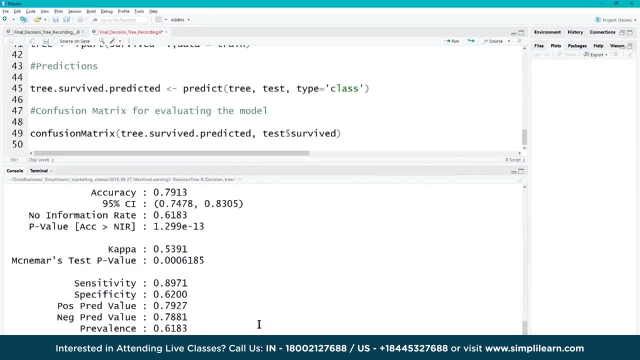 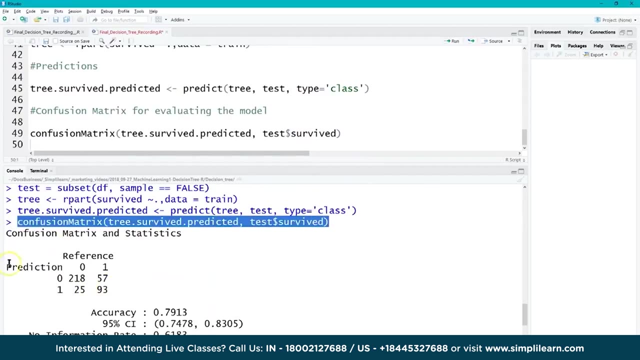 Specifically The survived column, And let's go ahead and run this And see what that looks like. And so let's go ahead and scroll up a little bit here To where it first executed the confusion matrix And the most important part of this. 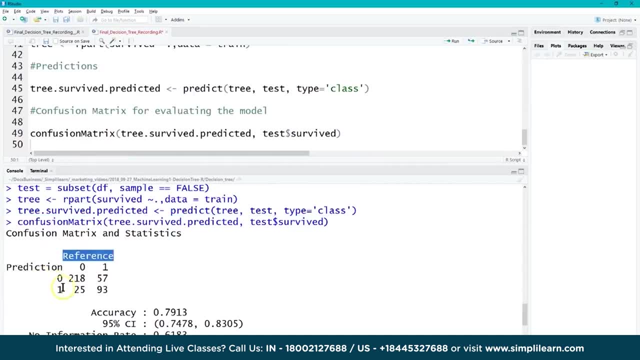 Is that we have our prediction And our reference. So zero means they didn't survive, One means they survived. We had our prediction on here Versus the actual, And that's what these two columns mean. And so when you read this little chart, 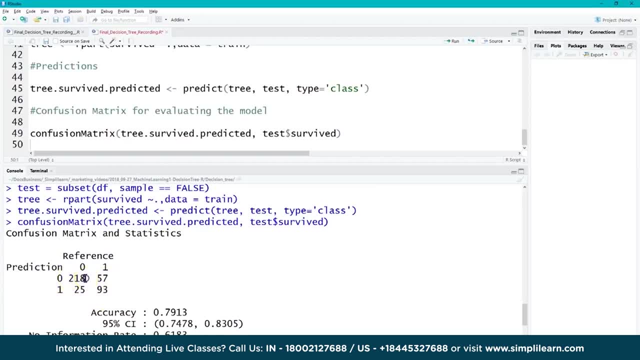 We have zero, zero. So both the prediction And the actual reference said We agreed on 218.. Values for people who did not survive. A little grim there for data. Remember I'm talking, This is morbid data. It says that they both agreed on 93.. 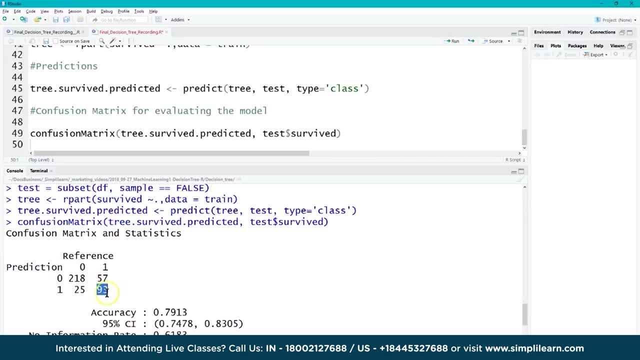 So 93 of them, Where we predicted the value That they would survive And the reference came up. the same. Likewise, Where it predicted one And the reference said No, these people didn't survive. Well, our prediction got 25 wrong. 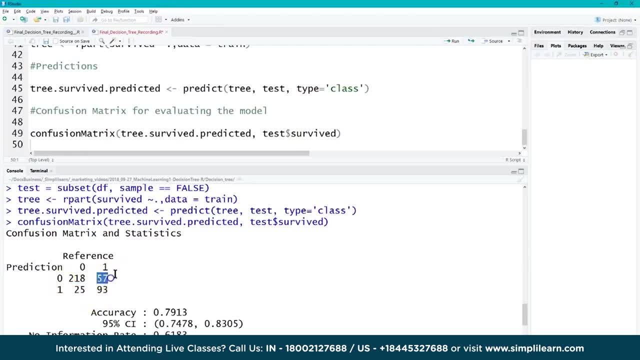 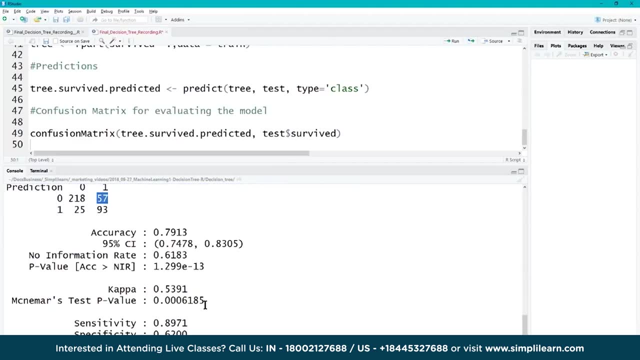 And where it says They didn't survive And they actually did. It got 57 wrong And we can come on down To the diffusion matrix And we can look at the accuracy Comes up with the 0.7913. 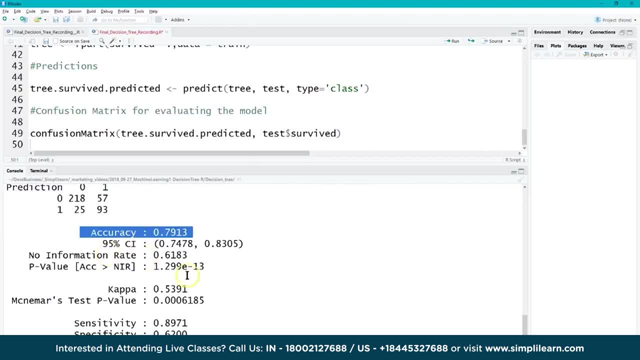 Or 95% CI. So, yeah, you're looking at pretty high accuracy Information ratio, P value. When you're getting statistics, The P value is one of the things we look at. Remember that there are certain values If it's over 0.95.. 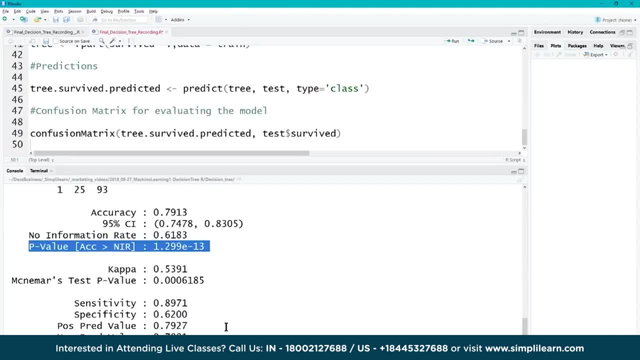 It's considered highly valuable variable. 0.5 means maybe Anything less than that Means it's probably not connected P value. a little bit more on that. And then they just have more information down here Which you can go through. 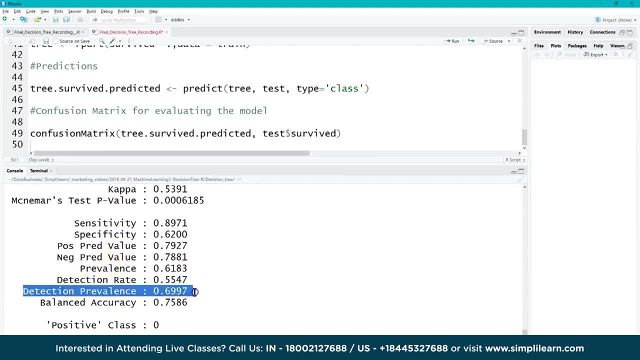 And Which you can go through, But the important part is that we have a very high accuracy. That's what we're looking at. This is a very accurate model And, again, always remember the domain you're working with. Certainly this is an example. 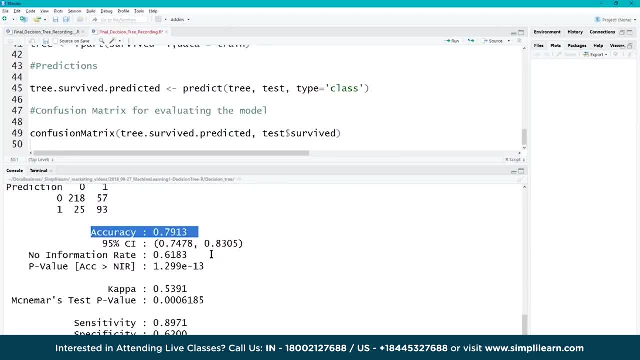 And this is a good little piece of data You can play with. But if I was, say, betting money And it came up as 79% Or over 95% CI, I'd be like, yes, Let's bet on that, That's a good bet. 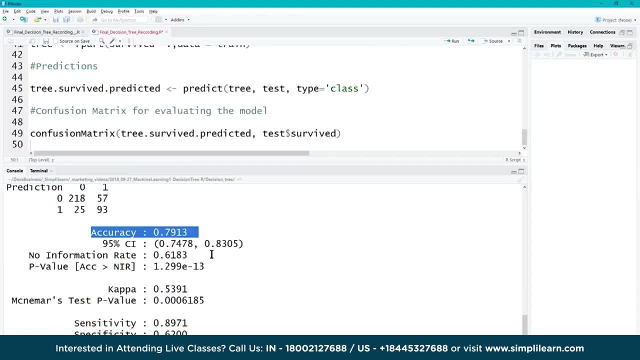 But if I was betting on a life or death situation, I might kind of rethink that a little bit. If it's going to affect my life that way, You can also look at this as if you're trying to figure out where the boats go. 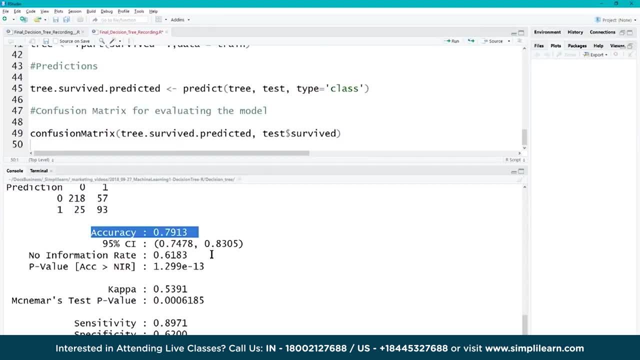 In this particular example, And where to put the lifeboats. That's actually pretty good Be able to say, hey, We can increase the chances of people surviving this accident By putting the lifeboats in the appropriate places, And then this is always fun. 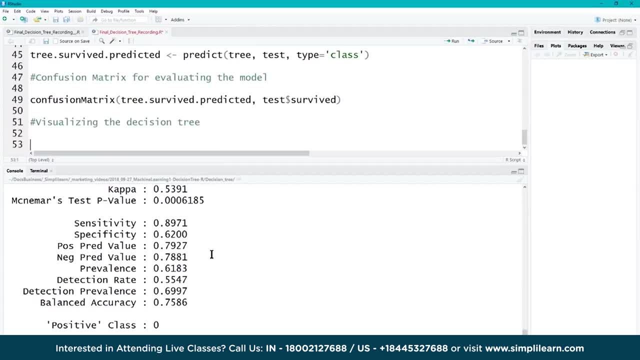 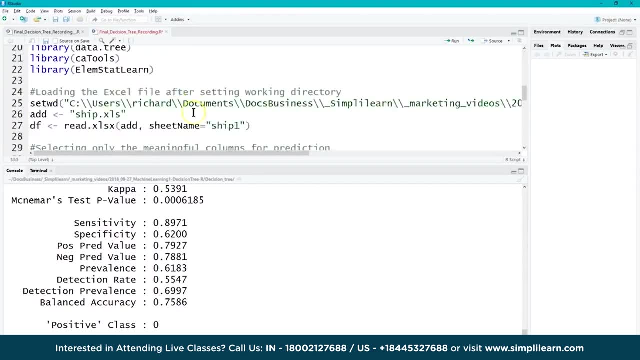 Let's visualize the decision tree. One of the cool things you can do inside of R Real easily And, if you remember, one of the modules we brought in Has a rpartplot. We're going to take that And we're going to dump that into the PRP. 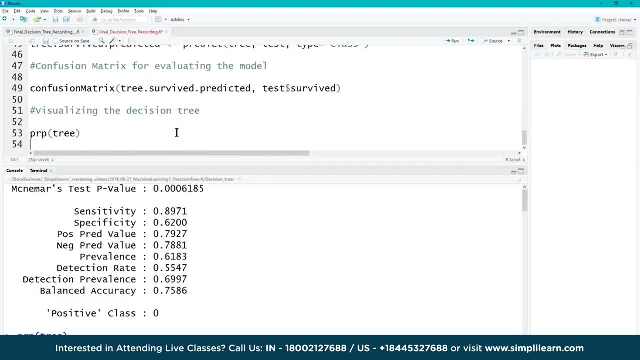 For the tree And let's go ahead and hit enter. And this is fun. Let me move this over so you can get a nice view, You can see how it actually split it up, And let me just rerun that again. You'll see right here. 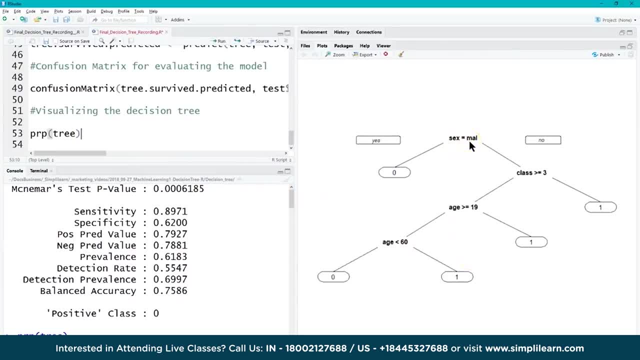 Where one of the biggest splits was Whether the person was male or female. Didn't know. that was probably one of the biggest breaks As far as lowering the entropy And increasing the information gain. And then, Once sex is male, It came down here: 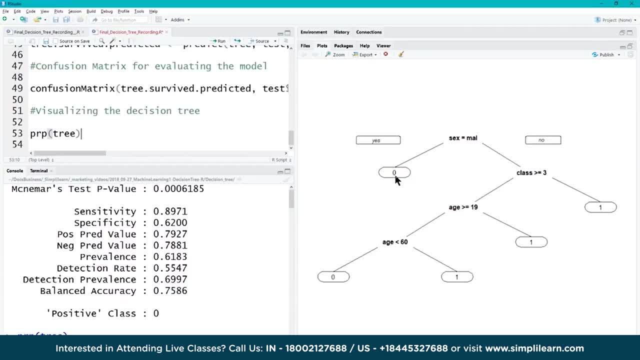 And it said: you're not going to survive. I guess the men were throwing themselves overboard on the boat. I don't know, Maybe they're being very gallant And letting the women and children survive, Which is what I hope that means. 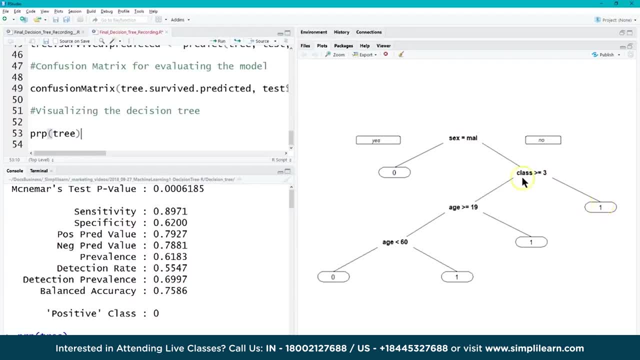 If you're in class 3 or above, You had a high chance of surviving. If you're less, in class 3. Class 1 or 2.. Then it was based on age, So you can see where age was greater than 19.. So anybody over 19. Had a high chance of surviving, And then if they were Or less than 19.. I'm sorry If the age was a little confusing on that one, But if the age was one side of 19.. They probably survived. If not, People who are older Probably didn't make it out of the boat in time, So elderly have a much higher risk, Which you would expect. You would expect that to be the case- That elderly would have a hard time getting off into the lifeboats. 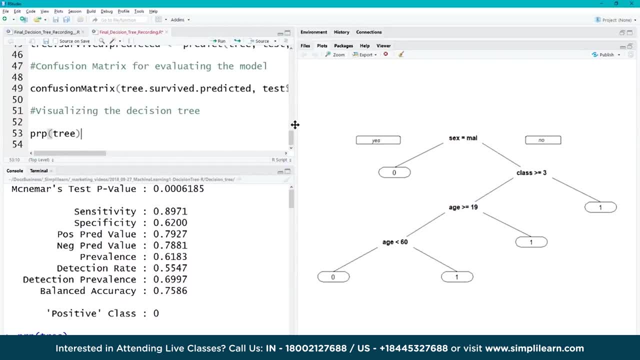 And they would probably step aside for the younger generation- I know I would. That might be more of a social norm statistic As opposed to survival rate. Let's go ahead and put this back on over here And see what else we can do with this data. 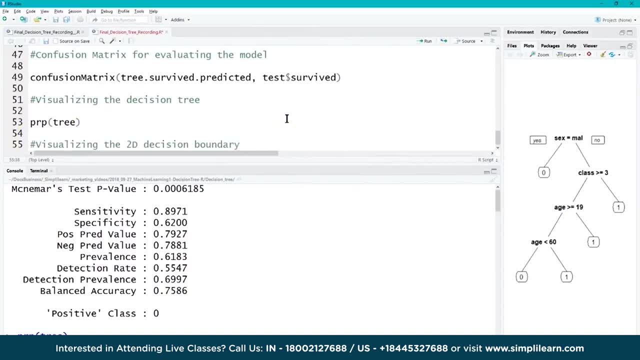 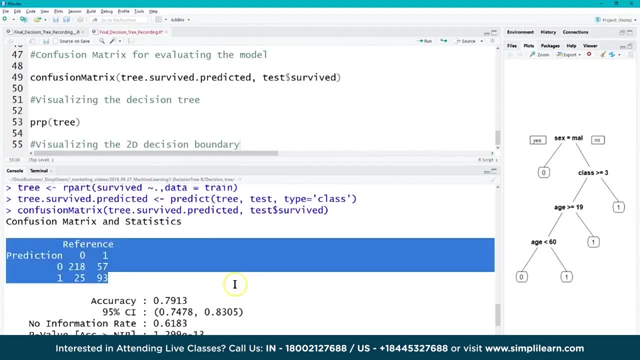 Now, if you're working with the shareholders, It's good to have a lot of tools As far as how to display. I mean, they'll want to see this number here Where you say, hey, This is what the confusion matrix looks like. 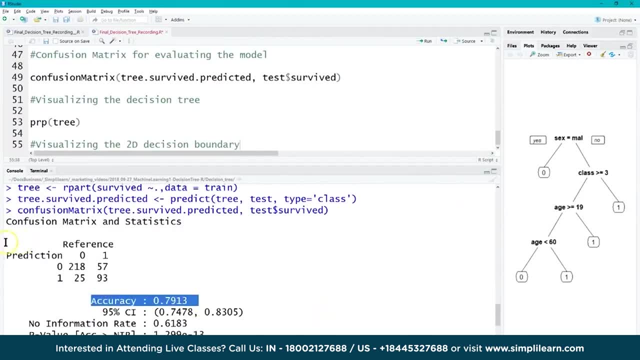 And we got a .79 accuracy. That would be like the number one thing You would talk to the shareholders about. Other data scientists care about the p-value And the information rate And information like that, But this is really the core right here. 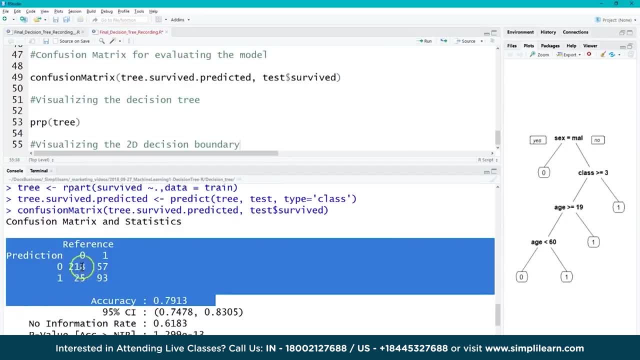 This is how much data And this also shows them how much data was looked at. So you can actually just add these numbers together And you can see how many different people were in this particular data set Or how many lines in the data set. 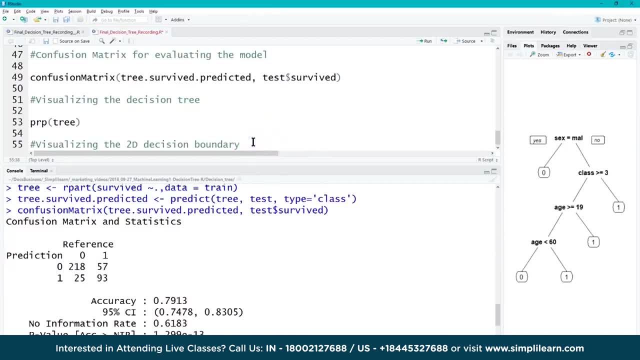 But we go ahead and visualize The 2D decision boundaries And let's take a look at that. That's kind of fun. That's a little bit more complicated So I'm not going to go into it in too much detail today. 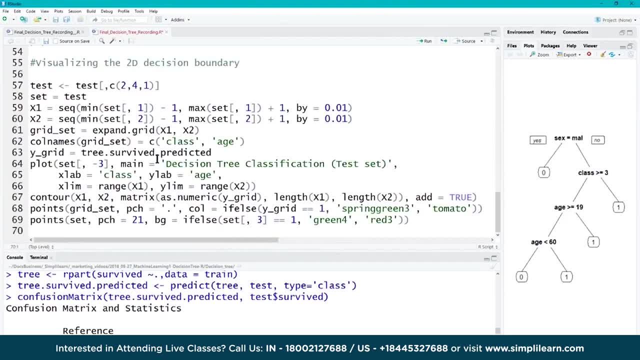 Now the guys in the back put this code together for me, Which is great, So I'm just going to paste that in, Because, like I said, we're not going to go into it in too much detail. I wanted to show you that there's some other ways to display the data. 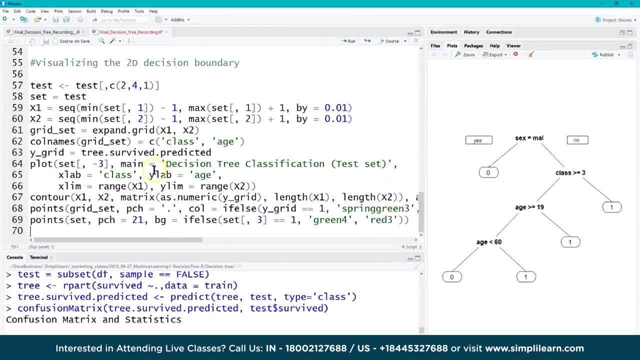 That it's not just this nice little tree over here Which gives us a little bit more, Maybe, view of what's going on. As you dig deeper into data. It might not be something so simple Where you can look at in this case. 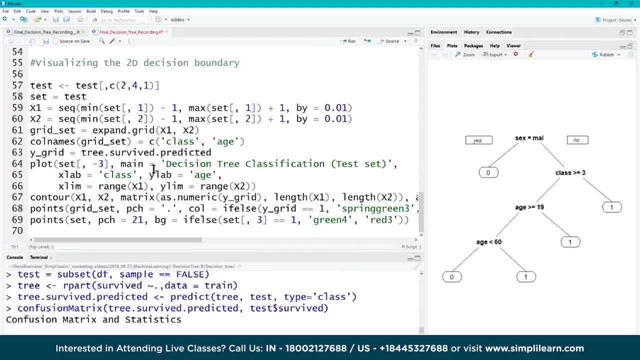 One, two, three, four nodes. So they have four major nodes That they split the data in. So we're looking at this. We're going to go ahead and create a set test Equal to test comma C241.. We're just assigning color column. 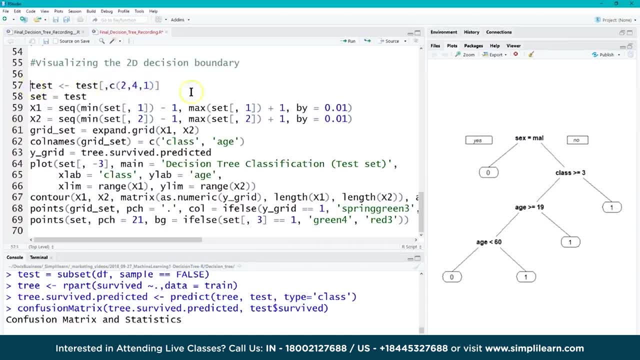 To go with the data. Okay, That's what that is. And then we're going to take set And have it equal to test, And we'll do that. We're going to set that to X1.. And we're going to set that equal to. 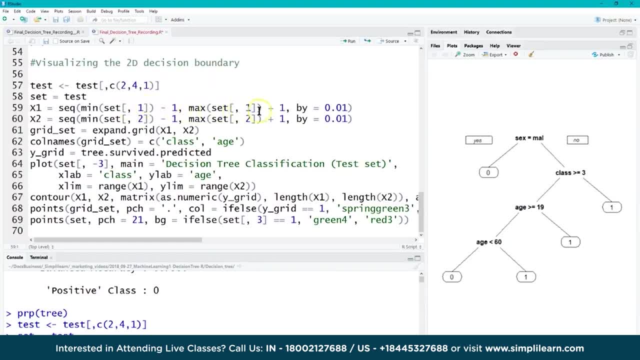 Minimum set of one Minus one. Max set of one plus one By equals point zero one. They had to play with these numbers a little bit To get this to look right, So we're creating a sequence on here From our. 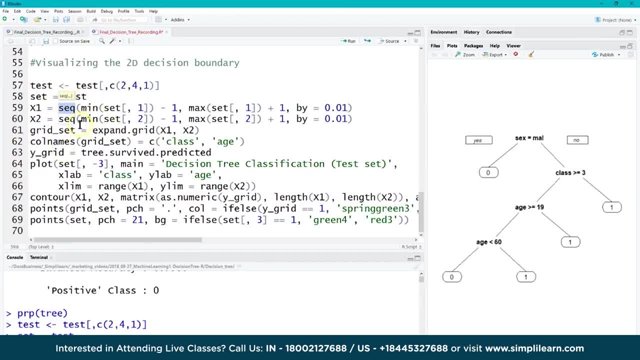 The set we created, So our test set, And then X2 is also creating a sequence Based on different values, And then we're going to put that all into a grid. So let's go ahead and run that through All the way down to the grid. 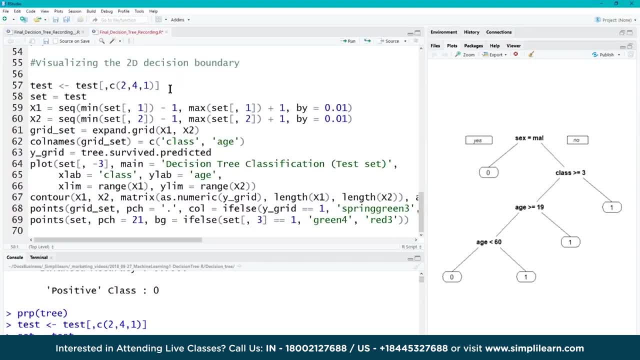 And it'll make a little more sense When we add the column names to the grid. Okay, So we'll set our test, We'll create our X1 sequence And our X2 sequence. Remember, a sequence is just like In this case, starting with point one. 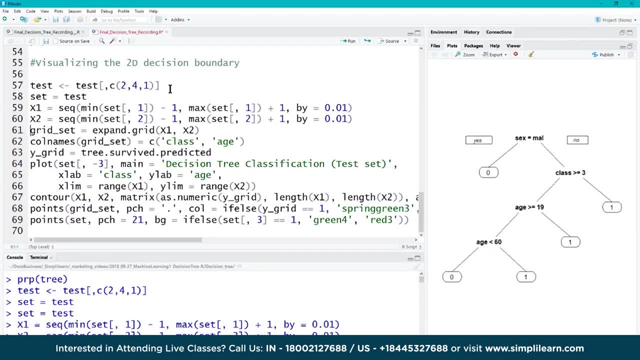 It's like point O1, point O2, point O3,, point O4.. So we're going to create a grid With all these values separated by point O1.. So that's all we're doing right now. Let's go ahead and set that up. 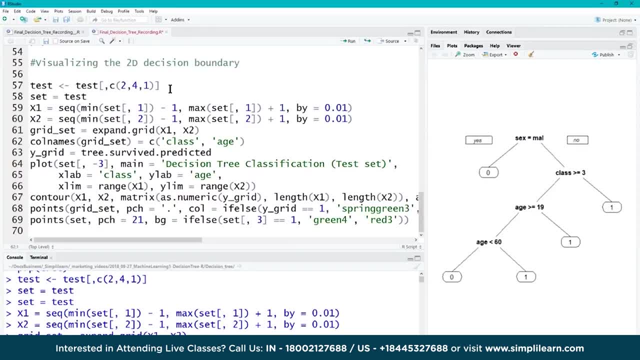 And then we want to go ahead And create some column names And for our grid set We're going to have our C class and age. So we're just doing the class And the age on here. Remember we did sex also before. 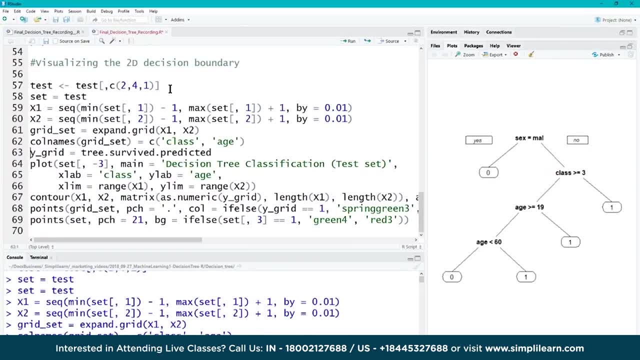 So it's just class and age on this chart That we're pulling out And we're going to create a Y grid And the Y grid is going to equal Tree survived, predicted. Okay. So here's our Y grid And our predicted values on there. 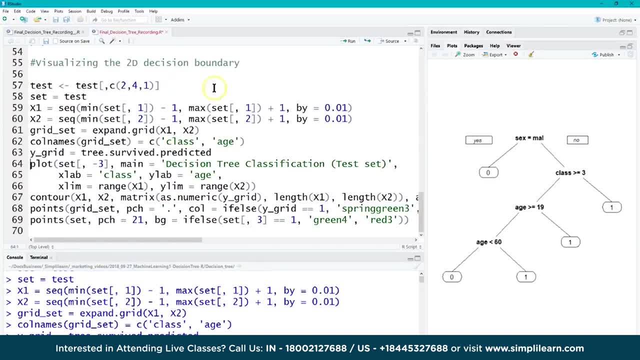 Now we're actually going to do something. We're going to plot And we're going to plot the Y grid. Oops, hold on, let me see what's in here And let me go ahead and just run the plot. It's got to be the. 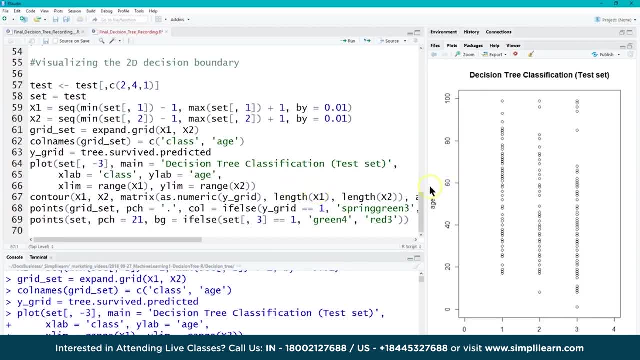 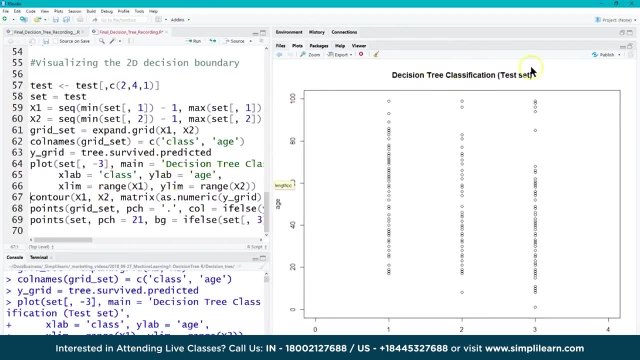 There we go. So let's take a look at this And see if we can make a little sense of this code And what's going on here, Because there's a couple things going on. What we've done is we've plotted. 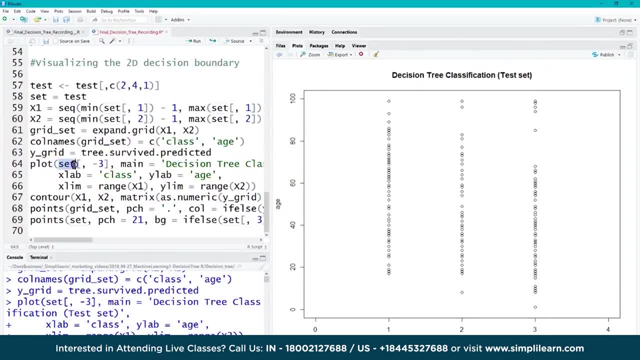 A decision tree classification data set. We've done our plot. That's equal to our test data, And then we have our main. We went ahead and gave it a name: Decision tree. And then we have our X lab And our X limit. 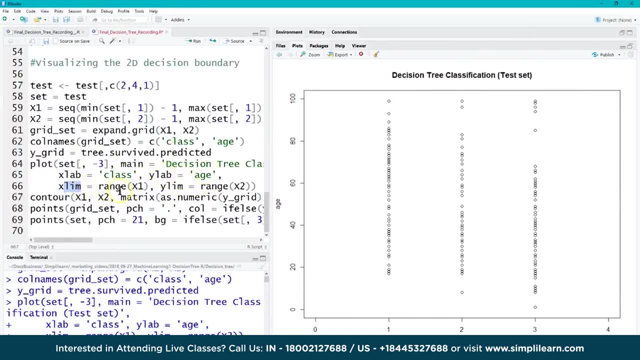 And we've set those up as class With our Y lab equals age, And our X limit equals range X1. comma Y limit equals range of X2.. And when you look over here You can see that we have Age on the left: 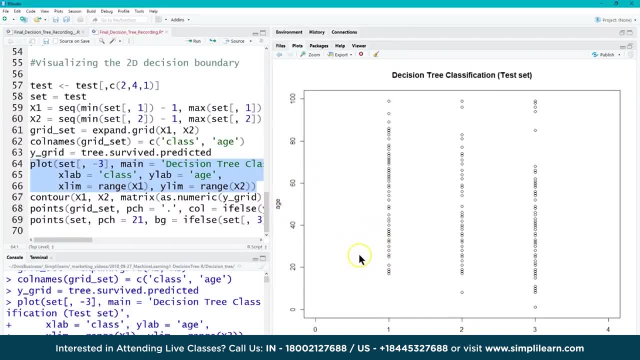 And class on the bottom, And so based on age and class. And so once we put in This nice graph here, We want to go ahead and add our contours And our points. So let's go ahead and run that And I'm going to run all three of these. 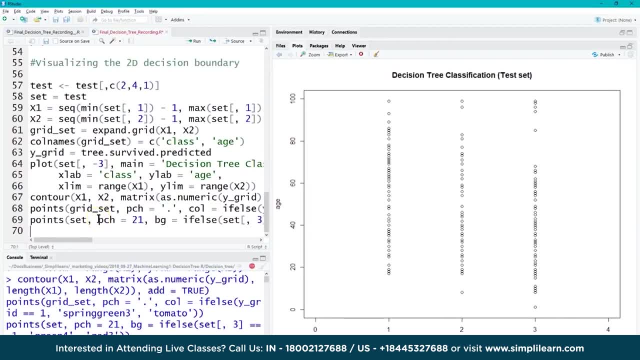 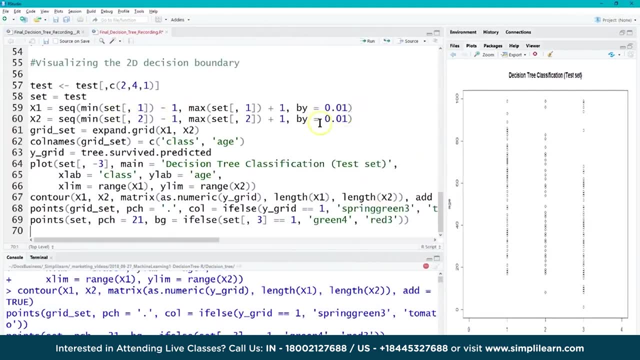 So we can see all the colors come in on the graph. And this is actually going to take a little bit Because, remember, You can make it go a little faster By changing a couple of the notes up here. When we did .01 from the min to max. 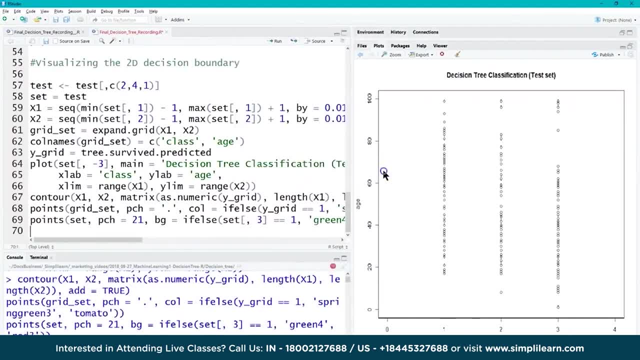 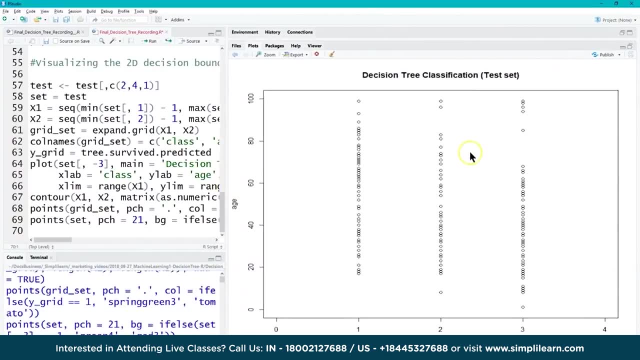 By changing that to .1.. Or other values. You can actually- And we're going to create a nice little Decision tree classification test set Just to see what that looks like And how that data displays. Now, that was taking so long. 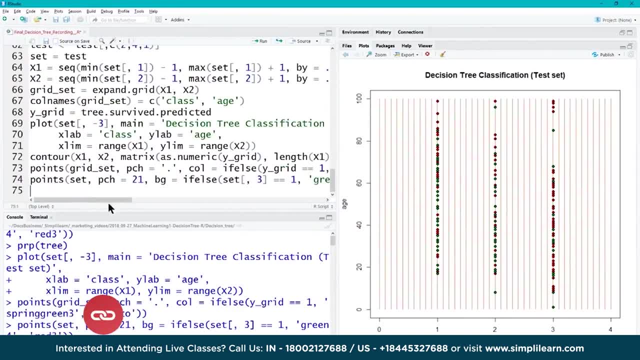 To run with .01.. I went ahead and just did a .1.. So instead of filling the whole page With different colors for a really pretty view, Now I just have these different colored lines Coming across, And it gives us another model. 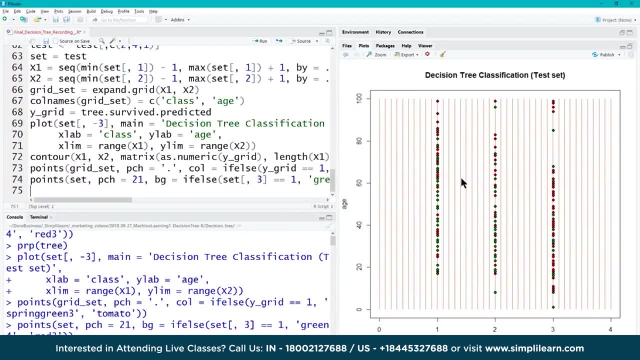 That we can show for whoever you're working with- In this case, your shareholders of the company Or the individuals- To the web for And you can see where we have the green and the red And we've set those up to identify. 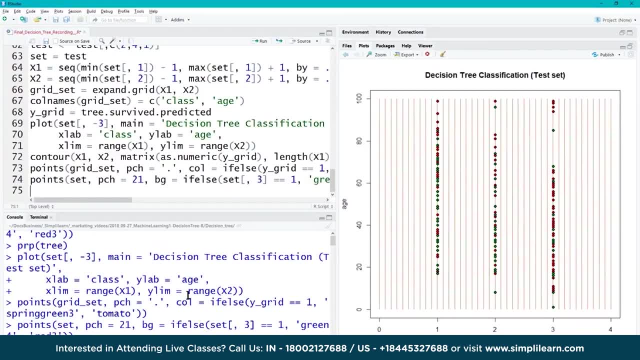 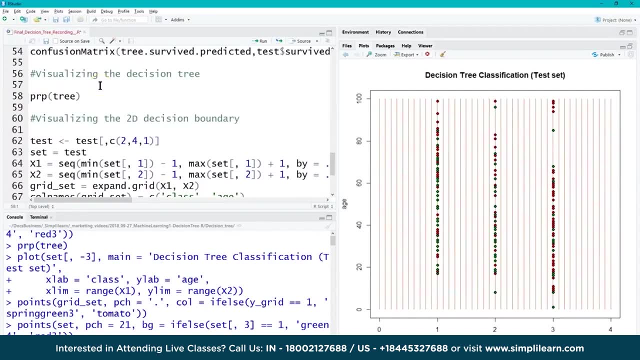 From the decision who's going to make it And who's not, based on age and class. Now, my favorite one on this- And I'm going to go back and just highlight this really quick- Was- let me just rerun that: Go back to PRP tree. 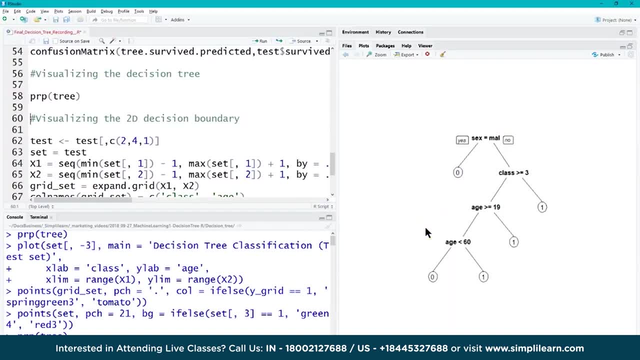 Where we display the tree And that's where we split it, in part Because this information gives us some keys That we can then use In other models. So it's good to know that sometimes And maybe you create a bucket For people under 19.. 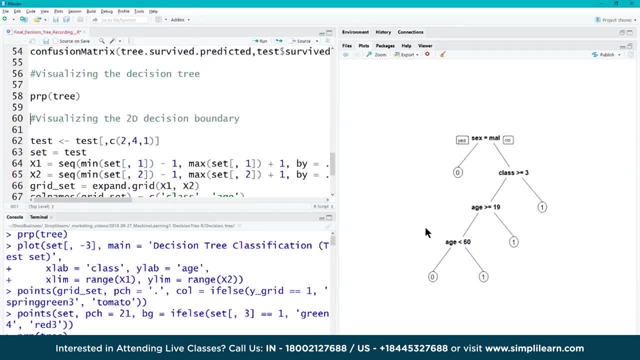 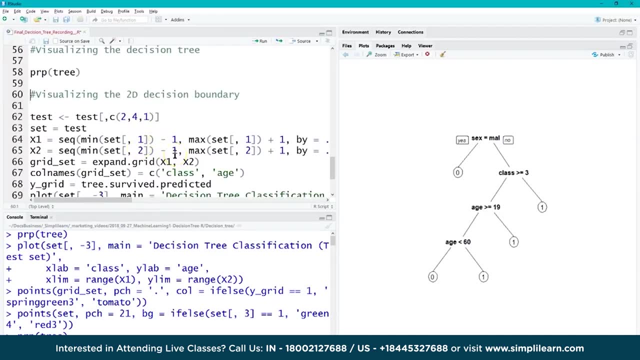 Between 19 and 60 and over 60. And different things like that, So you can actually put people in buckets In a class age split. Just a quick note on there. Again, you know lots of different things From which you can display the data. 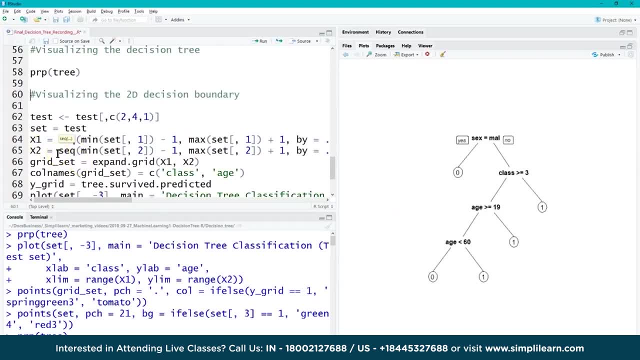 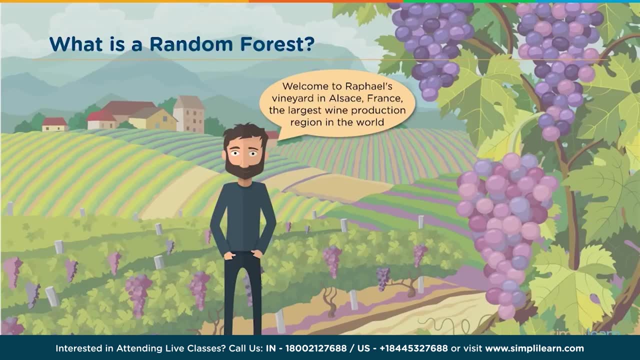 And you can see how we use the decision tree To figure out chances of somebody Surviving, based on their class and their age. What is a random forest? And welcome to Raphael's Vineyard. And I don't even know how to pronounce that. 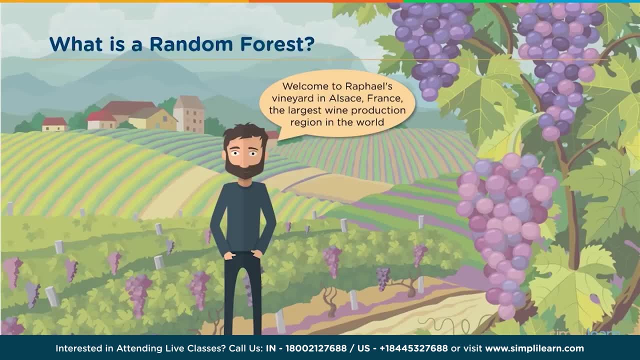 The largest wine production region In the world, So they have centuries of wine production And data they've collected On how to make the best, How to make their grapes and grow them, And how to properly get the right grapes And ferment them. 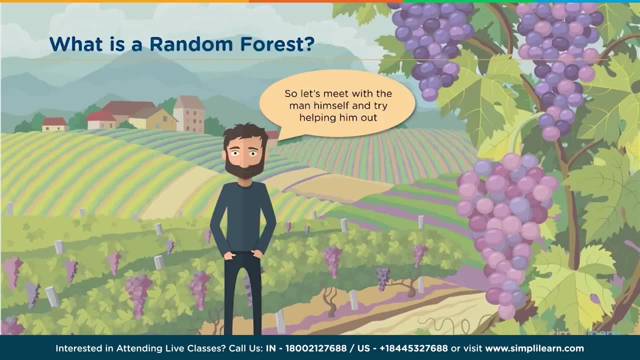 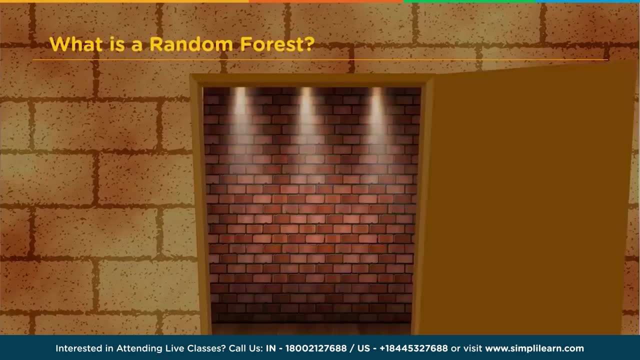 Like Raphael, Wine makers around the world Are facing a grave problem, So let's meet the man himself And try helping him out. What is a random forest? Of course? here comes Raphael. I'd probably look closer to Raphael Than I do to the young lad with the beard. 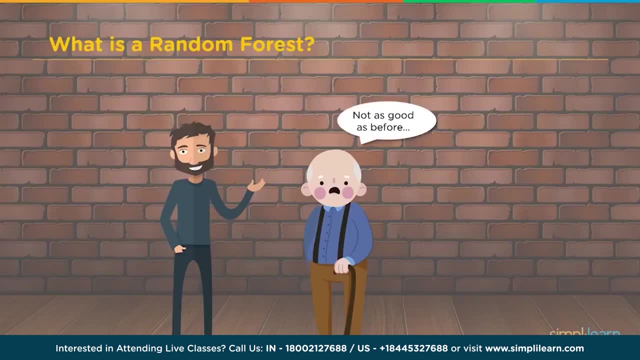 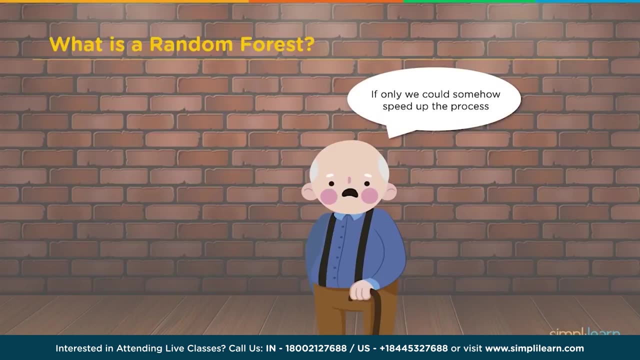 Hey, Raphael, So tell us how it's going. Not as good as before. Not many people work in this profession anymore, So every stage of production has gone slower. If only we could somehow speed up the process. Well, lucky for you, I'm a machine learning engineer. 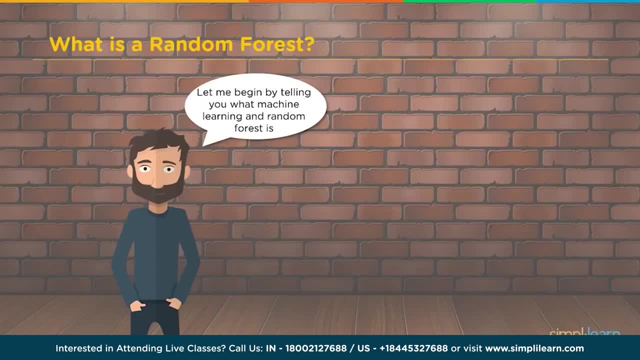 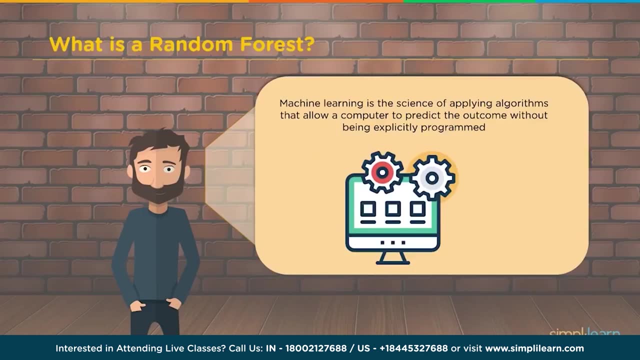 How about we automate the quality prediction process for wine? Let me begin by telling you what machine learning And random forest is. Machine learning is the science of applying Algorithms that allow a computer To predict the outcome Without being explicitly programmed. Random forest is an ensemble machine learning algorithm. 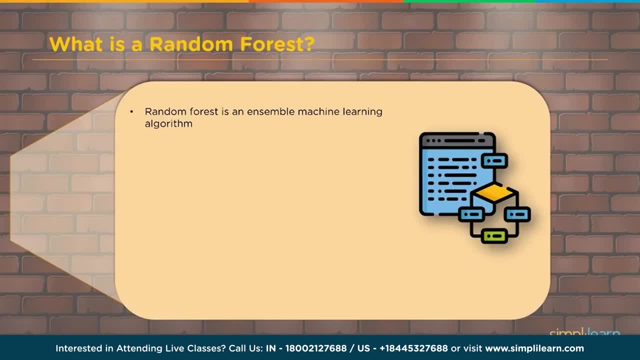 So we're bringing in different pieces And then putting those pieces together. It operates by building multiple decision trees. Remember I told you We don't want just a lone tree out there, We want a forest. They work for both Classification. 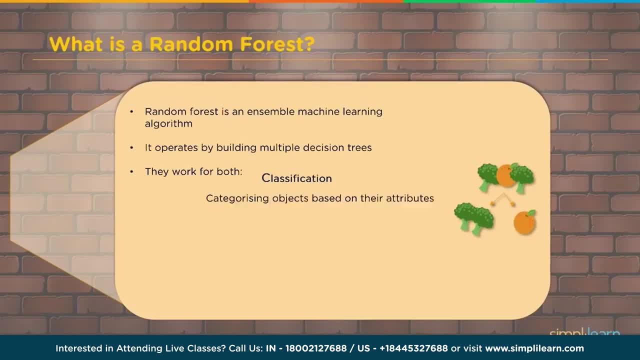 If you remember from part one, We had our vendor with his broccoli and oranges. I think he also had carrots. The majority of his decision trees Is the forest final output. So if you have a number of decision trees, You have five decision trees. 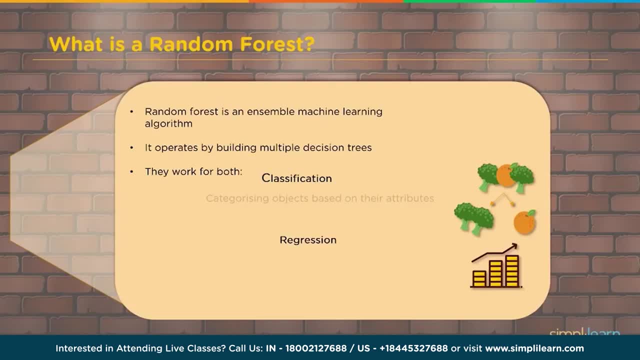 And four of them say it's broccoli, Then it's probably broccoli, And you can also use it as a regression model. The output given by the majority of decision trees Is the forest final output. Just like you do in classification, You can also come up with actual values. 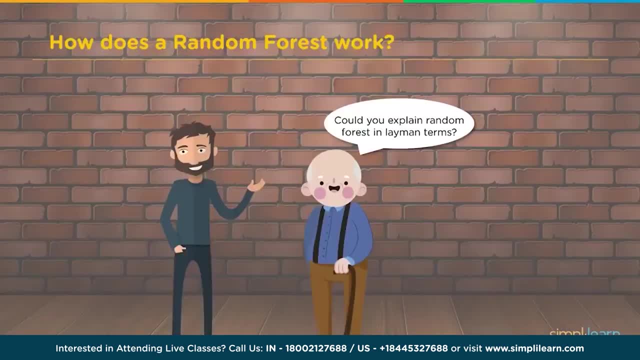 And numbers as a regression model. Could you explain how a random forest works in layman terms? It's always a good thing to explore the information On something a little bit easier To understand and see. Sure, Let's consider the case of Sam. 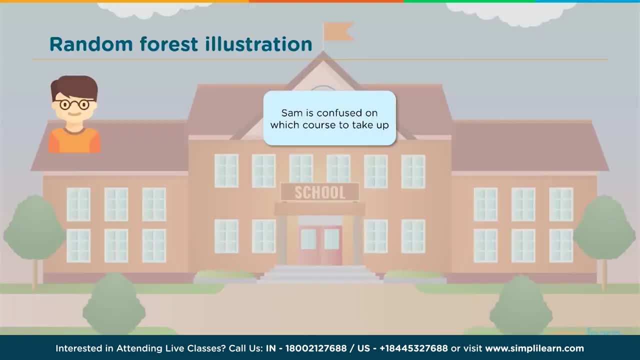 A high school student. This so reminds me of my own high school student Who just started his first year in college Asking all his friends. So Sam is confused on which course to take up, So he's trying to figure out what his next class is going to be at school. 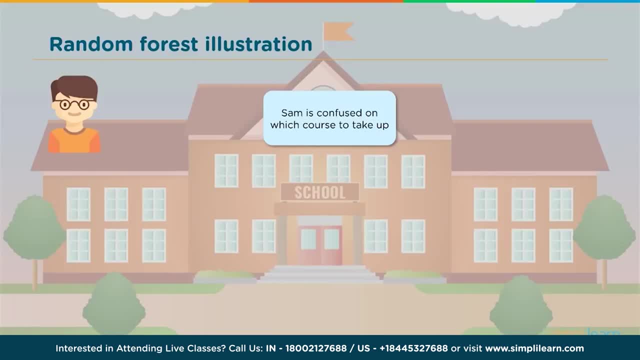 Should he take music lessons, Dance lessons, Math Science, Maybe social studies? So he decides to ask a couple of his friends for suggestions And Sam approaches Jane first: Which of these classes should I take? And Jane asks Sam a few questions. 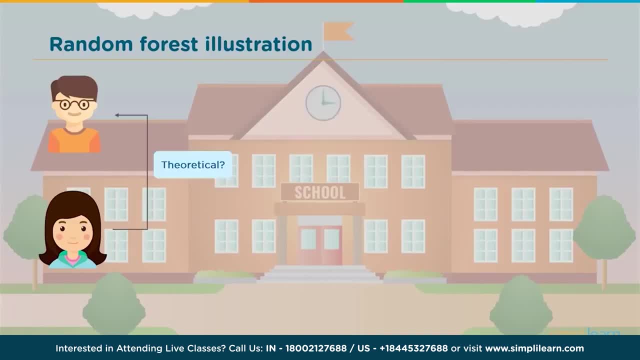 Based on which she can suggest: Theoretical: Do you like theory? No, He doesn't like the theory part. Calculative: Do you like calculative? He goes: yes, I like doing calculations. And so, Jane, based on a couple questions, 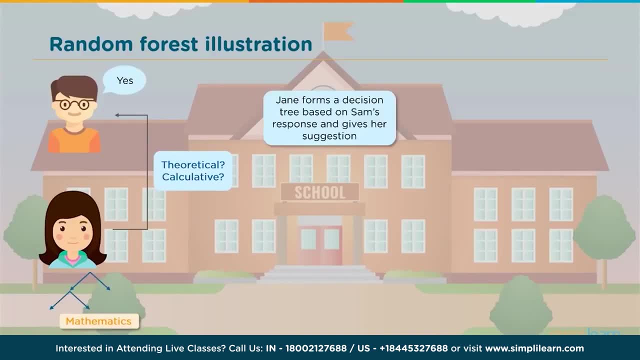 She has her little decision tree there going. She goes, mathematics sounds good. So Jane forms a decision tree Based on Sam's response And gives her suggestion, And of course this is based on Jane's views And her history, Which she collected over her years in high school. 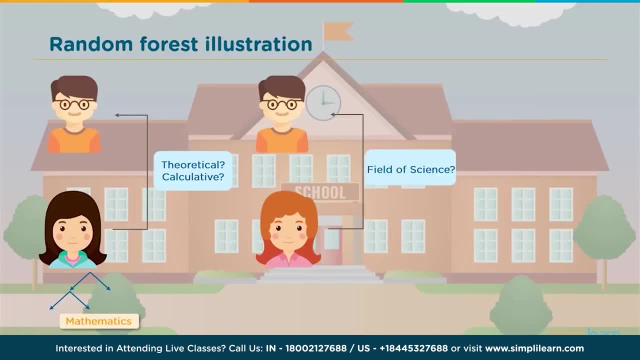 Next, Sam approaches Bella. Bella asks him: hey, do you like the field of science? And Sam goes yes, And then Bella goes: do you like new in industry? Do you like new things coming up in industry? And Sam goes yes And Bella goes. you know you should. 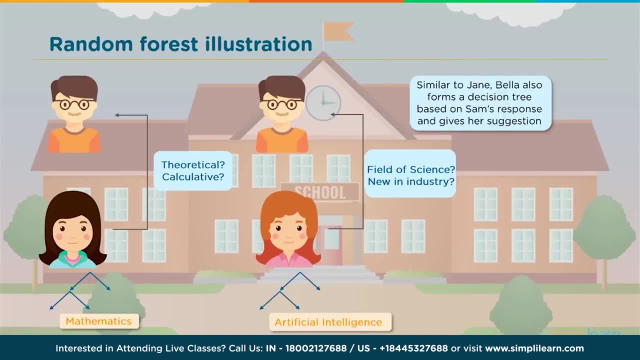 similar to Jane, Bella also forms a decision tree based on Sam's response And gives her suggestion And says: hey, how about artificial intelligence? Sam's like: oh, artificial intelligence. So Sam next asks Terry for his suggestion And Sam goes: do you like scoring things? 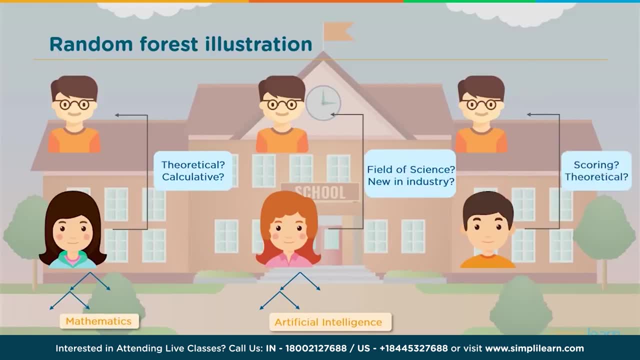 And he goes yes, And he goes. do you like theoretical? And he goes no, And he comes up and says mathematics. So you have two people saying mathematics And one person suggesting artificial intelligence, Since two out of three friends suggested math. 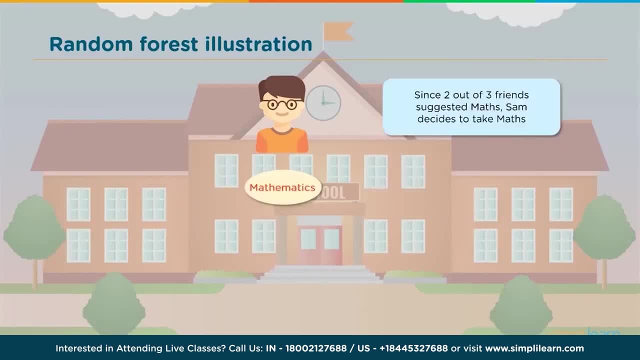 Sam decides to take mathematics, And there's a lot of subtleties in this example. It's actually a really good example. Some of the things we run into in data science Is when we collect data And we collect data, And we collect data. 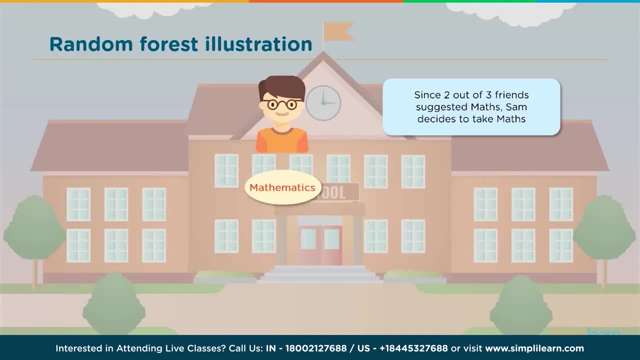 From different sources. We might have data from one source That measures one thing, Or one set of instruments, And we might have data from another source That measures something else. We saw that with each of his friends Are measuring different things. 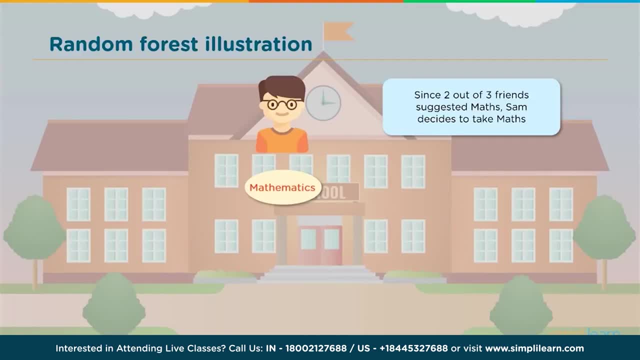 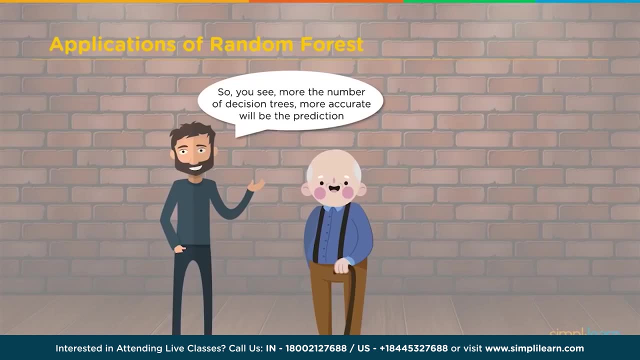 And asking different questions. That's a little bit beyond the scope of this particular tutorial. So let's go back to our wine cellar. So you see More the number of decision trees, More accurate will be the prediction. Random forests have a number of applications. 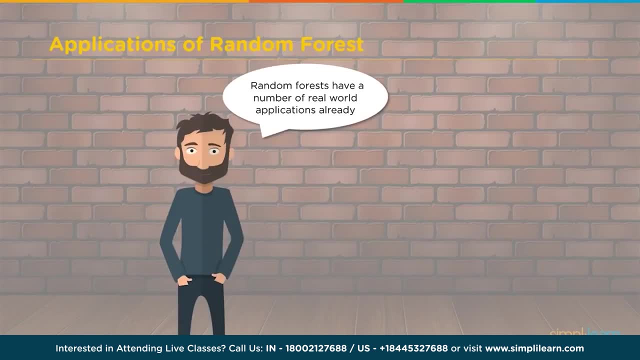 In market already. If you've been watching any of our other tutorials, You'll see that these are very common We have in banking. It can be used to predict fraudulent customers. It is used to analyze symptoms of patients And detecting the disease. 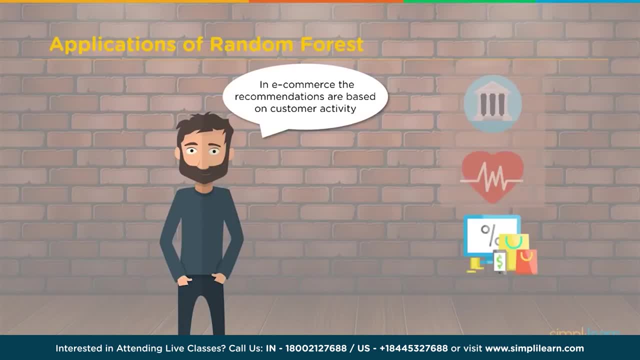 In e-commerce. The recommendations are predicted based on customers activity. Stock market trends Can be analyzed to predict profit or loss. Most recently, I was watching a review on weather Here in the United States And the data they pull in for that. 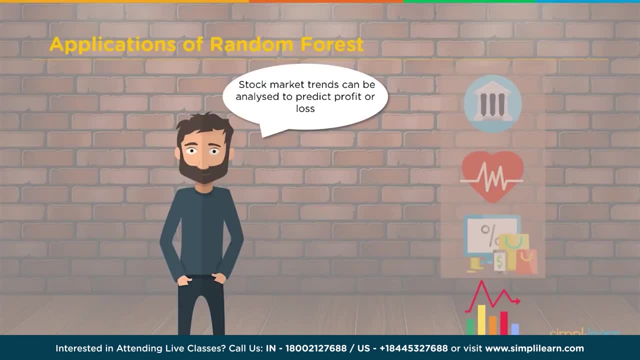 One of the top weather places actually uses Five different models. Random forest was one of them, I believe. They use five different models To predict the weather And, depending on what the models come up with And what's going on, Some of the models do better than others. 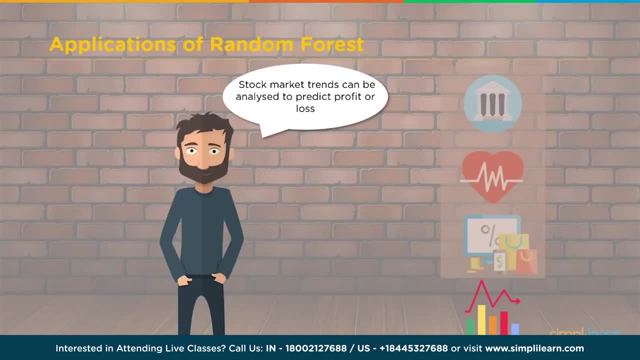 I thought that was really interesting. It's important to note. So when you see us repeat the same things over and over And you're looking at the different machine learning tools, You realize that we use multiple tools To solve the same problem. 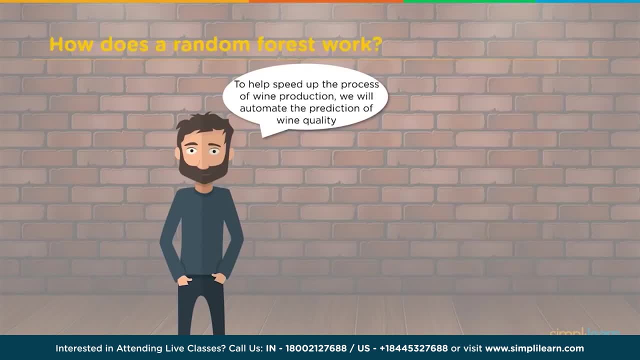 And we can find the best one that fits In a particular situation. So let's see How that fits back in our wine production. To help speed up the process of wine production, We will automate the prediction of wine quality. Suppose our random forest. 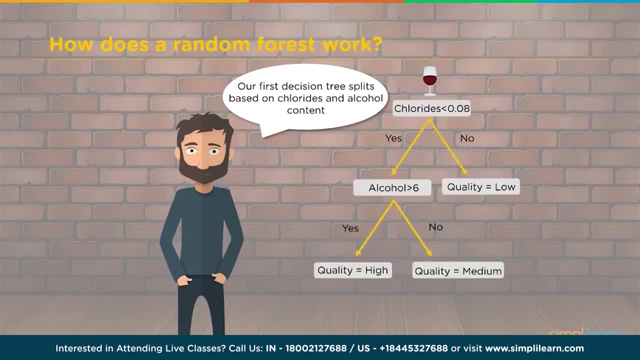 Builds three decision trees. We have the first decision tree Which is going to divide everything by chlorides Less than .08.. And it's either yes or no. And then it's going to look at alcohol greater than six: Yes or no. 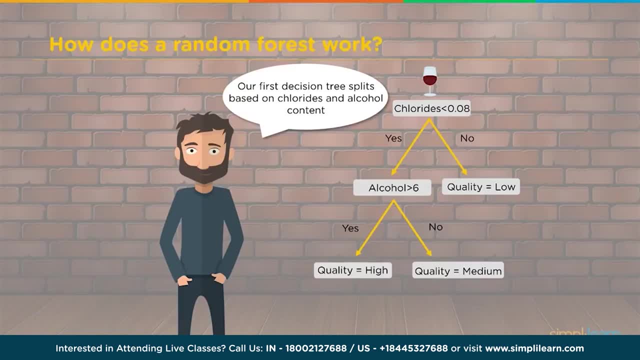 Quality equals high Quality, not so good. So there's our first tree, And then our second tree is going to split it On. sulfates less than. .6.. And pH, pH less than 3.5.. And again we have it coming down here. 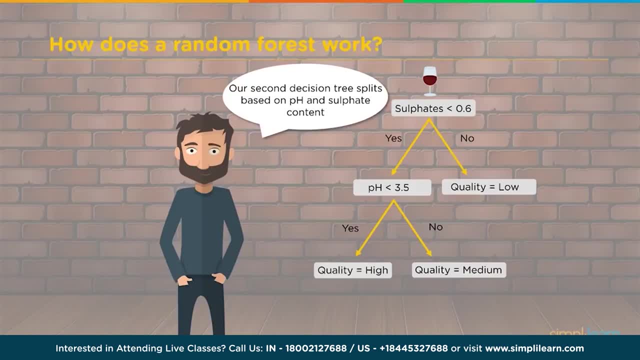 That if the pH is low And the sulfides are low, The quality equals high. If the pH is a little higher But the sulfides are low, It's not so good, And if the sulfides are greater than .6.. 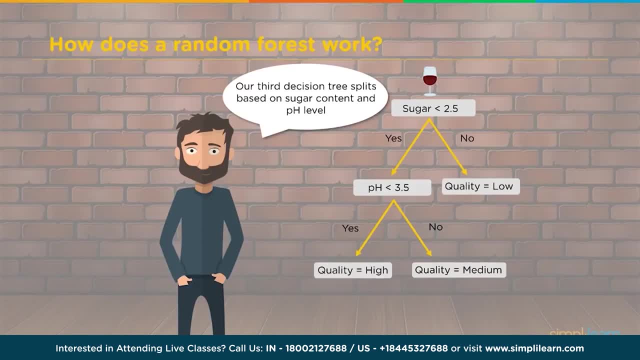 We have a quality equal low And then we'll do a third decision tree. If it's not, It's a quality equals low, It's a real low quality, And if it is less than 2.5. Then the pH decide whether it's going to be a quality high. 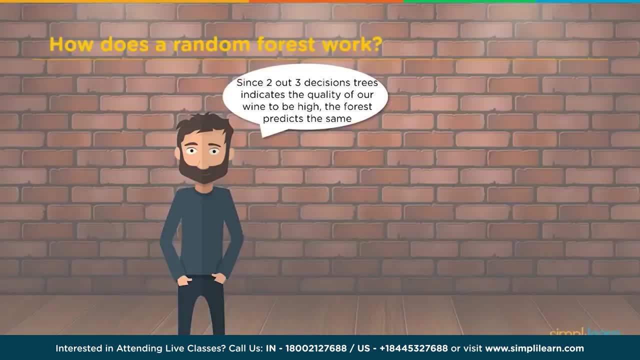 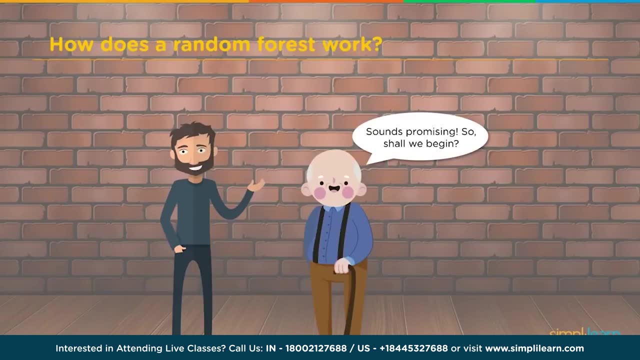 Or not so good. And if we track one of our wines down the list, We'll look at it. We'll say, oh, two out of three decision trees Indicate the quality of our wine to be high. The forest predicts the same. 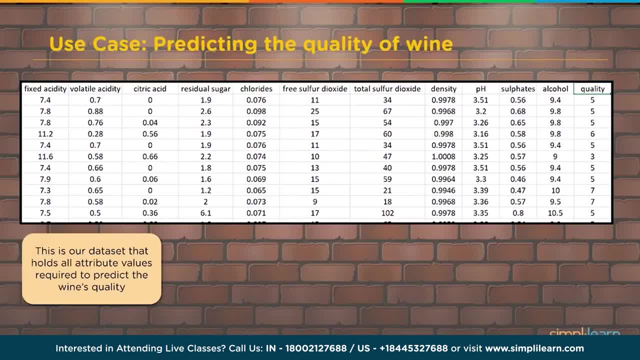 So this sounds promising. So let's go ahead and dive in And see what that actually looks like. So we're here to predict the wine's quality And I'll pull this up in a spreadsheet in just a moment. But you can see here we have fixed acidity. 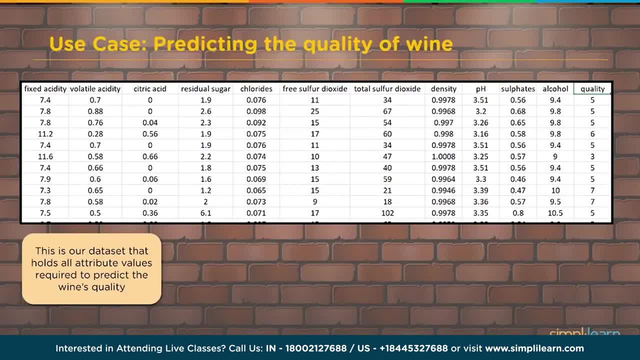 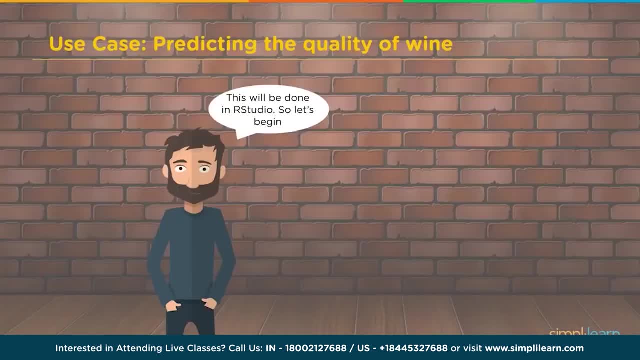 Volatile acidity, Citric acid, All the way to quality, And then quality is like a 4,, 5,, 6 or 7, I believe, And this will be done in R. So let's go ahead and get started in our coding. 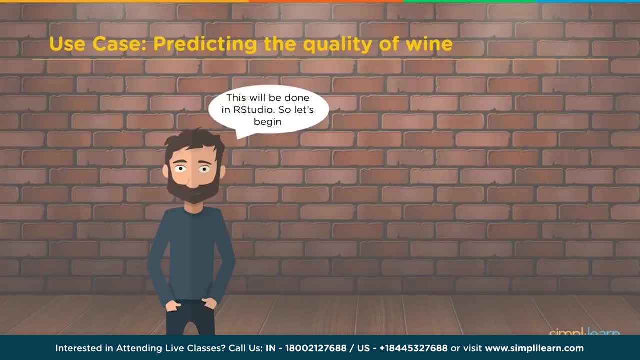 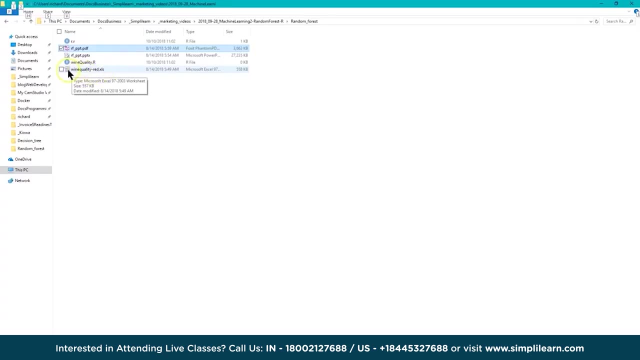 We'll be using RStudio. Before we dive into RStudio, I always like to open up the data in the spreadsheet And look at the actual data that I have. And they've called it winequality-redxlsx. And they've called it winequality-redxlsx. 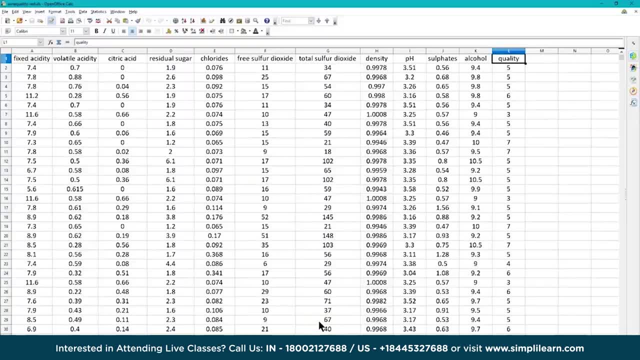 So it's a spreadsheet, A Microsoft spreadsheet, And when we open it up We'll see that it matches what we had before. As far as the slide was showing us, We have 12 different columns. The first 11 are our features. 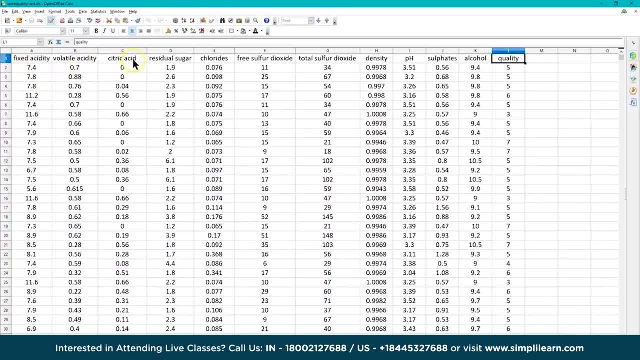 Our fixed acidity, Volatile acid, Citric acid- Things you always want to look at when you're looking at your data, And we've done this before in the part 1.. But just a reminder, We want to note that we have decimal places here. 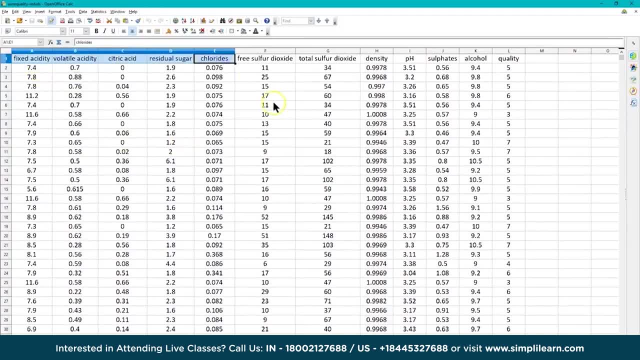 Float values, Especially the first number of columns. Our free sulfur dioxide looks to be an integer. Our free sulfur dioxide looks to be an integer, But it varies a lot. I see some values all the way up to 51.. 7, 4.. 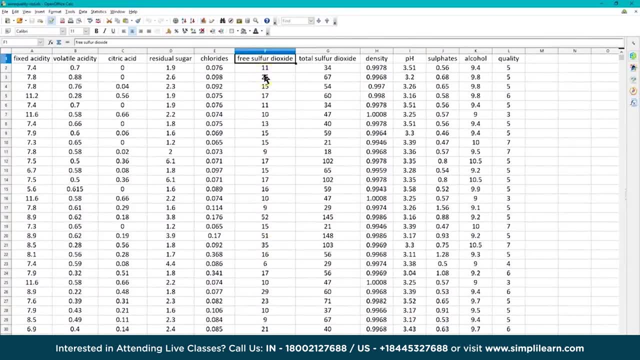 So we'd probably keep this as a linear model kind of thing. So we'd probably keep this as a linear model kind of thing. Same thing with the sulfur dioxide Densities- again Decimal places. Sulfides Alcohol Quality. 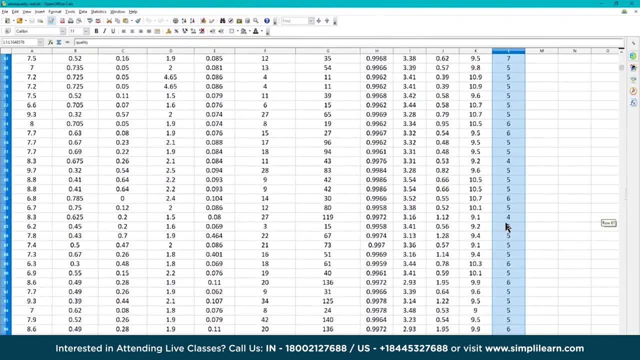 I want you to note in the quality That we only have a few qualities here, Like a spread between 0 and 100.. It looks to be 3, 4,, 5,, 6 and 7.. It looks to be 3,, 4,, 5, 6 and 7.. 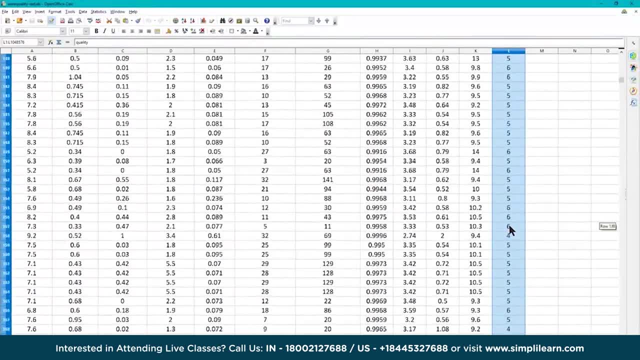 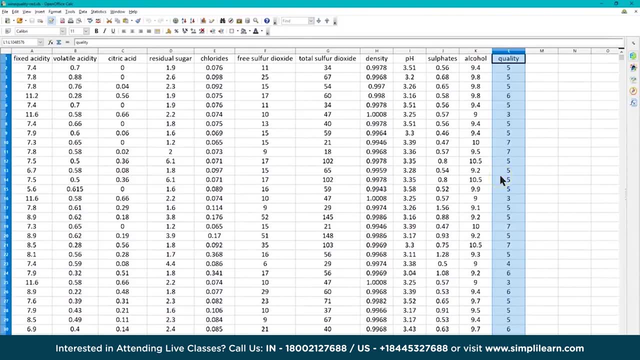 And so when we start looking at the processes, And so when we start looking at the processes, We can have the option of either doing this as a A series of integers Or float values going from 3 to 7. Or we can convert that to a categorical 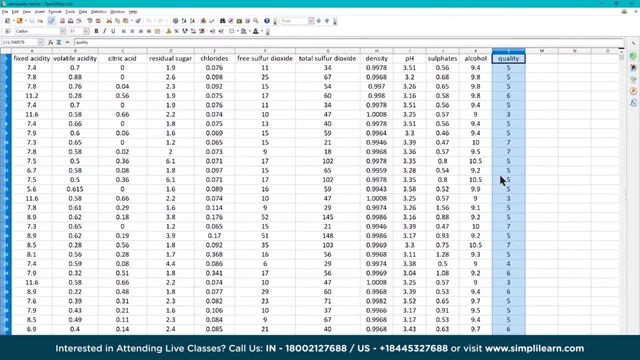 Or we can convert that to a categorical, 3,, 4,, 5,, 6 and 7 being the categories. But we'll look at that in the coding here in just a minute. But we'll look at that in the coding here in just a minute. 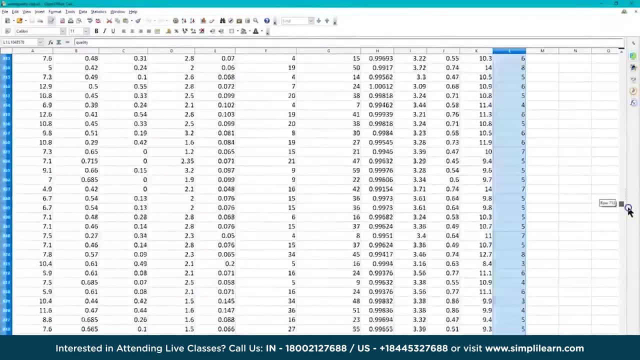 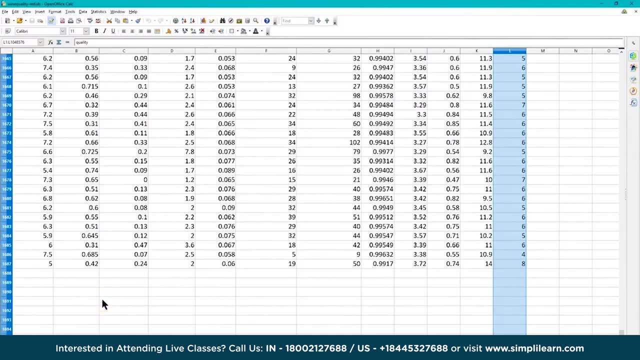 And finally, you'd want to go ahead And scroll down through the data for missing data or anything weird. obviously, working with big data, you wouldn't be able to do that if this was spread across numerous computers and you had millions of rows. we have what? sixteen hundred and eighty seven rows. 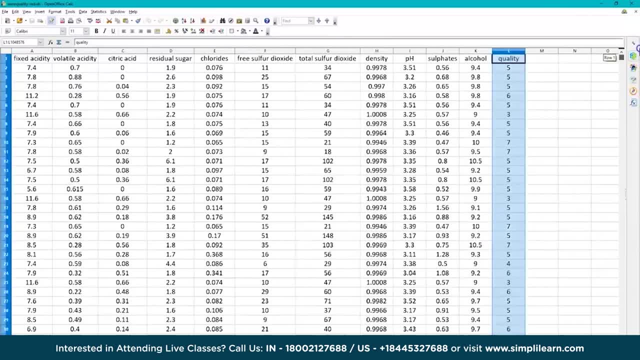 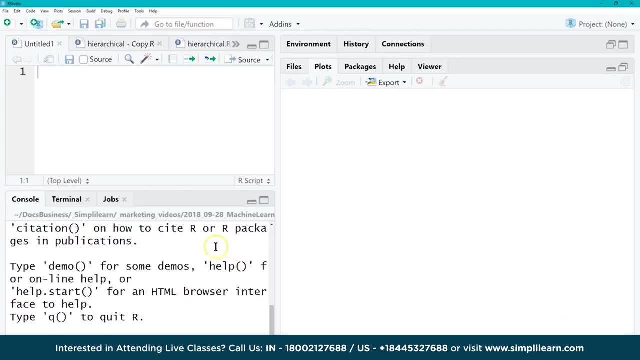 here. so it's a nice size spreadsheet, still considered a small data set. let's go ahead and switch over and let's take a look at this in the R. so here we are in our R studio and, if you remember, it's comes up automatically in three panels. I 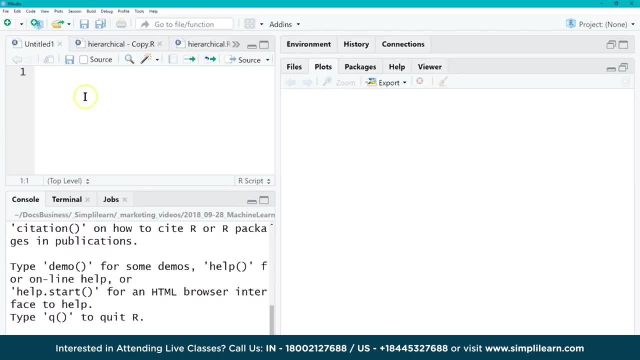 have my font on fairly large to help out. the upper left panel is a file that's opening them. multiple files and tabs open, as you can see on mine right now. I'll probably close most of those in just a minute and this is where you can put in your commands. then you can execute these commands by either. 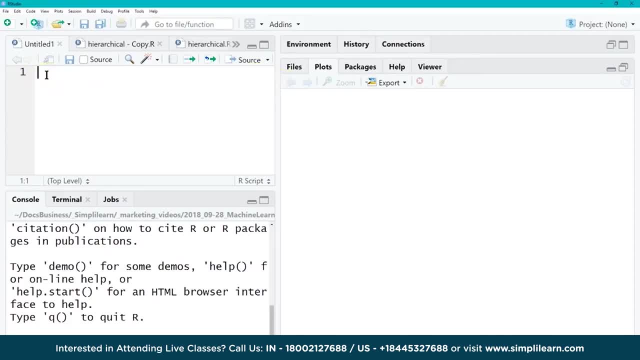 clicking on the run box or ctrl enter is the hotkeys for that- and all that does is then puts it down in the console and executes that line of command. you could just paste these directly into your computer and then you could just paste them in the console. I've certainly been known to do that. if I'm loading up some, 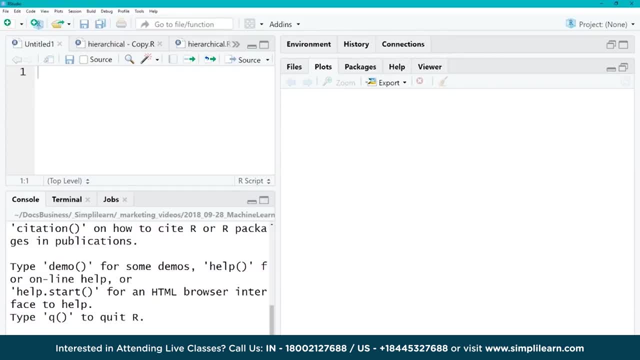 data and I just want to take a quick look at it in R because I'm doing the coding and something else, or if I just want to do a quick explore before I dive in and figure out what needs to be done. that's one of the tricks you can do, and 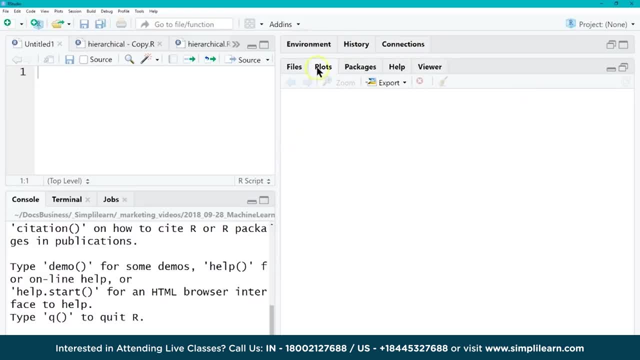 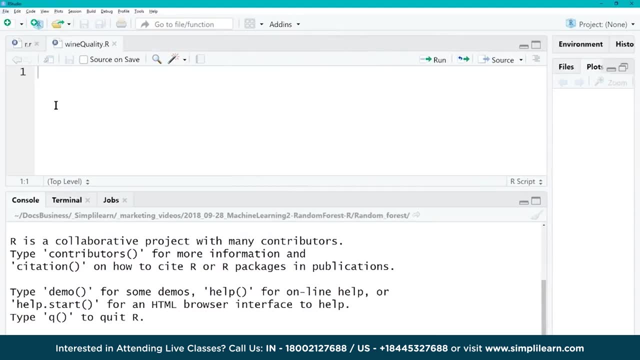 then, on the right hand side, we have our environment, history connections. we mainly are going to just be sitting on plots, and I'm just going to minimize this for right now, out of the way, while we dive in. if you haven't yet, you do need to go ahead and install the package random. 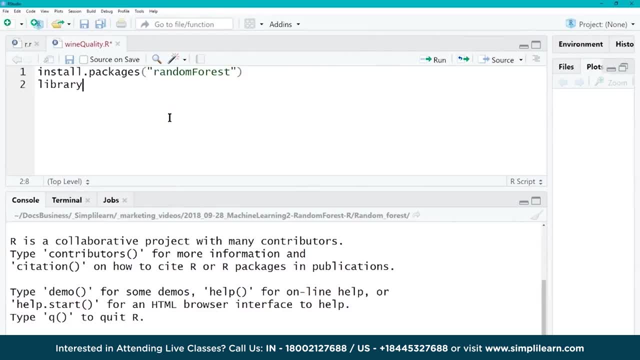 forest. I'm not actually going to do that because I've already run that. we don't need to rerun that. but I am going to go ahead and import it into our project with the library and then random forest. we'll do the ctrl enter. you can. 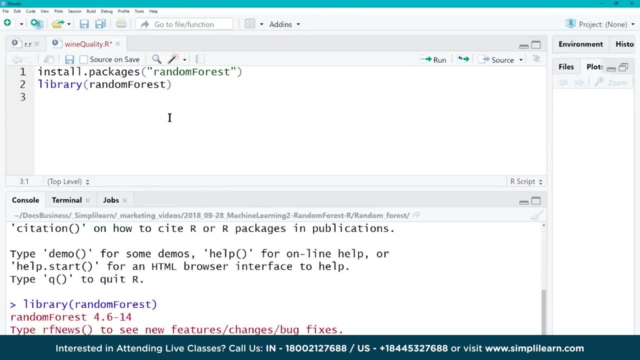 always hit the run button up there too, and then now the library has been uploaded in there and you can see down below, it takes us and just copies it and paste it down below and runs it in our console. and then just a quick troubleshooting thing: my Java happens to be the developers job. 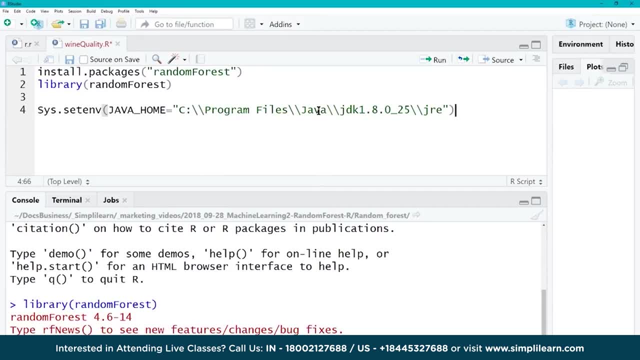 the latest release of the developers Java from last week is clashing with my R and rerouting my Java files, so your chances are you don't need to look this up or find out where your Java is, but there's a JRE folder. if you do have an, 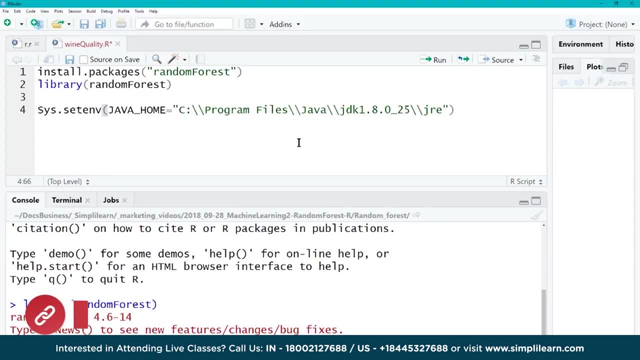 error that comes up next in the next library. you look that up- it's usually under program files, Java, and you'll see JDK, depending on what version you have on there, and then find that JRE folder and I'm just going to set the environment on there. you have to do that every time you run the script. 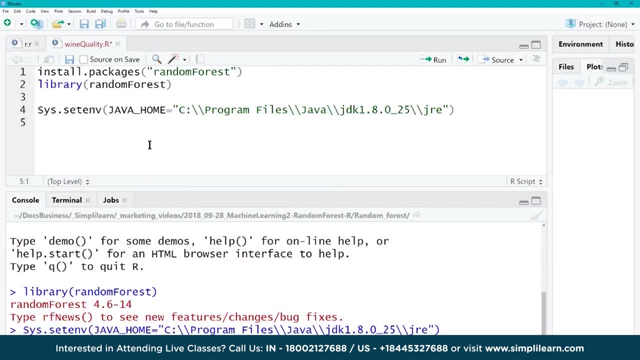 so with R. there is a place in R where you can set it permanently, but generally it's set to whatever your system variables are set to, so you don't want to mess with that. so you just want to put this in your code. if you're having 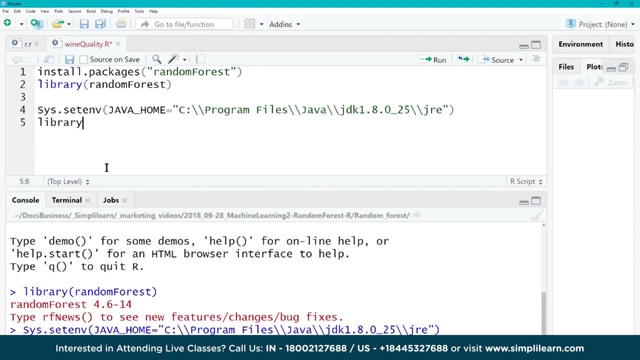 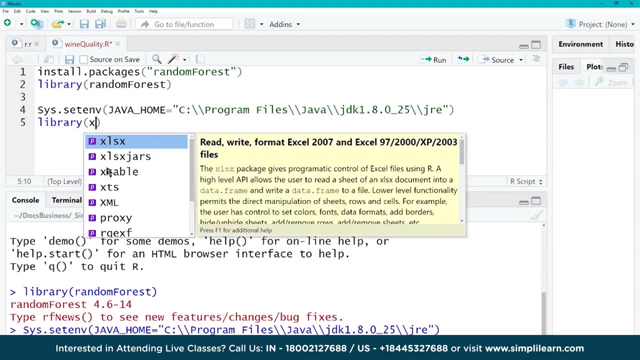 problems and you can always take it out. then we need to go ahead and bring in another library and we're going to be importing a the spreadsheet. so it's an X, the XLSX, since it's a Microsoft spreadsheet, and I'll go ahead and run. 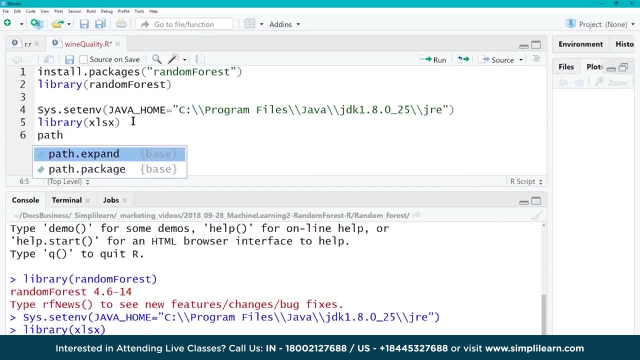 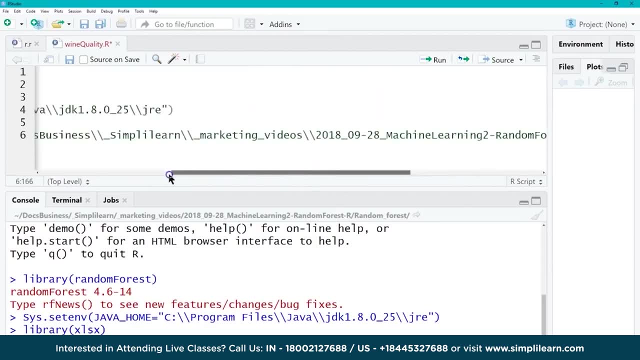 that let's go ahead and create a variable path. we're going to assign to variable path the location of our folder. so this is a very lengthy one. you'll have to copy and paste it off your computer. my name is Richard and you can see under it's, under C, column users: Richards. 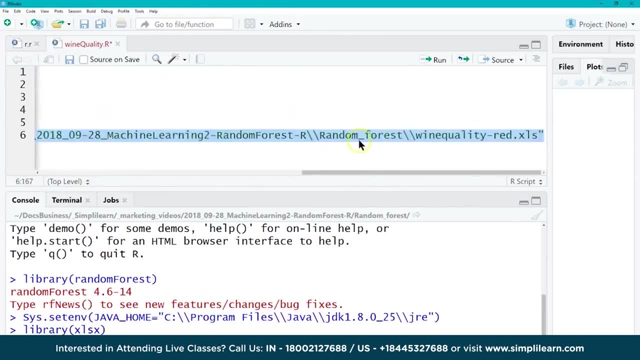 documents, Docs, business, simply learn, marketing, random forest, and then the actual file which is wine quality dash, red dot XLS. so I put in the whole path in here. you could also set the computer path to whatever folder you have it in and then just use just the name of the file. but I went ahead and did this. 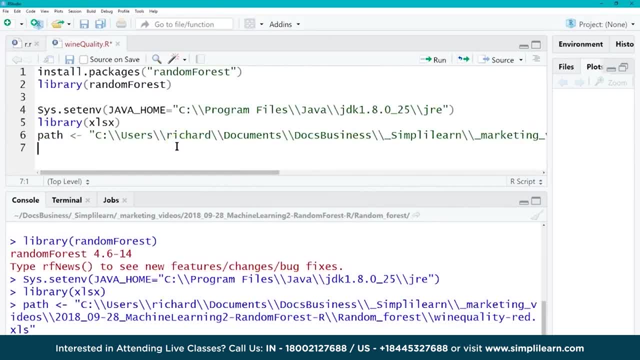 because it a lot of times it's good to be where your paths are going, where you're pulling your data from. and again it went the ctrl enter so I could you'll see that that pushed the line down below and ran that line, so our path is now set. 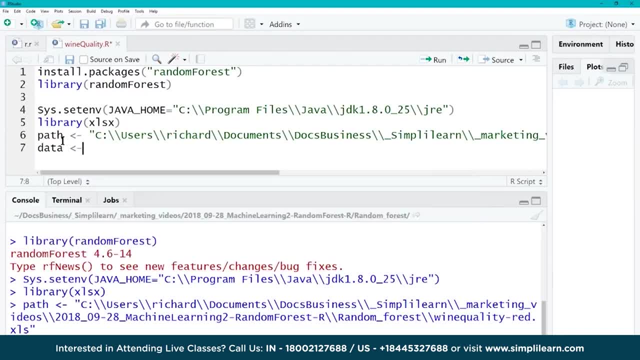 and then let's create a variable called data and we'll assign that to a read and we're going to be reading. see where is it there? it is um spreadsheet and then an. And before I put in, we need the path, but we also need one more thing on the spreadsheet. 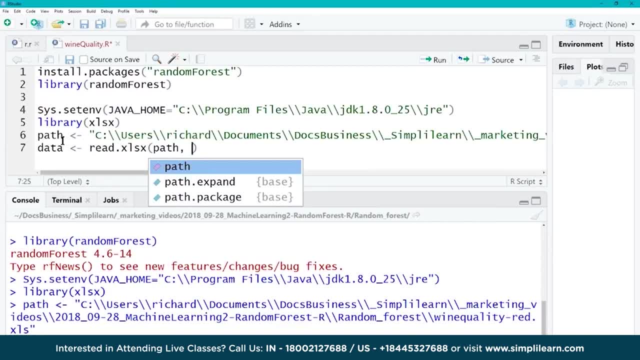 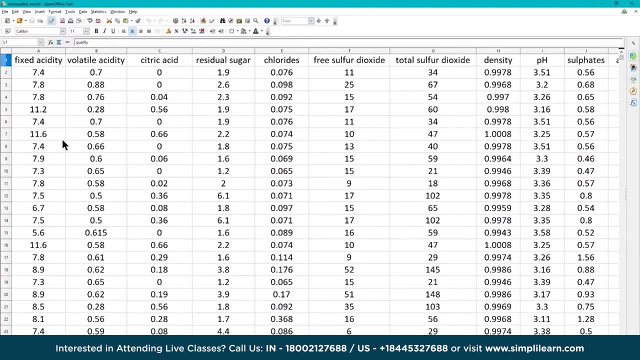 because it is an Excel spreadsheet. We need to know which page we're on. so let's go look that up. And in the spreadsheet this might be a little hard to see because it's a very tiny font down there, but you'll see the page tabs on the bottom. 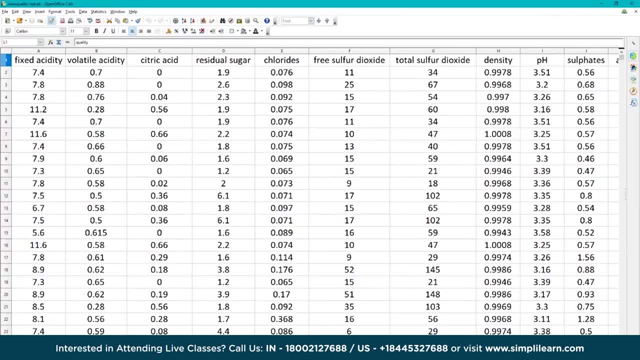 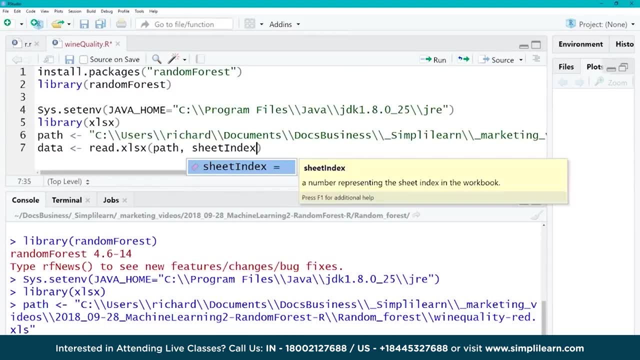 This actually has two different pages and we want page one for this project, So let's flip back over and put that in our code. The term they use is sheet index. I always have to look that stuff up and it was sheet index of one. 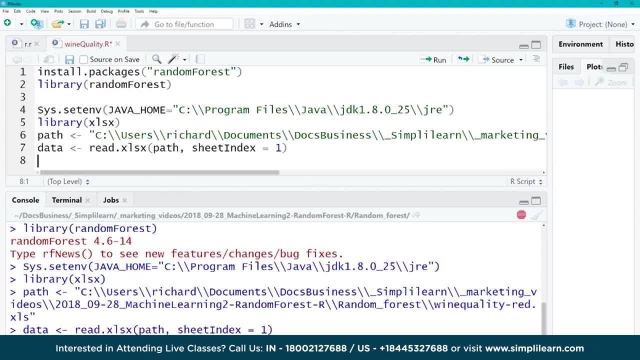 We'll go ahead and execute this. So at this point we've now loaded the data into the variable data and it's reading those in. I think there was, like you know, a couple thousand rows of data in there, so it takes. 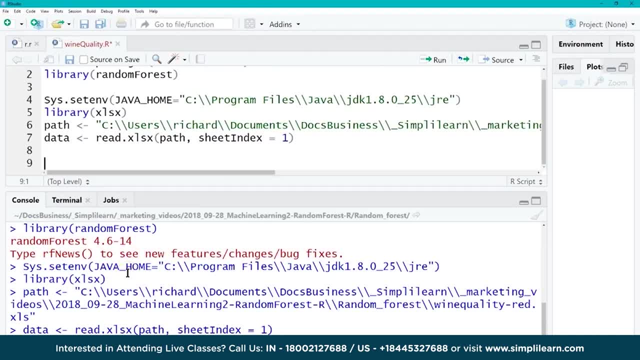 it just a moment to pull it in Once I have my data in there. I always like to do something like this data and in I always forget to do this. I always forget an R It's head data, and we can run that and you'll see it prints. out what we looked at in the spreadsheet. So we have our fixed acidity, volatile acidity, citric acid, residual sugar, chlorides, free sulfur, all the different things. We're actually looking for- quality. so you want to keep that in mind. that quality is. 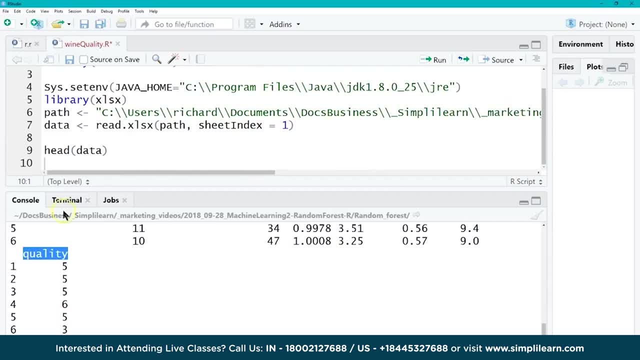 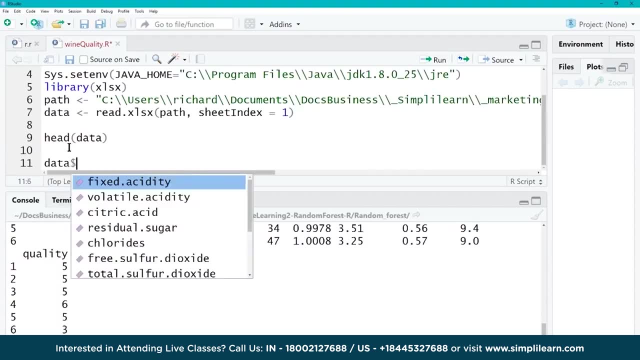 the final setting. Is it a three, four, five, six? What is the quality on there? And the first thing we need to do is we're actually going to take the data, The data quality, and let me see quality. there it is. 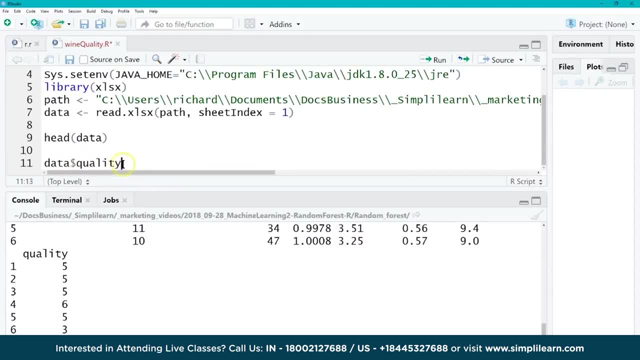 In R, the dollar sign means that you're looking at one of the columns in here, or features as it is. So we see data dollar sign quality in R. that means that's what we're going to be editing, And what we want to do is we want to change the quality just a little bit, and so we're. 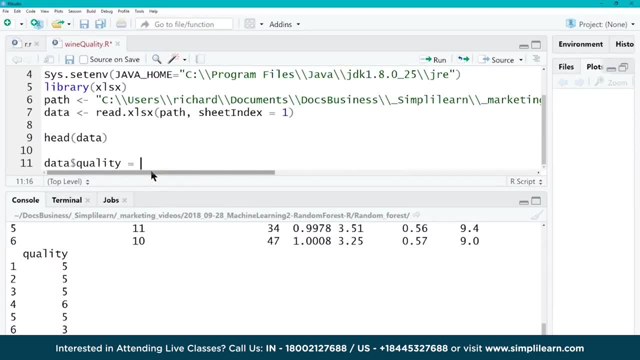 going to set it equal to now. we're not assigning a variable, we're altering it. so data dollar sign quality equals And we want to do as it's one of the functions in R and we're going to do as a factor. 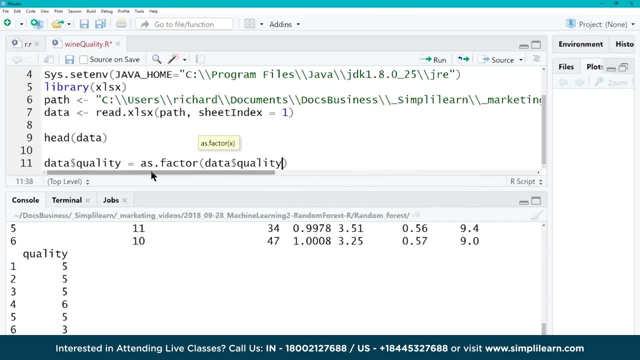 And then data quality, because that's what we're actually editing on there And let's stop just for a second and look at this. Factor takes this and looks at the data categorically So, instead of it being on a continual scale of zero to a hundred or something like that. 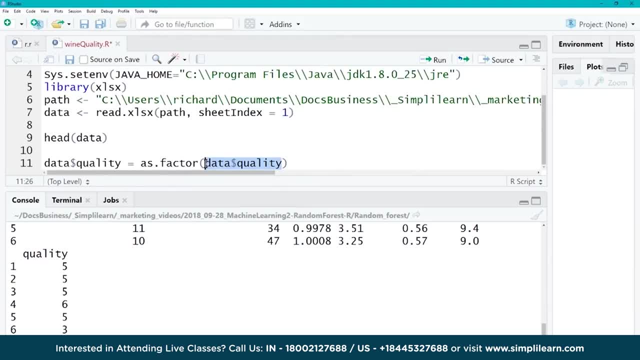 it actually looks at it as category of five, Category of six, category of A, category of cat, category of dog. They're yes or no categories versus a continual. Now, there's a lot of different things in here that we could do the same thing with, but 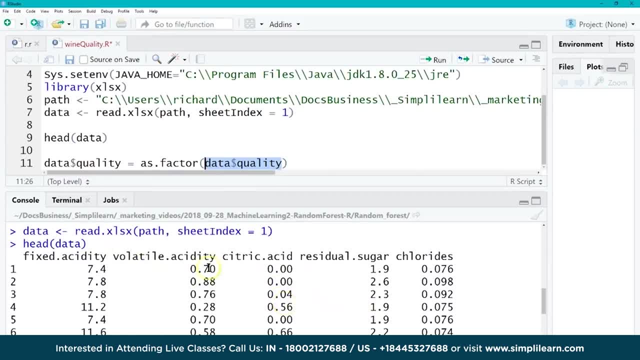 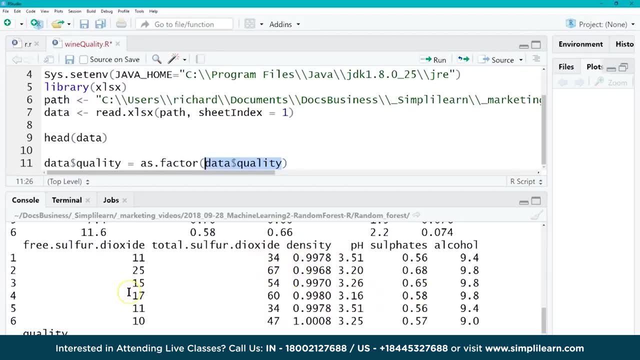 all of these really are linear numbers: 7.4, .70, sulfur dioxide: 34, 67.. So we really don't need to mess with any of the other variables in there, but we do want to go ahead and set this up. 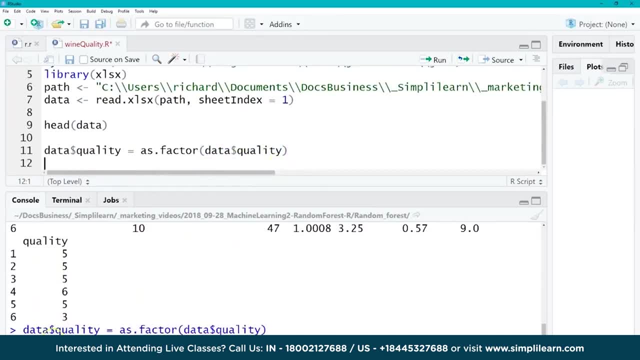 And we'll come up here, We'll do our control, enter and it'll run it down below and you'll see data quality equals as factor data quality. So we've now turned that into a factor or into a categorical data, And so let me just bring this down a little bit. 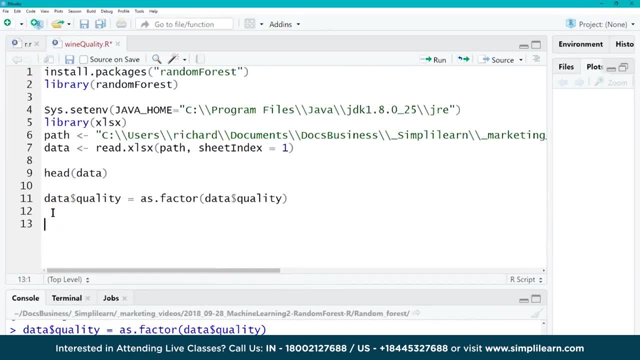 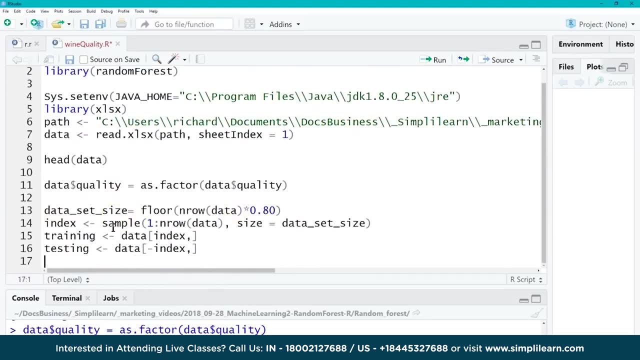 The guys in the back did the rest of this next piece of code. There are so many different ways And if you have been looking at any of our tutorials, this should look kind of familiar. This is one way to do it. You'll see, we have our training data and our testing data. 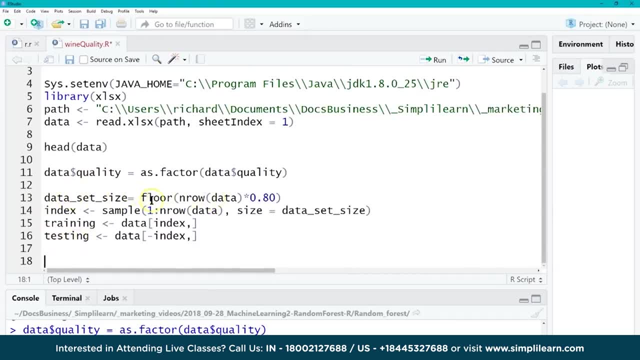 And so we've done here is: we've got it, We've got the data set, size equals and we're just going to do by the row, And so we want .8 or 80 percent of the data is going to be our training set to train our 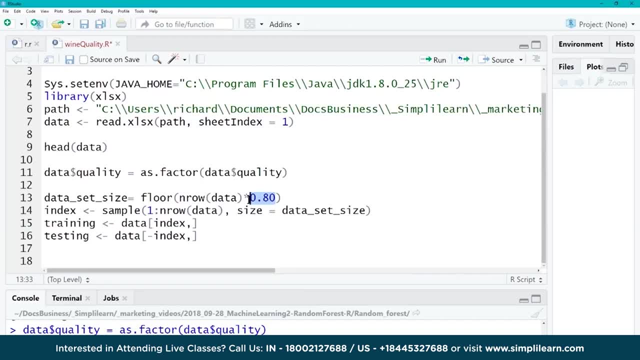 forest And if you train it forest or any machine learning model, of course, when to test it. So we're going to save 20 percent of the data for testing And when you look at this, we have the index which we set at 80 percent comma, and then 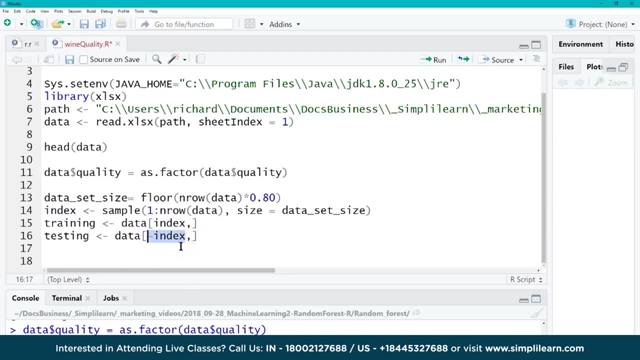 a negative index. So that's the remaining setup. So it goes from that index on. This is our notation for sorting out that data. And then we create the index and we use the term sample And this is just going to go in there and set our different samples for our in row size data set size and everything. 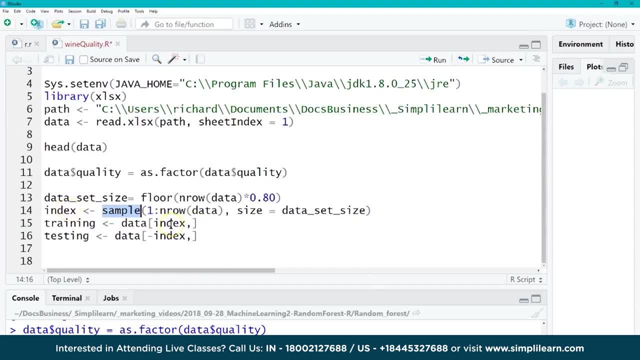 So we have an index now, So the data is indexed and we're just going to pull off the first set of index and the end of the index for our data And we can run all of this in one shot. We'll go under code and we'll run selected lines And so now we have our data in here. 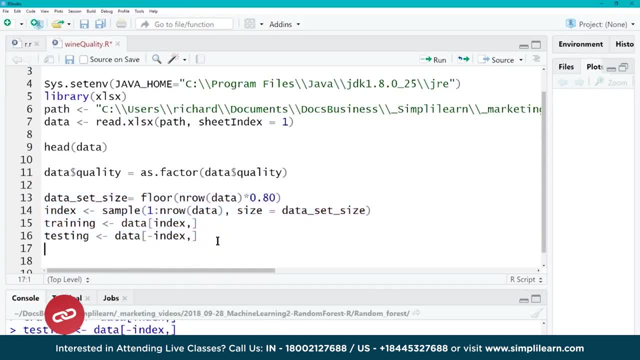 We have our training set and our testing set. That's what we wanted to get to. So once we've formatted all the data, then we get to the next real easy step, which is a single line to bring in our random forest. So let's go ahead and we'll use a variable. 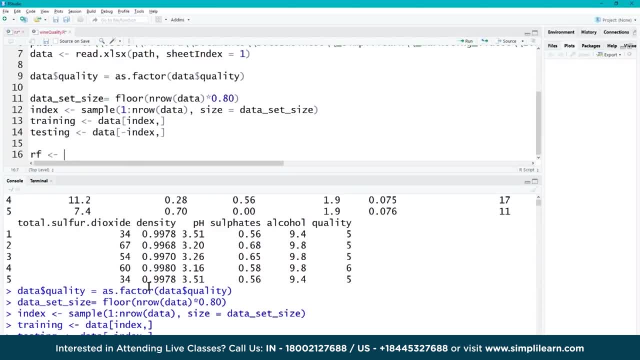 rf standing for random forest And we're going to assign. If you're going to do that, you're going to have to do a little bit more work on that. If you remember correctly, we brought in our library random. If you wonder why I go up, 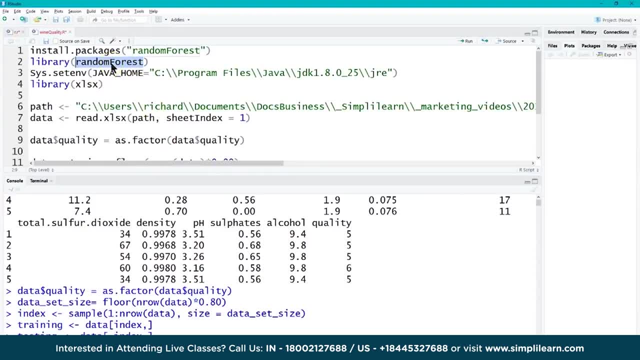 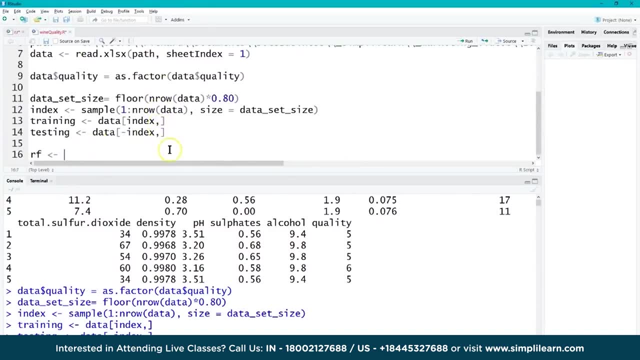 here all the time. it's because I'll forget which letters are capitalized in some of these because I switch between packages so much. But it's random with a capital F for forest, random forest. So the rf is going to equal random forest And of course we start by 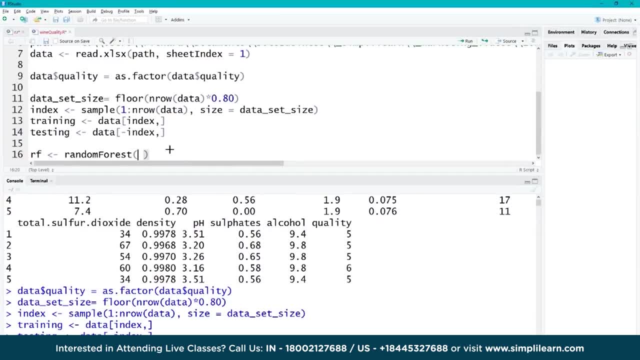 telling it which column we're trying to predict. And of course, you can always go down here and double check. We're running this on the right side of the screen And we're going to go down here and we're going to run a little test on the quality. there we go, Quality, and we're using just 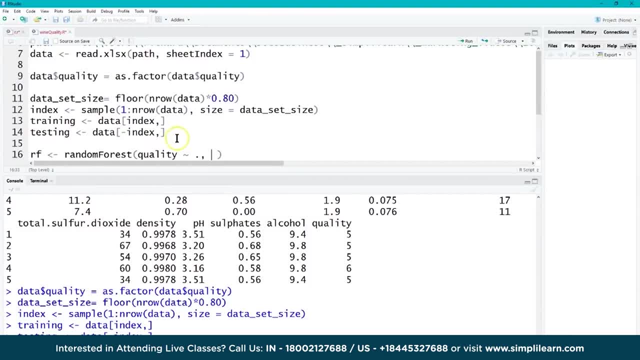 that column all the way to the end. And then we've added: our team in the back has gone in and played with this a little bit And we'll go a little bit over what they did. But I'm going to put in the values that they have set for the different options in the 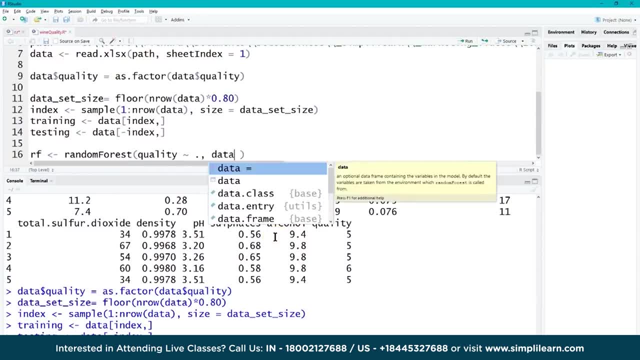 random forest. Before I do that, it would help if I tell it what data to use. Data's going to equal our training set. And then we have the variables that they put down here together and let's just talk a little bit about what these different variables mean. 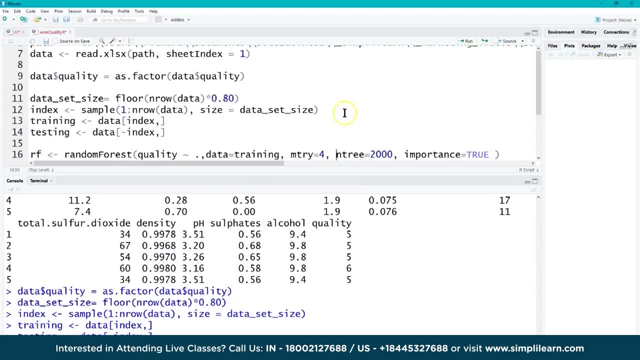 So mtri and intri, these are some of the variables you play with with the random forests. The mtri not so much. When they first put it out I think mtri was very common. 4 is a good value. 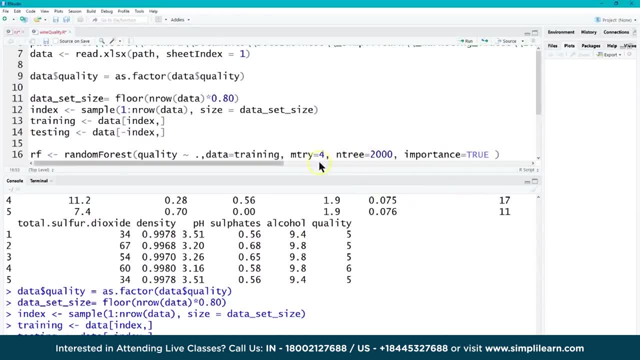 I can't remember what the default is, but it's probably 3,, 4, or 5, or something like that, depending. I think it depends on how many features you have going in there. So you could even just leave this as a default without too much troubles. The intri: this is where it gets. 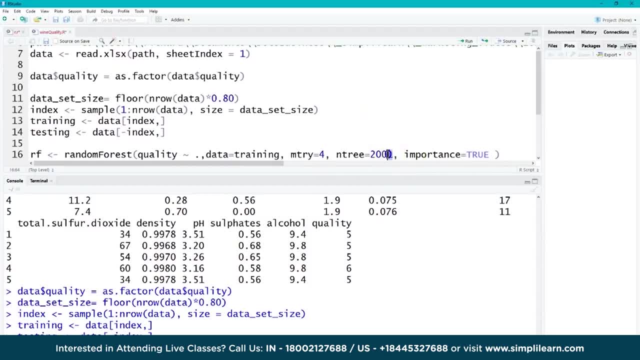 important and I'm going to make this 2001.. One of the suggestions is to always make this odd like a tiebreaker, just in case The default is like 500 or 501.. And then, finally, we have importance equals. true, I can't remember what it defaults to, but generally you want to set the. 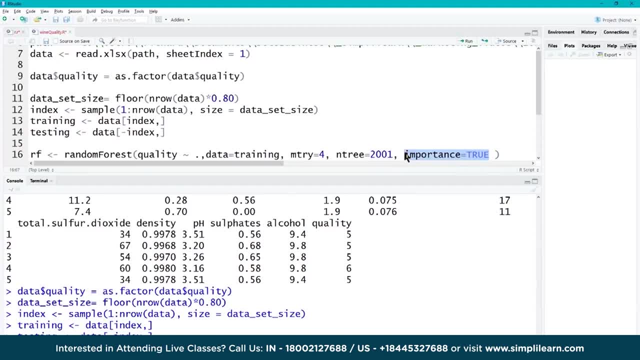 importance equals to true. It actually looks at the correlation between the two variables. So I'm going to make this 2001,. and I'm going to make this between the different features to make sure that there is some kind of correlation, as it's doing. 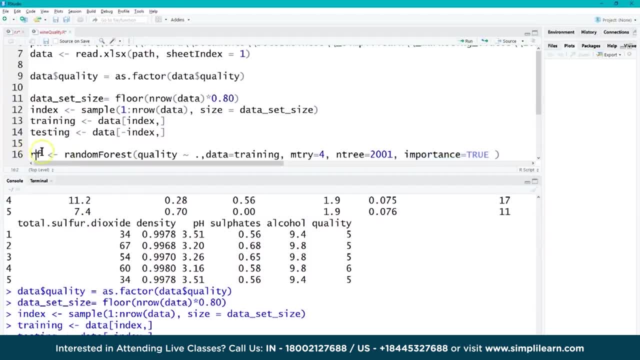 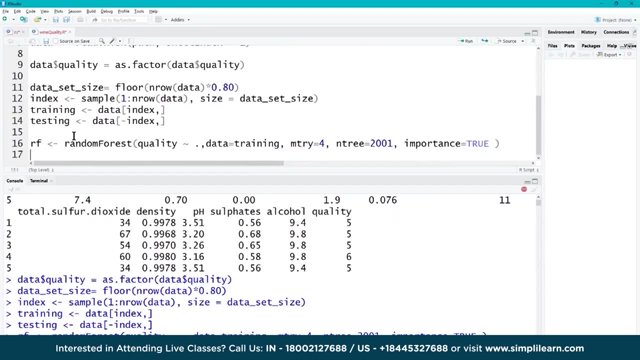 its calculations. So our one line of code is going to assign a random forest and go ahead and train a random forest, all in one execution. So this whole thing has been centered around getting to RF set to the random forest And let's go ahead and execute this variable or this line of code. 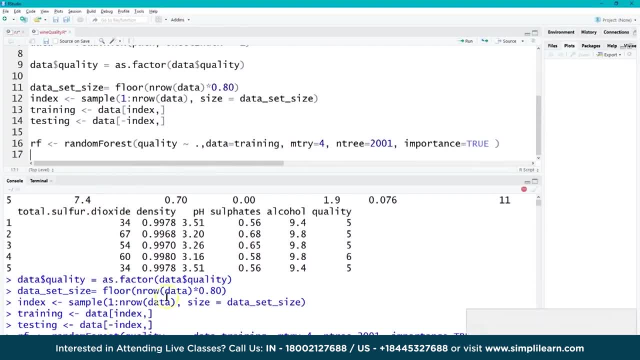 And you'll see it takes a little bit down here to execute as it goes through and sets it up. And you'll see it probably takes a minute or so to execute the code, depending on the size of the data and how good your machine is. And then, with all of our data, we can start looking at the 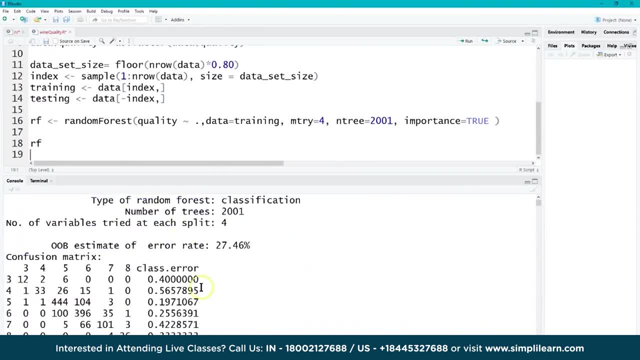 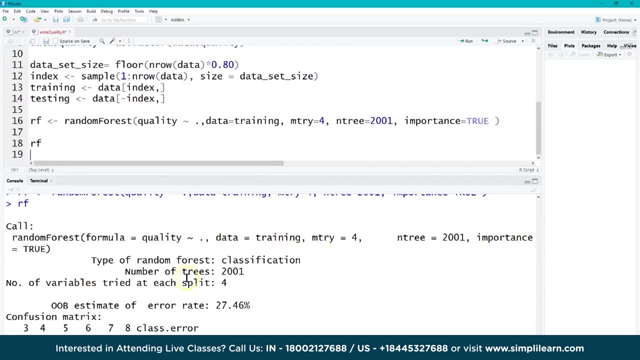 answers. We'll just do RF, We'll execute that And you'll see that the random forest does a nice job. You can see right here. it has our data, equals training. It basically goes over everything we talked about And you come down here and it has a confusion matrix, which is nice. We always 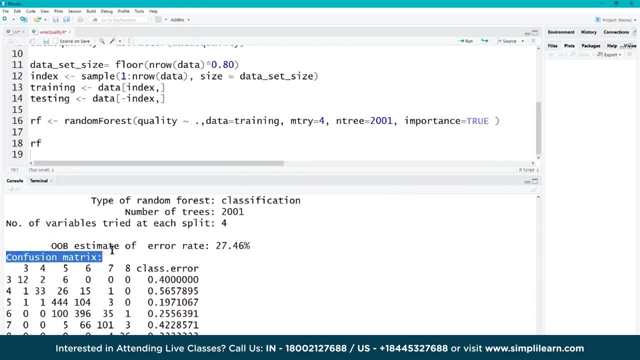 like our confusion matrix. So we're going to go ahead and do that, And we're going to do that When we're talking to our shareholders and explaining what the data comes out with and how it trains, And we can go ahead and plot our RF. Let's see what that looks like And as the number of 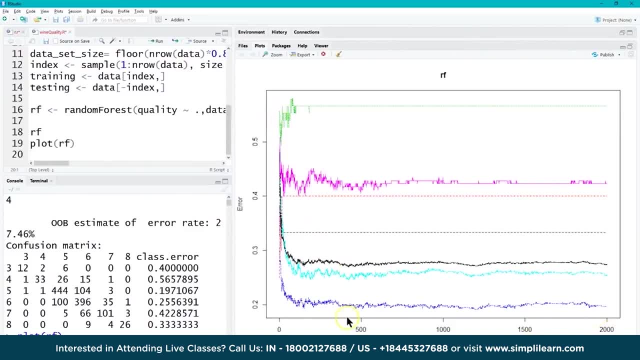 forests grows- remember we set it to 2001- forest. you can also see how the error comes in, how the different error on the different variables. This is kind of a nice graph that gives you an idea. It might help you adjust whether you really want to do. 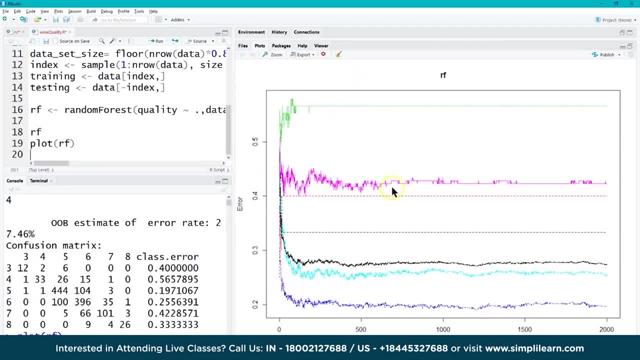 this. Let's say we're talking about about 200,000 different forests. You might actually truncate this off at around maybe 800, because you notice the lines kind of continue on Again. this is just still on the plot And of course the next step is we need to go ahead and predict, Remember we? 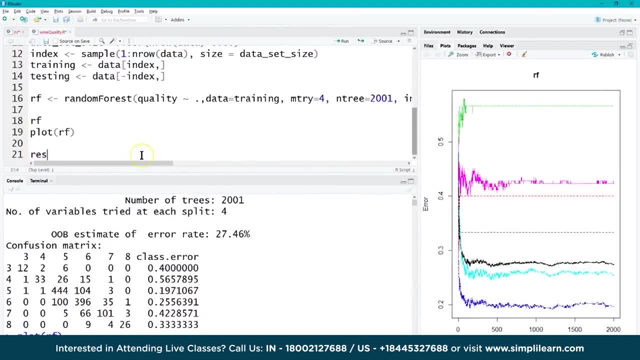 split our data into two groups. So let's go ahead and get a result. We'll call it result And we'll assign this one. There we go. We'll set this to a data frame. There we go. There's our data frame. 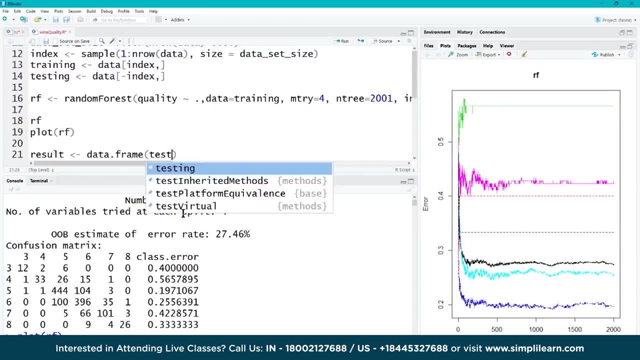 And then- oh, let's call this, we have our test, Our test quality, because we're we're setting up on our test group but the quality um on there. Then we want to have a predict, A nice little keyword there to go and run our random forests, And then we tell it that we're going to predict using our RF. 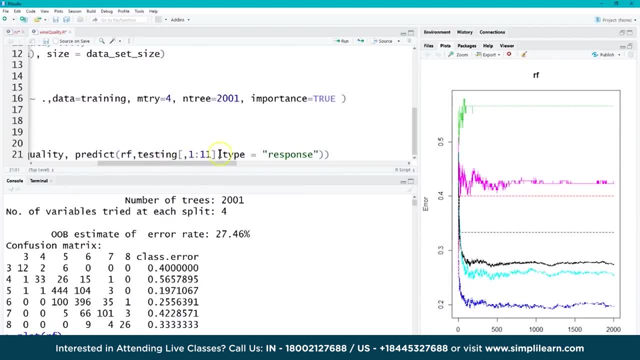 our random forest, our testing group. One to 11 is what we're using. type equals repeat, Minus the number of those hijacked. one to 10 is what we're using. Type equals repeat. And so you see, we come off our test. 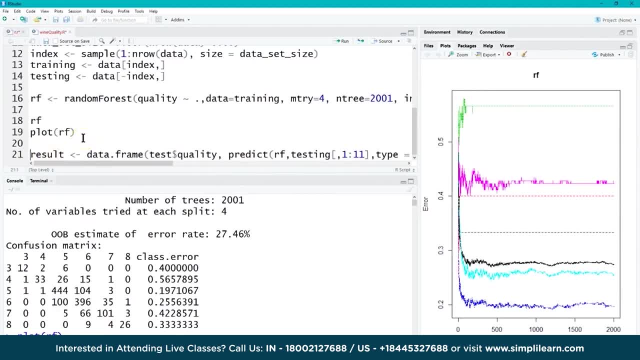 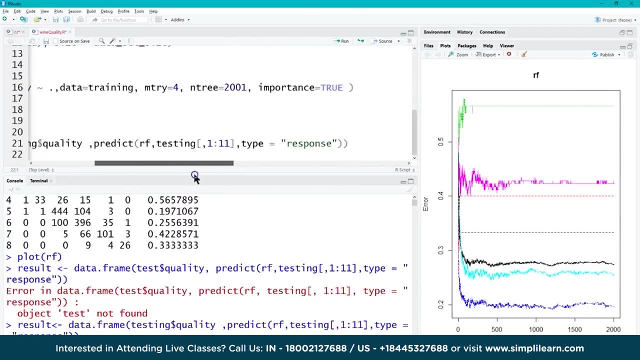 group, and I know that our test group isn't going to feature the value we set, but rather we're going to equals response. so let's go ahead and execute it. that's a mouthful on there. somewhere I left out a comma in there so it gave me an error, but you can see. 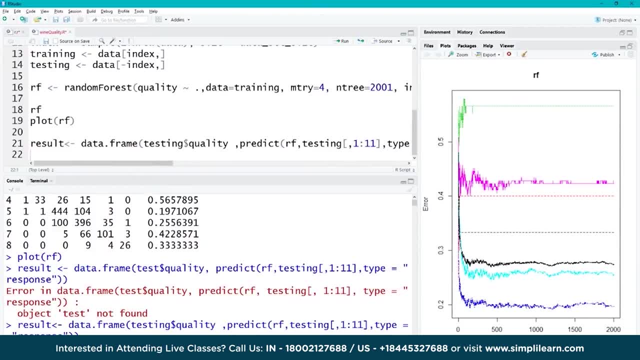 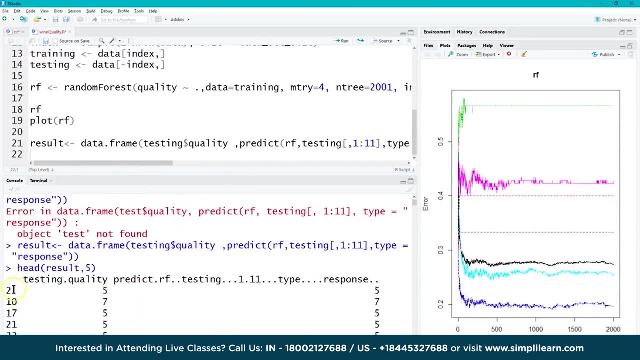 right here we've set in there. now we have a result and just real quick we could do the head of the result, result, comma 5, and just take a look at the first five lines and you'll see. we have the actual value and what we predicted. 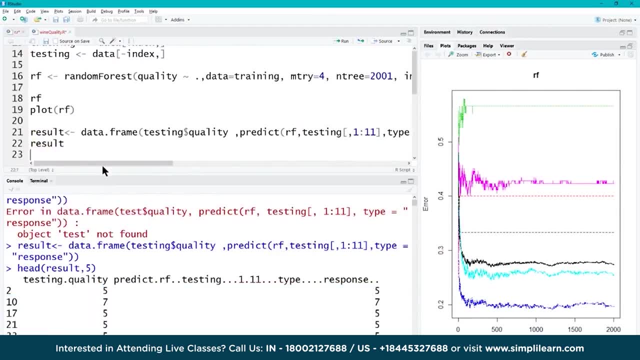 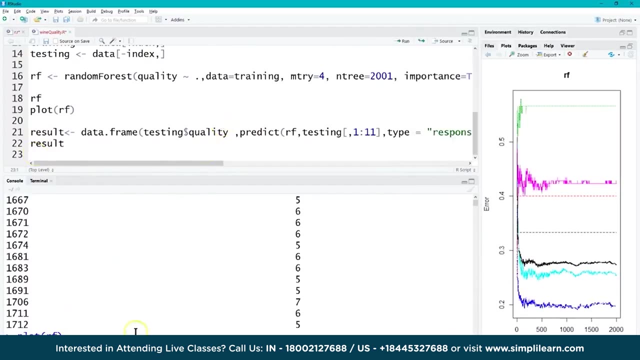 over here and we could also just do all of the result and just see what that looks like. oops, and print that out and so it has all the different data we're going through on there and finally let's just go ahead and plot. there we go, put plot up here, plot let's. 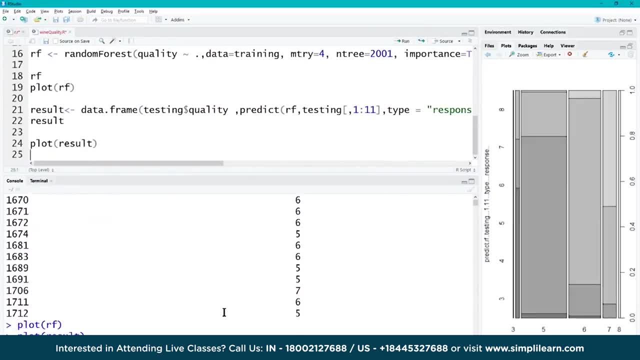 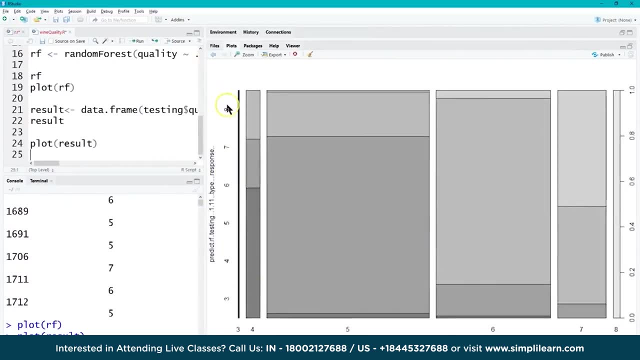 plot the result and just see what that looks like. maybe not the best one to show to the shareholders, but does give me an idea. on the left, on the y-axis, you'll see the that it predicted 8 and this tells you that a lot of the 8 and the 8 scale was 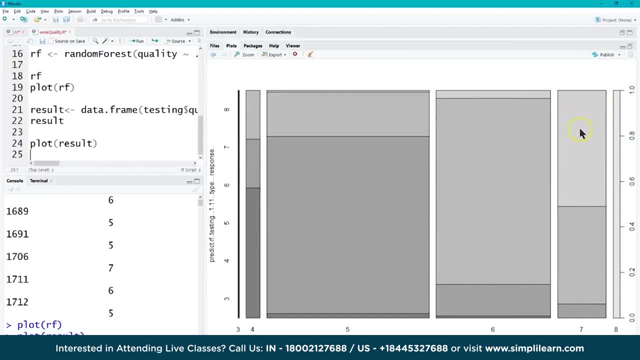 pretty probably gave us about 50%- came up there at 8- really maybe 50%, it didn't guess right- but it did come up there and say that it was at least a 4, 5 or 6, even where it was considered an 8 and so on. you can see these different blocks coming. 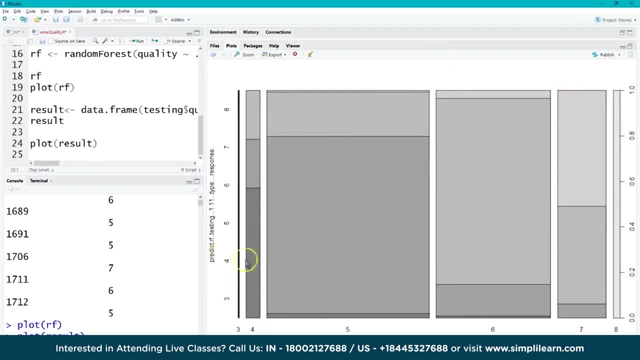 in so that if you line up the 3 with the 3, 4 with the 4 and you kind of cross index them, heatmap would probably do better. but for this example we'll just do a quick plot of the data as far as how it works and you can again see the results that we 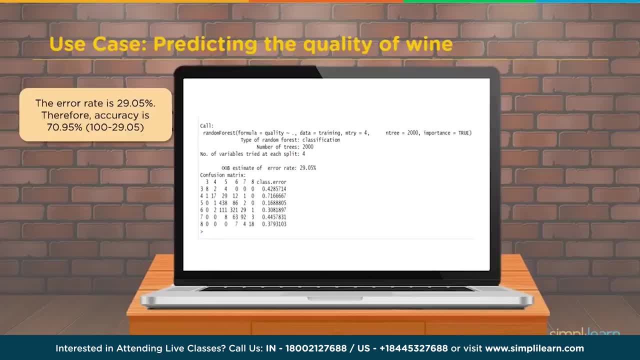 predicted over here and you can look those over, of course, back in the wine cellar we're talking to our vineyard owner and remember from before, we looked at this chart right here the error rate is 29.05 percent. therefore our accuracy is seventy point nine five percent. if you're doing a 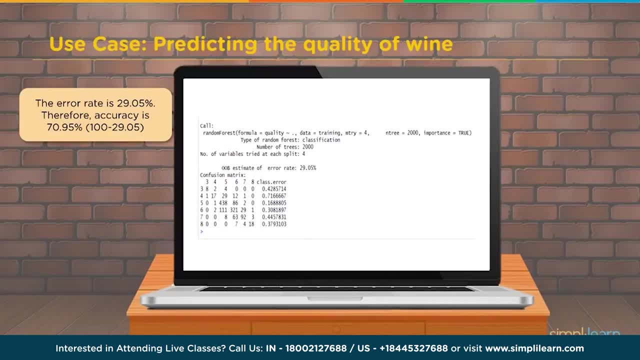 vineyard is probably pretty good accuracy, and always check your domain when you're sharing this stuff, because if you're doing something this life-or-death, maybe seventy percent accuracy might not be so good, but if you're looking at where you're going to distribute the bottles to for the wine and who's going to drink it, you know. 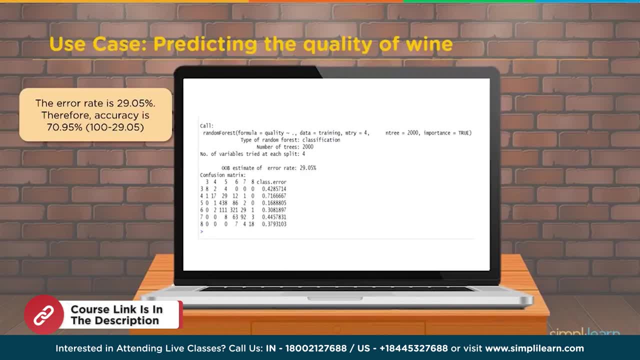 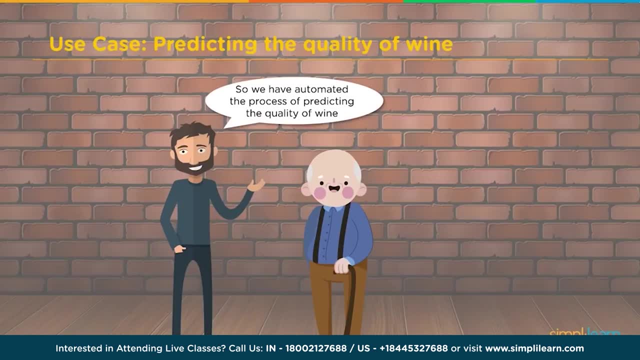 seventy percent accuracy is pretty good for that. that's probably a lot better than having no accuracy whatsoever and not even knowing what wines going out to who. so we have automated the process of predicting the quality of wine. I myself prefer to predict it by sampling it. that's great. 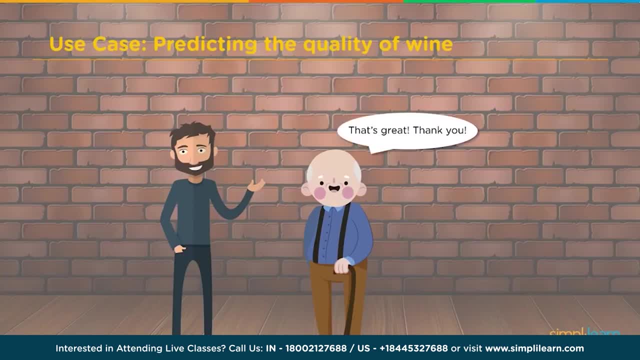 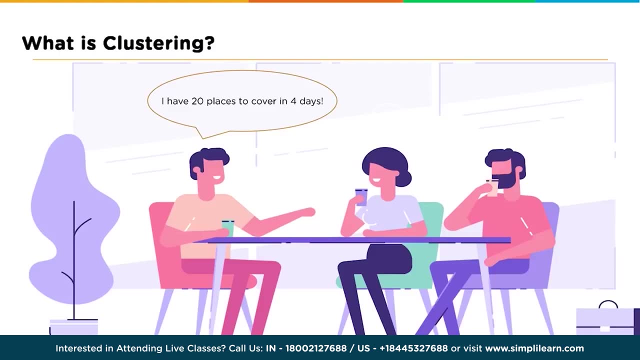 thank you. I'd like to visit this guy and sample his wine and find out just how good his different vineyards are. what is clustering? so we'll have a group of people here hanging out at a table or local coffee shop- i'm guessing coffee shop, since they all have the same mugs and one of them is trying to figure out. 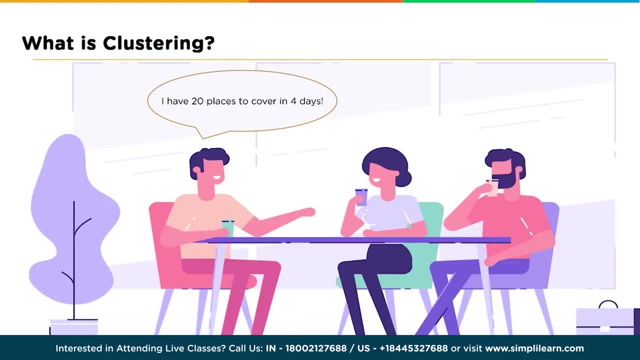 what they're going to do. I have 20 places to cover in four days. I guess he's going traveling- that sounds fun, one of those breeze through Costa Rica or visiting the US or going to to Europe to go visit all the highlights. she's got 20 places. he wants to go and he wants to. 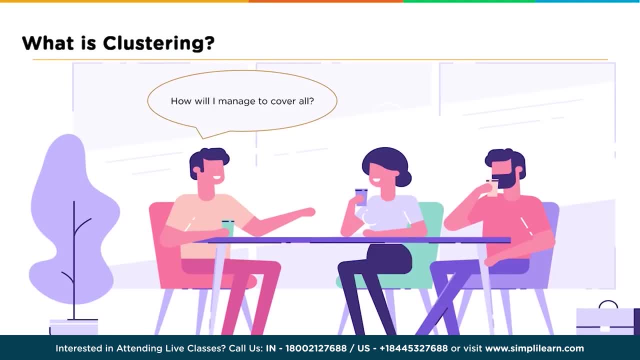 hit him in four days. very ambitious, and how will I manage to cover all of them? that's the question that he's coming up. how am I going to get to all these different places in the short time I have? maybe he's a sales team, so he has. 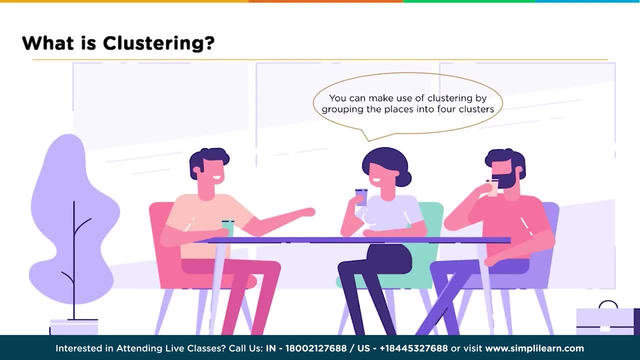 20 places he's got to do demos for. you can make use of clustering by grouping the places into four clusters. each of these clusters will have places which are close by, so we're going to cluster them together by what is closest to the other one. then each day you can visit one cluster and cover all the places in. 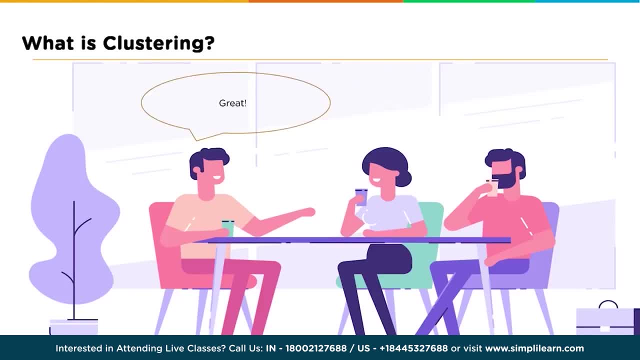 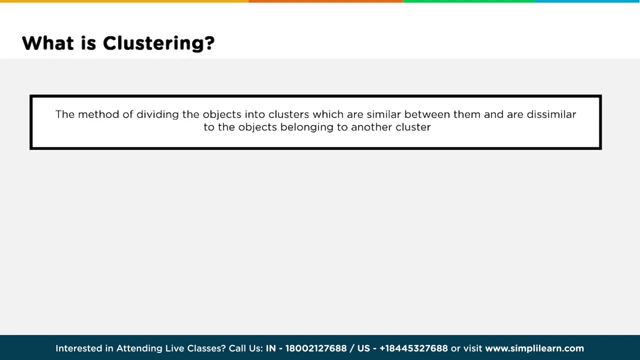 the cluster. great, that's a great idea. you know, if you're going to hit four different places, maybe you're going to cluster whatever streets are closest together, so you don't have to travel, spend all your time traveling. the method of dividing the objects into clusters which are similar between them and are dissimilar to the 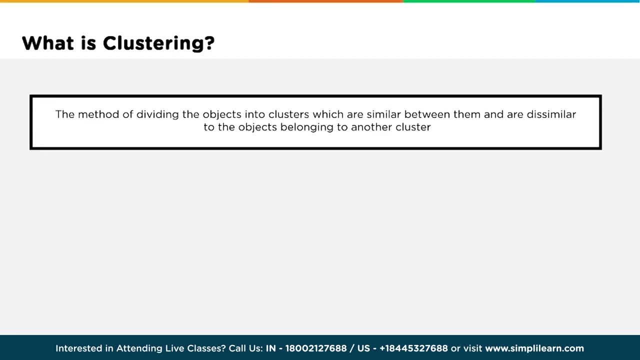 objects belonging to another cluster. so this is a formal definition of clustering and we have here. we have what we call hierarchical clustering and partial clustering, and we're going to go more into detail on hierarchical clustering and you'll see the difference between the two are: partial clustering doesn't have the descending graph, it just has groups of things and 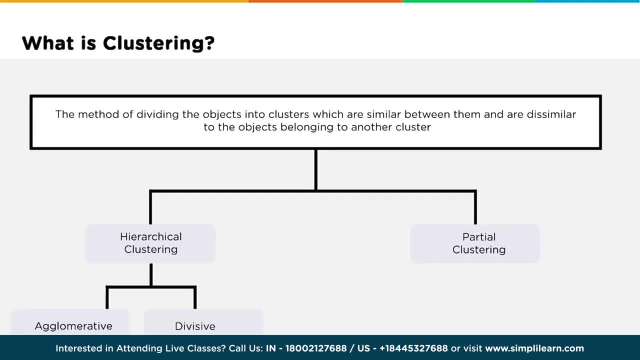 under hierarchical clustering we're going to go over a glomerative and divisive- and you can think of a glomerative, of bringing things together, and divisive as dividing them apart, and then partial clustering. the two most common ones are K means- that's probably the most common use for partial 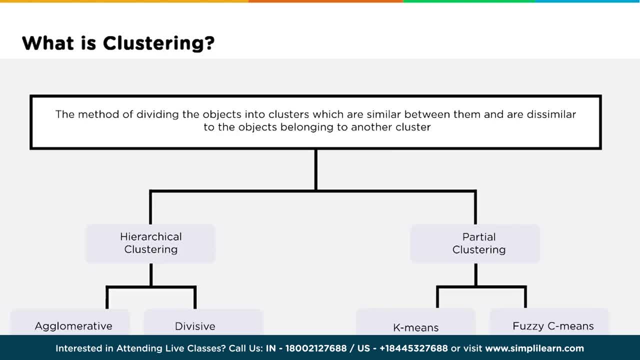 clustering. there's also fuzzy C means and there's other ways of clustering and other algorithms out there, but these are the two big ones, K means really being the most common one used, but we're not going to dig too deep into partial clustering because we're studying hierarchical clustering today. so 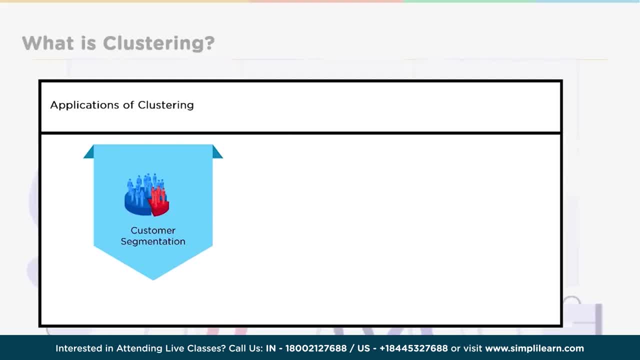 what is clustering? well, the applications of clustering are pretty numerous. we have things like customer segmentation: what people kind of belong together? how do we group them together? we have social network analysis. so social networks, we might look at sentiments. what group of people like something? what group of? 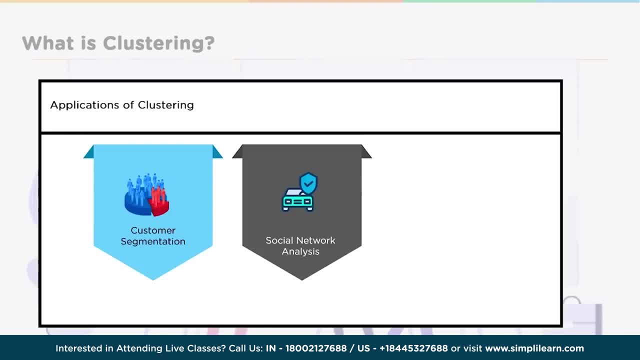 people don't like something and then we can use that sentiments to suggest new sales for them. you know this whole group is into Harley-Davidson motorcycles so we cater to them to sell them Harley-Davidson motorcycle parts. and we find out that people in that group also like leather jackets. they also like 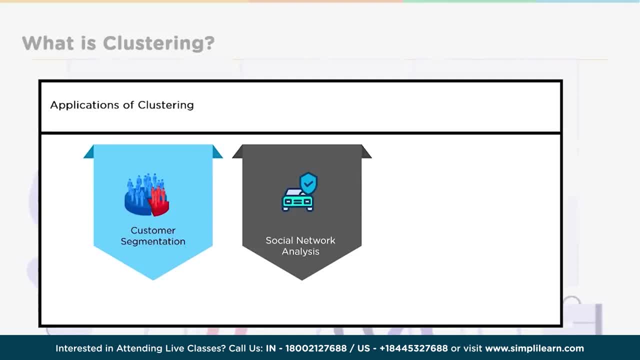 motorcycle boots and they like bandanas my brother's into Harley-Davidson. so that's why I picked that kind of funny example. but you can kind of see, we look for similarities between these people and then we group them together accordingly and that's a good sentimental clustering is very common in 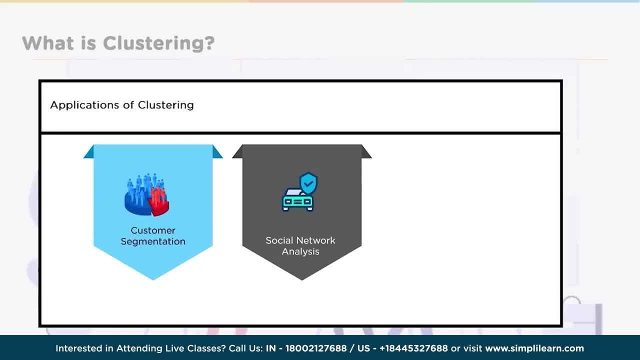 so many things today. we want to know the sentiments on stocks. who is interested in stocks? who's not? sentimental analysis: we talked about customer segmentation and sales. well, we want to know what kind of sentimental view people have on different restaurants. if we're gonna open up a new restaurant or a new, putting stores in and 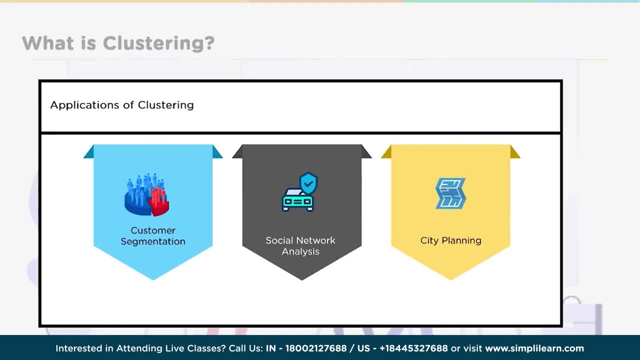 of course, city planning, a lot of this. I just kind of aimed at the city planning side sitting. planning is big with clustering. we want to cluster things together so that they work. we don't want to put a industrial zone in the middle of somebody's neighborhood where they're not going to enjoy it, or have a commercial zone right in the 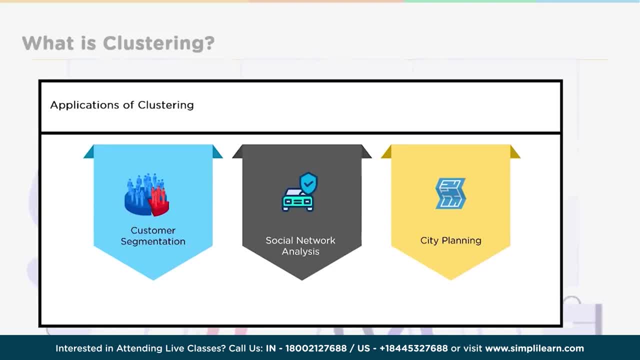 middle of the industrial zone where no one's going to want to go next to a factory to go eat a high-end meal or dinner. so it's very big in city planning. it's also very big in just pre-processing data into other models. so when we're exploring data, being able to cluster things together, reveal things in. 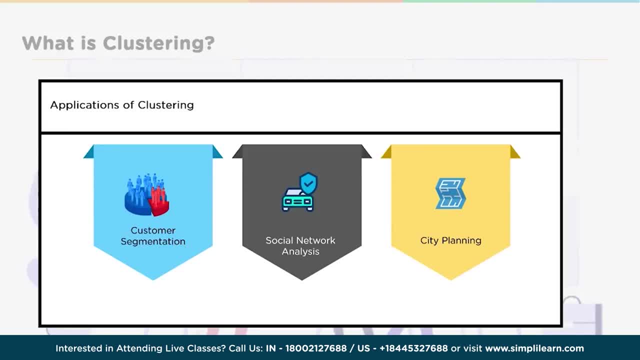 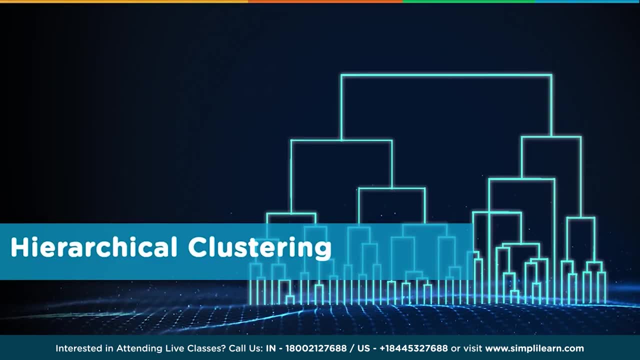 the data we never thought about. and then, once we have it clustered, we can put that into another model to help us figure out what it is we want for our solution. so let's go a little deeper into higher kill clustering. let's consider we have a set of cars and we have a group similar. 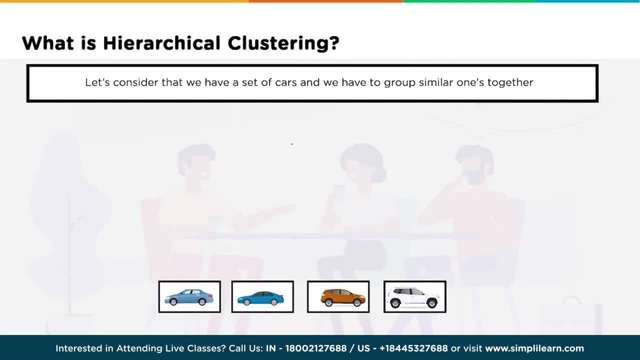 we want to group similar ones together. so below we have- you'll see four different cars down there- and we get two clusters of car types: sedan and SUV. so if you're just looking at it you can probably think: oh yeah, we'll put the sedans together and the SUVs together and then at last we can group everything. 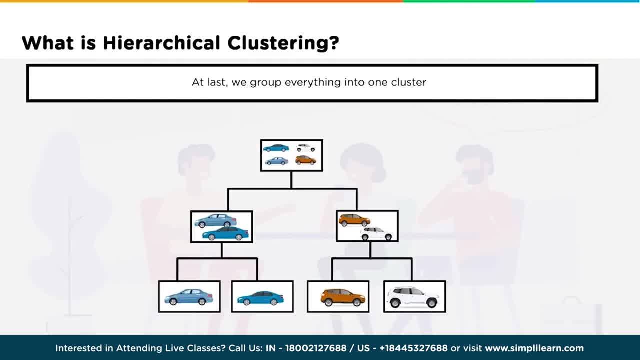 into one cluster. so we just have just cars. so you can see, as we have this, we make a nice little tree. this is very common. when you see anybody talks about hierarchical clustering, this is usually what you see and what comes out of it. we terminate when we are left with only one cluster. so we have, as you can see, we. 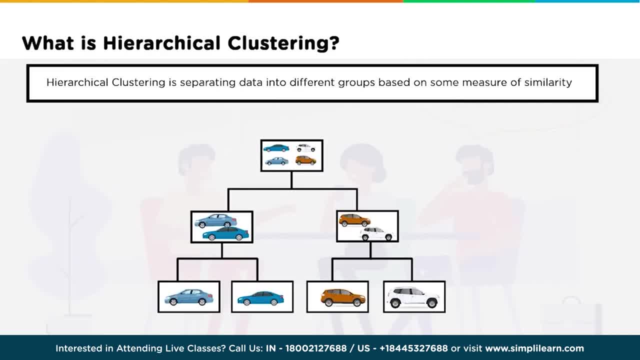 bring them all together. we have one cluster. we can't bring it together anymore because they're all together. hierarchical clustering is separating data into different groups based on some measure of similarity, so we have to find a way to measure what makes them alike and what makes them different. 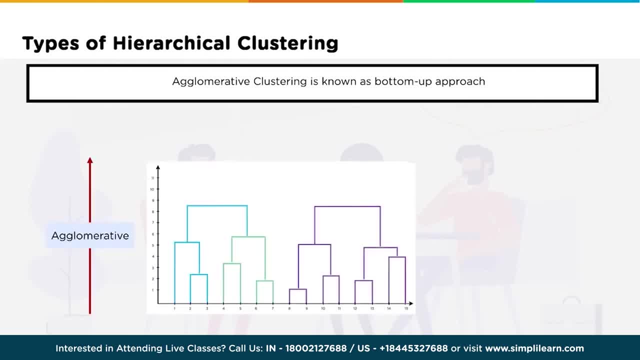 agglomerative clustering is known as a bottom-up approach. remember I said: think of that as bringing things together, do you see? think? the Latin term I glow is together because you have your glomerate rocks, where all the different pieces of rocks are in there. so we want. 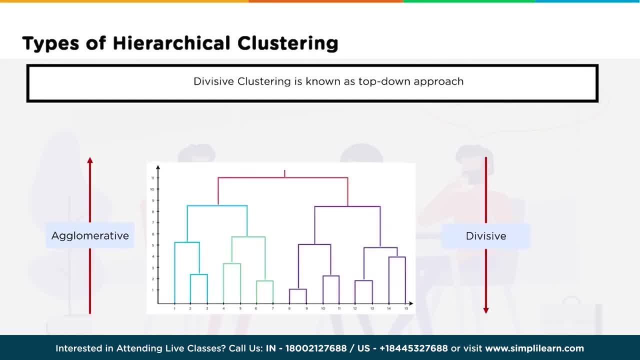 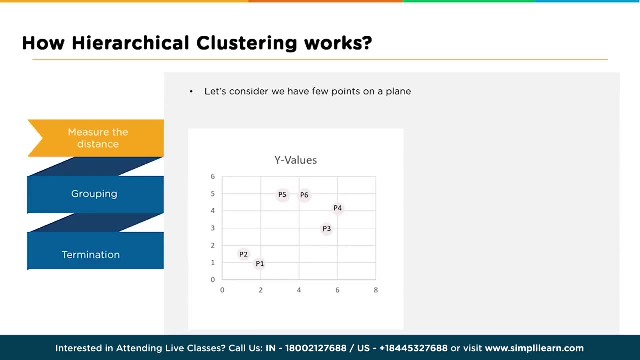 to bring everything together. that's a bottom-up and then divisive is. we're going to go from the top down. so we take one huge cluster and we start dividing it up into two clusters, into three, four or five and so on. digging even deeper into how hierarchical clustering works, let's consider we have a few points on a. 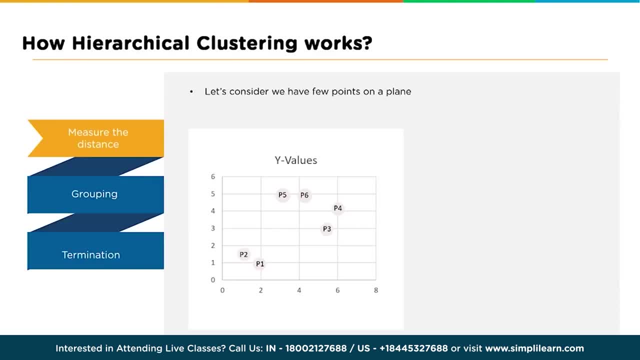 plane. so this plane is 2d y-coordinates. kind of makes it easy. we're going to start with measure the distance, so we want to figure a way to compute the distance between each point. each data point is a cluster of its own, remember, if we're going from the bottom. 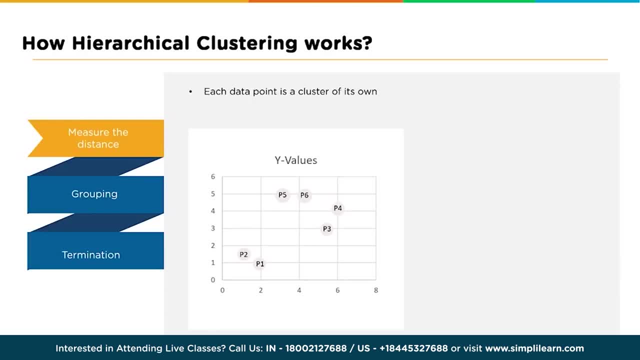 up agglomerative, then we have each point being its own cluster. we try to find the least distance between two data points to form a cluster and then, once we find those with the least distance between them, we start grouping them together, so we start forming clusters of multiple points. this is represented in a tree. 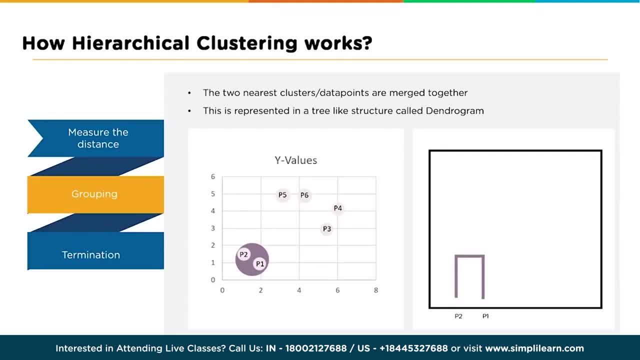 like structure called dendogram. so there's another keyword, dendogram, and you can see it is. it's just a branch we've looked at before and we do the second group of the same, so it gets its own dendogram, and the third gets its own dendogram, and then we might group two groups together. so now those two groups. 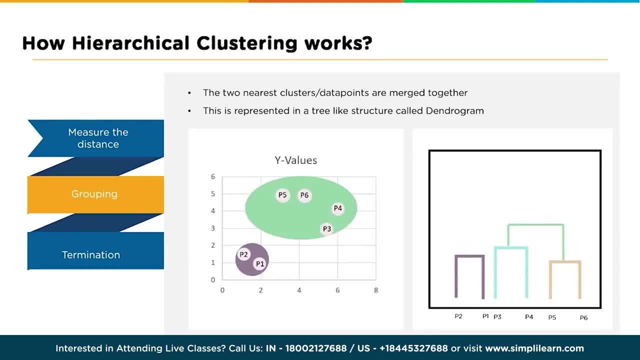 are all under one dendogram because they're closer together than the p1 and p2, and then we terminate when we are left with one cluster, so we finally bring it all together. you can see on the right how we've come up all the way up. 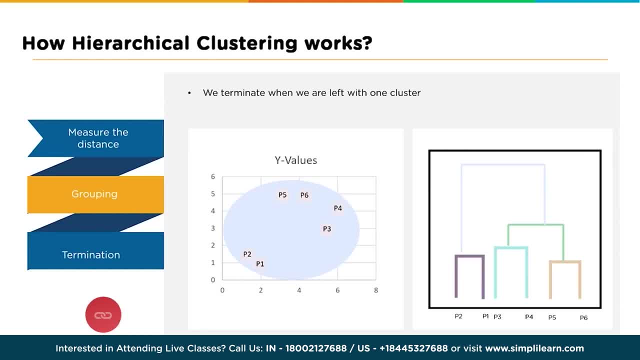 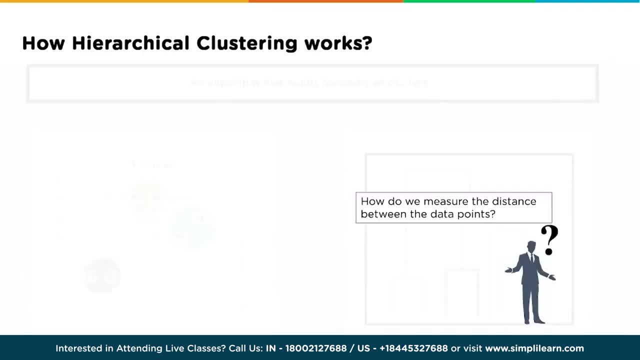 whoops, and we have the gray hierarchical box coming in there and connecting them, so we have just one cluster and that's a good place to terminate because there is no way we can bring them together any further. so how do we measure the distance between the data points? I mean, this is really where it starts getting. 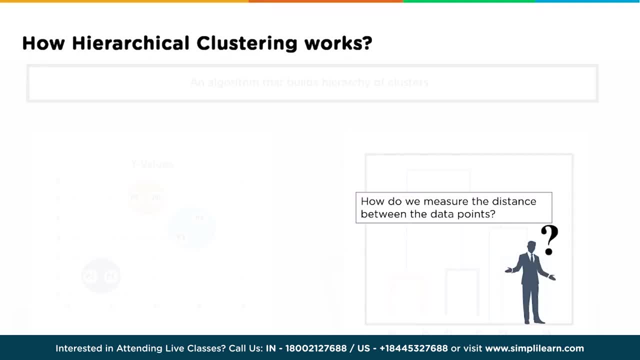 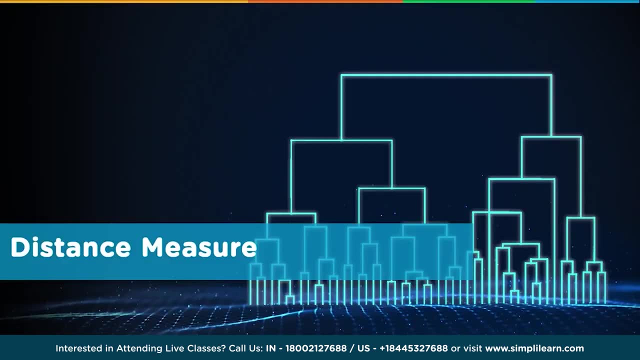 interesting. up until now you can kind of eyeball and say, hey, these look together. but when you have thousands of data points, how are we going to measure those distances? and there is a lot of ways to get the distance measure, so let's go ahead and take a look at that. distance measures will determine the 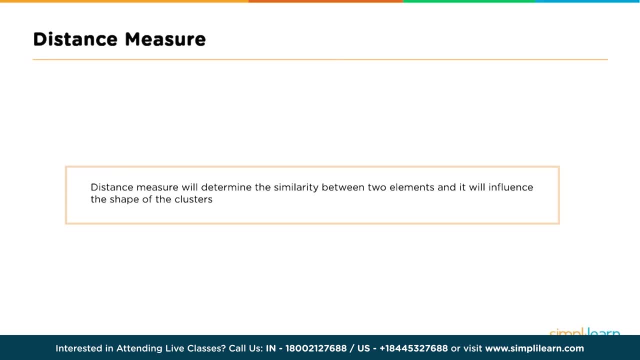 disparity between two elements and it will influence the shape of the clusters. and we have Euclidean distance measure, we have squared Euclidean distance measure, which is almost the same thing but with less computations, and we have the Manhattan distance measure, which will give you slightly different results, and 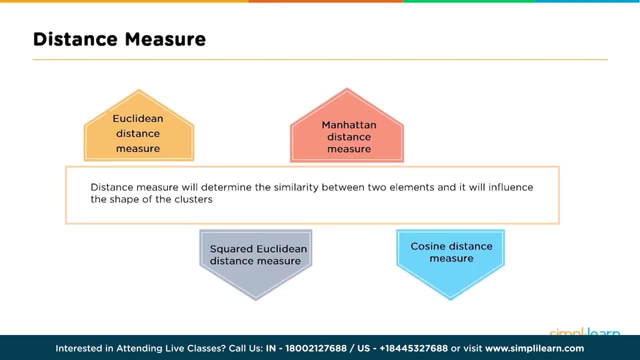 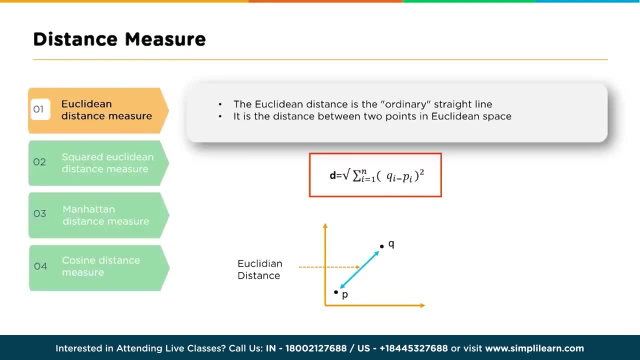 we have the cosine distance measure, which again is very similar to the Euclidean- playing with triangles, and sometimes it can compute faster, depending on what kind of data you're looking at. so let's start with the Euclidean distance measure. the most common is: we want to know the 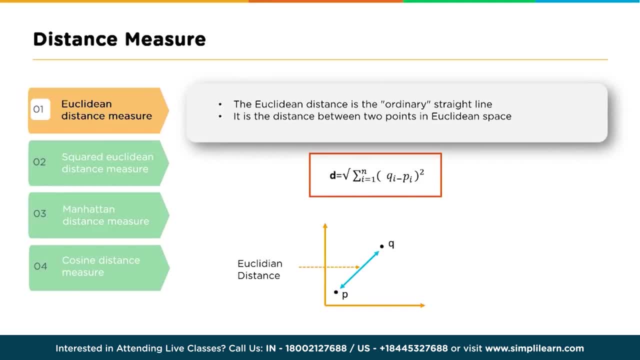 distance between the two points. so if we have point P and point Q, the Euclidean distance is the ordinary straight line. it is the distance between the two points in Euclidean space, and you should recognize D equals in this case. we're going to sum all the points, so if there was more than one point we could figure. 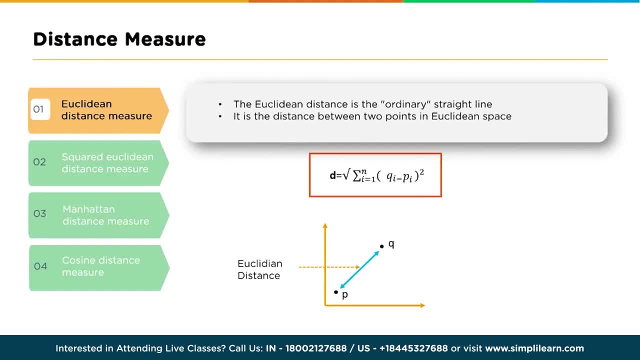 out the distance to the not more than one points. this is the sum of more than two dimensions, so we can have the distance between each of the different dimensions squared and that will give us and then take the square root of that and that gives us actual distance between them And they should look familiar from Euclidean geometry. Maybe you? 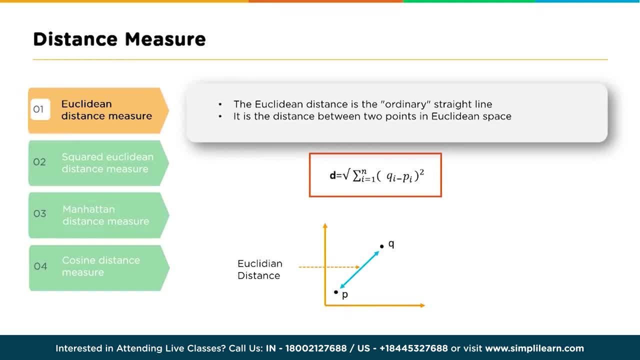 haven't played too much with multiple dimensions so the summation symbol might not look familiar to you, But it's pretty straightforward as you add the distance between each of the two different points squared. So if your y difference was 2 minus 1, squared would be 2.. And then you take 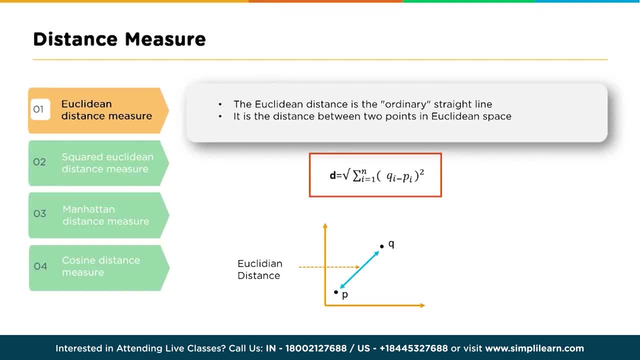 the difference between the x again squared, And if there was a z-coordinance it would be z1 minus z2 squared, And then take the square root of that, or sum it all together and then take the square root of it, So to make it compute faster, since the difference in distances, whether 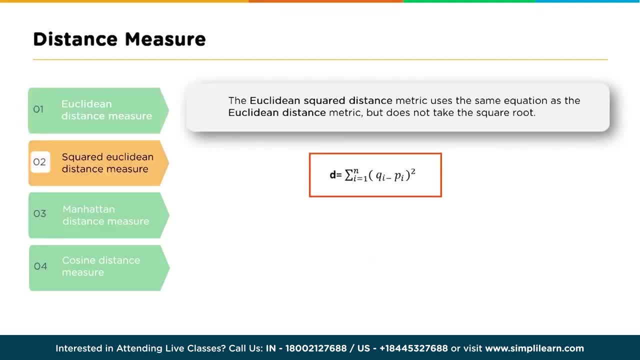 one is farther apart or closer together than the other, we can do what's called the squared Euclidean distance measurement. This is identical to the Euclidean measurement, but we don't take the square root at the end. There's no reason to. It certainly gives us the exact distance, but as 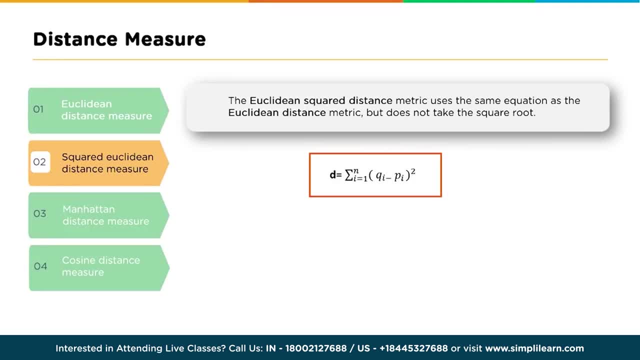 far as doing calculations as to which one's bigger or smaller than the other one, it won't make a difference, So we'll just go with it. So we just get rid of that final square root. It computes faster and it gives us pretty much the Euclidean squared distance on there Now the Manhattan. 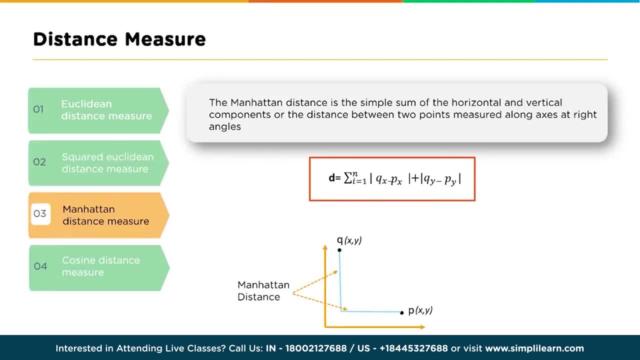 distance measurement is a simple sum of horizontal and vertical components, or the distance between two points measured along axes at right angles. Now, this is different because you're not looking at the direct line between them And in certain cases, the individual distances measured will. 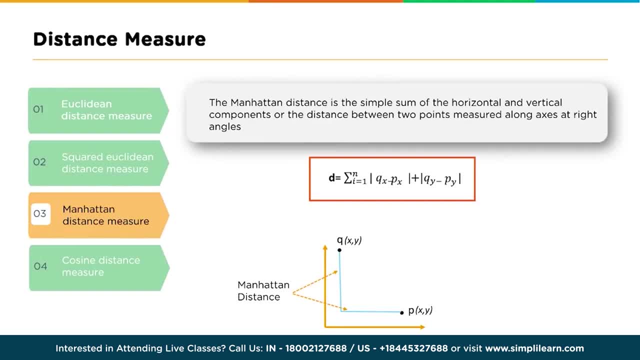 give you a better idea of the distance between the two points. So if you're looking at the result now, generally that's not true. Most times you go with the Euclidean squared method because that's very fast and easy to see. But the Manhattan distance is you measure just the y value and you 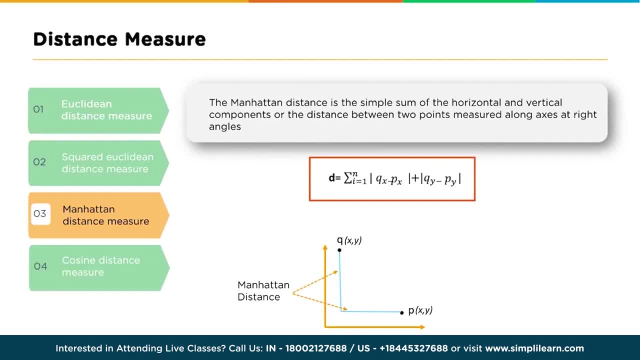 take the absolute value of it and you measure just the x difference and you take the absolute value of it and just the z. And if you had more, you know different dimensions in there: a, b, c, d, e, f. 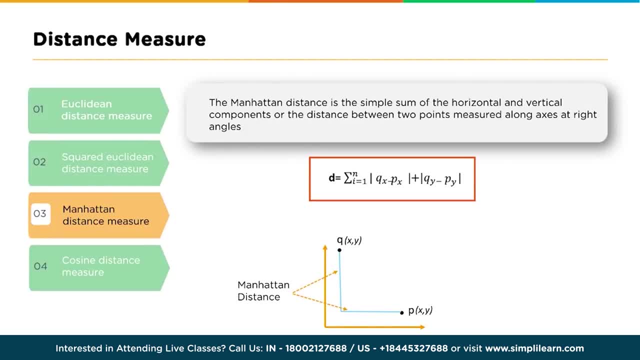 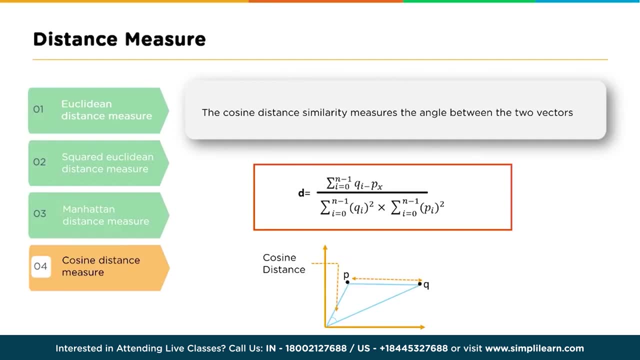 however many dimensions, you would just take the absolute value of the difference of those dimensions And then we have the cosine. distance Similarity measurement is a simple sum of the angles between the two vectors And, as you can see, as the two vectors get further and further, 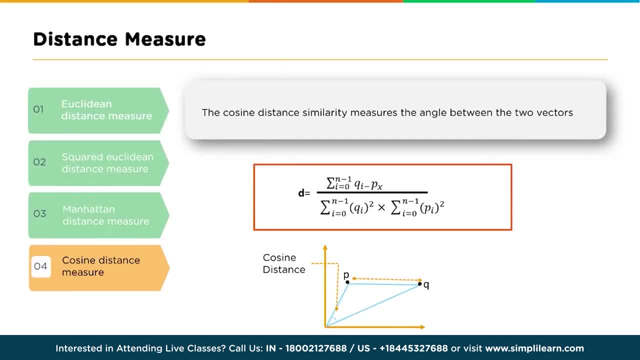 apart. the cosine distance gets larger. So it's another way to measure the distance, Very similar to the Euclidean. so you're still looking at the same kind of measurement. So it should have a similar result as the first two, But keep in mind the Manhattan will have a very different result. 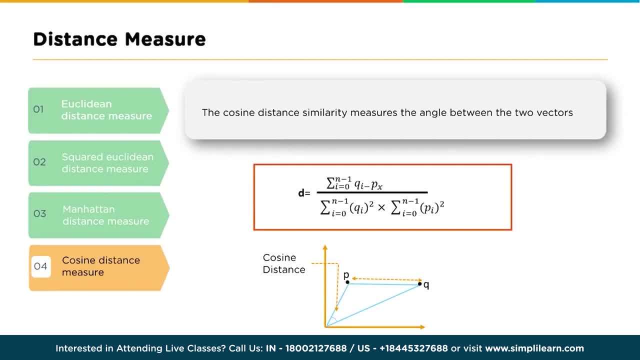 and you can end up with a bias with the Manhattan if your data is very skewed, If one set of values is very large and another set of values is very small. So you can measure the distance between the two vectors, But that's a little bit beyond the scope of this. It's just important to know that. 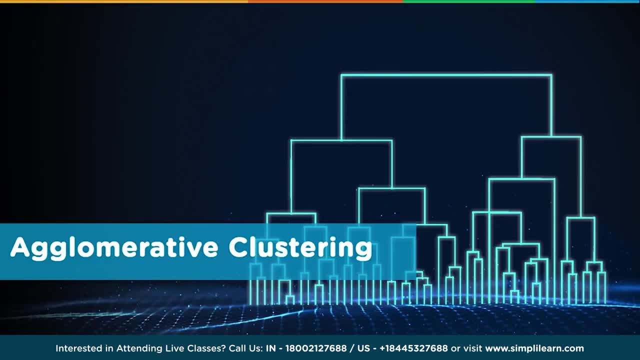 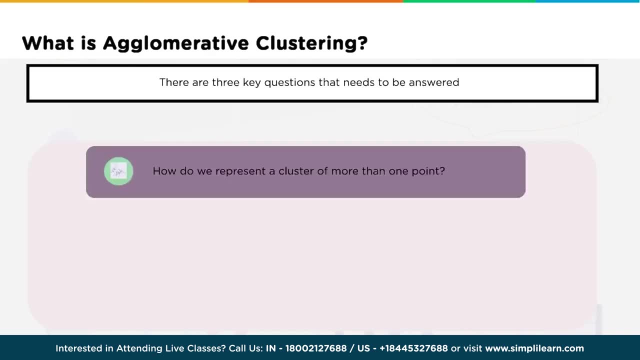 about the Manhattan distance. So let's dig into the agglomerative clustering. And agglomerative clustering begins with each element as a separate cluster and then we merge them into a larger cluster. How do we represent a cluster of more than one point? So we're going to kind of mix the 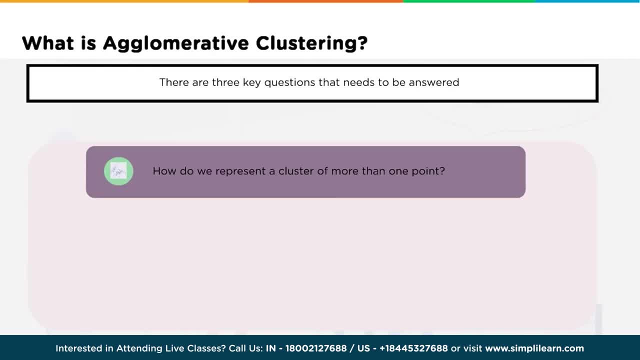 distance together with the actual agglomerative and see what that looks like. And we're actually going to have three key questions that are going to be answered here. So how do we represent a cluster of more than one point? So we're going to look at the math, what it looks like. 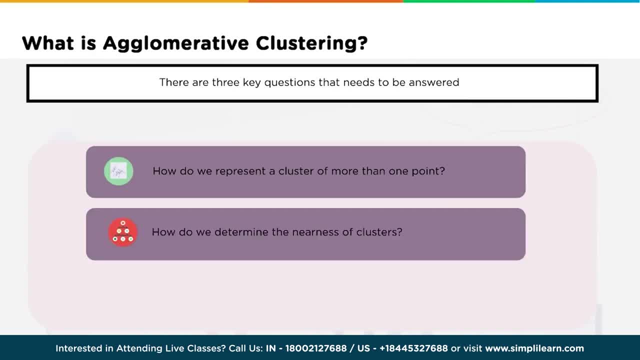 mathematically and geometrically. How do we determine the nearness of clusters? When to stop combining clusters? Always important to have your computer script, or whatever you're working on, have a termination point so it's not going on eternally. We've all done that. if you do any. 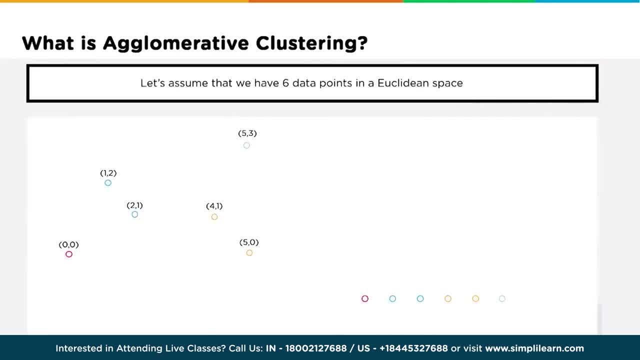 kind of computer programming or writing a script. Let's assume that we have six data points in a Euclidean space. So again, we're dueling with x, y and z And we're going to have six data points, in this case just x and y. So how do we represent a cluster of more than one point? Let's take a look. 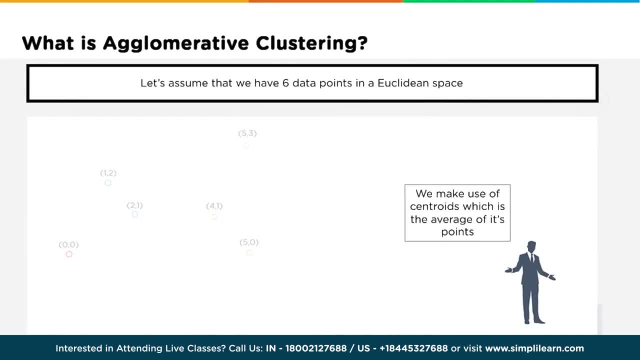 at that. First, we're going to make use of centroids, very common terminology in a lot of machine learning languages when we're grouping things together. So we're going to make use of centroids, which is the average of its points And you can see here we're going to take the one, two and the. 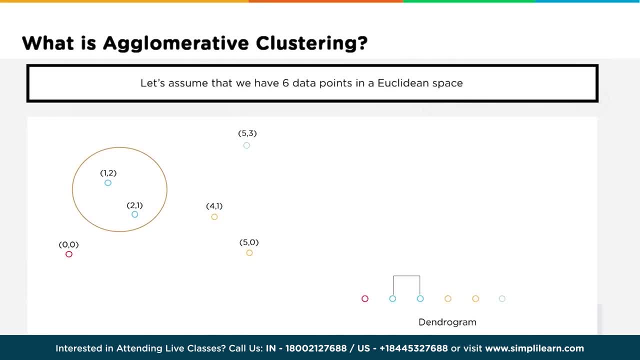 two, one, and we're going to group them together because they're close, And if we were looking at all the points, we'd look for those that are closest and start with those, And we're going to take those two. we're going to compute a point in the middle And we'll give that point 1.5, 1.5, 1.5.. 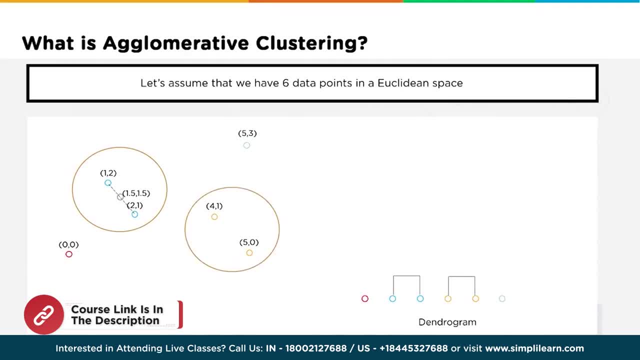 And that's going to be the centroid of those two points. And next we start measuring like another group of points. We've got 4, 1,, 5, 0. And they're pretty close together, So we'll go ahead and set up. 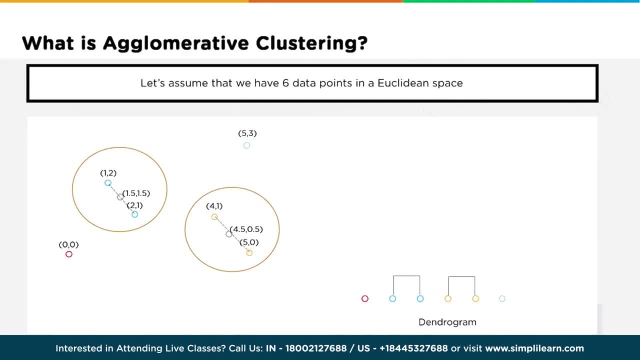 a centroid of those two points. In this case it would be the 4.5 and .5 would be the measurements on those two points. And once we have the centroid of the two groups, we find out that the next closest point to a center point is the center point, And that's going to be the center point, And that's. 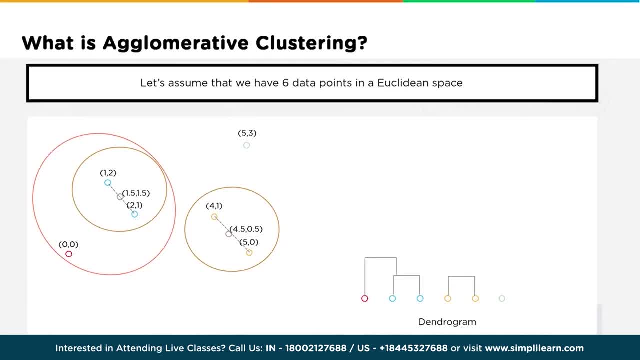 going to be. the centroid is over on the left, And so we're going to take this and say, oh, 0, 0 is closest to the 1.5, 1.5 centroid. So let's go ahead and group that together And we compute a new. 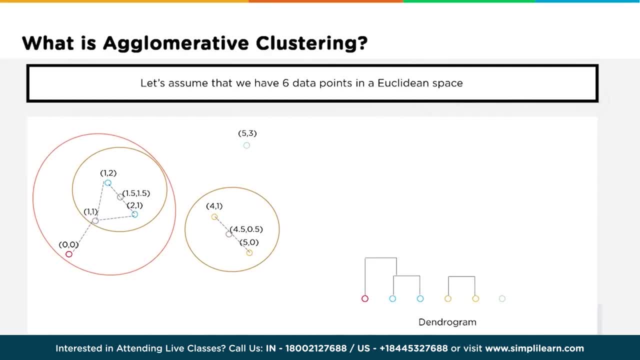 centroid based on those three points. So now we have a centroid of 1.1 or 1,, 1.. And then we also do this again with the last point, the 5,, 3, and it computes into the first group And you can see. 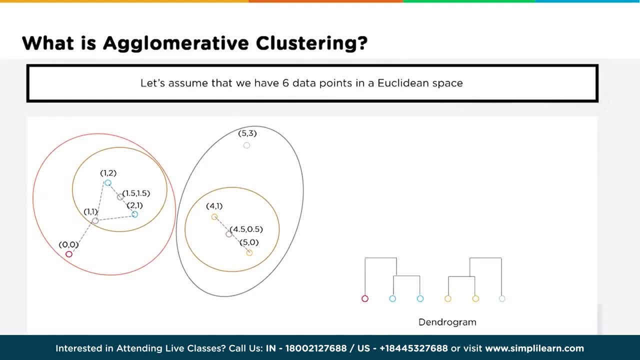 our dendrogram on the right is growing, So we have each of these points become connected and we start grouping them together And finally we get a centroid of that group too, And then finally the last thing we want to do is combine the two groups by their centroids, And you can see, here we end up with one large group and 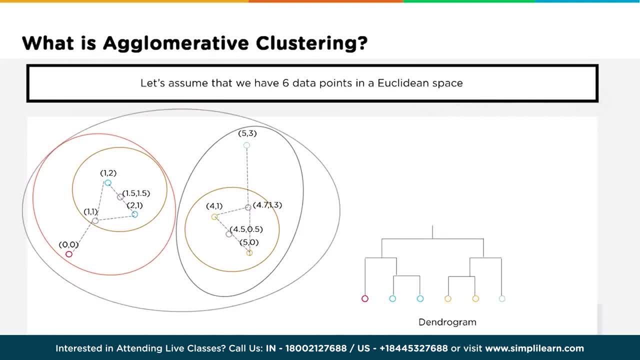 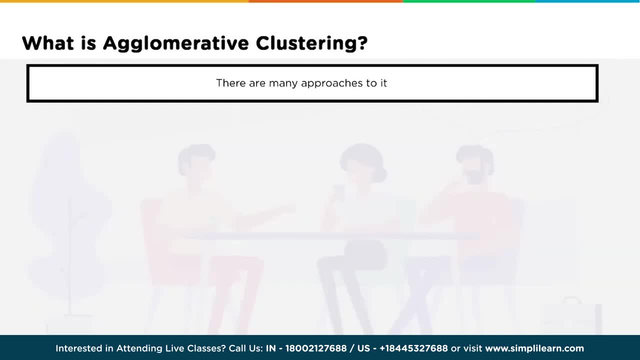 it'll have its own centroid, although usually they don't compute the last centroid, We just put them all together. So when do we stop combining clusters? Well, hopefully, it's pretty obvious to you In this case when they all got to be one, But there are actually many approaches to it. So first pick: 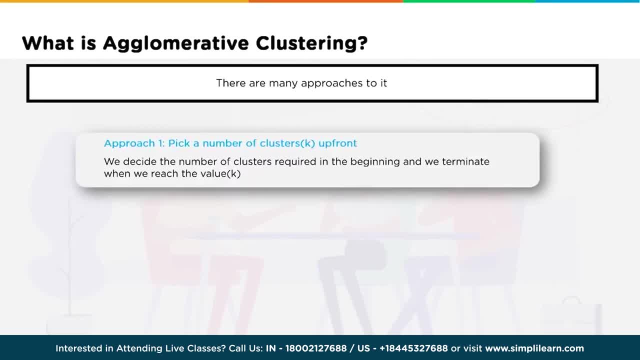 a number of clusters k up front, And this is done in the fact that we have a number of clusters that we don't want to look at- 200 in clusters. We only want to look at the top five clusters or something like that. So we decide the number of clusters required in the beginning and we terminate. 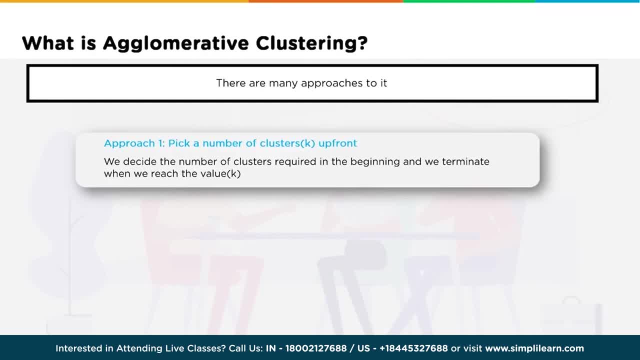 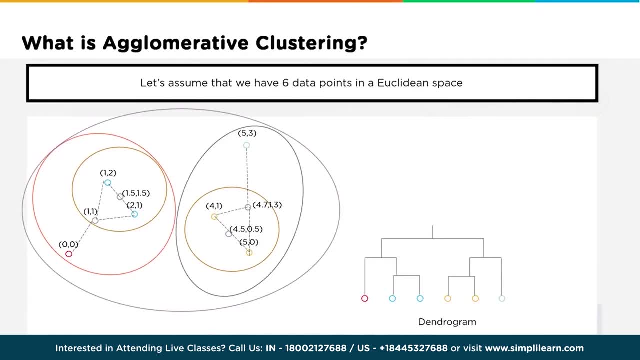 when we reach the value k. So if you looked back on our clustering- let me just go back a couple screens- you'll see how we clustered these all together And we might want just the two clusters, And so we look at just the top two, Or maybe we only want three clusters And so we would compute. 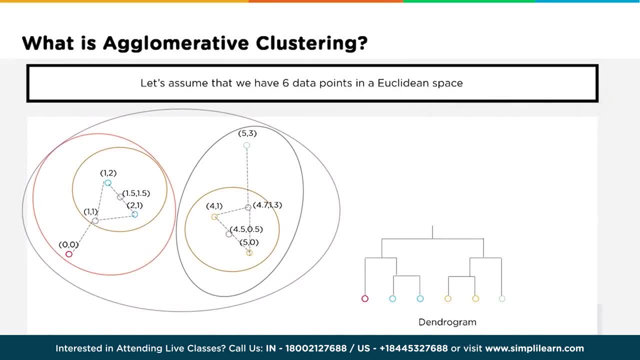 which one of these has a wider spread to it or something like that. There's other computations to know how to connect them And we'll look at that in just a minute. But to note that when we pick the k value we want to limit the information that's coming in, So that can be very important. 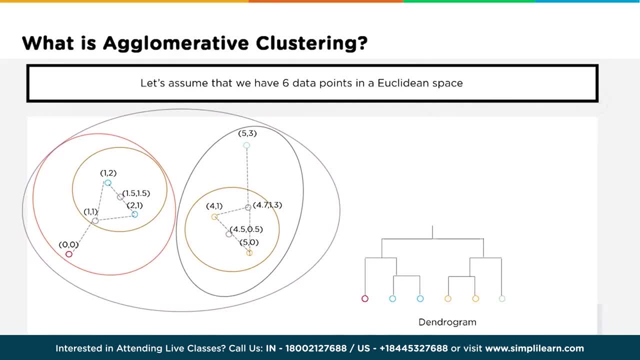 especially if you're feeding it into another algorithm that requires three values, or you set it to four values and you need to know that value coming in. So we might take the clustering and say, okay, only three clusters, That's all we want for k. So the possible challenges. This only makes sense when we 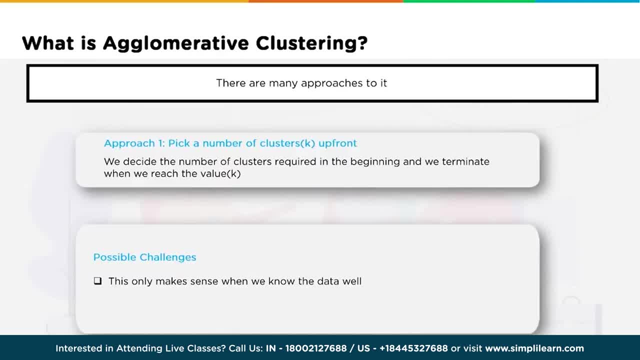 know the data well. So when you're clustering with k clusters, you might already know that domain and know that that makes sense, But if you're exploring brand new data, you might have no idea how many clusters you really need to explore that data with. Let's consider the value of k to be two. So in this case, in our 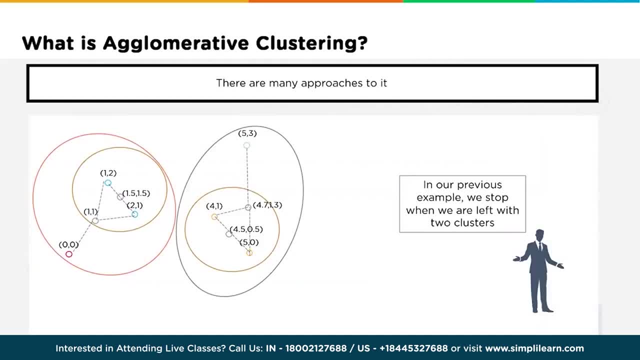 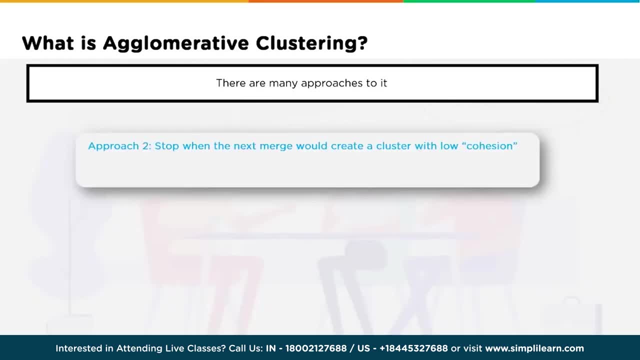 previous example. we stop when we are left with two clusters- And you can see here that this is where they came together the best, while still keeping separate the data. The second approach is stop when the next merge would create a cluster with low cohesion. So we keep clustering until the next merge of clusters creates a bad 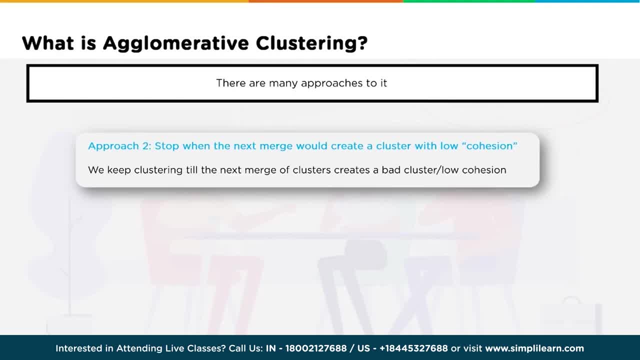 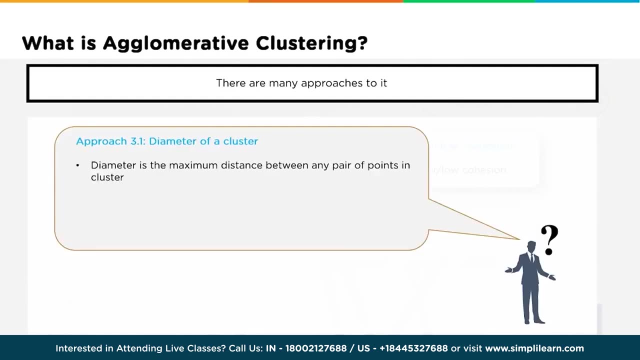 cluster, low cohesion set up on there. That means the point is so close to being between two clusters it doesn't make sense to bring them together. But how is cohesion defined? Oh, let's dig a little deeper into cohesion: The diameter of a cluster. So we're looking at the actual diameter of our cluster and the diameter is the maximum. 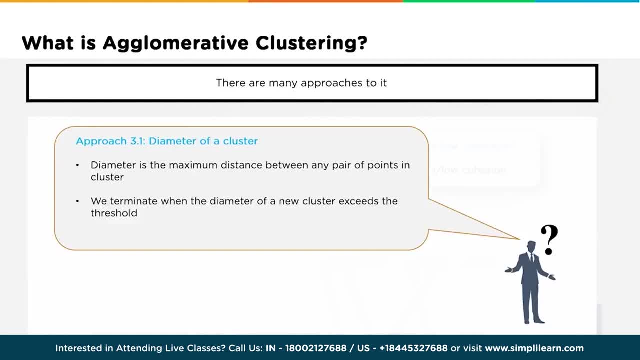 distance between any pair of points in the cluster. We terminate when the diameter of a new cluster exceeds the threshold, So as that diameter gets bigger and bigger, we don't want the two circles or clusters to overlap And we have radius of a cluster. Radius is the maximum distance of a point from centroid. We 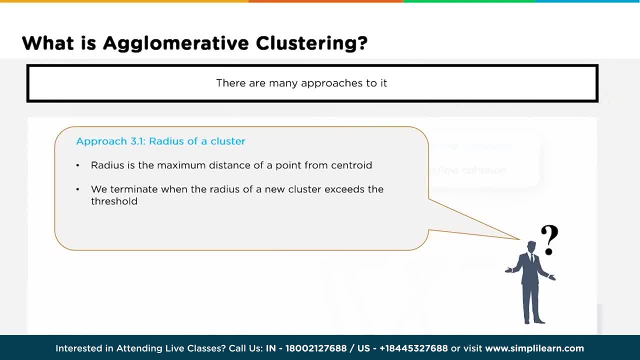 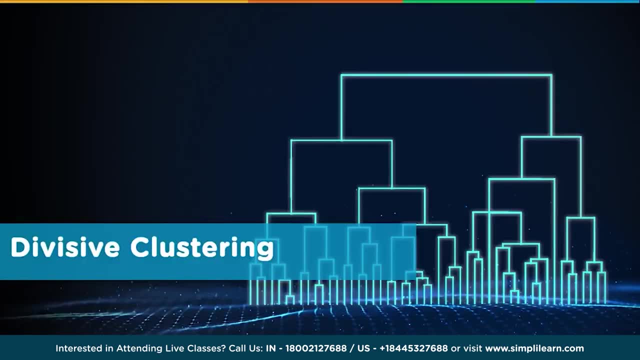 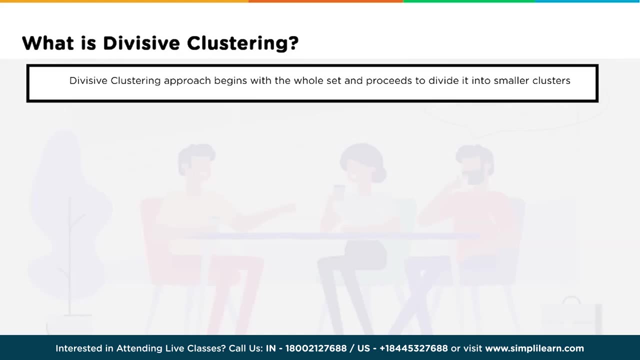 terminate when the radius of a new cluster exceeds the threshold. Again, we don't want things to overlap, So when it crosses that threshold and is overlapping with other data, we stop. So let's look at divisive clustering. Remember, we went from the bottom up, Now we want to go from the top down. Divisive clustering approach begins with a whole set and 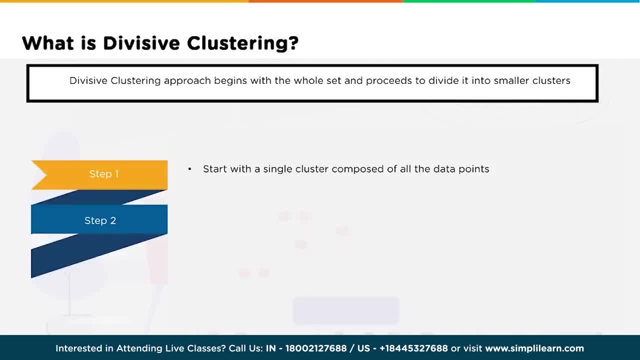 proceeds to divide it into smaller clusters. So we start with a single cluster composed of all the data points. We split it into different clusters. This can be done using monothetic divisive methods. What is a monothetic divisive method? And we'll go backwards and let's consider the example we took in the. 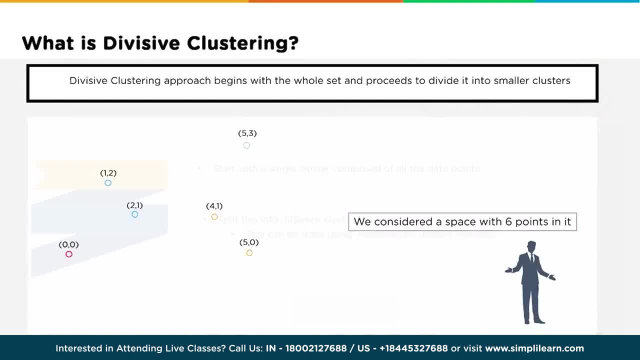 agglomerative clustering to understand this. So we consider a space with six points in it, just like we did before, same points we had before, And we name each point in the cluster. So we have in this case we just gave it a letter value- A, B, C, D, E, F. 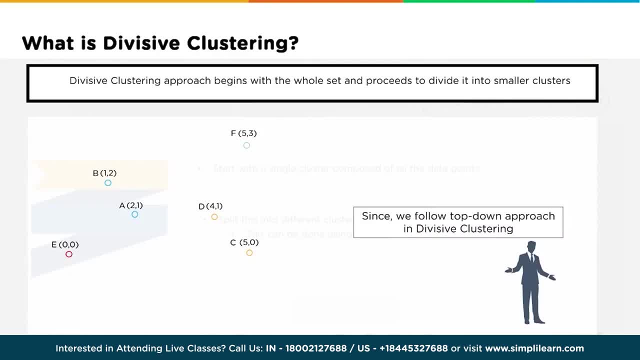 Since we follow top down approach in divisive clustering, obtain all possible splits into two columns. So we want to know where you could split it here And we could do like an A B split and a C, D E F split. We could do B, C, E, A D F And you can see this starts generating a huge amount of. 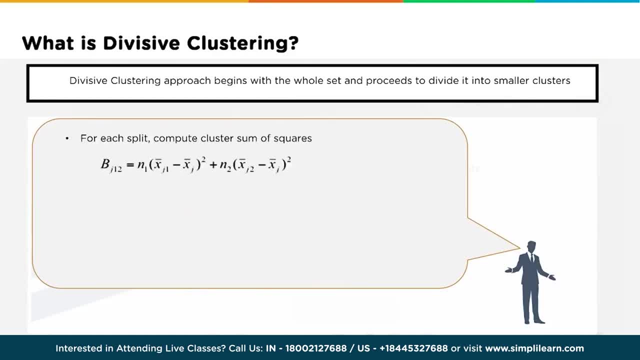 data: A, B, C, D, E, F, And so for each split we can compute cluster sum of squares And we can see- here we actually have the formula out for us: B J, 12 equals N1 of. 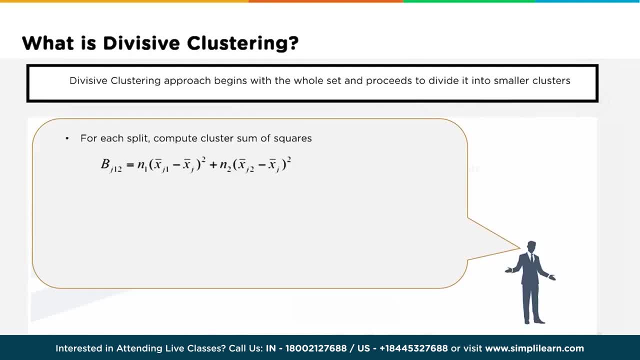 absolute value of X minus absolute value of X squared. So again we're computing all the different distances and they're squared Back to your kind of Euclidean distances on that, And so we can actually compute B? J between clusters one and two. We have the mean of the cluster and the grand mean, depending on. 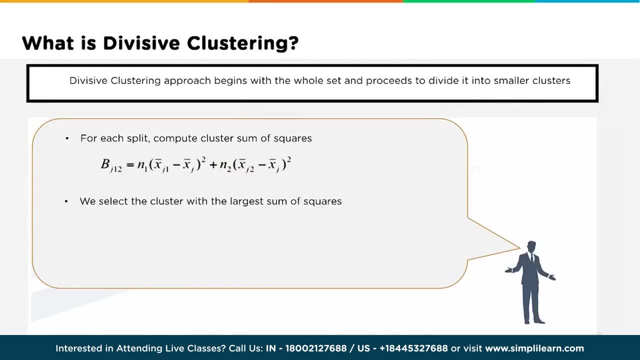 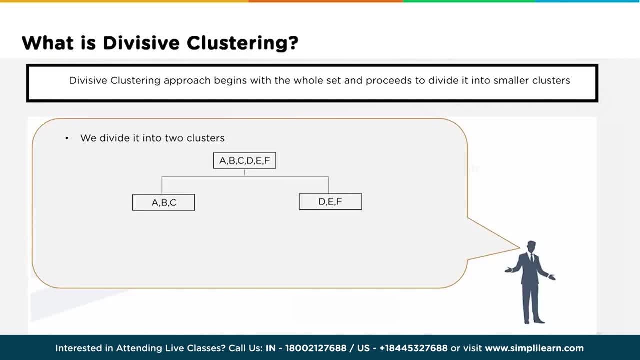 where we split the A B C out, And that's where we split the A B C out. And that's where we split the A B C out, And that's where we split the A B C out. And if we split the A B C out, we're left with the D E F. on the other side We again find the sum of squared distances and split it into clusters. So we go from A B C. we might find that the A splits into B, C and D into E, F, And again you start to see that hierarchical dendogram coming down as we start splitting everything apart. And finally we might have A splits in B and C and then each one gets their own D, E, F And it continues to divide until we get little nodes at the end and every data has its own point. Or we could have a 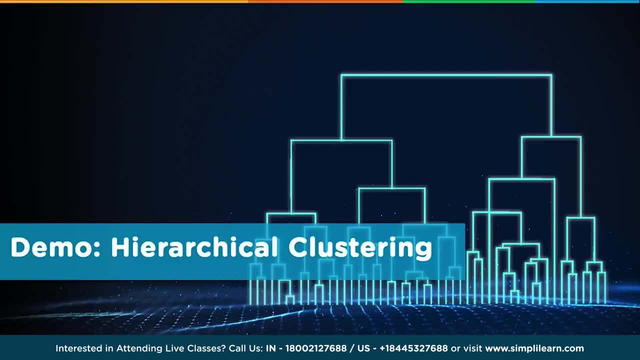 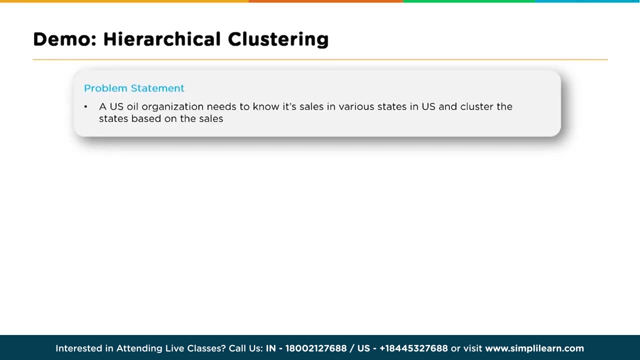 or until we get to K if we have set a K value. So we've kind of learned a little bit about the background and some of the math in hierarchical clustering. Let's go ahead and dive into a demo, And our demo today is going to be for the problem statement. we're going to look at US oil. So a US oil organization needs to know its cells in various states in US and cluster the states based on the cells. So what are the steps involved in setting this problem up? So the steps we're going to look at, and this is 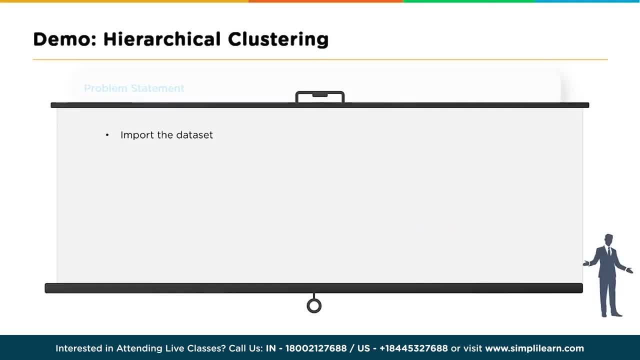 really useful for just about any processing of data, although I believe we're going to be doing this in R today. We're going to import the data set, So we'll explore our data a little bit there. Create a scatter plot. It's always good to have a visual if you can. Once you have a visual, you can know if you're really far off in the model you choose to cluster the data in or how many splits you need. And then we're going to normalize the data. So we're going to fix the data up so it processes correctly- And we'll talk in more detail about normalization when we get there- And then calculate the Euclidean distance. 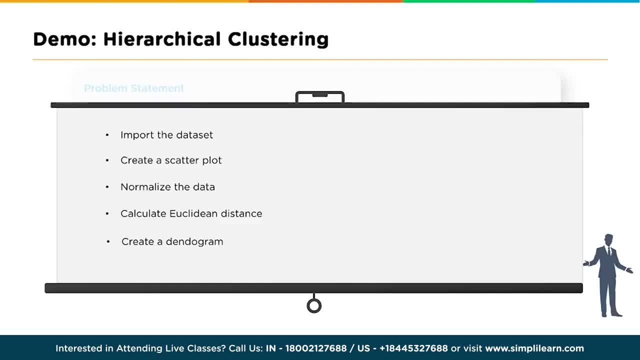 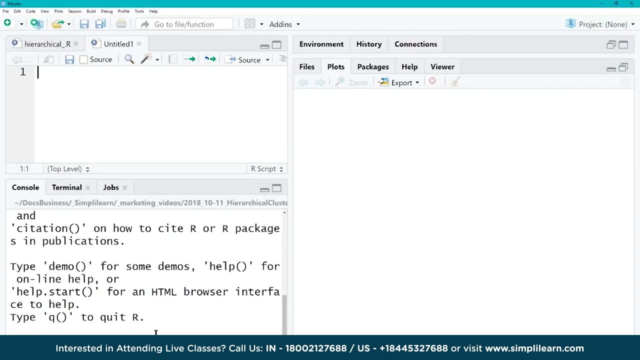 And finally, we'll create our dendogram so it looks nice and pretty and we have something we can show to our shareholders so that they have something to go on and know why they gave us all that money and salary for the year. So we go ahead and open up R And we're actually using RStudio, which really has some nice features in it. It automatically sets up the three windows where we have our script file on the upper left And then we can execute that script and it'll come down and put it into the 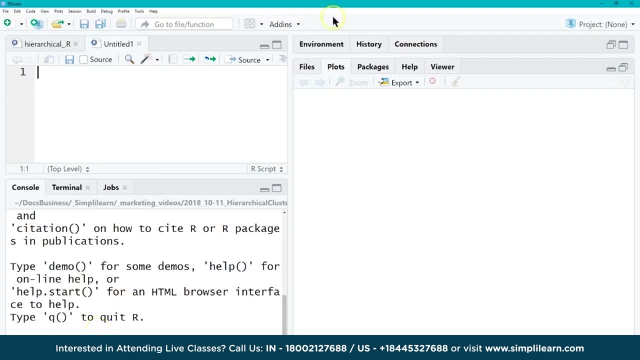 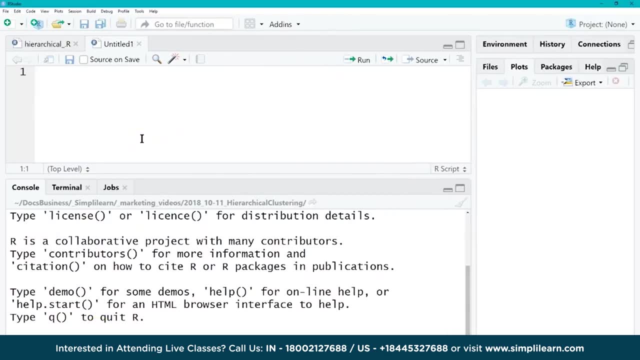 console bottom left and execute it. And then we have our plots off to the right And I've got it zoomed in, hopefully not too large a font but large enough that you can see it. And let's just go ahead and take a look at some of the script going in here. It's clustering analysis and we're going to work. we'll call it my data And we're going to assign it in R- This is a symbol for assigning- And we're going to go read CSV: Read CSV file. 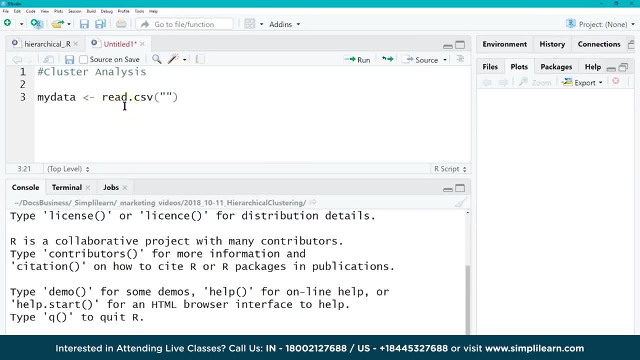 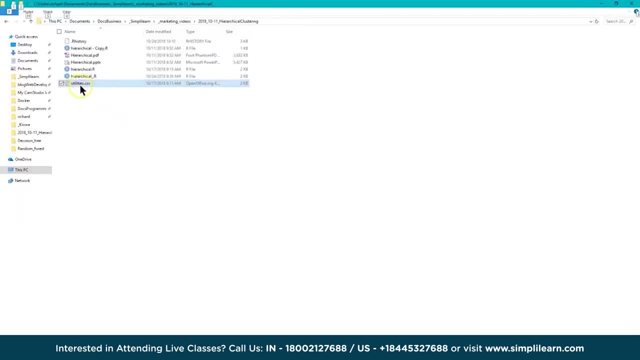 And we'll put that in brackets And let's. before we go any further, let's just look at the data outside of R. It's always nice to do if you can, And the file is going to be called utilitiescsv. This would also be the time to get the full path, so you have the right path to your file, And remember that you can always post in the comments down below, And when you post down there, just let us know you want to connect up with Simply Learn, so that we can. 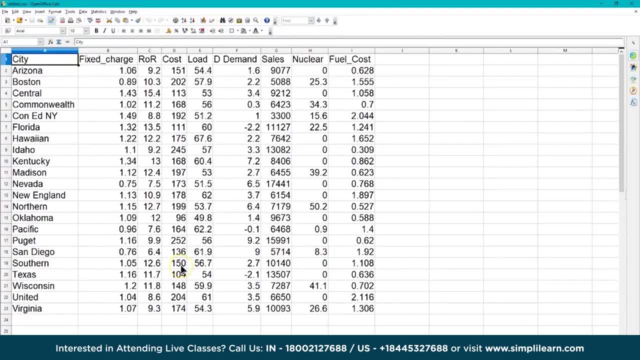 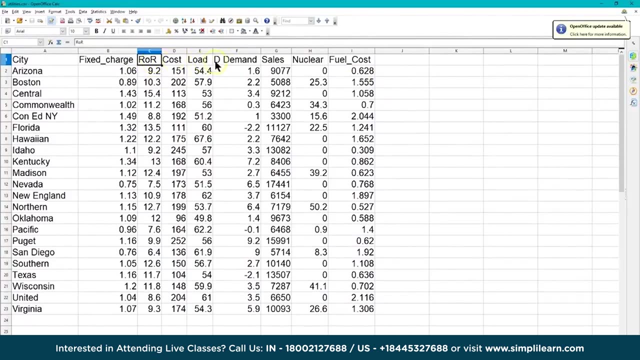 get you this file so you can get the same file we're working on and you can repeat it and see how this works. This is utilitiescsv. It's a comma separated variable file, so it's pretty straightforward And you can see here they have the city fixed charge and a number of different features to the data And so we have our ROR cost, load demand, cells, nuclear fuel cost on here And then, going down the other side, we have US cities- Arizona, Boston, They have central US, so I guess they're grouping a number of areas together. 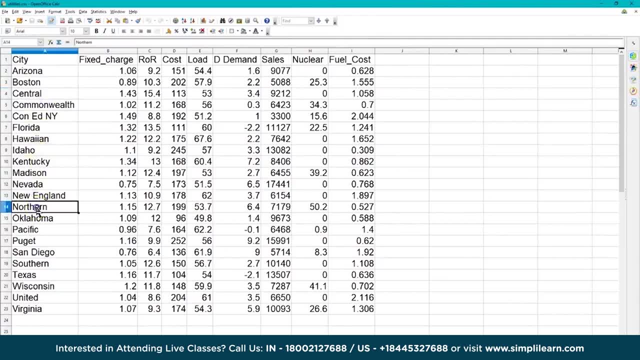 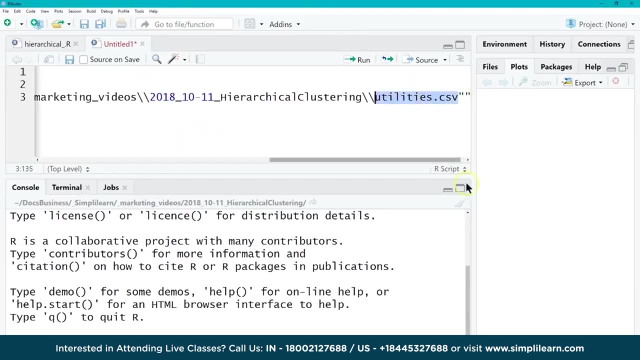 The Commonwealth area you can see down here: Nevada, New England, Northern US, Oklahoma, the Pacific region and so on. So we have a nice little chart of different data they brought in And so I'm going to take that complete path that ends in the utilitiescsv and we're going to import that file. Let me just enlarge this all the way. I hope I have an extra set of brackets here somehow. Maybe I missed a set of brackets. 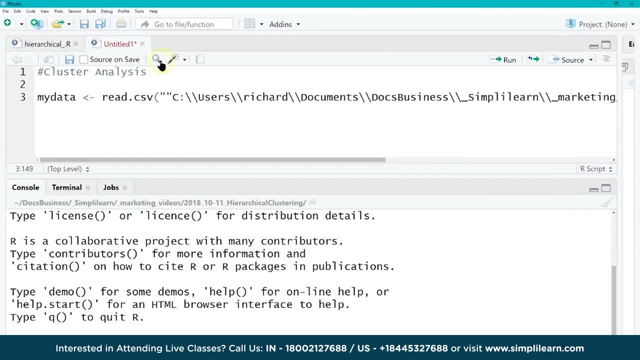 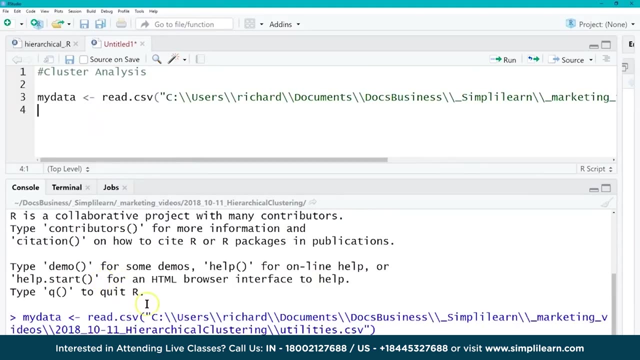 This can happen. if you're not careful, You can get broken. There we go, And then the magic hotkeys in this case are your control enter, which will let me go ahead and run the script, And so I've now loaded the data And, as you can see, I went ahead and shrunk the plot, since we're going to be looking at the window down below. 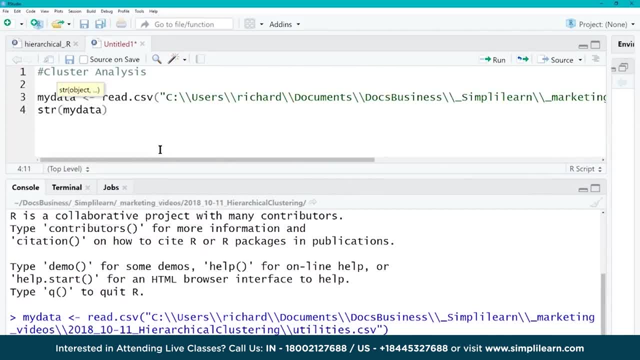 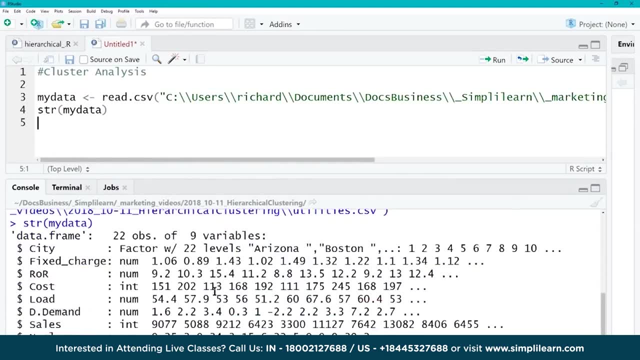 And we can simply convert the data to a string. Now, all of us do this automatically the first time. We say, hey, just print it all out as a string, And then we get this huge mess of stuff that doesn't make a whole lot of sense. 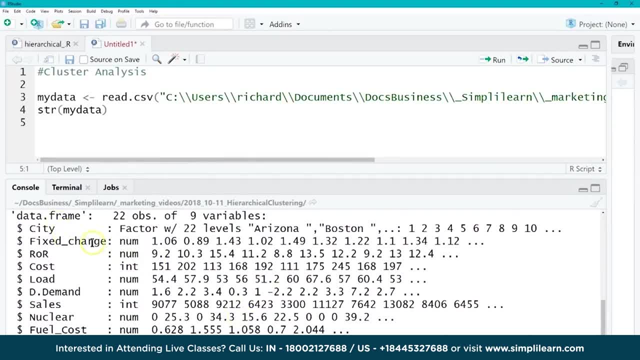 So what you can see here they have, you can probably kind of pull it together as looking at it, But let's go ahead and just do the head And we'll do the head of my data. There we go And control, enter on that. 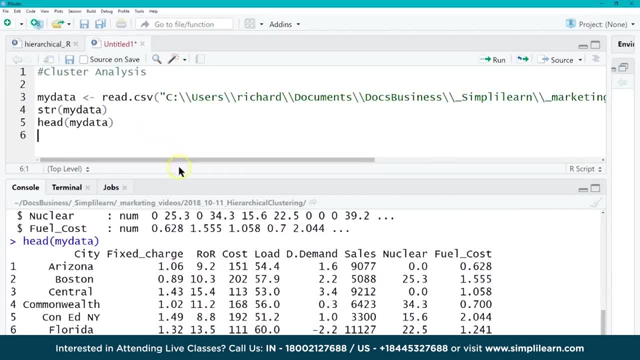 And the head shows the first five rows. You'll see this in a lot of different scripts. In R it's you type in head and then, in brackets, you put your data And it comes through and lists the first five rows, as you can see below. 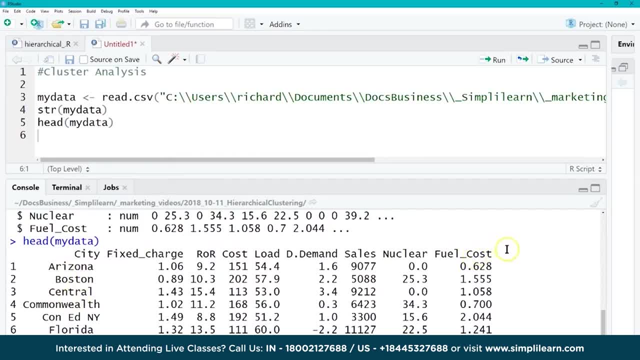 And it shows Arizona, Boston, Central, and it has the same columns we just looked at. So we have the fixed charge, the ROR, the cost, the load, the D demand. I'm not an expert in oil so I'm not even sure what D demand is. 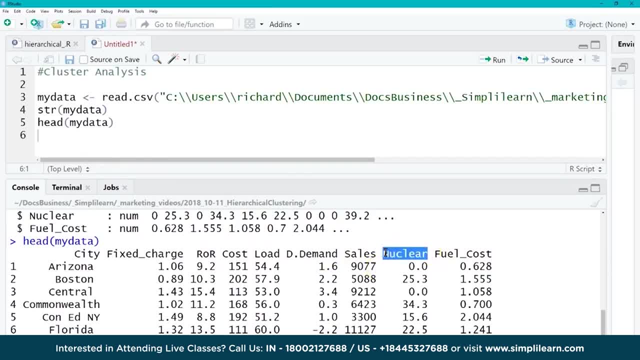 Cells, I'm guessing nuclear, how much of it is supplied by nuclear and the actual fuel cost, And then the different states that it's in or different areas. And one of the wonders of R is all these cool, easy-to-use tools that are so quick. So we'll do pairs, And pairs creates a. 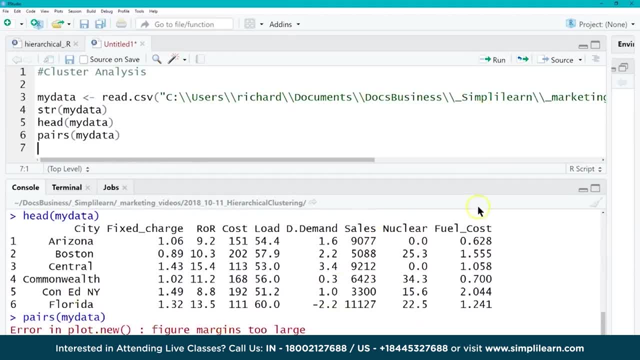 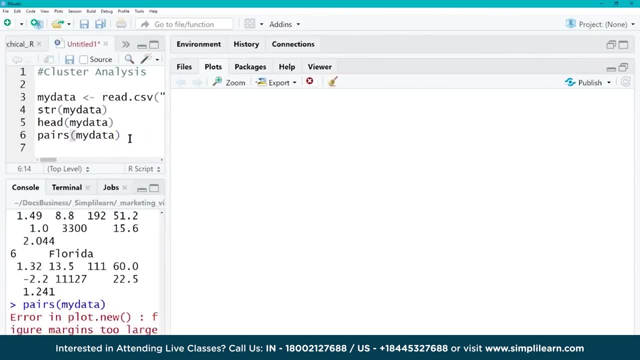 nice graph, So let me go ahead and run this. Whoops. The reason it gave me an error is because I forgot to resize it, So let me bring my plot way out so we can see it, And let's run that again And you'll. 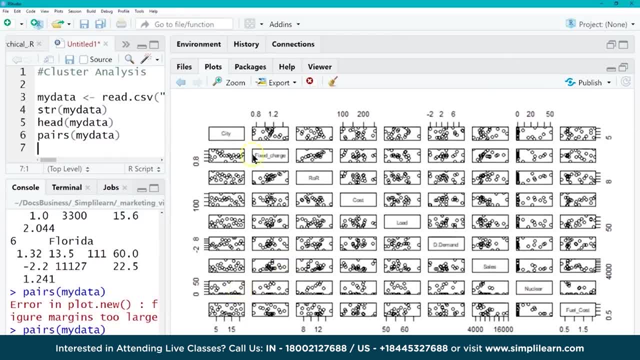 see here that we have a nice graph of the different data and how it plots together, how the different points kind of come together. This is neat because if you look at this, I would look at this and say, hey, this is a great candidate for some kind of clustering. And the reason is is when I look at 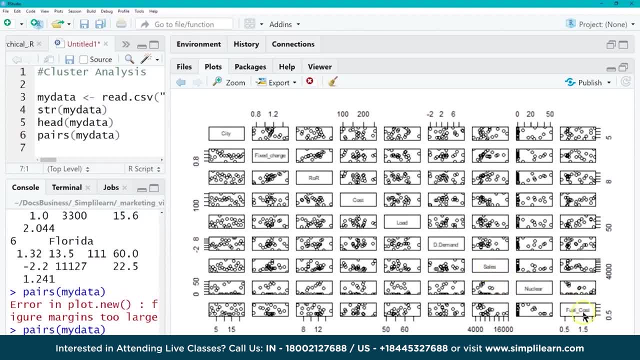 any two pairs. let's go down to say cells and fuel cost, towards the bottom right, And when you look at them where they cross over, you sort of see things how they group together. but it's a little confusing. You can't really pinpoint how they group together. You could probably 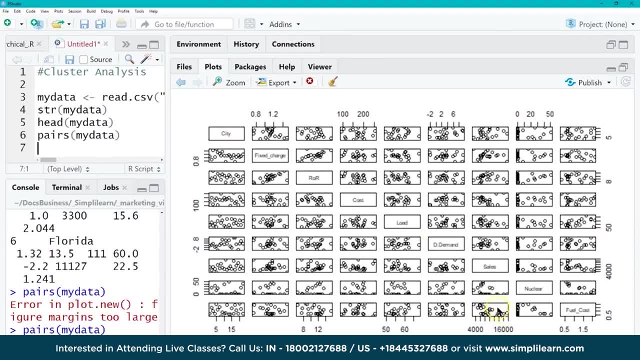 look at these two and say, yeah, there's pretty good commonalities there. And if you look at any of the other pairs, you'll start seeing some patterns there also, And so we really want to know what are the patterns on all of them put together, not just any two of them, but the whole. 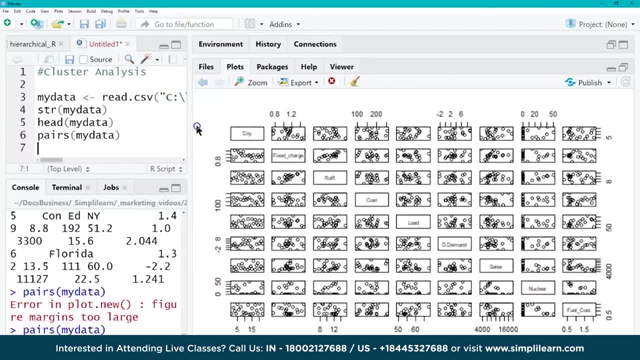 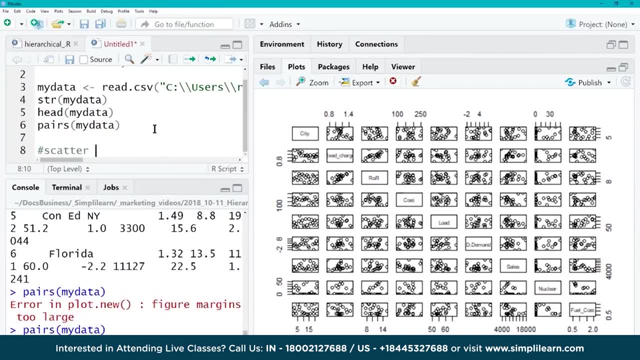 setup. Let me go ahead and shrink this down for just a second, just a notch here, And let's create a scatter plot, And this is simply just use the term plot in brackets. And then which values do we want to plot? And if we remember when we looked at the data earlier, let me just go back. 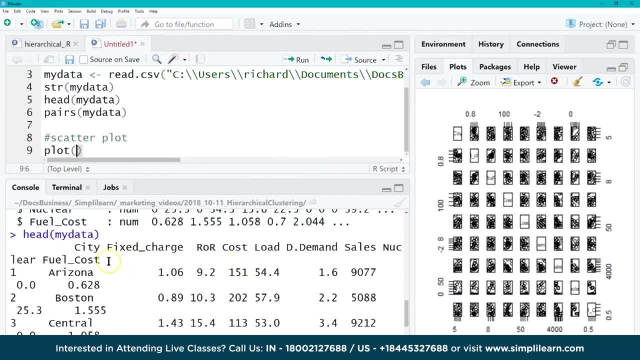 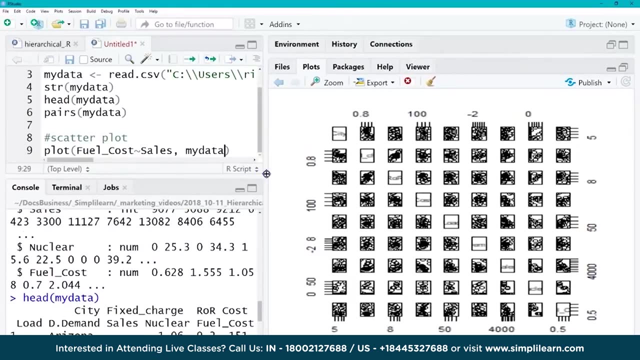 this way. In this case, let's go ahead and compare two- just two values to see how they look, And we'll do fuel cost and cells And it's in my data. So we got to let her know which two columns we're looking at next to each other And it will open up our plot thing and then go ahead and 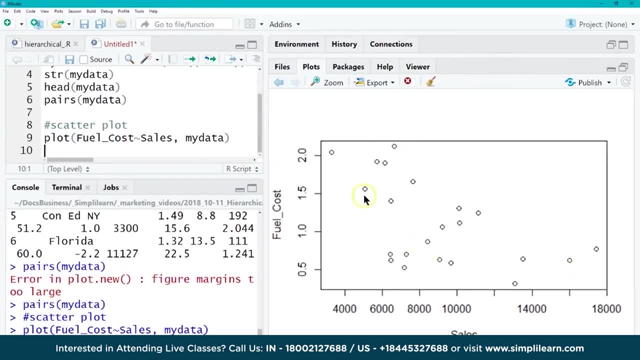 execute that And we can see on those close up of what we were just looking at in the data. And if I was eyeballing this I would say, oh look, there's a kind of a cluster up here of five items And this one it's hard to tell which cluster it'd be with, but maybe it's six to go in. 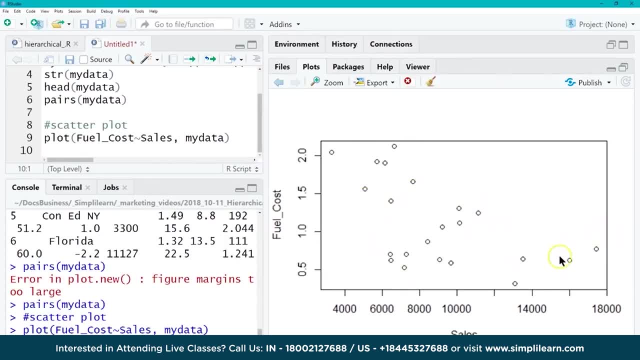 the top one, And you have a middle cluster and a bottom cluster, maybe two different clusters, So you can sort of group them together- fuel cost and the cells- and see how they connect with each other. And again, that's only two different values we're looking at. So in the long run, 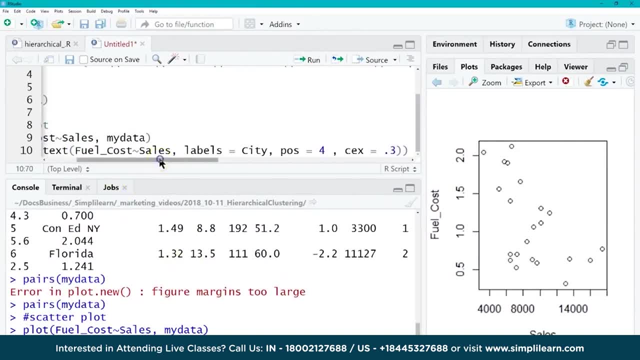 we want to look at all of them. And then the people in the back, they sent me the script so we can go ahead and add labels. So with my data text- fuel cost cells, the labels equals city position four. These are numbers you can kind of play with till they look. 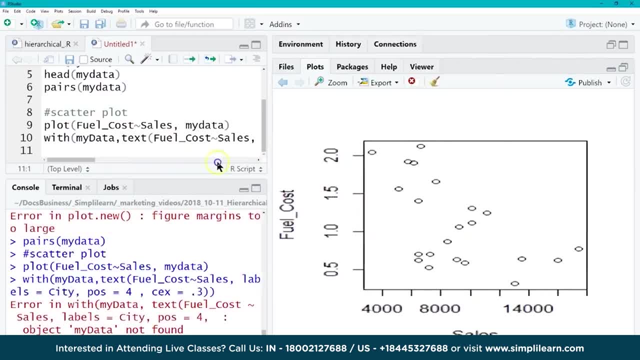 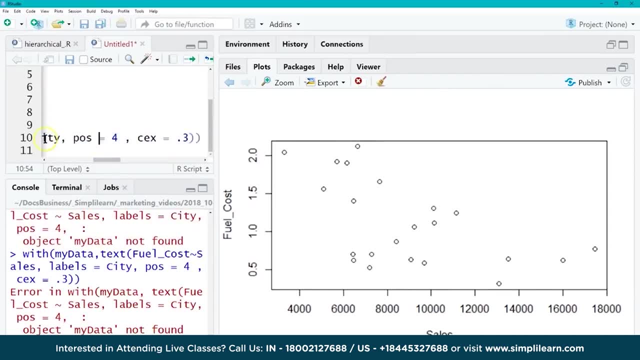 nice. And oops, again, I forgot to resize my plot. It doesn't like having it too small And we'll run that. I mistyped something in here. Oh, I did a lowercase d and they did a capital D. There we go. 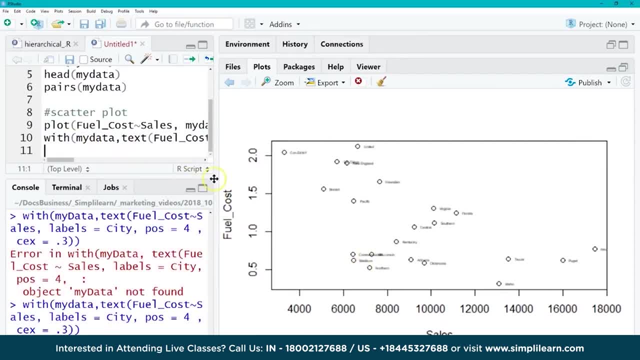 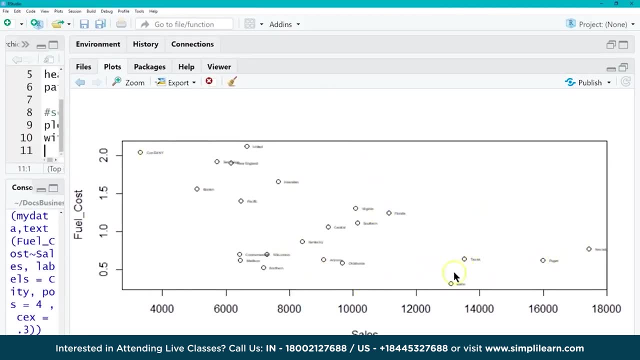 So now we can go in here and do this with my data And you can see a little hard to see on my screen with all the different things in there. It plots the actual cities. So we can now see where all the cities are in connection with, in this case, fuel cost and cells. So you have a nice label to go with. 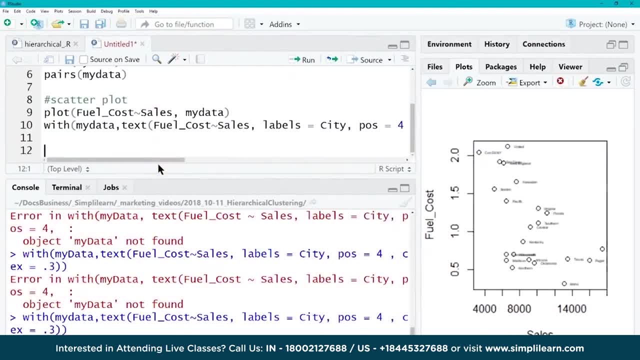 the graph. And then we can also go ahead and plot. in this case, let's do: oh the ROR, Oops, And we'll do that. And then we can also go ahead and plot. in this case, let's do: oh the ROR, And we'll do that. 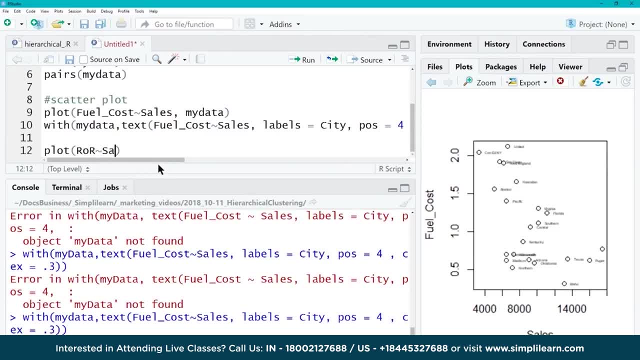 Also with the cells, I can do my data. Remember to leave it lowercase this time. So we plot those two. We'll come over here and it's going to- I'm surprised it didn't give me an error- And then we'll also add in. 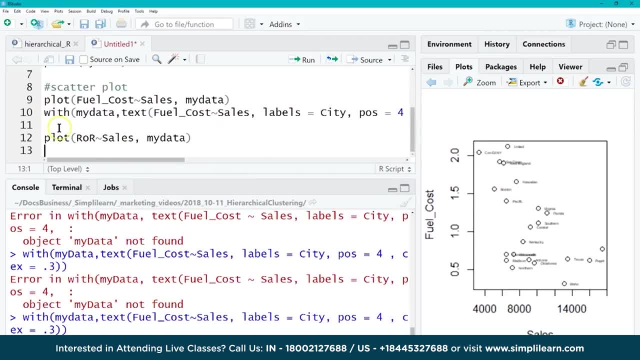 the with statement. So we put some nice labels in there And it's going to be the same as before, except instead of doing the fuel cost cells, we want the R cells, And we'll execute that, And then we'll go ahead. 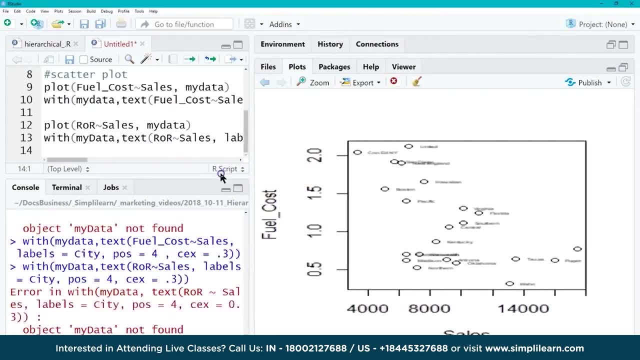 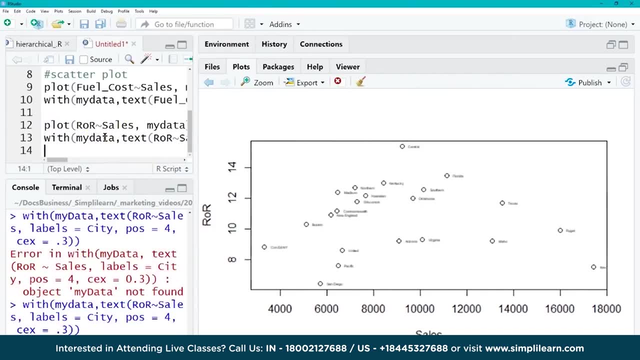 and plot that Oops, And of course it gives me an error because I shrunk it down. So let's redo those two again. There we go And we can see. now we have the ROR with cells And we'd probably get a slightly different. 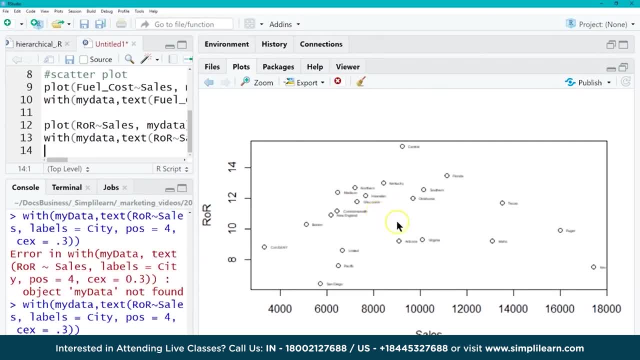 clustering here. if I was looking at these cities, They're probably different than what we had before. But you could probably look at this and say, eh, these kind of go together and those kind of go together, But again, we're going to be looking at all of them instead of just one or two. 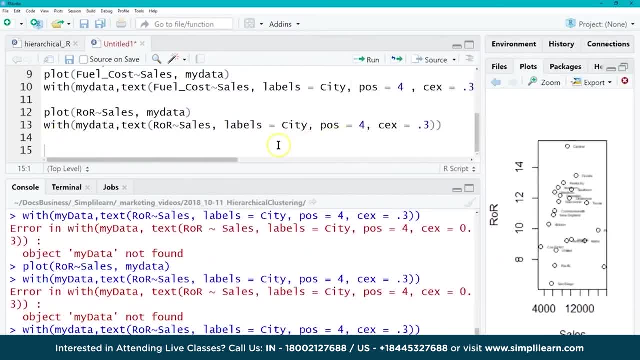 And so at this point we want to dive into the next step. We're going to start looking at a little bit of coding or scripting here. This is very important because we're going to be looking at normalization. We put that in there: normalization. 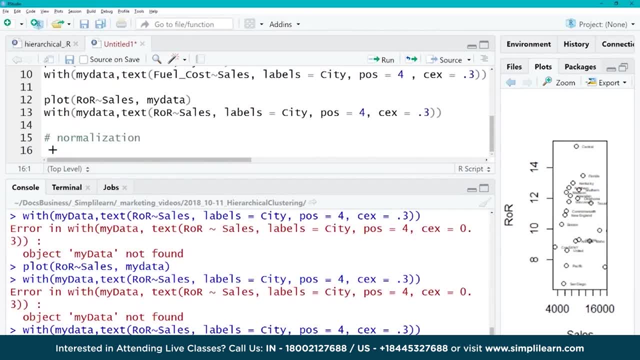 And if you've done any of the other machine learning skills and setup, this should start to look very normal in your pre-processing of data, Whether you're in R or Python or any of these scripts. we really want to make sure you normalize your data so it's not biased. Remember we're dealing with distances. 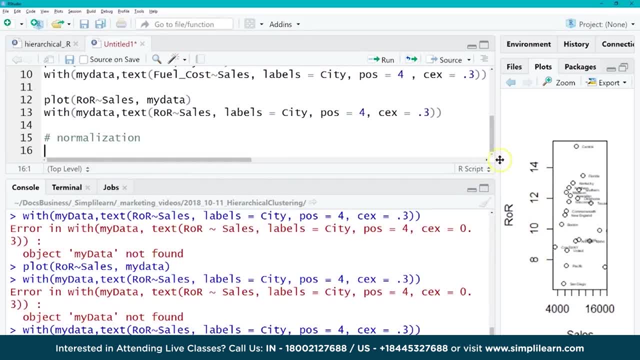 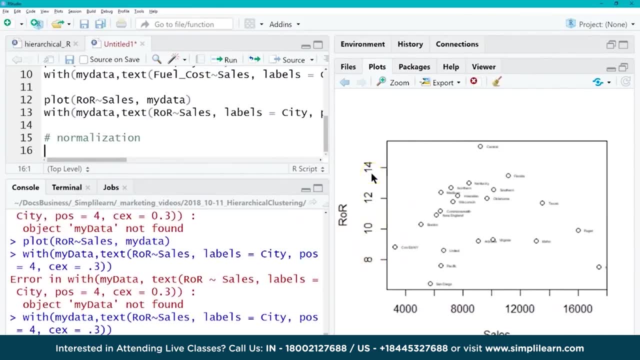 And if I have, let's say, the ROR is. even look at this graph here on the right. you can see where my ROR varies between 8 and 14.. That's a very small variable And our cells varies between 4,000 and 16,000.. 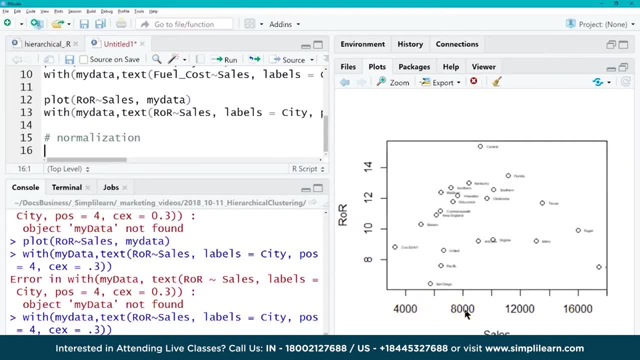 So you can imagine the distance between 4,000 and 8,000,- which is a distance of 4,000, versus 8 to 10, versus 2,- the cells is going to dominate. So if we do any kind of special work on this, it's going to look at cells and it's going to 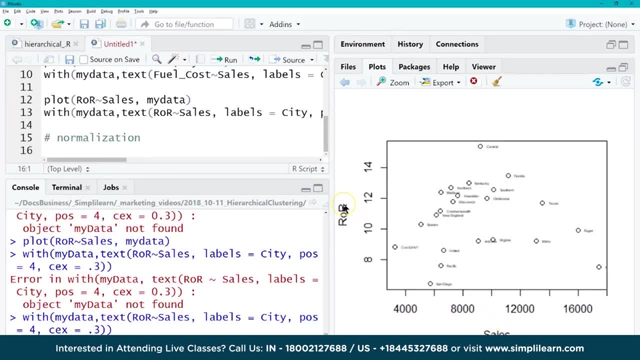 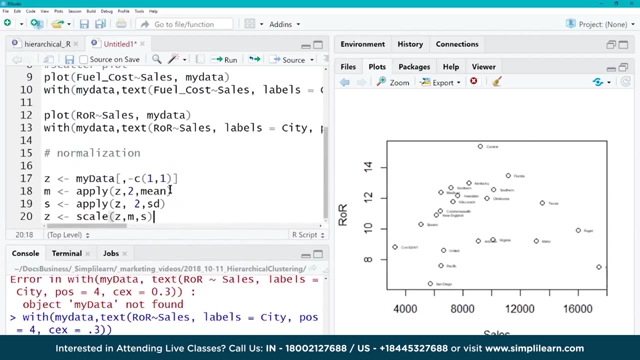 cluster them just by the cells alone, And then ROR might have a little tiny effect of 2 versus 4,000.. We want to level the playing field. Turns out there's actually a number of ways in script to normalize, So I'm just going to put in the code that they put together in the back for me. 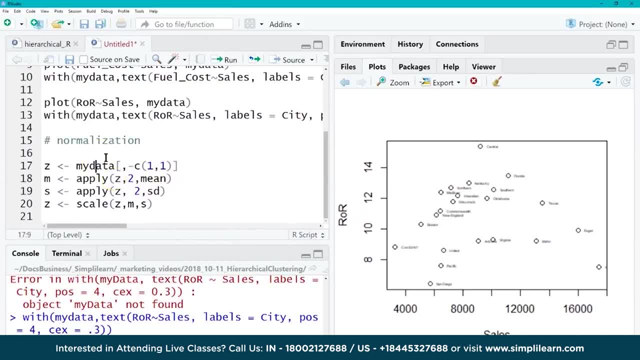 And let's talk about it a little bit. So we have Z, we're going to assign it to my data And it's go ahead, and we're going to do a little reshaping across all rows, Or I mean across all columns, so each of the rows is going to have a little reshaping there. 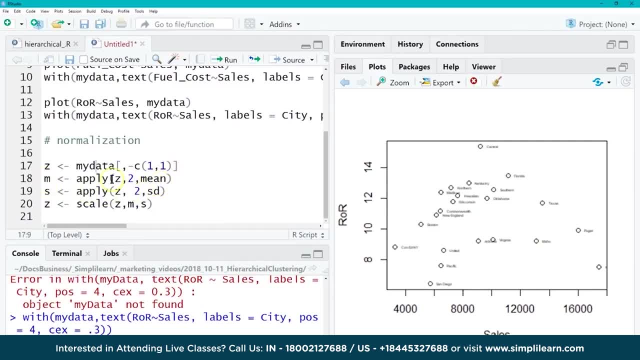 And then we're going to get M, which stands for means, And we're going to apply it to my data. So again, we want to go ahead and create the most common variable in there, And then S is going to be. SD stands for standard deviation. 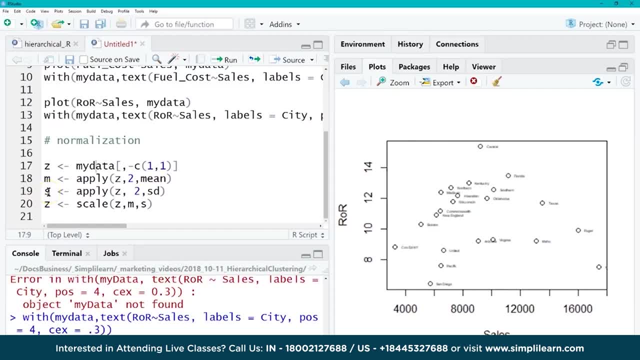 So, instead of just doing a lot of times, what they do with normalization of data is we just reshape the data, everything between 0 and 1. So that if the lower end is 8,, that now becomes 0. And if the upper end is 14, that now becomes 1.. 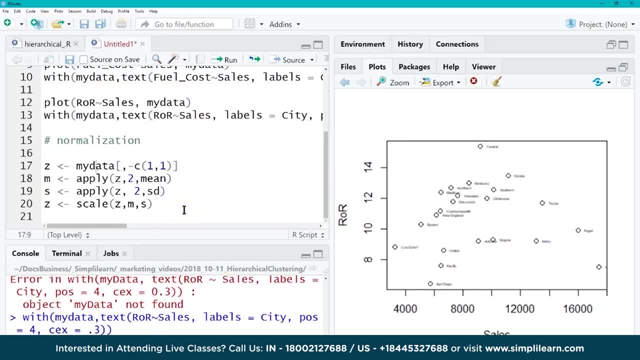 That doesn't help if it is not a linear set of data. So with this we're going to look for the means and the standard deviation for reshaping the data, And that way the most common values now become kind of like the center point. 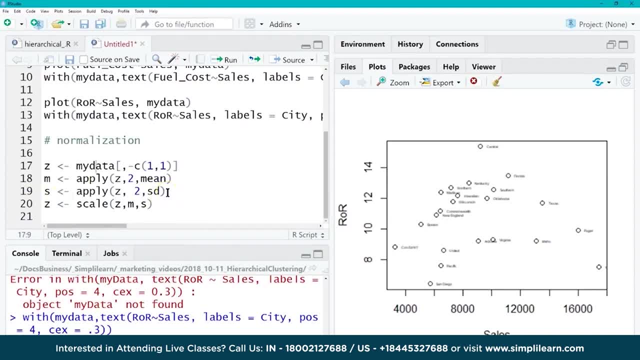 And then the standard deviation is how big the spread. So we want the standard deviation to be equal amongst all of them. And then, finally, we go ahead and take Z And with the Z, we're going to reassign it And we're going to scale the original, my data, which we reshaped. 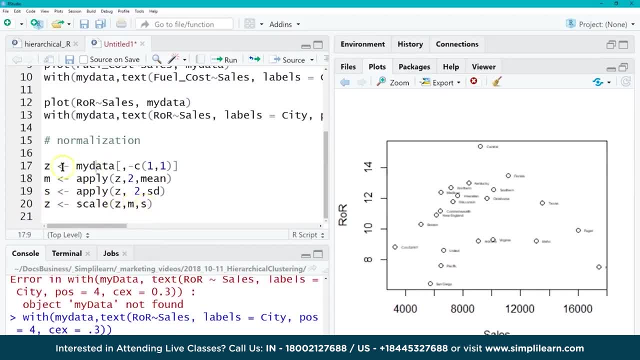 based on M and based on the standard deviation And the 2 in here. That just means we're looking at everything in kind of a XY kind of plot And we can quickly run these Control-Enter, Control-Enter, Control-Enter, Control-Enter. 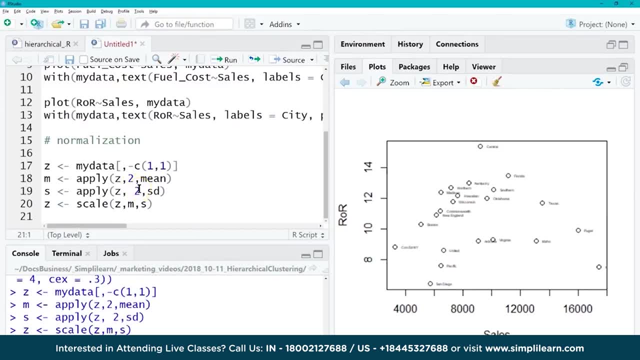 So now we have Z, which is a scaled version of my data, And now we can go ahead and calculate the Euclidean distance. Oops, Calcu, There we go. And in R- this is so easy. Once you've gotten to here- we've done all that pre-data processing. 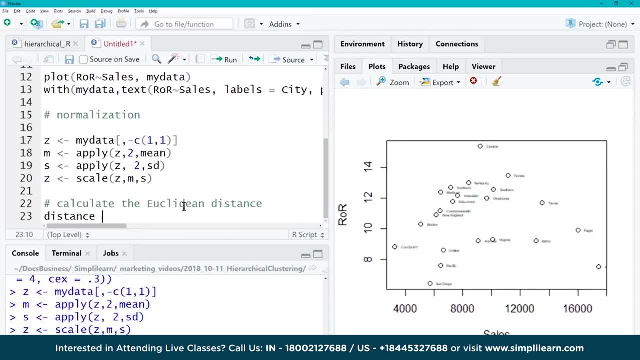 We'll call it distance And we'll assign this to dist. So D-I-S-T is the computation for getting the Euclidean distance, And we can just put Z in there, because we've already reformatted and scaled Z to fit what we want. 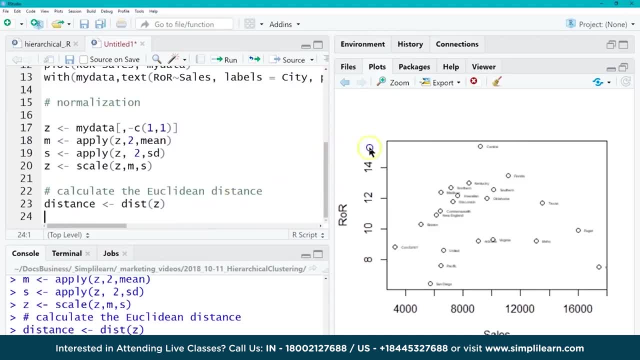 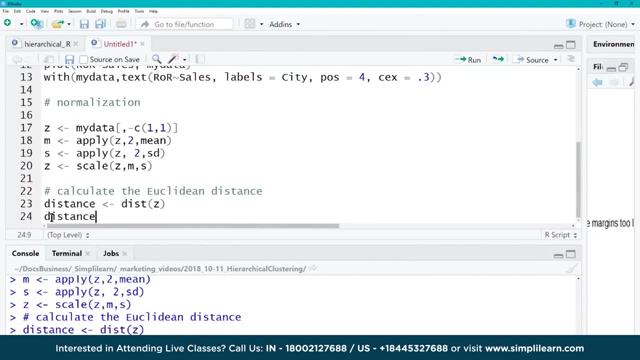 Let me go ahead and just hit Enter on that, And I'm going to widen my left-hand side again. I'm always curious: what does this data look like? So let's just type in distance, which will print the variable down below. 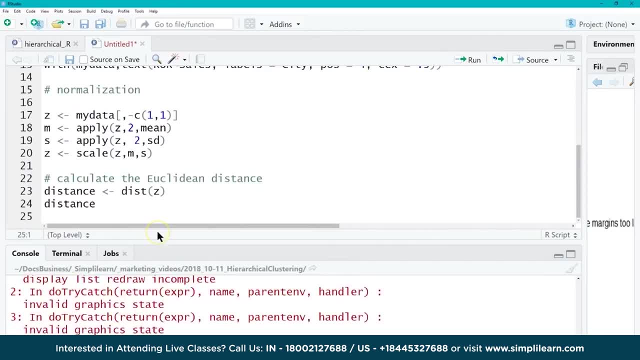 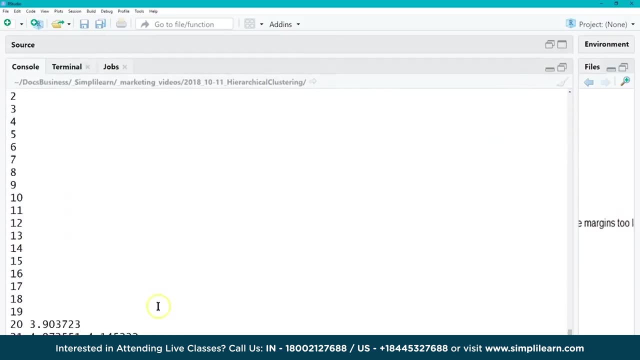 Oops, You have to hit Control-Enter And this prints out a huge amount of information. As you can see, it just kind of streams down there And let's go ahead and enlarge this. And I don't know about you, but when I look at something like this, 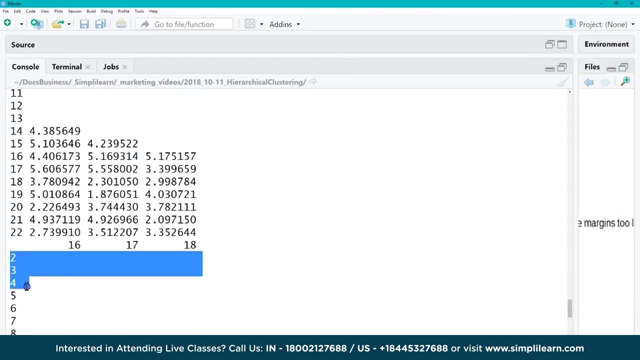 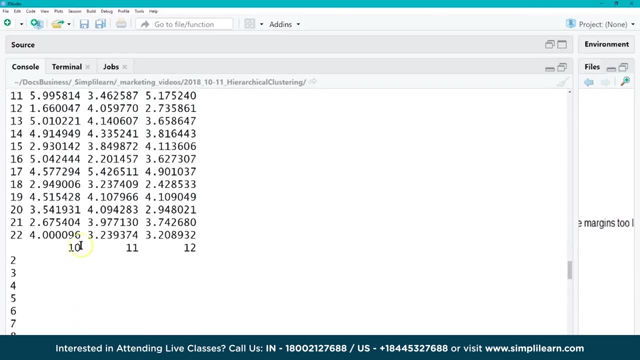 it doesn't mean a whole lot to me, other than I see 2,, 3,, 4,, 5,, 6.. And then you kind of have the top part: 6,, 17,, 18.. So imagine this is like a huge chart. is what we're looking at? 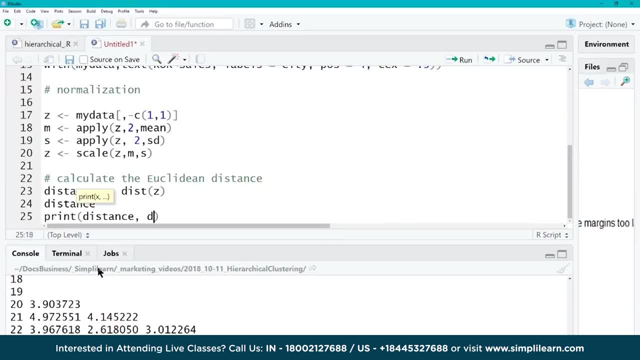 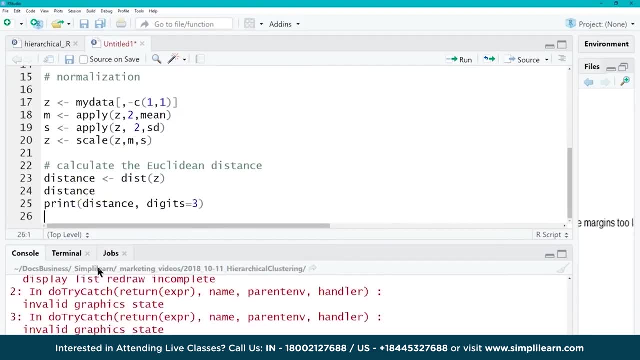 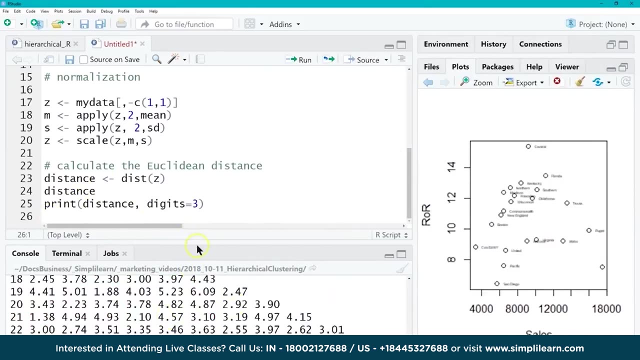 And we can go ahead and use print: Oh, distance digits equal 3.. And let's run that. Oops, I keep forgetting that it has to go through the graph on the right And we see a slightly different output in here. 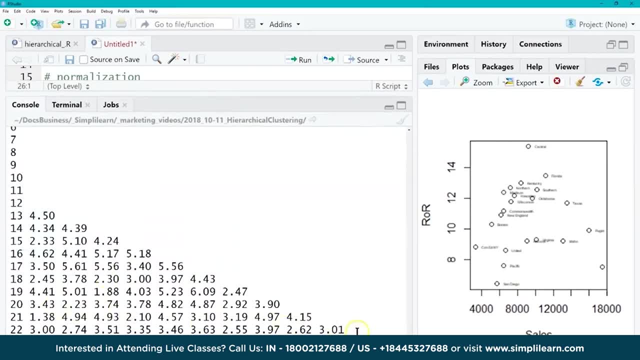 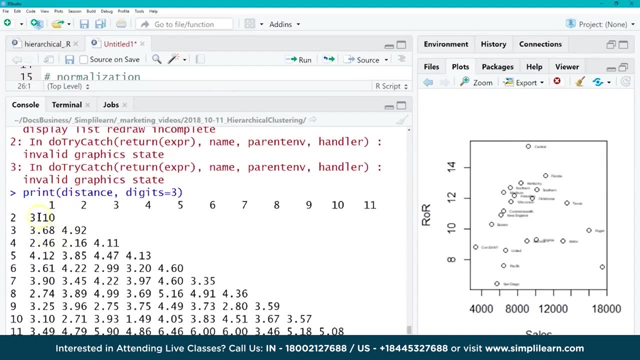 Let me just open this up so we can see what we're looking at, And by cutting down the distance you can start to see the patterns here, if it's looking at the different distances. So if I go to the top, we have the distance between 1 and 2,. 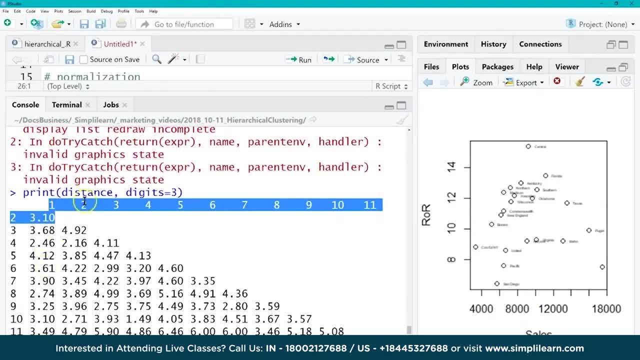 1 and 3, 1 and 4, 1 and 5, 1 and 6, and then 2 and 3, and so on. Obviously, the distance between itself is 0. And it doesn't repeat the data. so we don't care to see 2 versus 1 again. 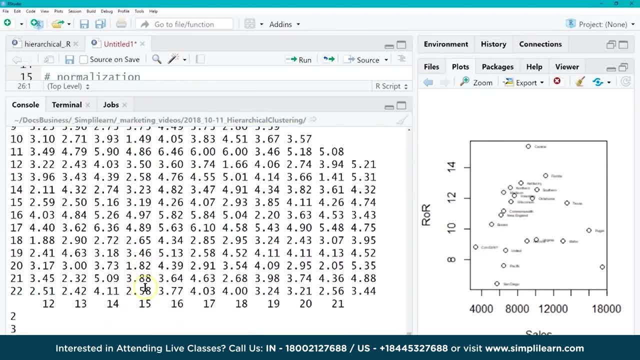 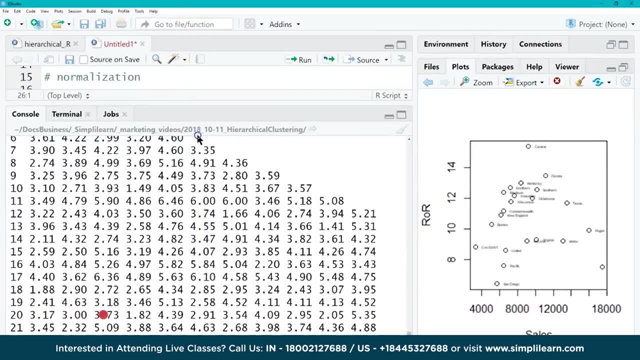 because we already know the distance between 1 and 2. And so we have a nice view of all the distances in the chart and that's what we're looking at right here And it's a little easier to read. That's why we did the print statement up here to do digits equals 3,. 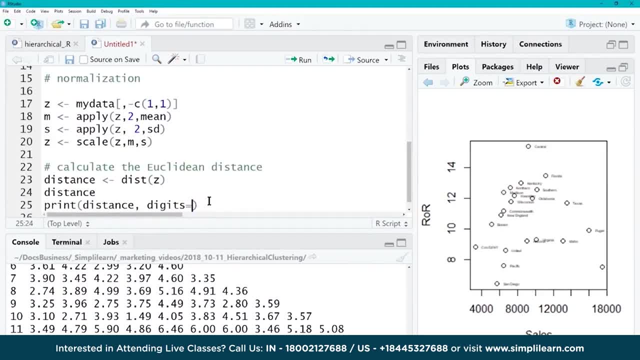 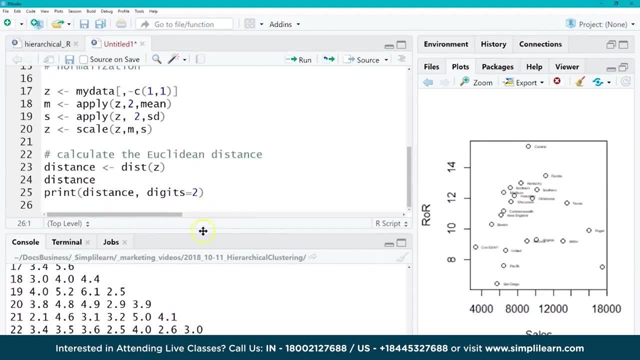 make it a little bit smaller. We could even just do digits. Oh, let's just do 2, see what that looks like. We might lose some data on this one if something's way off, But we have a nice setup and we can see the different distances. 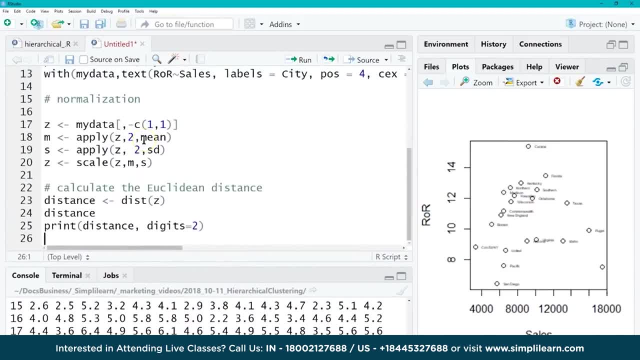 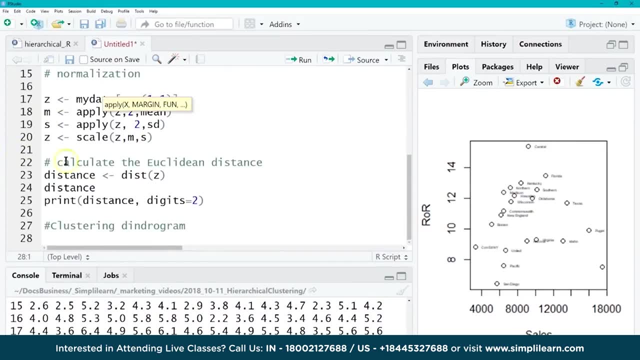 And that's what we've computed here between each of the points, And then the whole reason we're doing this is to get ourselves a nice dendogram going, a nice clustering dendogram. We'll do a couple of these, looking at different things. 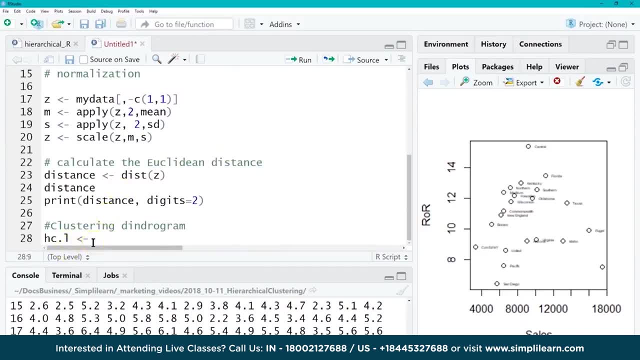 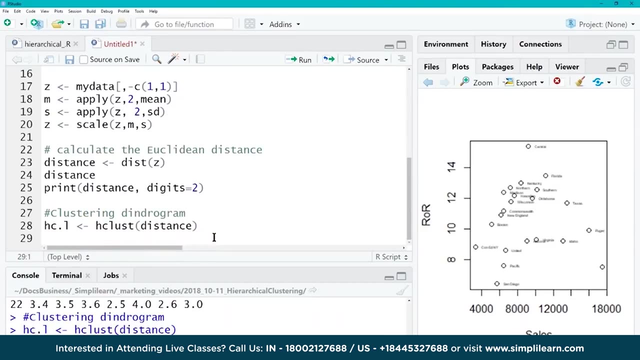 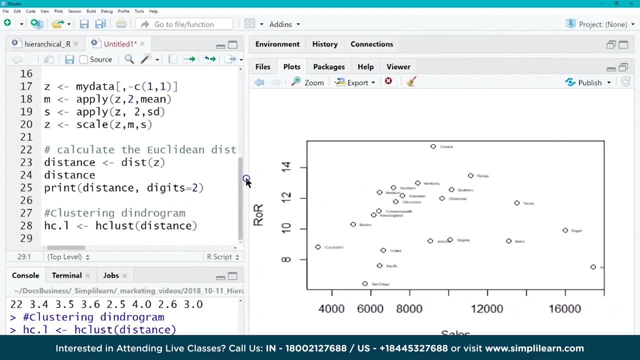 We'll take a variable hcl and we're going to assign it h cluster and then distance. That easy. We've already computed the distances, so the h clustering does all the work for us, And let me hit enter on there. So now we have our hcl, which has assigned the h clustering computation based on distances and apart. 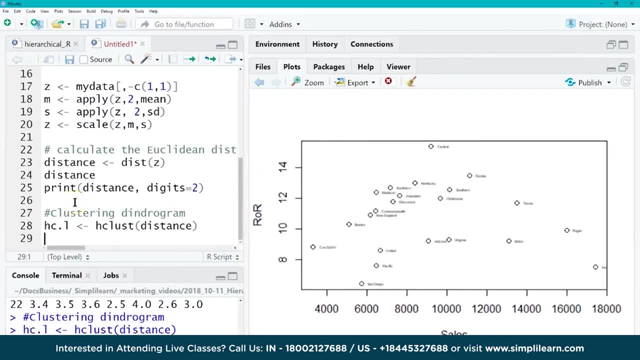 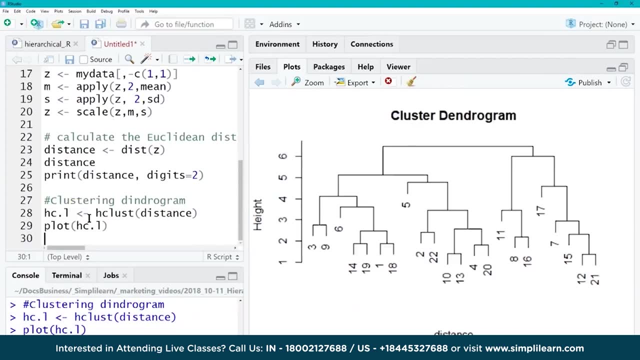 And then I'm going to expand my graph because we would like to go ahead and see what this looks like And we can simply plot that and hit the control enter, so it runs. And look at that, We have a really nice clustering dendogram. 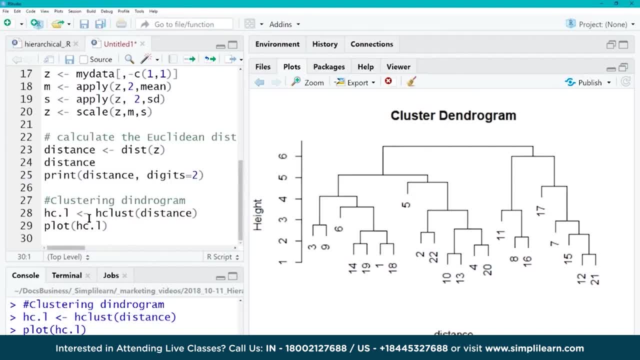 Except when I look at it, the first thing I notice is it really shows like numbers down below. Now, if you were a shareholder and some data scientist came up to you and said: look at this, this is what it means- you'd be looking at that going. 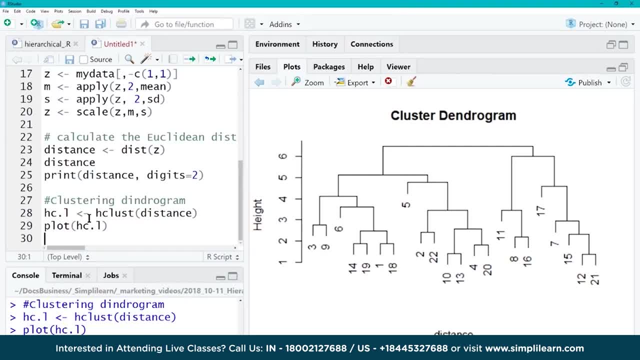 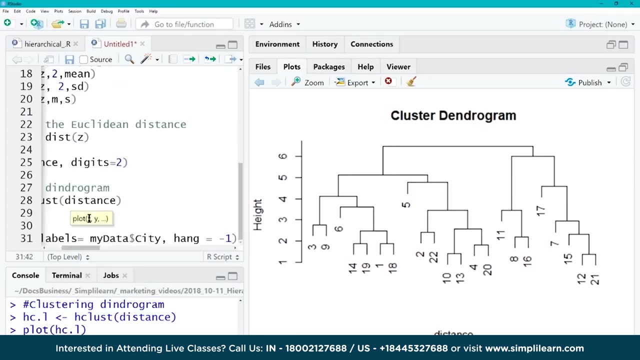 what the heck does. 3,, 9,, 14,, 19,, 1, 18 mean. So let's give it some words there. So let's do the same plot with our hcl, hc. there we go And let's add in labels. 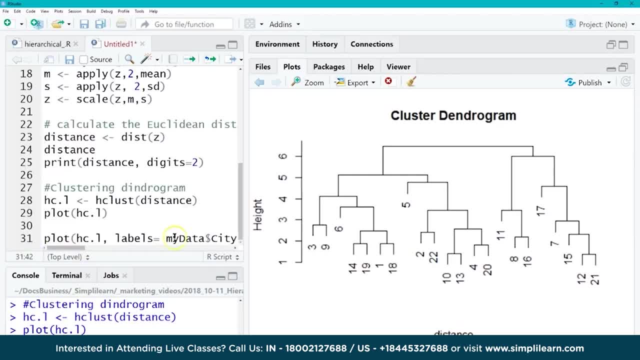 And this is just one of the commands in plots. So we have labels. We have labels equals my data And then, under my data, we want to know the city And we'll have it hang minus 1.. That's just the instructions to make it pretty. 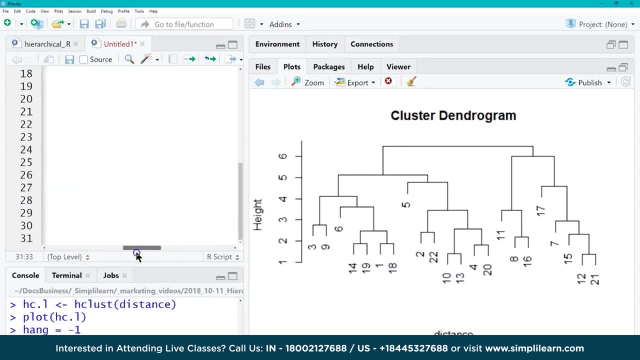 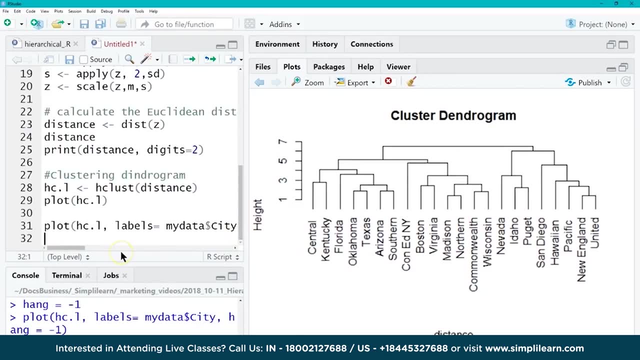 So we'll run that. Oops, I accidentally ran, just hang my 1.. Let me try that again. There we go, OK, So now you can see what it's done, And the hang my 1 turns it sideways. That way we can see central, which is central US, and Kentucky. 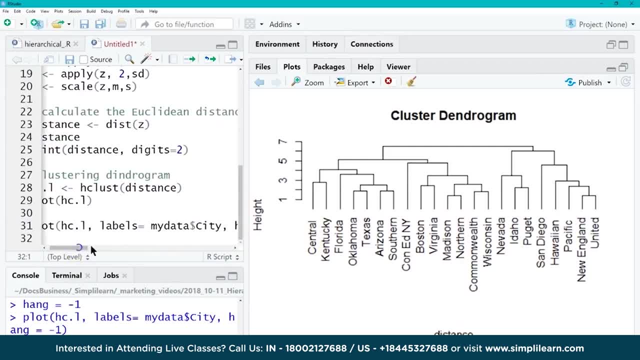 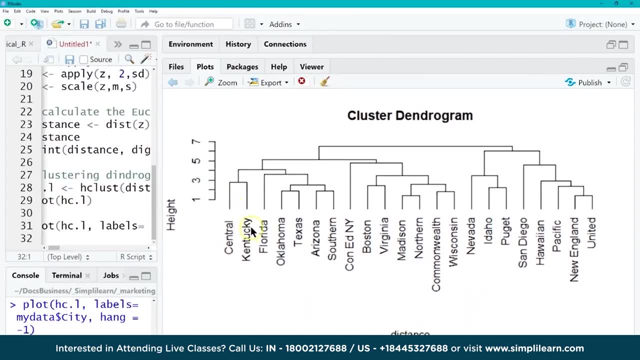 We start to actually get some information off our clustering setup, And the information you start looking at is that, when we put all the information together, you probably want to look at central America and Kentucky together. Oklahoma and Texas has a lot of commonality, as does Arizona and southern US. 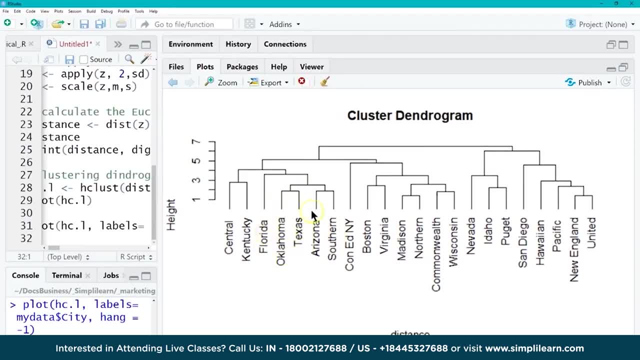 And you can even group all five of those: Florida, Oklahoma, Texas, Arizona and southern US. These regions for some reason share a lot of similarities, And so we want to start asking what those similarities are. But this gives us a place to look. 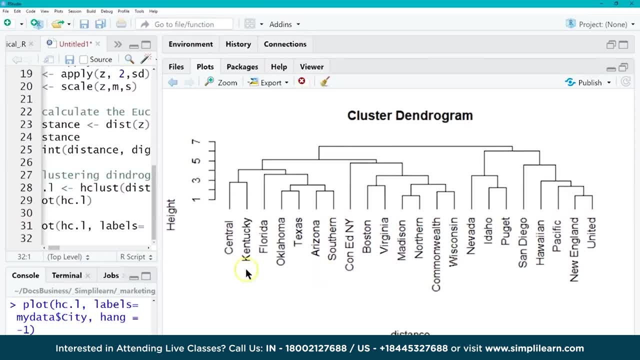 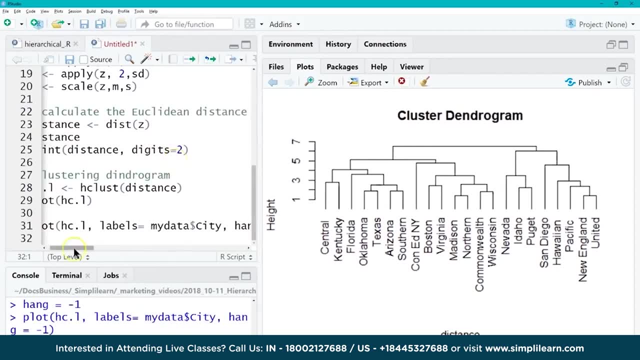 It says, hey, these things really go together. You should be grouping these together as far as your cells and what you're doing, And then one of the things you might want to do is there's also- we can do- the dendrogram average. 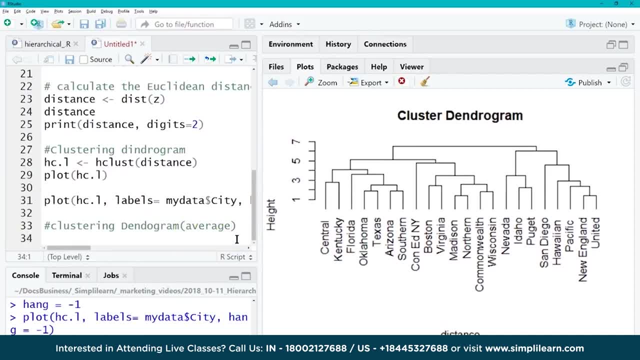 And this changes how we do the clustering, So it looks very similar like we had before. OK, And those are HCL. We're going to assign it. We're going to do an H cluster. We're still doing it on distance. 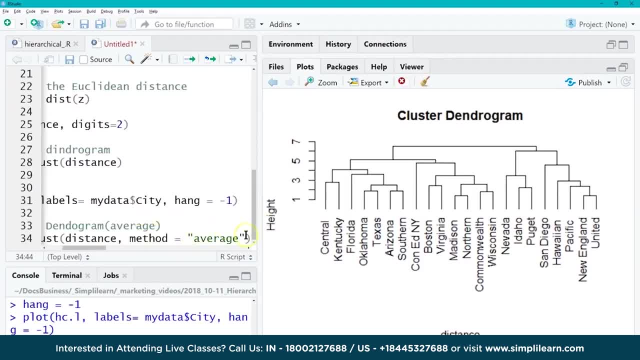 Oops distance, And this time we're going to set the method to average, So we can change the methodology in which it computes the values. And before, if you remember correctly, we did median. Median is a little bit different than means. 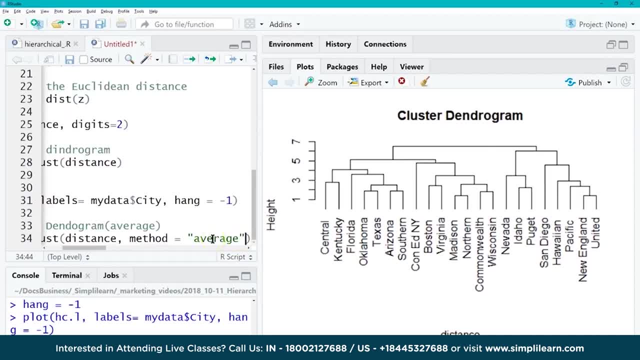 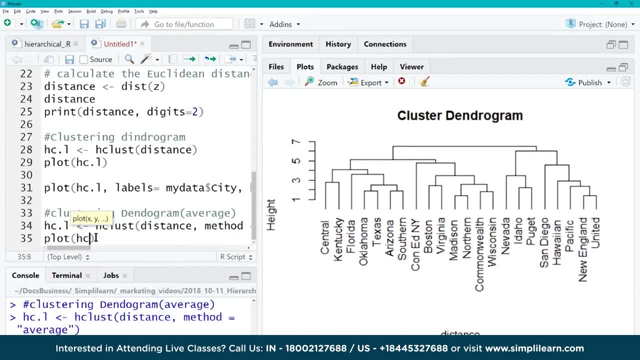 We did the most common one. And then we want the average of the median, And let's go ahead and run that. And then we can plot. And here's our HCL. Oops, there we go, Here's our HCL. 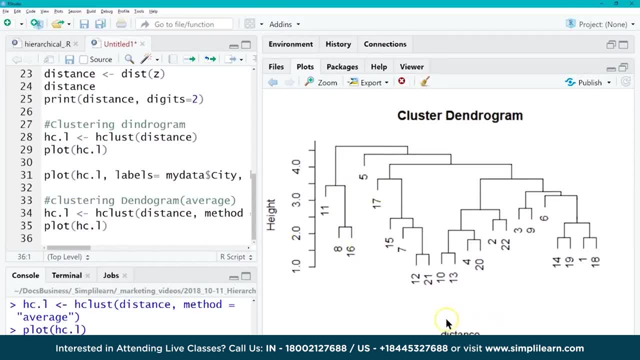 And I can run that plot And you can see this changed a little bit. So our way it computes and groups things looks a little different than it did before And let's go ahead and put the cities back in there and do the hang. 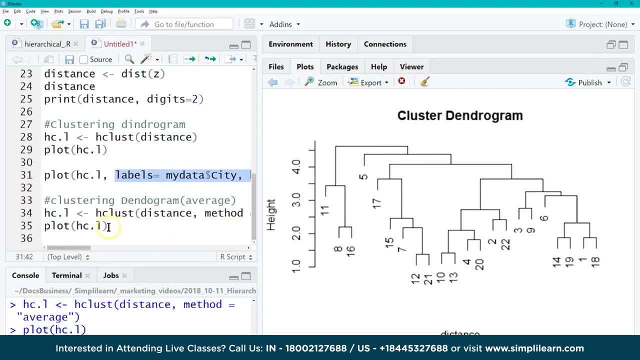 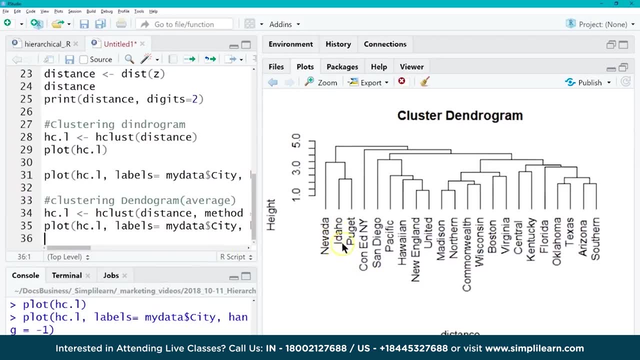 Control copy. Let me just real quickly copy that down here Because we want the same labels. And again you can see Nevada, Idaho, Puget, I remember we were looking at southern US and Arizona, Texas and Oklahoma, Florida. 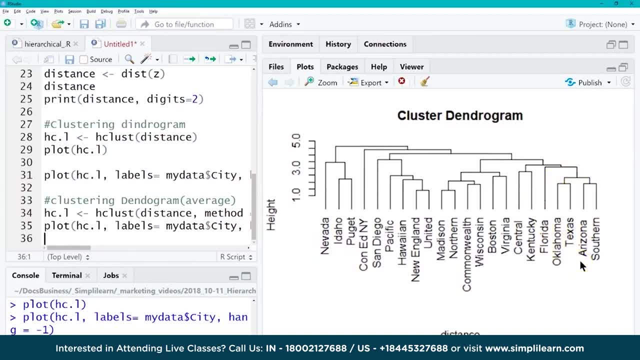 So the grouping really hasn't changed too much. So we still have a very similar grouping. It's almost kind of flipped it as far as the distance based on average has, But this is something you could actually take to the shareholders and say, hey look. 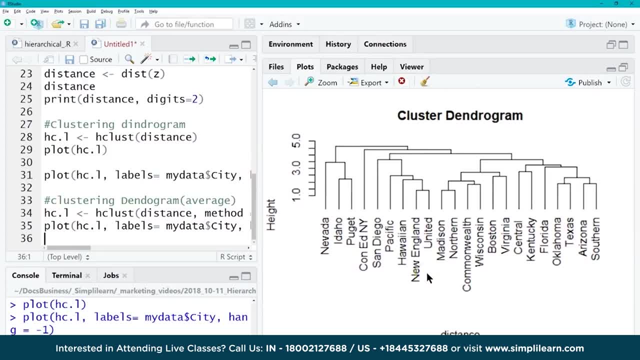 These things are connected And at which point you want to explore a little deeper as to what's going on. You want to explore a little deeper as to why they're connected, Because they're going to ask you: okay, how are they connected and why do we care? 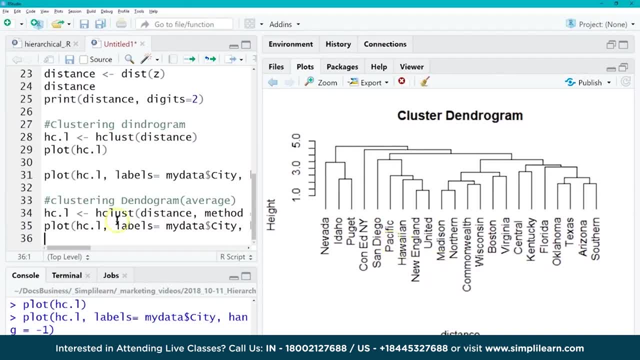 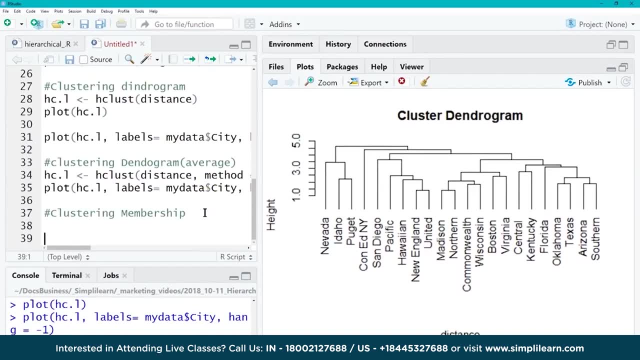 But that's a little bit beyond the actual scope of what we're working on today. But we are going to cover membership- What's called clustering membership- on there And let's create a member. We'll just call it member one. Oops there. 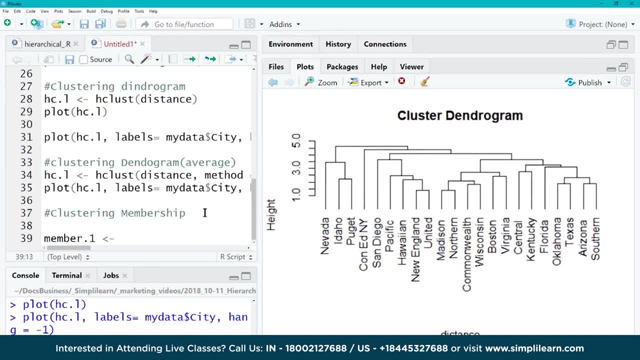 Member dot one, And we're going to assign to this. We're going to do cut tree And cut tree, it limits it. So what that means is I take my hc dot l in here. Oops, there we go Dot l. 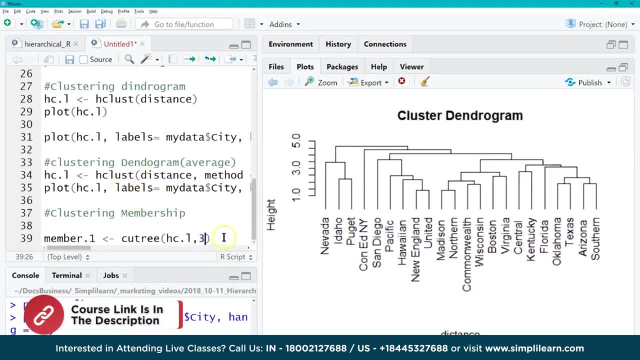 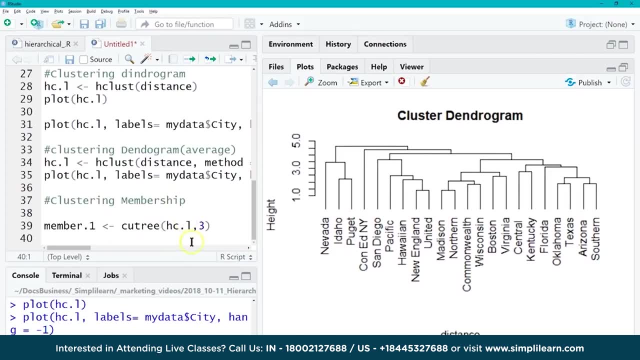 And so I'm taking the cluster I just built And we want to take that cluster and we want to limit it to just a depth of three. So we go ahead and do that and run that one. Oops, let me go run. There we go. 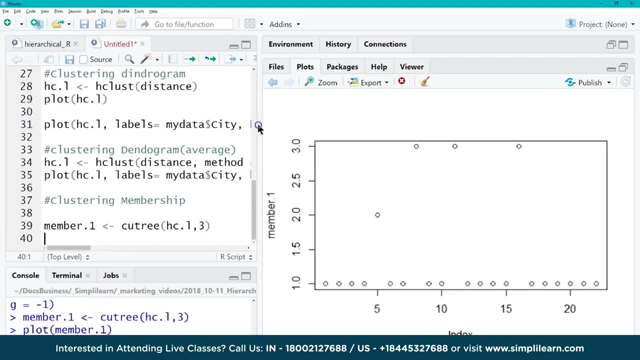 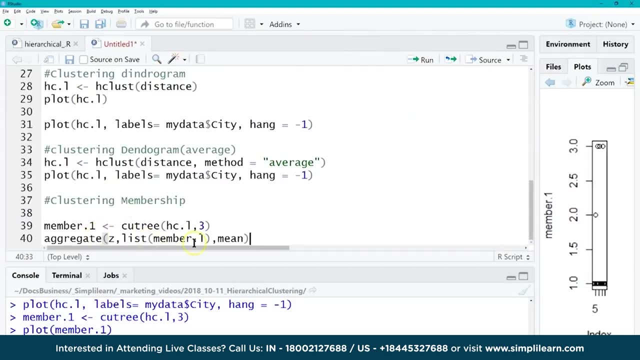 So now I've created my member one And then whoops, let me just move this out of the way. We're going to do an aggregate And we're going to use z- Remember z- from above, And we're going to turn member one into a list. 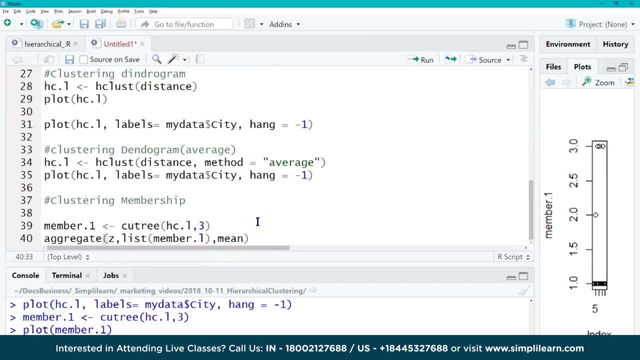 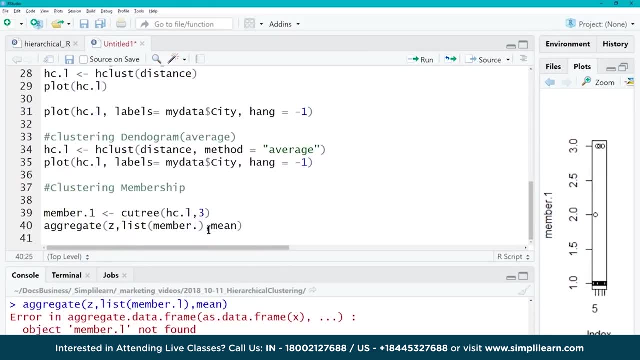 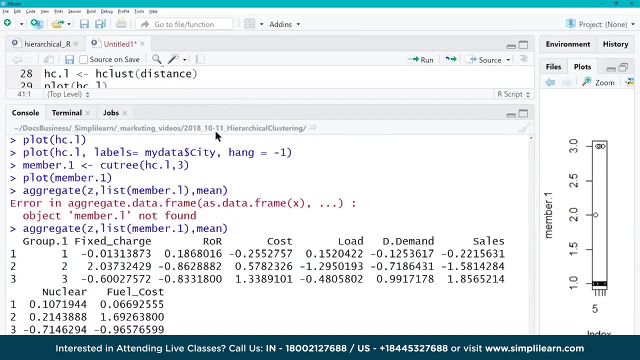 And then we're going to aggregate that together based on the mean. Let me go ahead and hit enter and run that. Oops, I did member l. It's actually member one. There we go, And if we take a look at this, we now have our group, one fixed charge and then all your different columns listed there. 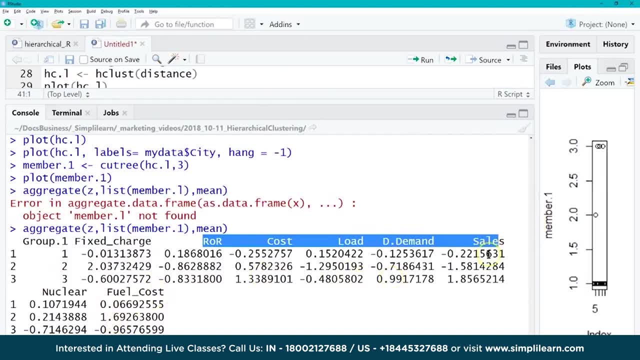 And most of them should come up kind of looking between zero and one. But you'll see a lot of variation because we're varying it based on the means. So it's a means, a standard deviation, not just forcing it in between zero and one. 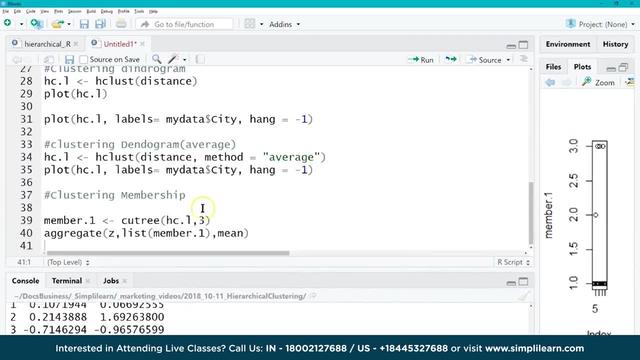 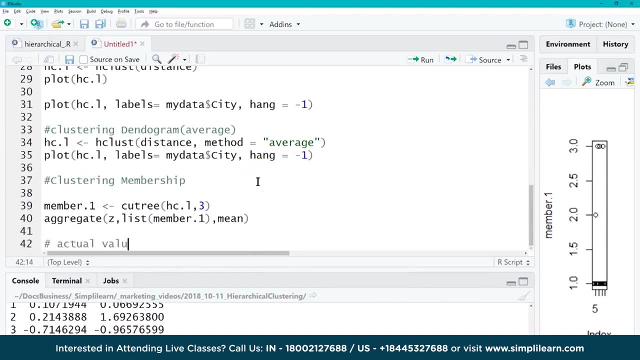 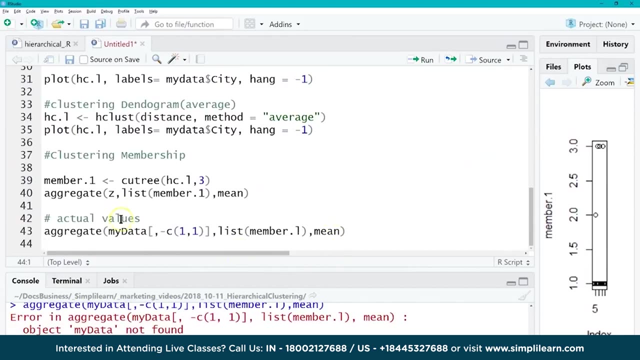 Which is a much better way usually to normalize your data than just doing the zero one setup. And finally, we can actually look at the actual values in the same chart we just did- Oops, I made a mistake on there with my data. There we go. 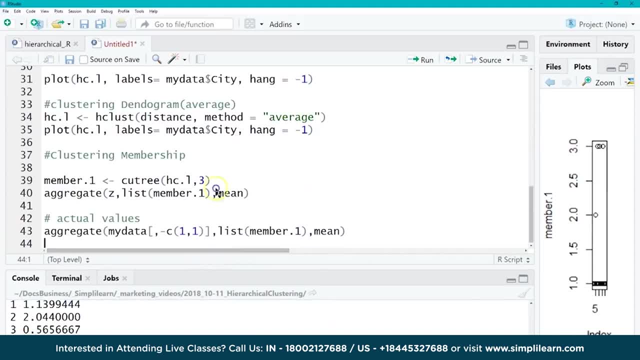 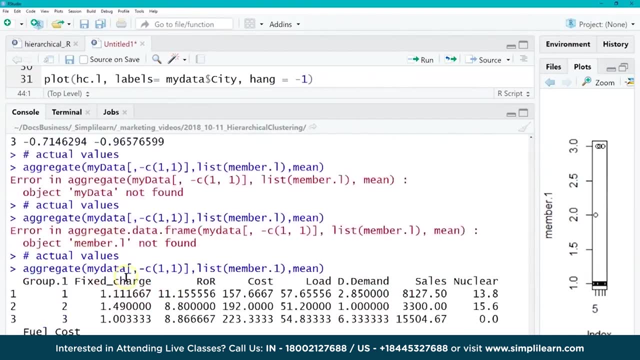 Okay, And again we now have our actual data, instead of looking at just the. if you looked up here, it's all between zero and one, And when we look down here, we now have some actual connections in between zero and one. 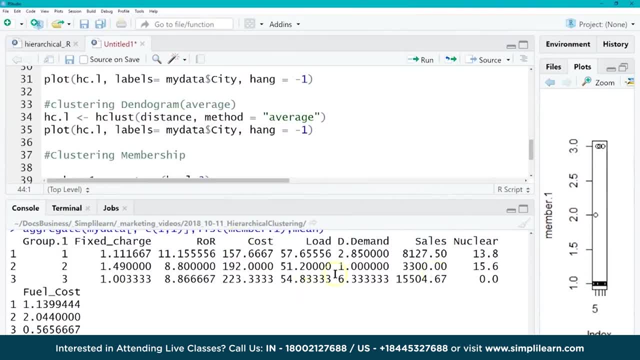 We now have some actual connections in how far distance this different data is, Again because more of a domain issue and understanding the oil company and what these different values means And you can look at these as being the distances between different items. So a little bit different view and you have to really dig deep into this data. 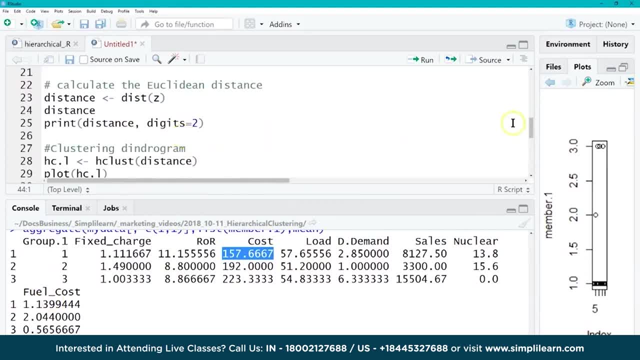 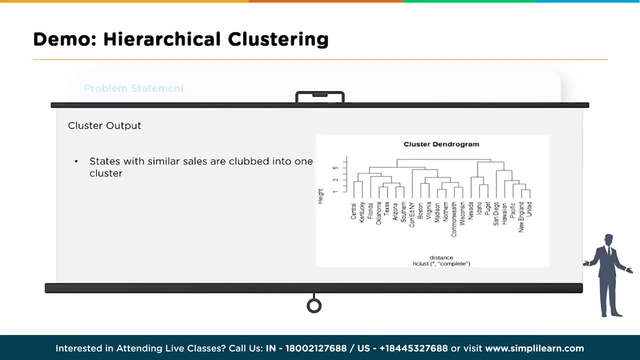 What we really want you to take away from this is the dendogram and the charts that we did earlier, And that is the cluster output and our nice dendogram. So this would be stage one in data analysis of the cells. Again, you'd have to have a lot more domain experience to find out what all the individual numbers we looked at mean. 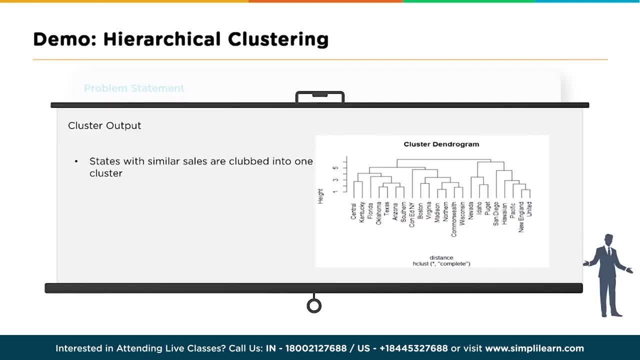 And what the distance is and what's the difference between Central America and Kentucky and why they're similar And why it groups all of Central Kentucky, Florida, Oklahoma, Texas, Arizona and Southern US together into one larger group. So it'd be way beyond the scope of this. 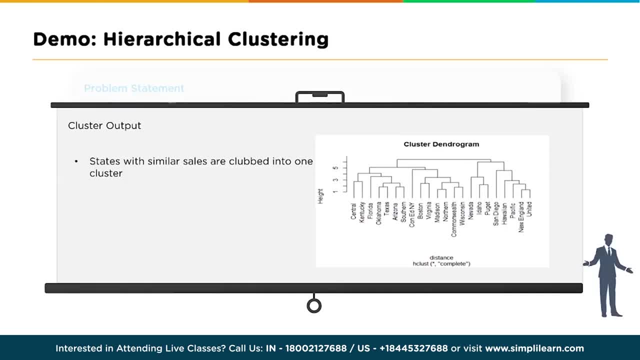 But you can see how we start to explore data and we start to see things in here, where things are grouped together in ways we might not have seen before, And this is a good start for understanding and giving advice for cells and marketing, maybe logistics, city development, 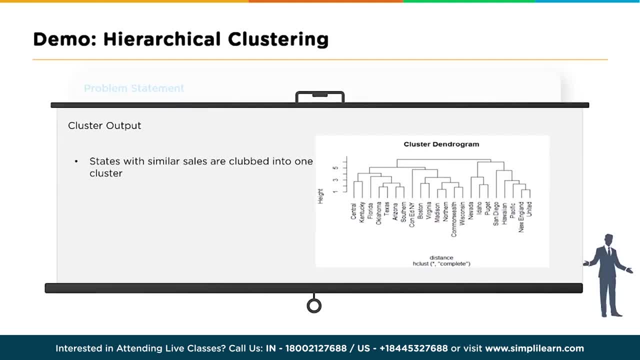 There's all kinds of things that kind of come together in the hierarchical clustering as you begin to explore data, And we just want to point out that we get three clusters: of regions: with the highest cells, region with average cells, region with the lowest cells. 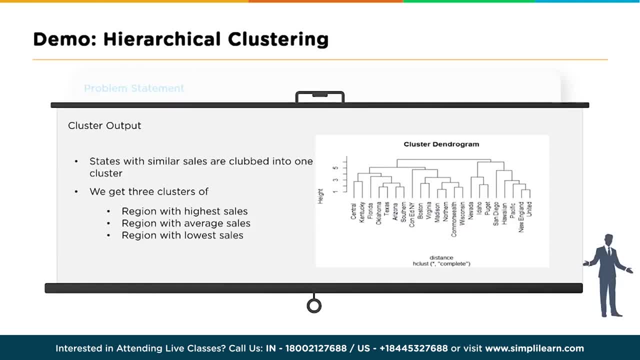 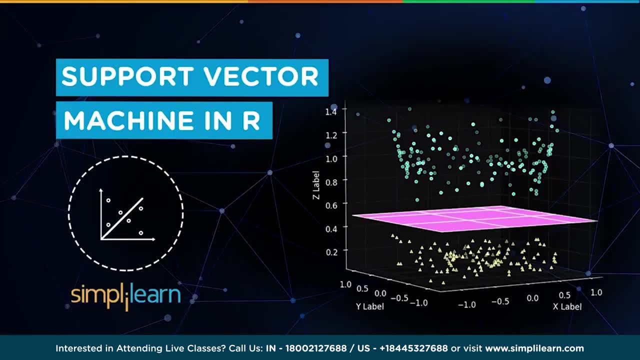 Again, those are some of the things that they clustered it around and you could actually see where things are going on or lacking, In this case, if you're the lowest cells. no one wants to be in the region of the lowest cells. Support Vector Machine is a binary classifier, a supervised machine learning algorithm. 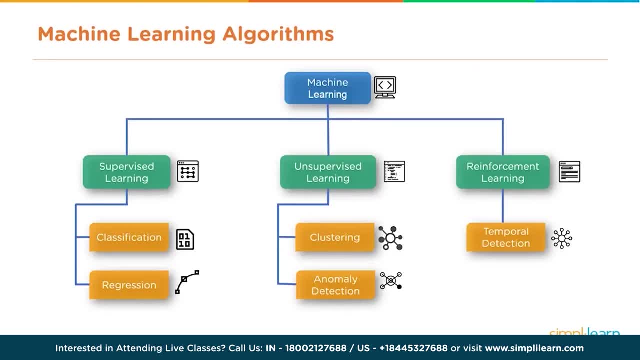 And in this video we will learn what all that means. Machine learning algorithms come in three major flavors: Supervised learning algorithms, unsupervised learning algorithms and reinforcement learning. And today we'll cover classification under supervised learning. Supervised meaning the data set has known outcomes. 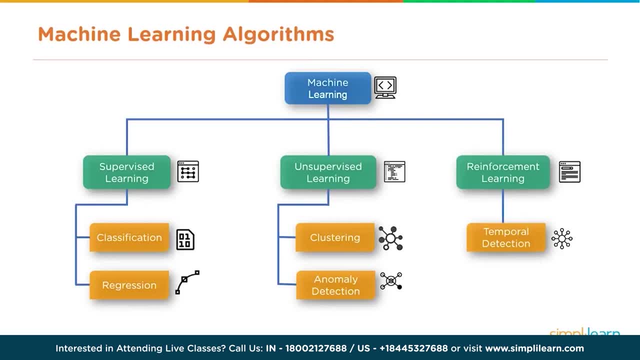 If it were unsupervised it would not have known outcomes And we wouldn't have the categories or classes necessary for the machine to learn. But under supervised learning we do have the known outcomes in the data set And under supervised learning there are two major types of machine learning algorithms. 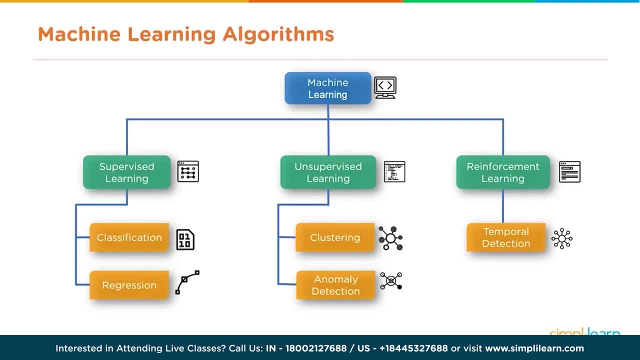 Classification, which we'll cover today, support vector machine and regression. Classification. you predict categories And in regression you generally predict values. So while we look at supervised learning, keep in mind that classification can really be considered multidimensional, In the sense that sometimes you only have two classes: yes or no, true or false. 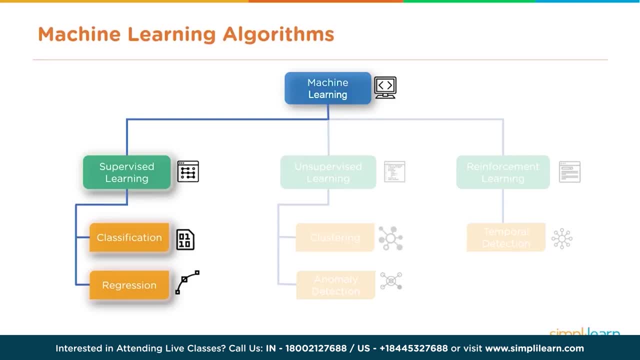 And sometimes you have more than two classes. Sometimes you have, say, under risk management or risk modeling, low risk, Low risk, medium risk or high risk, And SVM is a binary classifier. It is a classifier used for those true-false, yes-no types of classification problems. 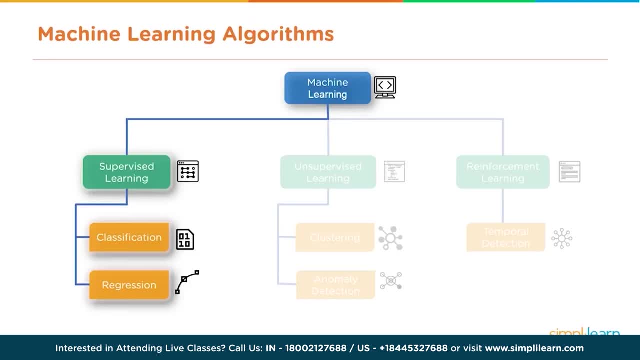 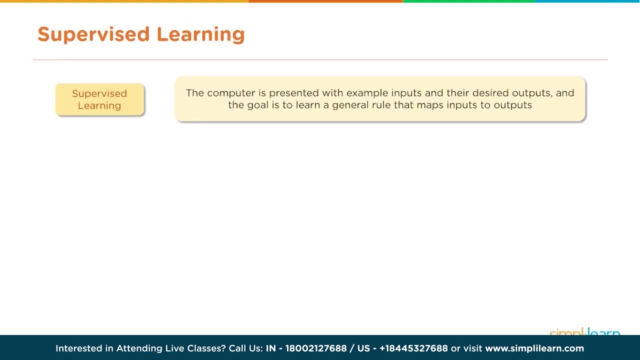 And in supervised learning, features are important. If there are a lot of features, SVM may be the better classification algorithm choice As opposed to say logistic regression. So for supervised learning, the computer is presented with examples. It is presented with example inputs and their desired outputs, those known outcomes. 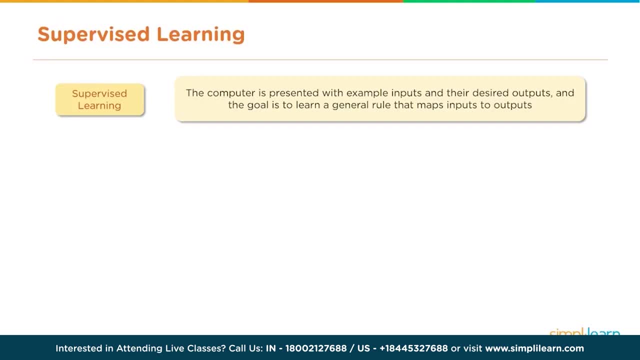 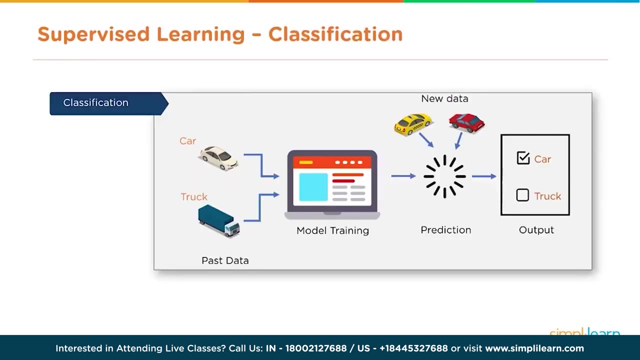 And the goal is to learn a general rule that maps inputs to those outputs, For example, bug detection or customer churn, or stock price prediction- Not the value of the stock price, but whether or not it will rise or fall. And weather prediction: sunny, not sunny, rain, no rain. 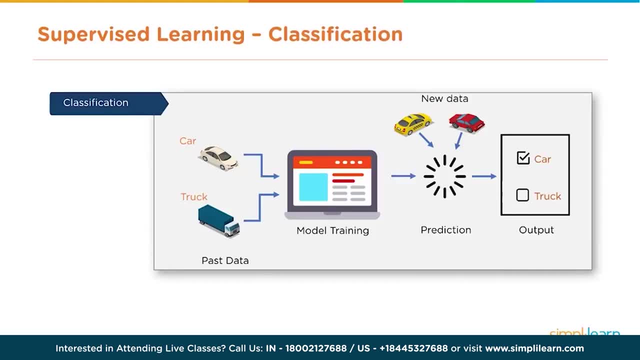 Classification algorithms generally take past data, data that we have, those known outcomes. train the model, take new data once the model is trained, ingest it into the model and create predictions- Is it a truck or is it a car? And keep in mind that I said features are important. 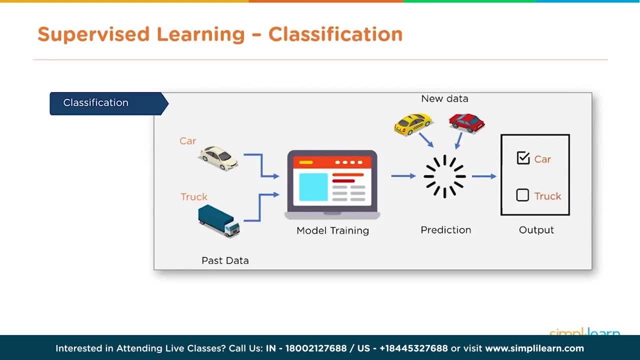 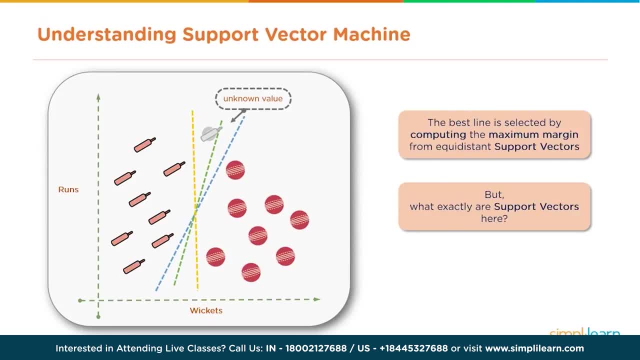 What line best separates the data. We'll find the best line by computing, by computing the maximum margin from equidistant support vectors. support vectors in this context simply means the two points, one from each class, that are closest together, but that. 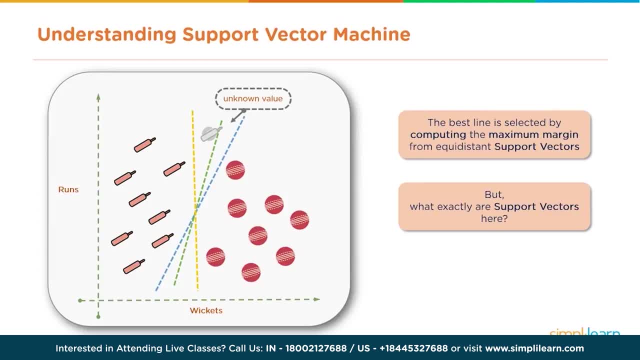 maximize the distance between them or the margin. So the word vector here you may think, Well, he really means points, data points. data points, Well, in two-dimensional space, yes, data points, Well, in two-dimensional space, yes. 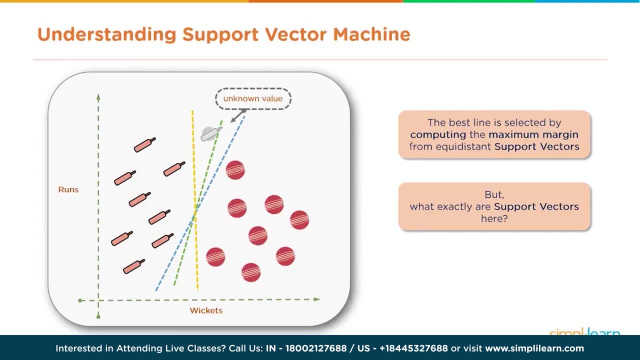 maybe even in three-dimensional space. but once you get into higher dimensional spaces, when you get more and more features in your data set, you have to consider these as vectors. you can no longer really describe them as points, so we call them vectors and the reason they're support vectors. 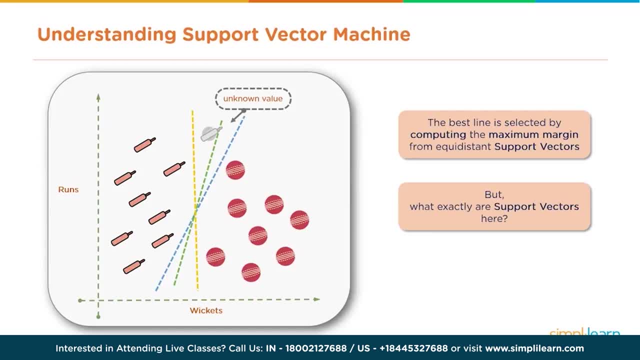 is because the two vectors that are closest together, that maximize the distance between the two groups, support the algorithm. so that's why we call them support vectors. so if you look at our example, there are a couple of points at the top that are pretty close to one another and a couple 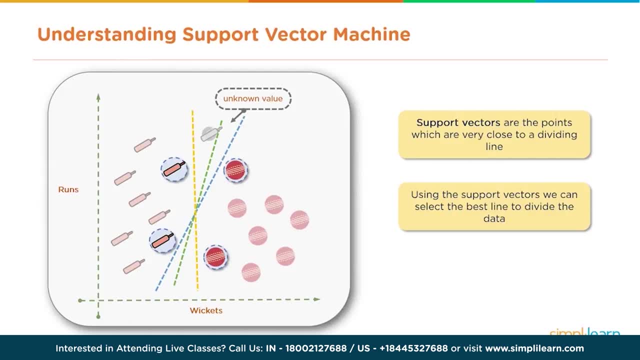 of points at the bottom of that graph that are pretty close to each other and we're not really sure, looking at the graph, which two are closest, but clearly those points are the ones we need to consider. the rest of the other points are too far away from the rest of. 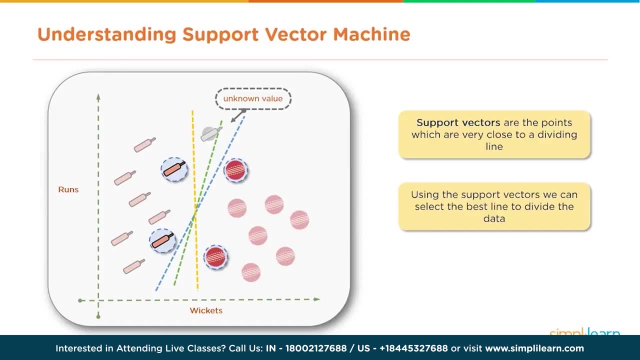 you. the other points, in other words the bowler points, are far to the right and the batsman data points are far to the left. so we'll look at these four points. to begin with, mathematically, we would calculate the distance among all of these points and we would minimize that distance once we pick. 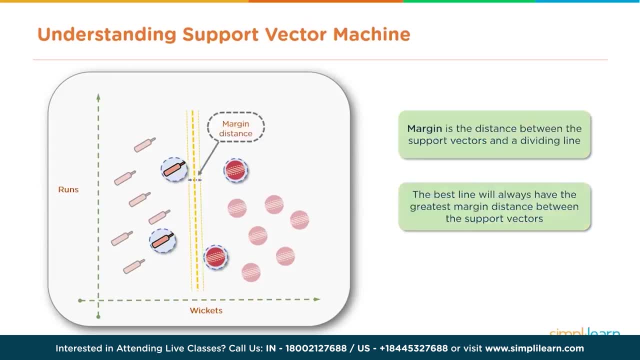 the support vectors. we'll draw a dividing line and then measure the distance from each support vector to the line. the best line will always have the greatest margin or distance between the support vectors. if we consider the yellow line as a decision boundary, the player with the new data point would be considered a bowler. the margins don't appear to be maximum, though, so maybe 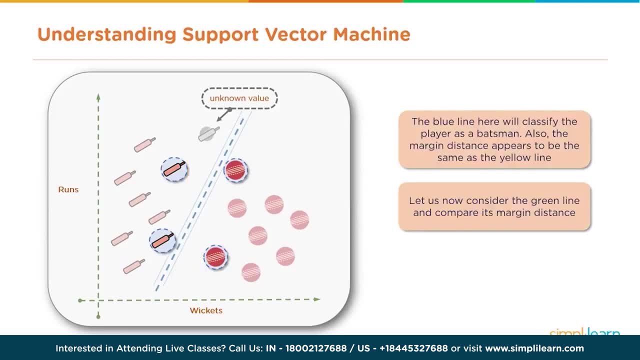 we can come up with a better line. so let's take two other support vectors and we'll draw the decision boundary between those, and then we will calculate the margin and notice now that the unknown data point, the new value, would be considered a batsman- we would continue doing this- and obviously, a 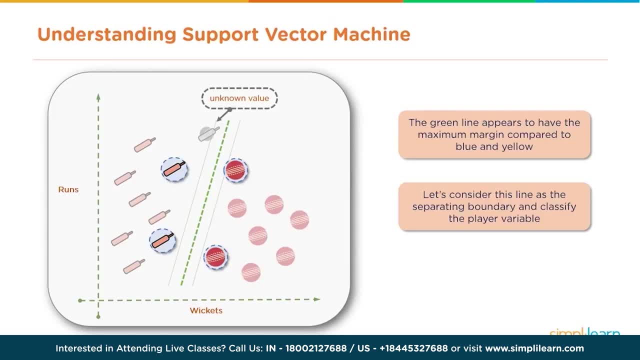 computer does it much quicker than a human being. over and, over and over again, until we found the correct decision boundary with the greatest margin. and in this case, if you look at the green decision boundary, the green line appears to have the maximum margin compared to the other two, and so 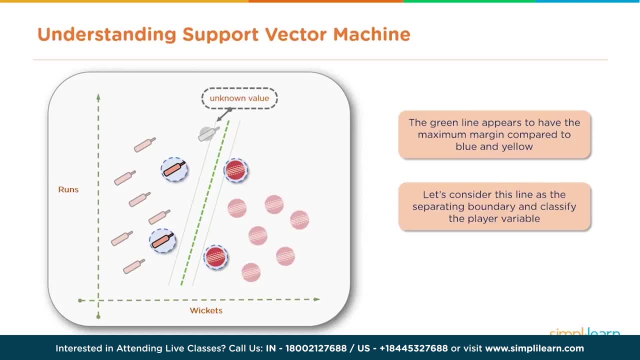 let's consider this, the boundary of greatest margin, and now classifier unknown data value. and now clearly it belongs in the batsman's class. the green line divides the data perfectly because it has the greatest margin, or the maximum margin between the support vectors, and now we can have: 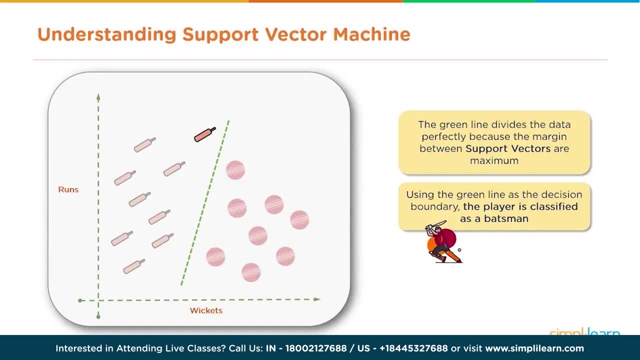 confidence in our classification that the new data point is indeed a batsman. technically this dividing line is called a hyperplane, and the reason it's called a hyperplane will become a little bit more evident in a few minutes. generally in two-dimensional space we consider those lines, but in 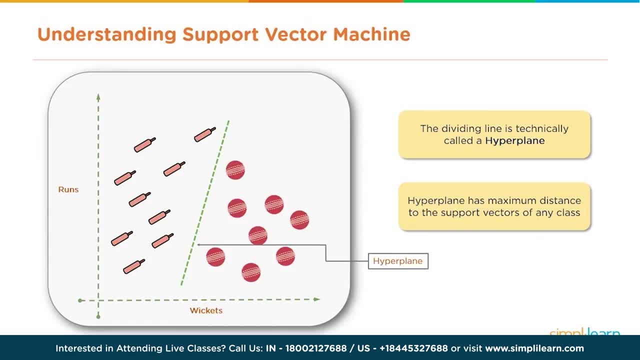 three-dimensional space and higher dimensional spaces. they're considered planes or hyperplanes, so we always tend to refer to them as hyperplanes, and the hyperplane that has the maximum distance from the support vectors is the one we want, so sometimes called the positive hyperplane. d plus is 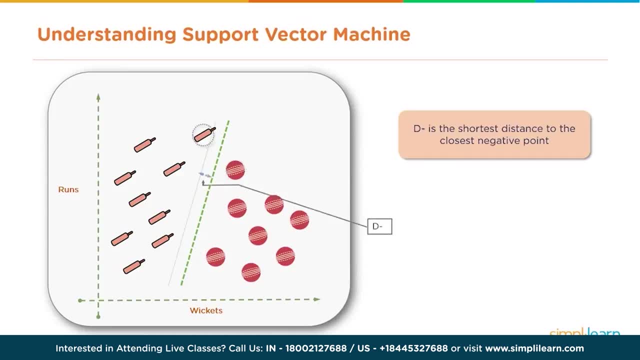 the shortest distance to the closest positive point and d minus, sometimes called the negative hyperplane, is the closest shortest distance to the closest negative point and the sum of d positive and d negative is called the distance margin. so if you calculate those two distances and add them up, 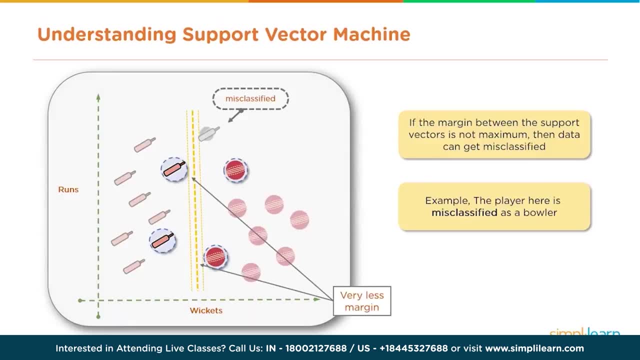 to make that the distance margin and we always want to maximize that. if we don't maximize it we can have a misclassification and you can see the yellow margin is much smaller than the green margin. so this problem set is two-dimensional because the classification is only between two. 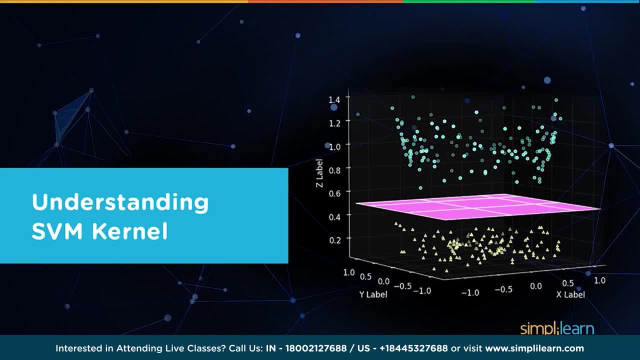 classes, and so we would call this a linear SVM. now we're going to take a look at kernel SVM, and if you notice in this picture, this is a great depiction of a plane, not a line. this is three- dimensional space. so that's the plane. that's going to be a three-dimensional space. 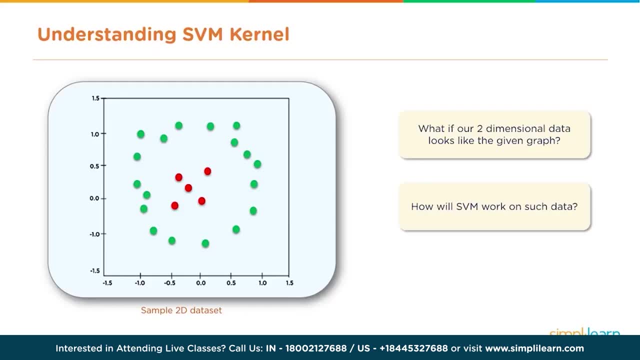 that separates those two classes. So what if our two-dimensional data looks like this? What if there's no clear linear separation between the two classes and machine learning parlance? We would say that these are not linearly separable. How could we get support vector machine? 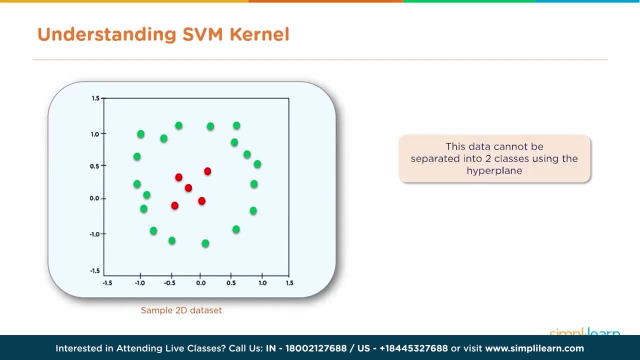 to work on data that looks like this: Since we can't separate it into two classes using a line, what we're going to do, and clearly there's no line- I mean, convince yourself, there's no line that goes and separates those two classes. 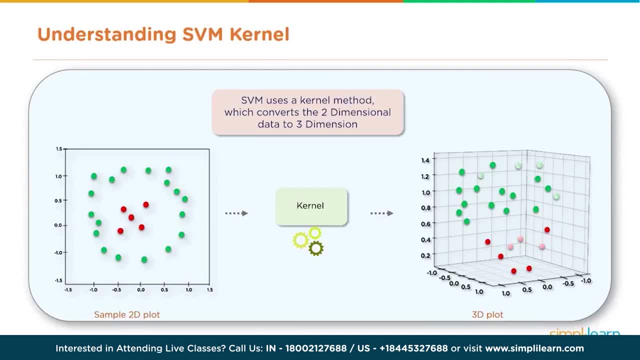 So what we would do is we would apply some type of transformation to a higher dimension. We would apply a function called a kernel function to the dataset, such that the dataset would be transformed into a higher dimension, a dimension high enough where we could clearly separate the two groups. 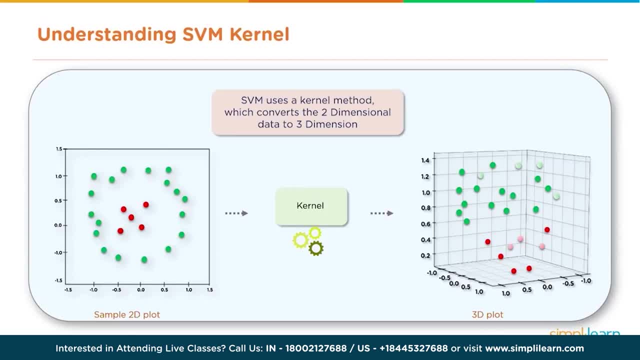 the two classes, in this case with a plane, much the same way. you saw the picture a few slides ago where the plane was separating the two classes. Here we clearly could draw some planes between the green dots and the red dots, And of course we could draw an infinite number of planes. 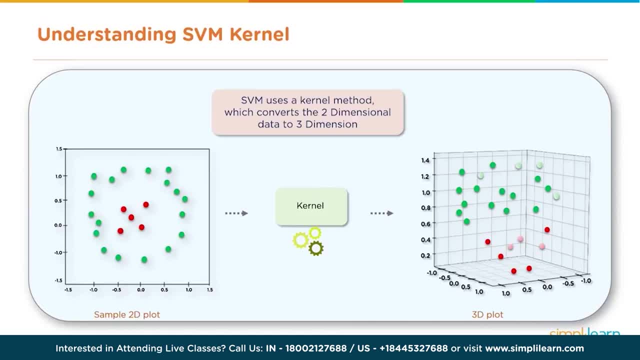 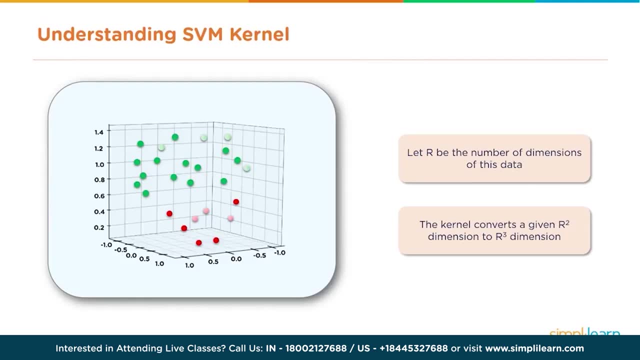 separating those two classes, but we would draw the one that would maximize the margin. So if we let r be the number of dimensions, then the kernel function would convert a given two-dimensional space to a three-dimensional space And, as I said, once the data is separated in three dimensions, 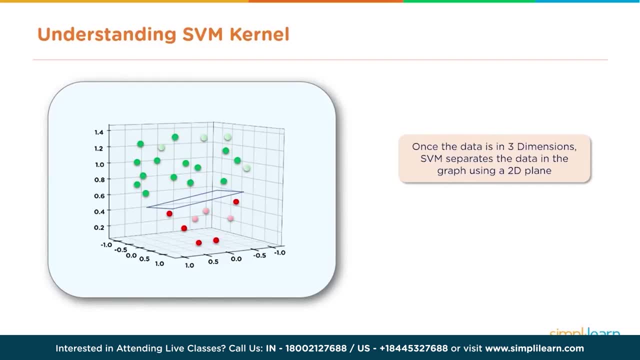 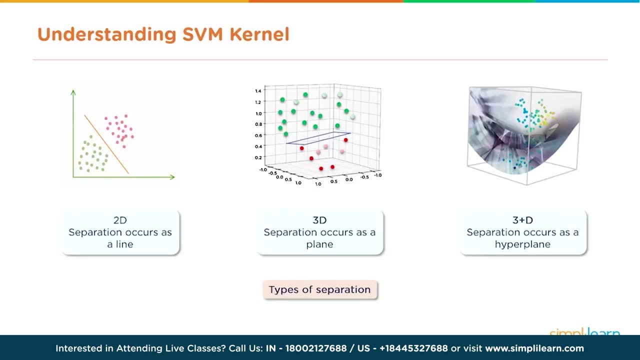 we can separate the two groups using a two-dimensional plane And this is analogous in the higher dimensions- And that last picture on the right-hand side would be some type of depiction of a higher dimension hyperplane- And there are more than one type of kernel function. 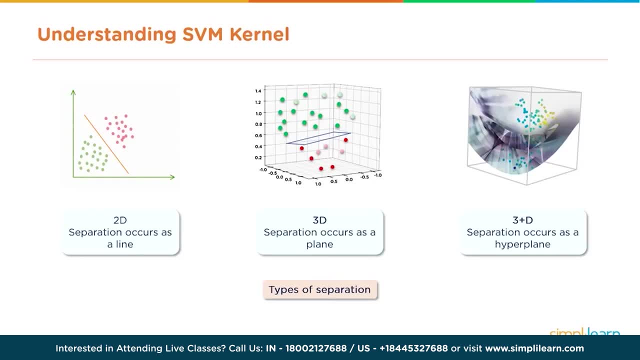 There's Gaussian RBF kernel, sigmoid kernel, polynomial kernel, depending on the dimension and how you want to transform the data. There are more than one choice for kernel functions. So now let's go through a use case. Let's take a look at horses and mules. 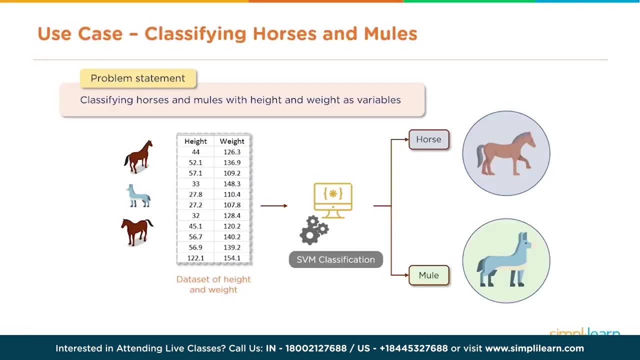 and see if we can use SVM to classify some new data. So the problem statement is classifying horses and mules And we're going to use height and weight as the two features And obviously horses and mules typically in general. 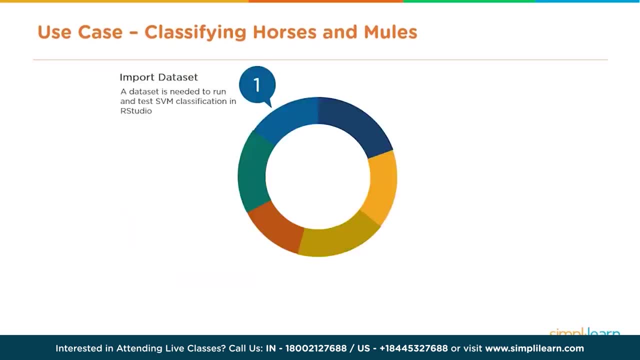 tend to weigh differently and tend to stand taller. So we'll take a data set, We'll import the data set, We'll make sure we have our libraries. The E1071 library has the data set. It has support vector machine algorithms built in. 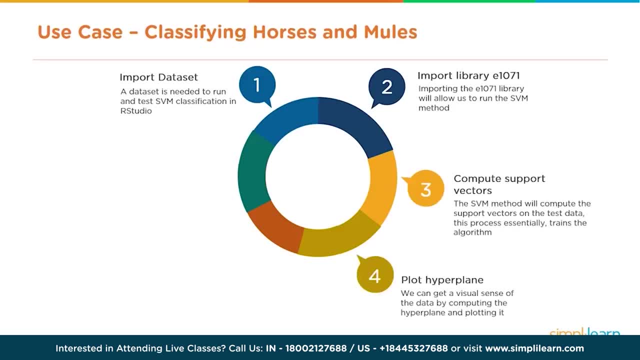 We'll compute the support vectors using the library. Once the data is used to train the algorithm, we'll plot the hyperplane, get a visual sense of how the data is separated, And if it's two-dimensional or three-dimensional, that's great. 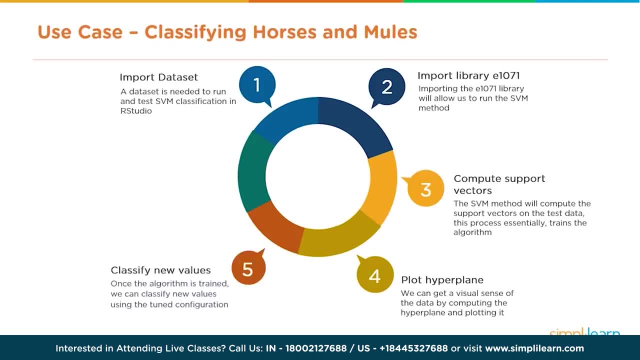 Remember, if it's higher dimensional, it's tough to plot those. And then we'll use the new model, the trained model, to classify new values. In general, we would have a training set, a test set, then ingest the new data, but for our example, we're just going to use the 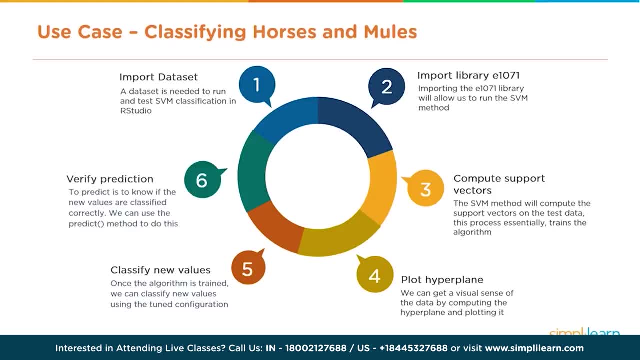 whole data set to train the algorithm and then see how it performs. and once we see how it performs we'll see: did we get a horse? did we predict a horse when we had a horse? did we predict a mule when we had a mule? so here's the R code of 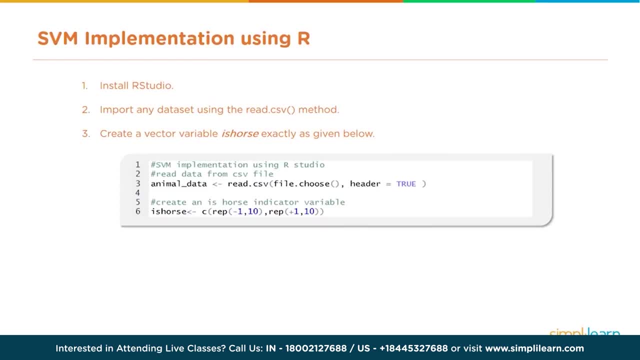 course, if you want to run this R code, you'll have to install R and then R studio. then you'll have to ingest the data and then you'll have to create an indicator variable to help us with our plots. we'll install our libraries, install the package if you don't already have it installed- I do- and then 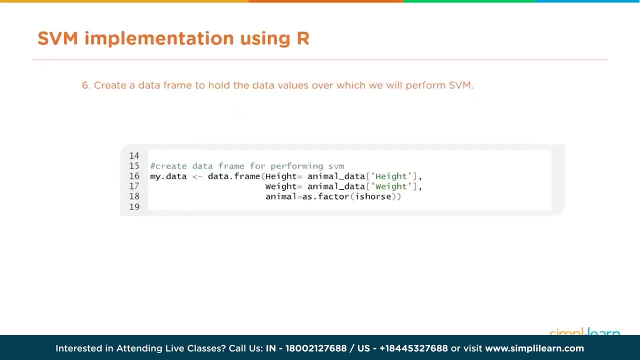 call the library up into the our session that you're working. we'll create the data frame from the data that was ingested. we will then view the data frame and, of course, we have to explore the data frame, hoping that we don't have missing values or we don't have outliers. if we do have missing values or outliers, 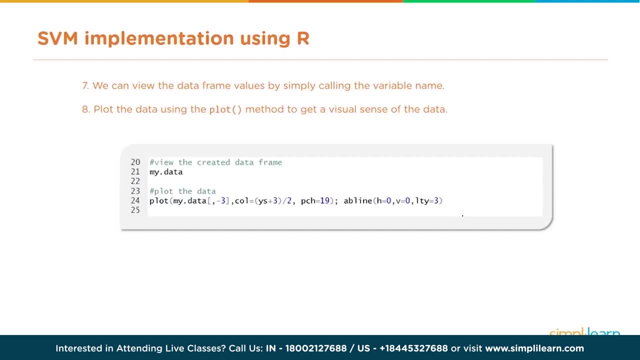 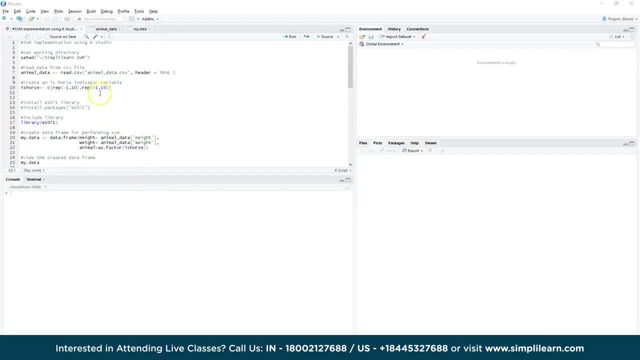 we'll have to either impute those values or delete those values, but in this case let's hope we don't have any. and now for a quick demo on support vector machines. so we have a working directory where my data is stored and I'm going to set the working directory to that data source and read the data. 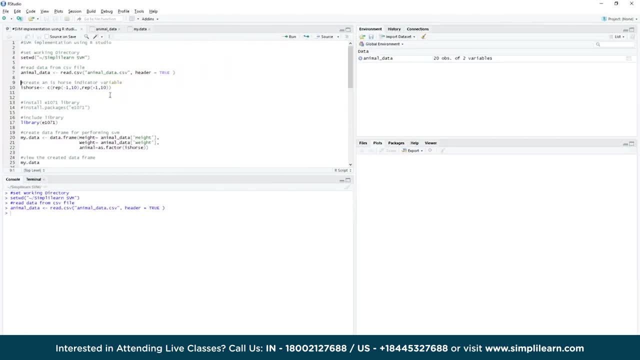 file into R, and now I'm going to create a vector that really is just an indicator variable. it's the negative ones and the ones that indicate whether it's a mule or a horse- negative one for a mule, positive one for a horse. so I'll 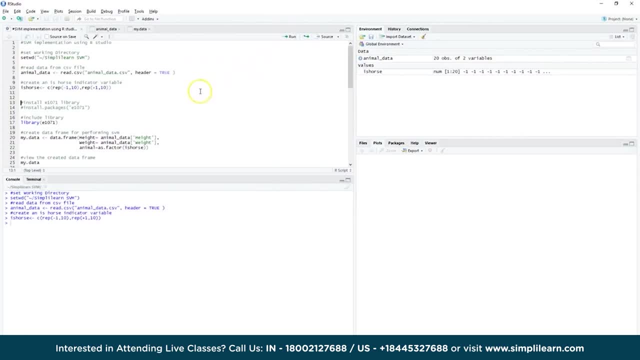 create that vector and SVM. there's a great package, e1071, great library that has the support vector, machine functions that we're going to use. and now I'm going to create the data frame. I'm going to take my data and I'm going to add to. 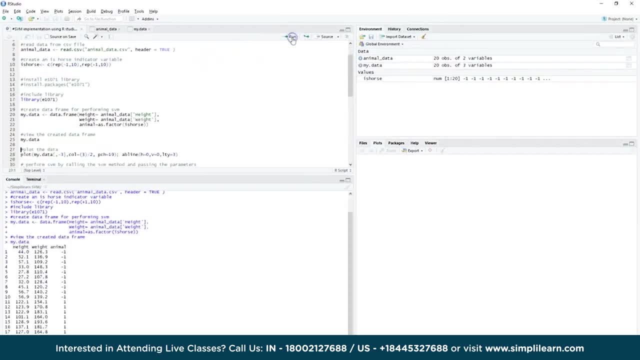 it, the is horse vector. and now let's just take a peek and, as you can see, there's the height, weight and whether or not the animal was a mule or a horse. so remember machine learning, we take a data source with known outcomes and we apply. 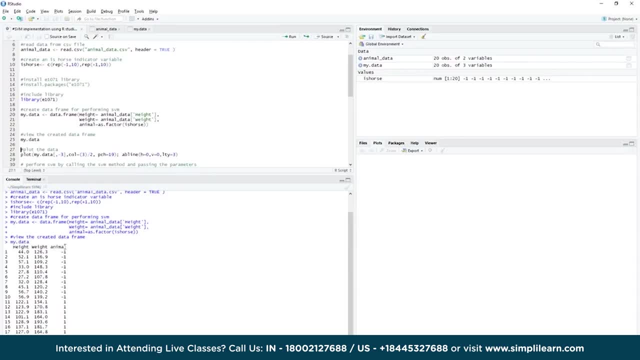 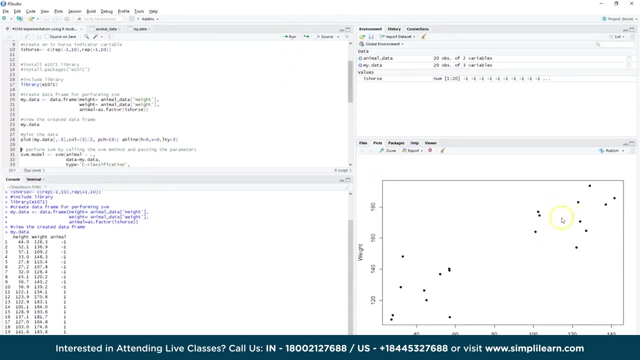 the algorithm to that data source, in this case a data frame of heights, weights and the indicator variable, and then we use the machine learning algorithm to learn from that data with those known results. so now let's plot the data, the height versus weight- and as you can see, the horses tend to be a lot taller. and 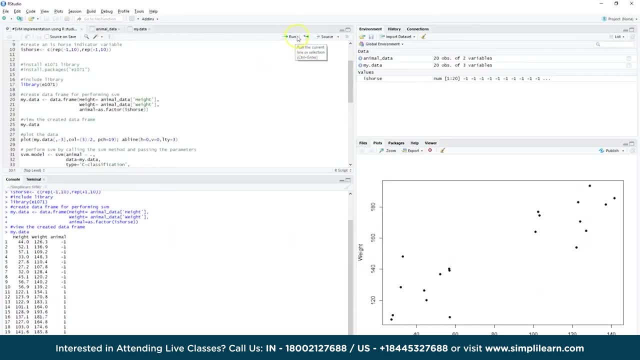 weigh a lot more than the mules. so now let's run our algorithm, our SVM model, against the data, and the key here is to run the algorithm against the data, and the key here is to run the algorithm against the data, and the key here is to. 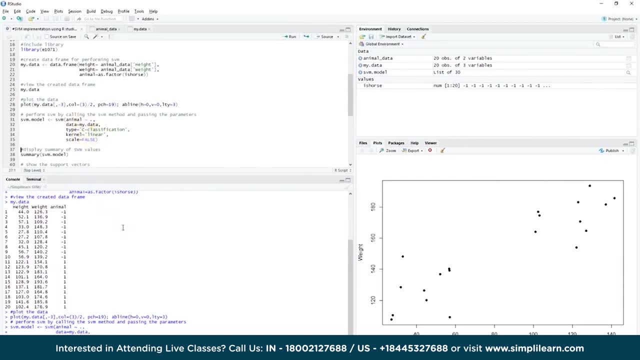 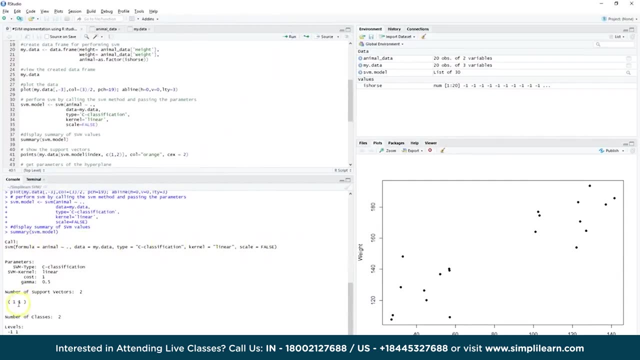 personas, two ofosium functions on the left, and the key here is, of course, was mean human procedure, and the interesting about this is that it's a linear model and we've run it and great, now we have a model. let's look at the summary of the. 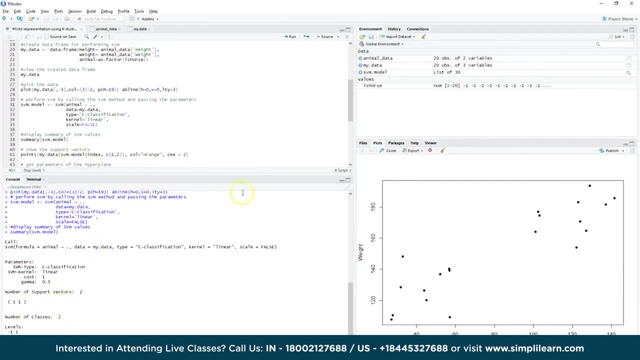 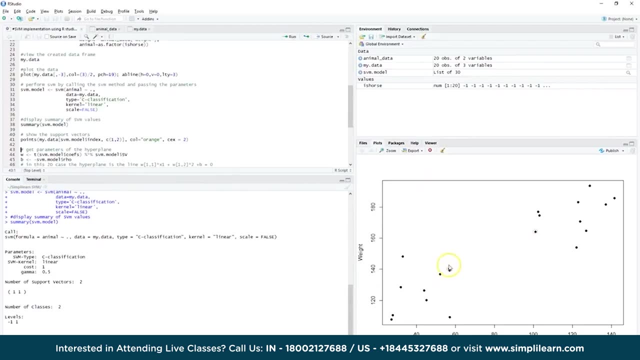 model and, as you can see, there's the formula that Iran and some of the information about the vectors and the classes, and there are two support vectors. so now let's find those two support vectors. on our graph and this might be a little hard to see- the orange outline around this point and this point. 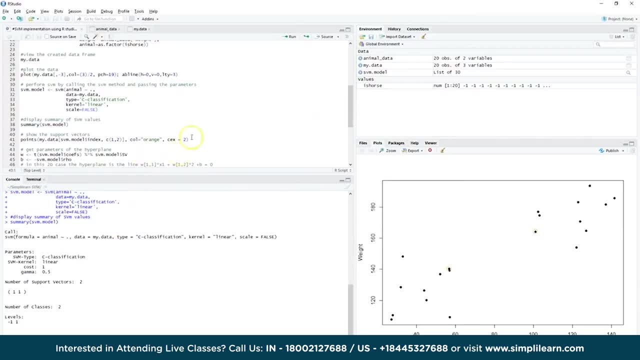 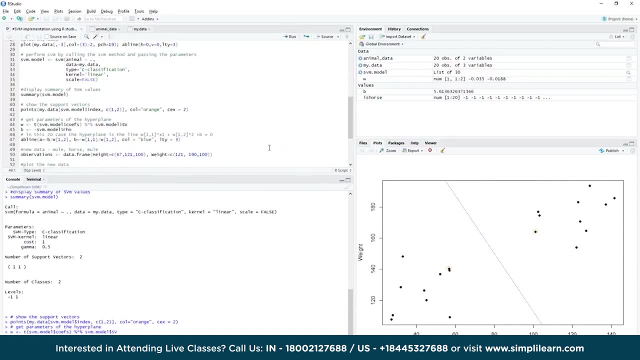 and thus we call them the support vectors. Now let's get the parameters of the hyperplane from the model and let's plot a line that will be our hyperplane. There's our hyperplane line, and therefore to the left and below are mules and to the right and above are horses. above that line, 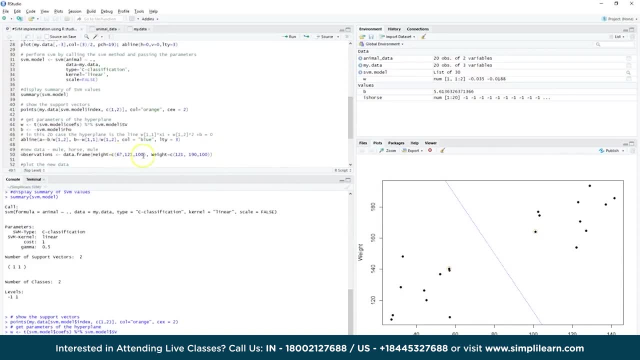 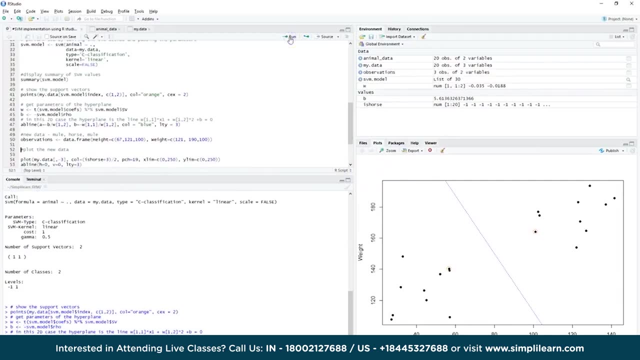 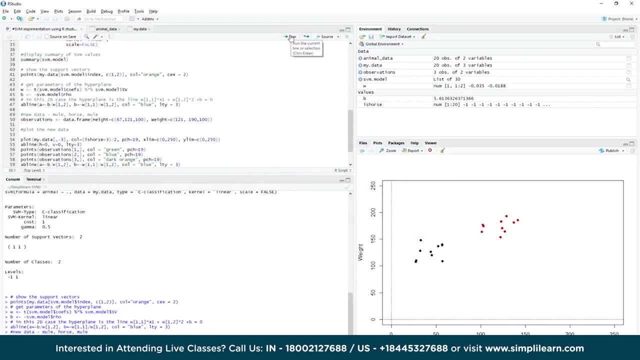 Let's take a few new observations, and I've encoded these so that it would be illustrative. We'll take these new observations and we'll plot them, and I'm going to generate a new plot, Red being the horses, black dots being the mules. I'll create an x and y axis. I'm going to plot three dots and you. 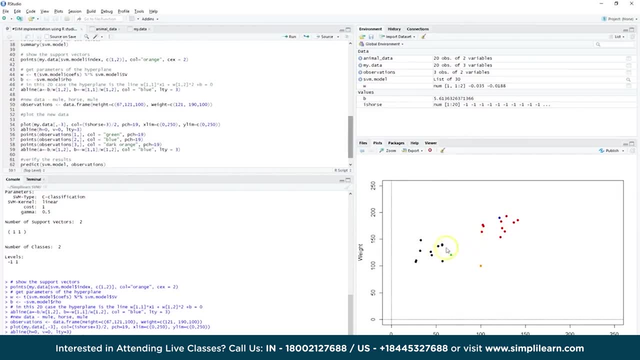 can see one of them: the green dot. the first one kind of falls near the mules, The blue one kind of falls near the horses and visually we might conclude, hey, one's a mule, one's a horse. But what about the orange dot? Well, for the orange dot we really need our hyperplane, We really need something. 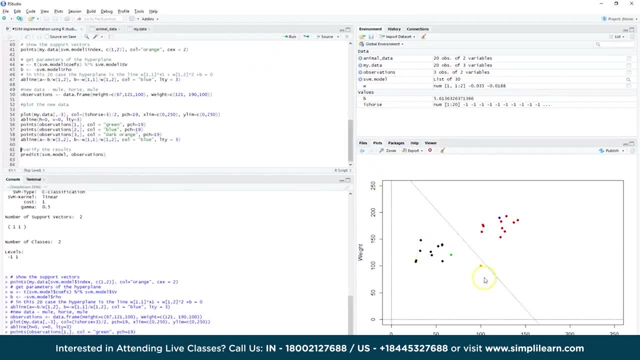 to do with the hyperplane. We really need something to do with the hyperplane. We really need something to clearly indicate which side it's on. and, of course, by looking at this data visualization you can tell that the orange dot is probably a mule. and let's verify those results by sticking those 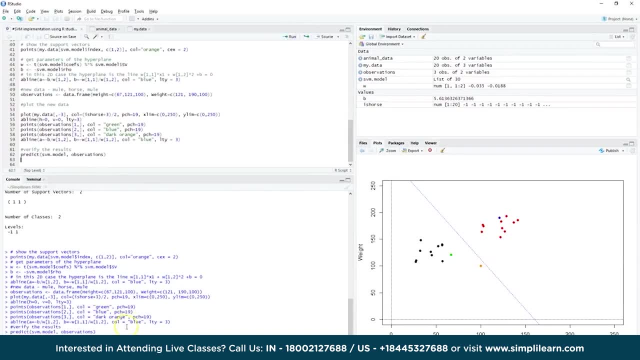 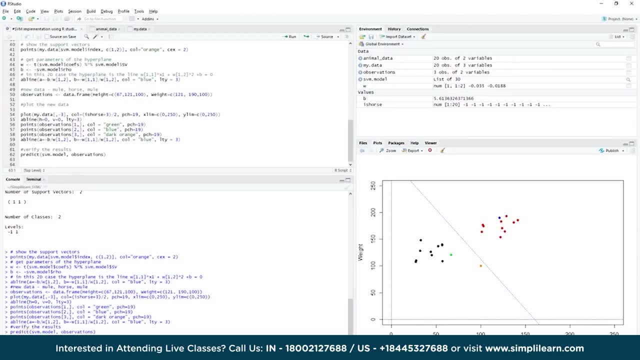 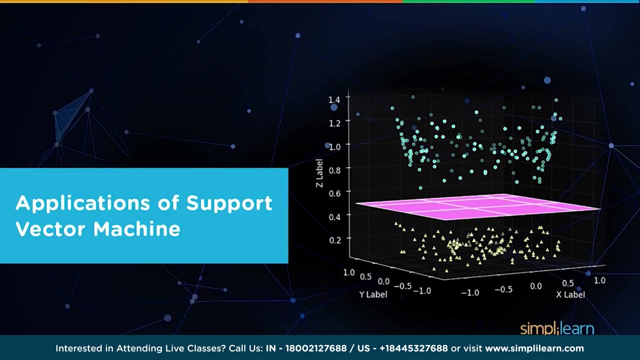 clearly the SVM model correctly predicted that that third point would be a negative one would be a mule, and we can visually see that by the hyperplane on the graph. So that's a quick example of SVM In general. support vector machines are binary classifiers. We don't use them for higher level. 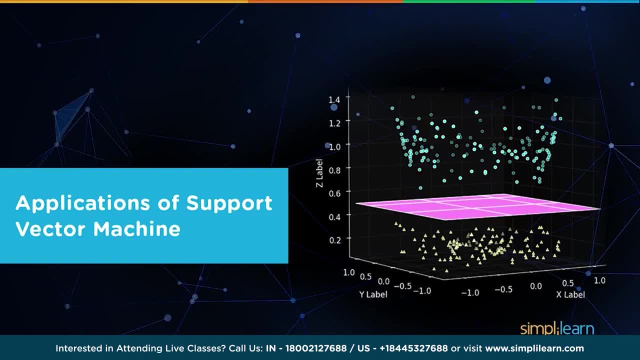 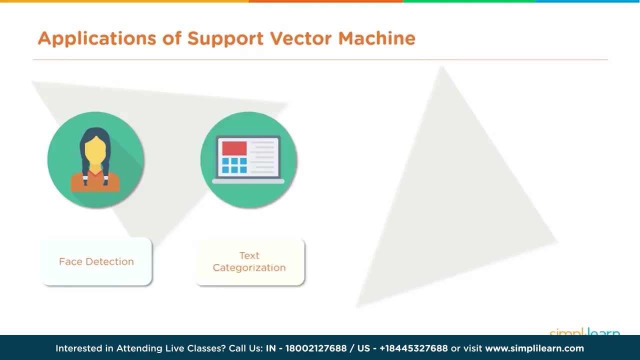 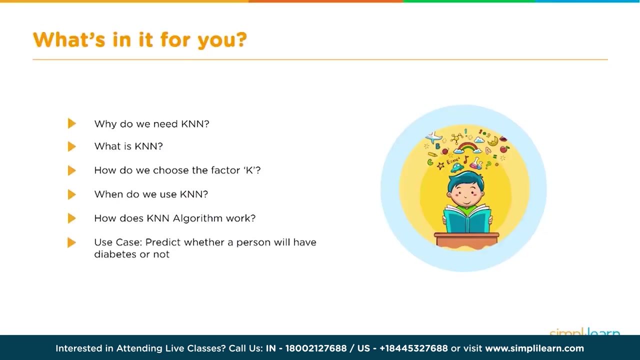 classification. If you had three or more classes, you might want to use something like random forest. What applications You can use it for: face detection, text categorization, image classification and bioinformatics- Really anywhere that you have the need to classify things into two groups. Today we're going to cover the K nearest neighbors, a lot referred to as KNN And KNN. 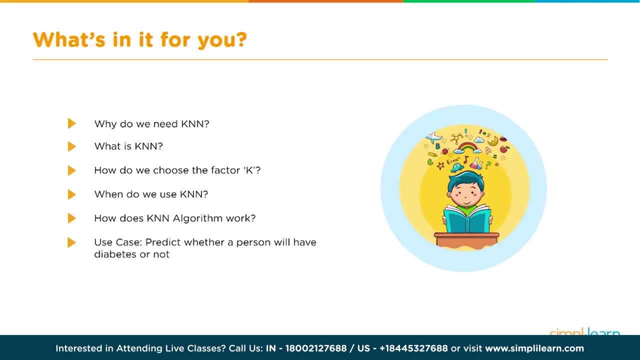 is really a fundamental place to start in the machine learning. It's a basis of a lot of other things, and just the logic behind it is easy to understand and incorporated in other forms of machine learning. So, today, what's in it for you? Why do we need KNN? What is it that you need to? 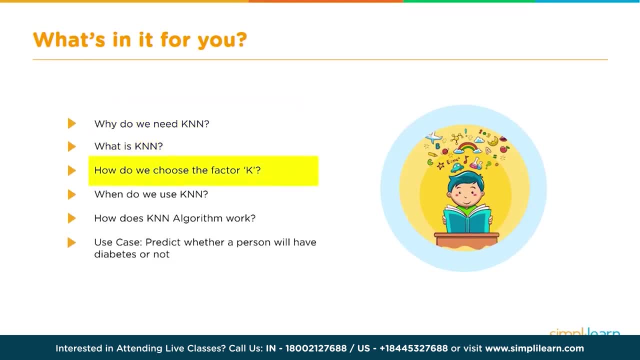 use. Why is KNN? How do we choose the factor K? When do we use KNN? How does KNN algorithm work? And then we'll dive in to my favorite part: the use case Predict whether a person will have diabetes or not. 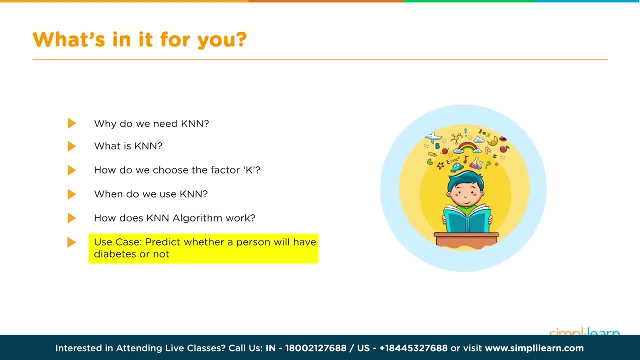 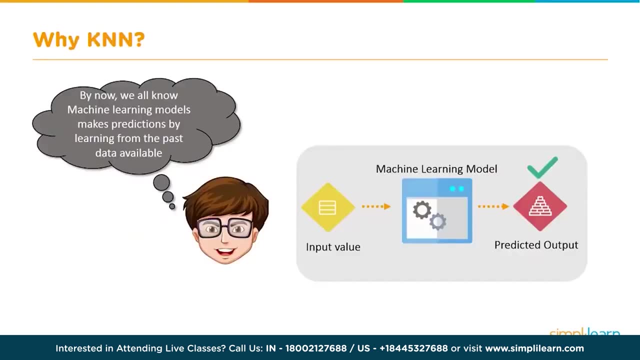 That is a very common and popular used data set. as far as testing out models and learning how to use the different models in machine learning, By now we all know machine learning models make predictions by learning from the past data, Which is good for all the applications available for training purposes. 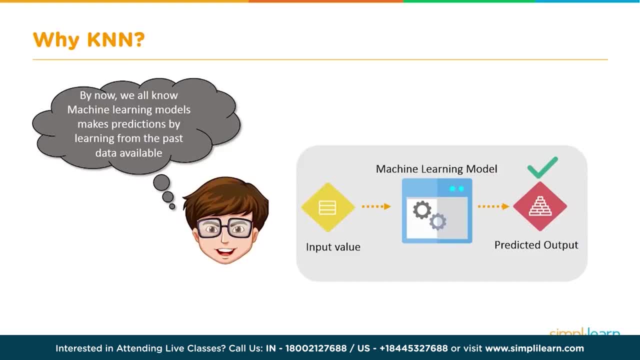 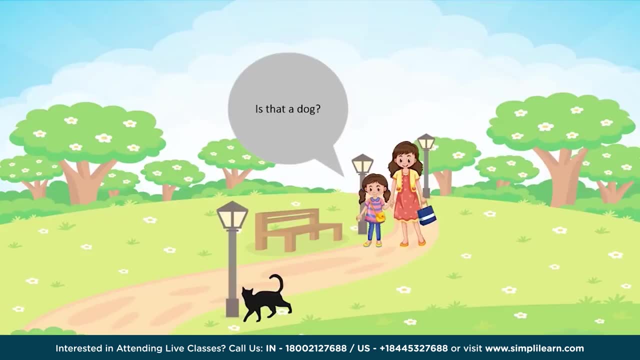 So we have our input values. our machine learning model builds on those inputs of what we already know, And then we use that to create a predicted output. Is that a dog, A little kid looking over there watching a black cat cross their path? 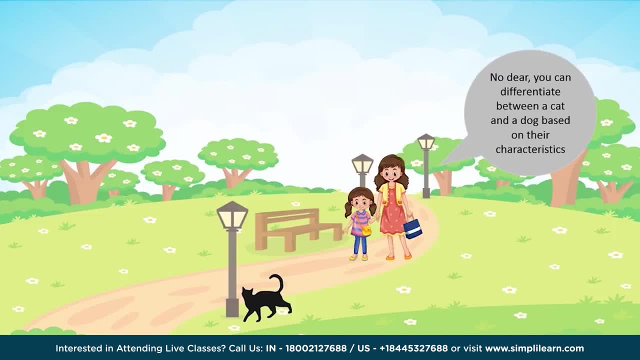 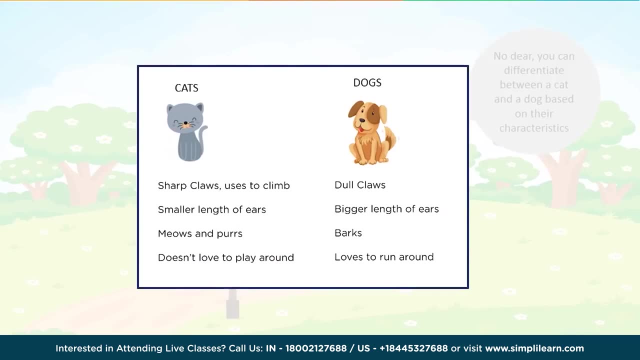 No dear, You can differentiate between a cat and a dog based on their characteristics. Cats- Cats have sharp claws, uses to climb, Smaller length of ears, Meows and purrs. Doesn't love to play. They have dull claws, bigger length of ears, barks and loves to run around. 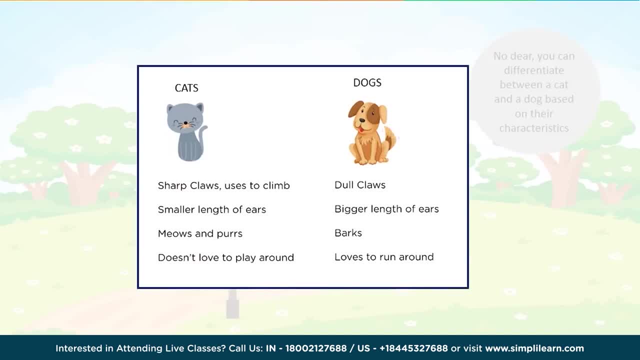 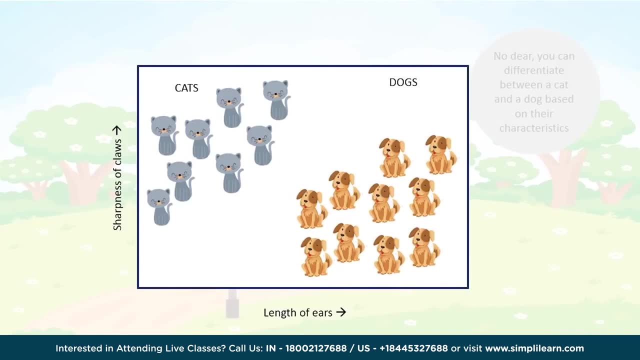 You usually don't see a cat running around people- although I do have a cat that does that- where dogs do. We can look at these and say we can evaluate the sharpness of the claws- how sharp are their claws? and we can evaluate the length of the ears and we can usually sort out cats. 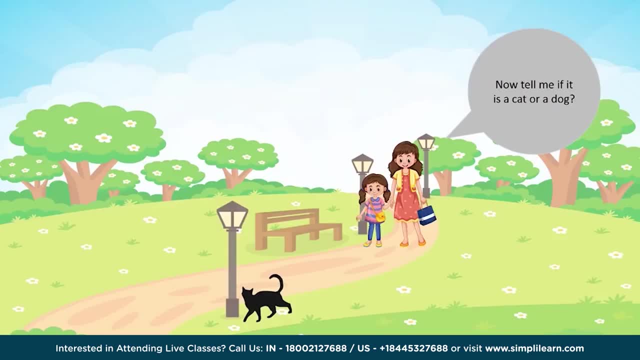 from dogs based on even those two characteristics. Now tell me if it is a cat or a dog. An odd question. usually little kids know cats and dogs by now, Unless they live in a place where there's not many cats or dogs. So if we look at the sharpness of the claws, the length of the ears, and we can see that. 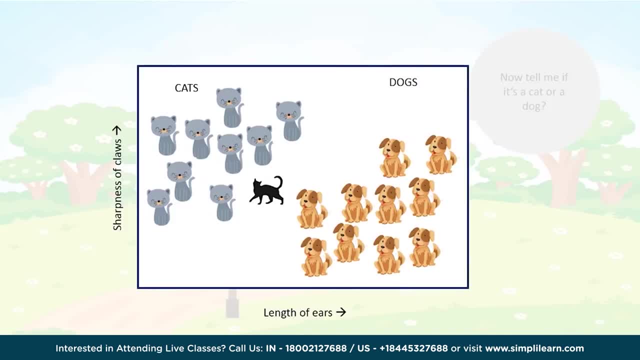 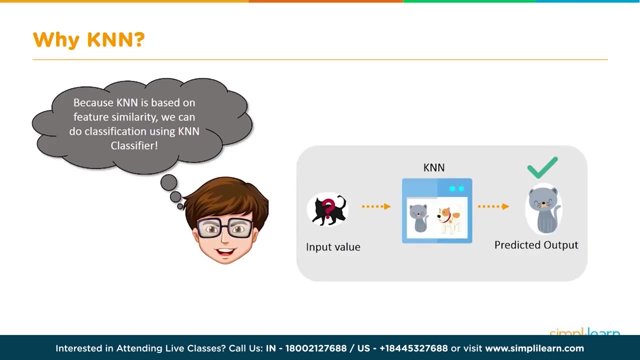 the cat has smaller ears and sharper claws than the other animals. Its features are more like cats. it must be a cat- Sharp claws, length of ears- and it goes in the cat group. Because KNN is based on feature similarity, we can do classification using KNN classifier. 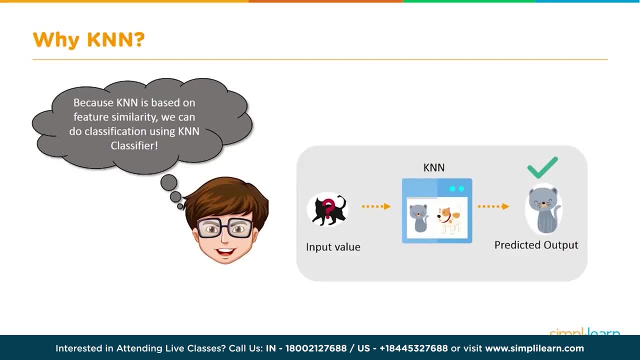 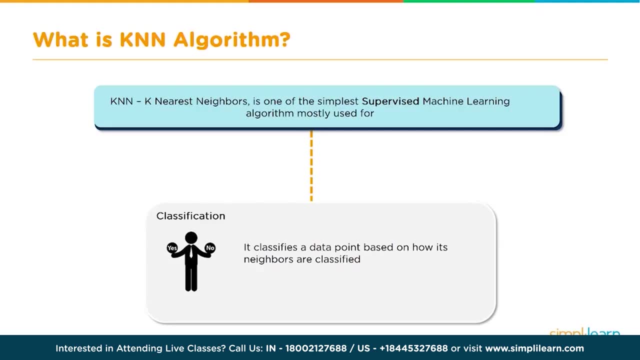 So we have our input value, the picture of the black cat. It goes into our trained model And it predicts that this is a cat coming out. So what is KNN? What is the KNN algorithm? K nearest neighbors is what that stands for. 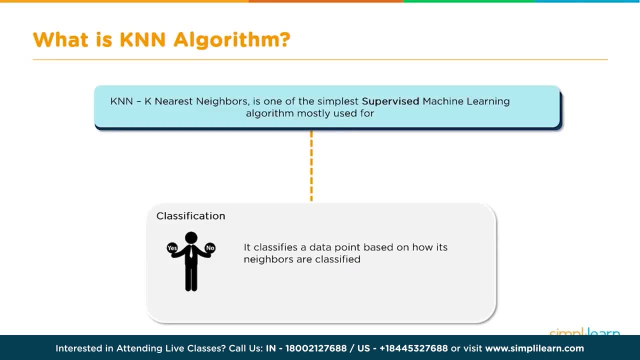 It's one of the simplest supervised machine learning algorithms mostly used for classification. So we want to know: is this a dog or it's not a dog? Is it a cat or not a cat? It classifies a data point based on how its neighbors are classified. 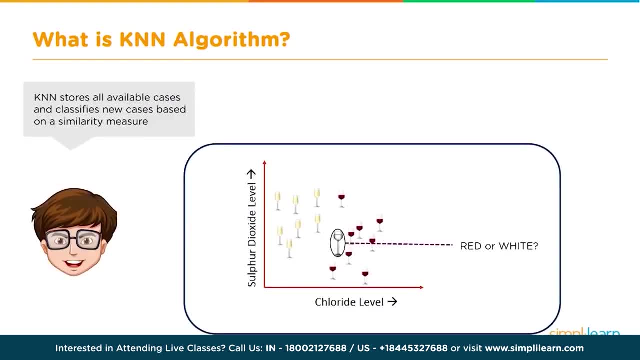 KNN stores all available cases and classifies new cases based on a similar data point. So we can do classification using KNN classifier. So we want to know: is this a dog or it's not a dog? Is it a cat or not a cat? 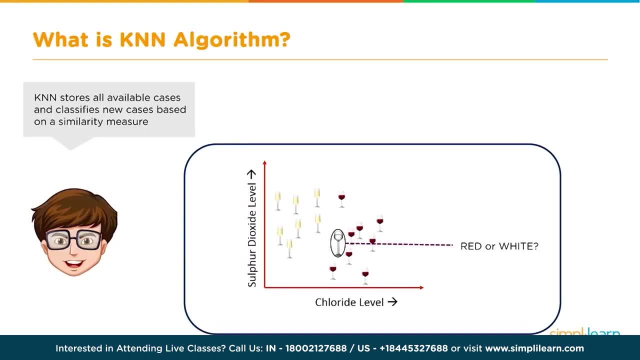 It classifies all available cases and classifies new cases based on a similarity measure. And here we've gone from cats and dogs right into wine. another favorite of mine, KNN stores all available cases and classifies new cases based on a similarity measure. 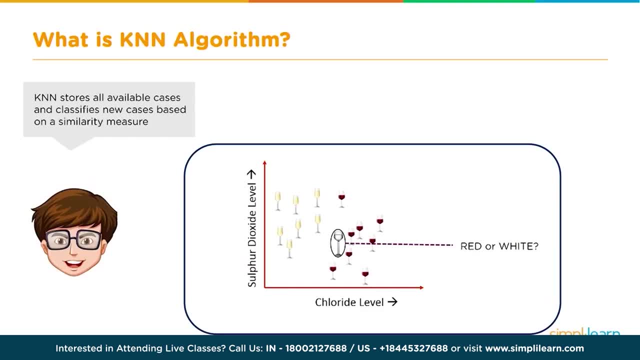 And here you see, we have a measurement of sulfur dioxide versus the chloride level And then the different wines they've tested and where they fall on that graph, based on how much sulfur dioxide and how much chloride. K in KNN is a perimeter that refers to the number of nearest neighbors to include in. 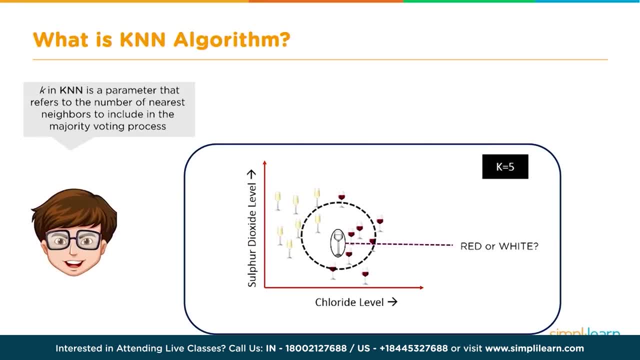 the majority of the voting process, And so if we add a new glass of wine there- red or white- we want to know what the neighbors are. In this case, we're going to put k equals 5.. We'll talk about k in just a minute. 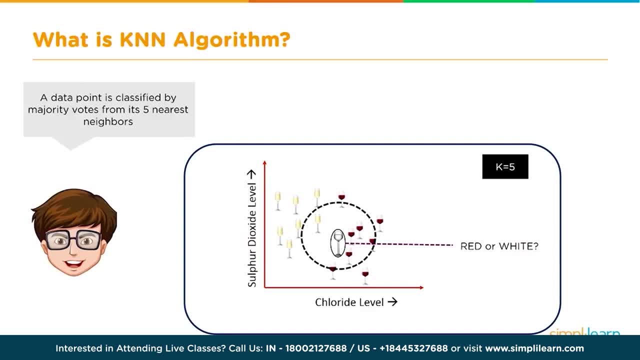 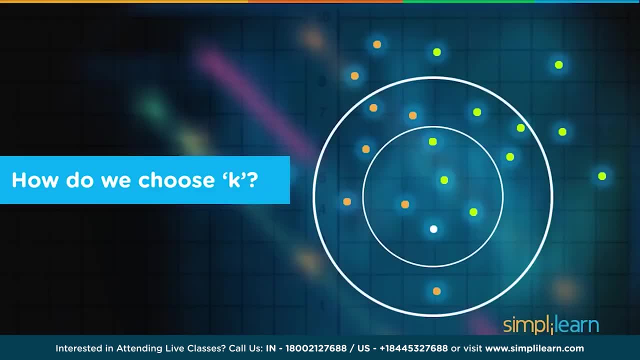 A data point is classified by the majority of votes from its five nearest neighbors. Here, the unknown point would be classified as red, since four out of five neighbors are red. So how do we choose k? How do we know k equals 5?? 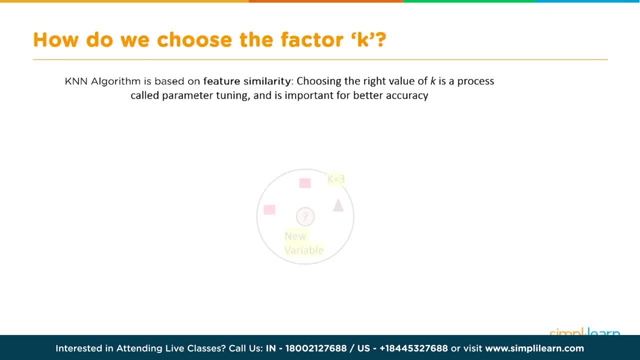 I mean, that was the value we put in there, so we're going to talk about it. How do we choose the factor k? KNN algorithm is based on feature similarity. Choosing the right value of k is a process called parameter tuning and is important for better accuracy. 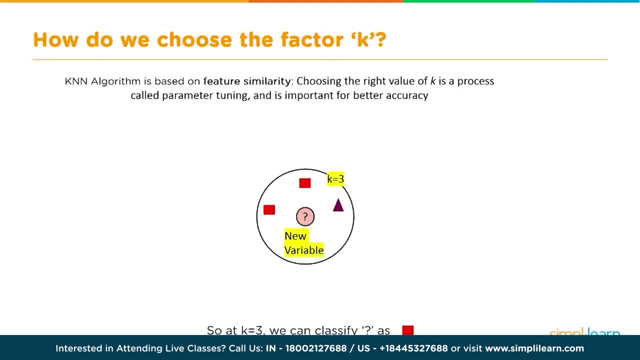 So, at k equals 3, we can classify- we have a question mark in the middle- as either a square or not. Is it a square or is it, in this case, a triangle? And so if we set k equals to 3, we're. 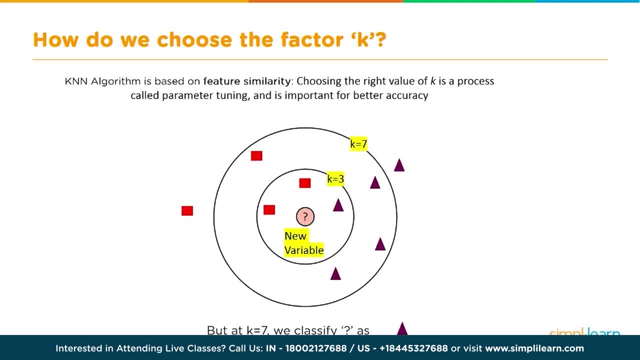 going to look at the three nearest neighbors. We're going to say this is a square And if we put k equals to 7, we classify as a triangle depending on what the other data is around it, And you can see as the k changes. 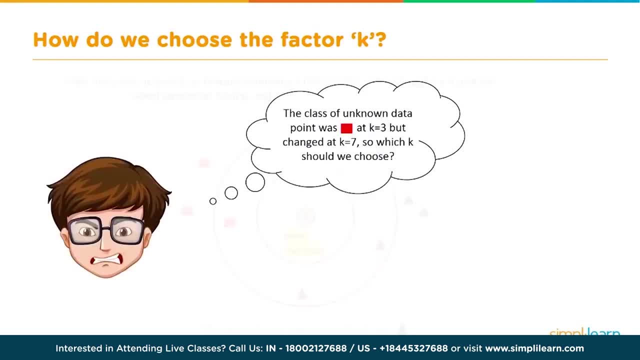 depending on where that point is. that drastically changes your answer. And we jump here and we go. how do we choose the factor of k? You'll find this in all machine learning: Choosing these factors, that's the face you get. 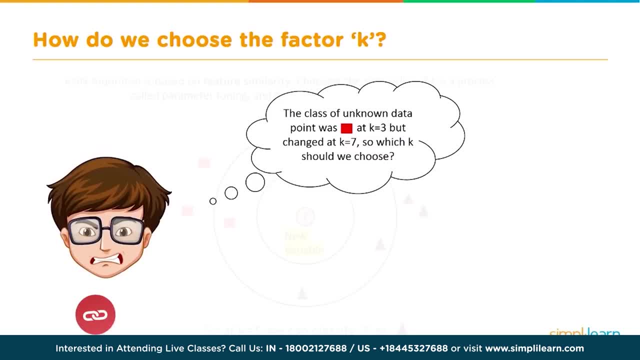 It's like, oh my gosh, did I choose the right k? Did I set it right- my values- in whatever machine learning tool you're looking at, so that you don't have a huge bias in one direction or the other? 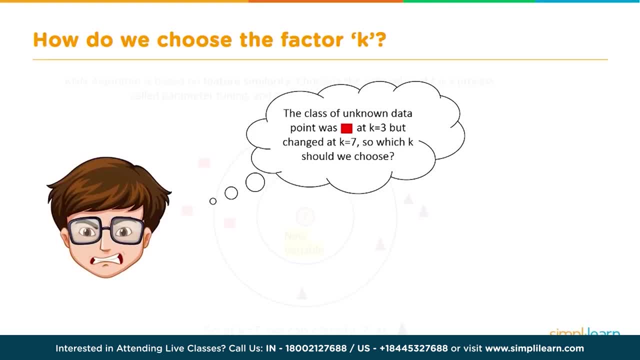 And in terms of KNN, the number of k, if you choose it too low the bias is based on, it's just too noisy, It's right next to a couple of things and it's going to pick those things and you might get a skewed answer. 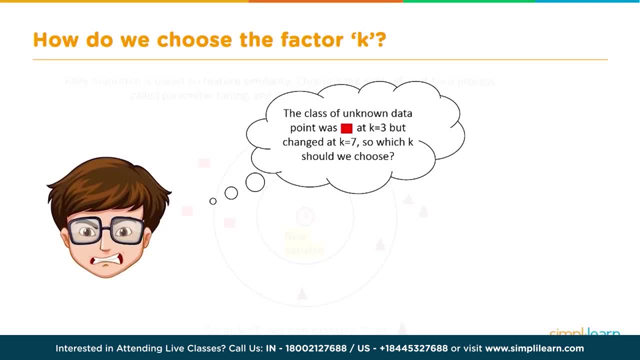 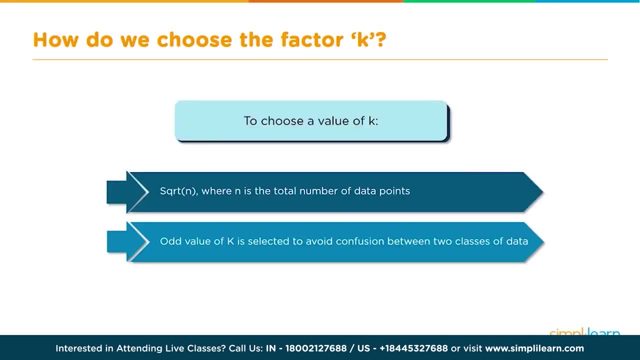 And if your k is too big then it's going to take forever to process, So you're going to run into processing issues and resource issues. So what we do, the most common use- and there's other options for choosing k- is to use the square root of n. 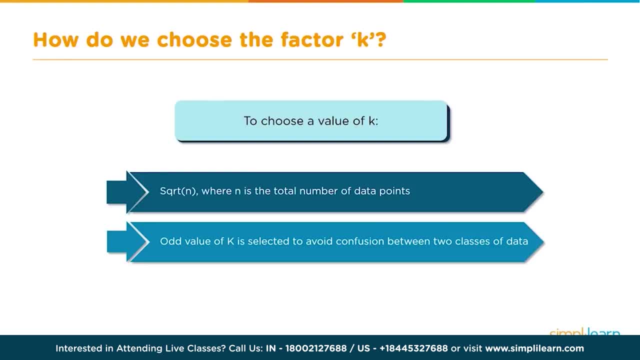 So n is a total number of values you have and you take the square root of it. In most cases you also if it's an even number. so if you're using, like in this case, squares and triangles, if it's even, you want to make your k values. 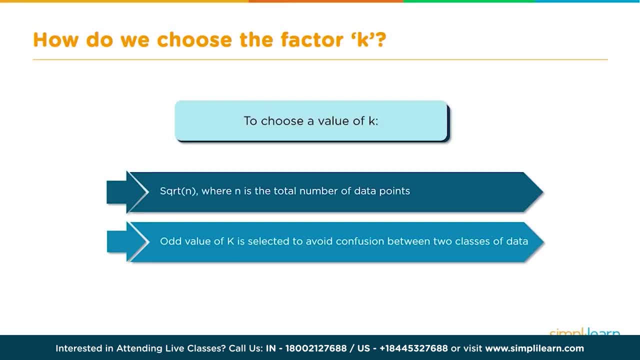 If it's even, you want to make your k value odd. That helps it select better. So, in other words, you're not going to have a balance between two different factors that are equal. So you usually take the square root of n. 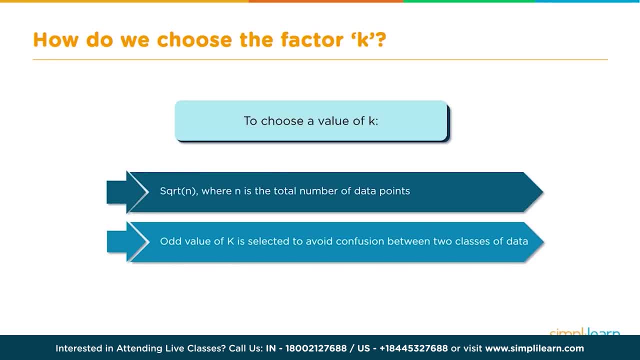 and if it's even, you add one to it or subtract one from it and that's where you get the k value from. That is the most common use and it's pretty solid. It works very well. When do we use KNN? 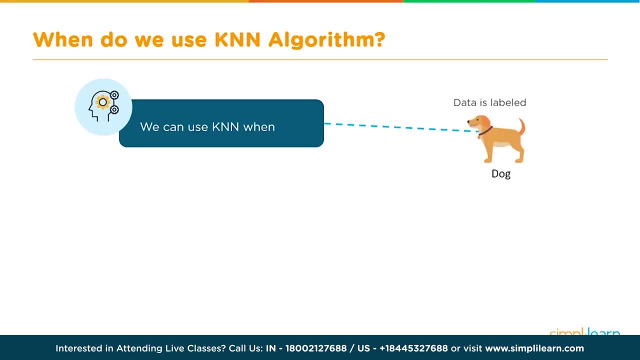 We can use KNN when data is labeled, So you need a label on it. We know we have a group of pictures with dogs, dogs, cats, cats. Data is noise-free And so you can see here. you can see. 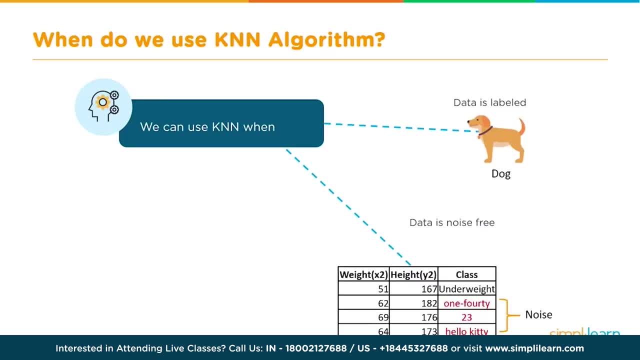 when we have a class and we have, like, underweight 140,, 23,, Hello Kitty, normal, that's pretty confusing. We have a high variety of data coming in, so it's very noisy And that would cause an issue. 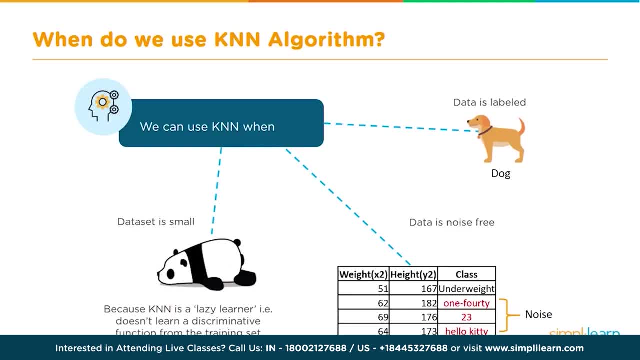 Data set is small, so we're usually working with smaller data sets where you might get into a gig of data if it's really clean, doesn't have a lot of noise, Because KNN is a lazy learner, ie it doesn't learn a discriminative function. 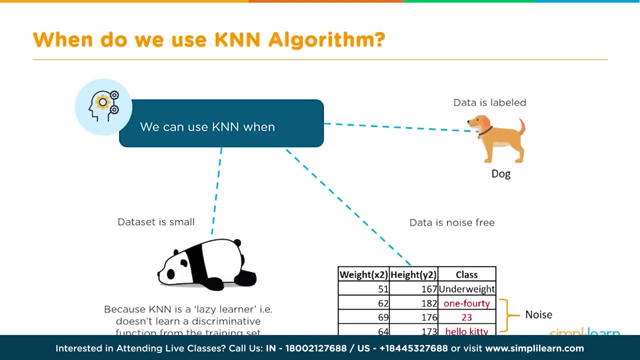 from the training set, so it's very lazy. so if you have very complicated data, a large amount of it, you're not going to use the KNN, But it's really great to get a place to start, even with large data. 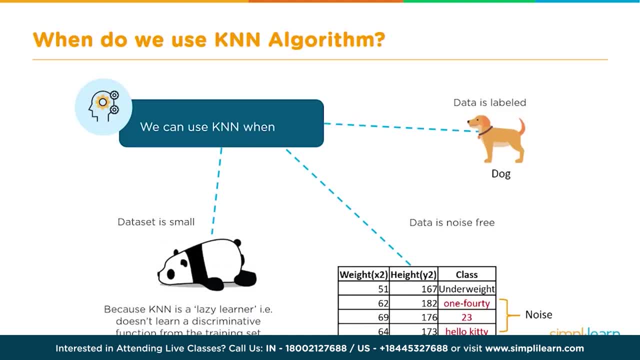 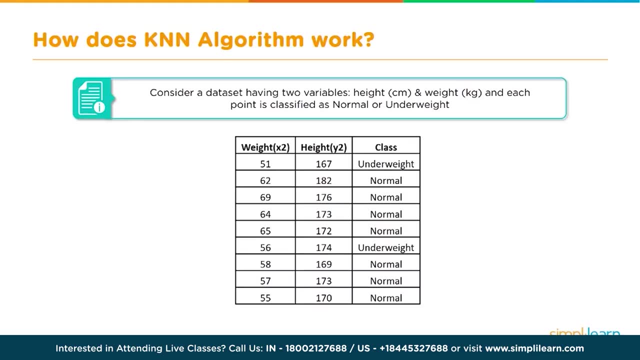 you can sort out a small sample and get an idea of what that looks like. using the KNN And also just using for smaller data sets, KNN works really good. How does a KNN algorithm work? Consider a data set having two variables. 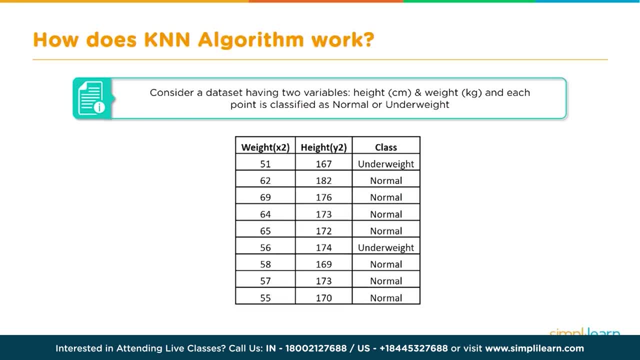 height in centimeters and weight in kilograms, And each point is classified as normal or underweight. So we see, right here we have two variables. they're not, they're underweight. On the basis of the given data, we have to classify the below set. 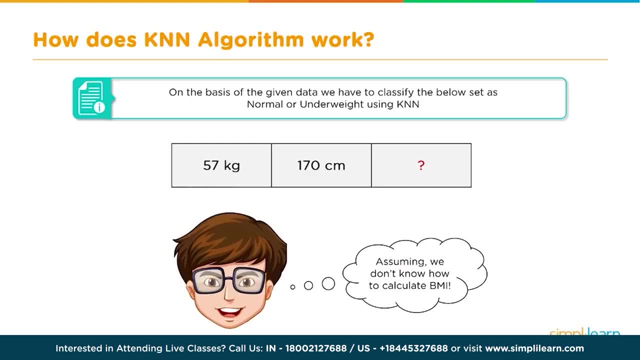 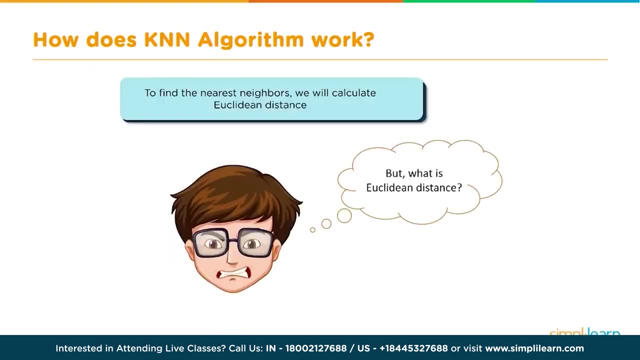 as normal or underweight using KNN. So if we have new data coming in that says 57 kilograms and 177 centimeters, is that going to be normal or underweight? To find the nearest neighbors, we'll calculate the Euclidean distance. 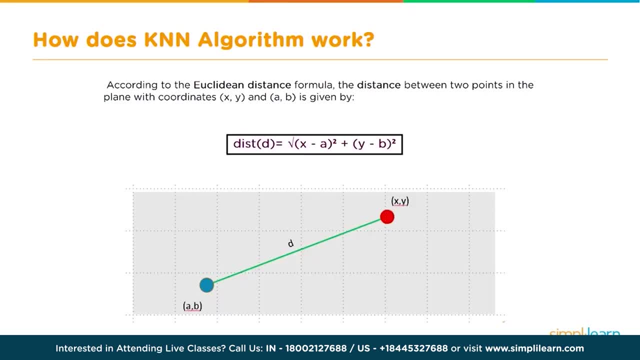 According to the Euclidean distance formula, the distance between two points in the plane with the coordinates is given by distance. D equals the square root of x minus a squared, plus y minus b squared, And you can remember that from the two edges of a triangle. 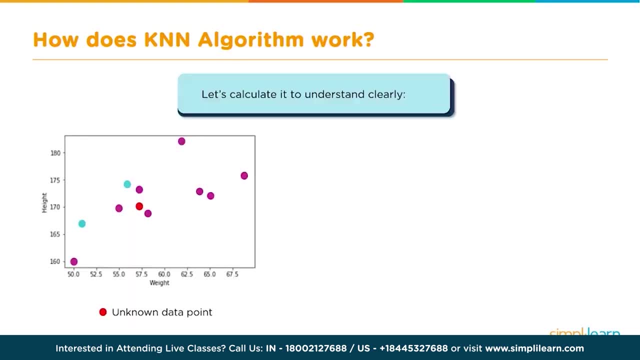 We're computing the third edge. since we know the x side and the y side, Let's calculate it to understand clearly. So we have our unknown point, We placed it there in red, And we have our other points where the data is scattered around. 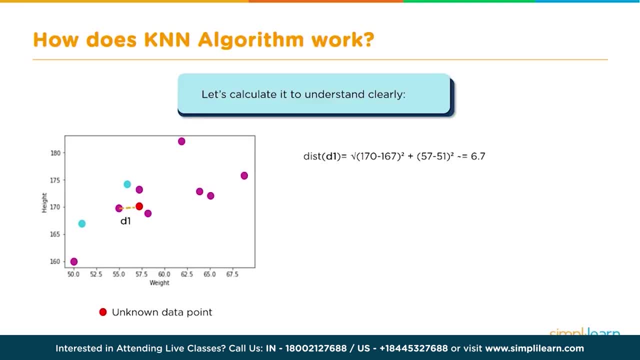 The distance D1 is the square root of 170 minus 167 squared, plus 57 minus 51 squared, and distance 2 is about 13.. And distance 3 is about 13.4.. Similarly, we will calculate the Euclidean distance of unknown. 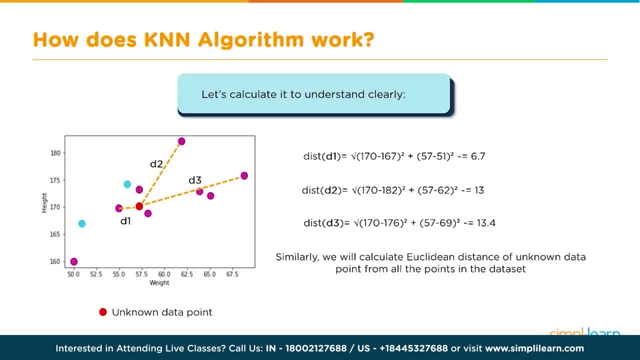 data point from all the points in the data set And because we're dealing with small amount of data, that's not that hard to do. It's actually pretty quick for a computer And it's not a really complicated math. You can just see how close is the data. 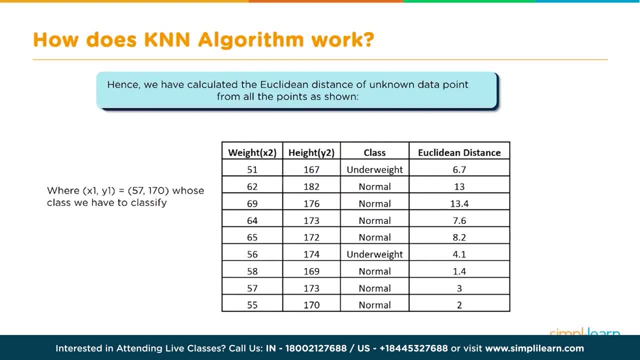 based on the Euclidean distance. Hence we have calculated the Euclidean distance of unknown data point from all the points as shown, where x1 and y1 equal 57 and 170, whose class we have to classify. So now we're looking at that and saying: 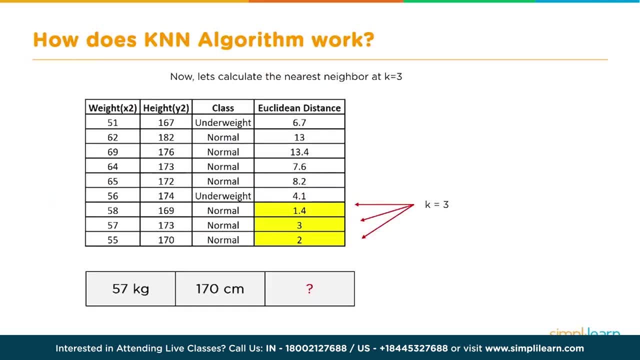 well, here's the Euclidean distance. Who's going to be the closest neighbors? Now let's calculate the nearest neighbor at k equals 3. And we can see the three closest neighbors. puts them at normal And that's pretty self-evident. 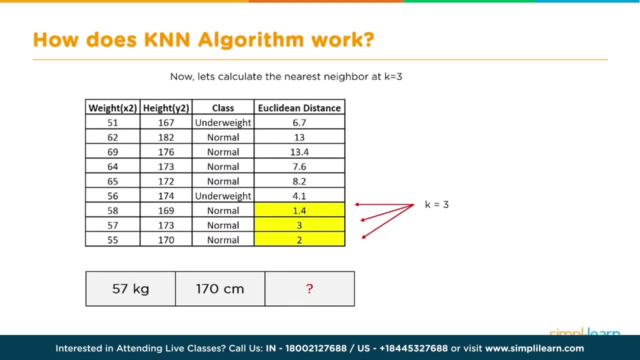 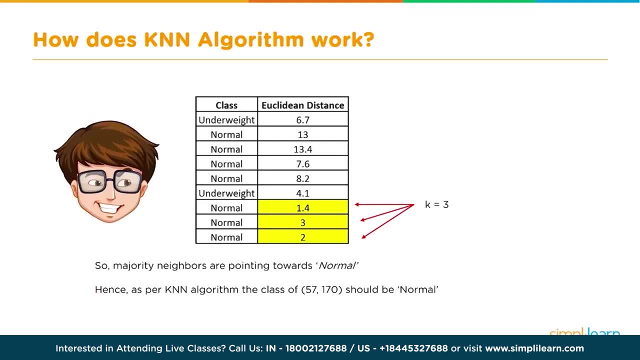 When you look at this graph, it's pretty easy to say: okay, we're just voting Normal, normal, normal. Three votes for normal Plus a 57, 170 should be normal. So a recap of KNN: Positive integer k is specified. 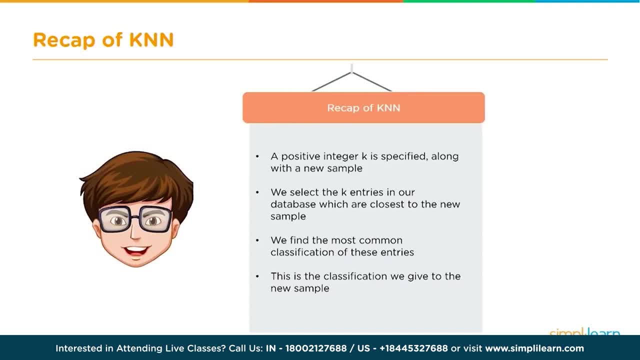 along with a new sample. We select the k entries in our database which are closest to the new sample. We find the most common classification of these entries. This is the classification we give to the new sample. So, as you can see, it's pretty straightforward. 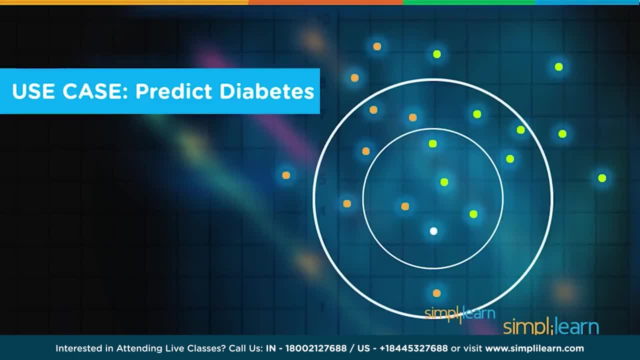 We're just looking for the closest things that match what we got. So let's take a look and see what that looks like in a use case in Python. So let's dive into the predict diabetes use case. So use case: predict diabetes. 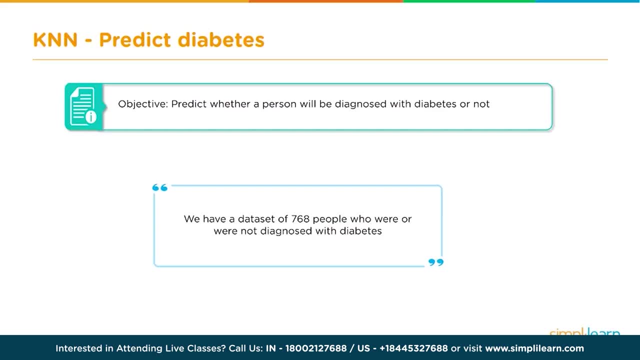 The objective: predict whether a person will be diagnosed with diabetes or not. We have a data set of 768 people who were or were not diagnosed with diabetes, And let's go ahead and open that file and just take a look at that data. 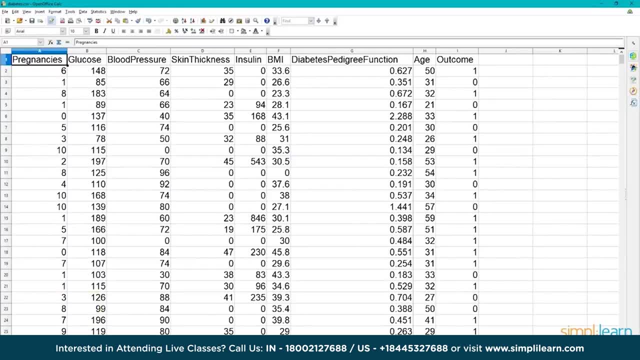 And this is in a simple spreadsheet format. The data itself is comma separated, Very common set of data And it's also a very common way to get the data And you can see here we have columns A through I, One, two, three, four, five, six, seven, eight. 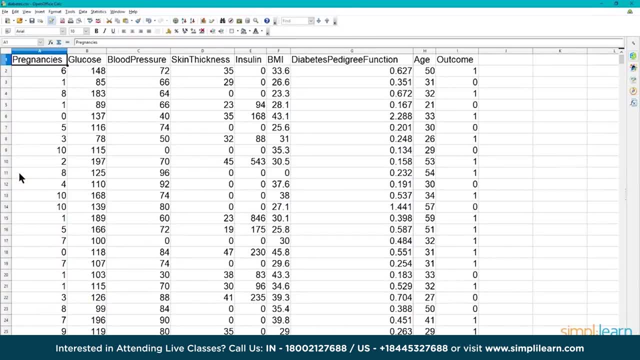 Eight columns with a particular attribute, And then the ninth column, which is the outcome, is whether they have diabetes. As a data scientist, the first thing you should be looking at is insulin. Well, you know, if someone has insulin, they have diabetes because that's why they're taking it. 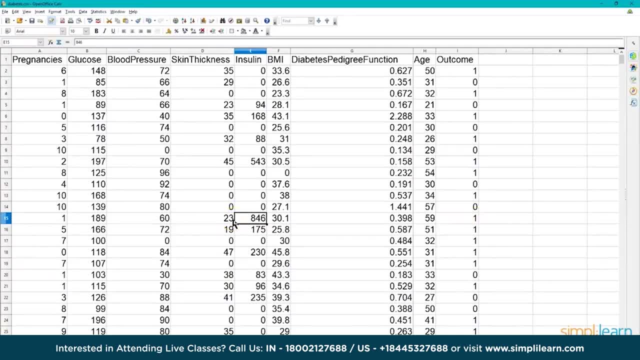 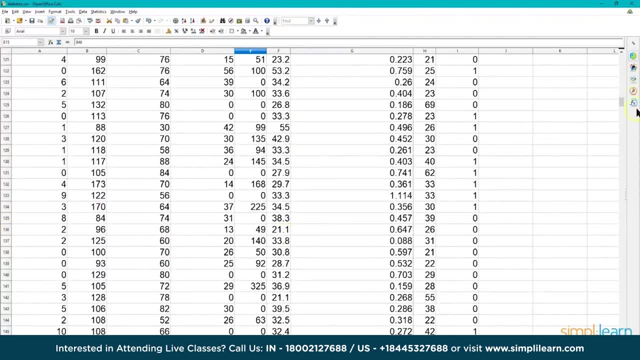 And that could cause issue in some of the machine learning packages. But for a very basic set up this works fine for doing the KNN And the next thing you notice is it didn't take very much to open it up. I can scroll down to the bottom of the data. 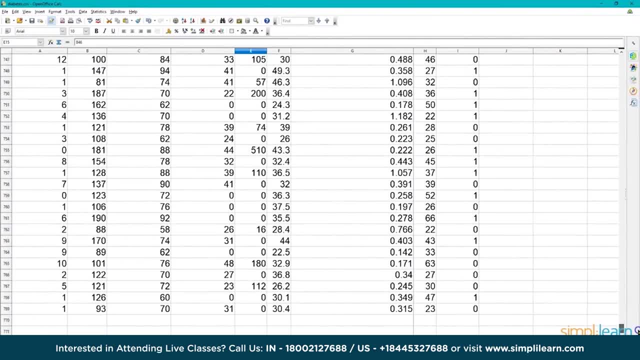 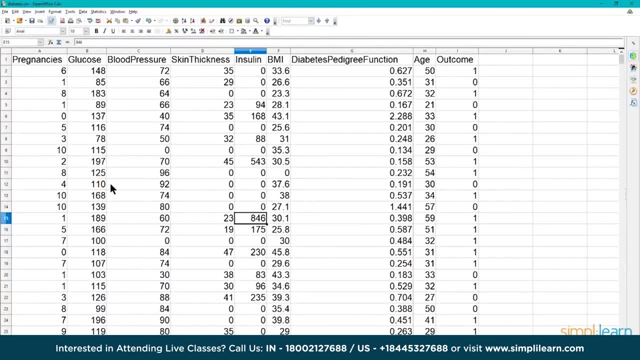 There's 768.. It's pretty much a small data set. You know, at 769 I can easily fit this into my RAM on my computer. I can look at it, I can manipulate it And it's not going to really tax, just a regular desktop. 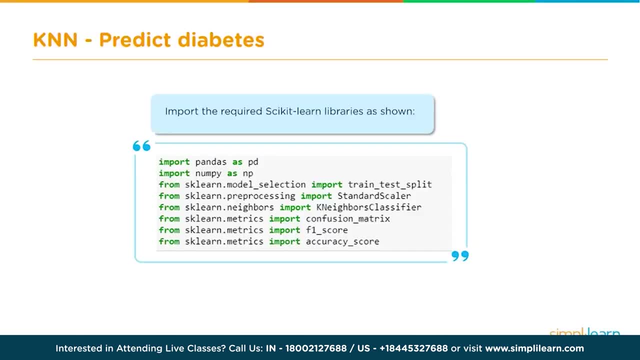 computer. You don't even need an enterprise version to run a lot of this. So let's start with importing all the tools we need, And before that, of course, we need to discuss what IDE I'm using. Certainly, you can use any particular editor for Python. 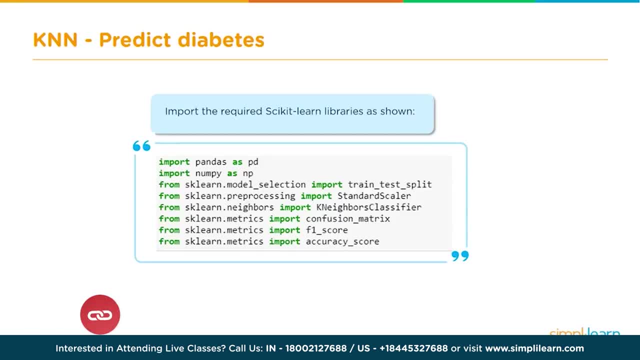 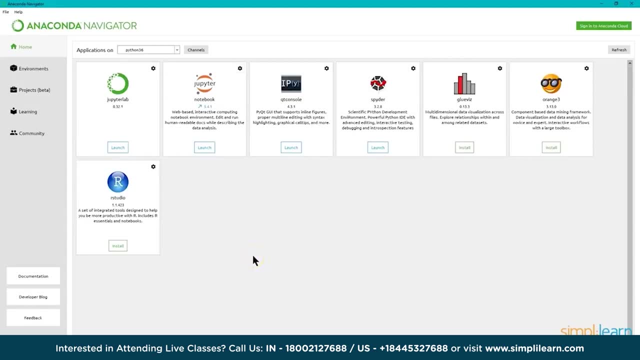 But I like to use for doing very basic visual stuff, the Anaconda, which is great for doing demos with the Jupyter Notebook, And just a quick view of the Anaconda Navigator, which is the new release out there, which is really nice You can see under home. I can choose my application. 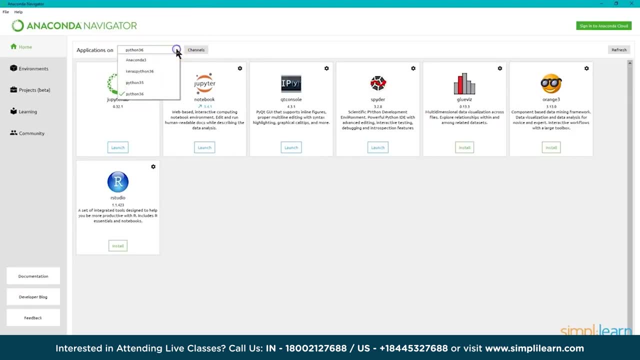 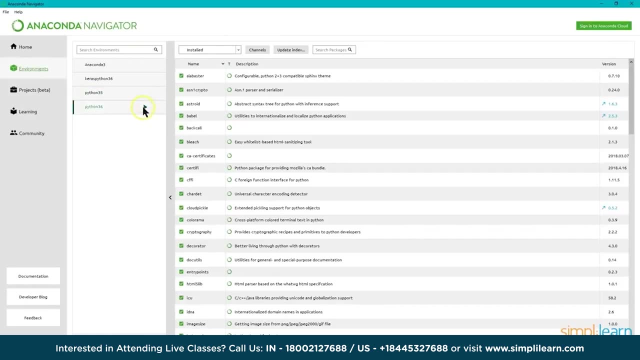 We're going to be using Python 3.6.. I have a couple different versions on this particular machine. If I go under environments, I can create a unique environment for each one, which is nice, And there's even a little button there where I can install different packages. 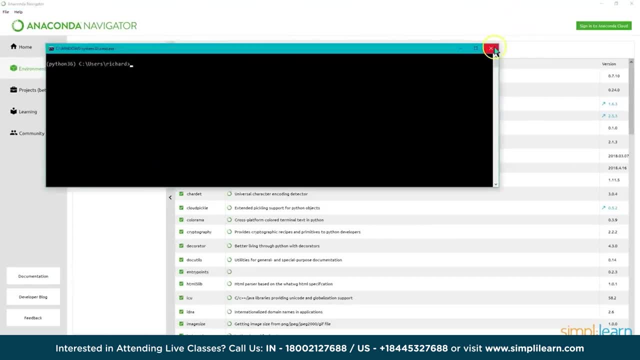 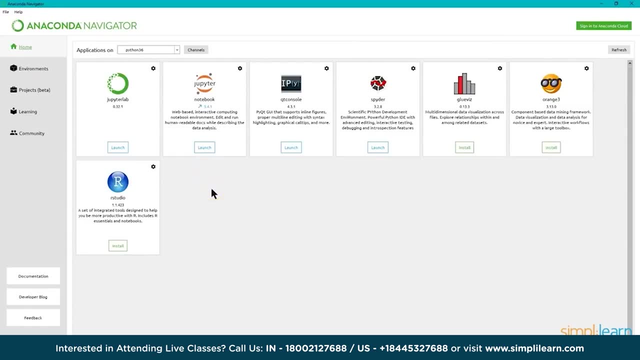 So if I click on that button and open the terminal, I'm going to have pip install to install different packages I'm working with. Let's go ahead and go back under home and we're going to launch our notebook And I've already kind of like the old cooking shows. 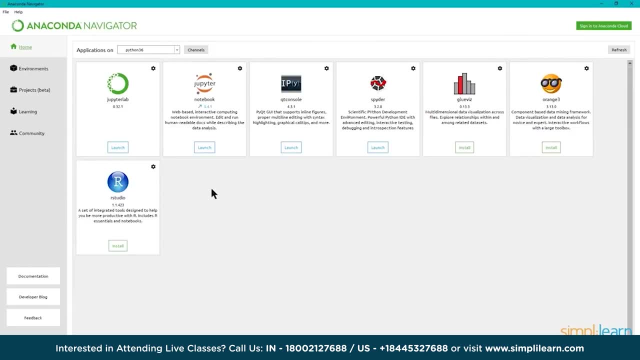 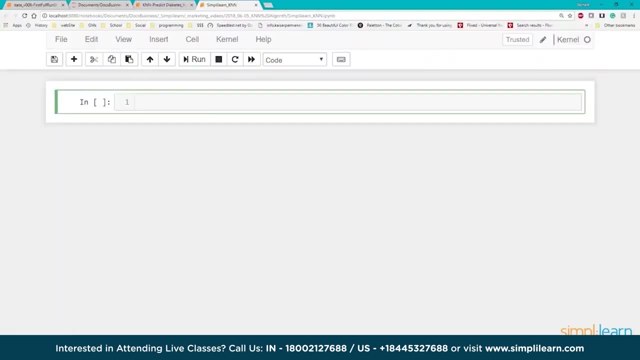 I've already prepared a lot of my stuff, so we don't have to wait for it to launch, because it takes a few minutes for it to open up a browser window. In this case, it's going to open up Chrome because that's my default that I use. 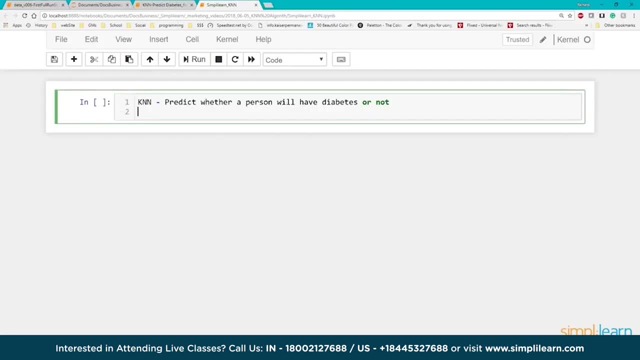 And since the script is pre-done, you'll see I have a number of windows open up at the top, The one we're working in. And since we're working on the KNN predict, let's go ahead and put that title in there, And I'm also going to go up here. 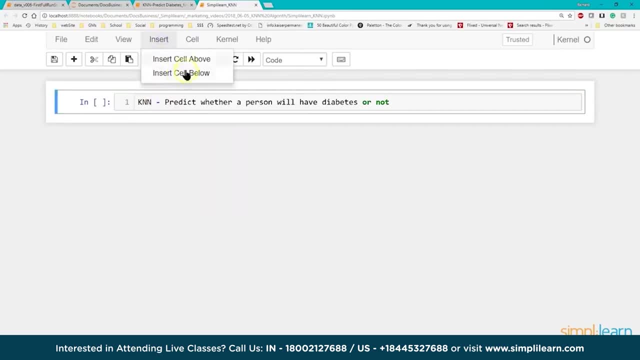 and click on cell. Actually, we want to go ahead and first insert a cell below and then I'm going to go back up to the top cell and I'm going to change the cell type to markdown. That means this is not going to run as Python. 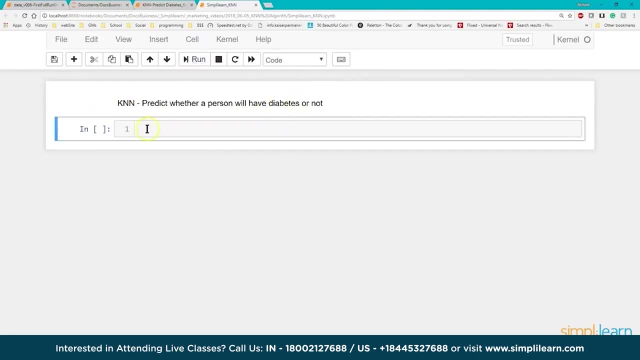 it's a markdown language, So if I run this first one it comes up in nice big letters, which is kind of nice, Reminds us what we're working on, And by now you should be familiar with doing all of our imports. We're going to import the pandas as pd. 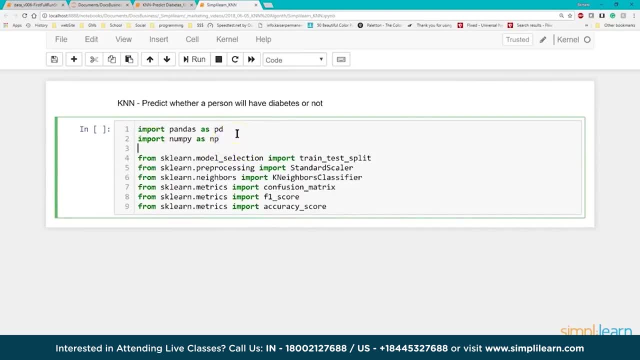 import numpy as npd. pandas is the pandas data frame and numpy is the number array- Very powerful tools to use in here. So we have our imports. So we've brought in our pandas, our numpy, our two general Python tools And then you can see over here. 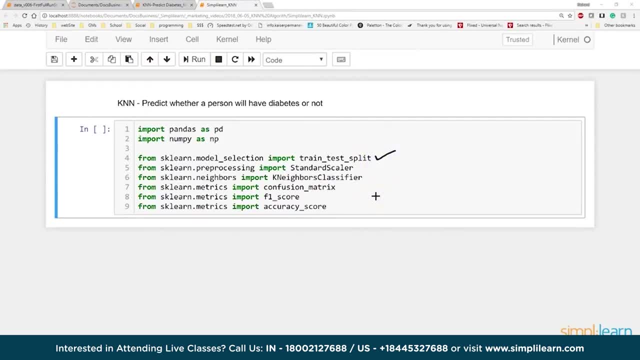 we have our train test split By now. you should be familiar with splitting the data. We want to split part of it for training our thing and then training our particular model, And then we want to go ahead and test the remaining data to see how good it is. 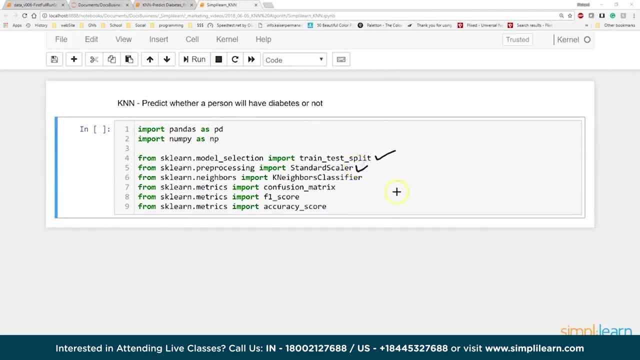 Pre-processing, a standard scalar pre-processor, so we don't have a bias of really large numbers. Remember, in the data we had, like number of pregnancies isn't going to get very large, where the amount of insulin they take can get up to 256. 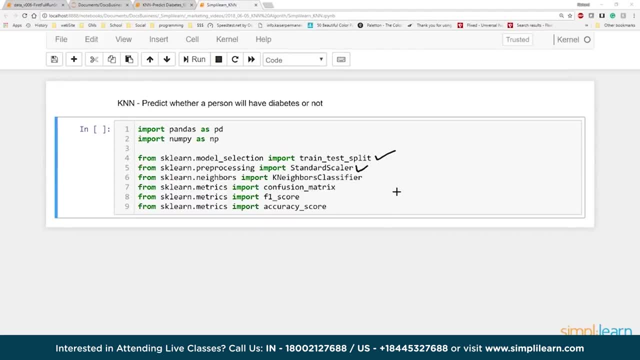 So 256 versus 6. that will skew results. So we want to go ahead and change that so that they're all uniform between minus 1 and 1.. And then the actual tool. This is the k-neighbors classifier we're going to use. 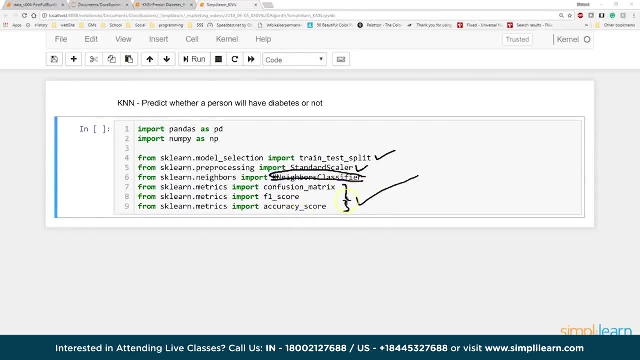 And finally, the last three are three tools to test. All about testing our model. How good is it? And we have our confusion matrix, our F1 score and our accuracy. So we have our two general Python modules we're importing, and then we have our six. 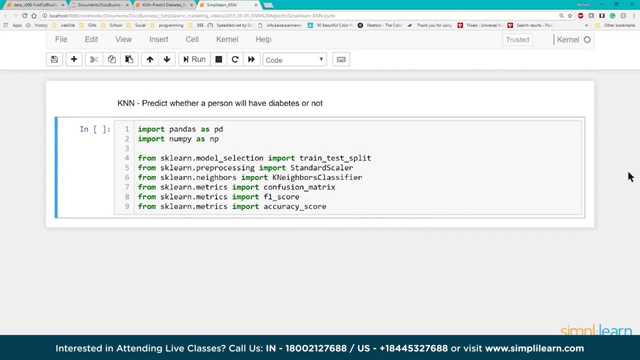 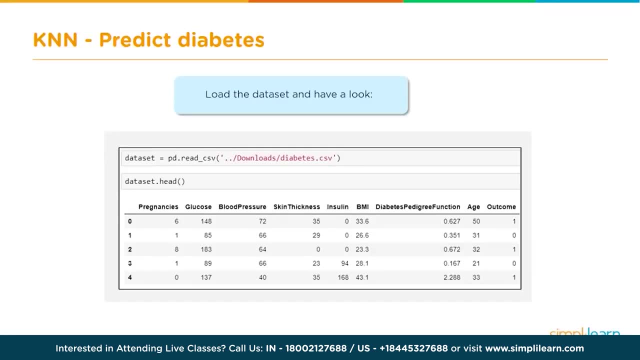 modules specific from the sklearn setup, And then we do need to go ahead and run this so that these are actually imported. There we go And then move on to the next step, And so in this set we're going to go ahead and load. 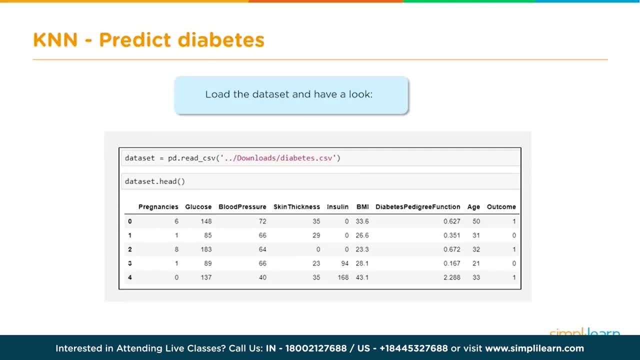 the database We're going to use: pandas. Remember pandas is pd And we'll take a look at the data in Python. We looked at it in a simple spreadsheet, But usually I like to also pull it up so that we can see what we're doing. 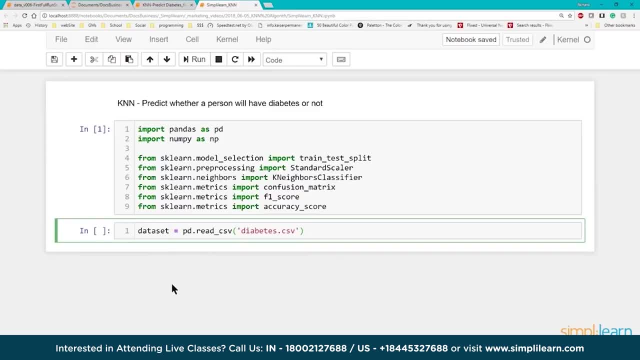 So here's our dataset: equals pdreadcsv. That's a pandas command. And the diabetes folder I just put in the same folder where my IPython script is. If you put it in a different folder you'd need the full length on there. We can also do a quick length. 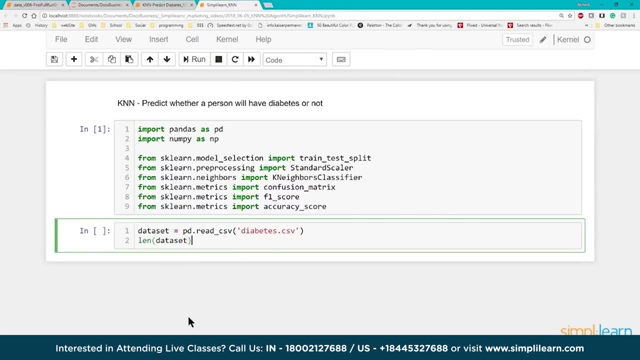 of the dataset. That is a simple Python command, len for length. Let's go ahead and print that. If you do it on its own line, we've got dataset in the Jupyter notebook. It'll automatically print it. But when you're in most of your different setups, 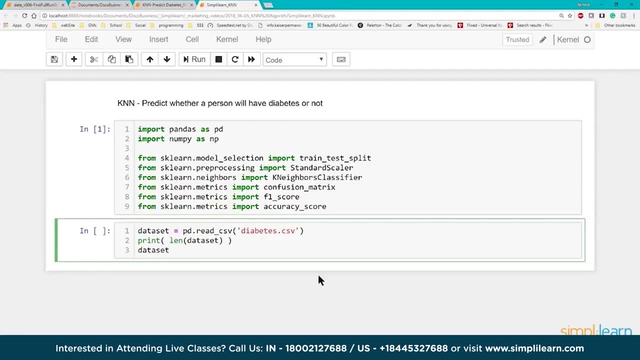 you want to do the print in front of there And then we want to take a look at the actual dataset And since we're in pandas, we can simply do dataset head And again. let's go ahead and add the print in there. 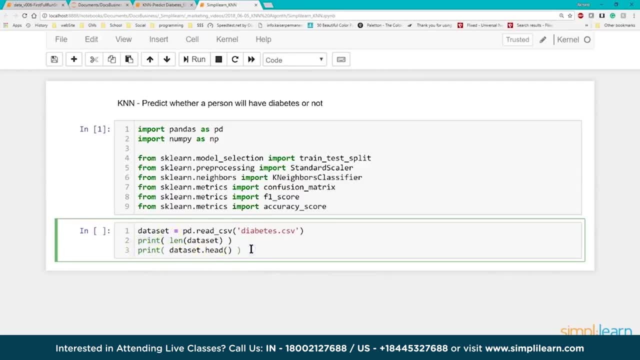 If you put a bunch of these in a row, you know the dataset one head, dataset two head. it only prints out the last one. So I always like to keep the print statement in there. But because most projects only use one data frame, pandas data frame. 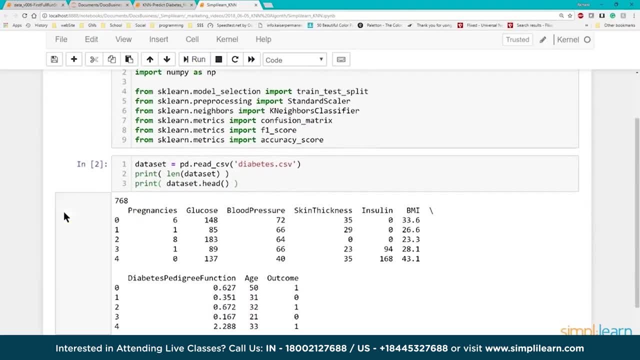 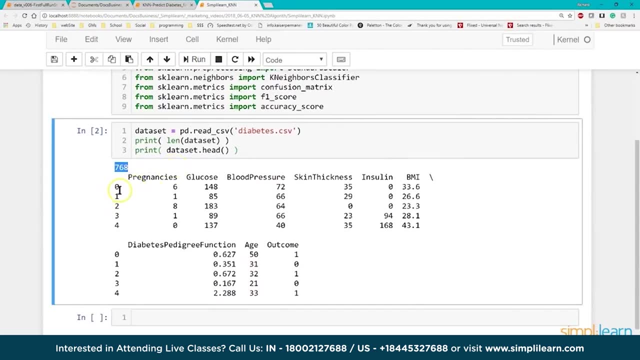 it doesn't really matter. The other way works just fine And you can see when we hit the run button we have the 768 lines which we knew And we have our pregnancies. It's automatically given a label on the left. Remember, the head only shows the first. 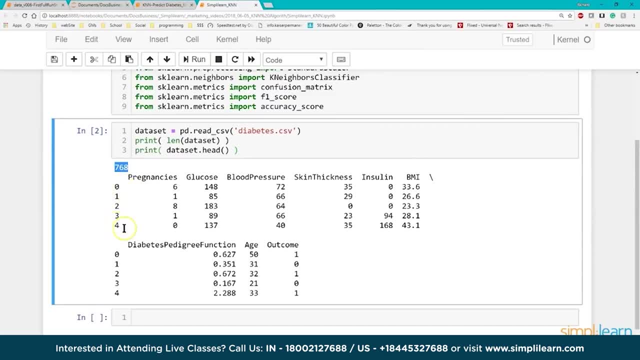 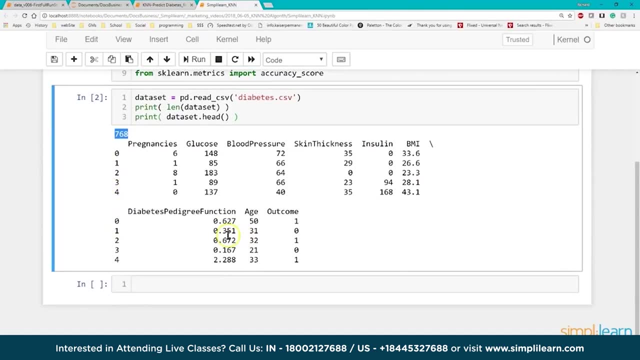 five lines, So we have zero through four And just a quick look at the data you can see it matches what we looked at before. We have pregnancy, glucose blood pressure, all the way to age, And then the outcome on the end. 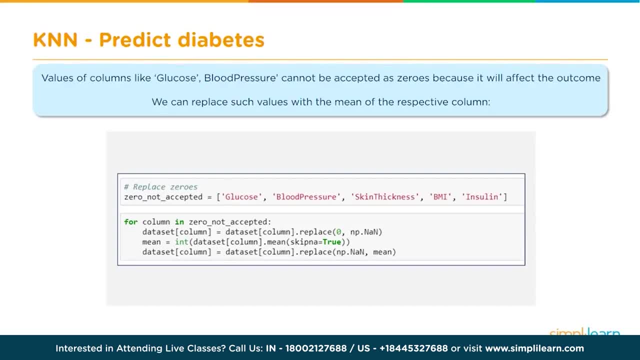 And we're going to do a couple things in this next step. We're going to create a list of columns where we can't have zero. There's no such thing as zero skin thickness or zero blood pressure or zero glucose. Any of those, you'd be dead. 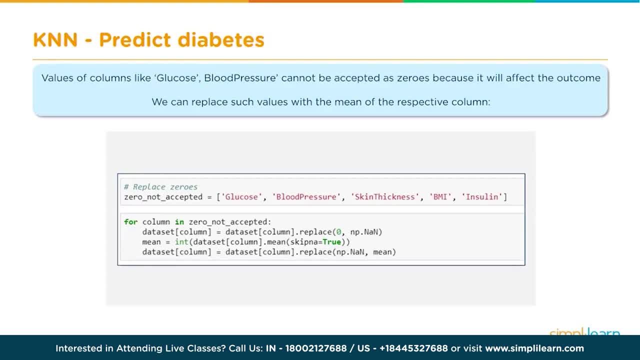 So not a really good factor if they have a zero in there because they didn't have the data, And we'll take a look at that because we're going to start replacing that information with a couple of different things And let's see what that looks like. 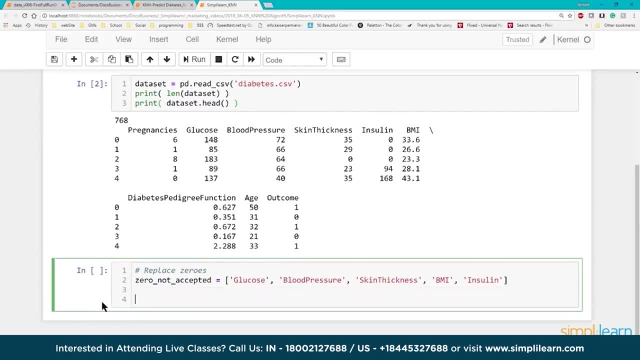 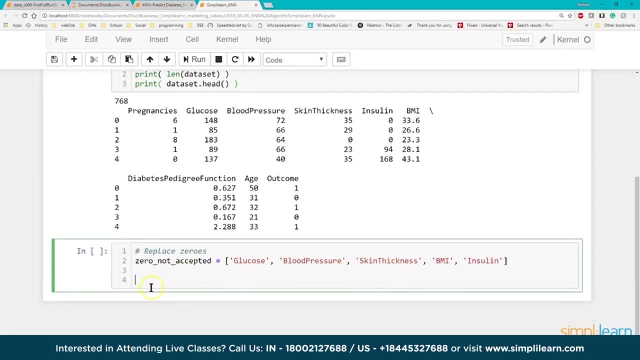 So first we create a nice list. As you can see, we have the values we talked about- glucose, blood pressure, skin thickness- And this is a nice way when you're working with columns is to list the columns you need to do some kind of transformation on. 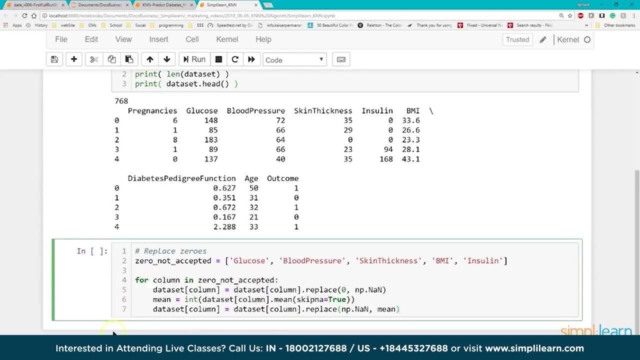 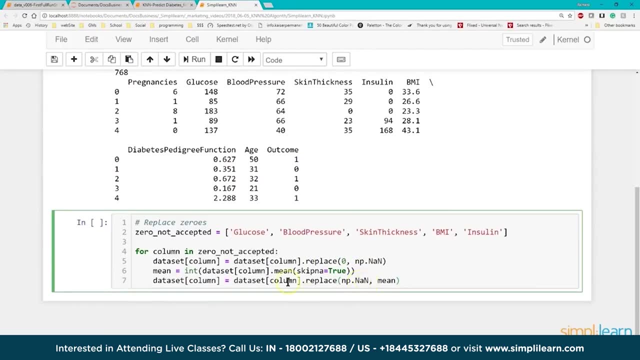 A very common thing to do, And then, for this particular setup, we certainly could use the- there's some panda tools that will do a lot of this- where we can replace the NA, But we're going to go ahead and do it as a dataset column. 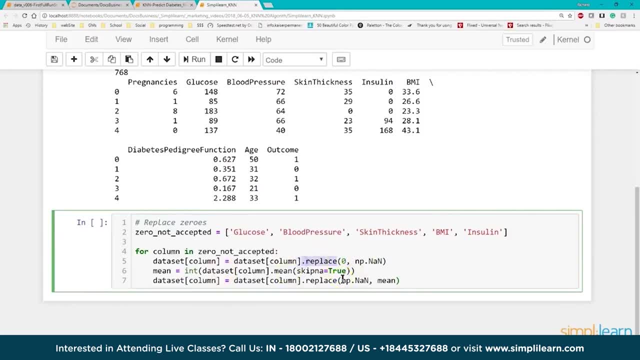 equals dataset column dot replace. this is still pandas. you can do it direct. there's also one that you look for, your NAN. a lot of different options in here, But the NAN numpy NAN is. what that stands for is none. it doesn't exist. 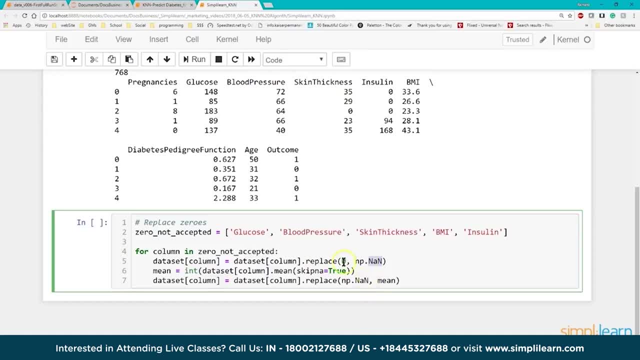 So the first thing we're doing here is we're replacing the zero with a numpy NUN. there's no data there. that's what that says. That's what this is saying right here. So put the zero in and we're going to replace. 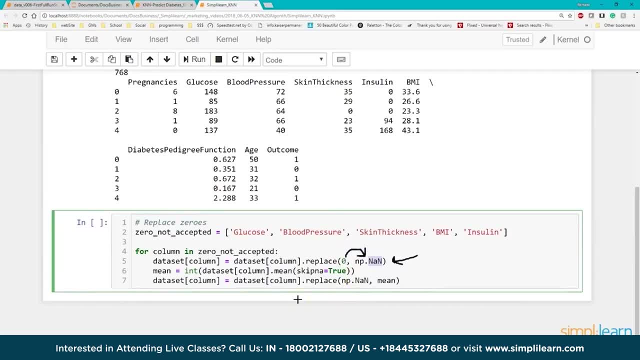 zeros with no data. So if it's a zero, that means the person's well, hopefully not dead, hopefully just didn't get the data. The next thing we want to do is we're going to create the mean, which is the integer from the dataset. 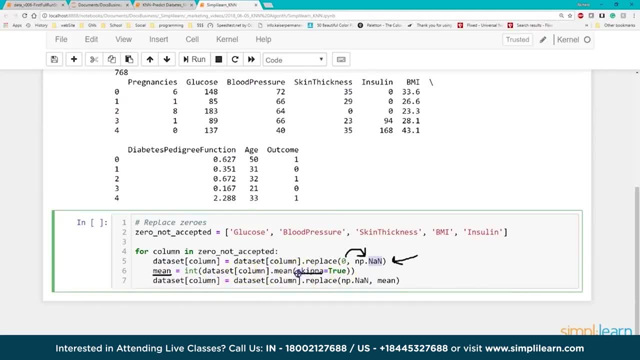 from the column dot mean where we skip NAs. That is a pandas command, there the skip NA. So we're going to figure out the mean of that dataset And then we're going to take that dataset column and we're going to replace all the 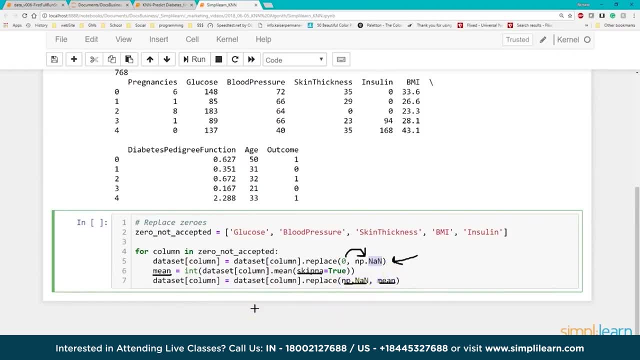 NPNAN with the means. Why did we do that? We could have actually just taken this step and gone right down here and just replaced zero and skipped anything where except there's a way to skip zeros and then just replace all the zeros. But in this case we want to go ahead and do it this way. 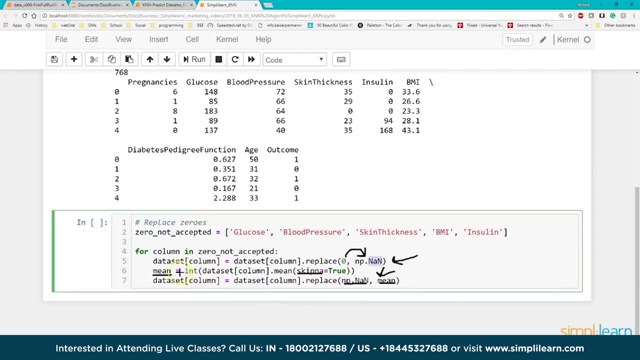 so you can see that we're switching this to a non-existent value. Then we're going to create the mean, and this is the average person. So if we don't know what it is, if they did not get the data, and the data is missing, 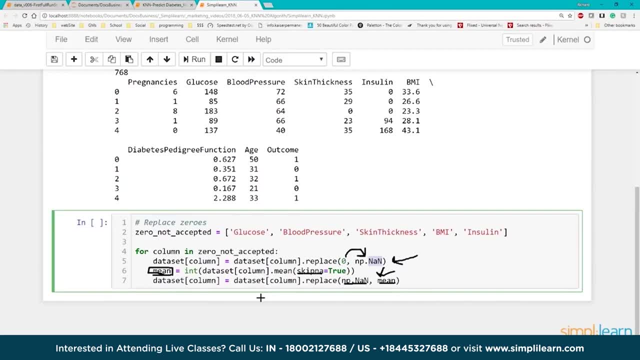 one of the tricks is you replace it with the average, What is the most common data for that. This way you can still use the rest of those values to do your computation and it kind of just brings that particular value, those missing values, out of the equation. 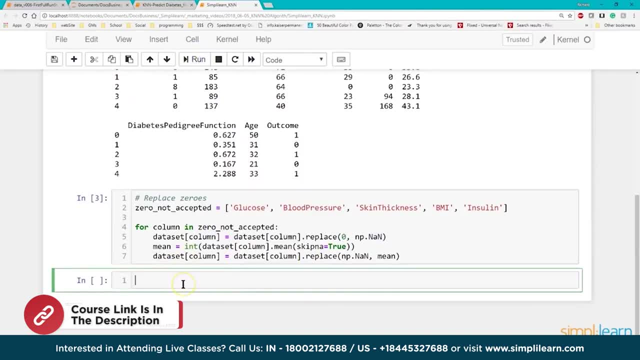 Let's go ahead and take this and we'll go ahead and run it. It doesn't actually do anything, so we're still preparing our data. If you wanted to see what that looks like, we don't have anything in the first few lines, so it's not going to show up. 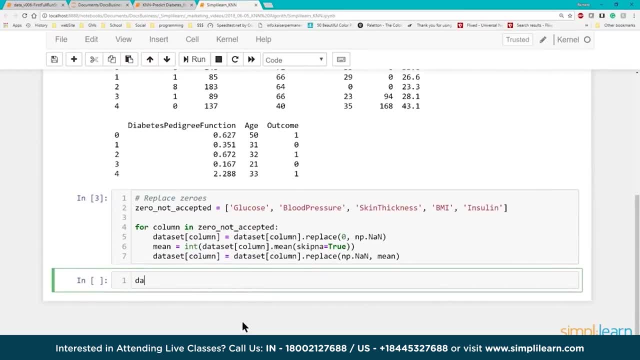 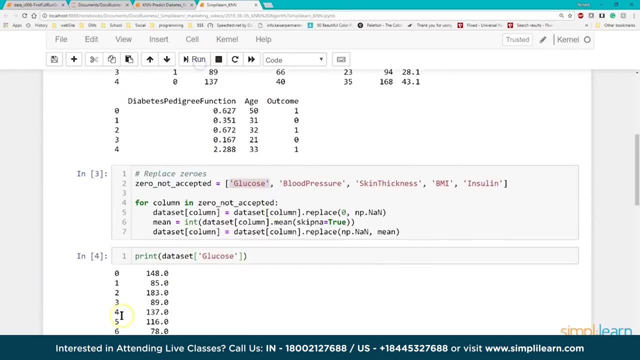 but we certainly could look at a row. Let's do that. Let's go into our data set, let's print a data set and let's pick. in this case, let's just do glucose, and if I run this, this is going to print. 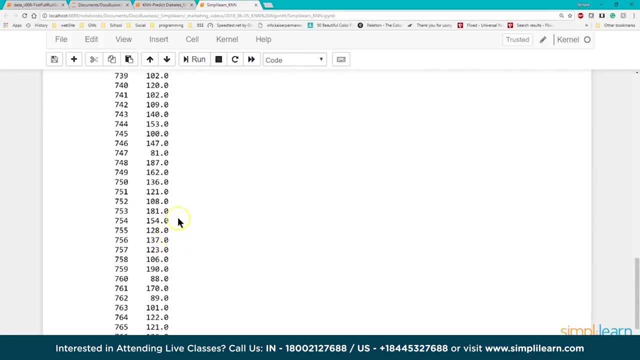 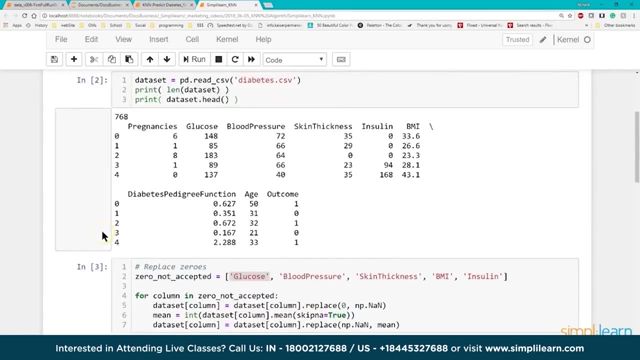 all the different glucose levels going down, and we thankfully don't see anything in here that looks like missing data. at least on the ones it shows, you can see it skipped a bunch in the middle, because that's what it does If you have too many lines. 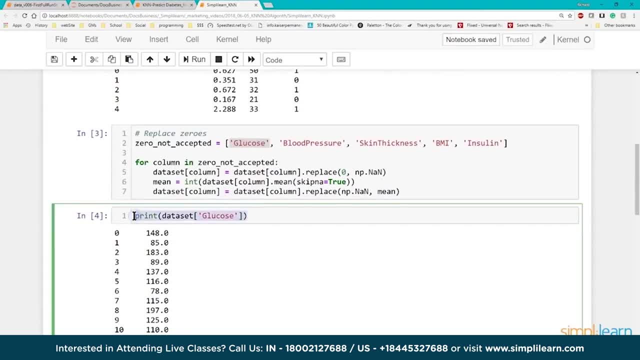 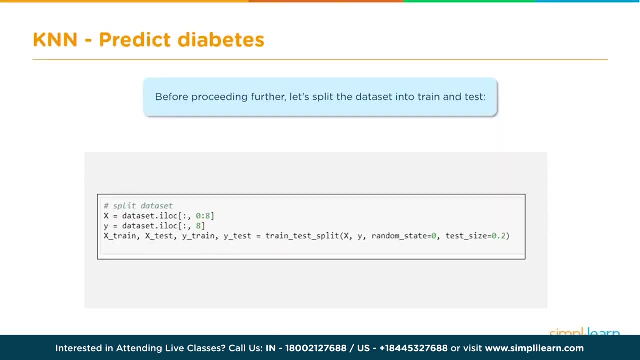 in Jupyter Notebook, it'll skip a few in the data set. Let me go ahead and remove this and we'll just zero out that. and, of course, before we do any processing, before proceeding any further, we need to split the data set into our train and testing data. That way we have something. 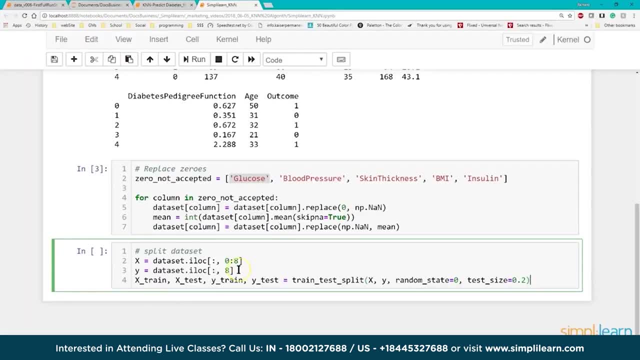 to train it with and something to test it on. And you're going to notice, we did a little something here with the Pandas database code. There we go, my drawing tool. We've added in this right here off the data set, and what this says is that the first one. 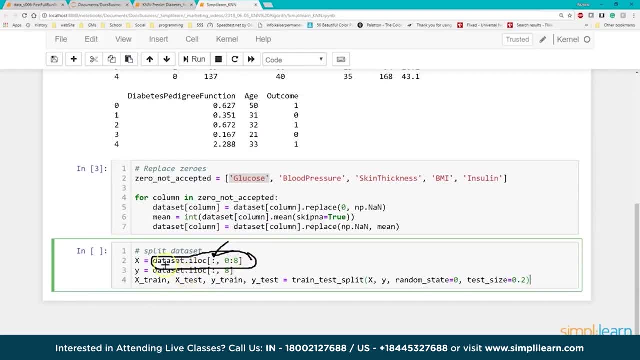 in Pandas- this is from the PD Pandas. it's going to say: within the data set, we want to look at the i location and it is all rows. that's what that says. So we're going to keep all the rows, but we're only looking at zero. 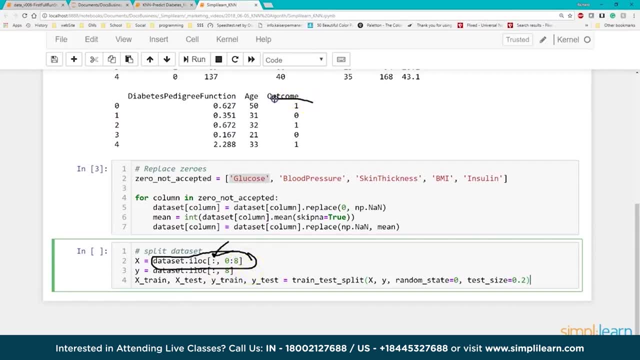 column zero to eight. Remember column nine? here it is right up here. we printed it in. here is outcome: Well, that's not part of the training data. that's part of the answer. Yes, column nine, but it's listed as eight, number eight, So zero. 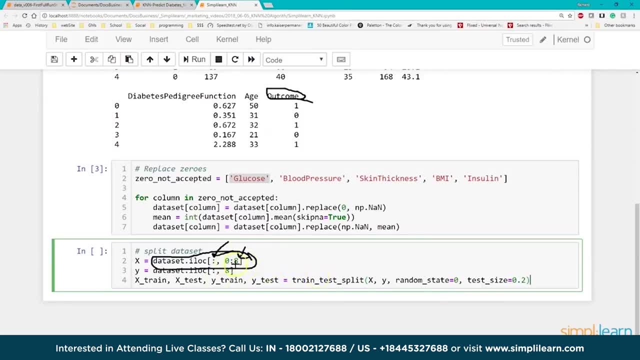 to eight is nine columns, So eight is the value, And when you see it in here, zero. this is actually zero to seven. It doesn't include the last one. And then we go down here to y, which is our answer, and we want just the last one. 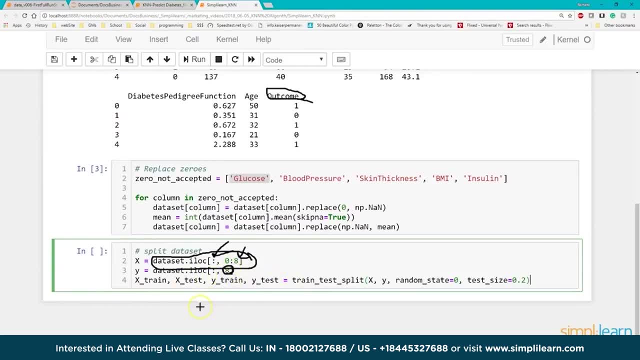 Just column eight And you can do it this way with this particular notation. And then, if you remember, we imported the train test split- That's part of the sklearn right there, And we simply put in our x and our y. We're going to do random state. 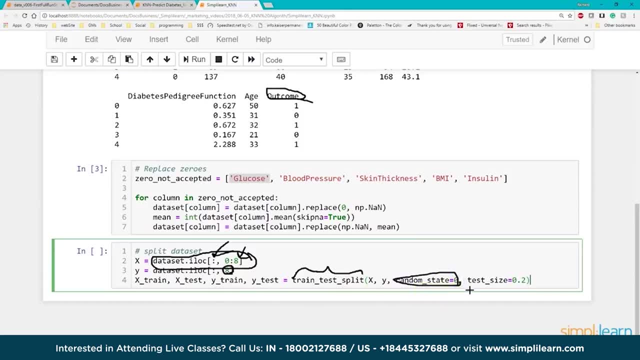 equals zero. You don't have to necessarily seed it. That's a seed number. I think the default is one when you seed it. I'd have to look that up. And then the test size. Test size is point two. That simply means we're going to. 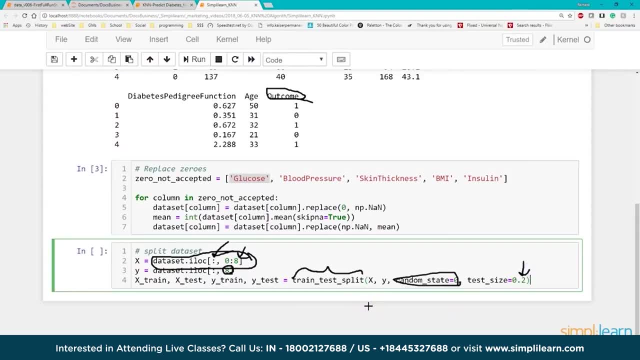 take twenty percent of the data and put it aside so that we can test it later. That's all that is, And again we're going to run it. Not very exciting. So far we haven't had any printout other than to look at the. 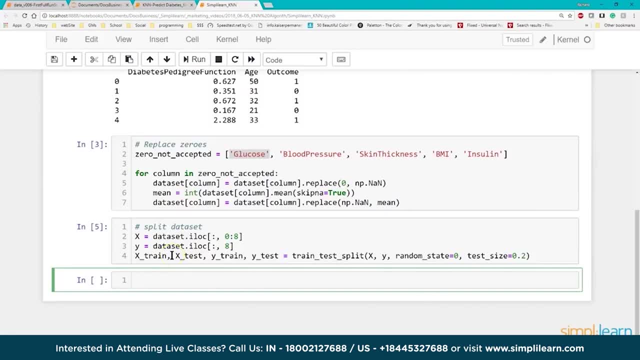 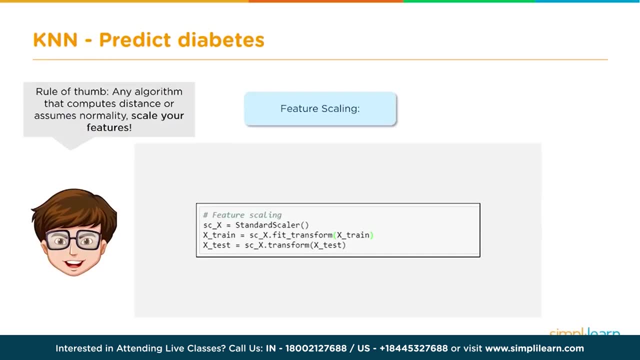 data, But that is a lot of. this is prepping this data. Once you prep it, the actual lines of code are quick and easy And we're almost there with the actual running of our knn. We need to go ahead and do a scale the data. 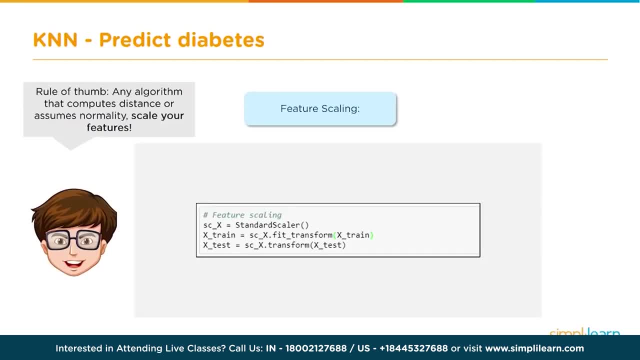 If you remember correctly, we're fitting the data in a standard scaler, which means instead of the data being from five to three hundred and three in one column and the next column is one to six. We're going to set that all so that all the data is between. 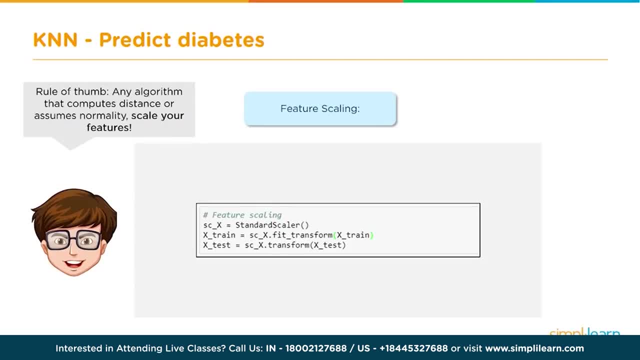 minus one and one. That's what that standard scaler does, Keeps it standardized, And we only want to fit the scaler with the training set. but we want to make sure the testing set is the x test going in is also transformed, So it's processing it the same. 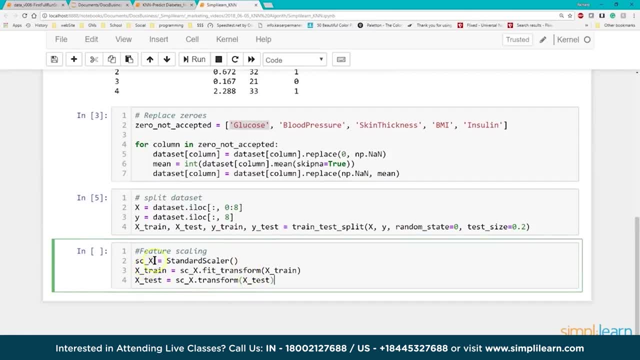 So here we go with our standard scaler. We're going to call it sc underscore x for the scaler And we're going to import the standard scaler into this variable, and then our x train equals sc underscore x, dot fit transform. So we're creating the scaler on the 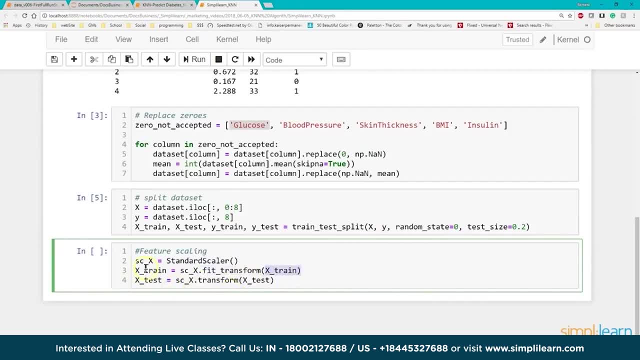 x train variable And then our x test. we're also going to transform it. So we've trained and transformed the x train and then the x test isn't part of that training. It isn't part of training the transformer, It just gets transformed. That's all it does. 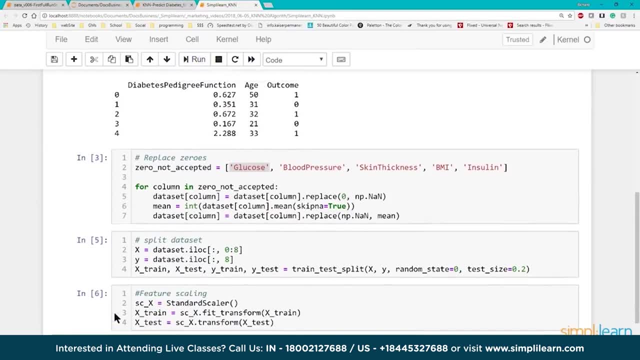 And again, we're going to go ahead and run this And if you look at this, we've now gone through these steps, All three of them. We've taken care of replacing our zeros for key columns. that shouldn't be zero And we've replaced that. 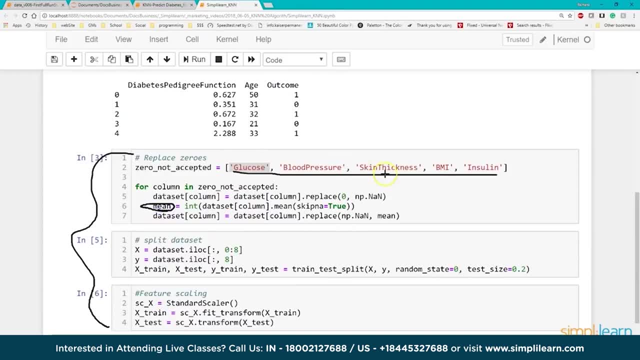 with the means of those columns, That way that they fit right in with our data models. We've come down here and we've split the data, So now we have our test data and our training data, And then we've taken and we've scaled the data. 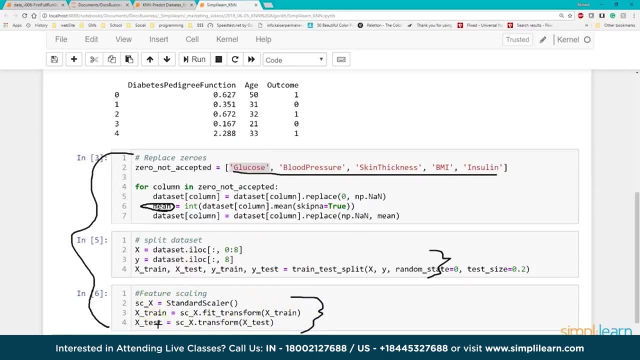 So all of our data going in Now? no, we don't train the y part, The y train and y test. That never has to be trained. It's only the data going in. That's what we want to train in there Then. 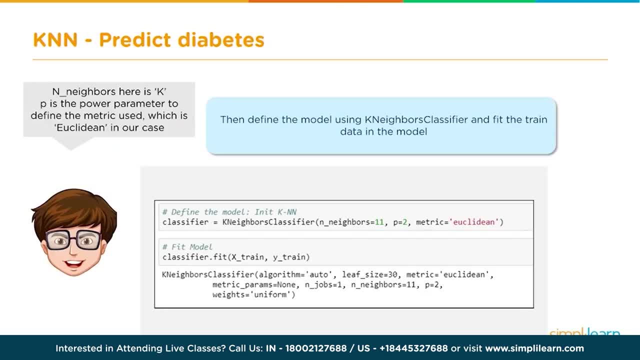 we find the model using kNeighborsClassifier and fit the train data in the model. So we do all that data prep and you can see down here we're only going to have a couple lines of code where we're actually building our model and training it. That's one of the cool. 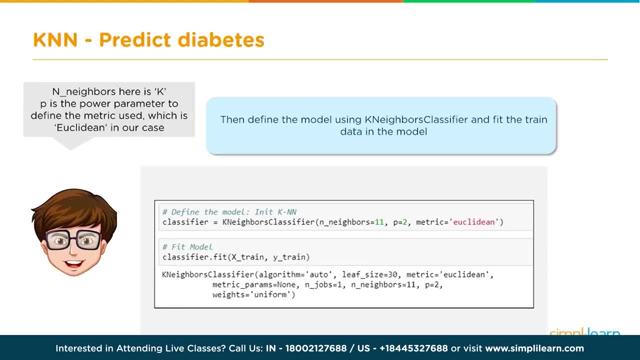 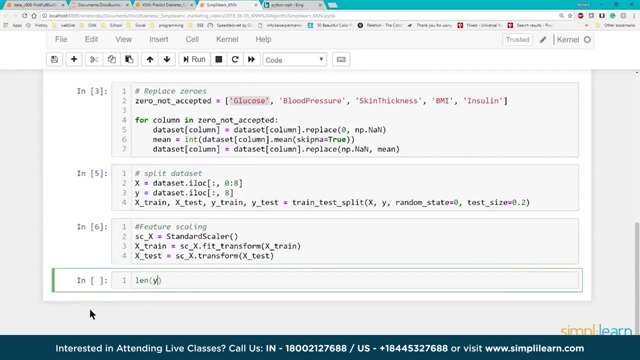 things about Python and how far we've come. It's such an exciting time to be in machine learning because there's so many automated tools. Let's see before we do this. let's do a quick length of and let's do y We want. 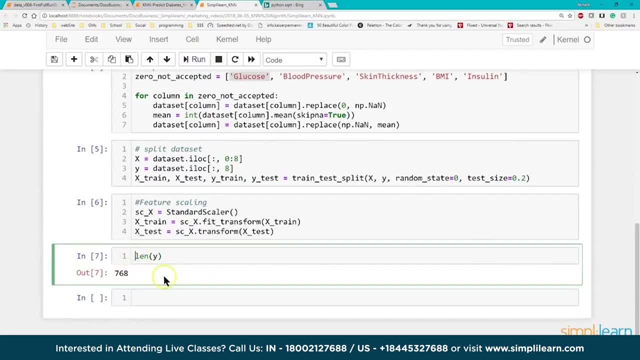 let's just do length of y And we get 768.. And if we import math, we do math, dot square root. Let's do y train. There we go. It's actually supposed to be x train Before we do this, let's go. 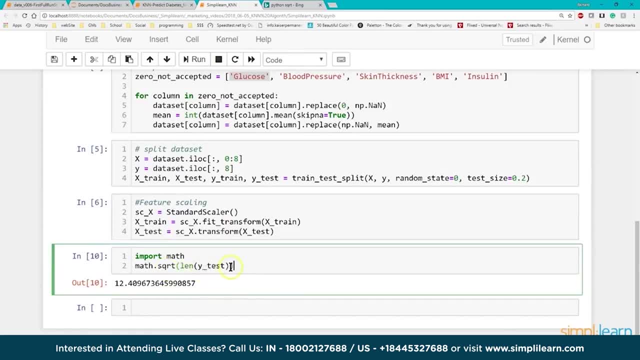 ahead and do import math and do math square root length of y test, And when I run that we get 12.409.. I wanted to show you where this number comes from. we're about to use 12 is an even number, So if you know if you're ever voting- 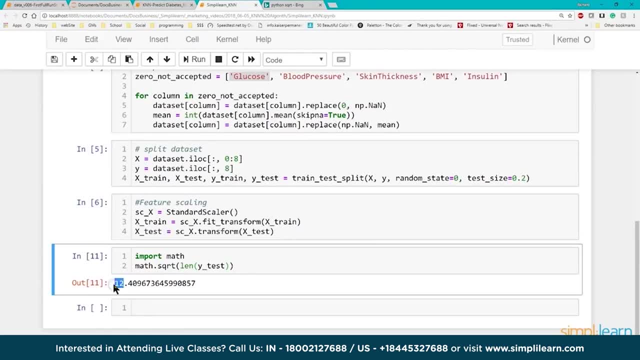 on things. Remember the neighbors all vote. Don't want to have an even number of neighbors voting, So we want to do something odd And let's just take one away and we'll make it 11.. Let me delete this out of here. That's one of the reasons. 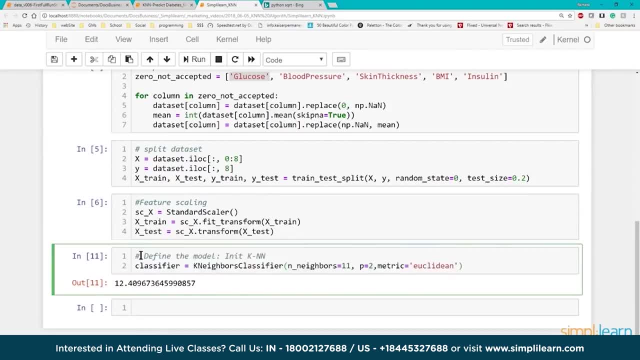 I love Jupyter Notebook because you can flip around and do all kinds of things on the fly. So we'll go ahead and put in our classifier. We're creating our classifier now And it's going to be the kNeighbors classifier: nNeighbors equals 11.. Remember we did. 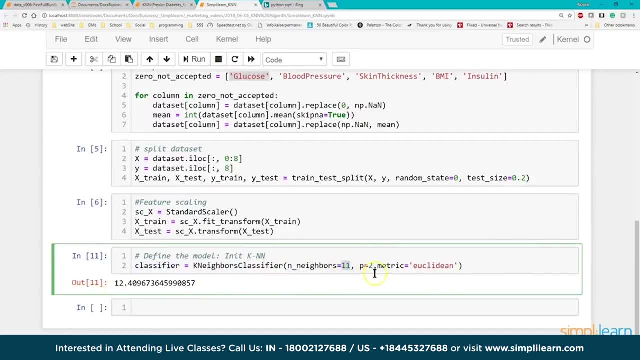 12 minus 1 for 11, so we have an odd number of neighbors. p equals 2, because we're looking for are they diabetic or not, And we're using the Euclidean metric. There are other means of measuring the distance. You could do like square. 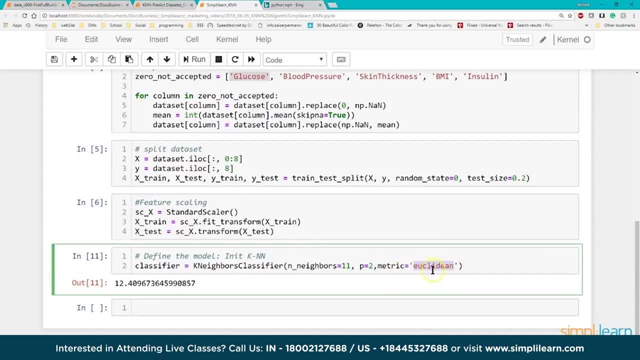 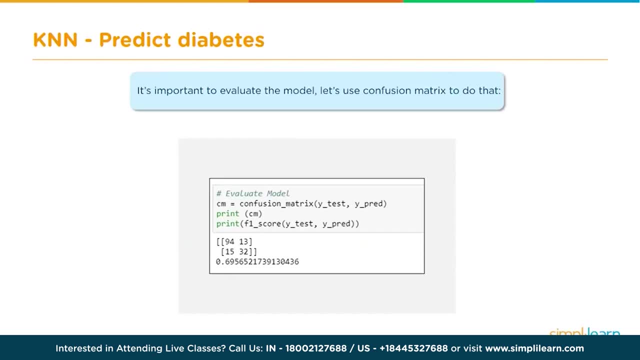 square means values, All kinds of measure this- But the Euclidean is the most common one and it works quite well. It's important to evaluate the model. Let's use the confusion matrix to do that. And we're going to use the confusion matrix, Wonderful tool. 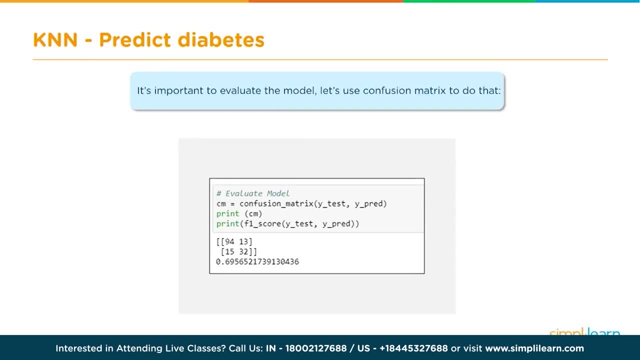 And then we'll jump into the F1 score And, finally, accuracy score, which is probably the most commonly used quoted number when you go into a meeting or something like that. So let's go ahead and paste that in there And we'll set the CME. 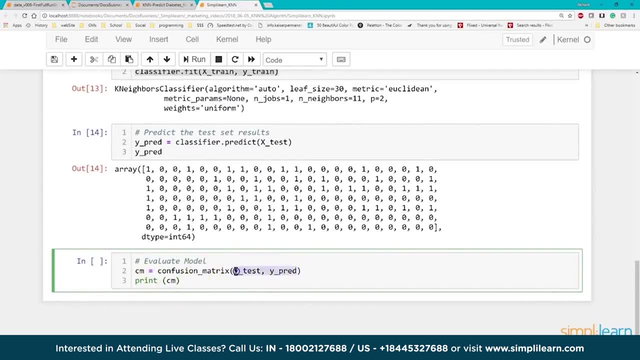 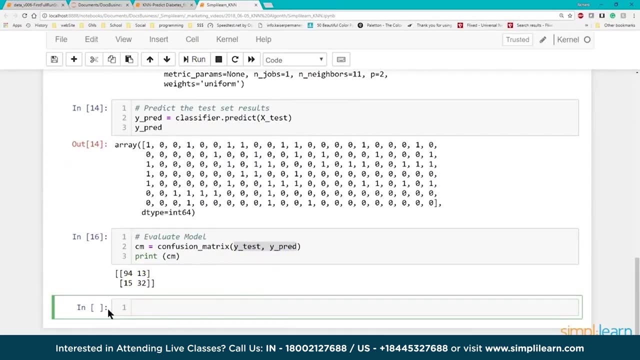 equal to confusion. matrix Y test: Y predict. So those are the two values we're going to put in there. Let me go ahead and run that and print it out And the way you interpret this is: you have the Y predicted, which would be your. 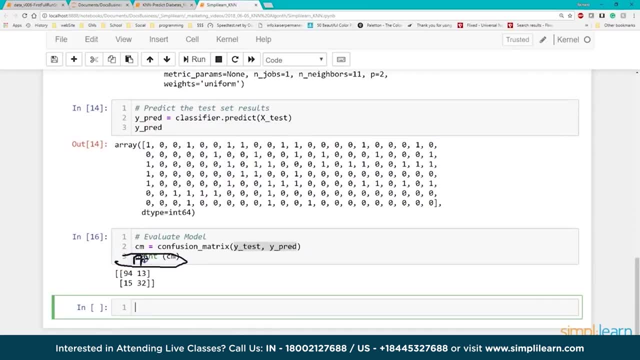 title up here Let's just do P-R-E-D: Predicted across the top and actual going down. Actual- It's always hard to write in here. actual- That means that this column here down the middle that's the important column And it means that our prediction. 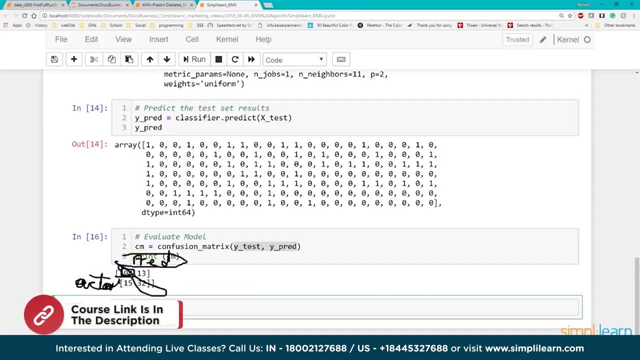 said 94 and prediction in the actual agreed on 94 and 32.. This number here, the 13 and the 15, those are what was wrong. So you could have like three different if you're looking at this across three different variables. 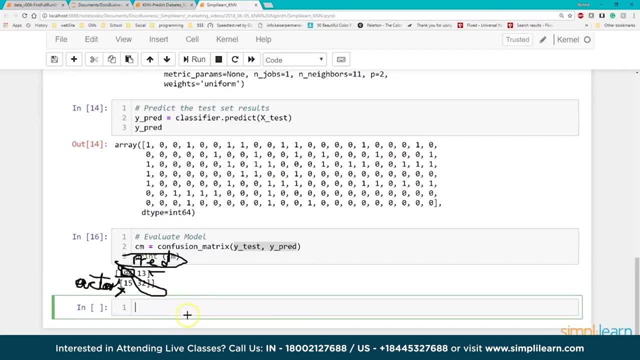 instead of just two. you'd end up with the third row down here and the column going down the middle. So in the first case we have the and I believe the zero is a 94, people who don't have diabetes. The prediction said: 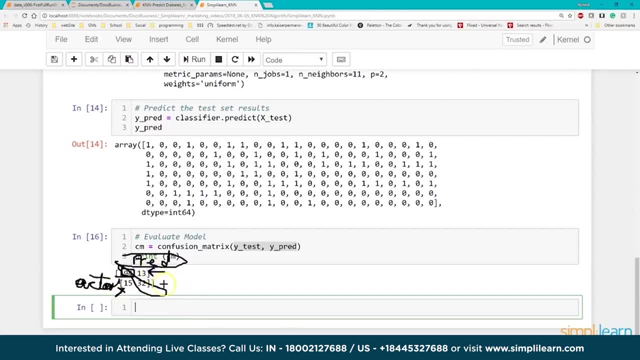 the 13 of those people did have diabetes and were at high risk And the 32 that had diabetes it had correct, But our prediction said another 15. out of that 15 it classified as incorrect, So you can see where that classification comes in. 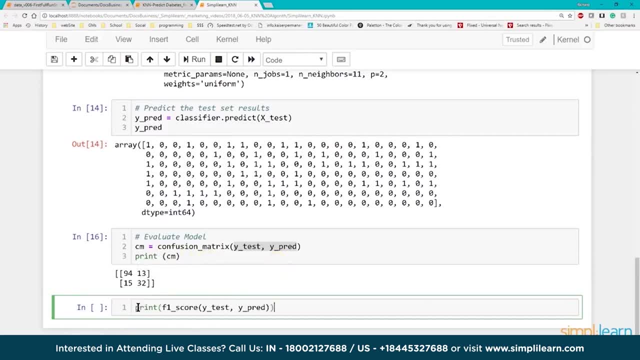 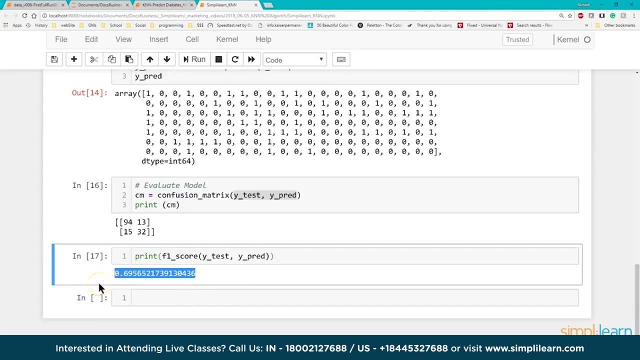 and how that works on the confusion matrix, Then we're going to go ahead and print the F1 score. Let me just run that And you see we get a .69 in our F1 score. The F1 takes into account both sides of the balance. 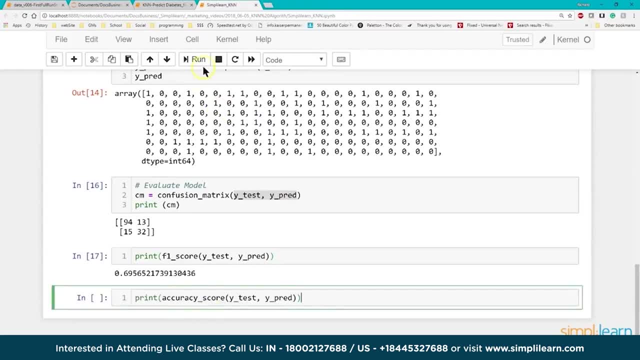 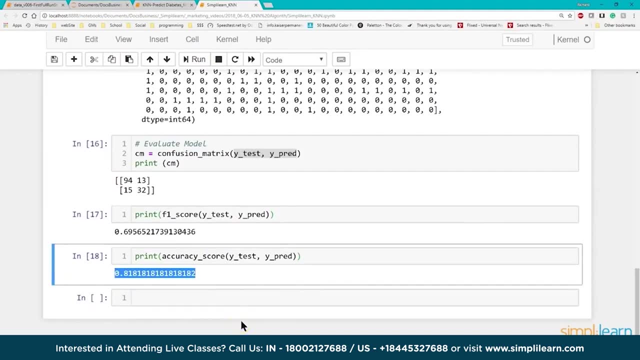 of false positives, Where, if we go ahead and just do the accuracy account- and that's what most people think of is- it looks at just how many we got right out of how many we got wrong. So a lot of people, when you're a data scientist and you're 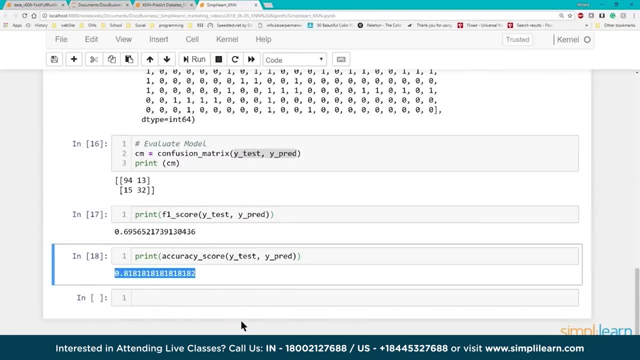 talking to other data scientists, they're going to ask you what the F1 score, the F score, is. If you're talking to the general public or the decision makers in the business, they're going to ask what the accuracy is, And the accuracy is always better. 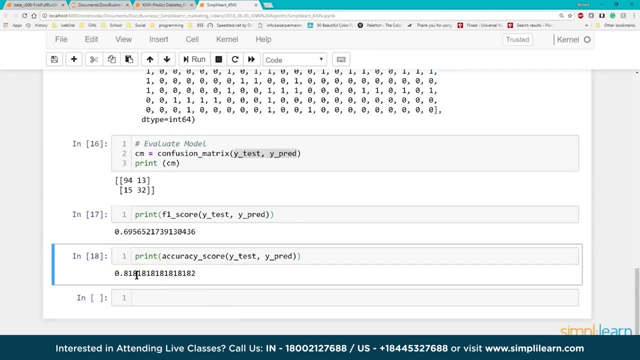 than the F1 score. But the F1 score is more telling. It lets us know that there's more false positives than we would like on here. But 82%, not too bad for a quick flash. look at people's different statistics and running an sklearn and running. 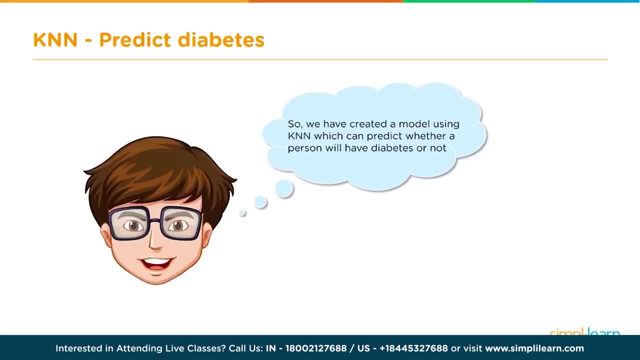 the KNN, the K nearest neighbor on it. So we have created a model using KNN which can predict whether a person will have diabetes or not or, at the very least, whether they should go get a checkup and have their glucose checked regularly or not. 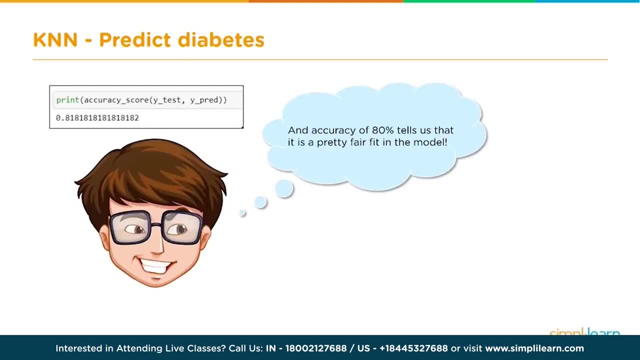 The print accuracy score. we got the 0.818, it was pretty close to what we got and we can pretty much round that off and just say we have an accuracy of 80%. It tells us it is a pretty fair fit in the model Introducing Naive Bayes. 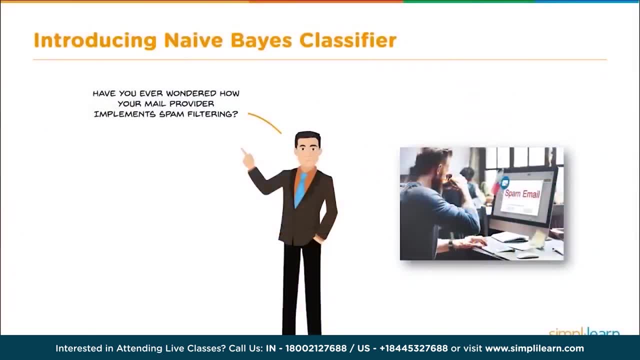 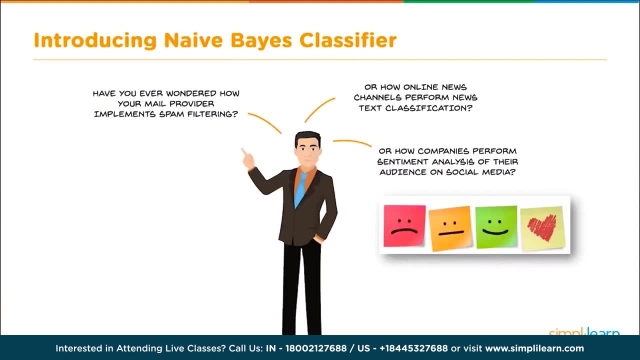 Classifier. Have you ever wondered how your mail provider implements spam filtering, or how online news channels perform news text classification, or how companies perform sentimental analysis of their audience on social media? All of this and more is done through a machine learning algorithm called Naive. 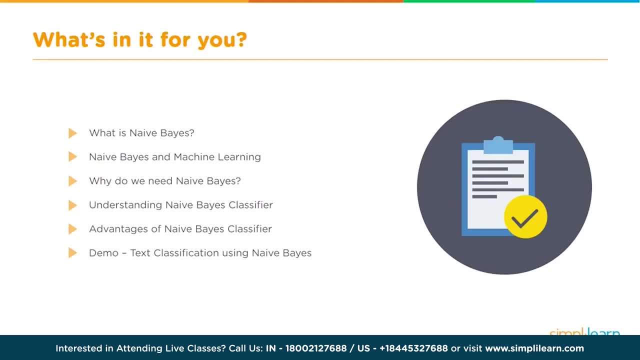 Bayes Classifier. We'll start with what is Naive Bayes- a basic overview of how it works. We'll get into Naive Bayes and machine learning, where it fits in with our other machine learning tools. why do we need Naive Bayes and understanding? 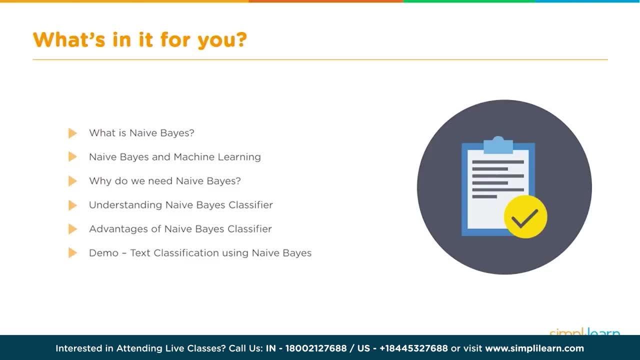 Naive Bayes Classifier a much more in-depth of how the math works in the background. Finally, we'll get into the advantages of the Naive Bayes Classifier in the machine learning setup, and then we'll roll up our sleeves and do my favorite part. 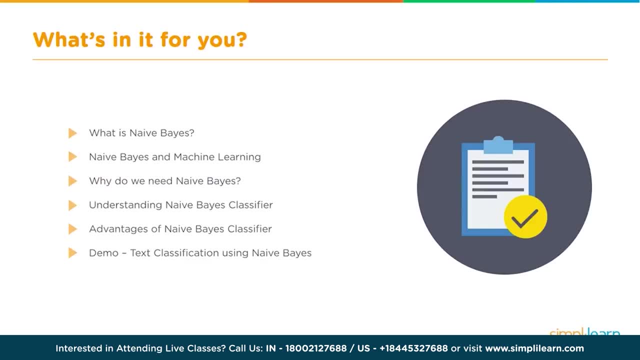 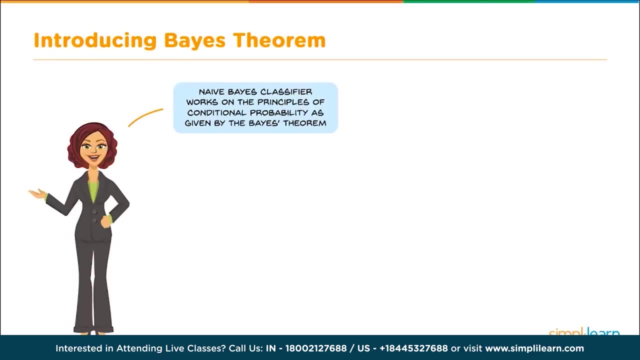 we'll actually do some Python coding and do some text classification using the Naive Bayes. What is Naive Bayes? Let's start with a basic introduction to the Bayes Theorem named after Thomas Bayes from the 1700s, who first coined this? 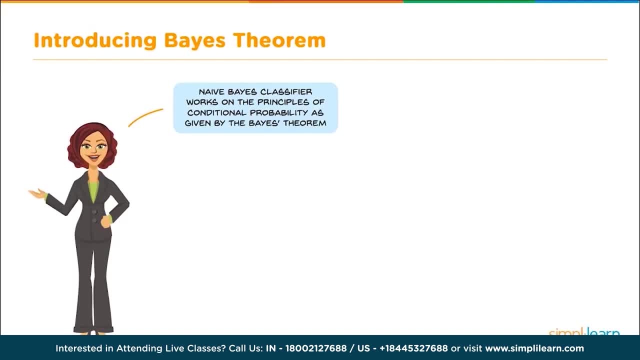 in the western literature, Naive Bayes Classifier works on the principle of conditional probability as given by the Bayes Theorem. Before we move ahead, let us go through some of the simple concepts and the probability that we will be using. Let us consider the following example of tossing: 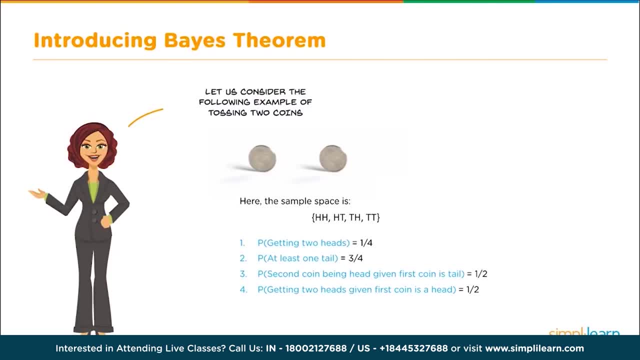 two coins Here we have two quarters and if we look at all the different possibilities of what they can come up, as we get that, they can come up as head heads, come up as head, tell, tell, head and tell, tell When doing the math. 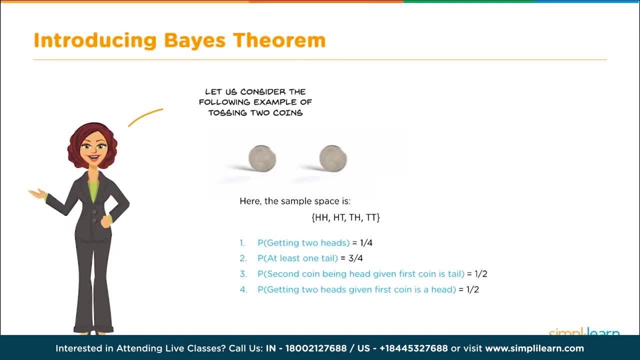 on probability. we usually denote probability as a P, a capital P. So the probability of getting two heads equals one fourth. You can see on our data set we have two heads and this occurs once out of the four possibilities. And then the probability of at least. 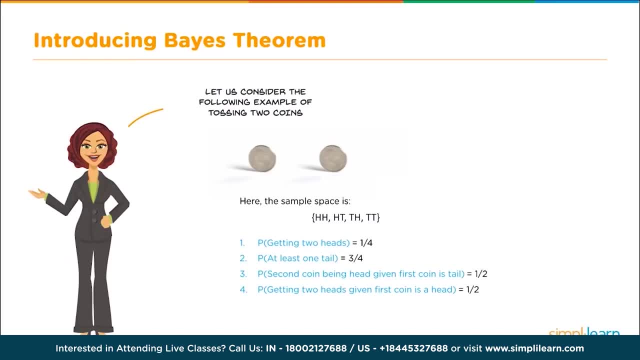 one tell occurs three quarters of the time. You'll see, on three of the coin tosses we have tells in them and out of four that's three fourths. And then the probability of the second coin being head, given the first coin is tell is one half and the 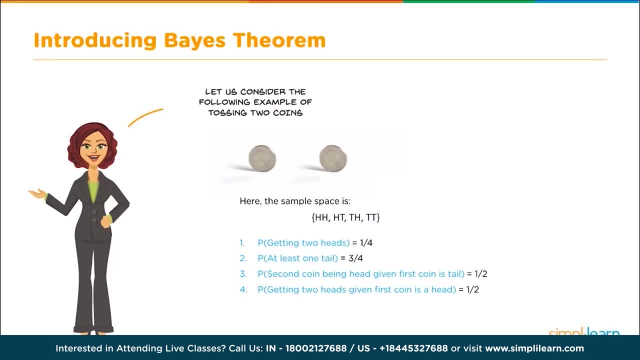 probability of getting two heads. given the first coin is a head is one half. We'll demonstrate that in just a minute and show you how that math works. Now, when we're doing it with two coins, it's easy to see, but when you have something more complex, 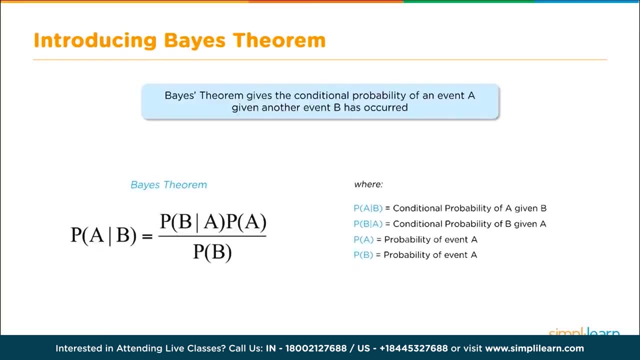 you can see where these formulas really come in and work. So the Bayes theorem gives us the conditional probability of an event A given another event B has occurred. In this case, the first coin toss will be B and the second coin toss A. This could be confusing. 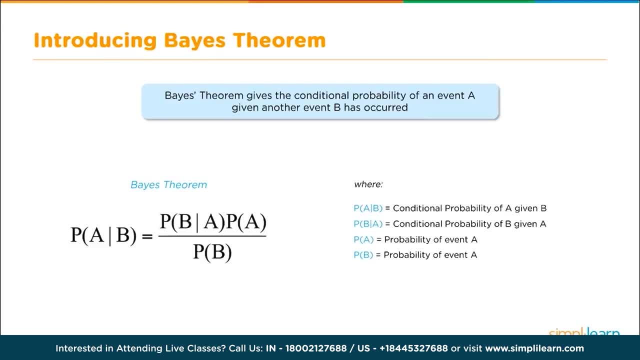 because we've actually reversed the order of them and go from B to A instead of A to B. You'll see this a lot when you work in probabilities. The reason is we're looking for event A. We want to know what that is, So we're going to label that A. 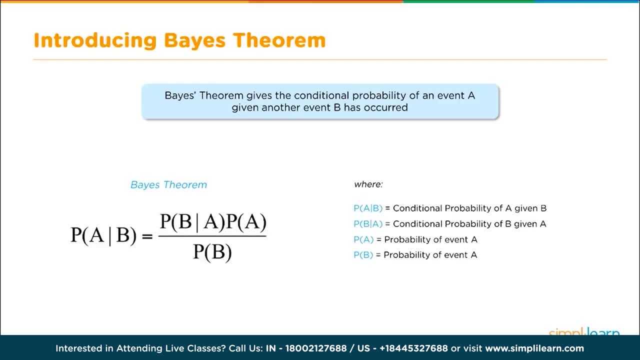 since that's our focus, And then, given another event, B has occurred In the Bayes theorem, as you can see on the left, the probability of A occurring given B has occurred equals the probability of B occurring given A has occurred, times the probability of A over the. 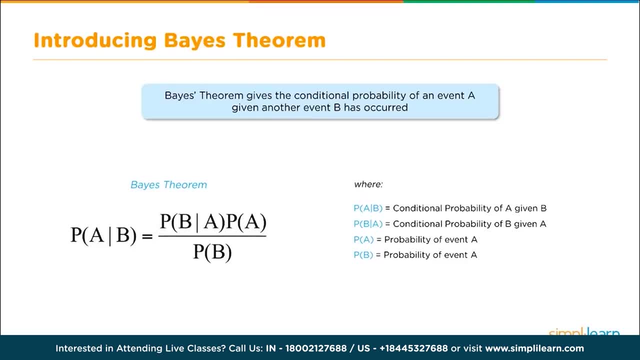 probability of B. This simple formula can be moved around just like any algebra formula And we could do the probability of A after a given B times probability of B equals the probability of B given A times probability of A. You can easily move that around and multiply it and divide it out. 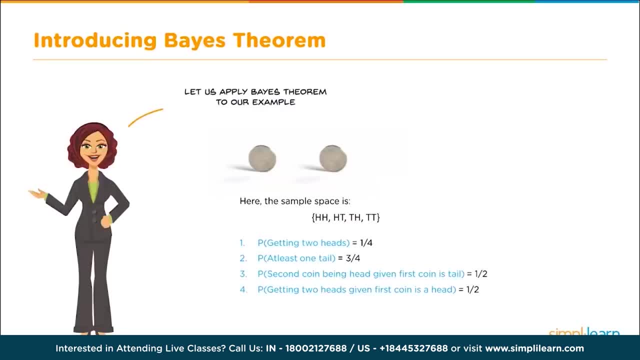 Let us apply Bayes theorem to our example. Here we have our two quarters and we'll notice that the first two probabilities of getting two heads and at least one tail we compute directly off the data. So you can easily see that we have one example, HH. 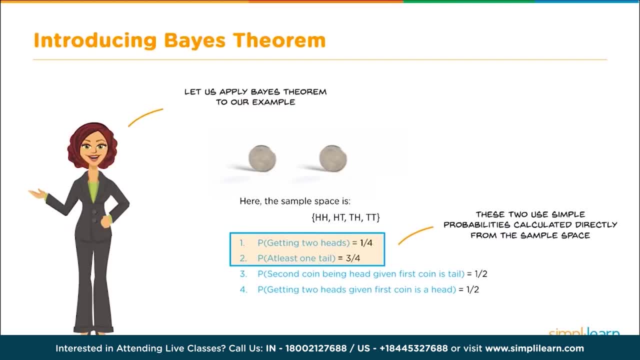 out of four, one fourth, and we have three with tails in them, giving us three quarters or three fourths, 75%. The second condition, the second set, three and four. we're going to explore a little bit more in detail. 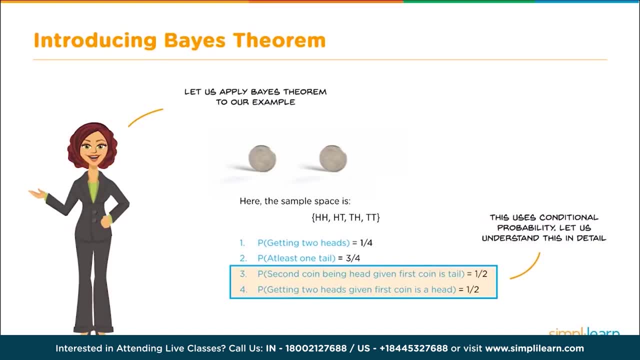 Now we stick to a simple example with two coins, because you can easily understand the math. The probability of throwing a tail doesn't matter what comes before it, and the same with the heads. So it's still going to be 50% or one half, But when? 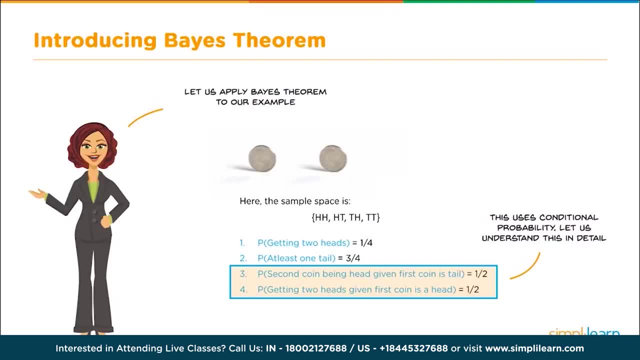 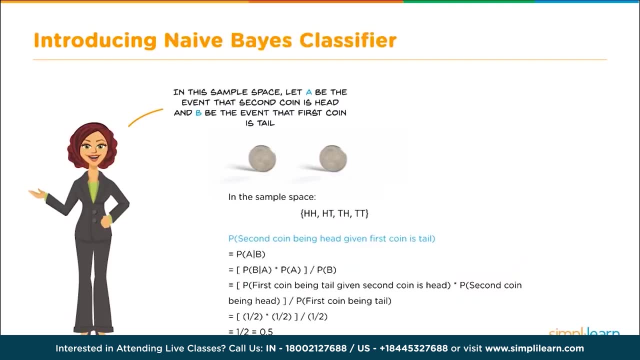 that probability gets more complicated. let's say you have a D6 dice or some other instance, then this formula really comes in handy. But let's stick to the simple example for now. In this sample space, let A be the event that the second coin is head and 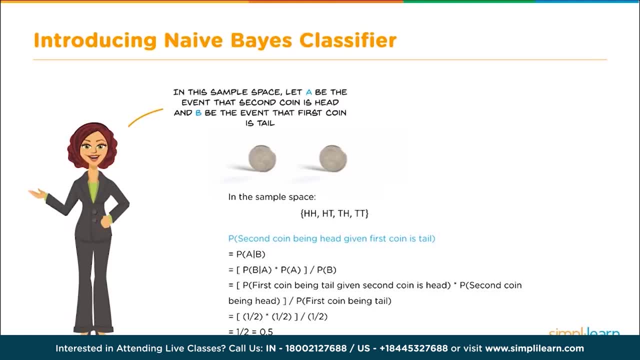 B be the event that the first coin is tails. Again, we reversed it because we want to know what the second event's going to be. So we're going to be focusing on A And we write that out as the probability of A given B. 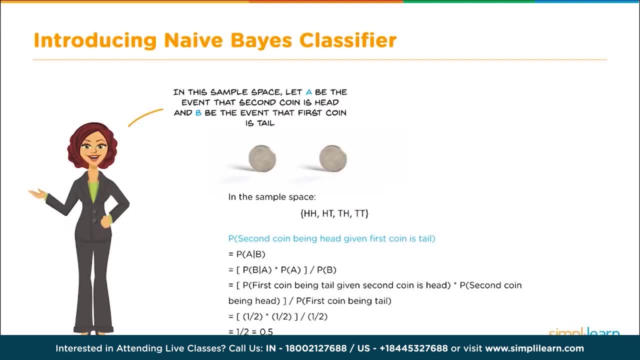 And we know this from our formula- that that equals the probability of B given A times the probability of A over the probability of B. And when we plug that in we plug in the probability of the first coin being tails, given the second coin is heads. 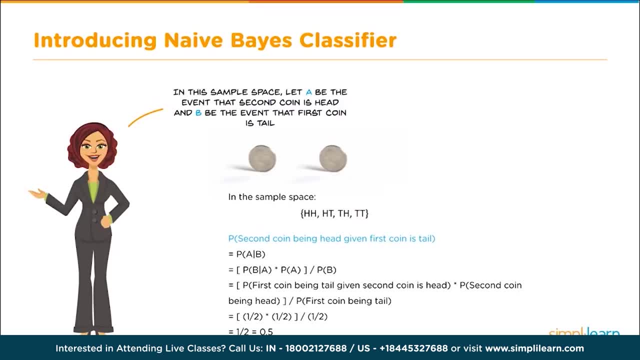 and the probability of the second coin being heads, given the first coin being over the probability of the first coin being tails When we plug that data in and we have the probability of the first coin being tails, given the second coin is heads. 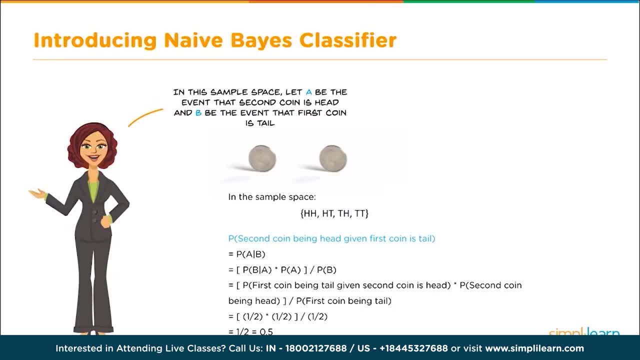 times the probability of the second coin being heads over the probability of the first coin being tails. You can see it's a simple formula to calculate. We have one half times one half over one half, or one half equals .5 or one fourth. 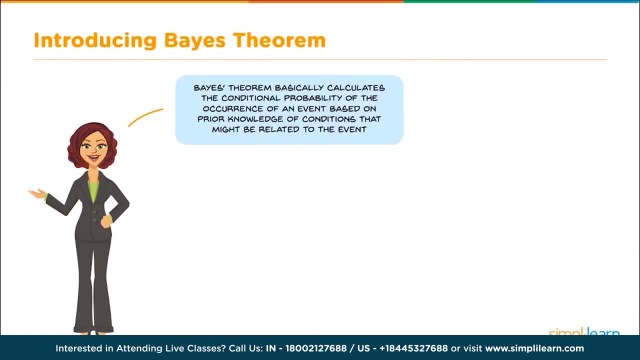 So the Bayes Theorem basically calculates the conditional probability of the occurrence of an event based on prior knowledge of conditions that might be related to the event. We will explore this in detail when we take up an example of online shopping further in this tutorial. 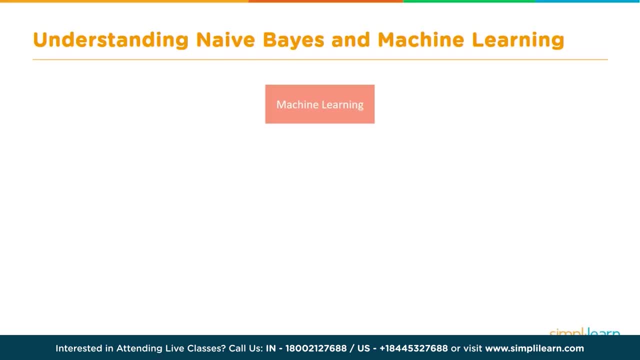 Understanding naive Bayes and machine learning. Like with any of our other machine learning tools, it's important to understand where the naive Bayes fits in the hierarchy. So under the machine learning, we have supervised learning And there is other things like unsupervised. 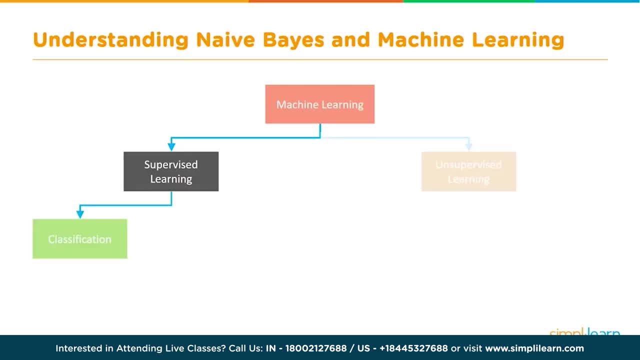 learning. There's also reward system. This falls under the supervised learning. There's classification, There's also regression, But we're going to be in the classification side. And then, under classification, is your naive Bayes. Let's go ahead and glance. 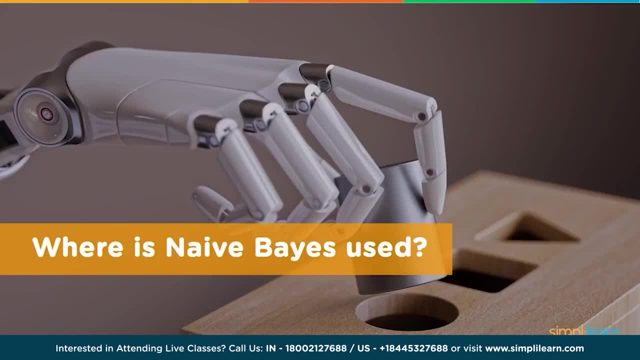 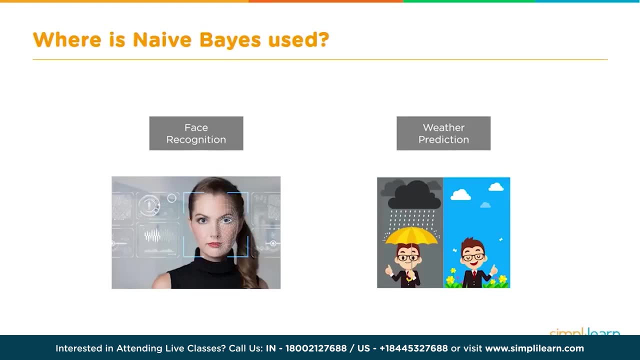 into. where is naive Bayes used? Let's look at some of the used scenarios for it. As a classifier, we use it in face recognition- Is this Cindy, Or is it not Cindy? Or whoever. Or it might be used to identify parts of the face that they then. 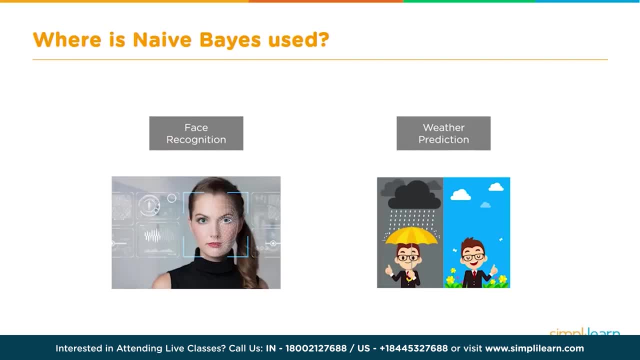 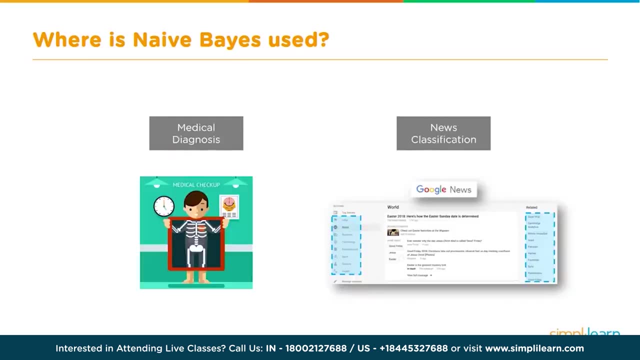 feed into another part of the face recognition program. This is the eye, This is the nose, This is the mouth. Whether prediction Is it going to be rainy or sunny, Medical recognition- News prediction. It's also used in medical diagnosis. 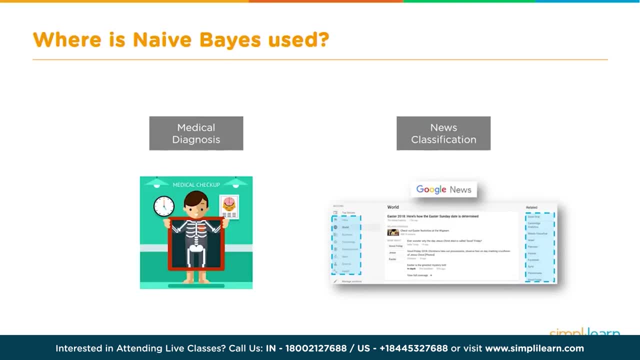 We might diagnose somebody as either as high risk or not as high risk for cancer or heart disease or other ailments, And news classification. We look at the Google News and it says: well, is this political Or is this world news? Or a lot of, that's all. 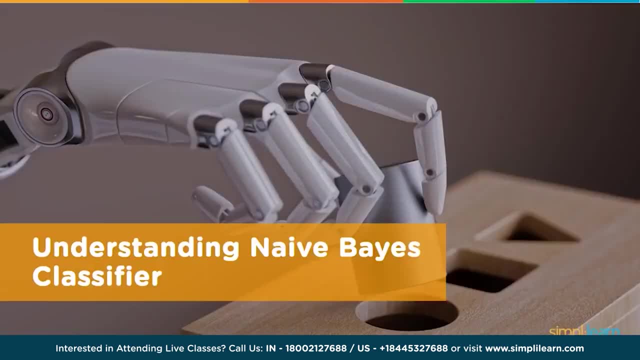 done with the naive Bayes Understanding naive Bayes classifier. Now we already went through a basic understanding with the coins and the two heads and two tells and head tell, tell heads, etc. We're going to do just a quick review on that. 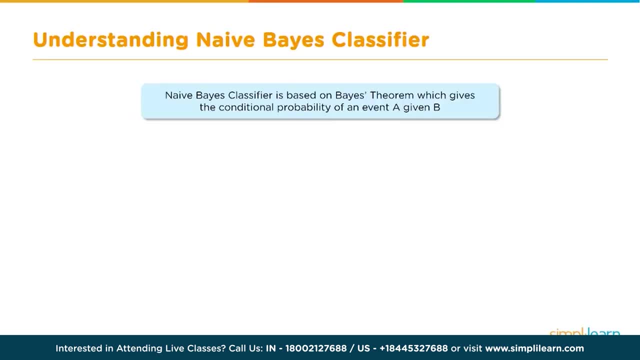 and remind you that the naive Bayes classifier is based on the Bayes theorem, which gives a conditional probability of event A given event B, And that's where the probability of A given B equals the probability of B given A times probability of A over probability of B. Remember, this is an algebraic 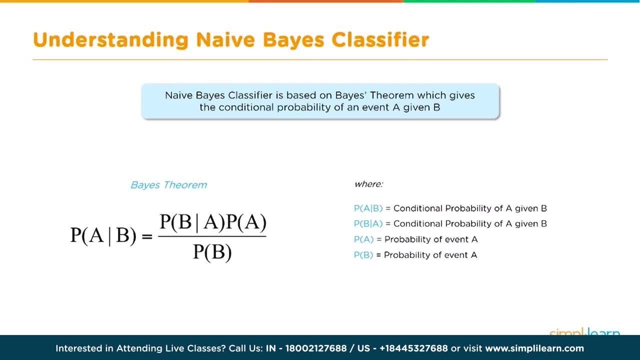 function so we can move these different entities around. We can multiply by the probability of B, So it goes to the left hand side, And then we can divide by the probability of A given B And just as easily come up with a new formula. 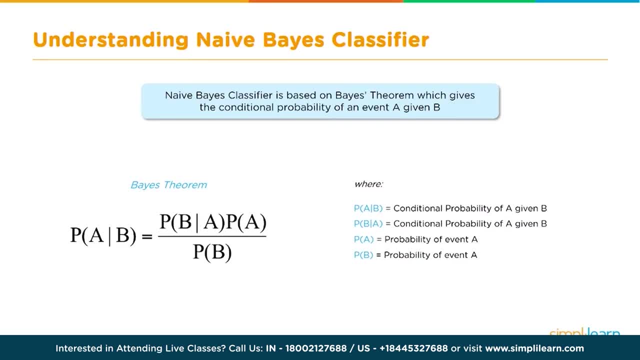 for the probability of B. To me, staring at these algebraic functions kind of gives me a slight headache. It's a lot better to see if we can actually understand how this data fits together in a table, And let's go ahead and start applying it. 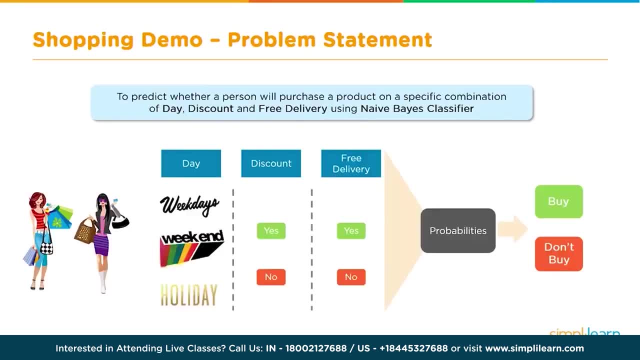 to some actual data so you can see what that looks like. So we're going to start with the shopping demo problem statement And remember we're going to solve this first in table form so you can see what the math looks like, And then we're going to solve it in Python. 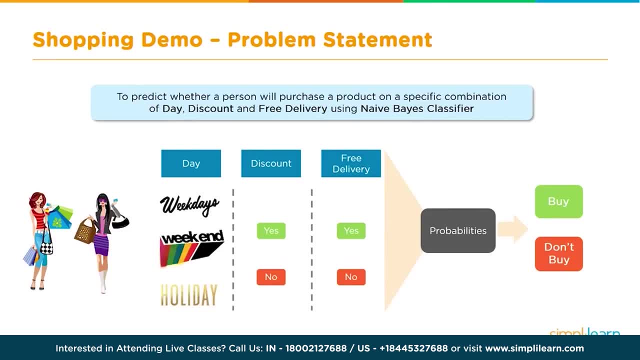 And in here we want to predict whether the person will purchase a product. Are they going to buy or don't buy? Very important: if you're running a business, you want to know how to maximize your profits or at least maximize the purchase of the people. 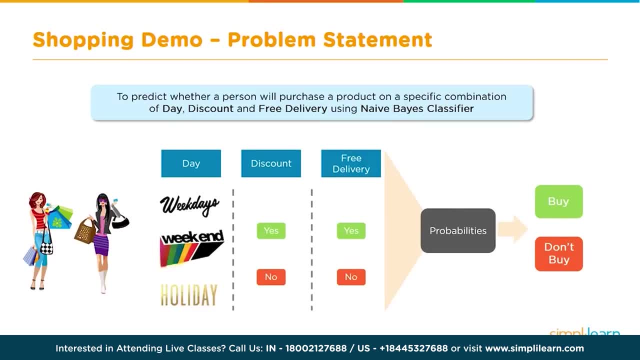 coming into your store And we're going to look at a specific combination of different variables. In this case, we're going to look at the day, the discount and the free delivery And you can see here under the day. we want to know. 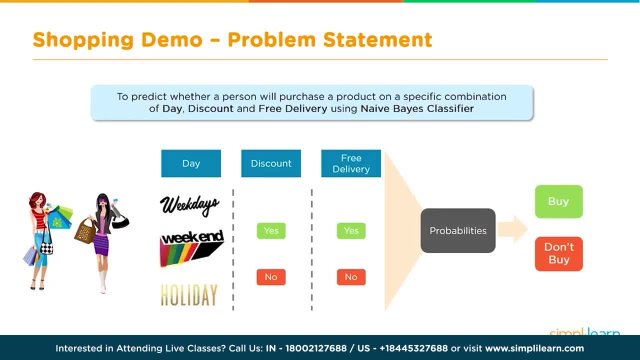 whether it's on the weekday, you know somebody's working. they come in after work or maybe they don't work Weekend. you can see the bright colors coming down there being in work or holiday. And did we offer a discount that day, Yes or no? 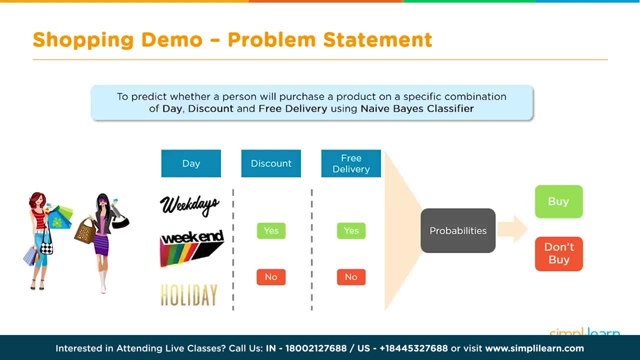 Did we offer free delivery that day, Yes or no? And from this we want to know whether the person's going to buy based on these traits, so we can maximize them and find out the best system for getting somebody to come in and purchase our goods and products from our store. 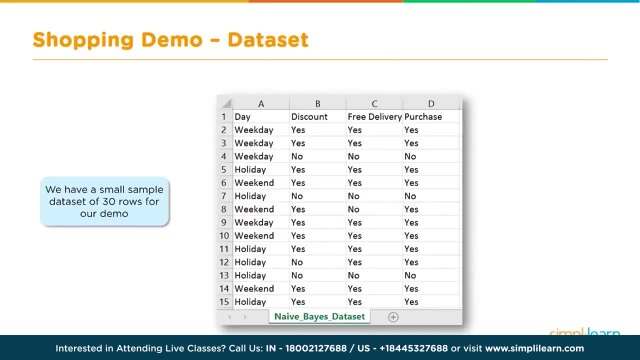 Now, having a nice visual's great, but we do need to dig into the data. So let's go ahead and take a look at the data set. We have a small sample data set of 30 rows. We're showing you the first 15 of those rows for this demo. 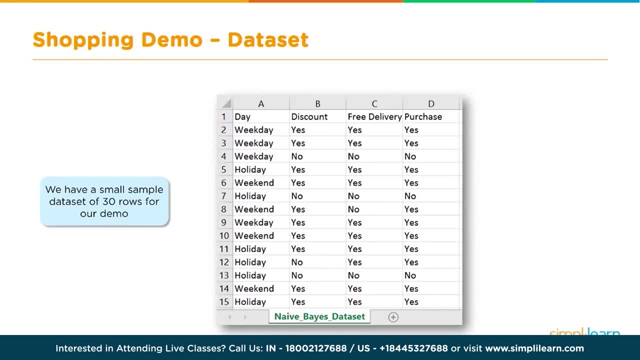 Now the actual data file you can request. Just type in below under the comments on the YouTube video, and we'll send you some more information and send you that file. As you can see here, the file is very simple: columns and rows. 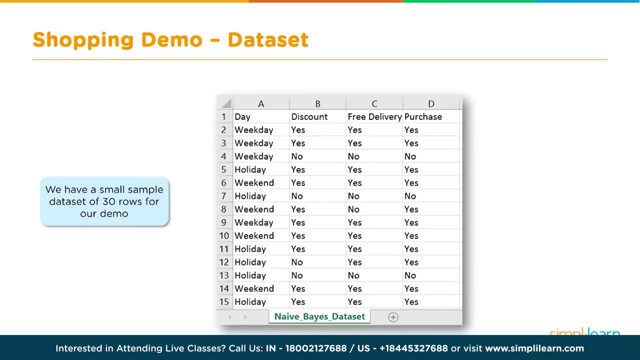 We have the day, the discount, the free delivery, and did the person purchase or not? And then we have under the day whether it was a weekday, a holiday, was it the weekend? This is a pretty simple set of data and long before computers. 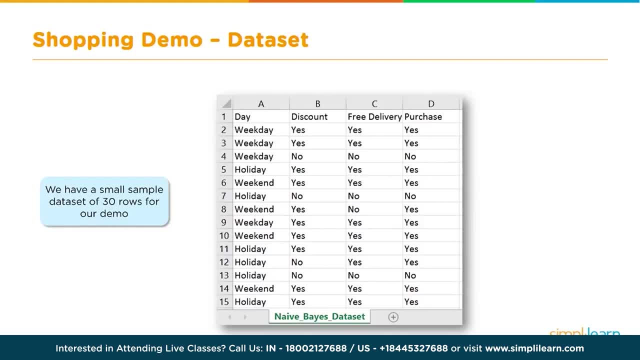 people used to look at this data and calculate this all by hand, So let's go ahead and walk through this and see what that looks like. We put that into tables. Also, note: in today's world, we're not usually looking at three different variables. 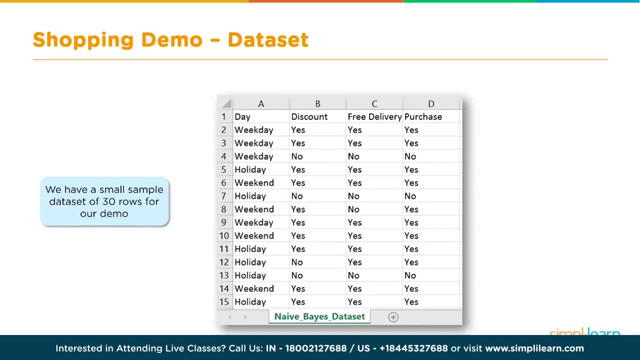 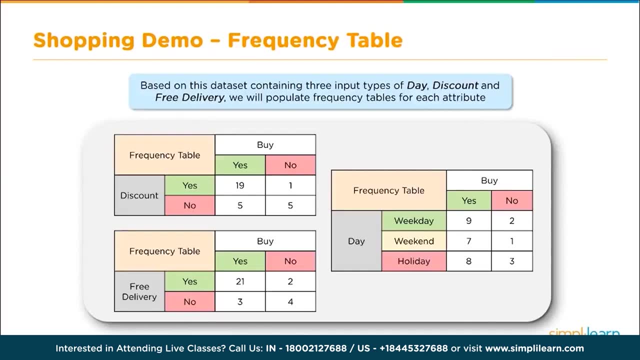 and 30 rows Nowadays, because we're able to collect data so much. we're usually looking at 27,- 30 variables across hundreds of rows. The first thing we want to do is we're going to take this data and, based on the data set containing our 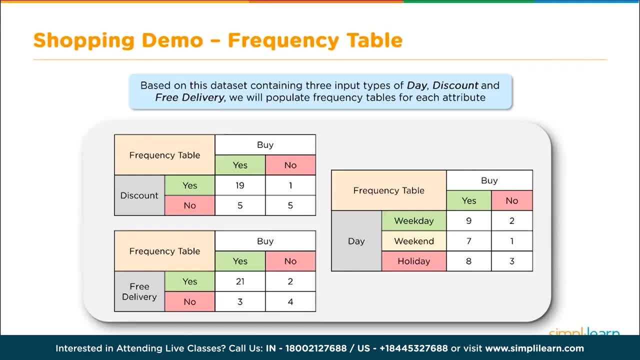 three inputs: day discount and free delivery. we're going to go ahead and populate that to frequency tables for each attribute. So we want to know, if they had a discount, how many people did buy and did not buy. did they have a discount, yes or no? 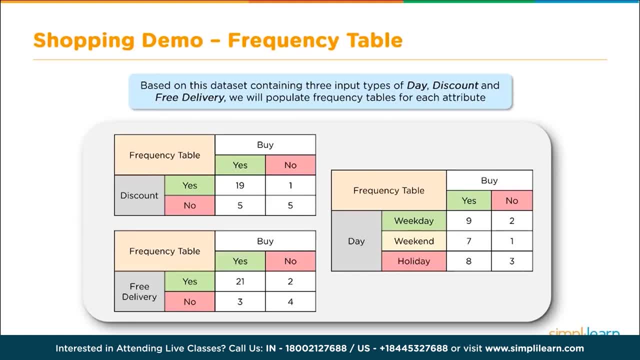 did we have a free delivery, yes or no, on those days? how many people made a purchase and how many people didn't? and the same with the three days of the week: Was it a weekday, a weekend, a holiday, and did they buy yes or no? 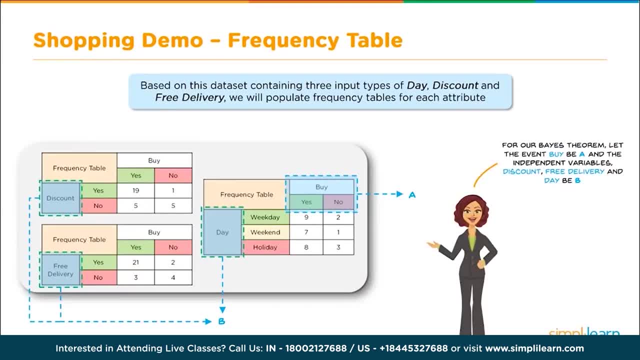 As we dig in deeper to this table for our Bayes Theorem, let the event buy be A. Now remember when we looked at the coins I said we really want to know what the outcome is. Did the person buy or not? And that's usually event A is what? 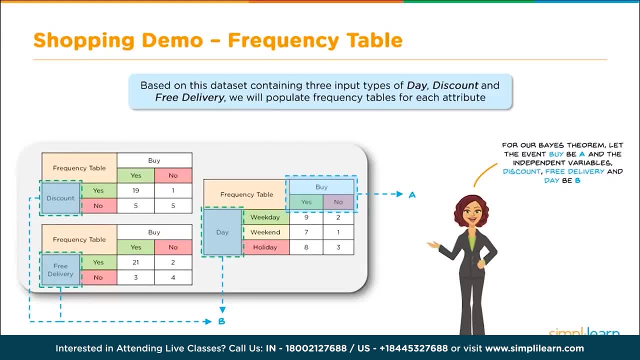 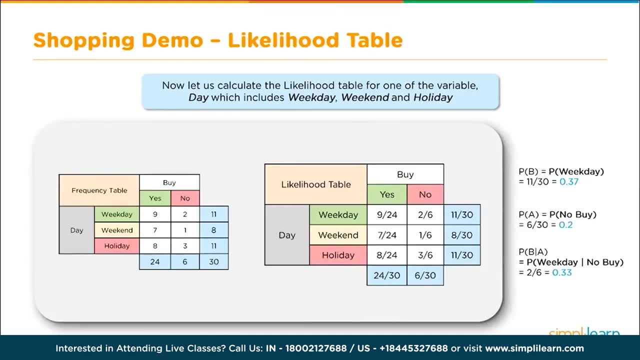 you're looking for And the independent variables discount, free delivery and probability of A be B. So we'll call that probability of B. Now let us calculate the likelihood table for one of the variables. Let's start with day which. 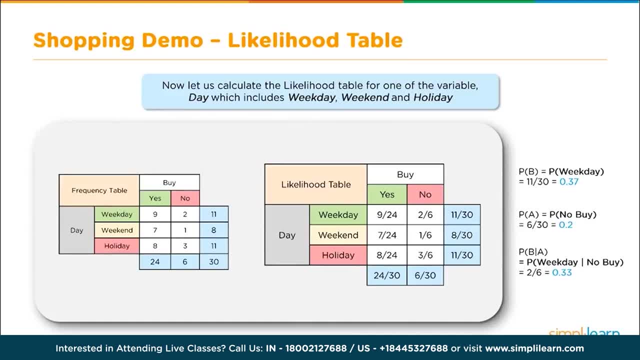 includes weekday, weekend and holiday, And let us start by summing all of our rows. So we have the weekday row and out of the weekdays there's 9 plus 2, so it's 11 weekdays. There's 8 weekend. 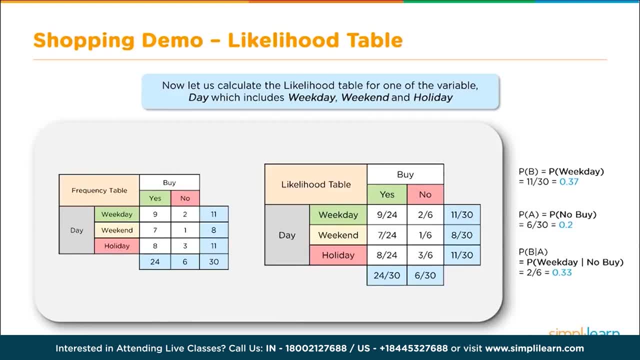 days and 11 holidays. Wow, that's a lot of holidays. And then we want to sum up the total number of days, So we're looking at a total of 30 days. Let's start pulling some information from our chart and see where that takes. 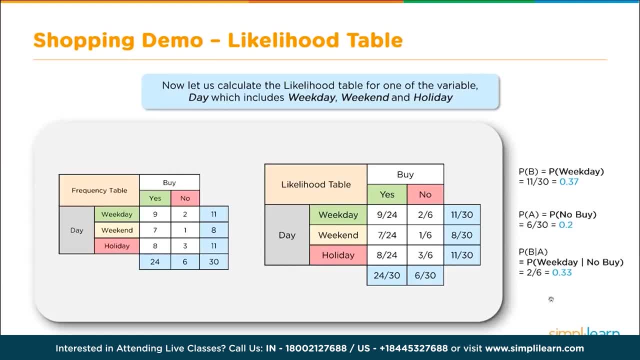 us And when we fill in the chart on the right, you can see that 9 out of 24 purchases are made on the weekday, 7 out of 24 purchases on the weekend and 8 out of 24 purchases on a holiday. 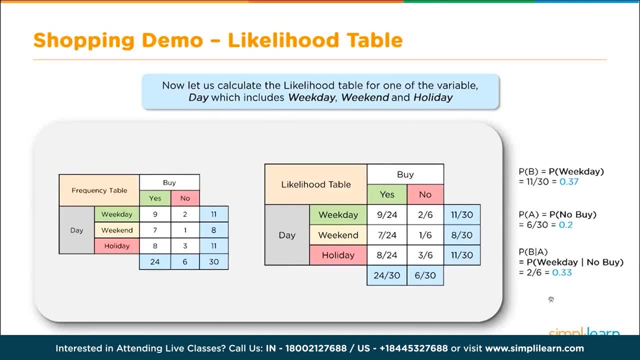 And out of all the people who come in, 24 out of 30 purchase. You can also see how many people do not purchase On the weekday: it's 2 out of 6 didn't purchase, and so on and so on. We can. 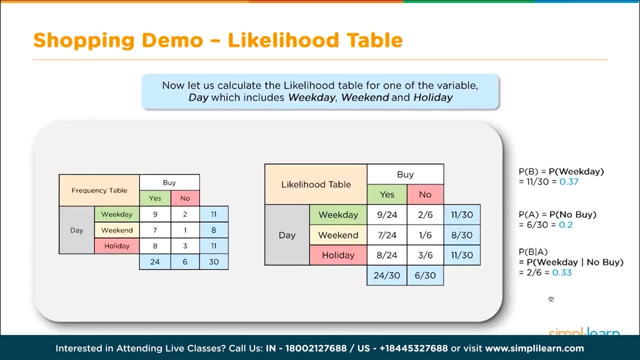 also look at the totals And you'll see. on the right we put together some of the formulas. The probability of making a purchase on the weekend comes out at 11 out of 30.. So, out of the 30 people who came into the store throughout the weekend, 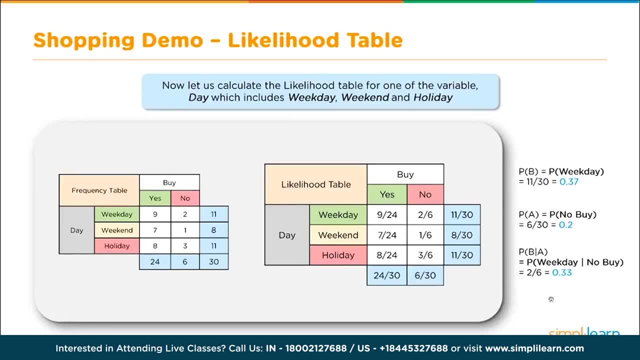 weekday and holiday. 11 of those purchases were made on the weekday, And then you can also see the probability of them not making a purchase, And this is done for it doesn't matter which day of the week, So we call that. 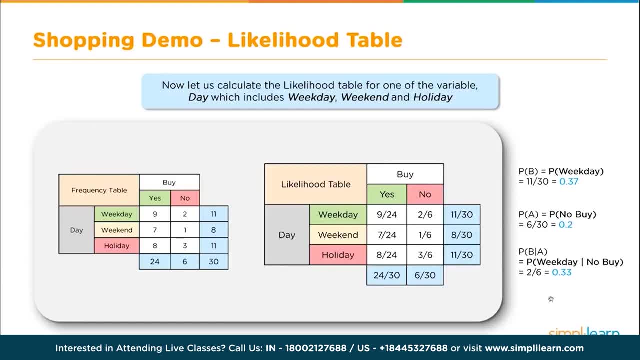 probability of no buy. It would be 6 over 30, or .2.. So there's a 20% chance that they're not going to make a purchase, no matter what day of the week it is. And finally, we look at the probability. 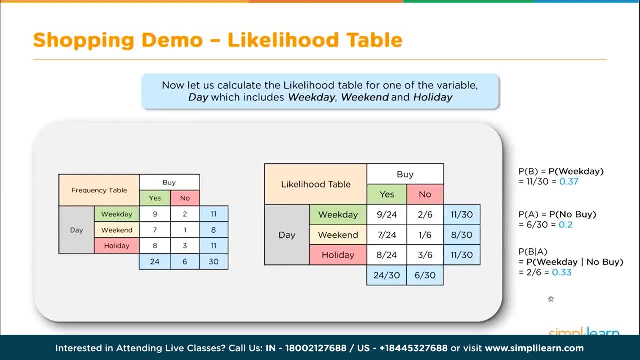 of B of A. In this case we're going to look at the probability of the weekday and not buying. Two of the no buys were done out of the weekend, out of the six people who did not make purchases. So when we look at that, the probability- 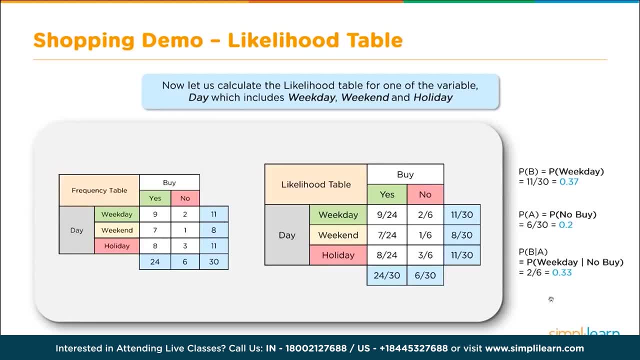 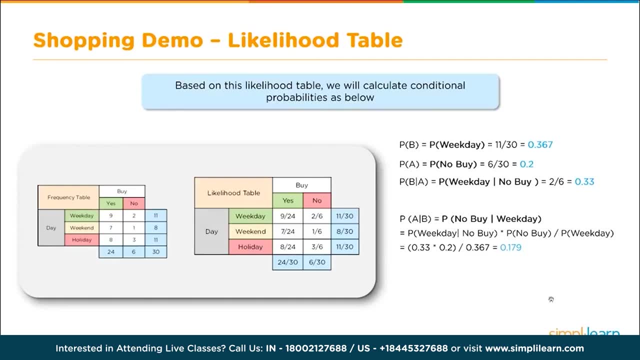 of the weekday without a purchase is going to be .33 or 33%. Let's take a look at this, at different probabilities And, based on this likelihood table, let's go ahead and calculate conditional probabilities as below The first three we just did, the probability of making. 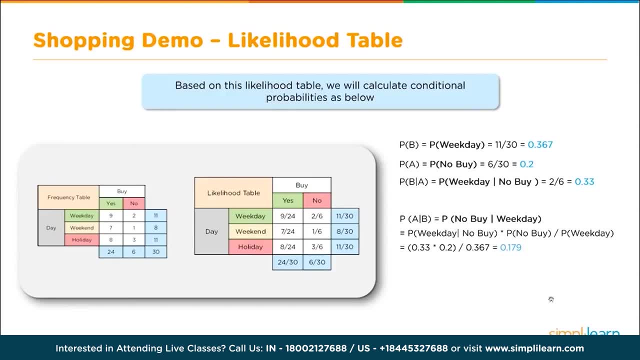 a purchase on the weekday is 11 out of 30, or roughly 36 or 37%- .367.. The probability of not making a purchase at all- it doesn't matter what day of the week- is roughly .2 or 20%, And the probability 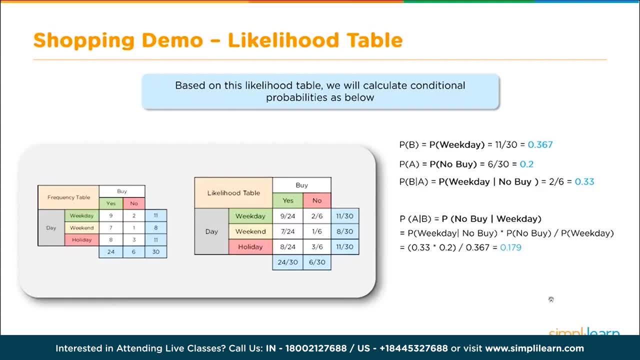 of a weekday no purchase is roughly 2 out of 6.. So 2 out of 6 of our no purchases were made on the weekday. And then, finally, we take our P of AB. If you looked, we've kept the symbols up there- We've got. 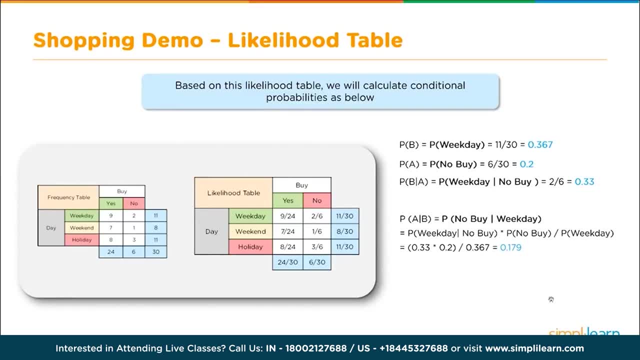 probability of B. probability of A. probability of B if A. We should remember that the probability of A if B is equal to the first one times the probability of no buys over the probability of the weekday. So we could calculate it both off the table we created. we can. 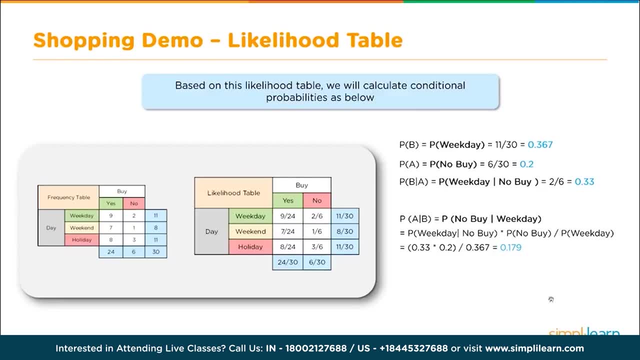 also calculate this by the formula and we get the .367, which equals or .33 times .2, over .367, which equals .179, or roughly 17 to 18%, And that would be the probability of no purchase done on the weekday, And this is 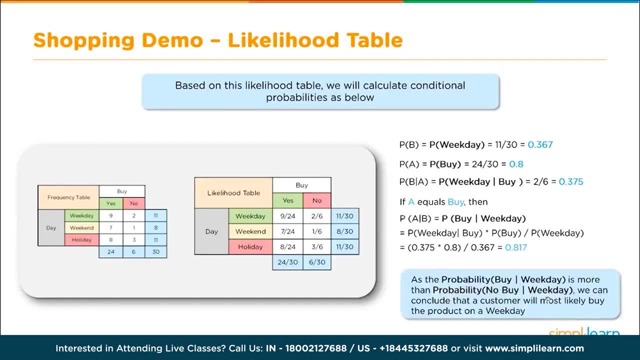 important because we can look at this and say: as the probability of buying on the weekday is more than the probability of not buying on the weekday, we can conclude that customers will most likely buy the product on a weekday. Now we've kept our chart simple and we're only looking at one. 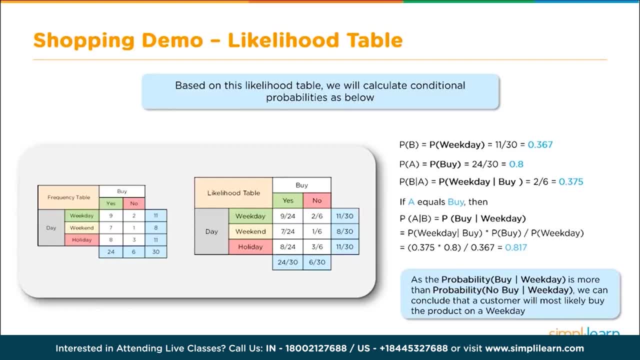 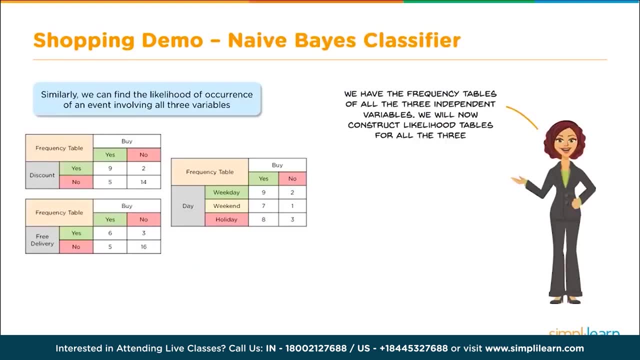 aspect. So you should be able to look at the table and come up with the same information or the same conclusion. That should be kind of intuitive at this point. Next, we can take the same setup. We have the frequency tables of all three independent. 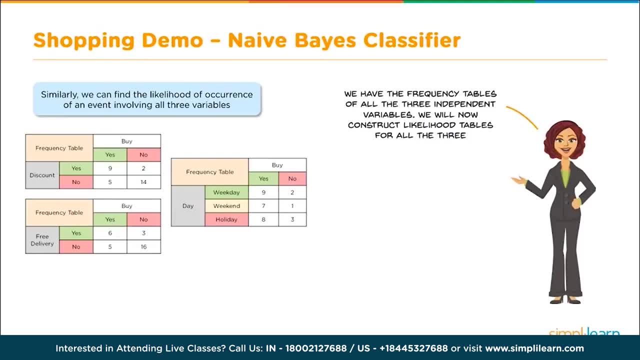 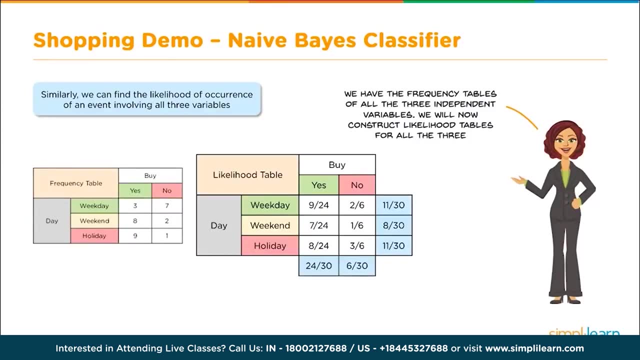 variables. Now we can construct the likelihood tables for all three of the variables we're working with. We can take our day like we did before. We have weekday, weekend and holiday. We filled in this table And then we can come in. 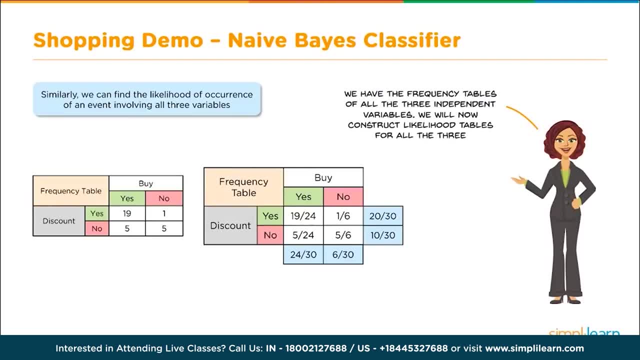 and also do that for the discount. Yes or no? Did they buy? Yes or no? We fill in that full table. So now we have our probabilities for a discount and whether the discount leads to a purchase or not, And the probability for free. 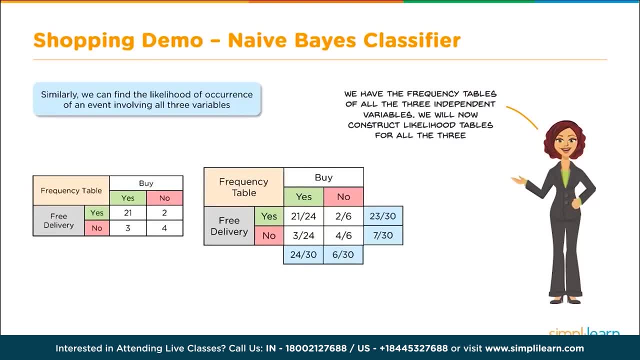 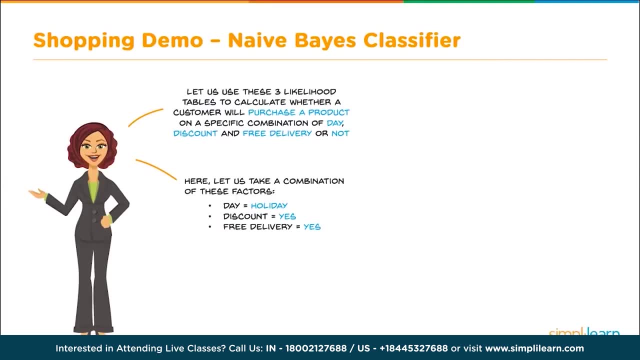 delivery. Does that lead to a purchase or not? And this is where it starts getting really exciting. Let us use these three likelihood tables to calculate whether a customer will purchase a product on a specific combination of day discount and free delivery or not purchase. Here let us take 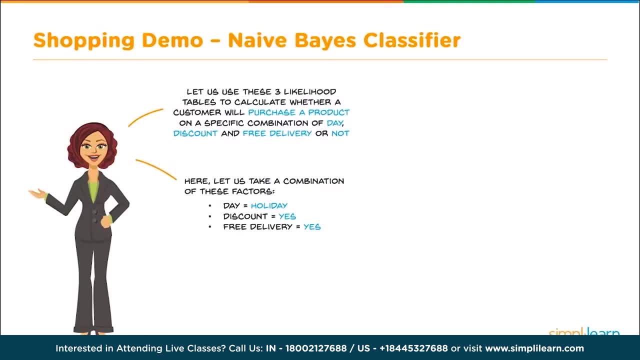 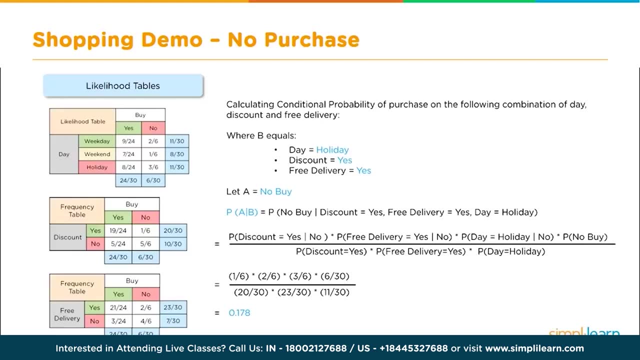 a combination of these factors: Day equals holiday. Discount equals yes. Free delivery equals yes. Let's dig deeper into the math and actually see what this looks like. We're going to start with looking for the probability of them not purchasing on the following combinations of: 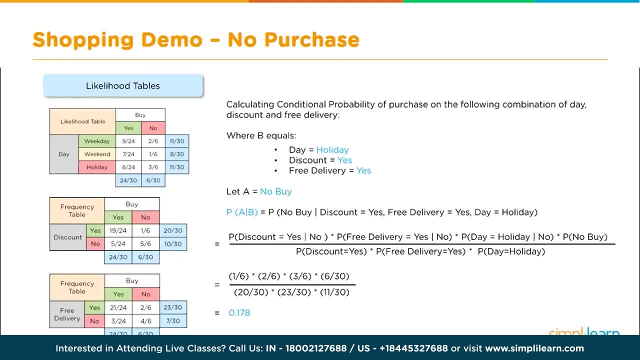 days. We're actually looking for the probability of A equals no buy, No purchase, And our probability of B we're going to set equal to. is it a holiday? Did they get a discount? Yes, And was it a free delivery? Yes? 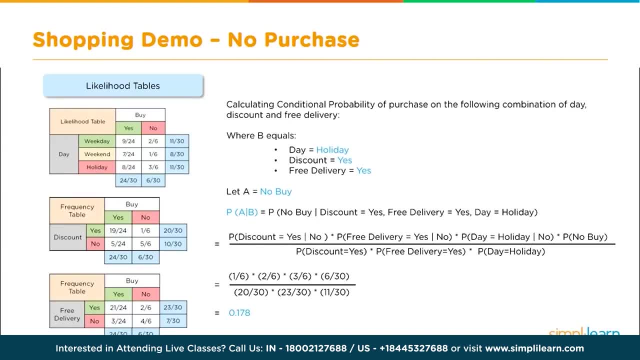 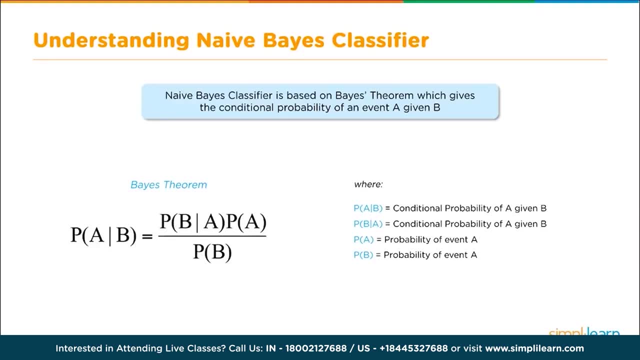 Before we go further, let's look at the original equation: The probability of A if B equals the probability of B, given the condition A and the probability times the probability of A over the probability of B occurring. Now this is basic algebra, so we can multiply this information. 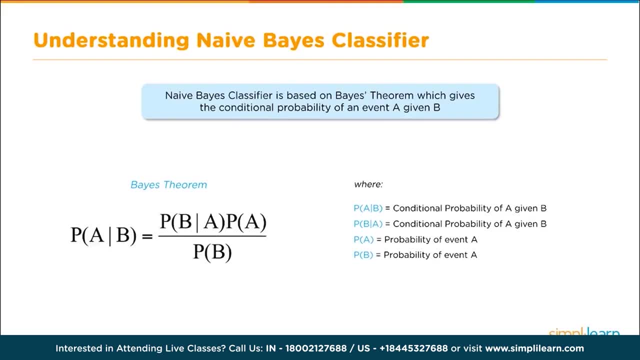 together. So when you see the probability of A given B, in this case the condition is B, C and D, or the three different variables we're looking at, And when you see the probability of B, that would be the conditions We're actually. 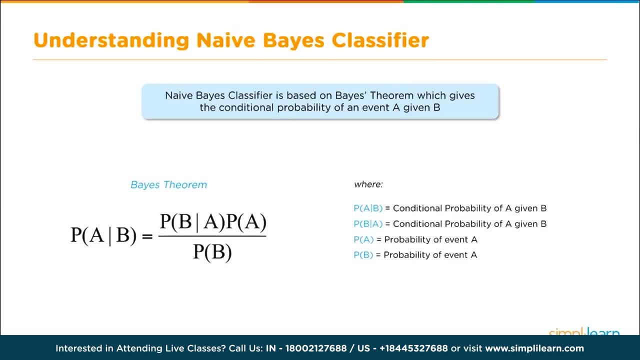 going to multiply those three separate conditions out: Probability of. you'll see that in just a second in the formula times the full probability of A over the full probability of B. So here we are back to this and we're going to have let A equal. 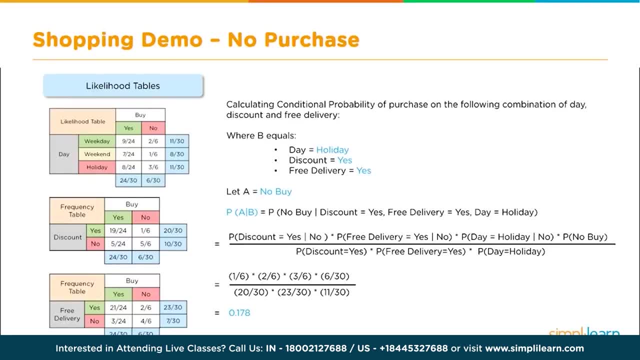 no purchase and we're looking for the probability of B on the condition A, where A sets for three different things. Remember that equals the probability of A given the condition B, And in this case we just multiply those three different variables together, So we have the probability of the. 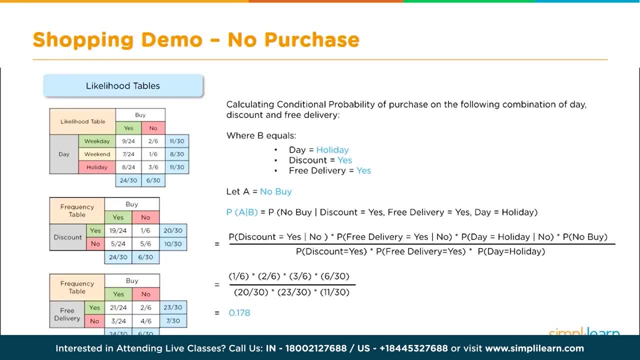 discount times, the probability of free delivery times. the probability is the day equal holiday. Those are our three variables of the probability of A, if B, And then that is going to be multiplied by the probability of them not making a purchase, And then we want to divide that by the total. 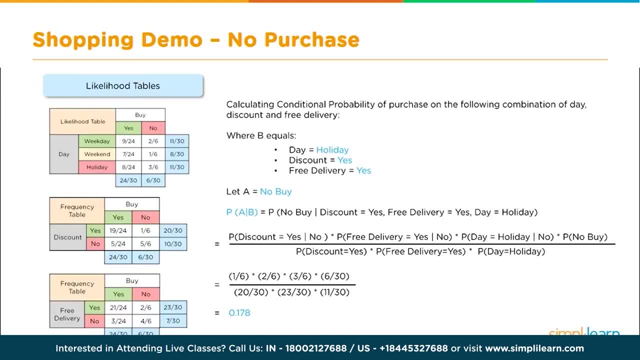 probabilities and they're multiplied together. So we have the probability of a discount, the probability of a free delivery and the probability of it being on a holiday. When we plug those numbers in, we see that one out of six were no purchase on a discounted day. 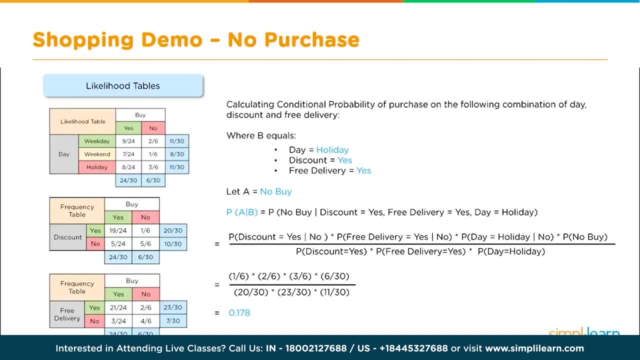 two out of six were no purchase on a free delivery day and three out of six were no purchase on a holiday. Those are our three probabilities of A if B multiplied out, And then that has to be multiplied by the probability of a no purchase. And remember the. 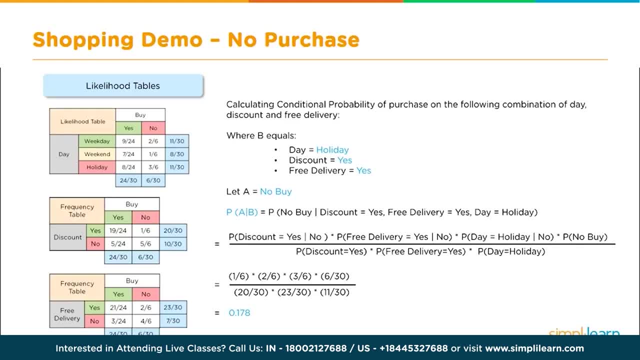 probability of a no buy is across all the data. So that's where we get the six out of thirty. We divide that out by the probability of each category over the total number, So we get the twenty out of thirty had a discount. twenty-three out of thirty. 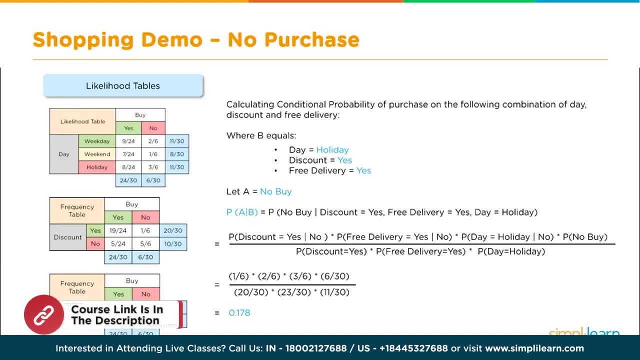 had a yes for free delivery and eleven out of thirty were on a holiday. We plug all those numbers in, we get .178.. So in our probability math we have a .178 if it's a no- buy for a holiday, a discount and a free delivery. 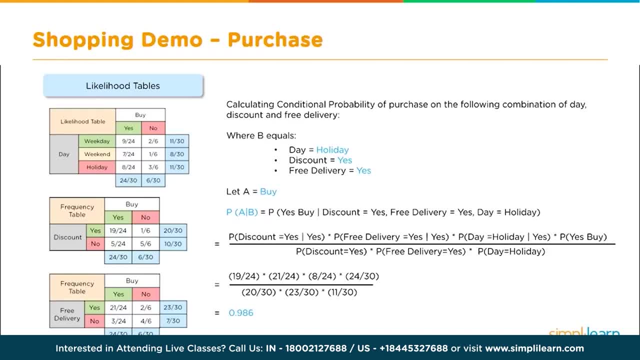 Let's turn that around and see what that looks like if we have a purchase. I promise this is the last page of math before we dig into the Python script. So here we're, calculating the probability of the purchase using the same math we did to find out if they. 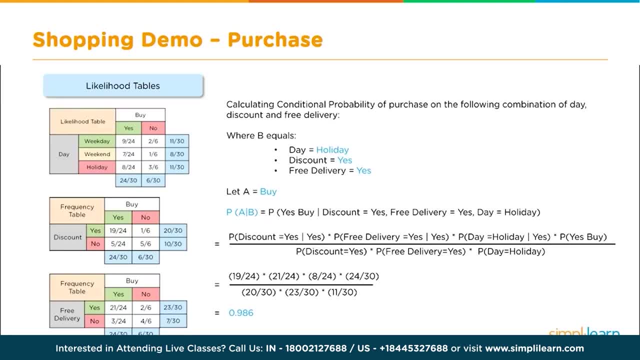 didn't buy. Now we want to know if they did buy. And again we're going to go by the day: equals a holiday discount equals yes, free delivery equals yes. and let A equal buy. Now, right about now. you might be asking: why are we doing both? 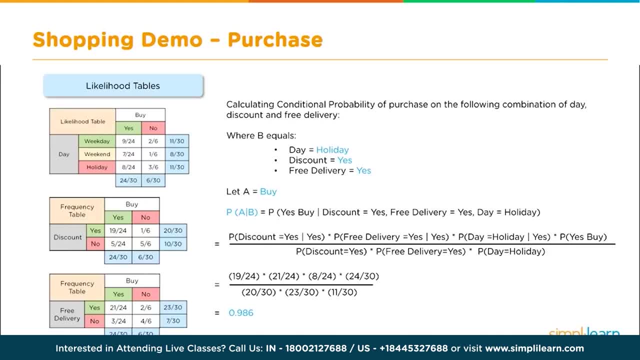 calculations. Why would we want to know the no buys and buys for the same data going in? Well, we're going to show you that in just a moment, but we have to have both of those pieces of information so that we can figure it out as a percentage as opposed. 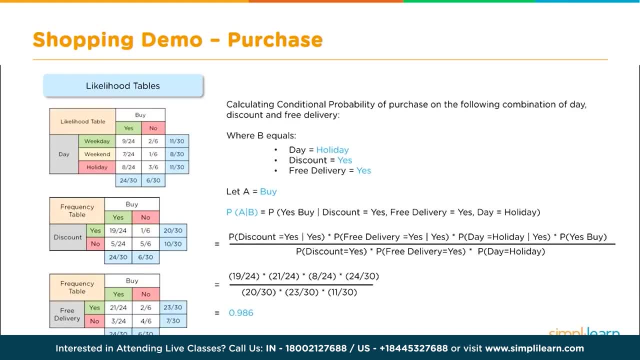 to a probability equation And we'll get to that normalization here in just a moment. Let's go ahead and walk through this calculation And, as you can see here, the probability of A on the condition of B, B being all three categories. 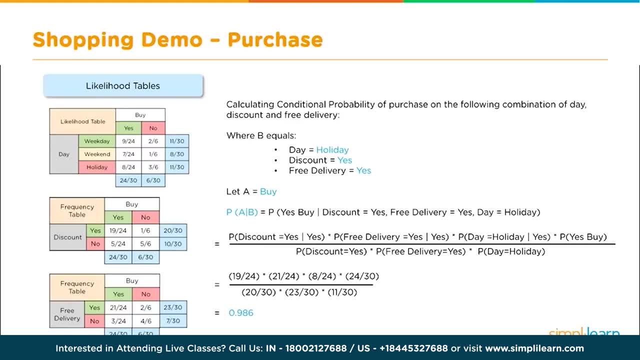 did we have a discount with a purchase? Did we have a free delivery with a purchase? And is a day equal to holiday, And when we plug this all into that formula and multiply it all out, we get our probability of a discount, probability of. 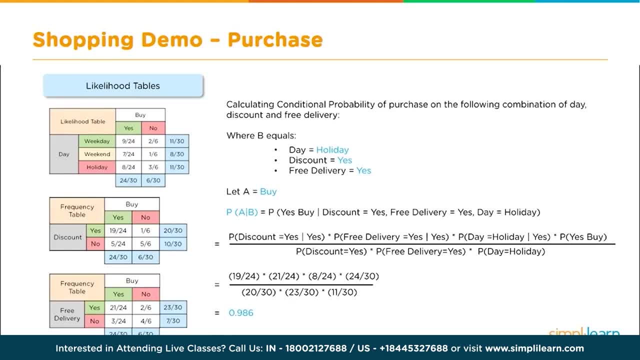 a free delivery. probability of the day being a holiday times. the overall probability of it being a purchase, divided by again multiplying the three variables out: the full probability of there being a discount, the full probability of being a free delivery and the full probability of there. 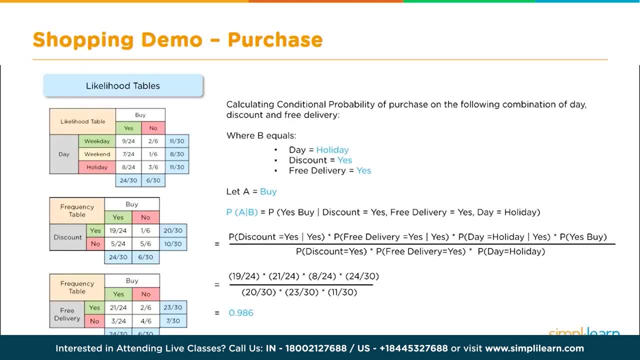 being a day equal holiday, And that's where we get this: 19 over 24 times 21 over 24 times 8 over 24 times the P of A 24 over 30 divided by the probability of the discount, the free delivery. 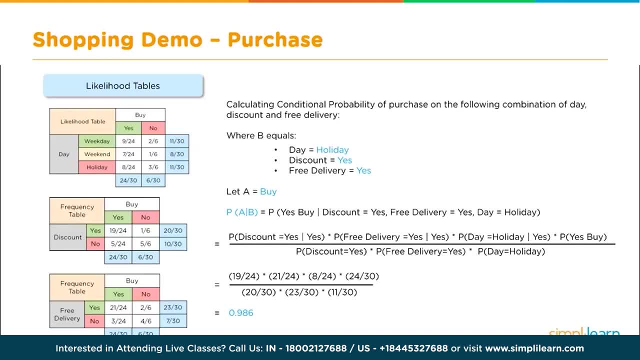 times the day, or 20 over 30,, 23 over 30 times 11 over 30,, and that gives us our .986.. So what are we going to do with these two pieces of data we just generated? Well, let's go ahead and go over them. 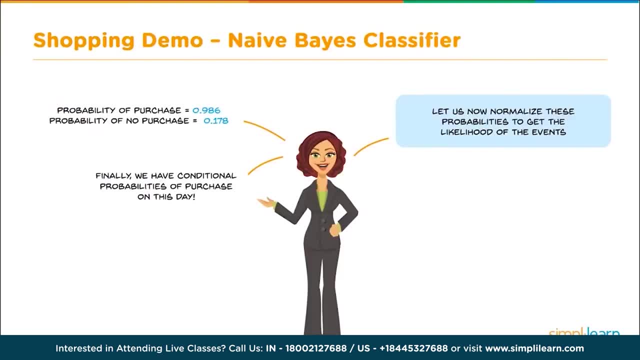 We have a probability of purchase equals .986.. We have a probability of no purchase equals .178.. So, finally, we have a conditional probability of purchase on this day. Let us take that we're going to normalize it and we're going to take these probabilities and turn. 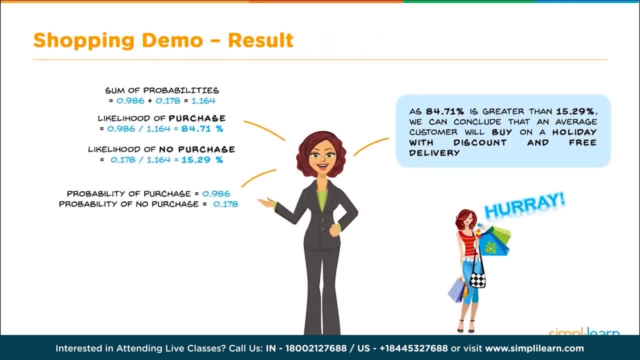 them into percentages. This is simply done by taking the sum of probabilities, which equals .986 plus .178, and that equals the 1.164.. If we divide each probability by the sum, we get the percentage, And so the likelihood of a purchase. 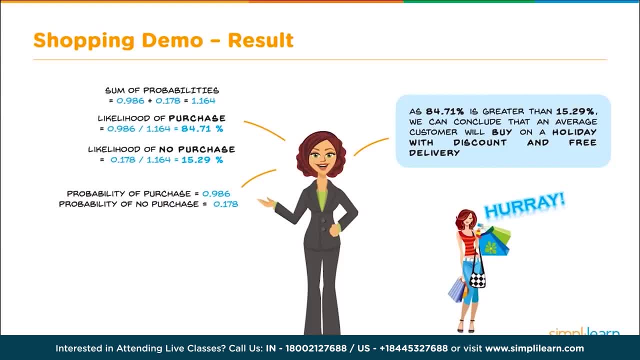 is 84.71% and the likelihood of no purchase is 15.29%, Given these three different variables. So if it's on a holiday, if it's with a discount and has free delivery, then there's an 84.71% chance that the 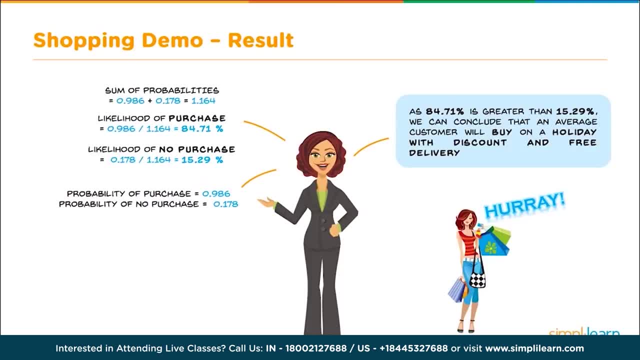 customer is going to come in and make a purchase. Hooray, They purchased our stuff, We're making money. If you're owning a shop that's like is, the bottom line is you want to make some money so that you can keep your shop open and have a living. 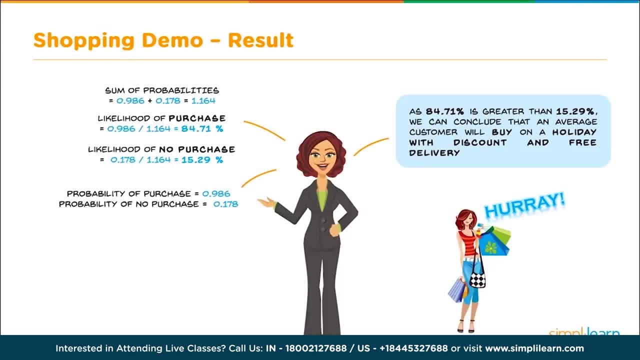 Now I promised you that we were going to be finishing up the math here with a few pages, So we're going to move on and we're going to do two steps. The first step is: I want you to understand why you want to use the. 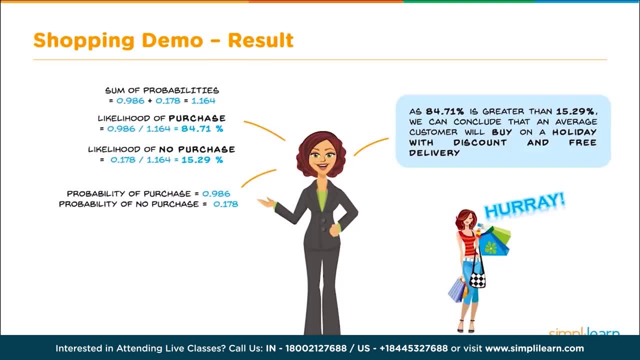 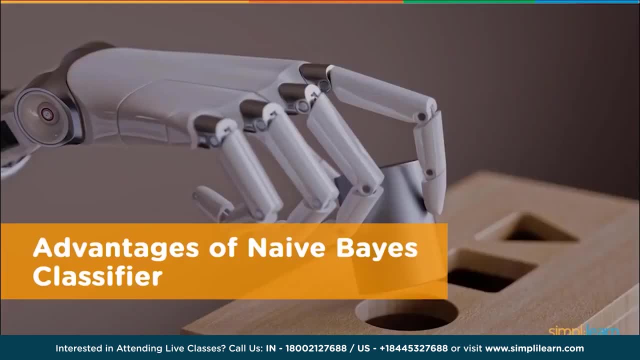 Naive Bayes. What are the advantages of Naive Bayes? And then, once we understand those advantages, we'll just look at that briefly. then we're going to dive in and do some Python coding. Advantages of Naive Bayes- Classifier. 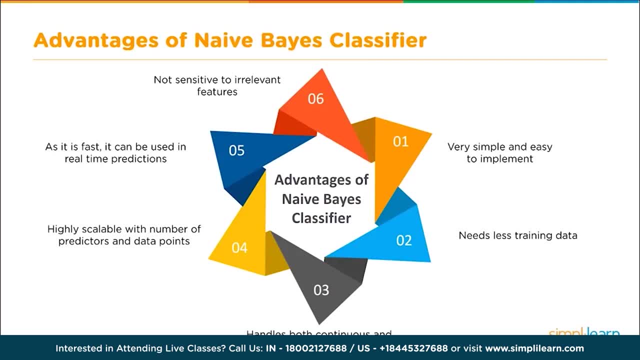 So let's take a look at the six advantages of the Naive Bayes Classifier And we're going to walk around this lovely wheel. It looks like an origami folded paper. The first one is very simple and easy to implement. Certainly you. 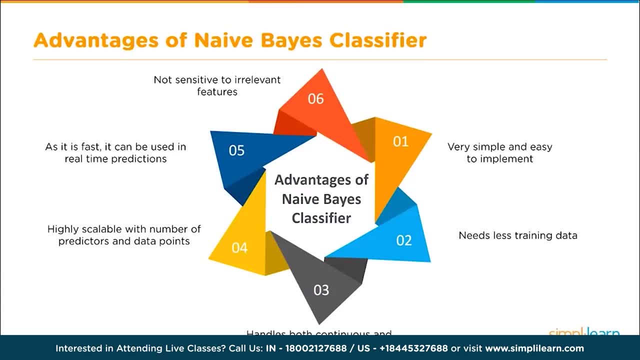 could walk through the tables and do this by hand. You've got to be a little careful, because the notations can get confusing. You have all these different probabilities and I certainly mess those up as I put them on. you know, is it on the top or the bottom? 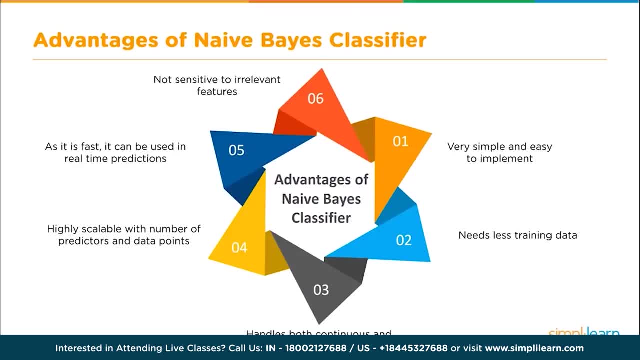 You've got to really pay close attention to that. When you put it into Python. it's really nice because you don't have to worry about any of that. You let the Python handle that, the Python module. But, understanding it, you can put it on a table. 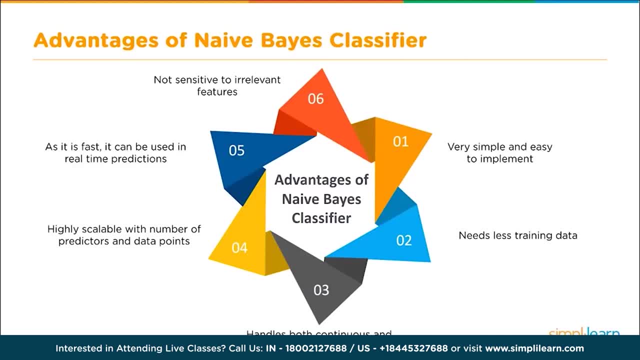 and you can easily see how it works. and it's a simple algebraic function. It needs less training data. so if you have smaller amounts of data, this is a great powerful tool for that Handles both continuous and discrete data. It's highly. 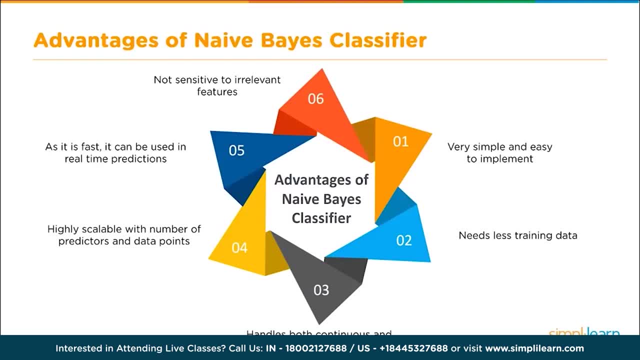 scalable with number of predictors and data points. So, as you can see, you just keep multiplying different probabilities in there and you can cover not just three different variables or sets. You can now expand this to even more categories. Number five, it's fast. 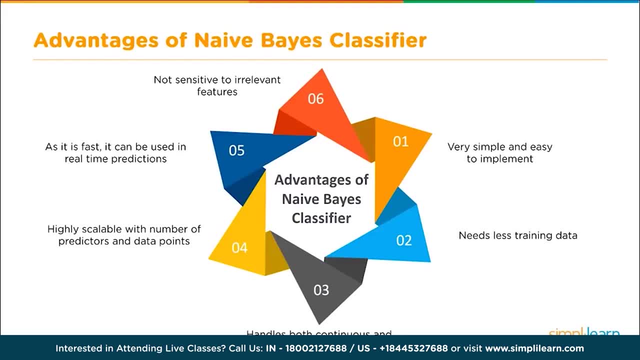 It can be used in real-time predictions. This is so important. This is why it's used in a lot of our predictions on online shopping carts, referrals, spam filters is because there's no time delay as it has to go through and figure out. 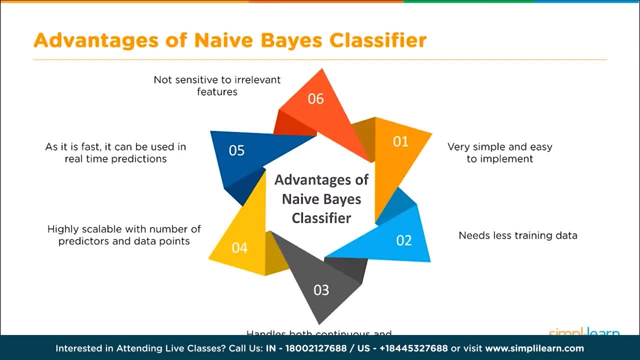 a neural network or one of the other mini setups where you're doing classification. And certainly there's a lot of other tools out there in the machine learning that can handle these, but most of them are not as fast as the Naive Bayes. 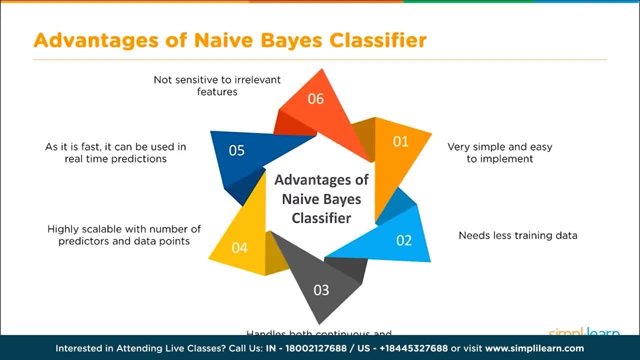 And then finally, it's not sensitive to irrelevant features. So it picks up on your different probabilities, and if you're short on data on one probability, you can kind of automatically adjust for that. Those formulas are very automatic, and so you can still get. 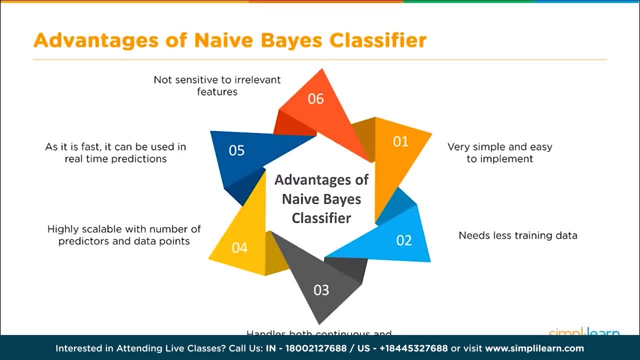 a very solid predictability, even if you're missing data or you have overlapping data for two completely different areas. We see that a lot in doing census and studying of people and habits, where they might have one study that covers one aspect and another one that overlaps, and because 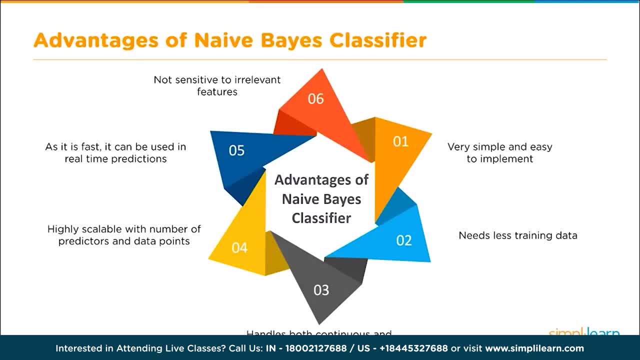 the two overlap. they can then predict the unknowns for the group that they haven't done the second study on, or vice versa. So it's very powerful in that it is not sensitive to the irrelevant features and in fact you can use it to help. 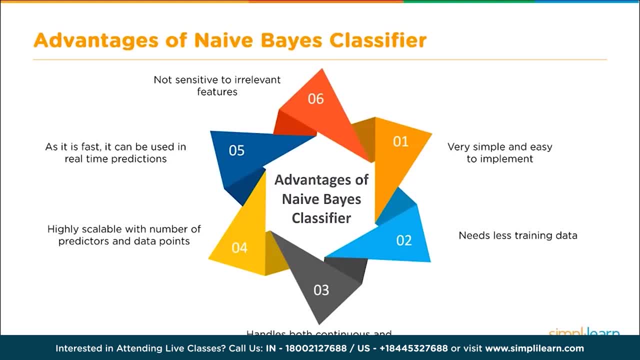 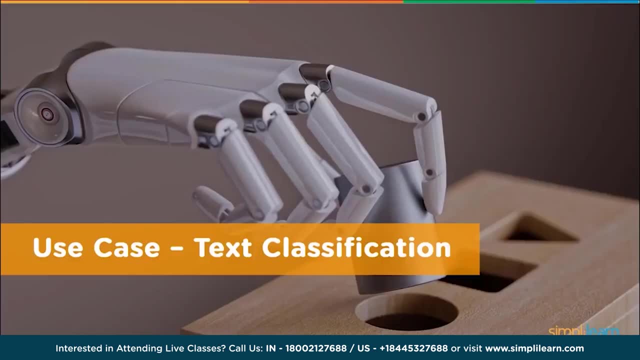 predict features that aren't even in there. So now we're down to my favorite part. We're going to roll up our sleeves and do some actual programming. We're going to do the use case text classification. Now I would challenge you to go back and send. 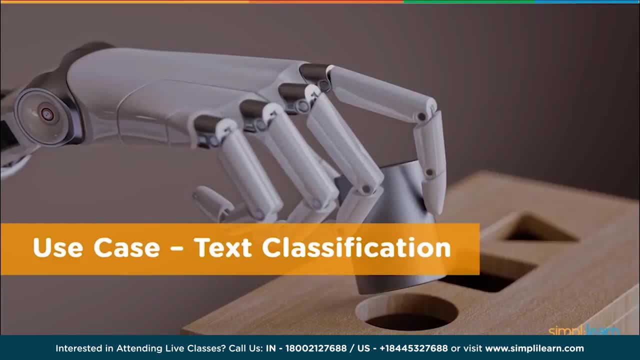 us a note on the notes below underneath the video and request the data for the shopping cart. So you can plug that into Python code and do that on your own time so you can walk through it, since we walked through all the information on it, But we're going to do a Python code. 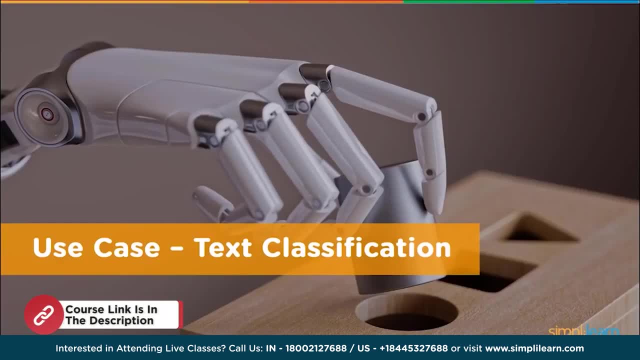 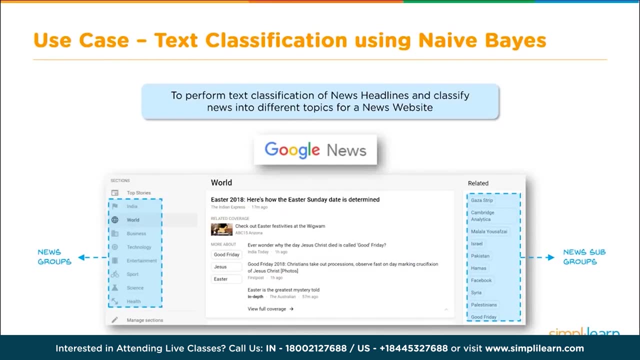 doing text classification- very popular for doing the naive bays. So we're going to use our new tool to perform a text classification of news headlines and classifications to classify news into different topics for a news website. As you can see here, we have a nice image of the Google News. 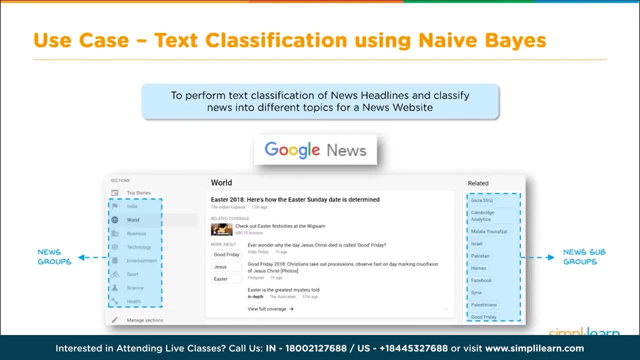 and then related on the right subgroups. I'm not sure where they actually pulled the actual data we're going to use from. It's one of the standard sets, But certainly this can be used on any of our news headlines and classification. So let's see how it can be done using 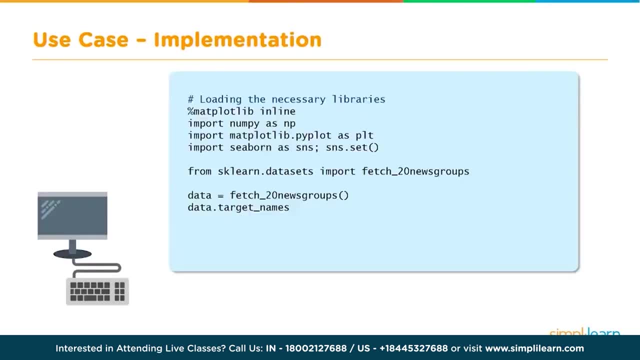 the naive bays classifier. Now we're at my favorite part. We're actually going to write some Python script, Roll up our sleeves And we're going to start by doing our imports. These are very basic imports, including our news group. We'll take a quick glance at the target. 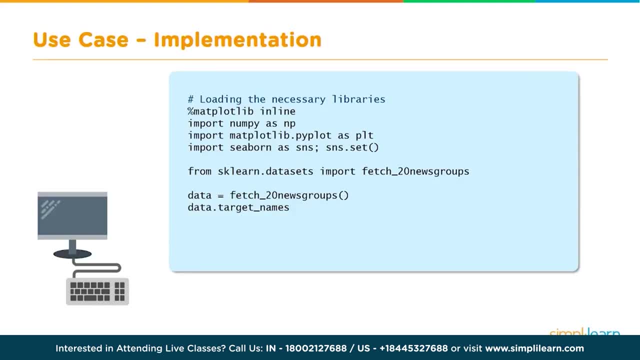 names, Then we're going to go ahead and start training our data set and putting it together. We'll put together a nice graph, because it's always good to have a graph to show what's going on. And once we've trained it and we've shown you a graph of what's going on, 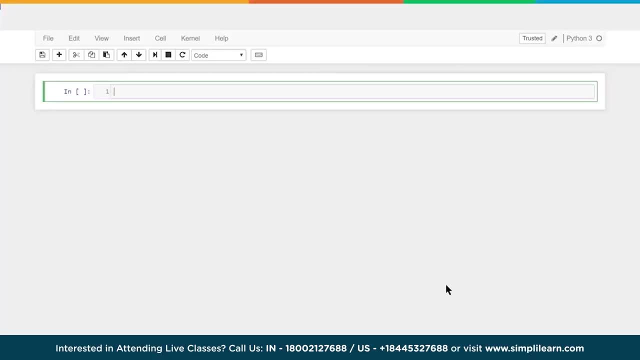 then we're going to explore how to use it and see what that looks like. Now I'm going to open up my favorite editor or inline editor for Python. You don't have to use this. You can use whatever your editor that you like, whatever interface. 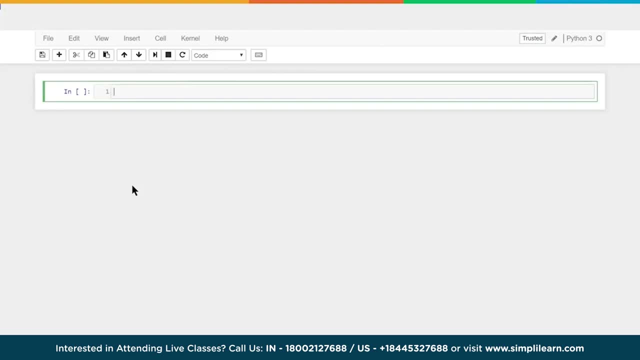 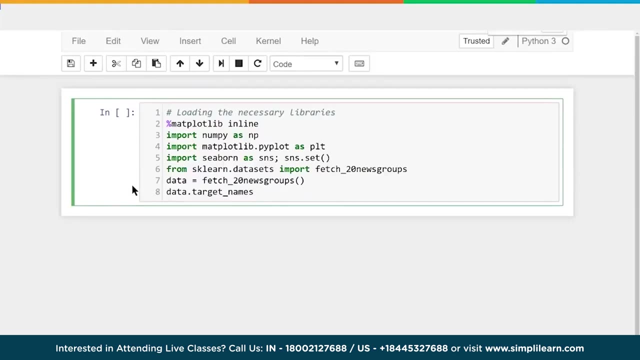 IDE you want. This just happens to be the Anaconda Jupyter notebook And I'm going to paste that first piece of code in here so we can walk through it. Let's make it a little bigger on the screen so you have a nice view of what's going on. 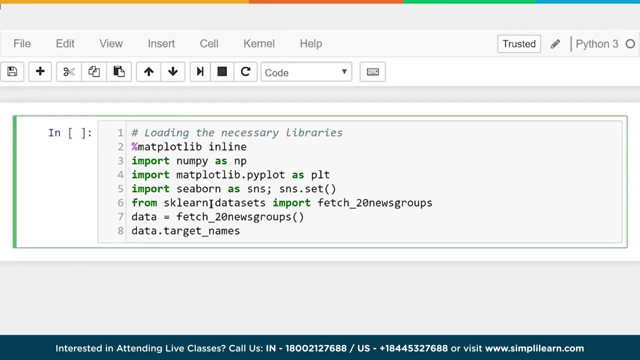 And we're using Python 3, in this case 3.5. So this would work in any of your 3x. If you have it set up correctly, it should also work in a lot of the 2x. You just have to make sure. 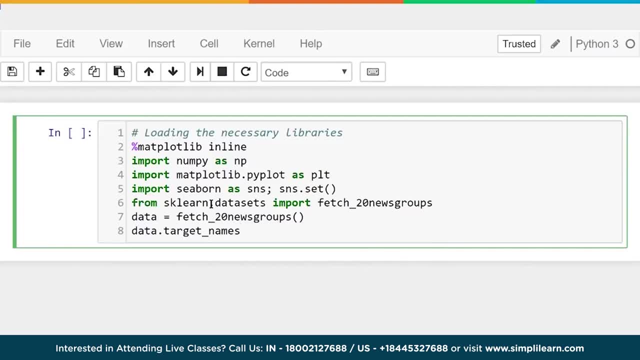 all of the versions of the modules match your Python version And in here you'll notice. the first line is your percentage matplotlibrary inline. Now three of these lines of code are all about plotting the graph. This one lets the notebook know, since this is an inline setup, that we 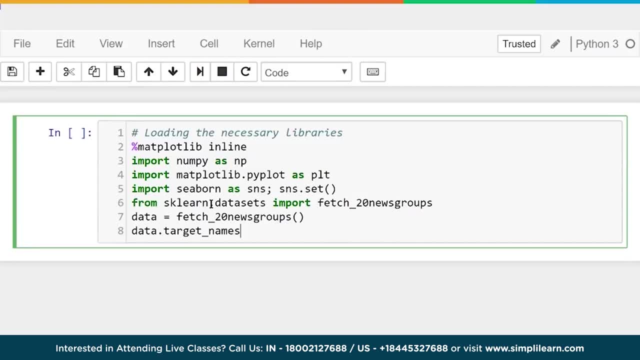 want the graphs to show up on this page. Without it, in a notebook like this, which is an explorer interface, it won't show up. Now, a lot of IDEs don't require that. A lot of them like if I'm working. 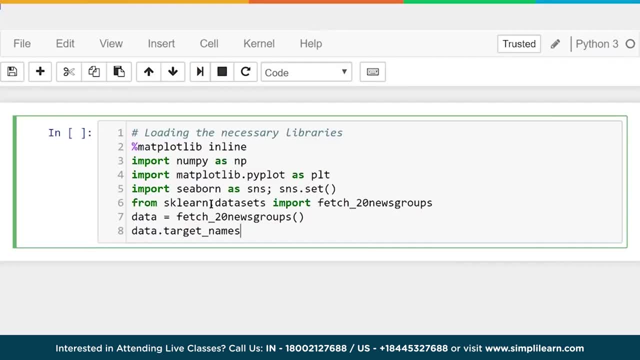 on one of my other setups. it just has a popup and the graph pops up on there. So you have that setup also. But for this we want the matplotlibrary inline, And then we're going to import numpy as np, That's number Python, which has 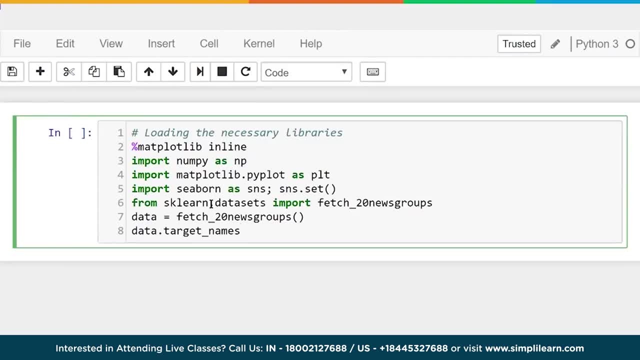 a lot of different formulas in it that we use for both of our sklearn module And we also use it for any of the upper math functions in Python And it's very common to see that as np, numpy as np. The next two lines are all about: 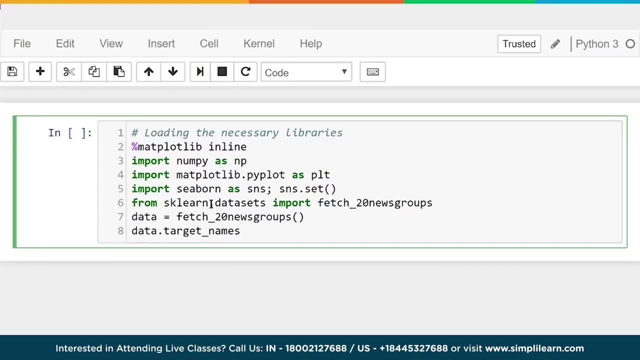 our graphing. Remember, I said three of these were about graphing. Well, we need our matplotlibrarypyplot as plt, And you'll see that plt is a very common setup, as is the sns, and just like the np, And we're going to. 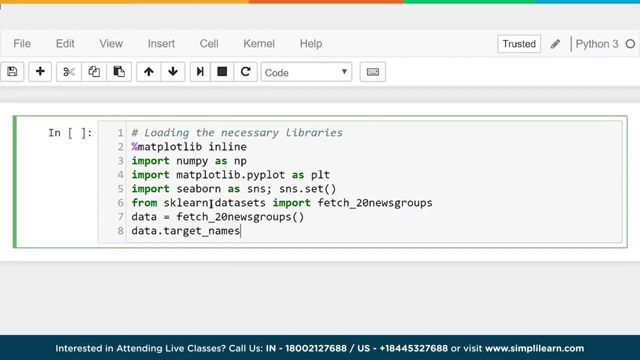 import seaborn as sns And we're going to do the snsset Now. seaborn sits on top of pyplot and it just makes a really nice heatmap. It's really good for heatmaps And if you're not familiar with heatmaps, that just means we give it a color. 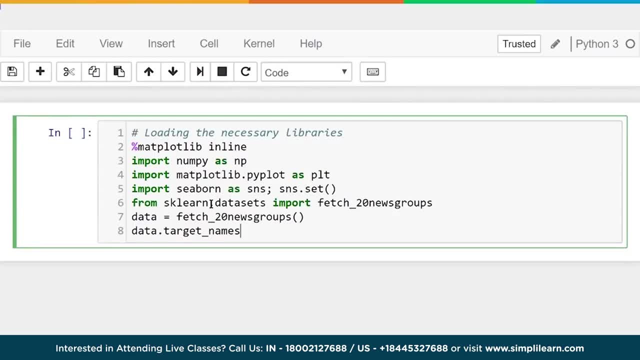 scale, The term comes from the brighter red, it is the hotter. it is in some form of data And you can set it to whatever you want And we'll see that later on. So you'll see that those three lines of code here are just. 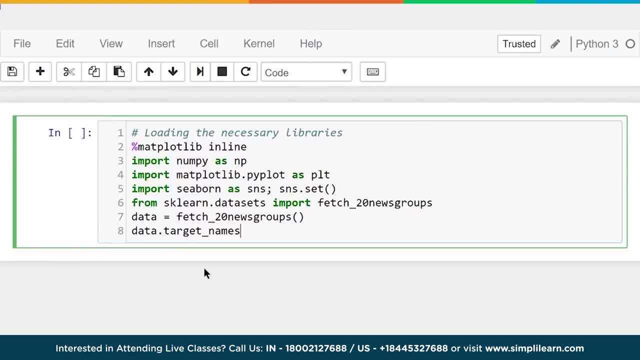 importing the graph function so we can graph it. And as a data scientist you always want to graph your data and have some kind of visual. It's really hard just to shove numbers in front of people and they look at it and it doesn't mean anything. And then from the 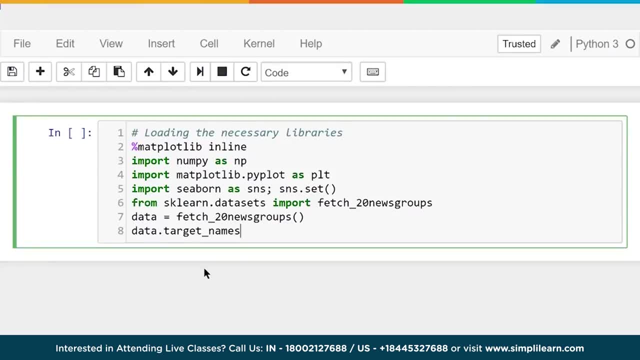 sklearndatasets. we're going to import the fetch20newsgroups- Very common one- for analyzing, tokenizing words and setting them up and exploring how the words work and how do you categorize different things when you're dealing with documents. And then we set 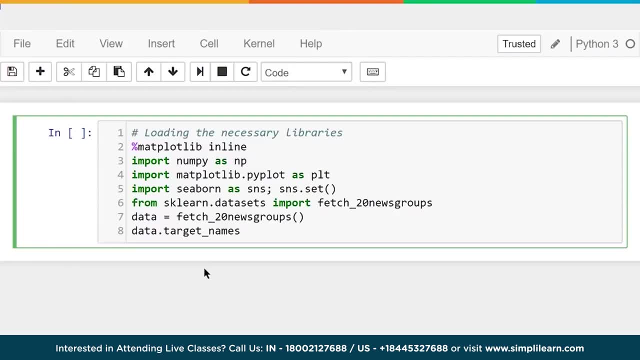 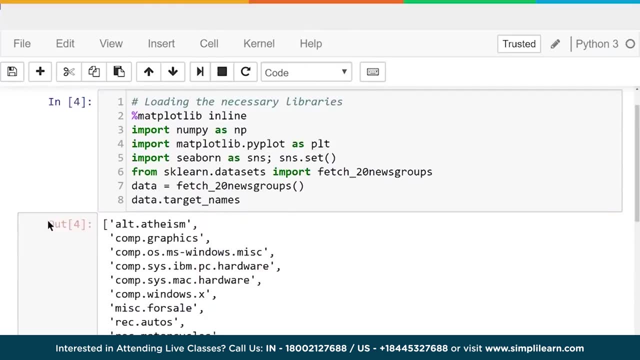 our data equal to fetch20newsgroups, So our data variable will have the data in it And we're going to go ahead and just print the target names- Datatargetnames- And let's see what that looks like And you'll see here we. 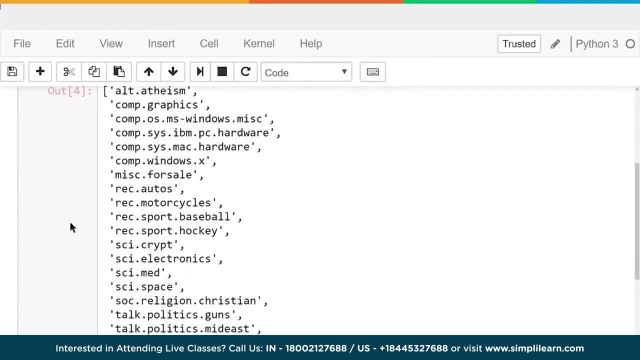 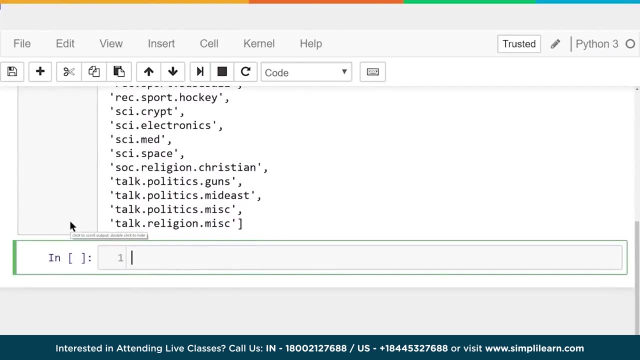 have alt atheism, comp graphics, comp os, ms, windowsmiscellaneous, And it goes all the way down to talkpoliticsmiscellaneous, talkreligionmiscellaneous. These are the categories they've already assigned to this newsgroup And it's called 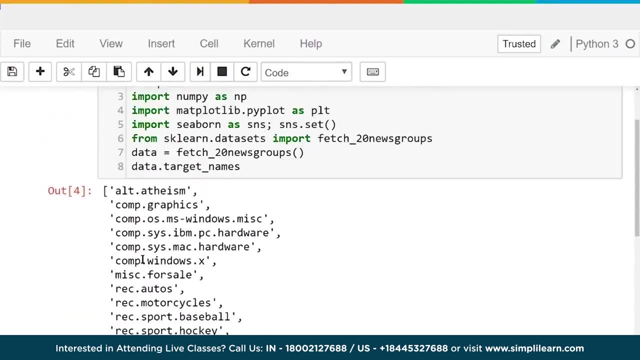 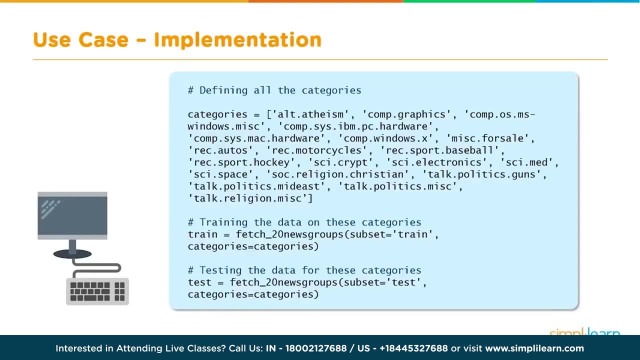 fetch20, because you'll see, I believe there's 20 different topics in here, or 20 different categories as we scroll down. Now we've gone through the 20 different categories and we're going to go ahead and start defining all the categories and set up our data, So we're 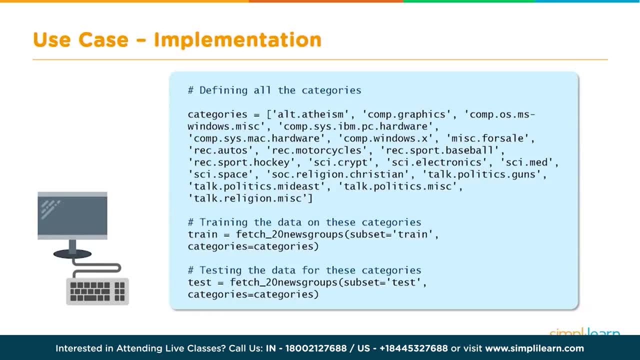 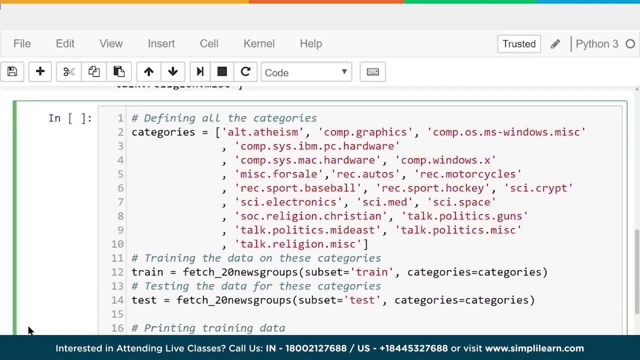 actually in here, going to go ahead and get the data all set up and take a look at our data, And let's move this over to our Jupyter notebook And let's see what this code does. First, we're going to set our categories. Now 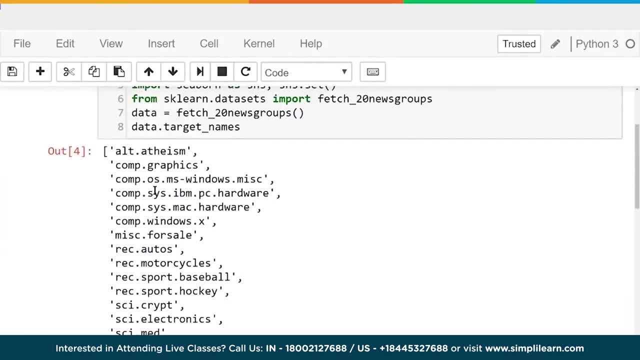 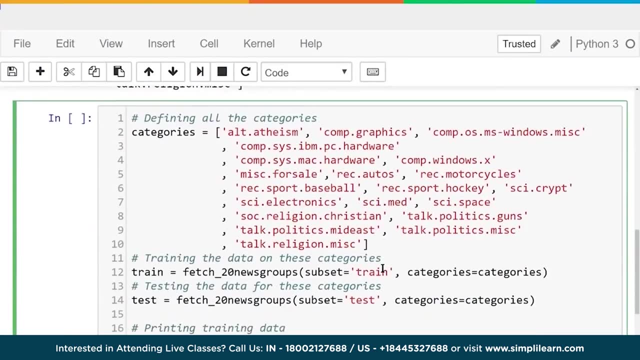 if you noticed up here, I could have just as easily set this equal to datatarget underscore names, because it's the same thing. But we want to kind of spell it out for you so you can see the different categories. It kind of makes it more. 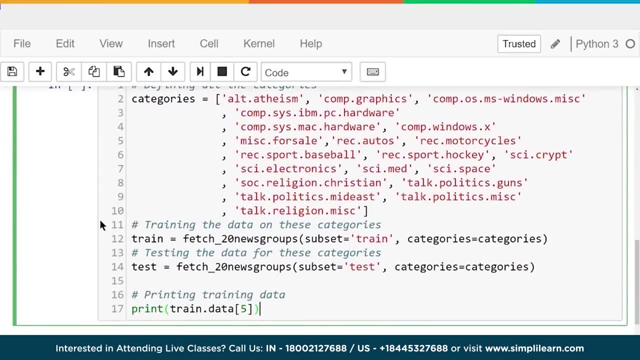 visual so you can see what your data is looking like. in the back, Once we've created the categories, we're going to open up a train set. So this training set of data is going to go into fetch20 newsgroups and it's a subset in there called train. 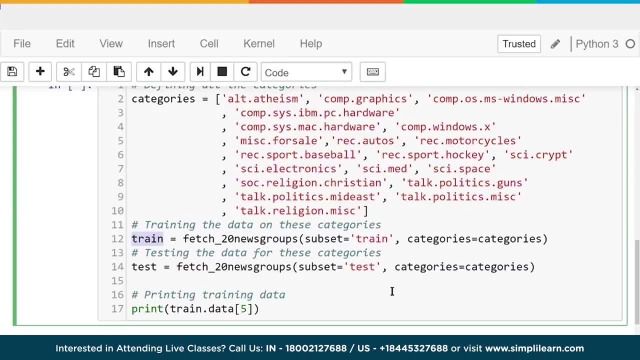 And categories equals categories. So we're pulling out those categories that match And then if you have a train set, you should also have the testing set. We have test equals fetch20, newsgroups, subset equals test and categories equals categories. Let's go down one size. 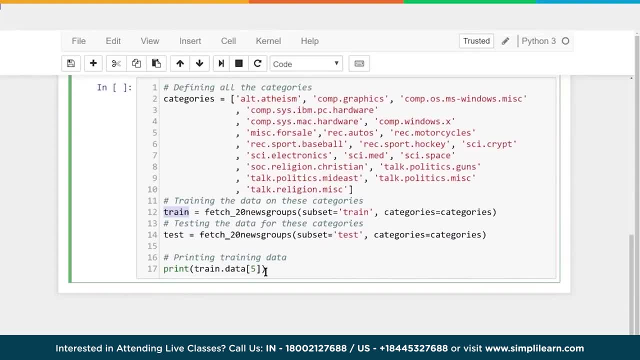 so it all fits on my screen. There we go, And just so we can really see what's going on. let's see what happens when we print out one part of that data. So it creates train and under train it creates traindata, And we're just going to look. 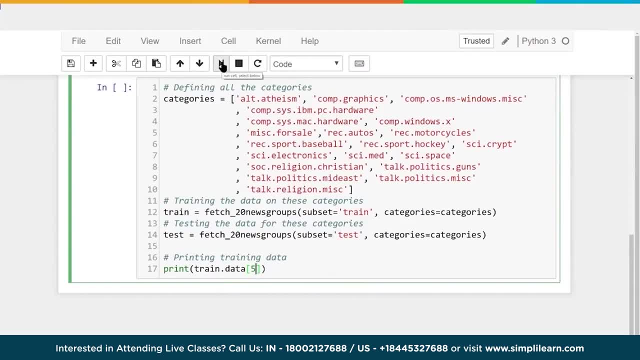 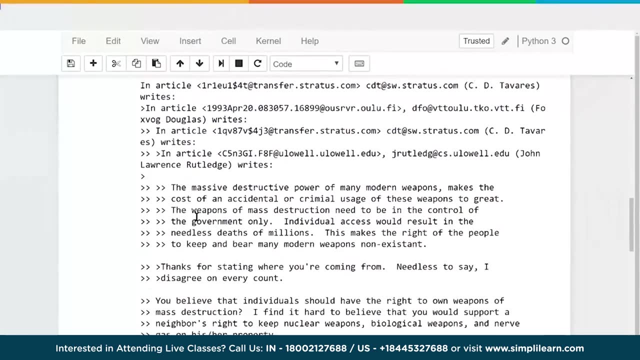 at data piece number 5.. And let's go ahead and run that and see what that looks like. And you can see, when I print traindata number 5 under train, it prints out one of the articles. This is article number 5.. 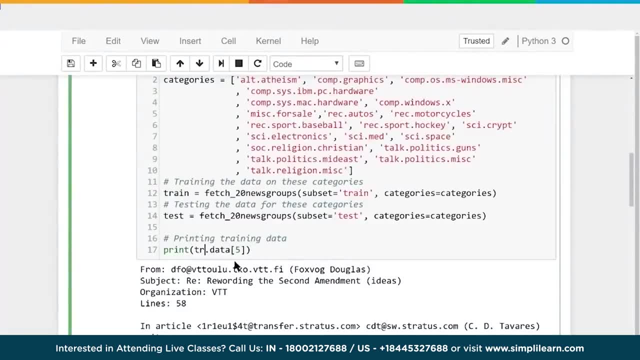 You can go through and read it on there And we can also go in here and change this to test, which should look identical because it's splitting the data up into different groups. train and test And we'll see. test number 5 is: 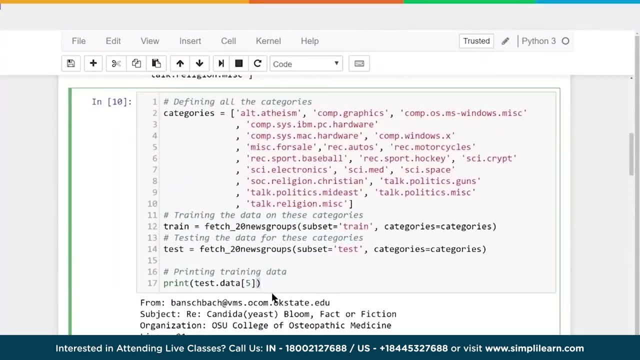 a different article but it's another article in here And maybe you're curious and you want to see just how many articles are in here. We could do length of train dot data And if we run that you'll see that the training data has. 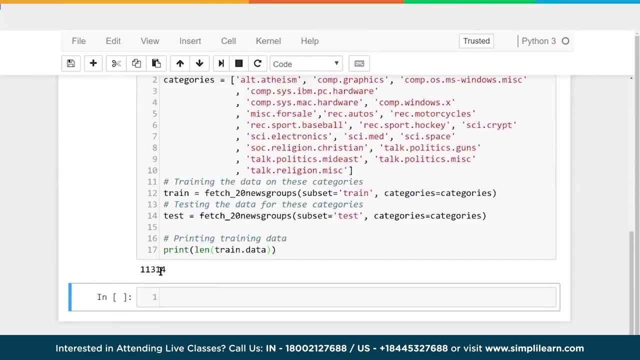 11,314 articles, So we're not going to go through all those articles. That's a lot of articles, But we can look at one of them just so you can see what kind of information is coming out of it and what we're. 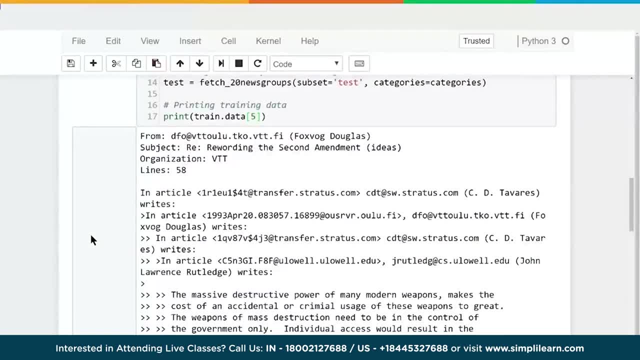 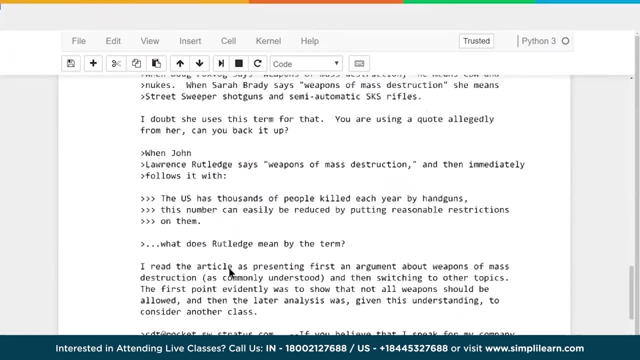 looking at- And we'll just look at number 5 for today. And here we have it, rewording the Second Amendment: IDs VTT, line 58, lines 58 in article, etc. And you can scroll all the way down and see all the different parts. 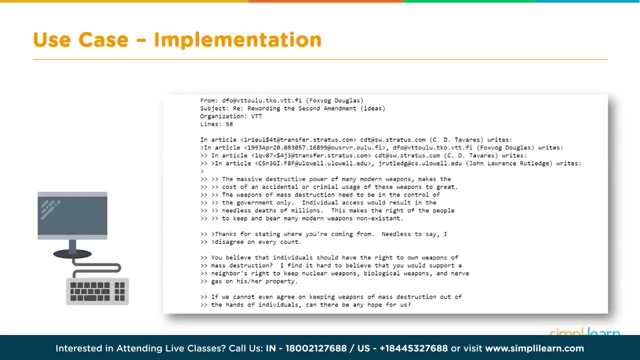 to there. Now, we've looked at it and that's pretty complicated when you look at one of these articles to try to figure out how do you weight this? If you look down here, we have different words and maybe the word from, Well from, is probably in all the articles. 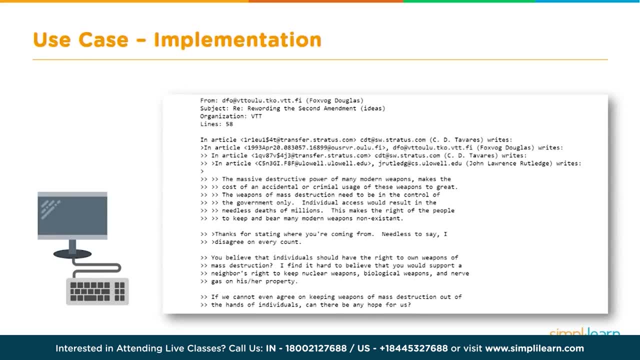 so it's not going to have a lot of meaning as far as trying to figure out whether this article fits one of the categories or not. So trying to figure out which category it fits in based on these words is where the challenge comes in. Now that we've viewed 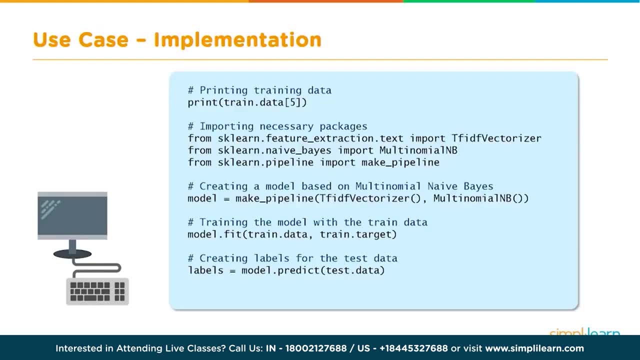 our data, we're going to dive in and do the actual predictions. This is the actual naive base And we're going to throw another model at you or another module at you here in just a second. We can't go into too much detail, but it deals specifically. 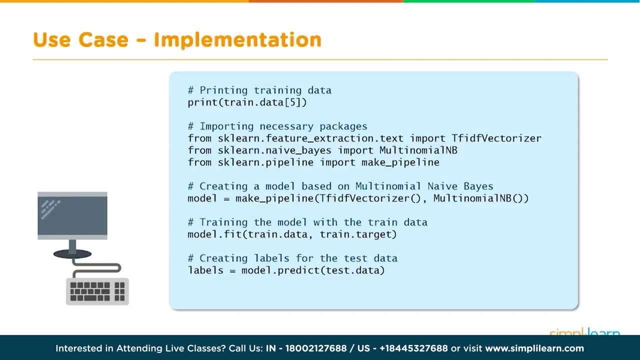 working with words and text and what they call tokenizing those words. So let's take this code and let's skip on over to our Jupyter Notebook and walk through it. And here we are in our Jupyter Notebook. Let's paste that in there, And I can. 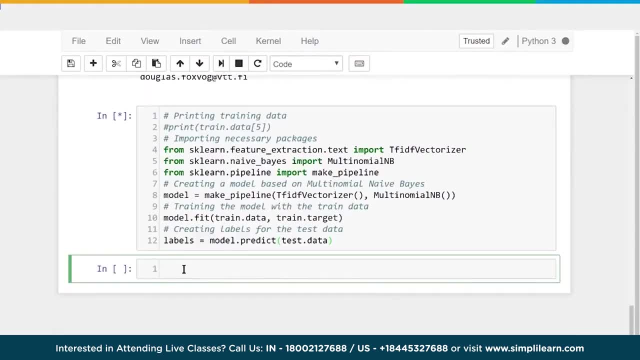 run this code right off the bat. It's not actually going to display anything yet, But it has a lot going on in here. So the top. we have the print module from the earlier one. I didn't know why that was in there. 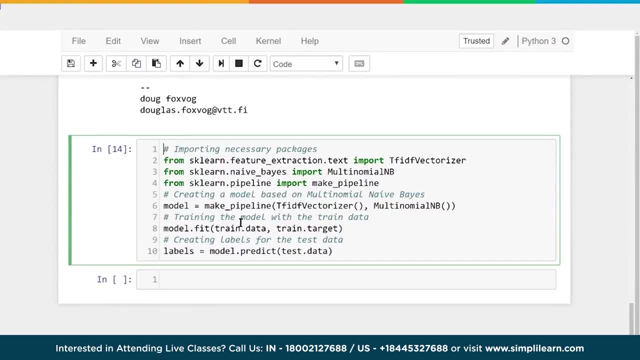 So we're going to start by importing our necessary packages And from the sklearnfeaturesextractiontxt, we're going to import tfidf vectorizer. I told you we were going to throw a module at you. We can't go too much into the math behind this, or? 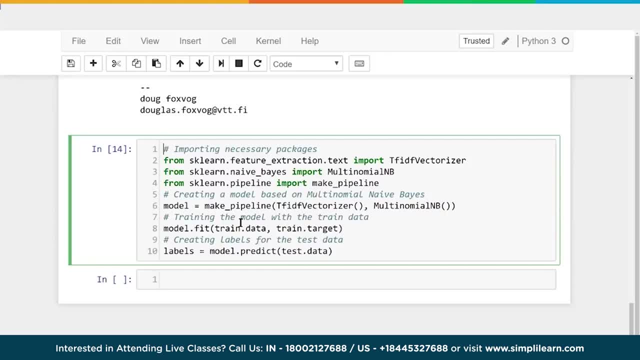 how it works. You can look it up. The notation for the math is usually tfidf And that's just a way of weighing the words, And it weighs the words based on how many times they're used in a document- how many times or how many. 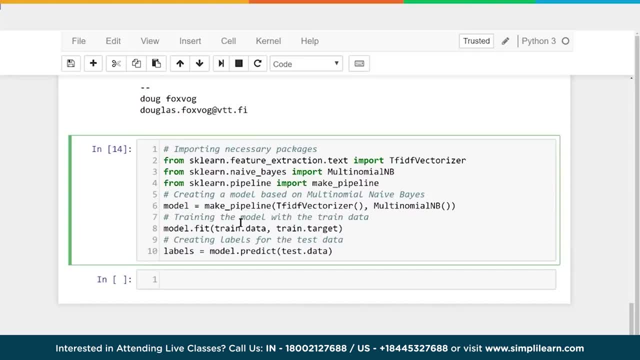 documents they're used in, And it's a well used formula. It's been around for a while. It's a little confusing to put this in here, But let's let it know that it just goes in there and weights the different words in the document. for us That 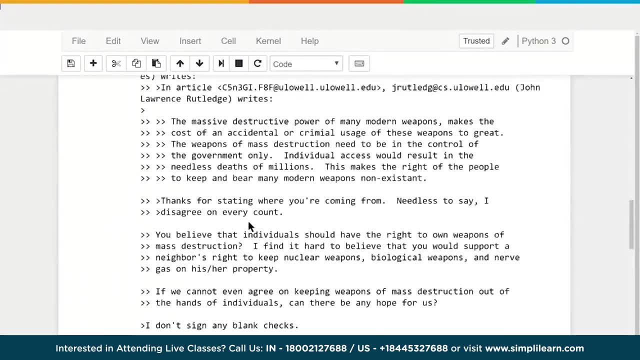 way we don't have to wait. And if you put a weight on it- if you remember I was talking about that up here earlier- If these are all emails, they probably all have the word from in them. From probably has a very low weight. 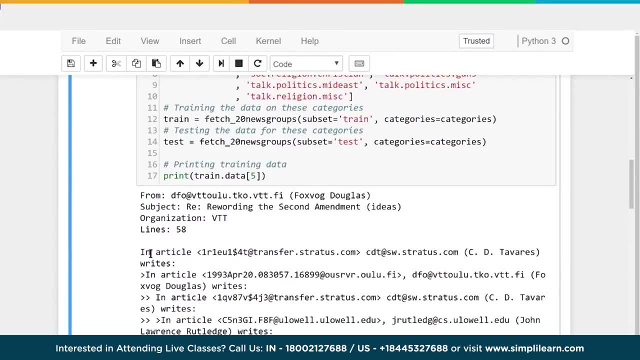 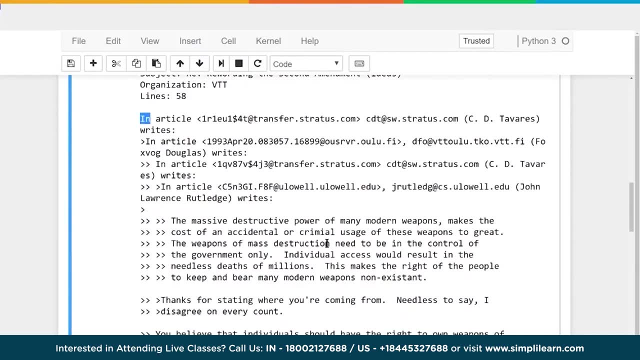 It has very little value in telling you what this document's about. Same with words like in, in article, in articles, in cost of un, maybe, cost, might, or where words like criminal weapons destruction. these might have a heavier weight because they describe a little. 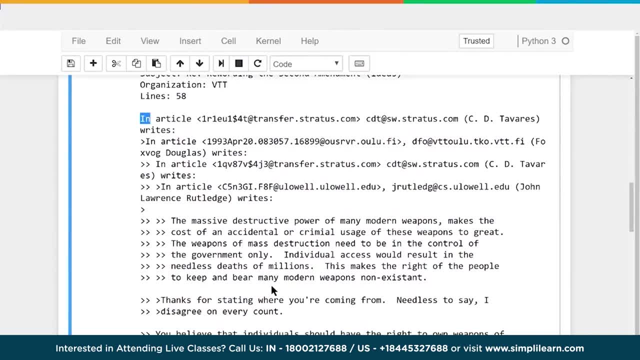 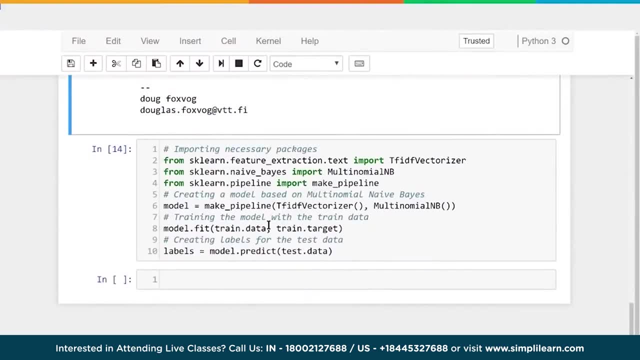 bit more what the article's doing. Well, how do you figure out all those weights in the different articles? That's what this module does, That's what the tfidf vectorizer is going to do for us, And then we're going to import our 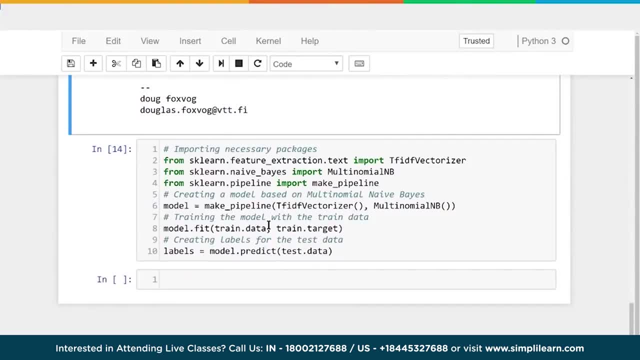 sklearnnaivebase, and that's our multinomial NB, Multinomial naive base. Pretty easy to understand that, where that comes from. And then, finally, we have the sklearn pipeline, import make pipeline. Now, the make pipeline is just a cool piece of code. 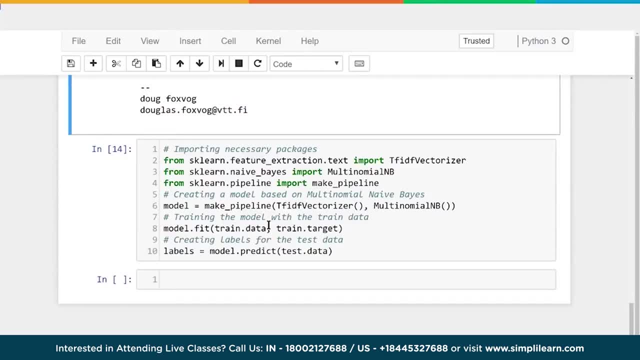 because we're going to take the information we get from the tfidf vectorizer and we're going to pump that into the multinomial NB. So a pipeline is just a way of organizing how things flow. It's used commonly. you probably already guessed what it is, if you've done any. 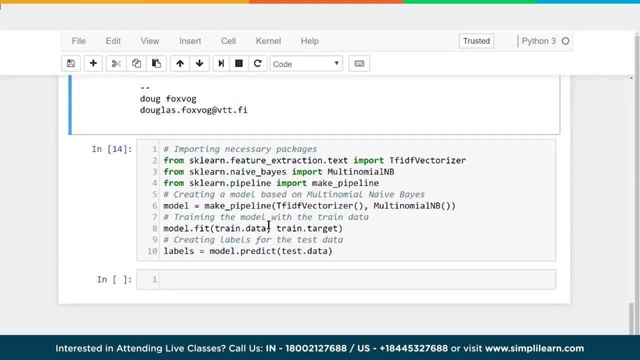 businesses. they talk about the sales pipeline. if you're on a work crew or project manager, you have your pipeline of information that's going through or your projects and what has to be done in what order. That's all this pipeline is. We're going to take the tfid. 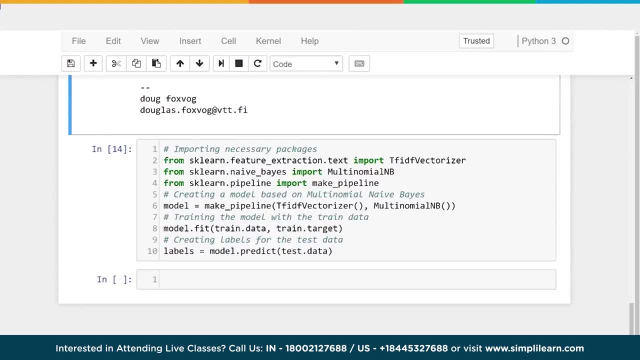 vectorizer and then we're going to push that into the multinomial NB. Now we've designated that as the variable model. We have our pipeline model And we're going to take that model. and this is just so elegant. this is done in just a couple. 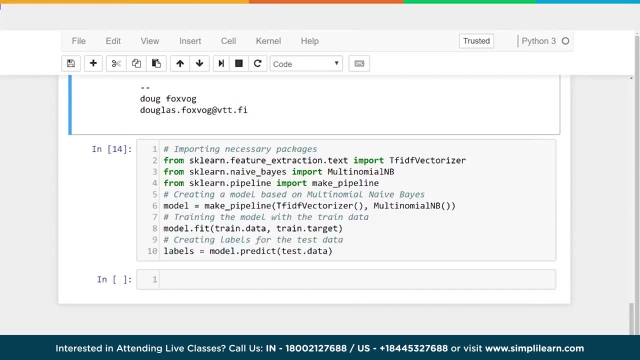 lines of code: Model dot fit And we're going to fit the data, and first the train data and then the train target. Now the train data has the different articles in it. You can see the one we were just looking at And the train dot target is. 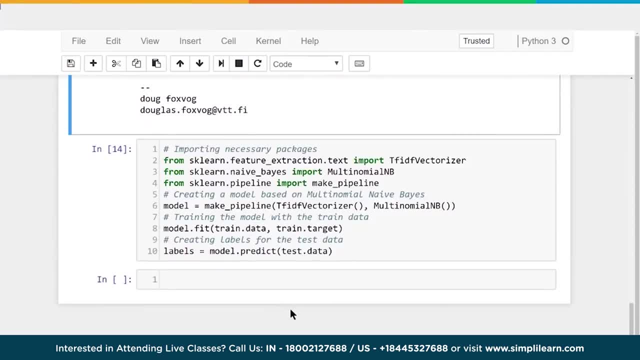 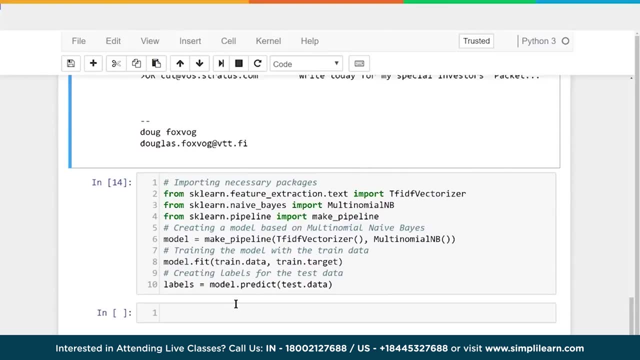 what category they already categorized that particular article as. And what's happening here is the train data is going into the tfid vectorizer. So when you have one of these articles, it goes in there. it weights all the words in there, So there's thousands of words. 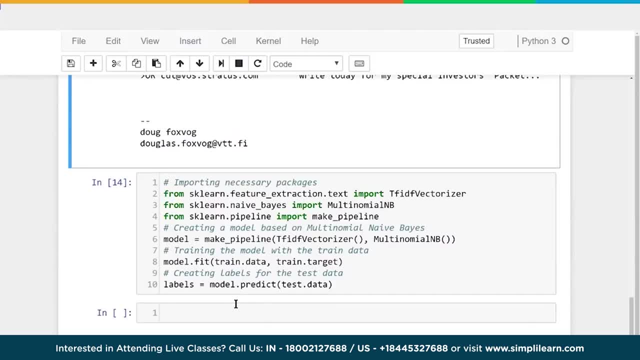 with different weights on them. I remember once running a model on this and I literally had 2.4 million tokens go into this. So when you're dealing with large document bases, you can have a huge number of different words. It then takes those words. 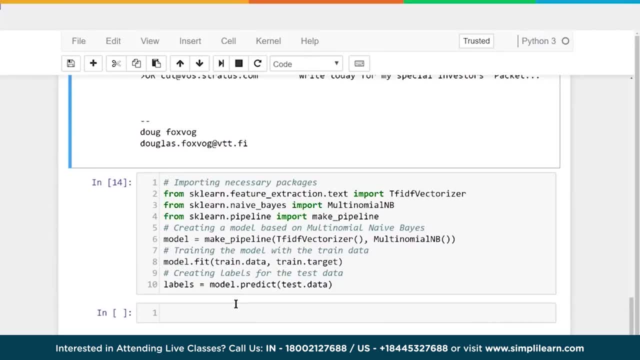 gives them a weight and then, based on that weight, based on the words and the weights, it then puts that into the multinomial NB And once we go into our naive base we want to put the train target in there, So the train data that's been 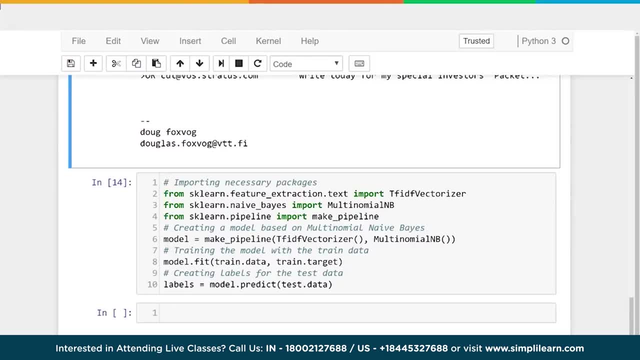 mapped to the tfid vectorizer, is now going through the multinomial NB. and then we're telling it: well, these are the answers. These are the answers to the different documents. So this document that has all these words, with these different weights from the first part, 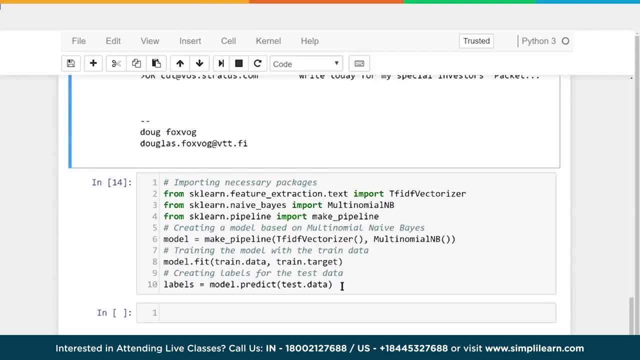 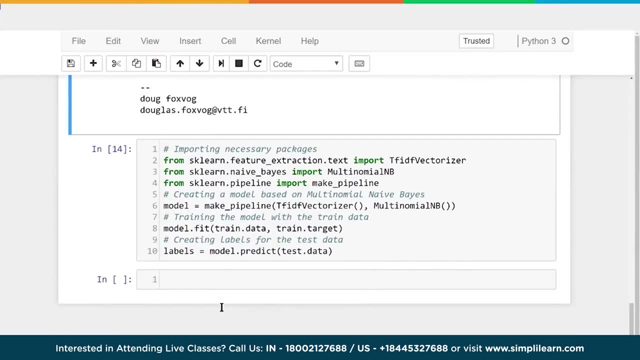 is going to be, whatever category it comes out of- Maybe it's the talk show or the article on religion- miscellaneous. Once we fit that model, we can then take labels and we're going to set that equal to modelpredict. Most of the sklearn use the term. 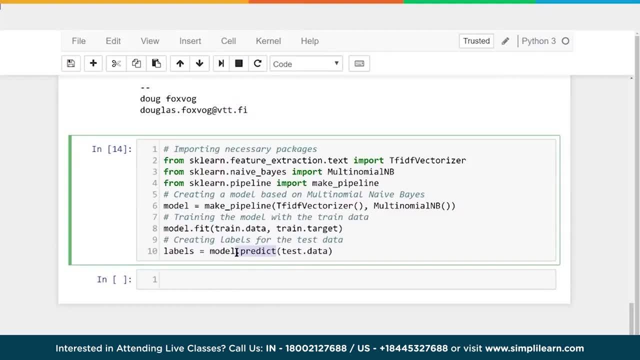 predict, to let us know that we've now trained the model and now we want to get some answers And we're going to put our test data in there, because our test data is the stuff we held off to the side. We didn't train it on there and we don't know what's. 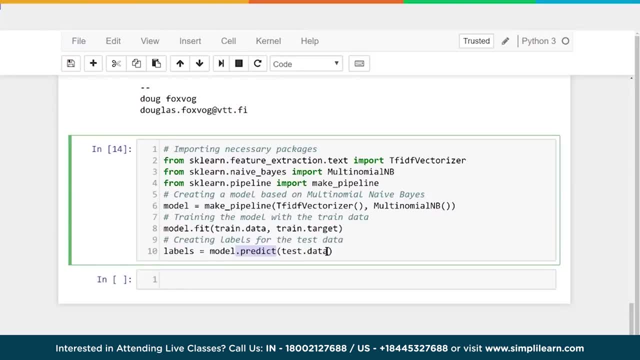 going to come up out of it and we just want to find out how good our labels are. Do they match what they should be? Now, I've already run this through. There's no actual output to it to show. This is just setting it. 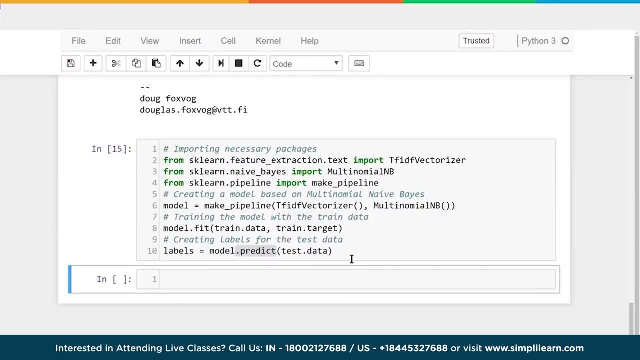 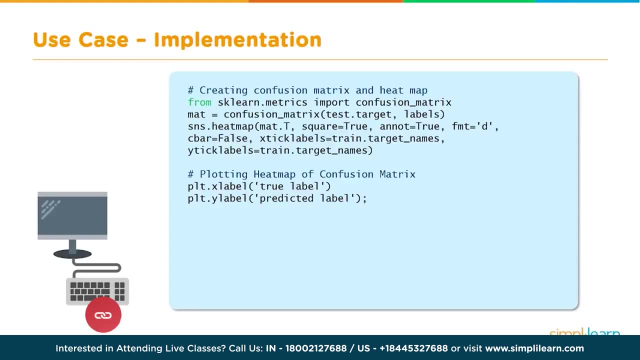 all up. This is just training our model, creating the labels so we can see how good it is, and then we move on to the next step, to find out what happened To do this. we're going to go ahead and create a confusion matrix and a heat. 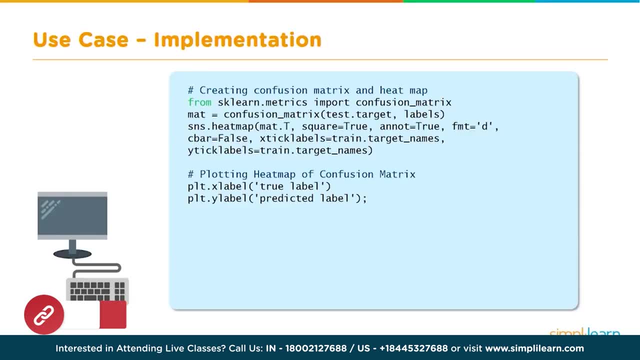 map. So the confusion matrix, which is confusing just by its very name, is basically going to ask: how confused is our answer? Did it get it correct or did it miss some things in there or have some missed labels? And then we're going to put that on a heat map. 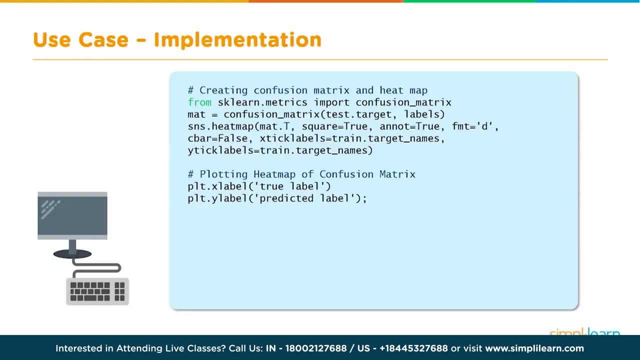 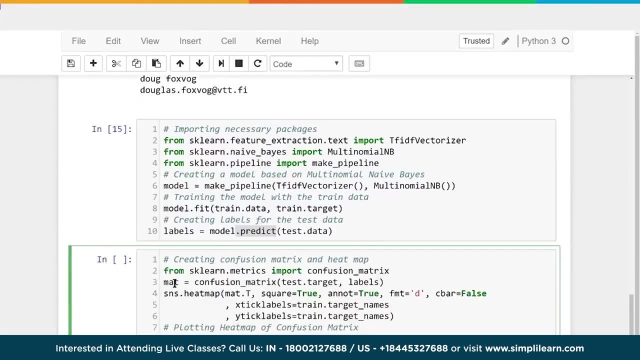 so we'll have some nice colors to look at to see how that plots out. Let's go ahead and take this code and see how that, take a walk through it and see what that looks like. So back to our Jupyter notebook. I'm going to put the code in there. 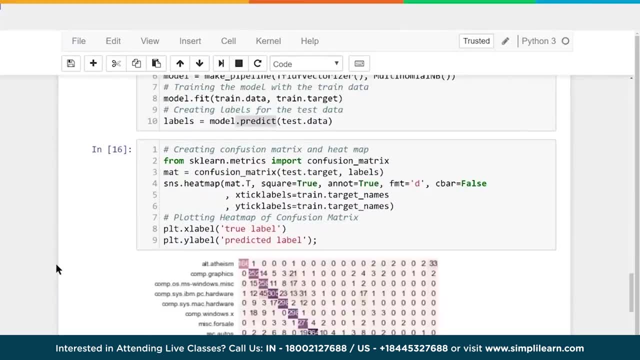 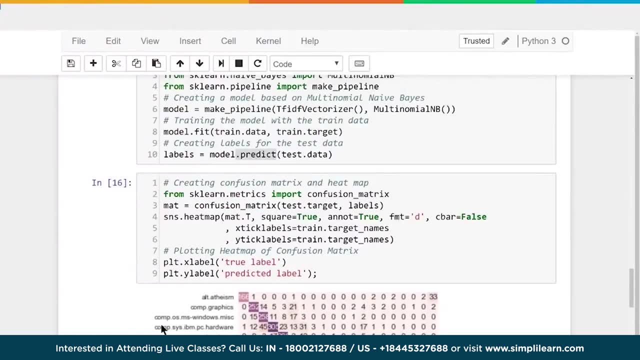 and let's go ahead and run that code. Take it just a moment and remember we had the end line. that way my graph shows up on the end line here And let's walk through the code and then we'll look at this and see what that means. 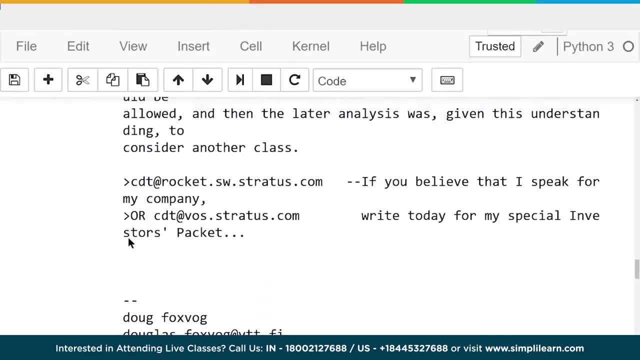 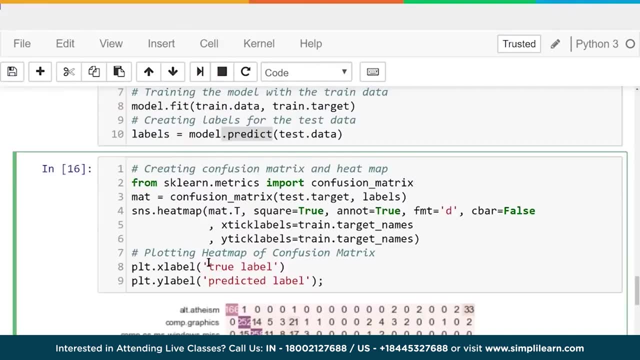 So let me make it a little bit bigger. there we go, No reason not to use the whole screen Too big. So we have here from sklearnmetrics import confusion matrix And that's just going to generate a set of data that says the prediction was such. 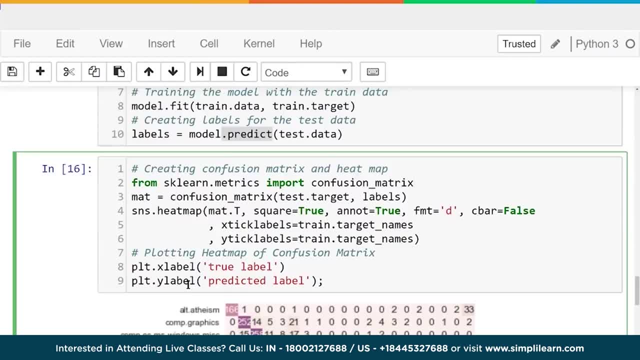 the actual truth was either agreed with it or it was something different. And it's going to add up those numbers so we can take a look and just see how well it worked. And we're going to set a variable mat equal to confusion matrix and we have our test target. 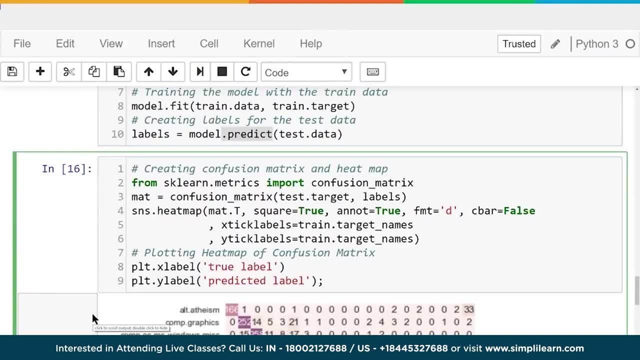 our test data. that was not part of the training- very important- in data science. we always keep our test data separate, otherwise it's not a valid model if we can't properly test it with new data. And this is the labels we created from that test data. 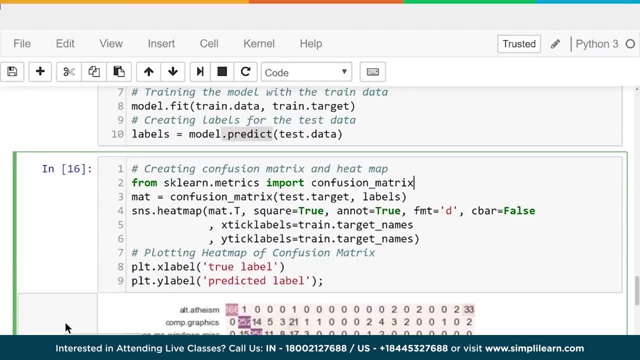 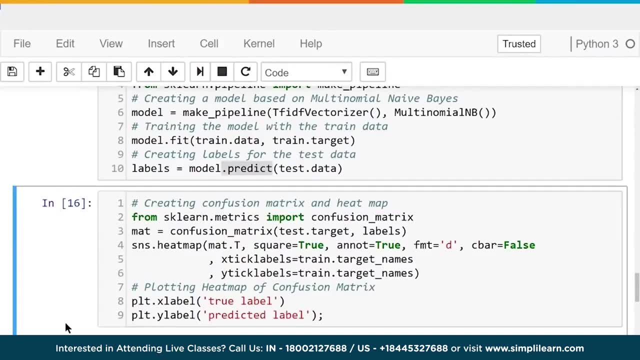 these are the ones that we predict it's going to be. So we go in and we create our snHeatmap. the sns is our seaborn, which sits on top of the piplot. So we create a snsheatmap, we take our confusion matrix and it's going to be matt. 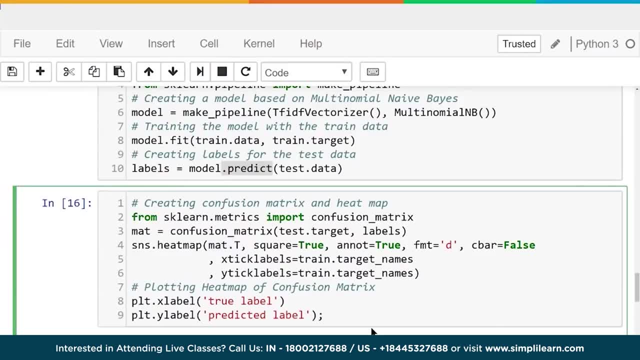 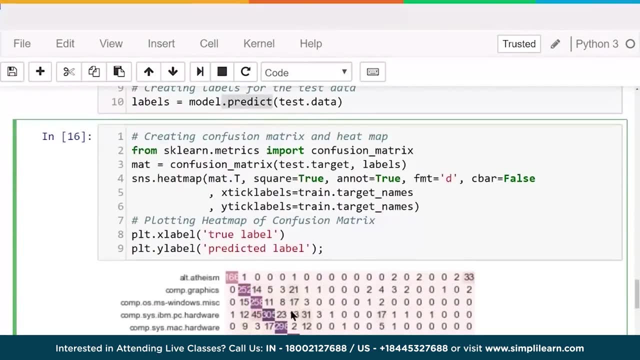 and do we have other variables that go into the snsheatmap? we're not going to go into detail what all the variables mean. the annotation equals true. that's what tells it to put the numbers here. so you have the 166, the 1, the 0001. 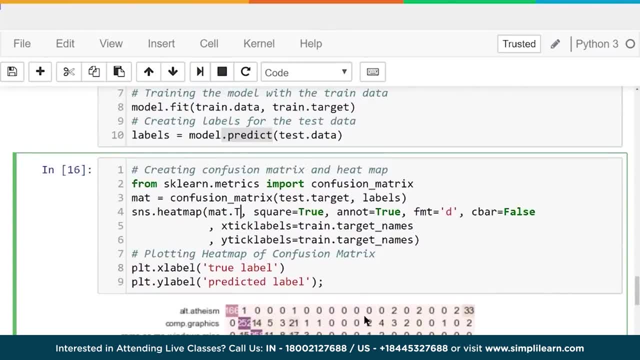 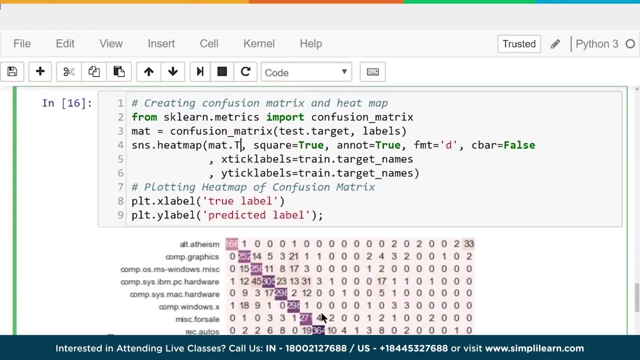 format d and cbar equals false- have to do with the format. if you take those out, you'll see that some things disappear. and then the xtick labels and the ytick labels- those are our target names and you can see right here. that's the alt atheism. 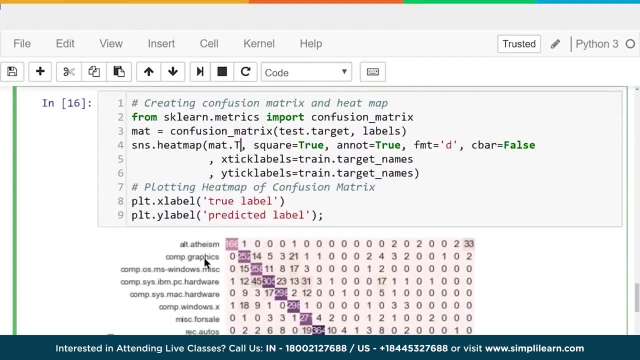 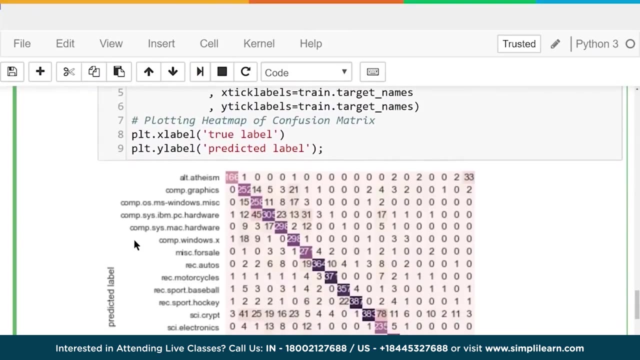 comp, graphics, comp, osms, windows, miscellaneous. And then, finally, we have our pltxlabel. remember the sns or the seaborn sits on top of our matplot library, our plt. and so we want to just tell it: xlabel equals a true is true, the labels are true. and then the 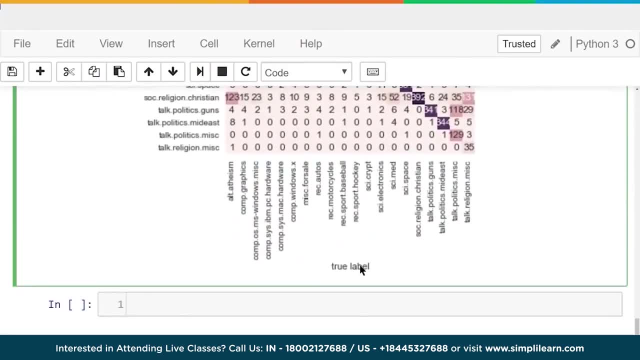 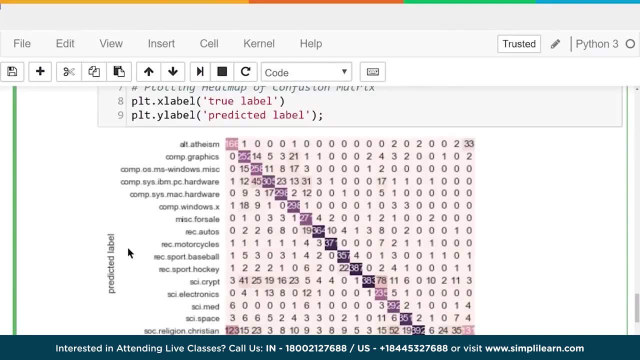 ylabel is prediction label. so when we say a true, this is what it actually is and the prediction is what we predicted. and let's look at this graph, because that's probably a little confusing the way we rattled through it, and what I'm going to do is I'm going to go ahead and flip back. 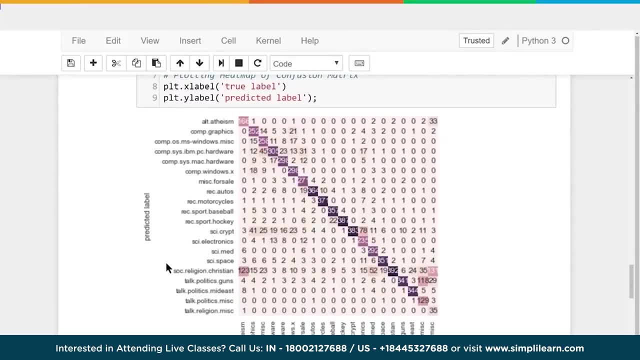 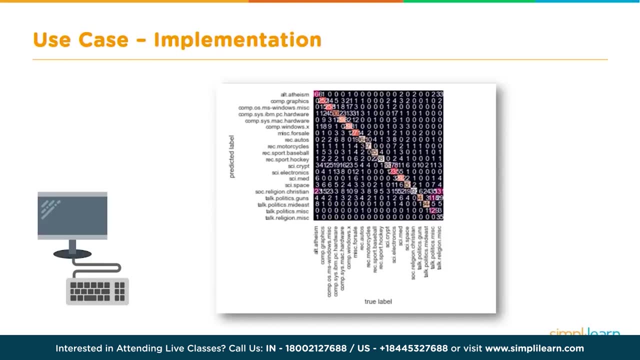 to the slides because they have a black background they put in there. that helps it shine a little bit better so you can see the graph a little bit easier. so in reading this graph, what we want to look at is how the color scheme has come out, and you'll see a line. 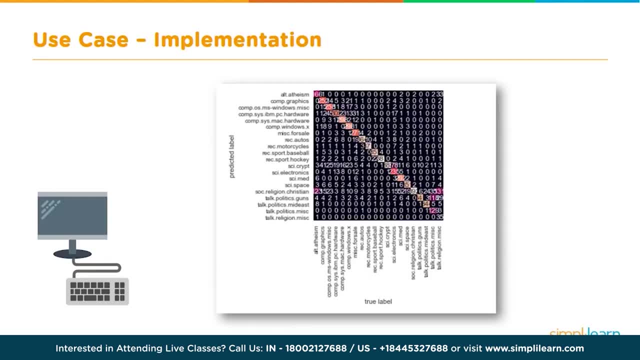 right down the middle, diagonally from upper left to bottom right. what that is is, if you look at the labels, we have our predicted label on the left and our true label on the right. those are the numbers where the prediction and the true come together, and this is what we want to see. is we want to see? 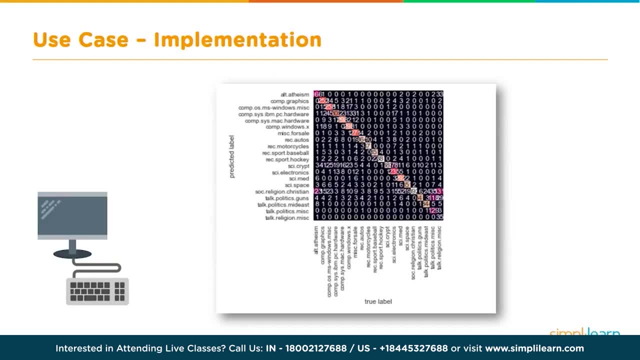 those lit up. that's what that heat map does, as you can see that it did a good job of finding those data and you'll notice that there's a couple of red spots on there where it missed. it's a little confused when we talk about talk religion, miscellaneous versus 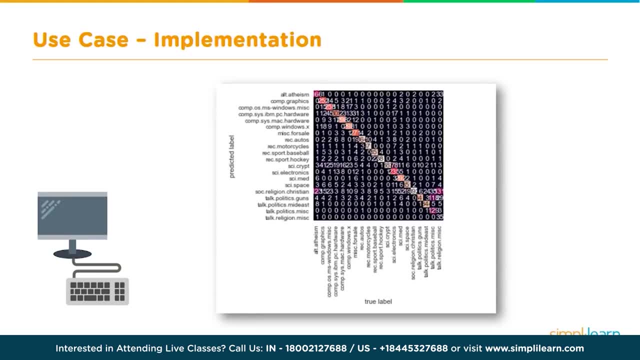 talk, politics, miscellaneous social religion, Christian versus alt atheism. it mislabeled some of those and those are very similar topics, so you can understand why it might mislabel them, but overall it did a pretty good job. if we're going to create these models, we want to go ahead and be able to 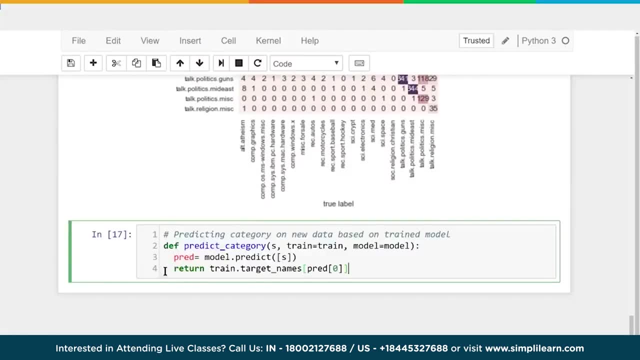 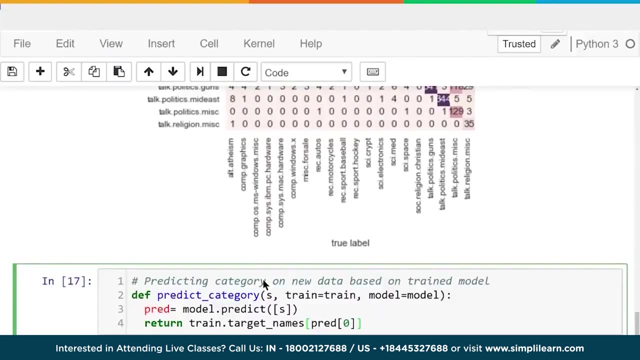 use them. so let's see what that looks like. to do this, let's go ahead and create a definition, a function to run, and we're going to call this function. let me just expand that just a notch here. there we go. I like mine in big letters: predict categories: we 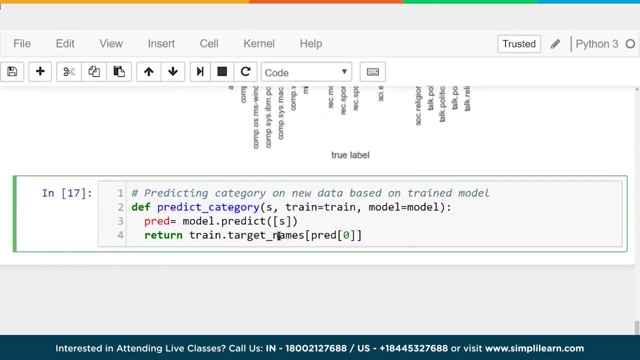 want to predict the category, we're going to send it s a string and then we're sending it train equals train. we have our training model and then we had our pipeline model equals model. this way we don't have to resend these variables each time. the definition knows that, because I said train. 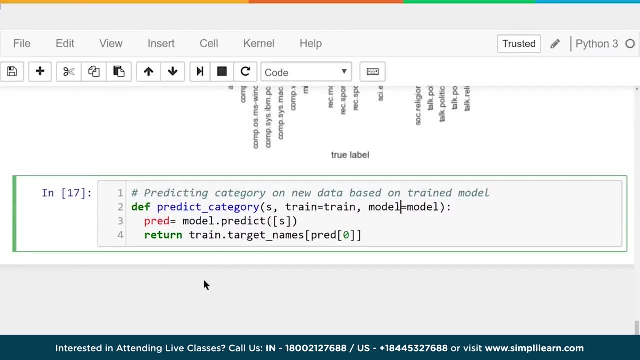 equals train and I put the equal for model and then we're going to set the prediction equal to the model dot predict s. so it's going to send whatever string we send to it. it's going to push that string through the pipeline, the model pipeline it's going to go through. 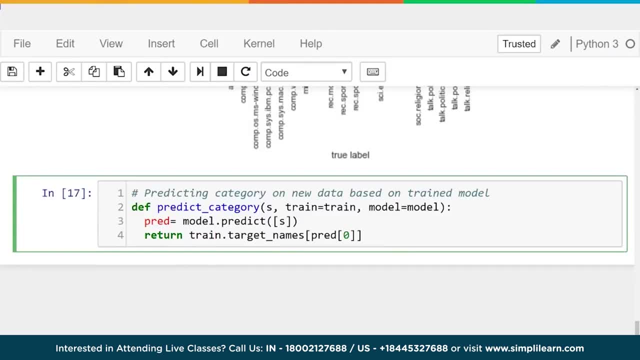 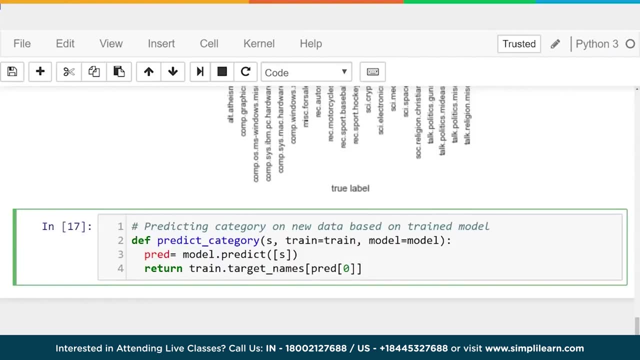 and tokenize it and put it through the tf, idf, convert that into numbers and weights for all the different documents and words, and then it'll put that through our naive bays and from it we'll go ahead and get our prediction we're going to predict. 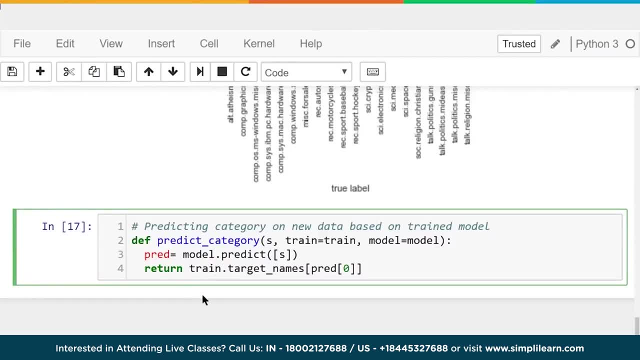 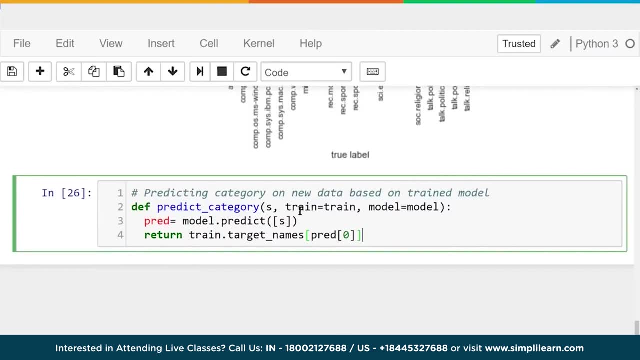 what value it is. and so we're going to return train dot target names- predict of zero, and remember that the train dot target names, that's just categories. I could have just as easily put categories in there- dot, predict of zero. so we're taking the prediction, which is a number, and we're converting. 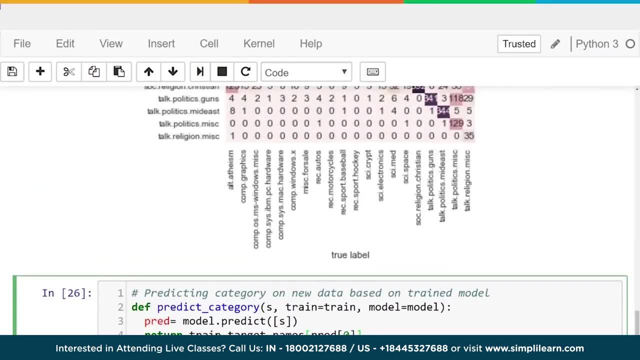 it to an actual category we're converting it from. I don't know what the actual numbers are, but let's say zero equals alt atheism. so we're going to convert that zero to the word or one. maybe it equals comp graphics. so we're going to convert number one into comp graphics. 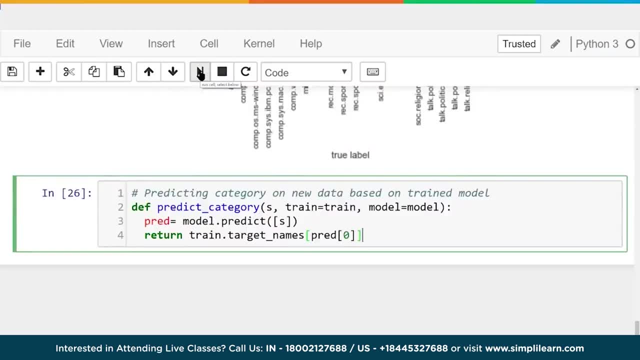 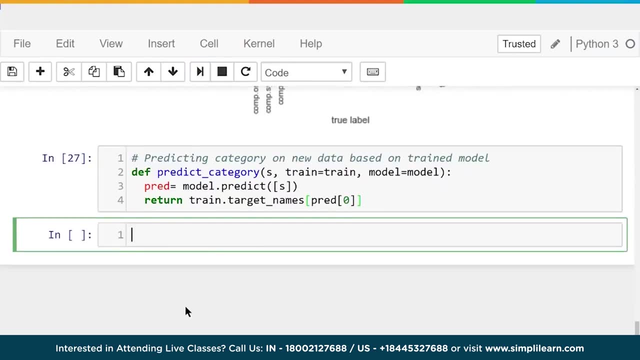 that's all that is. and then we got to go ahead and then we need to go ahead and run this, so I load that up and then, once I run that, we can start doing some predictions. let me go ahead and type in predict category and let's just do predict category. 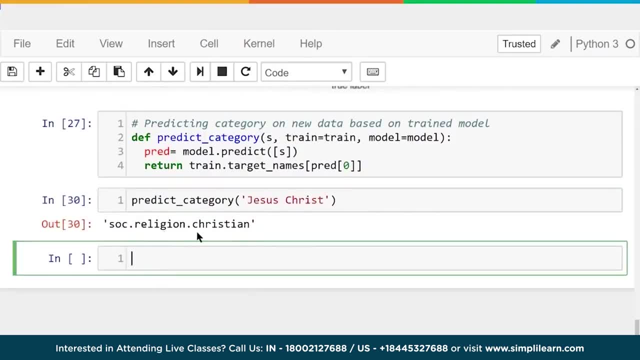 Jesus Christ and it comes back and says it's social religion Christian. that's pretty good. now note: I didn't put print on this. one of the nice things about the Jupiter notebook editor and a lot of inline editors is, if you just put the name of the variable out, it's returning. 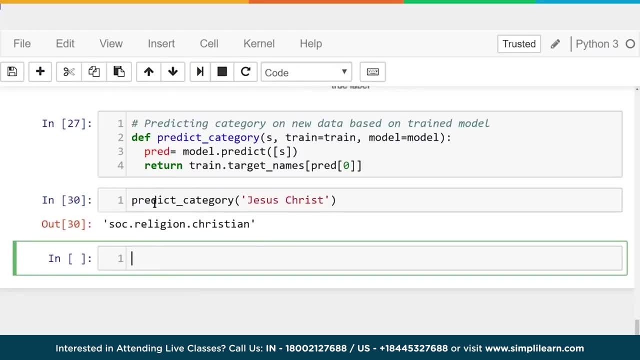 the variable train dot target underscore names, it'll automatically print that for you in your own ID. you might have to put in print. let's see where else we can take this. and maybe you're a space science buff. so how about sending load to international space station? 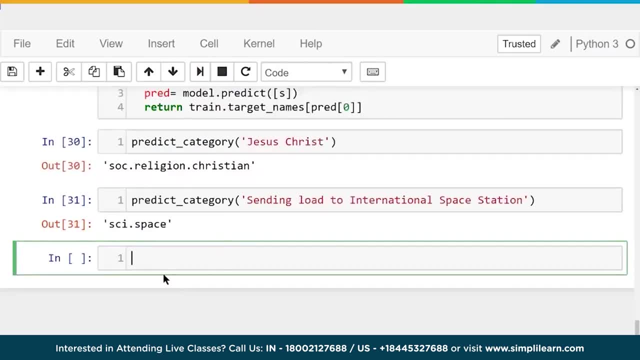 and if we run that, we get science, space. or maybe you're a automobile buff and let's do. they were going to tell me: Audi is better than BMW, but I'm going to do, BMW is better than an Audi. so maybe you're a car buff and we run that. 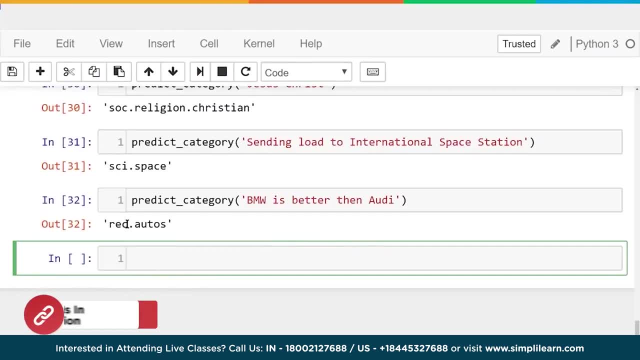 and you'll see it says recreational. I'm assuming that's what REC stands for autos. so I did a pretty good job labeling that one. how about if we have something like a caption running through there, president of India, and if we run that it comes up and says talk.